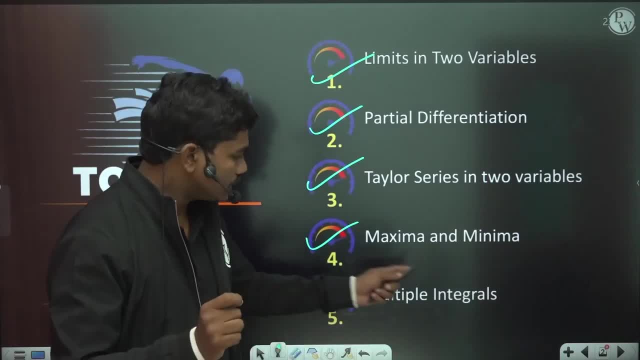 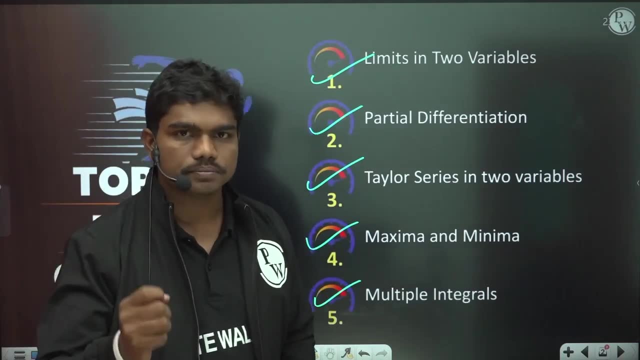 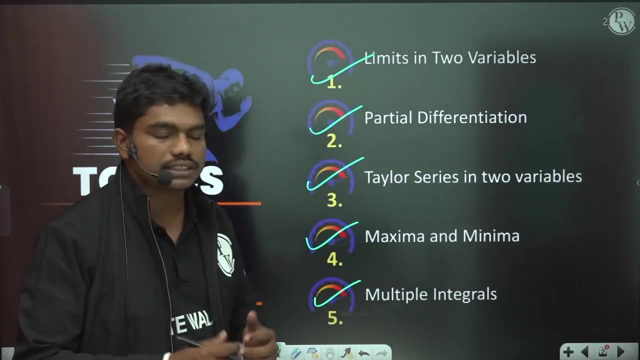 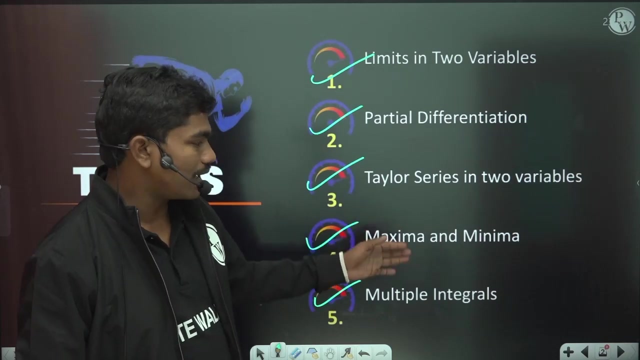 on the basic single variable lectures. so, if you see this multiple integrals is very much connected to those graphs and some slight preliminary idea. this multiple integrals is one very important and very easy topic in engineering mathematics. okay, So that's how we are going to cover in this module, basically So basic multi variable calculus, limits, partial differentiation, then Taylor series into variables, maxima and minima, and also multiple integrals. okay, Now coming to the point of 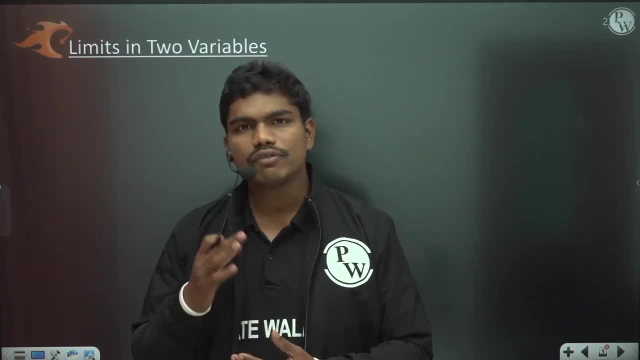 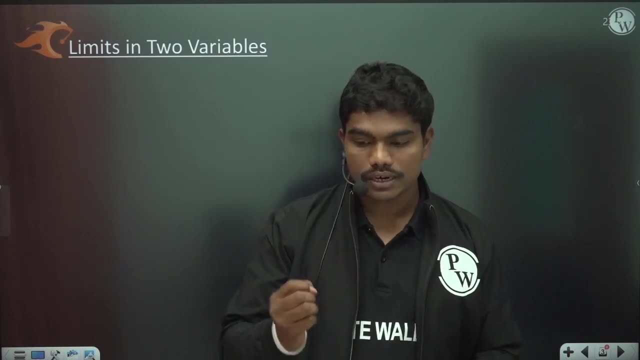 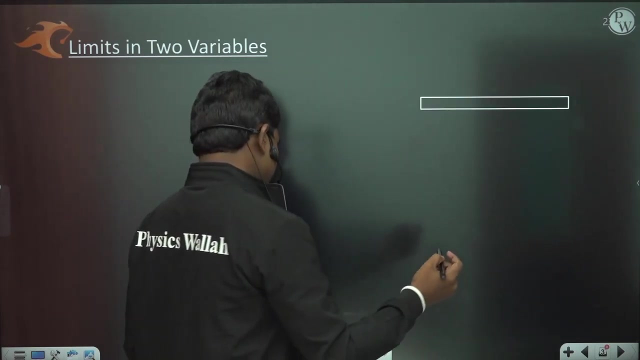 directly before going to limits. okay, we'll talk about limits, But straight away, before going to the limits, why we need to talk about multi variable functions. I want to give you some idea because my intention is to tell you that why functions don't depend on a single variable generally, why there is some necessity of multi variable functions. I'll explain you with a simple example. So you see, let us suppose. let us suppose I have a block. for example, I have a some bar. let us say, okay, this is some bar. Now what I'm doing? I have two. 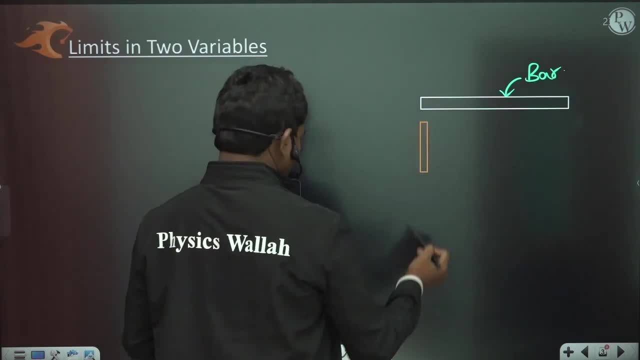 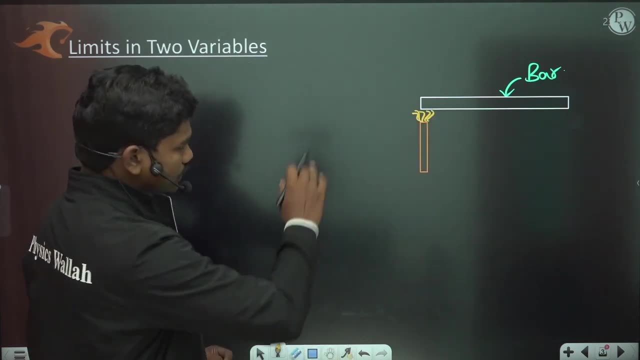 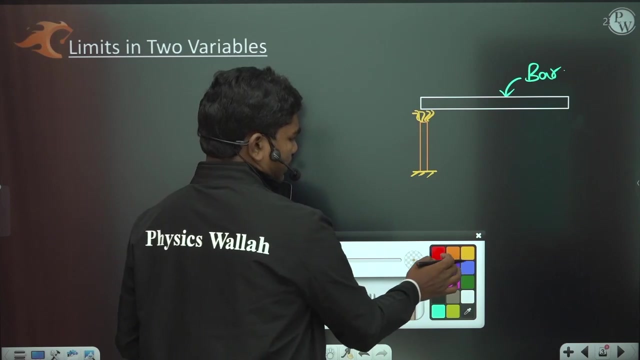 taken some small lighter kind of thing. And let us suppose I have started this heating. okay, So I have started this heating of this bar. Now tell me one thing: if this bar is the case, there is some length L. Now tell me one thing: if I start heating, it's a common example. what I'm telling you, you all can understand with some school level physics, okay, Sixth, seventh class physics okay. So now, as soon as I start heating, as soon as I start heating, then what happens if I take temperature at two different locations? 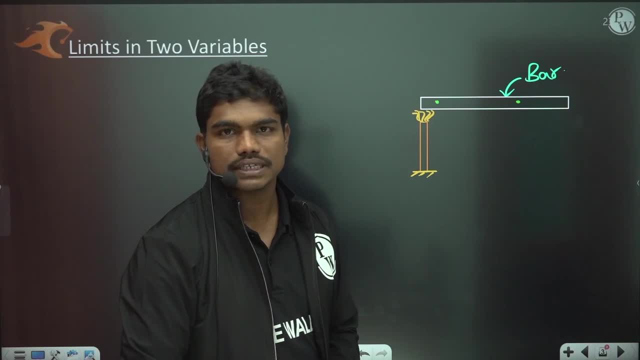 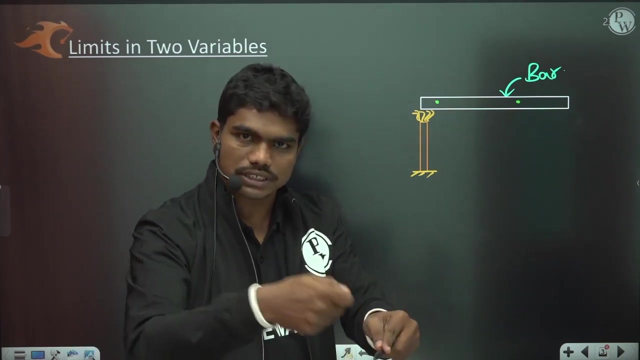 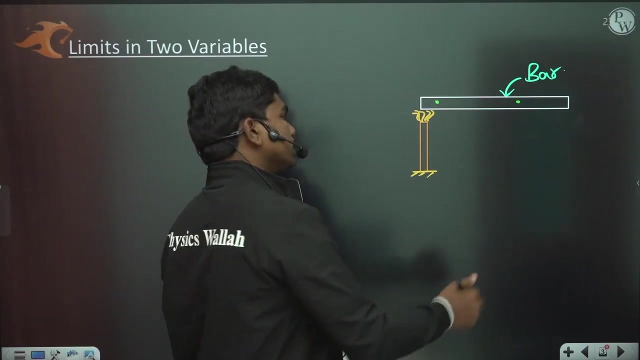 will the temperature be same at these two locations? No, it won't be same, okay, Because it takes some time for the heat to transfer from one point to another point. So definitely, which many of you might have seen, normally when your mom is cooking something with the pan stick or something, the other end of the pan stick will be very much hot because it's in contact with the pan, but the other end you can handle comfortably because it's not in. you know, it takes some time to get heated. So now, if you see this, if these two points, if I define this as oizen, if I define 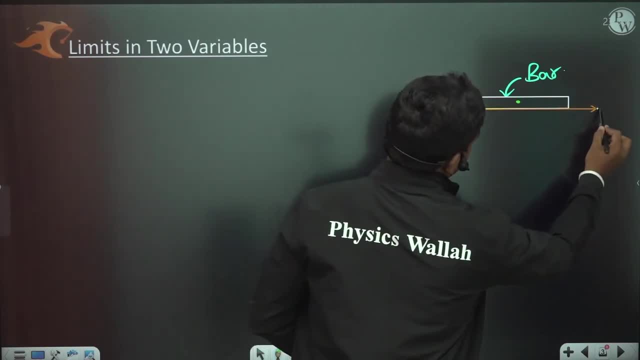 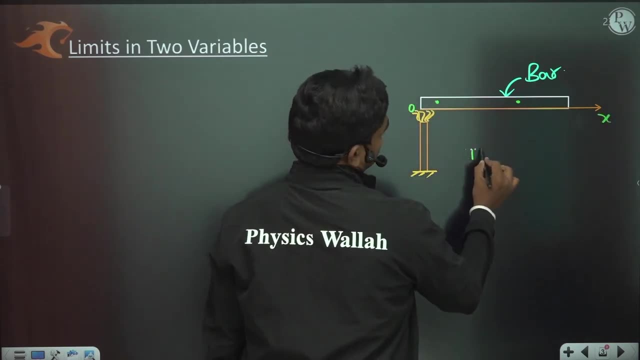 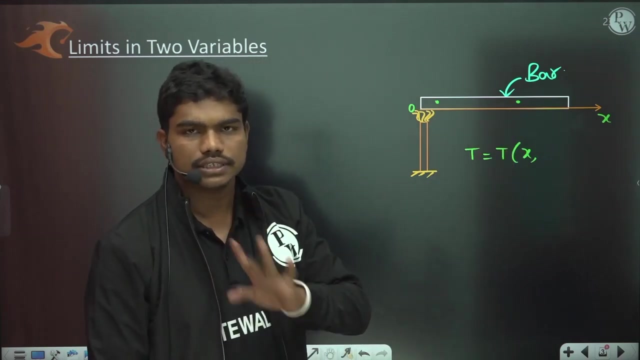 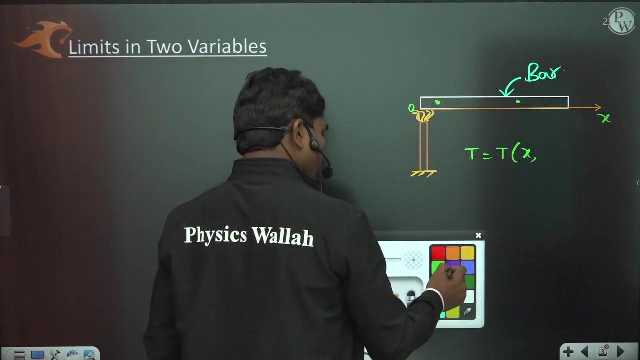 this as oizen and if I take this as x-axis, for example, if I take this as my x-axis and if this is oizen, then you know one thing: this temperature T is depending on this coordinate x, correct? Because as x changes, this temperature changes. This is first point. Now, let us suppose at the same point means: let us suppose, if I take a point here now at the same point A, let us call this point A at the same point. if I measure, 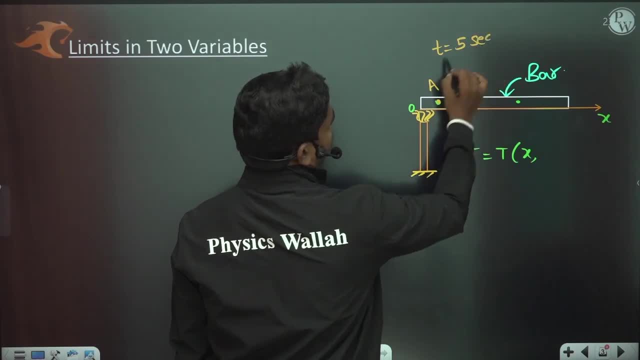 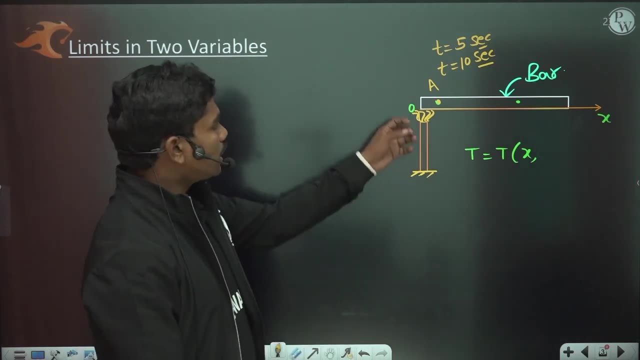 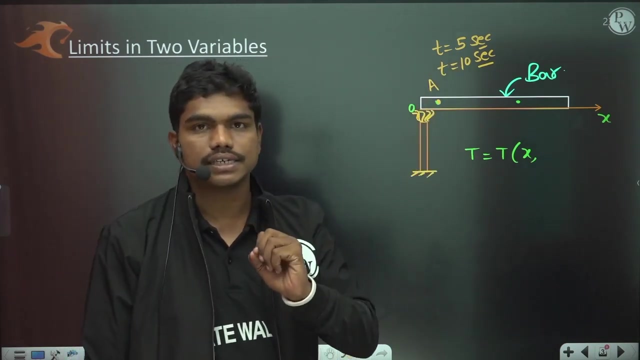 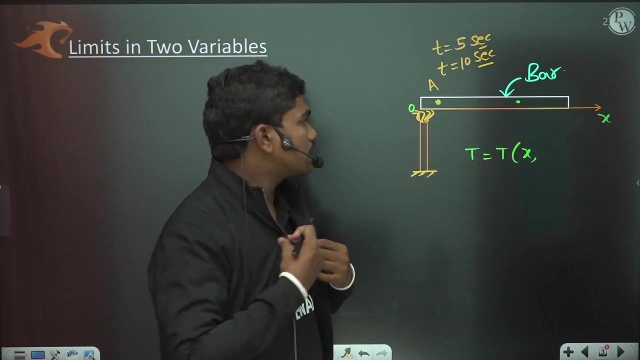 temperature after five seconds of heating and after 10 seconds of heating, for example. let us say I've heated this, I've started heating this block at room temperature. Now I've measured the temperature at the same point A at two different times. what is that? at five seconds and at 10 seconds. then obviously you know the temperature recorded at these two times is different, right? Because obviously, as time increases, the amount of heat supplied to this bar actually increases And obviously the temperature at this location will increase. So 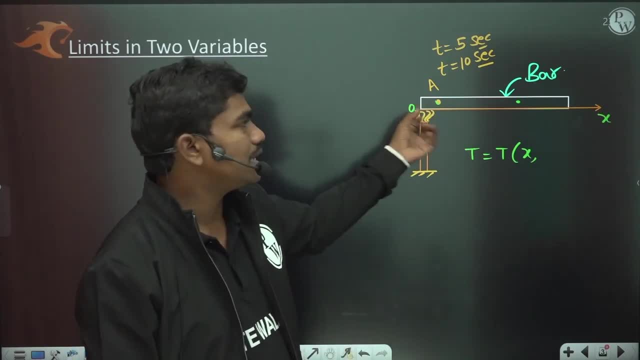 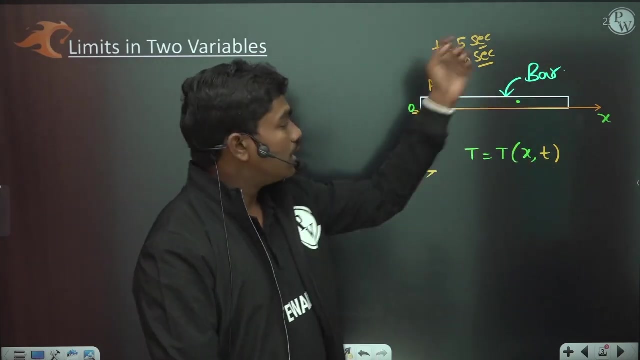 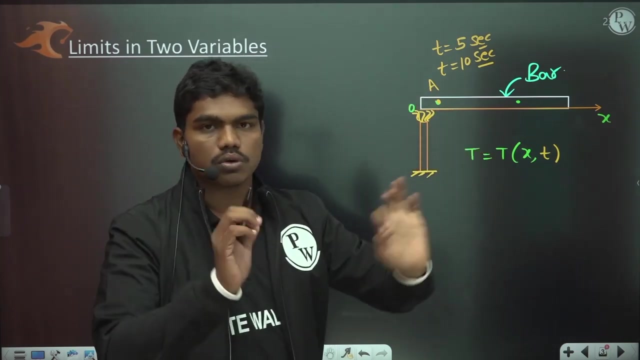 So means, if you talk about the unsteady state, means basically if in the initial stage of heating what happens, your temperature will be a function of both space and time. right, And of course there could be many other factors, But right now, in simple intuition, you can say temperature depends upon x as well, as time means at a given point the temperature can change with respect to time, or at a given time the temperature can change with respect to the coordinates of the point. So if you see this temperature is depending on two variables. okay, so it's a multivariable function. 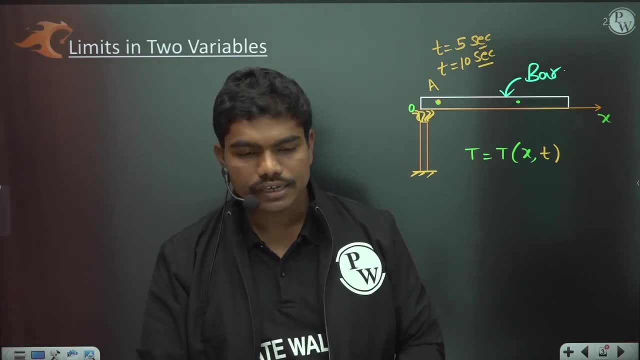 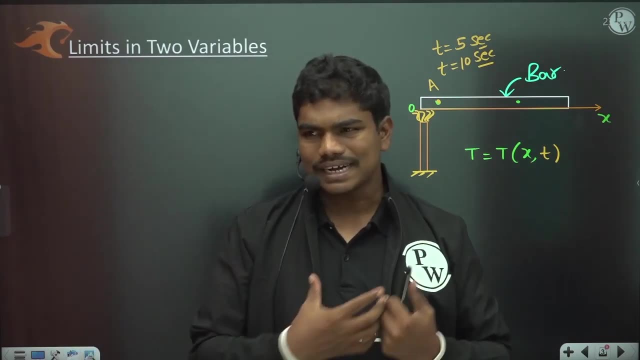 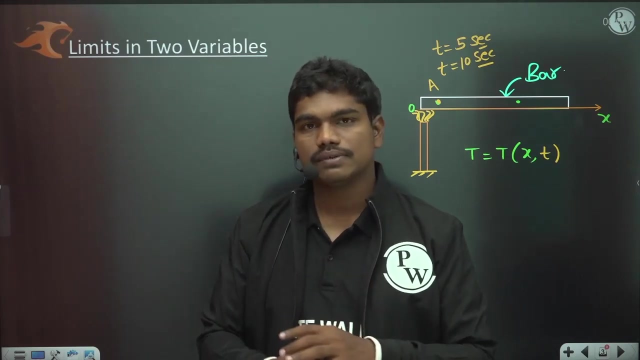 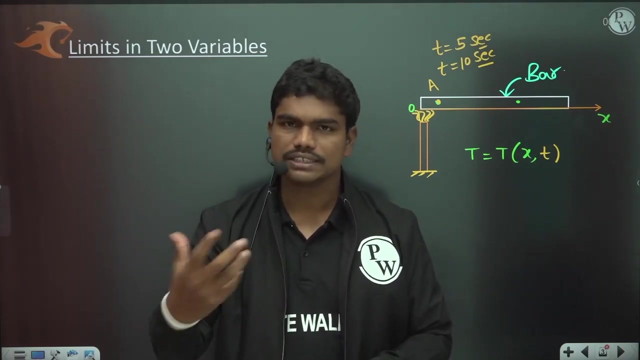 Basically. so that's how functions need not be always of single variable clear. If I want to identify t, I need to know two independent quantities, x and t. Okay, so this, practically this kind of examples we deal, you know, very much in day to day life. So that's why, if you see, talking about this multivariable functions is important. you take pressure, you take electric field intensity or you take anything generally they will change with us, but they can change with respect to time, location and all these things. Okay, so that's why we'll talk about this multivariable function. 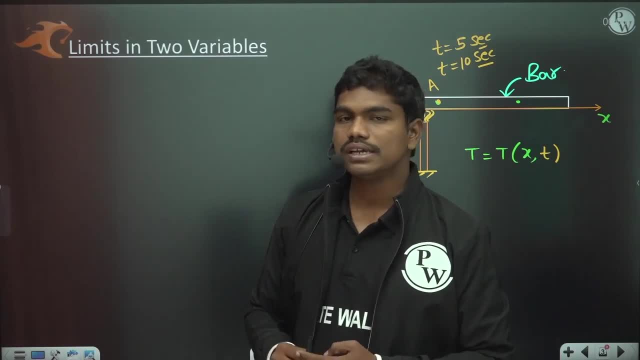 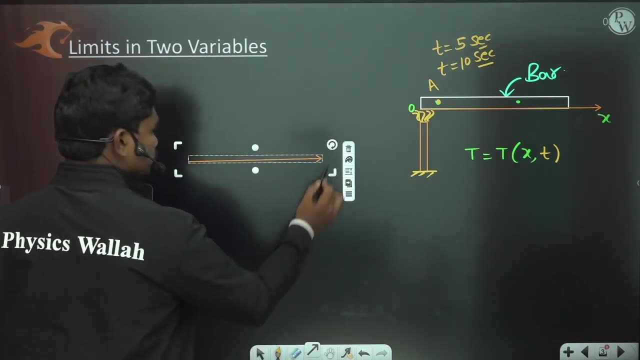 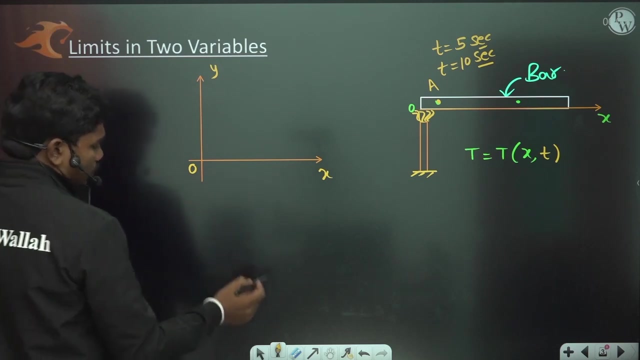 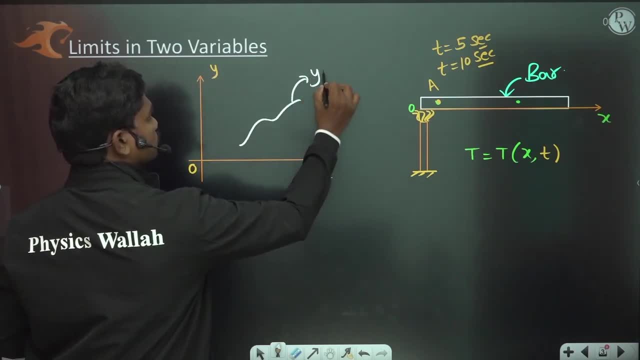 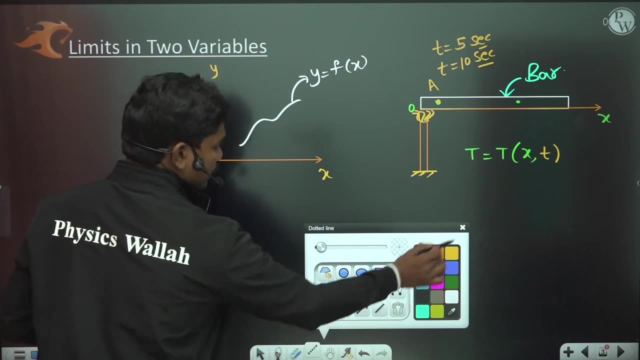 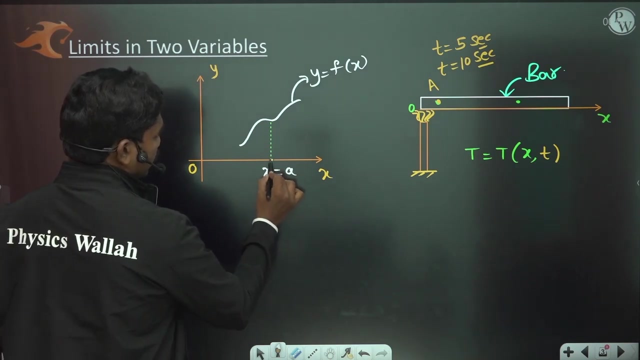 this is your function: y is equal to f of x, for example. Okay, y is equal to f of x. then what I have told you is: if you take a point, x is equal to a. if you take a point x is equal to a here, somewhere here, then let us suppose: if this value is l, if this value is l, then I told you you will write limit: x tends to a. f of x is equal to l. 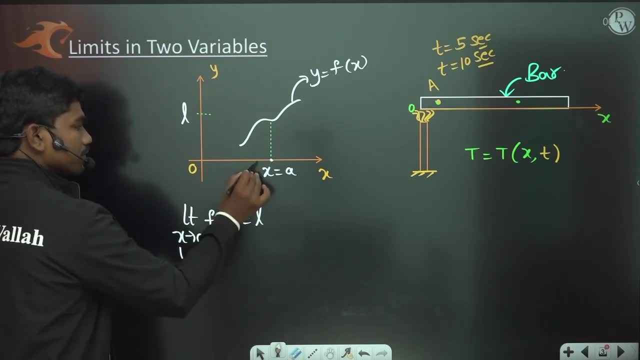 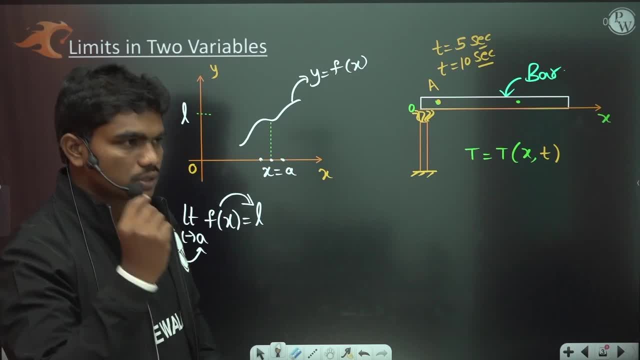 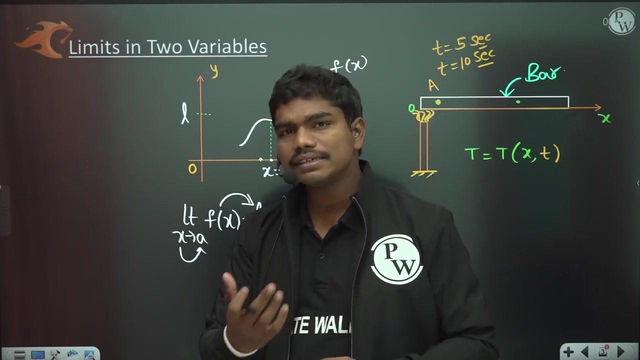 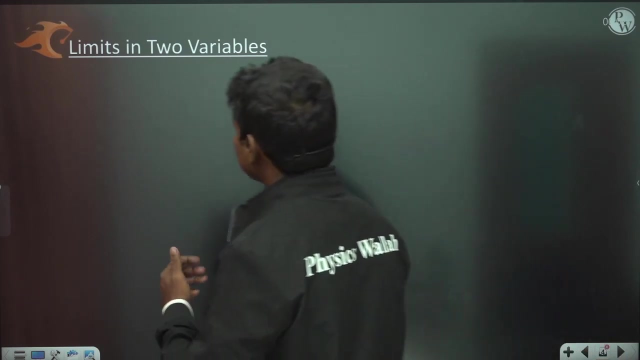 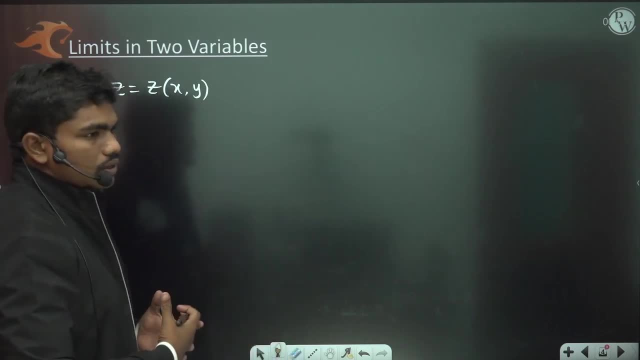 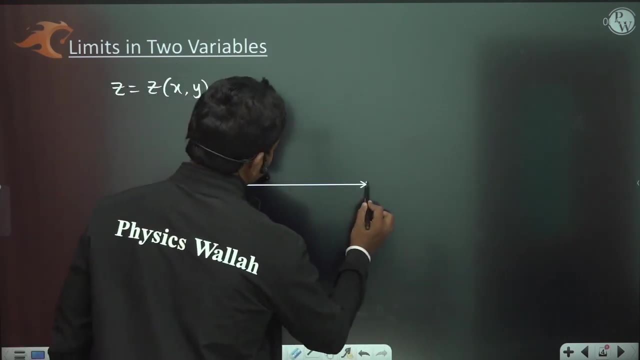 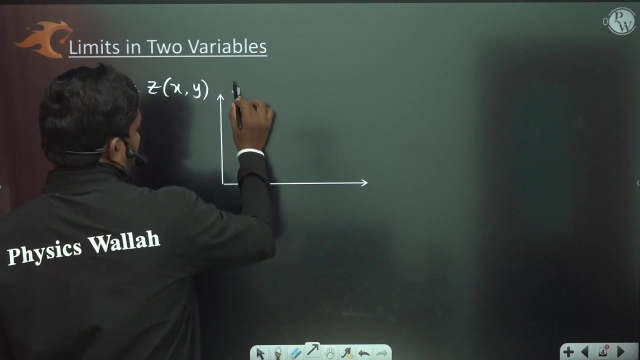 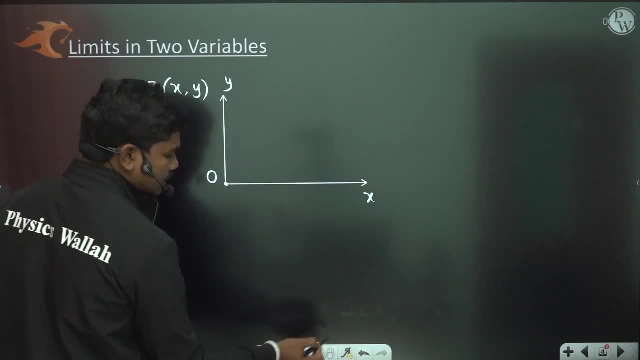 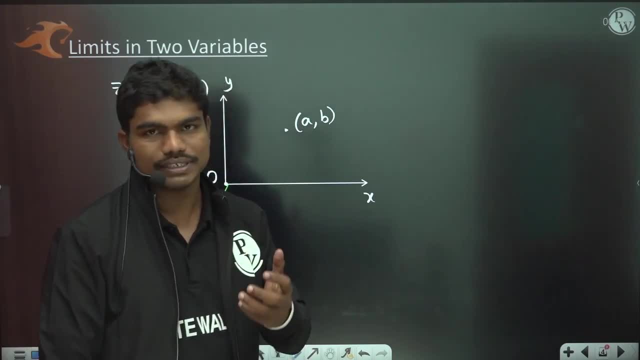 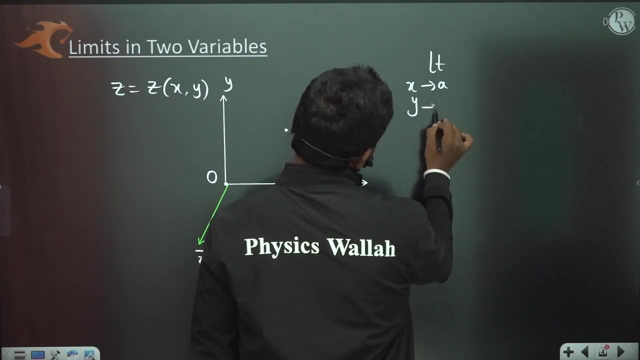 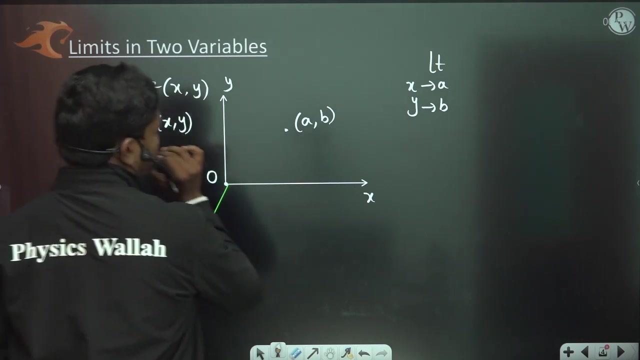 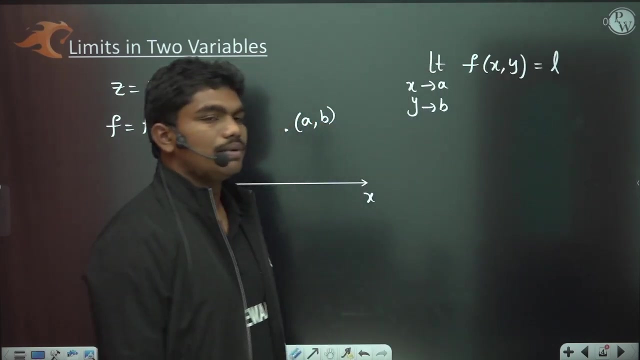 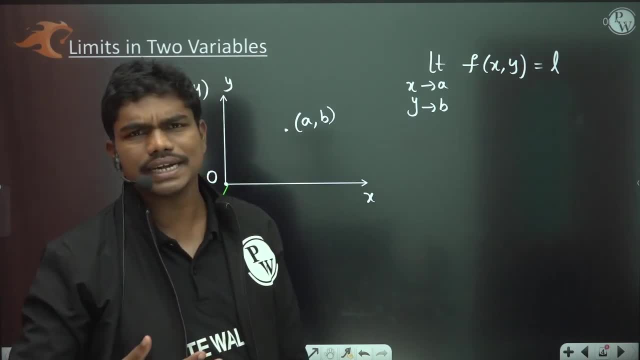 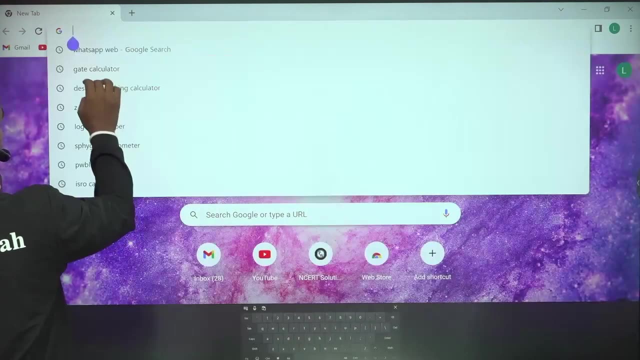 If you plot a point, for example, if you take z is equal to x square plus y square, something like that you can get. I will show you with the help of Desmos, because we have the graphing calculator, so you can see: z is equal to- let us take some simple function- x square. 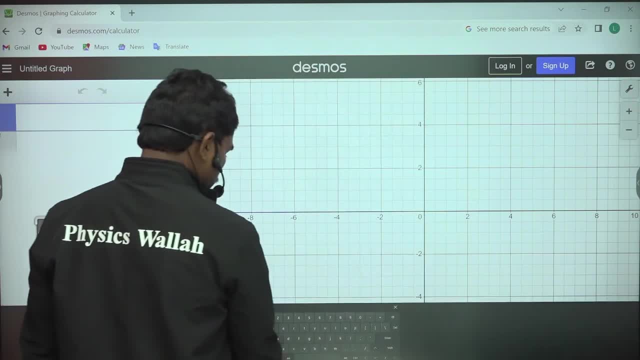 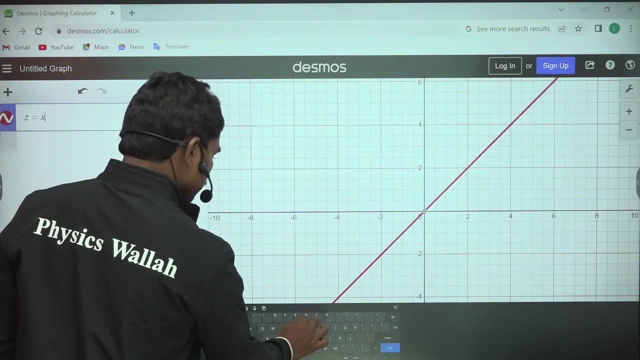 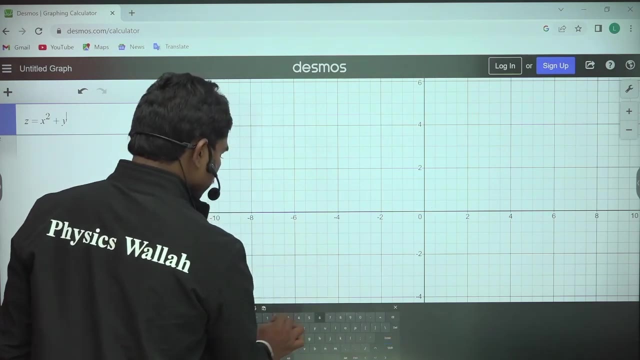 plus y square, for example, Because I want to show you anyhow drawing them is difficult, but using the techniques, I can show you x square plus y square. So let us suppose you have drawn this function. This is in 3D. actually I have taken only 2D plot, I think. 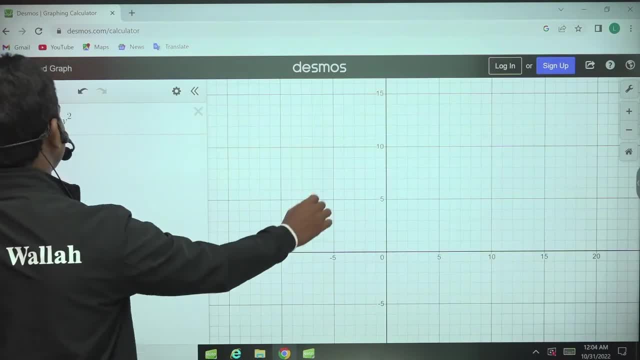 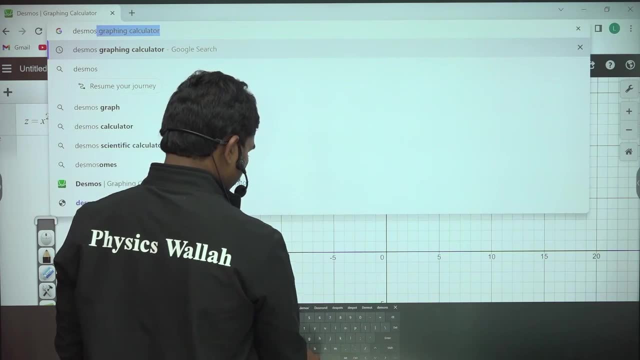 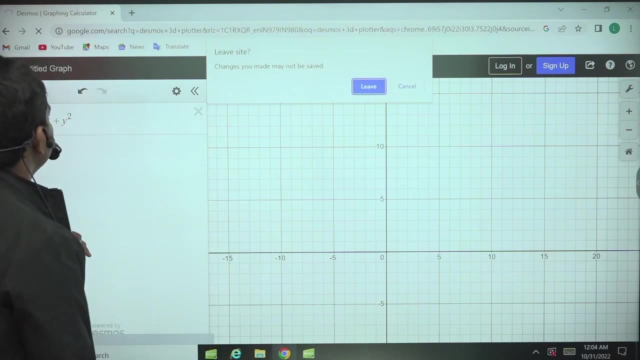 So that's why, you can see, you cannot find any graph here because it's a 2D plot. So we need to go for 3D plotter. in that case, 3D plotter. Okay, so we will open the 3D plotter and then I will show you. of course, 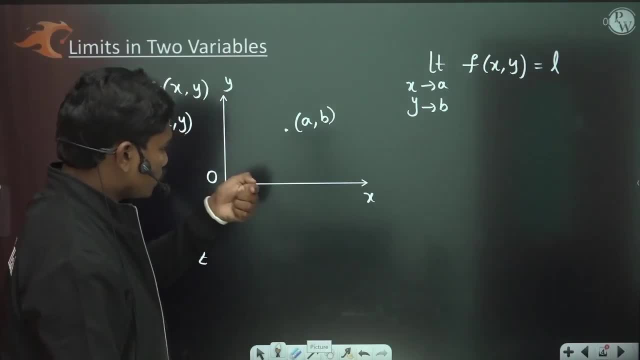 But right now I hope you understand, whenever you are plotting z on the other coordinate, you cannot see the function in this x-y plane. basically, okay, So how this function is same. Now tell me one thing: in single variable calculus, to which this point A, we have only. 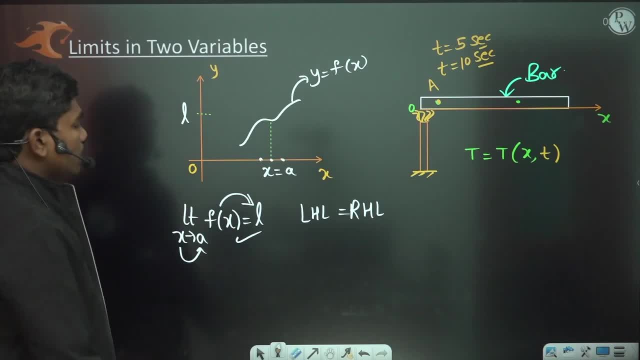 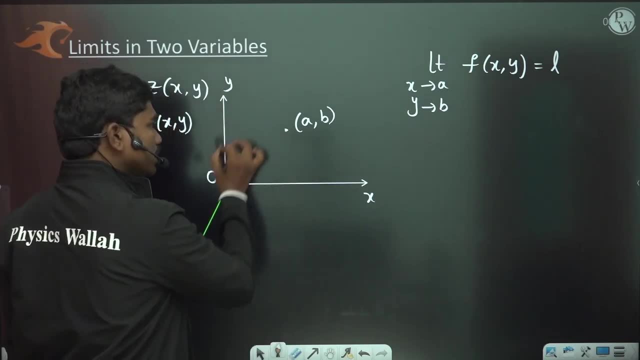 x tends to A here, correct? So we have only x tends to A. For x to tend to A there are two ways. So we have it in left hand limit and right hand limit. But now you tell me, in a two-dimensional system. 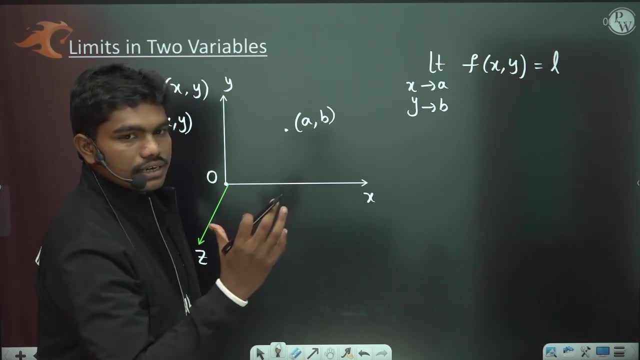 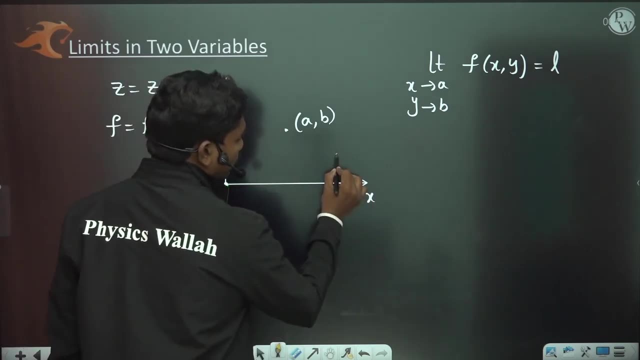 in a two-dimensional system, if you talk about neighborhood, then your neighborhood is actually a circle, correct? Because if you see, if this is the point, for example, if this is the point, then what happens? There are some points which are very close to this, correct? 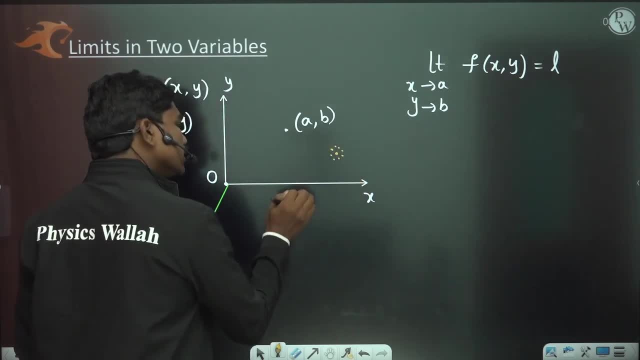 In all the directions. actually Here, if the point is on x-axis, there are only two ways, But if the point is in a 2D space, then definitely there are some many points which are very close to this. So you will actually define the neighborhood with the help of a circle. 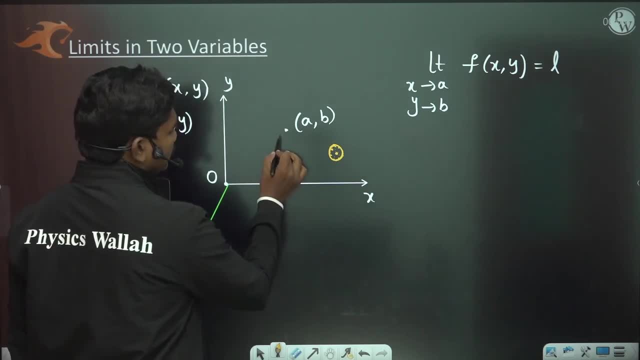 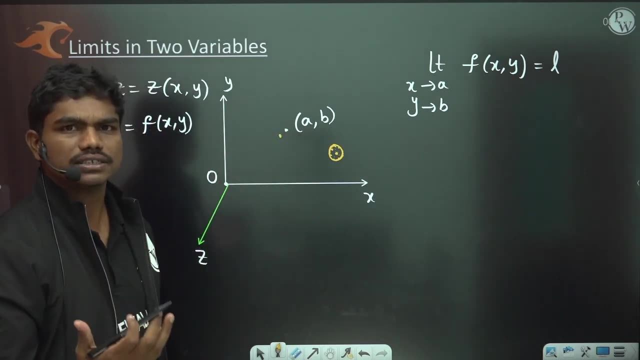 Now tell me If you see to which this point, If, let us suppose xy is somewhere here in the neighborhood of Now tell me how, in how many ways they can reach. There are many ways actually. Look, for example, if these two points has to be connected, I can connect them in many. 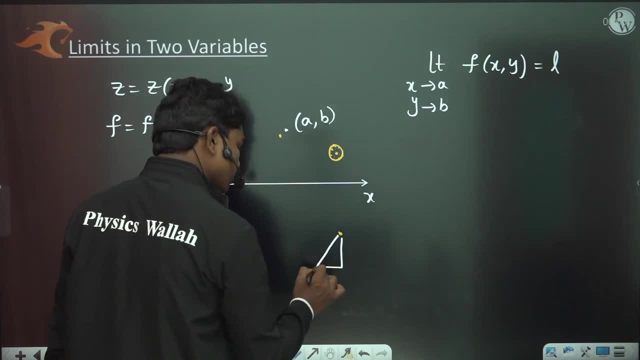 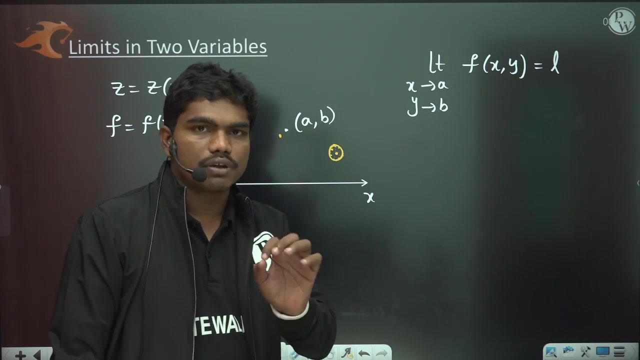 ways like this: then this path and this, then this path and this or maybe some Y is equal to x, some different path, some other path like this, So I can connect them using many paths. So cannot calculate something like left-hand limit or right-hand limit, and all because they generally 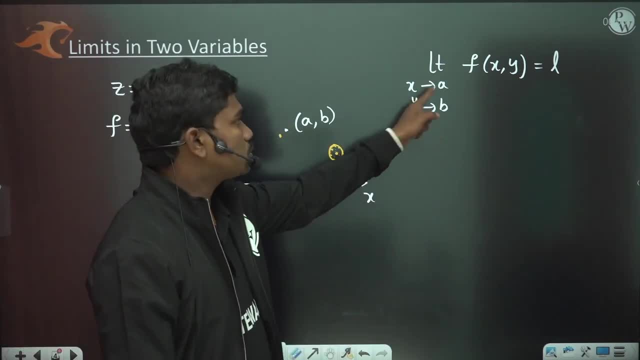 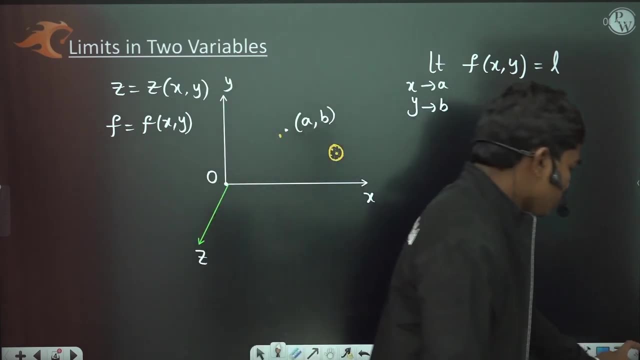 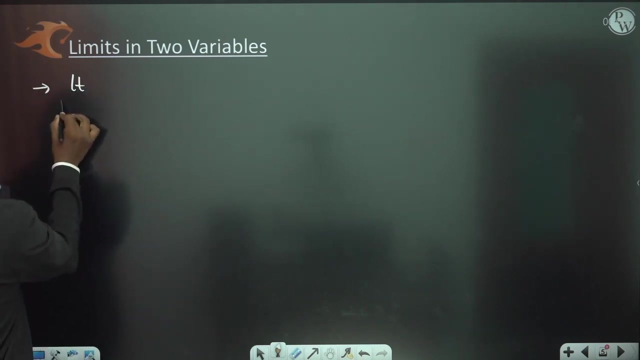 have infinitely possible ways for the x to tend to a and y to tend to b. so generally we actually check some generalized cases, okay. for example, i will give you one question. look one example, one quick example. look see, here let us suppose i am taking limit. x tends to 0, y tends to 0. 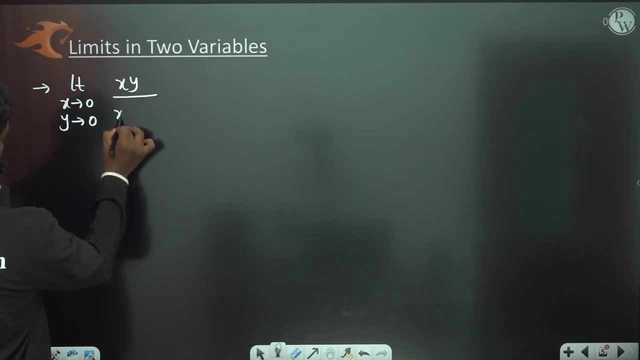 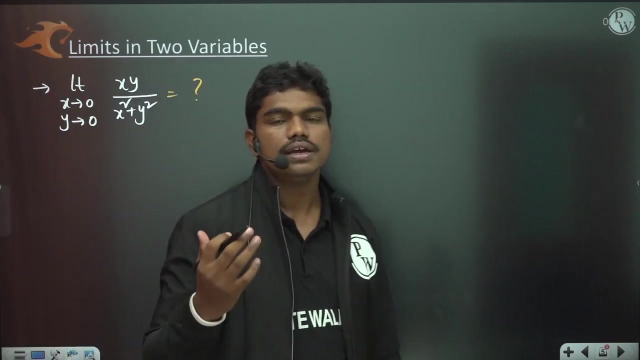 x, y divided by x square plus y square actually. so let us suppose i am taking this equation for example. okay, so if i am taking this equation, then obviously, if i ask you, what is the value of this limit, what is the value of this limit, for example? i have given you. okay, now, first of all, identify. 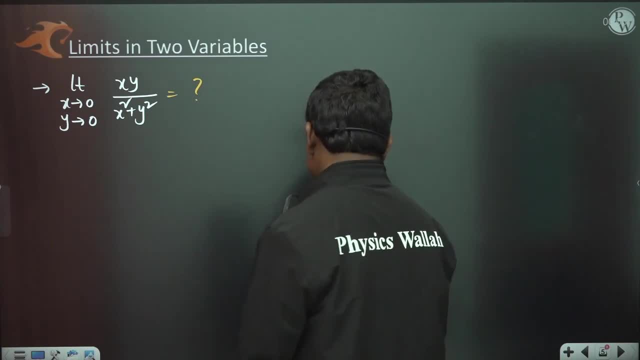 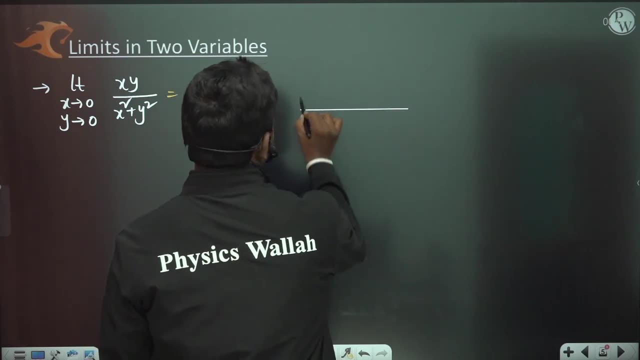 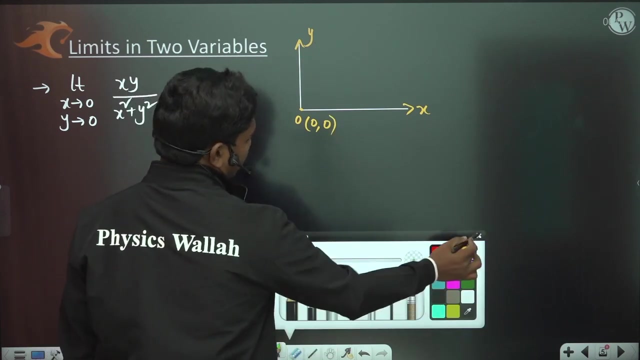 the point horizon: 0 comma 0, correct. now you tell me, on this 2d plane, on this 2d plane, x, y, for example, if i take this is horizon. now tell me one thing, this is the point of interest: 0 comma 0. so let us suppose this point is x comma y is in the neighborhood, so let us assume. 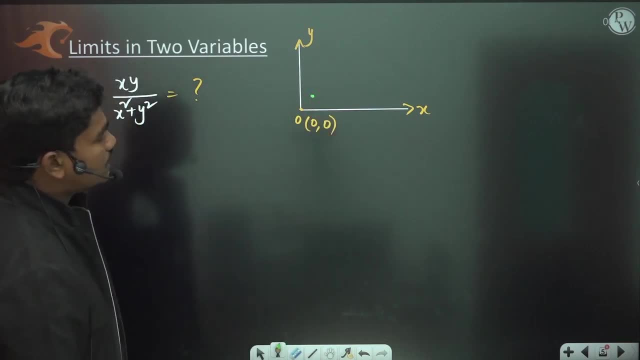 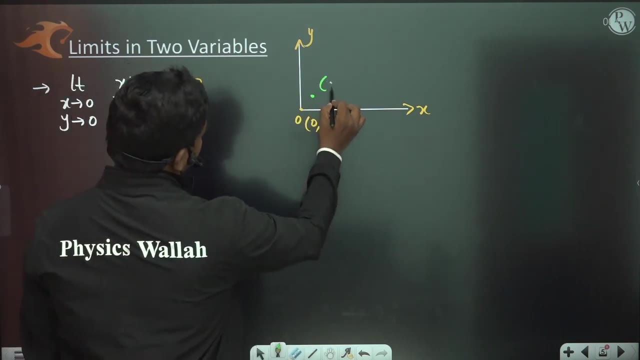 that it is somewhere here, for example. okay, so if that point is somewhere here now, let me take three paths. out of these three, one is very generalized path. look, this is the point x, comma y. now, if you see, if you want to move this point towards this point, there are generally many ways out of. 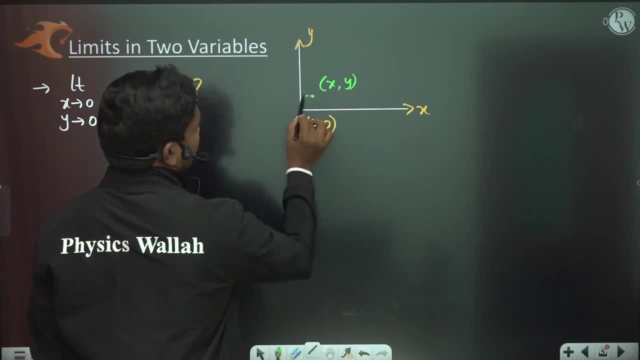 which i'll specify few things, okay. so see here: first this point can be moved like: this means making x coordinate zero, and then it can come to like this: this is one path in which this point can reach x comma y. or you can take this point, or first you break the y coordinate zero and then you 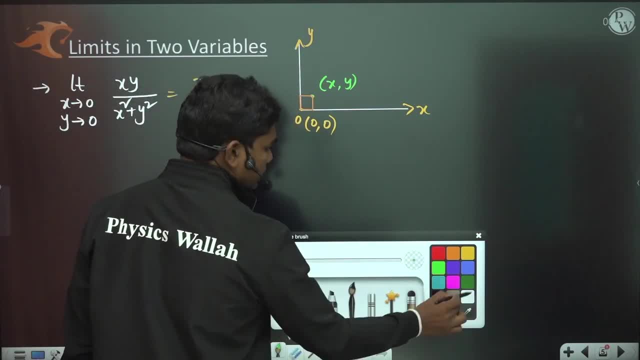 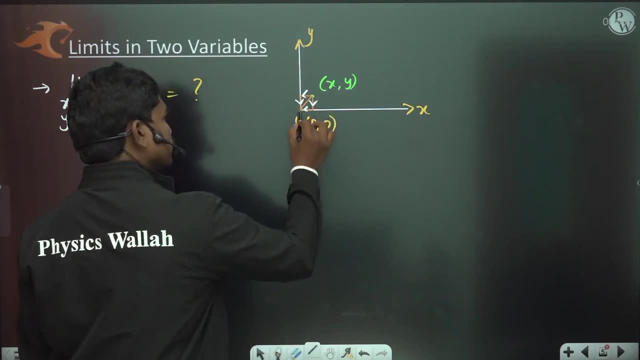 can transverse along the x direction. so this is another way. so if you see these are two ways and also you have the third way, the point can directly transverse along the equation: y is equal to some mx, depending upon the x comma y values. okay, so this equation is: y is equal to mx. so let us try. 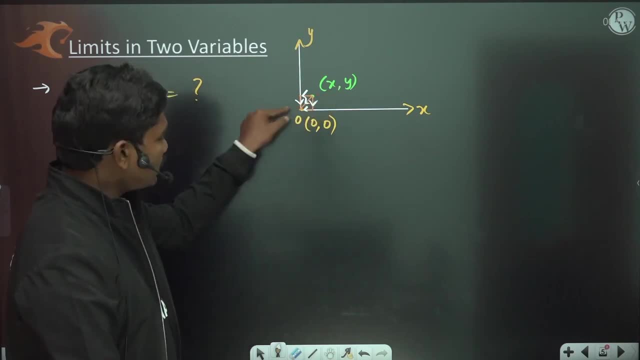 to calculate the limit in these three paths. okay, so x comma y is tending to zero comma zero along three different possible ways, out of which one is generalized. okay, so now, if you see first path, first path, what i have taken is you make the x coordinate zero and then y to zero. so in this limit, what we'll do in first, 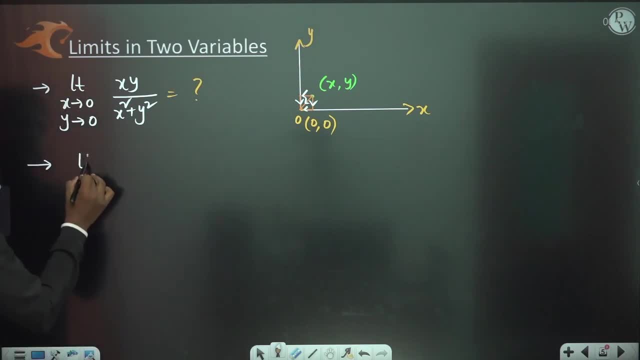 method or in first path. if you see limit first, you're making x coordinate to zero. so substitute x is equal to zero in this equation. so limit y tends to zero. zero times of y divided by zero square plus y square. so this is equal to zero. obviously zero into something divided by y square. 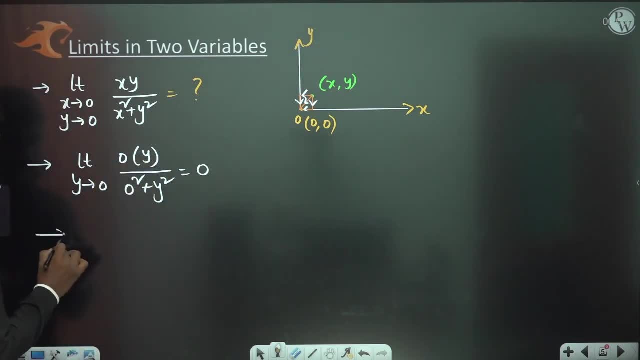 this value is zero. now, second path: in second path, what we have done, we made the y coordinate zero first and then made x coordinate zero. so limit x tends to zero because we have already made y zero. so let us substitute: y is equal to zero, x into zero by x square plus zero square. okay, so this value is also again zero, zero into something. 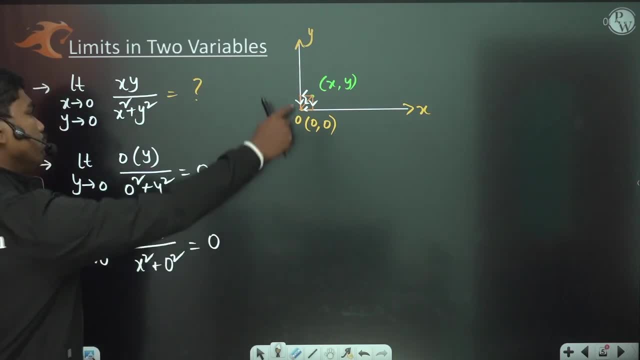 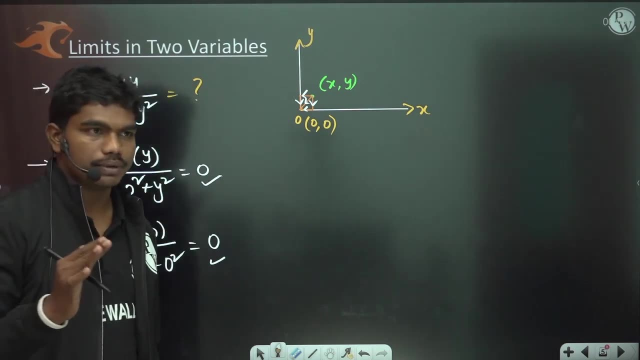 by x square, this is zero. so we feel that in both these paths the value is zero. so the value of this limit is also zero, but it need not be the case, because we have already made the y coordinate zero. Look, let us take the third part: generalized part. 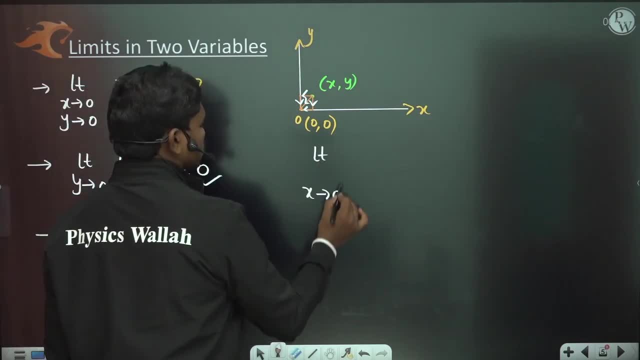 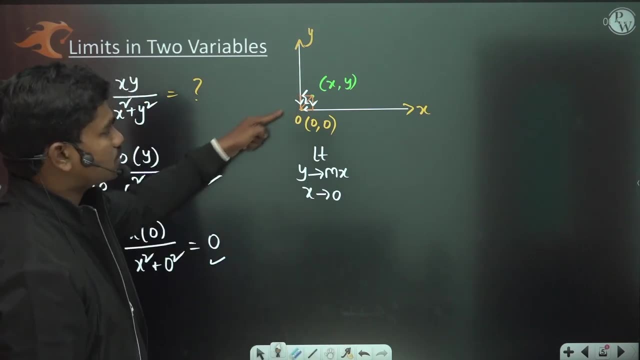 Limit. x tends to 0,, of course, because x comma y should tend to 0. But let us suppose y is coming to x along this equation, y is equal to mx. This is some straight line, actually okay. connecting the points x comma y and 0 comma 0, actually okay. 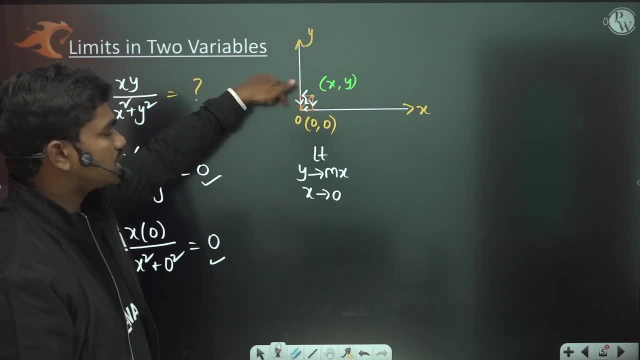 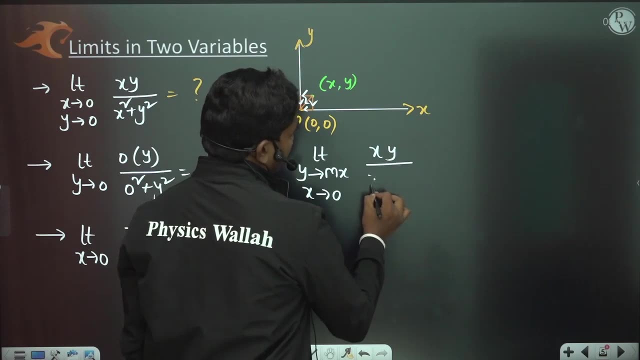 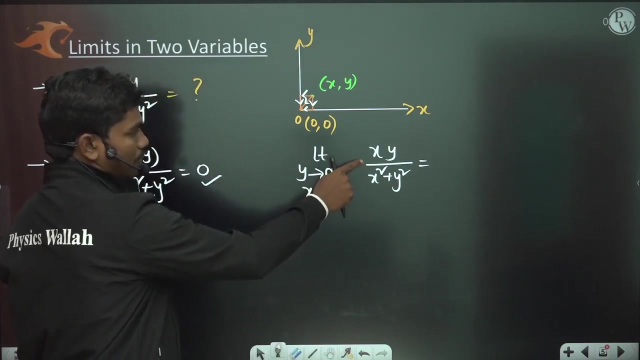 So, depending upon the xy values, this y is equal to some mx because it is passing through the horizon and x is tending to 0.. Now let us write the function xy divided by x square plus y square. So if you take this function, so this is equal to. now, first, if you substitute y is equal to mx in this equation. what comes out? 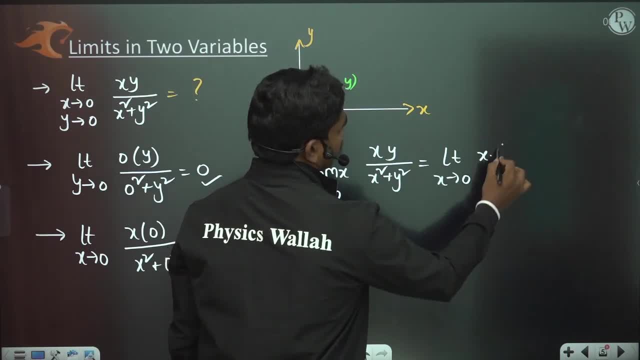 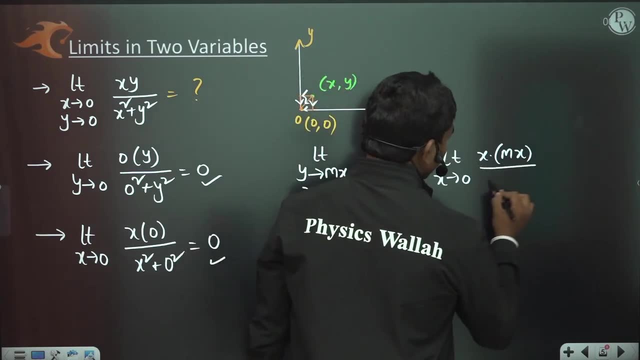 Limit x tends to 0, x into y is nothing but mx. So divided by, divided by x square plus y square, x square plus y square And this y square I can write as mx whole square. okay, So mx whole square. 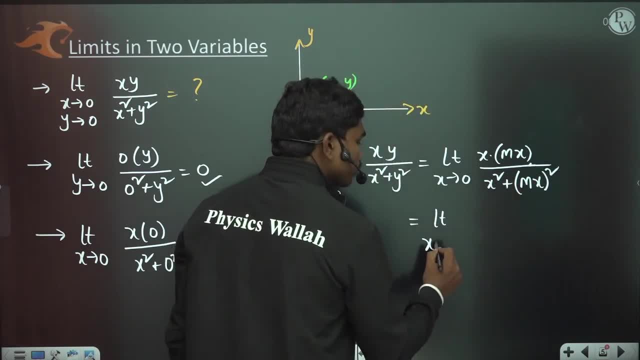 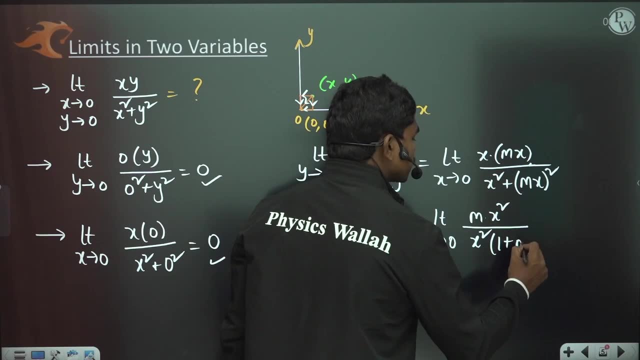 So if you simplify this limit, x tends to 0, m times of x square divided by. if you take x square common, you have 1 plus m square, So x square and x square gets cancelled. So, if you see, the answer is m by 1 plus m square. 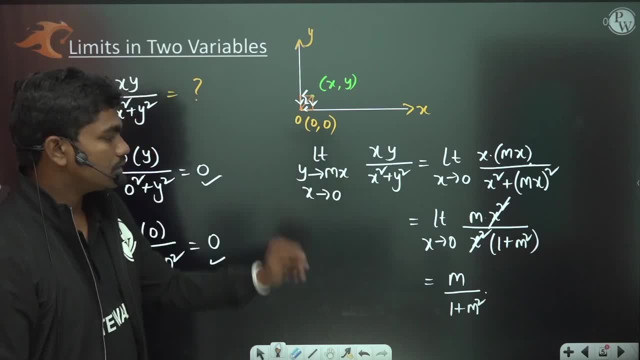 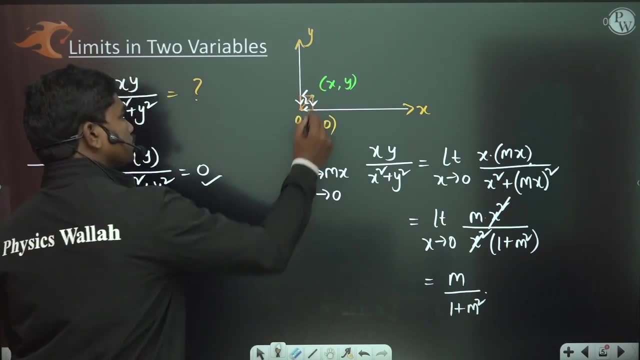 Now tell me one thing: This limit it is not 0 and forget about 0.. Now, if I take different values, of m means, let us suppose if I take some point, let us suppose somewhere here in the neighborhood. okay. 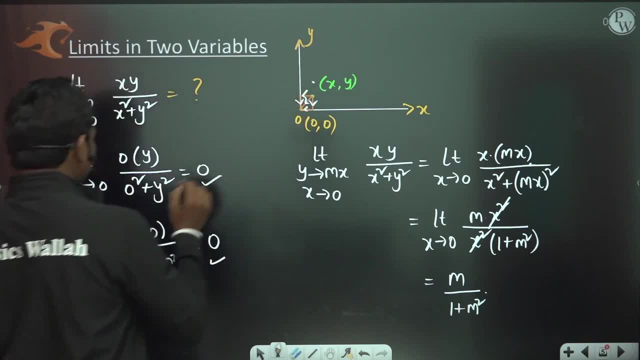 These two parts remain same means first making the x coordinate to 0, then y to 0, you will get the same result. Making y 0 and x 0, you will get the same result. But connecting this point and this horizon to you know, a straight line gives you some different value of m as compared to this case. 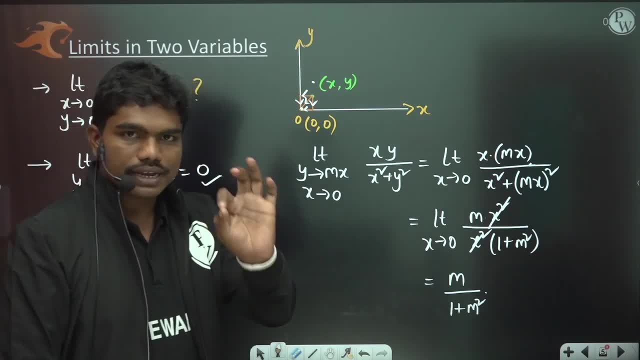 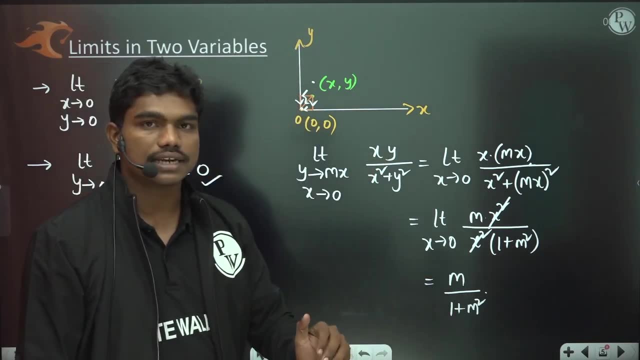 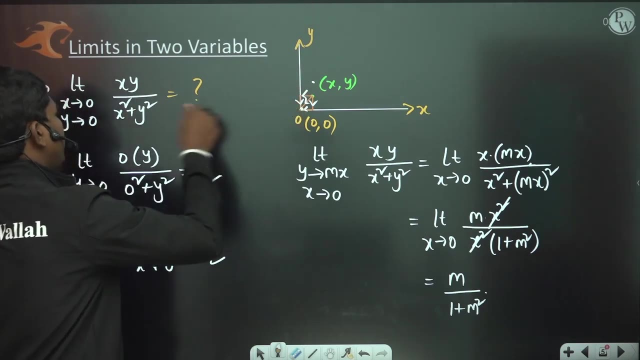 So, which means it depends In a neighborhood, if you take any particular point and if you tend towards 0, along different, you will get different answers because this m value is actually different, clear. So I am repeating normally in a 2D space for a point in the neighborhood, to tend to point a, comma b. 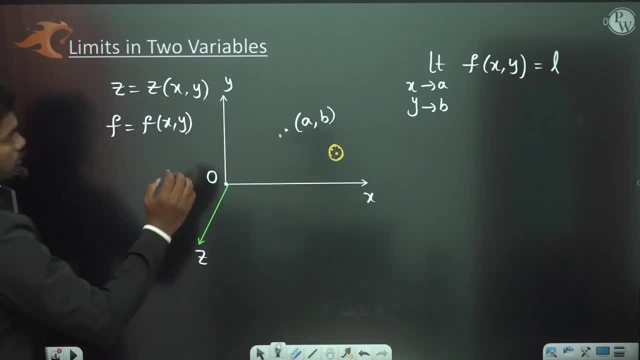 Of course, in this case I have taken 0 comma 0. Here I have explained you for a point in the neighborhood to tend to this location: a comma b. there are many possible ways, So we actually need to calculate this limit in many possible ways, of course, okay. 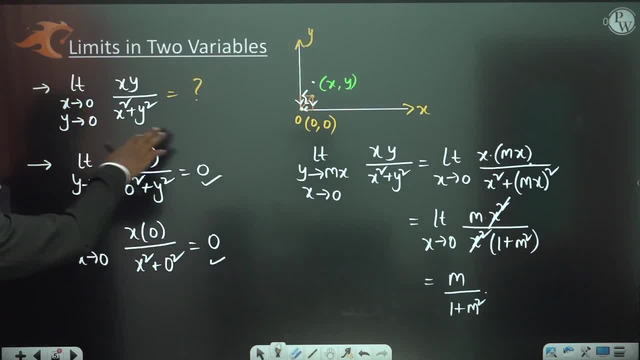 But at this BTEC level and all, we have this normal standardized 0. So you can take the values and all a simple limit even for the gait exam. these questions were asked- some, you know, a very few times actually. 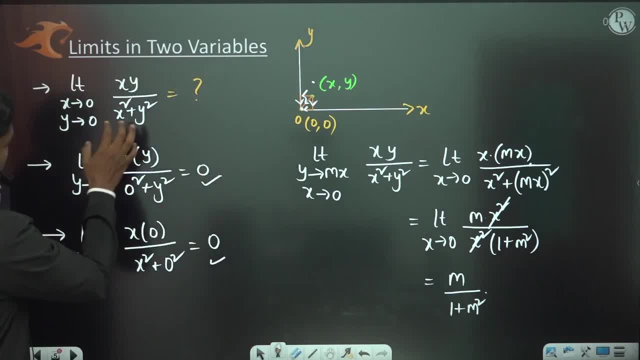 So that's why I have given you this particular example. So, if you see this question, for the point in the neighborhood of 0 comma 0, to touch horizon, we have taken three different ways, out of which two ways are very much standardized ways. 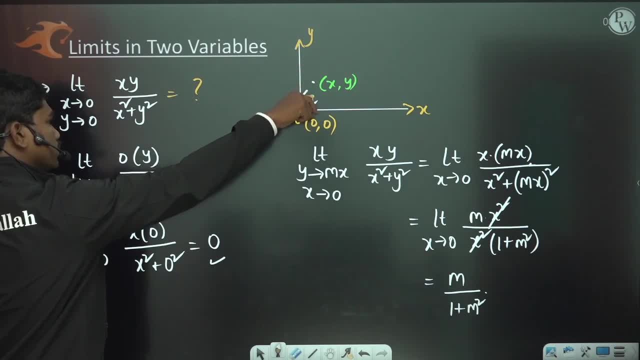 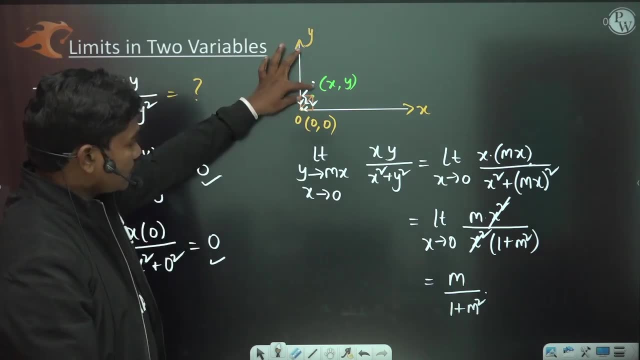 Making the x coordinate 0 and y 0, or making y 0 first and then x 0. or then we have taken the generalized case y tends to m x means basically this y tends to m x. And then we have taken the generalized case y tends to m x means basically this y tends to m x means basically this y tends to m x. 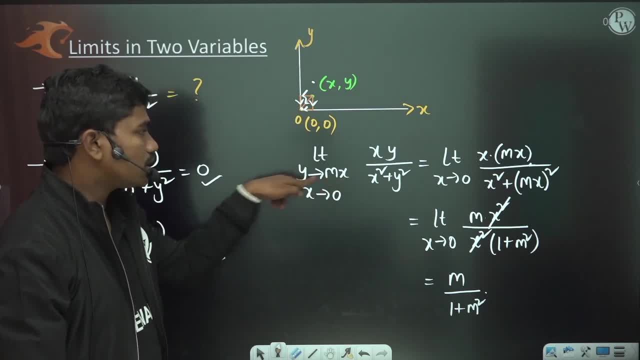 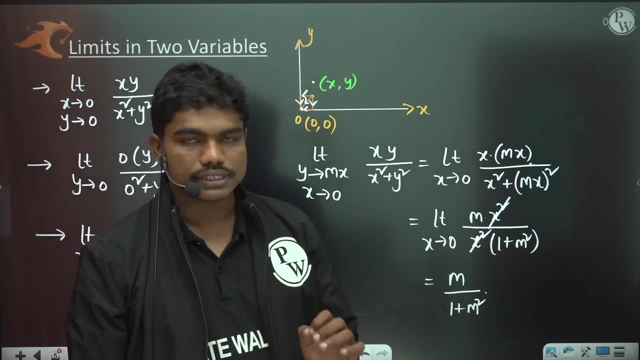 This point tends to 0 along the straight line, which is this path, and obviously X has to tend to 0, finally, Okay, so this we have substituted. We have got this expression, which means for different points in the neighborhood approaching in different ways this. 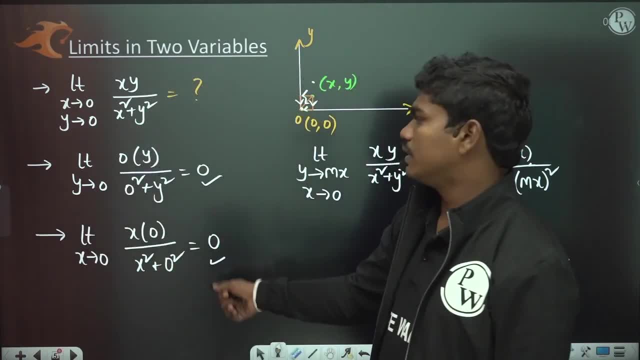 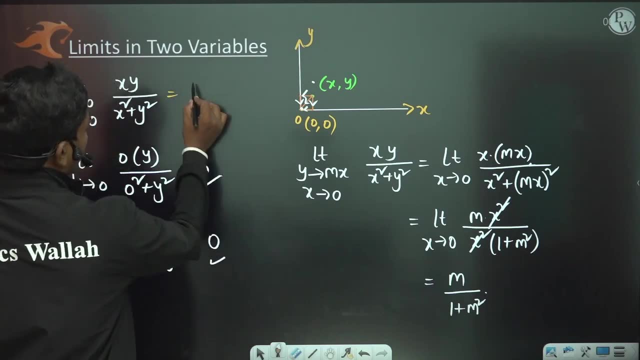 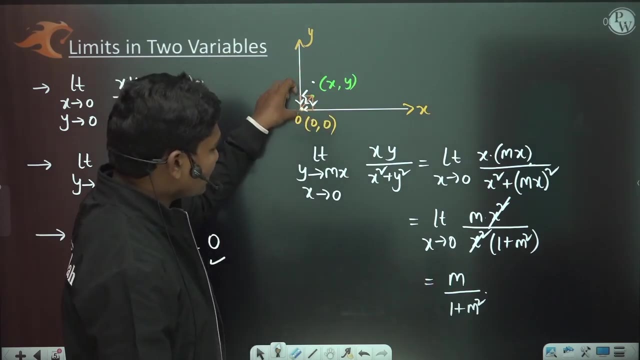 Value is actually different and this value is not equal to 0. So that's why we say this limit does not exist actually. Okay, so this limit Actually it does not exist because of this season, because, if you see, for different points approaching in at different slopes, 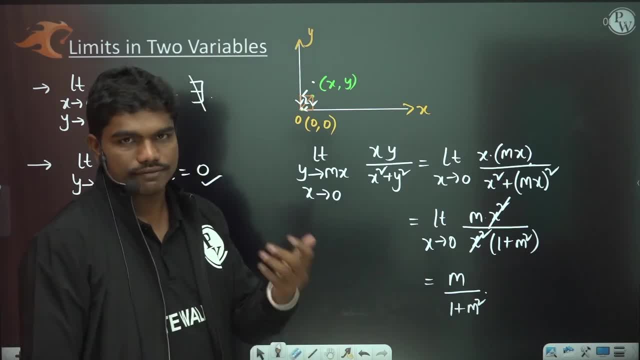 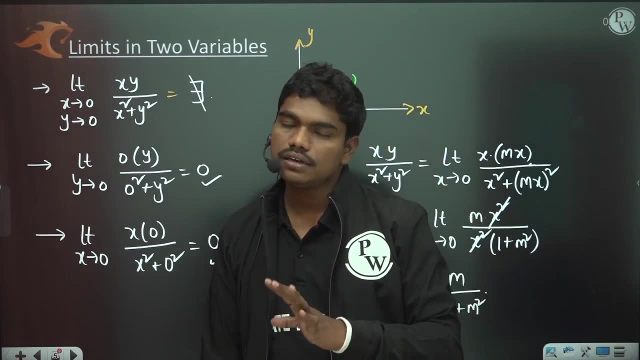 This value, M by 1 plus M square, gives different values. Okay, so that's why the value is not unique. So that's how we say this limit is actually not existing in this calculus, Okay. So, similarly, if you take some other function, like, for example, you can take some functions like: 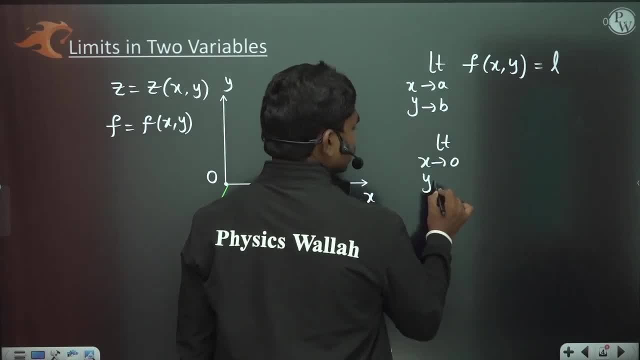 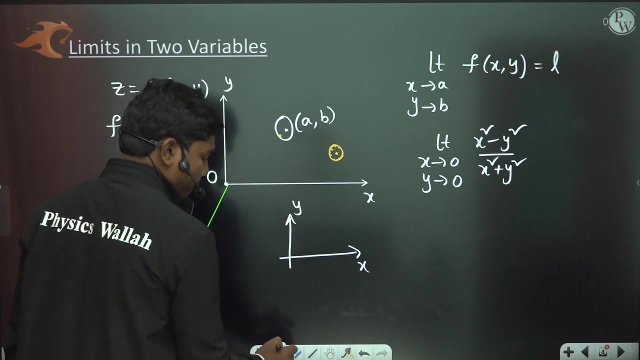 limit. X tends to 0, Y tends to 0, X square minus Y square by X square plus Y square. Now, if you take this point again, this curve, if I draw X, Y and Horizon, for example Horizon, so if you take a point in the neighborhood X comma Y, this X comma Y should tend to 0 comma 0. 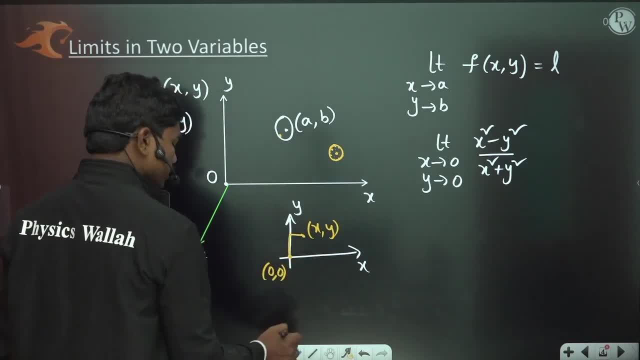 So let us take two paths. This is one path and this is an, you know- continuation, So this is one path. similarly, let us suppose I- I'm sorry excuse me, So now, if you see this, but X comma Y is 0 comma 0. 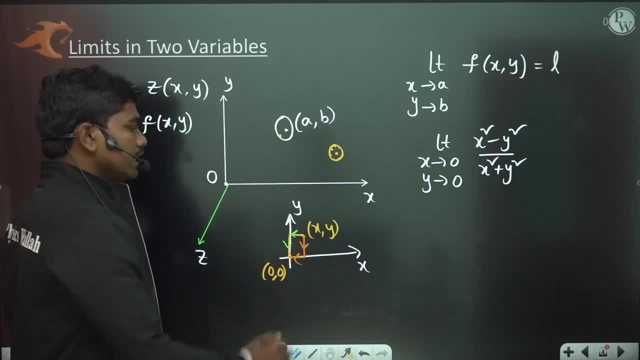 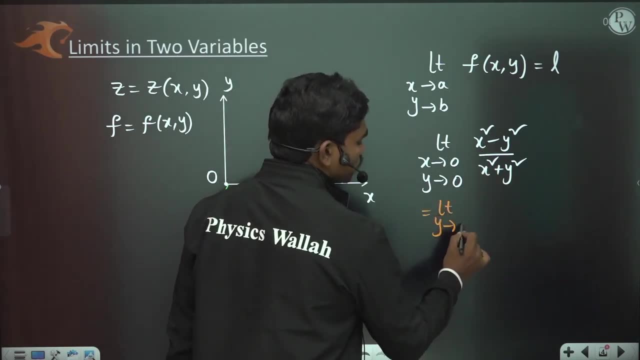 Now, if you take these two different paths, let us take the first path first, in first part. first you are making X coordinate to 0, so X is equal to 0. if you substitute directly you will get limit to Y tends to 0: 0 square minus Y square. 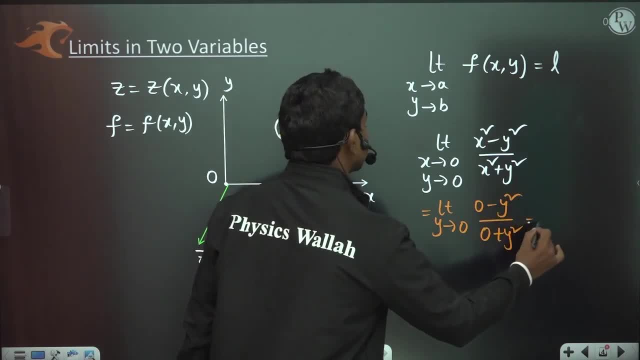 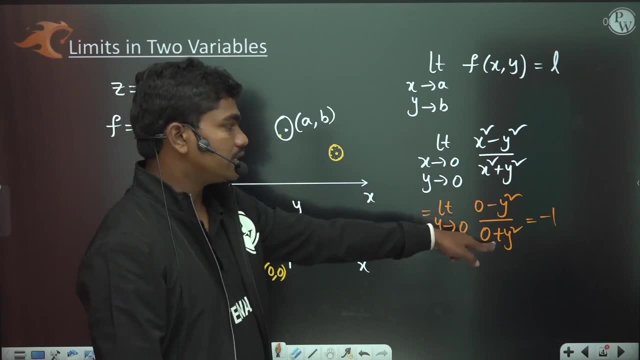 divided by 0 square plus y square, So the answer is minus 1, correct? because if we simplify minus y square by y square, y square, y square gets cancelled. You have minus 1. why I am cancelling y square and y square? because y is not actually 0, correct? 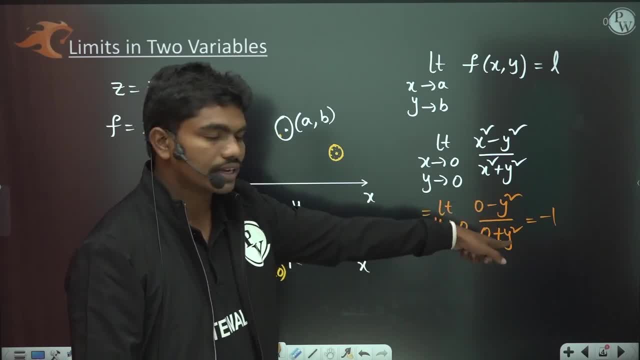 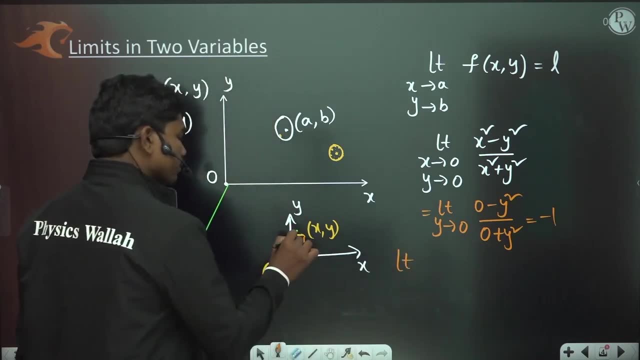 y is just tending to 0, which means y is not 0, so we can cancel them. so you got minus 1. now if you Take the second path like this, Limit first of all. in second path you are taking: y tends to 0, so we'll write limit: x tends to 0. 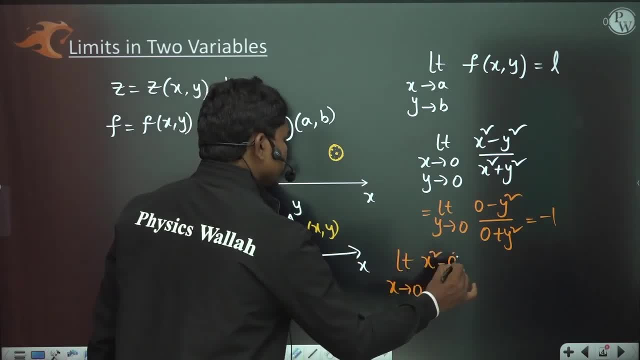 x square minus 0 square. because why? you have already substituted 0, because we have already made y is 0, so x square plus 0 square. okay, so if you simplify this, the answer is 1, of course x square and x square gets cancelled. 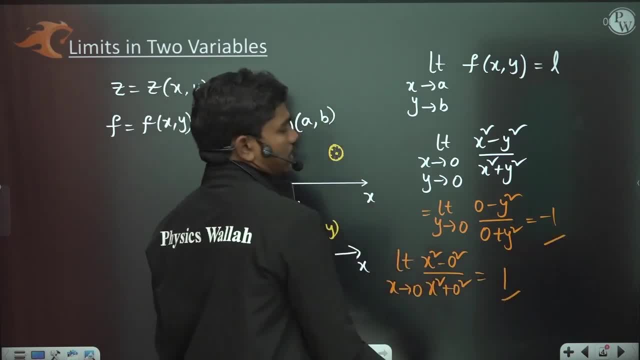 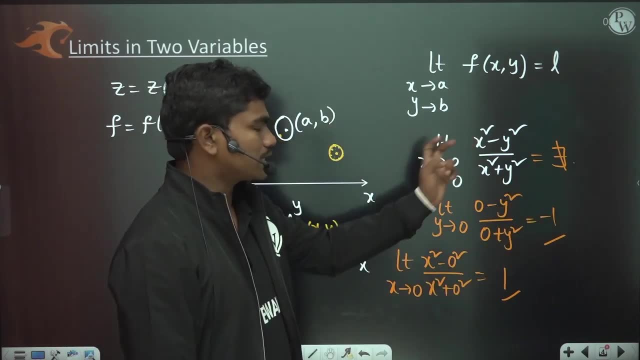 So if you see, in these two paths this have two different values, so that's why this limit also does not exist. but there will be some functions that First if you substitute x tends to 0, and then if you substan y tends to 0, first this will give you the same values. 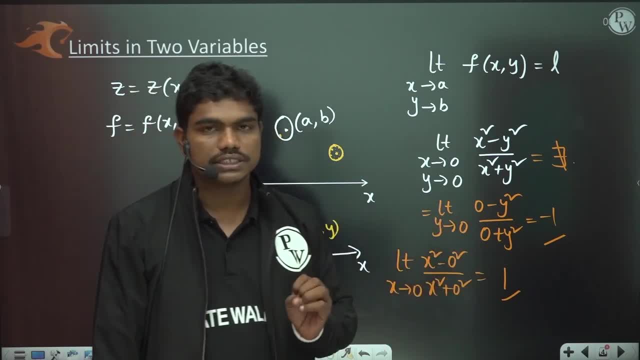 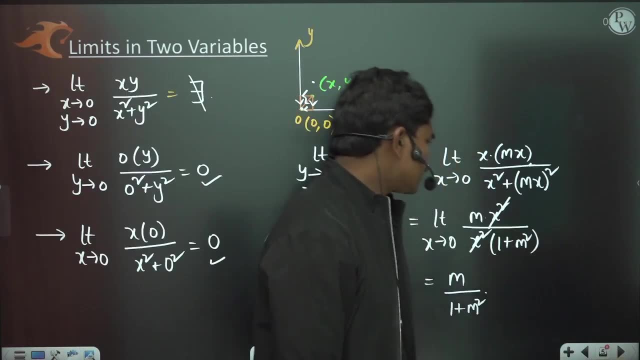 I, And also along any path, they'll give you same values actually. so in such cases you can declare the limit is some particular value, But right now, in this case, if you see The limit is straight away Not existing in these two cases. okay, so that's how, in general, it to calculate limits in, of course, 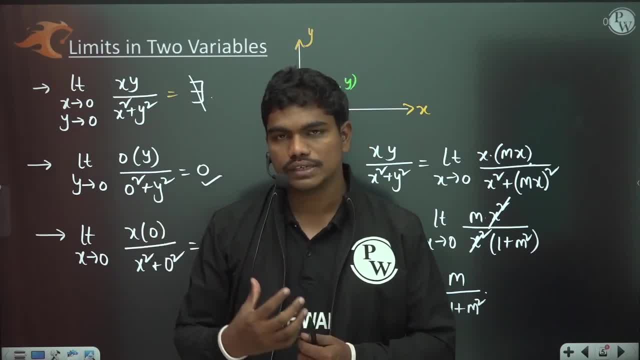 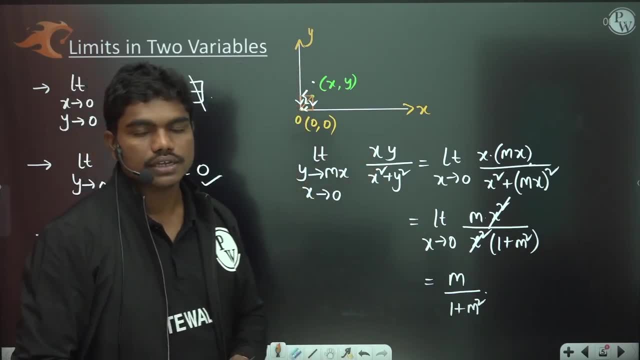 This is a two variable limits. So even if you want to calculate two variable limits, you need to check multiple paths, out of which generally one of the paths is Given. the most general path y tends to mx. okay, so it depends upon the point you are taking in a neighborhood. 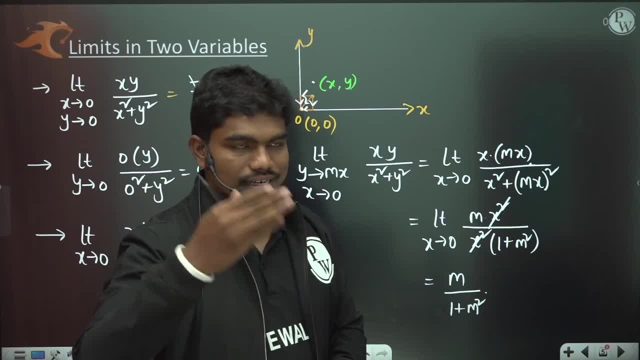 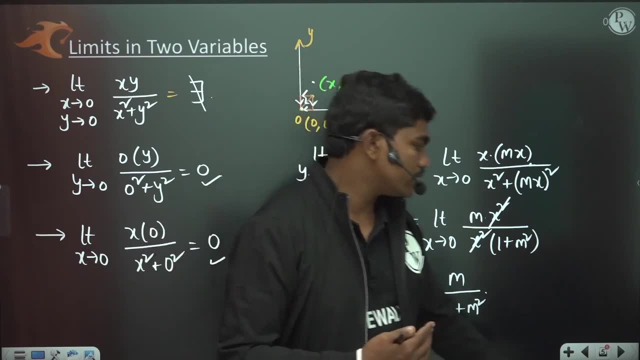 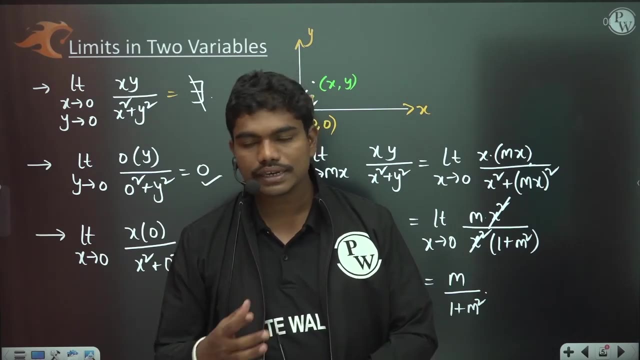 So that obviously the orientation of the point or the line connecting these two points will change definitely. okay. so that's how we calculate The limits in two variables. okay now. so once we have discussed limits, We have talked about continuity cut in single variable calculus, so in single variable calculus. 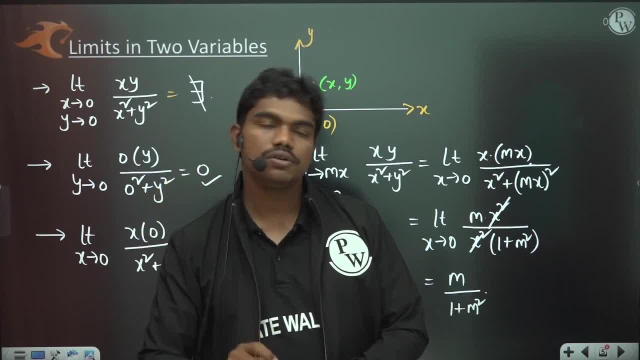 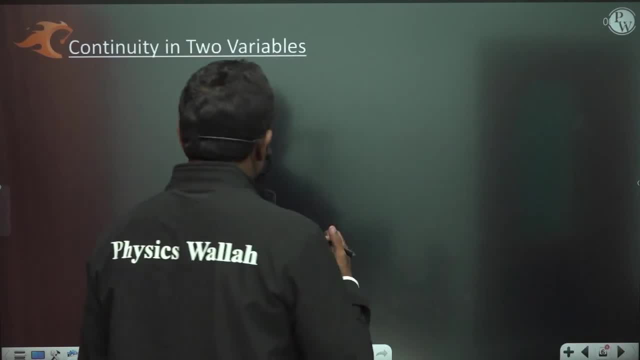 I told you, this limit value should be same as the functional value for the limit. I mean for the function to be continuous at that point. so, similarly, if you talk in two variables, Let us see how you define the Continuity of function in two variables. okay, so here, of course, we define a. 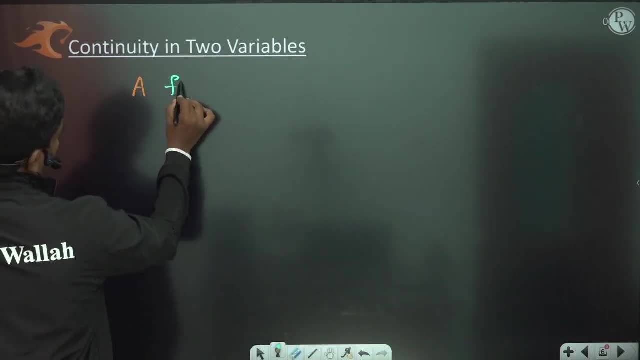 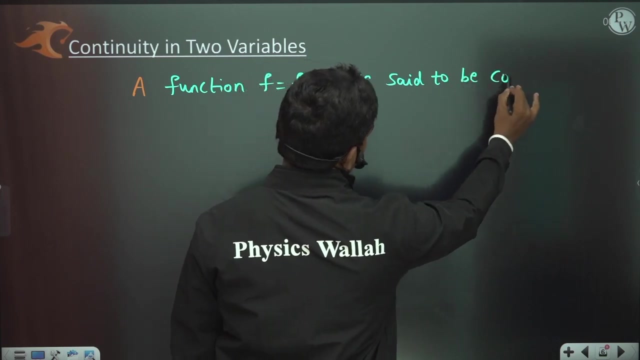 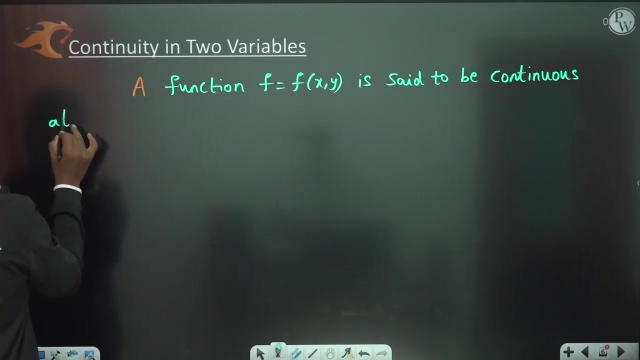 continuous. You can say a function, F is equal to f of x comma. y is said to be continuous, Is said to be Continuous, is said to be continuous at a comma b. at a comma b, if limit extends to a, y tends to be. or you can write in the reverse order also: y tends to be, extends to a. anything is fine. 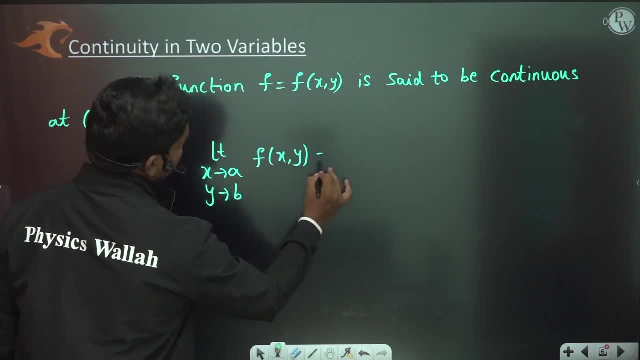 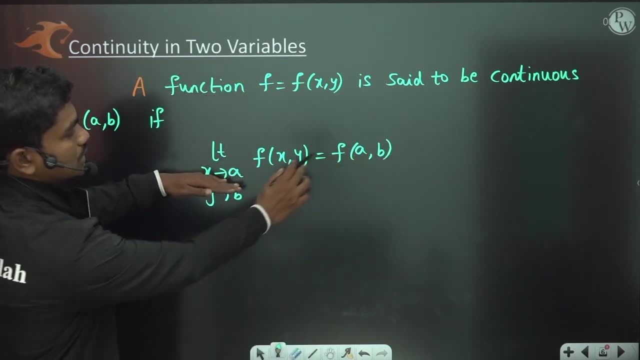 f of x comma y is equal to f of a comma b. So basically in single variable calculus we have only limit extends to a. f of x is equal to f of a, but here it's Two variable calculus. so at that point we have just seen how to calculate the limits, and once you have 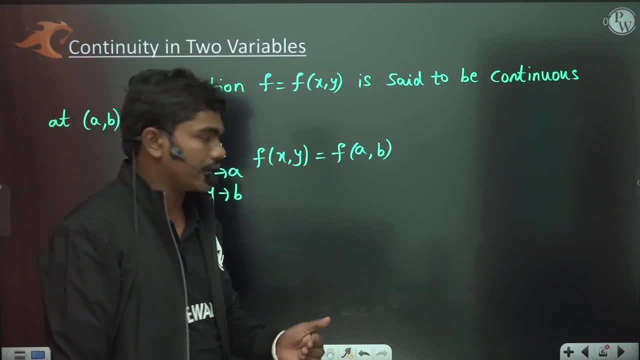 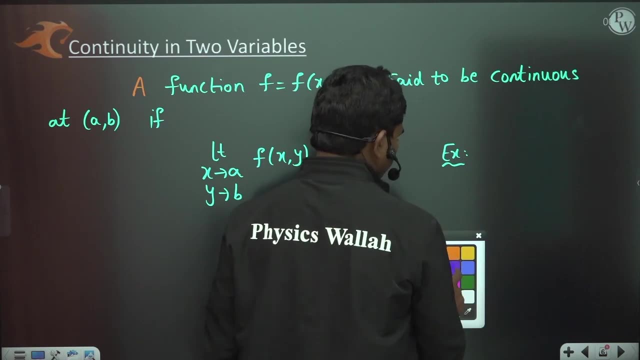 Calculated the limit. that limit value should be same as the functional value again. okay, So let us suppose if I give you some function like, for example, X example, What are continuous function? generally we have x square plus y square. okay, So let us suppose you have f is equal to f of x comma, y is equal to 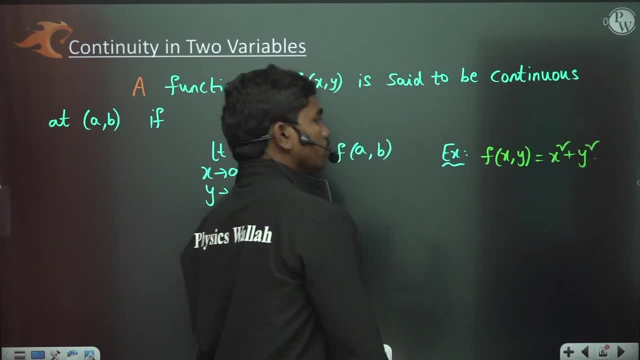 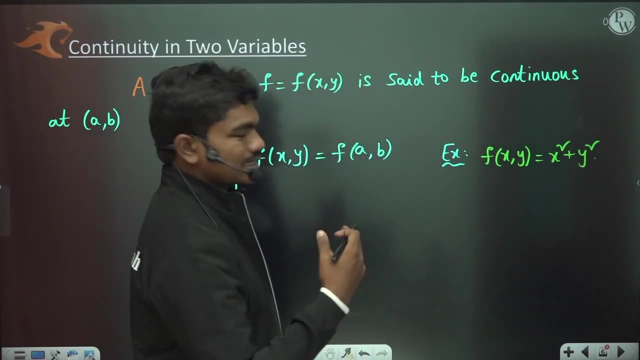 x square plus y square. okay, so x square plus y square. now let us suppose, if you take this point, this one is a continuous function, because whatever you take X and y values, definitely this function keep on being continuous. Okay, you always generate some value of z actually here. 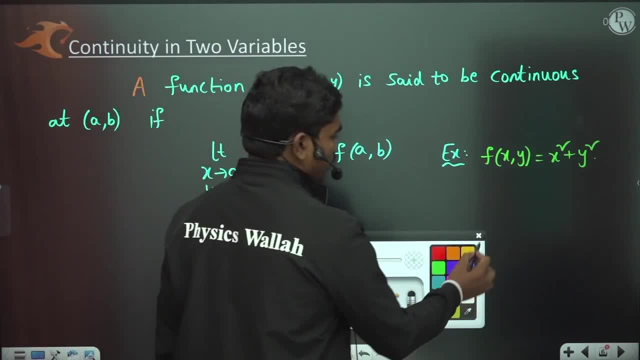 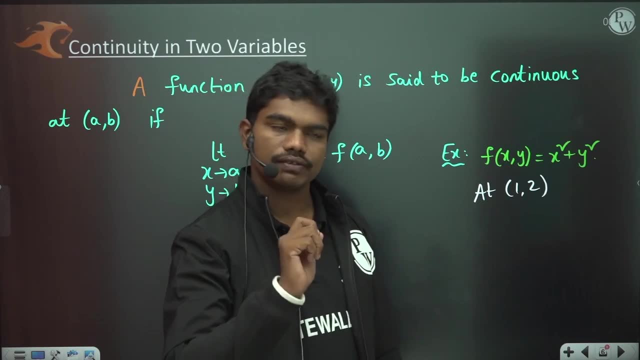 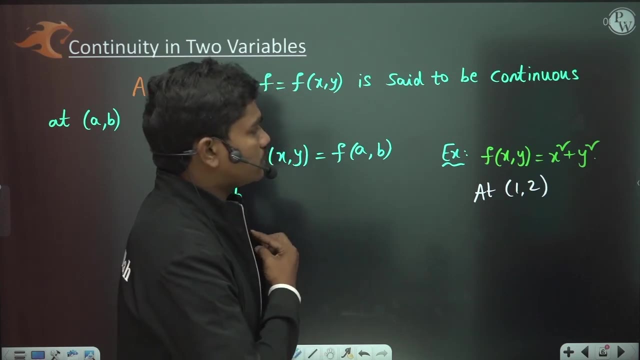 So at one point, if you want to calculate at 1 comma 2 if this function is continuous or not, We generally know this function is continuous because whatever the values you take for x and y, definitely there is always a z value. You don't have any denominator and it is a basically continuous and of course a differentiable function also. So now, if you see, 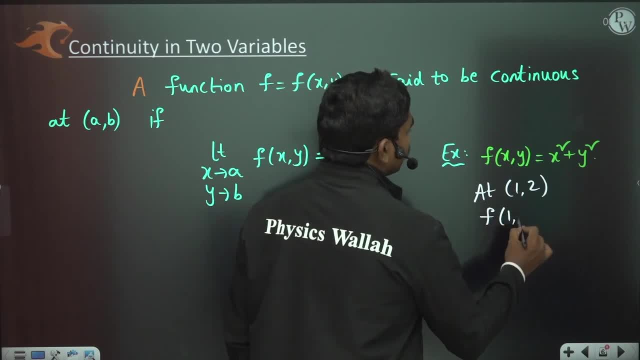 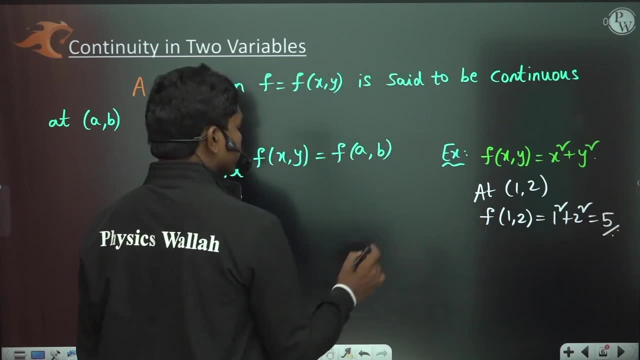 At 1 comma 2. how you will calculate the functional value: f of 1 comma 2 is equal to 1 square Press 2 square, which is 5, of course. now if you want to calculate the limit, you write: Limit at 1 comma 2 is the point of interest. So limit extends to 1. 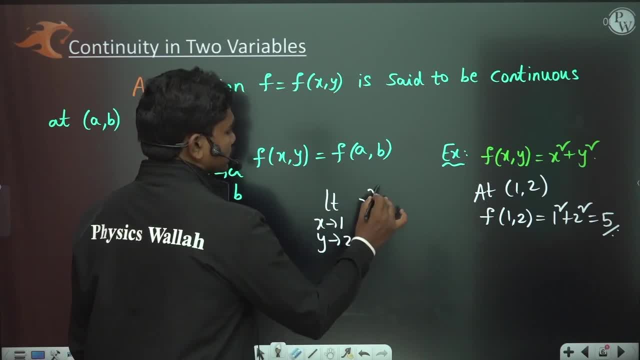 y tends to 2, f of x comma y, which is x square plus y square. okay, so which is x square plus y square? actually? Now, if you substitute these values, first of all let us substitute. if it keep, x is equal to 1 here. 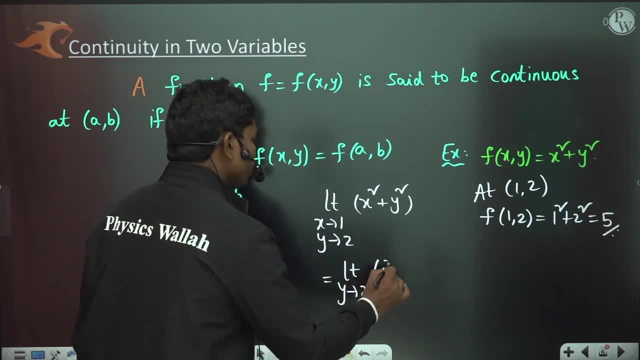 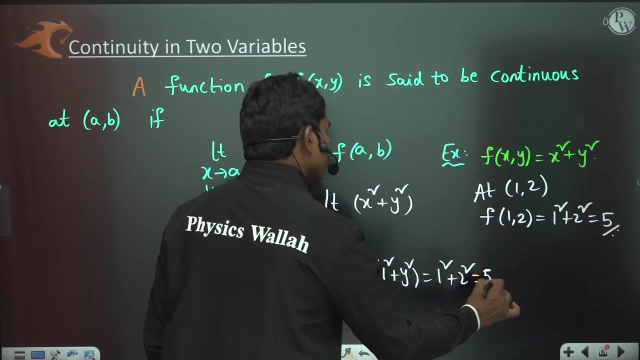 this changes to limit. y tends to 2, 1 square plus y square. So if you substitute y is equal to 2, this is 1 square plus 2 square, which is 5. Similarly, if you substitute y tends to 2 first and then extends to 1, obviously again. 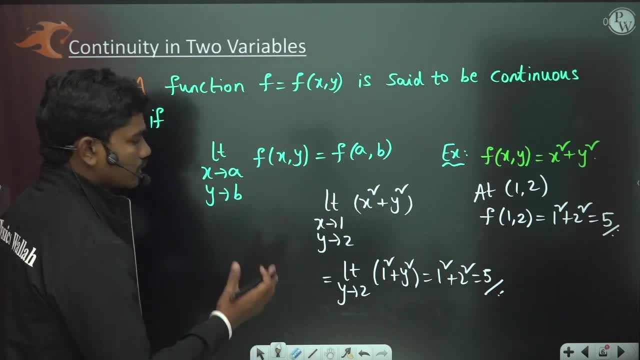 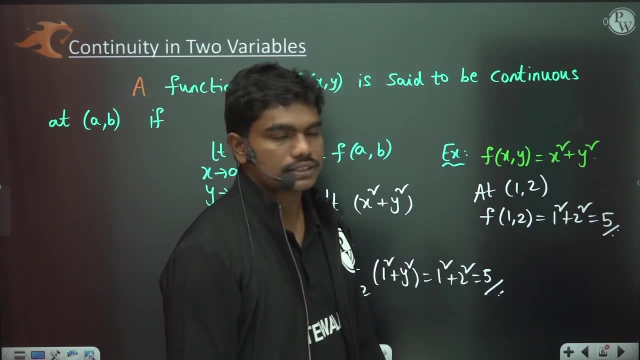 You will also get the same result, which is 5. So obviously this limit has the value of 5 at this function, at this point 1 comma 2, And this is also equal to the functional value. So that's how you will get this. 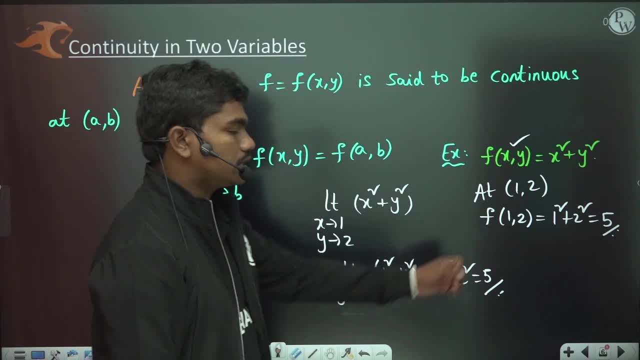 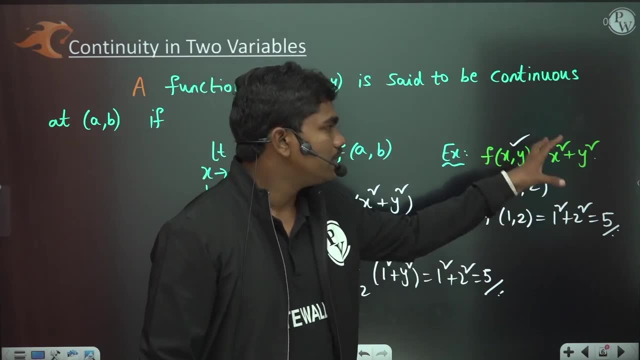 You will tell that this function is a continuous function And, of course, if you see, basically this function don't have any disturbance, Disturbance with respect to the substitution of the points. So that's why this x square plus y square is always a continuous function. Okay, so I think this 3d calculator is at least. 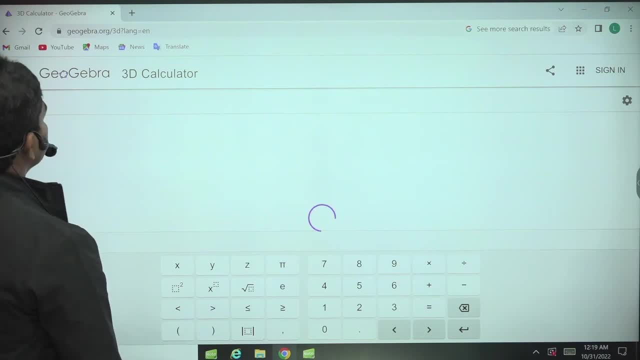 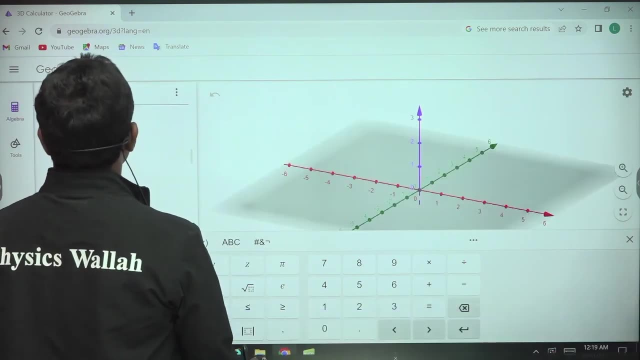 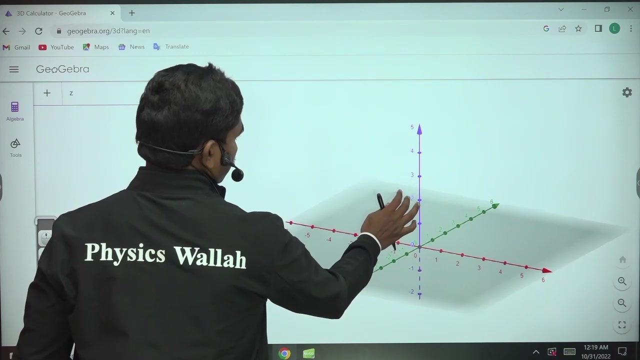 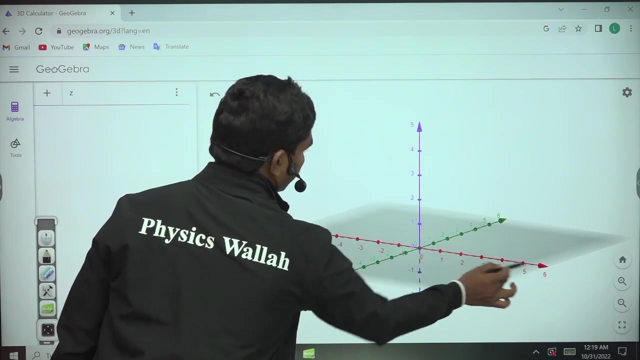 Ready by now? 3d calculator: Okay, so fine, if you type here, z is equal to Okay, fine, something is happening here Just a minute. Okay, This is planes. So if you see, we have the planes here, so We have three planes green. I mean this is the horizontal plane and this is the vertical plane. 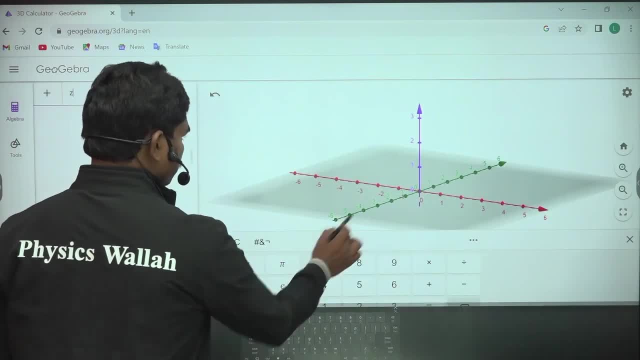 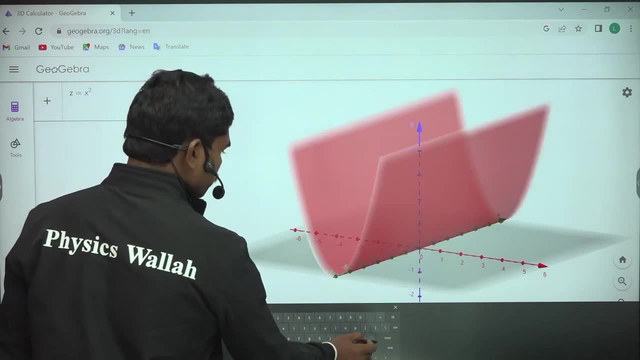 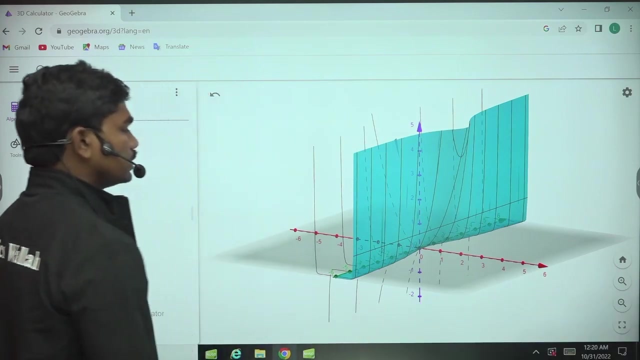 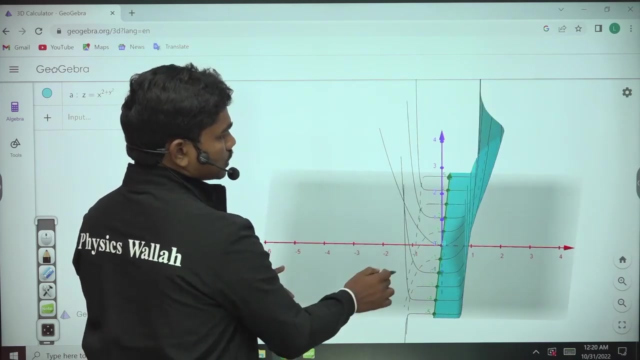 so here, if I type that z is equal to Z is equal to x Square plus Plus y Square. so now, if you see, this is how the graph of z is equal to x square plus y square is looking actually, of course, In a 3d, if you see, you will get some curve like this, of course. 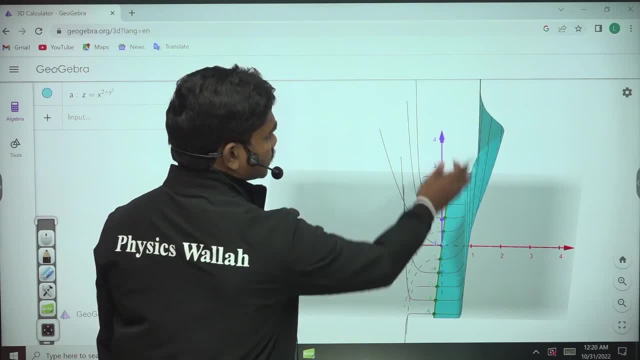 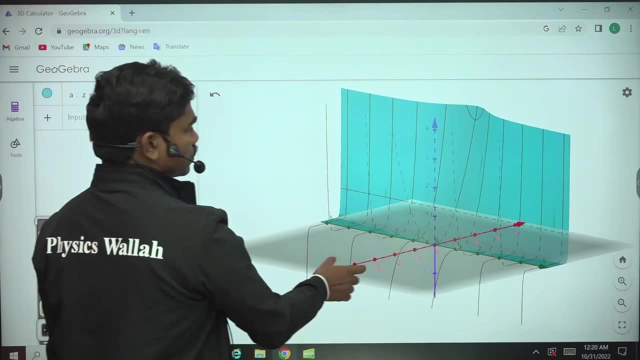 So if you see what are the values you take in the horizontal plane, definitely there is some z coordinate that's getting and this curve, This function don't have any breaking. Anyway, it's a surface, of course, because it's 3d, So practically drawing on board these 2d and 3d surfaces is difficult. 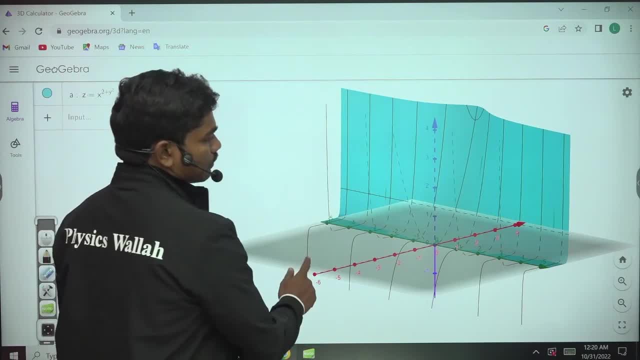 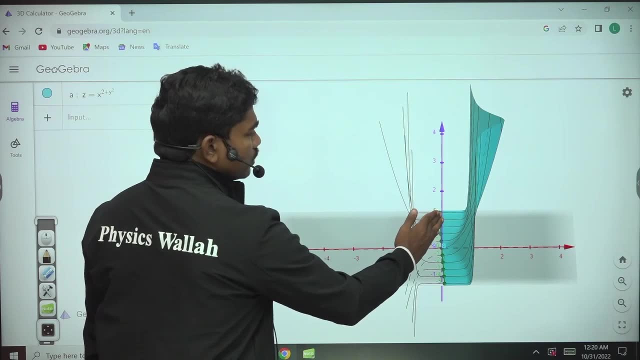 So I have taken this advantage of graphing calculator. but this is how. the graph of z is equal to x square plus y square. Looks like here: Okay, so if you see, We have only the values above this axis, correct. If you see there is no graph below, 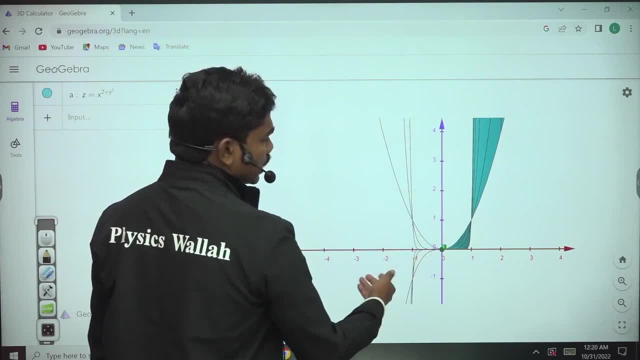 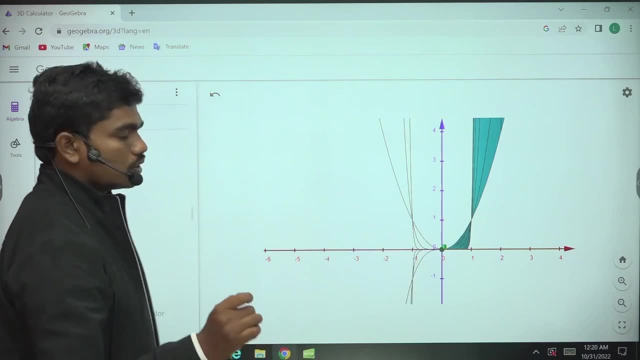 This means if you take the z axis, if you observe what the z axis, you don't have any graph below this. because if x and y Are any values, then z is always positive, because x square is always positive, y square is also positive, always Okay. so that's why z can never be negative. So if you see along this z axis, 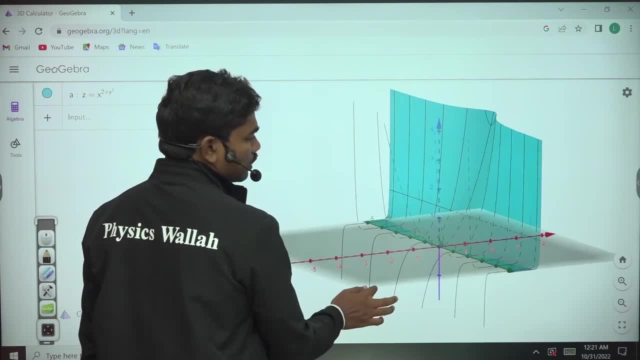 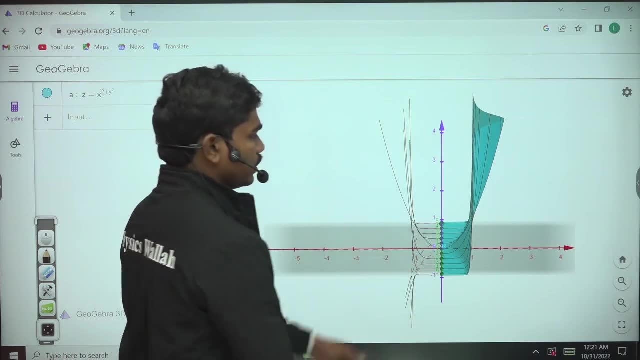 There is no graph below this. z is equal to 0. if you see, in the horizontal planes and vertical planes You can see all values, whatever you can plot, definitely you have a positive values and this function is Continuous. you don't have any breaking of the surface anywhere. So if you see, it's a continuous, neat surface, okay. 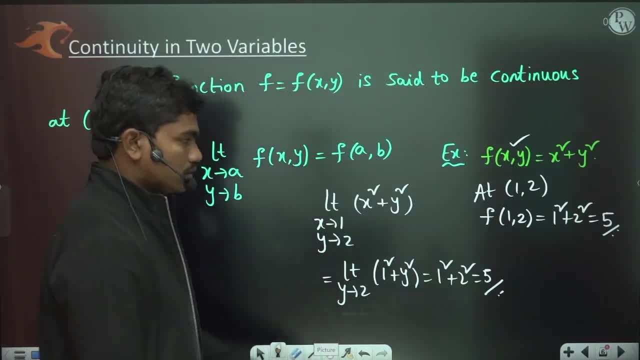 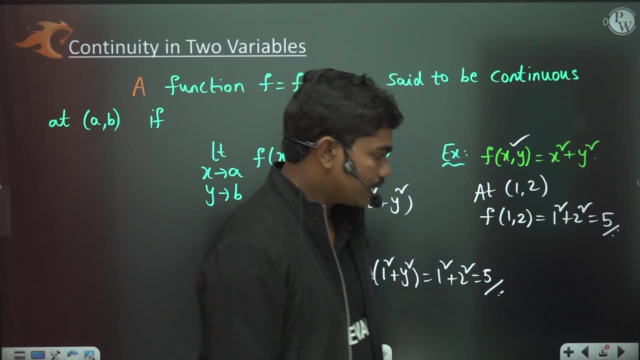 It's a clean surface with continuity all over. So that's how we can see that the graph is giving a value of 5 basically here. Okay, because practically we know this is a continuous function. Okay now, Once we are up to this, then let us talk about something called partial differentiation. 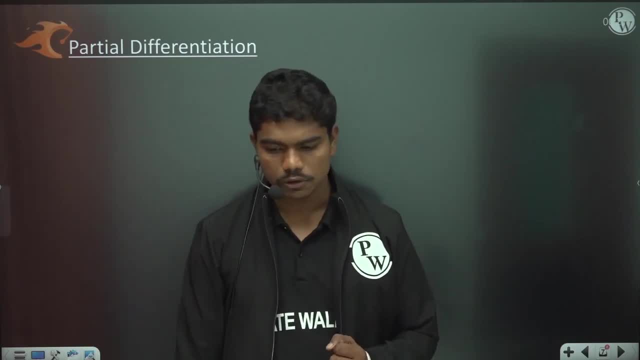 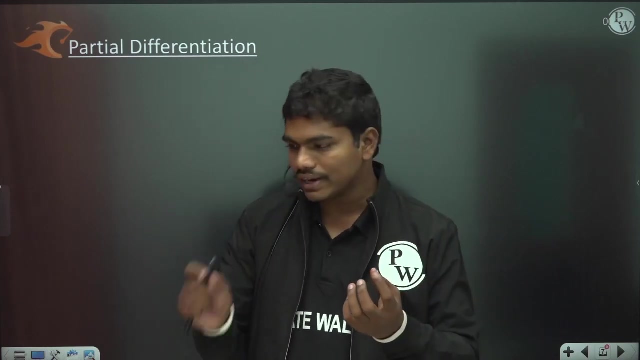 Why partial differentiation is very much important. Look, I'll tell you, Sorry. so, why partial differentiation is important. because differentiation basically tells you the change of quantity. Let us suppose if I write dy by dx, for example in single variables, that tells me when I change my x by some amount. 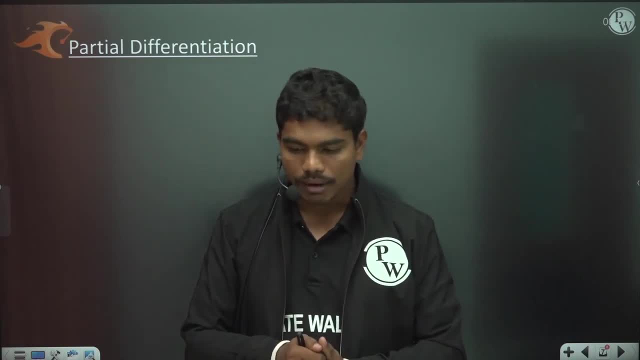 What is the change in my y? that? this is what it tells you. but even you come to multivariable functions. It's not easy for you to identify changes in all the directions simultaneously. Okay, So let us suppose if temperature is changing, pressure is changing, viscosity is changing, when all these things are changing simultaneously. 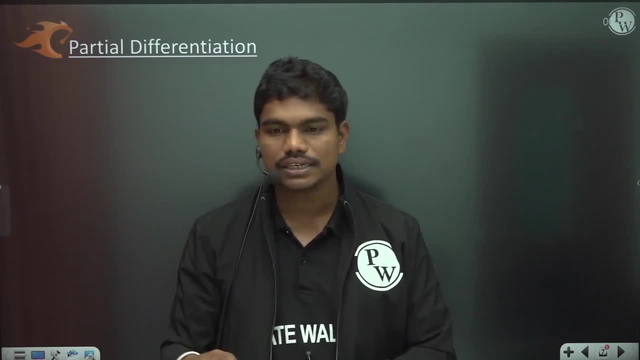 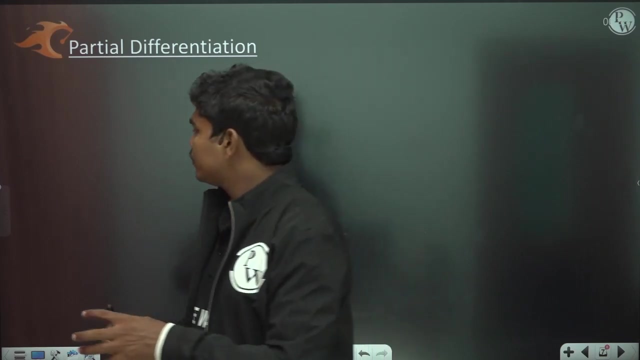 or some other parameters are changing Simultaneously, it's not easy for you to identify all the changes simultaneously. So for that reason, what we do, we will do. we will adapt some techniques, like we will differentiate Function with respect to some partial or terms, actually Okay. So now, if you see this partial differentiation, how we actually do this, if 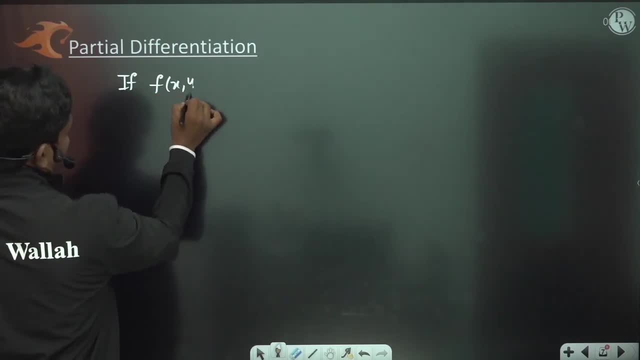 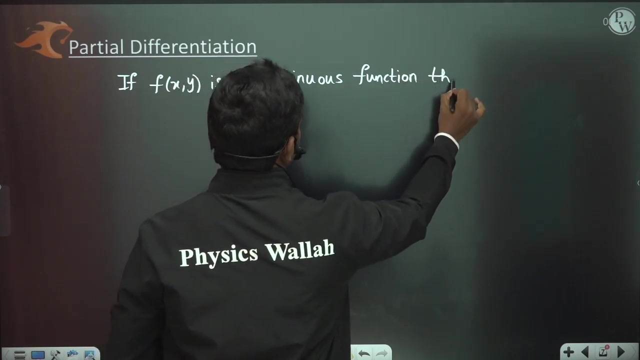 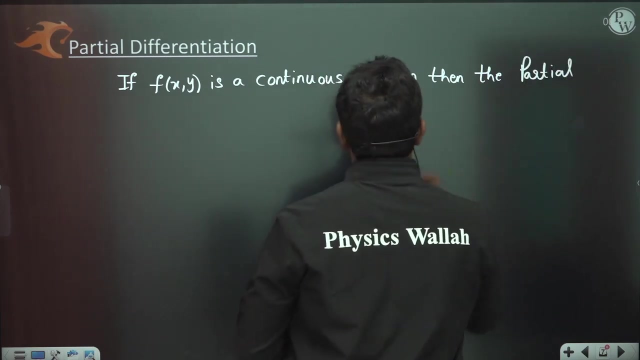 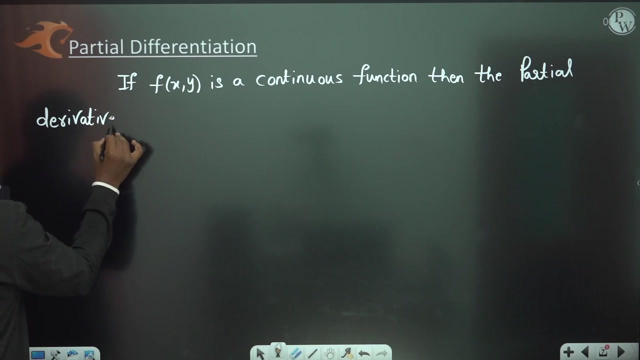 If F of X comma Y is a Continuous function. If F of X comma Y is a continuous function, Then The partial derivative of: Then the partial Derivative of F of X comma Y. then the partial derivative of F of X comma Y with respect to X, Then the partial derivative of F of X comma Y of f of x. 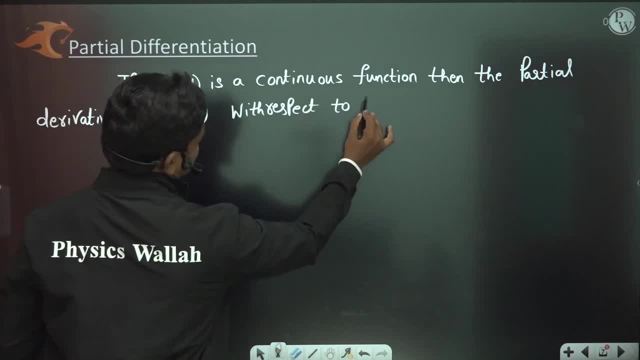 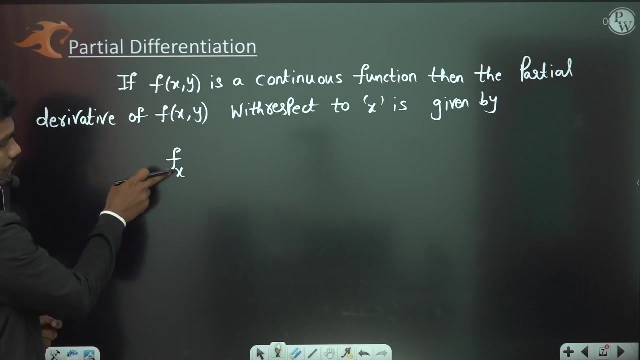 Then the partial derivative of F of x comma, F of x comma, f of x comma, which x minus x, X is given by X, is given by Pretty clear F, X, F, X. that denotation is normally like this: we denote F with a subscript. x means with differentiating this F with respect to X. or 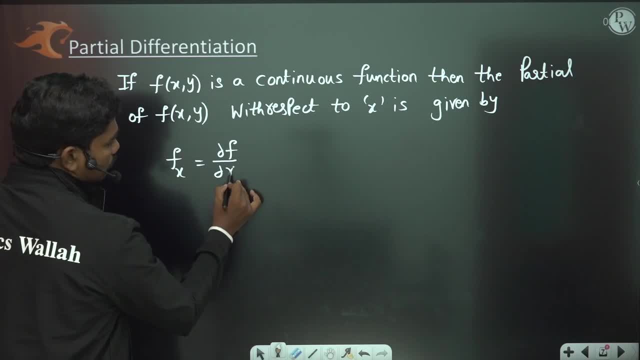 you will denote this has dou f by dou X. you know we'll write Dell for partial, inter partial. you know Differentials. so this can be called as del or do. okay, so in different books you have different notation: do f by do x. you can say so. 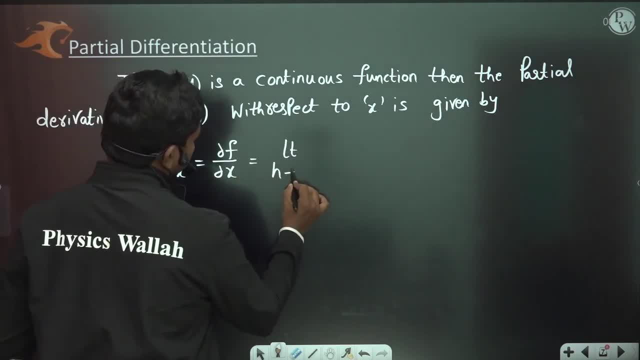 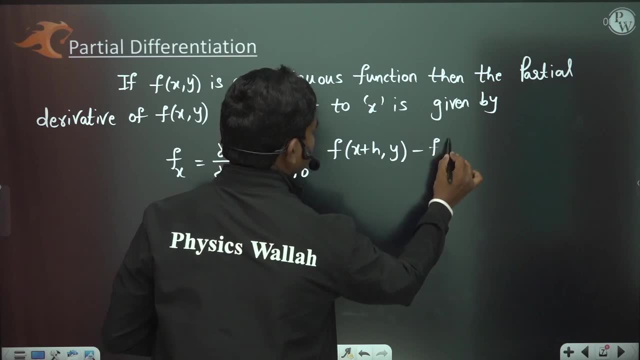 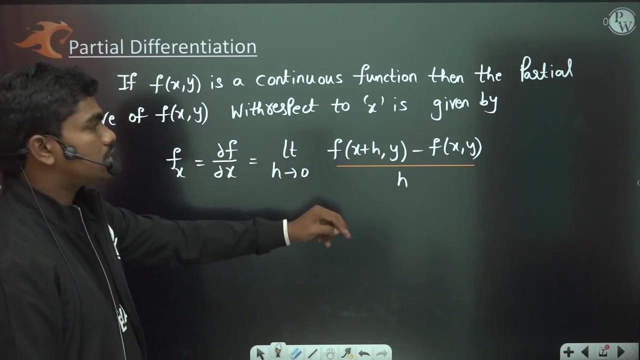 this is equal to limit. h tends to 0. f of x plus h comma y, minus f of x comma y, divided by h. actually okay. so if you see, divided by h is what you have. so basically what we are doing. we are assuming here, when you are differentiating partially with respect to x, you are changing only x here, correct? 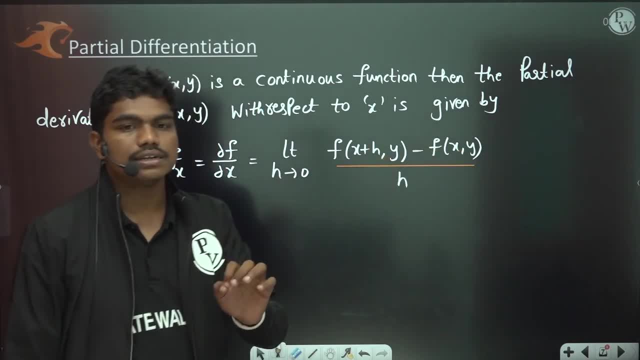 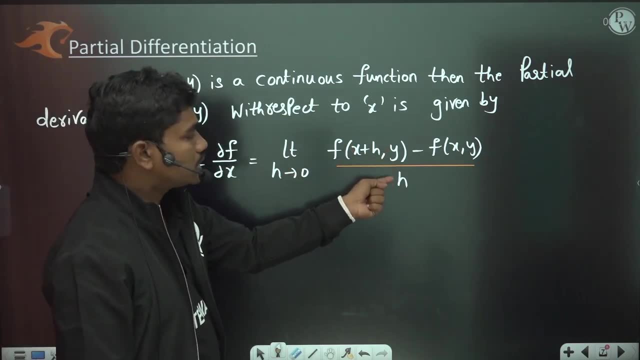 you are not changing y. y is same in both these cases means you are treating y as a constant in this definition, okay. and also we are changing. since this is differential terms, small terms, we have taken this. h is very small, so the difference between these two functions will. 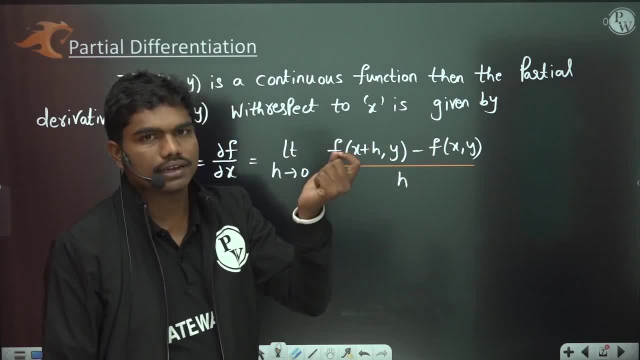 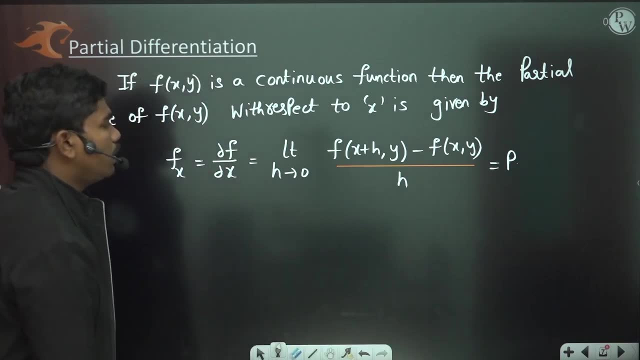 be very small, because the x coordinate is changing by very small amount, like in the previous case of differentiations. okay, sometimes this is also denoted with p. okay, we will, we'll see what is a y. we have different denoted with this, with the p in partial differential equations. okay, so this fx is given by this. 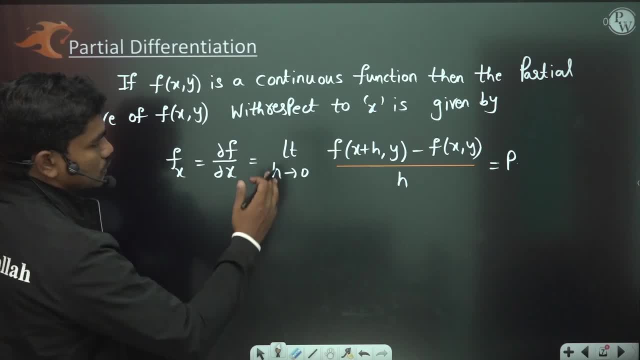 expression: do f by do x, which is equal to limit h tends to 0. f of x plus h, comma, y minus this value. but here we are assuming one thing: when you are differentiating with respect to x, you are treating y as constant. okay, now, similarly, similarly, partial derivative of partial derivative. 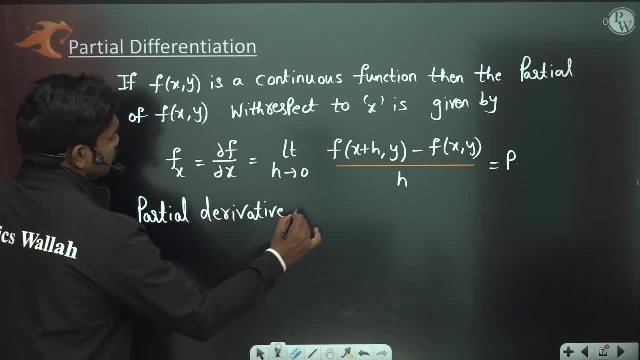 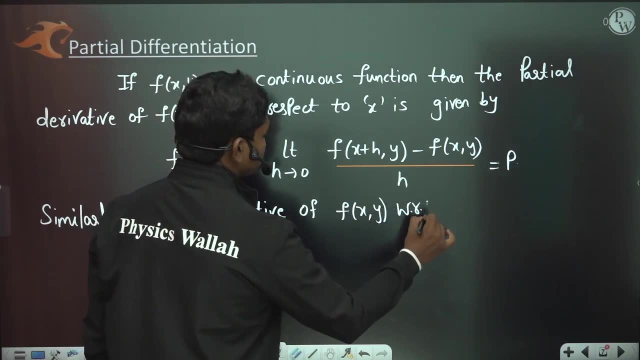 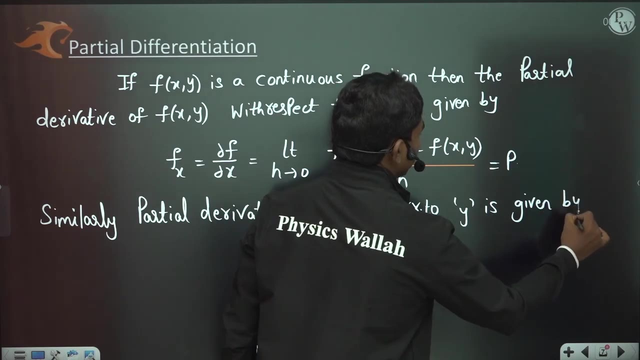 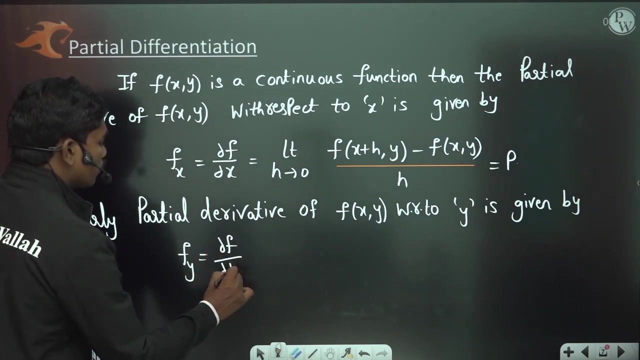 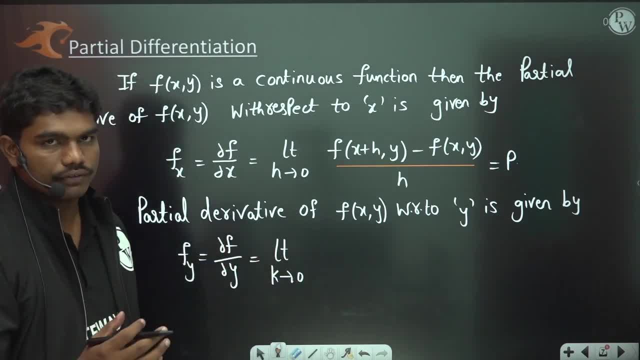 to 0. let us say now if you can pause the video for a moment. let us say if you can pause the video for a moment. let us say if you can pause the video for a second. and if you try to answer this second and if you try to answer this. 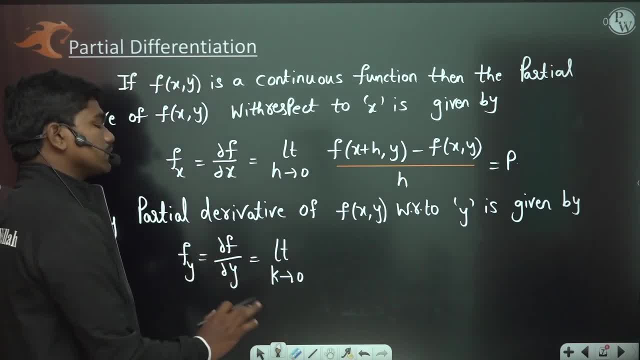 second, and if you try to answer this, you will get the answer okay. so if you see, you will get the answer okay. so if you see, you will get the answer okay. so if you see now you need to take x as a constant and y, now you need to take x as a constant and y. 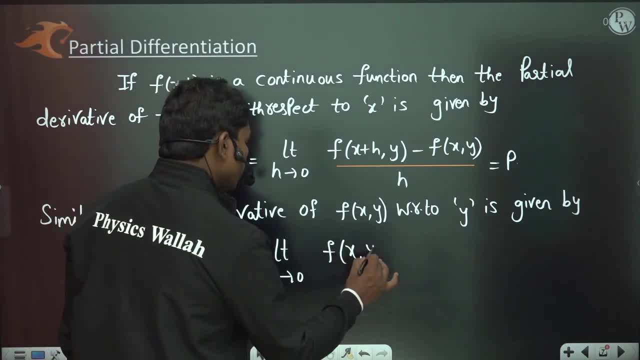 now you need to take x as a constant and y changes, correct, so we'll write f of x comma changes, correct, so we'll write f of x comma changes, correct, so we'll write f of x comma y plus k, minus f of x comma y, so we have. 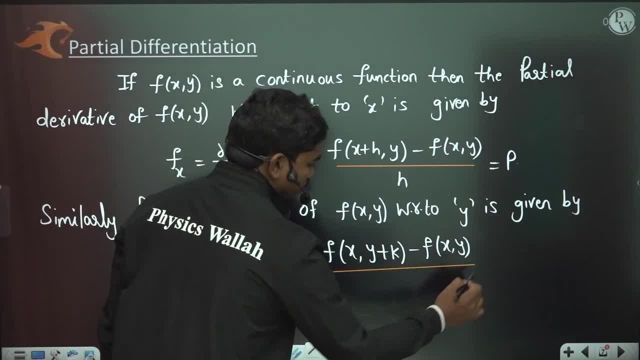 y plus k minus f of x comma y. so we have y plus k minus f of x comma y. so we have changed the y coordinate slightly, changed the y coordinate slightly, changed the y coordinate slightly. divided by h. divided by divided by h. divided by divided by h. divided by h: h. okay, sorry, k, we have taken k here, so 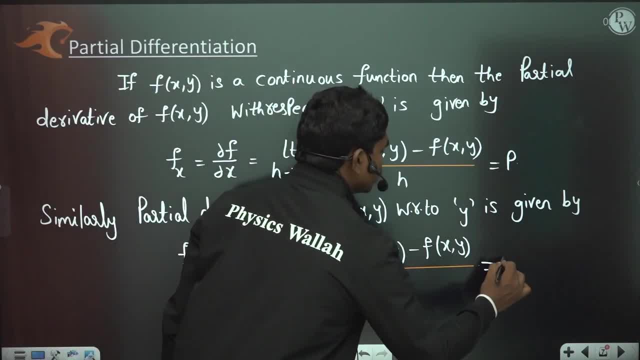 h h okay, sorry k, we have taken k here. so h h okay, sorry k, we have taken k here. so this is k. so this is also notated as q. this is k. so this is also notated as q. this is k. so this is also notated as q sometimes. okay, so first partial. 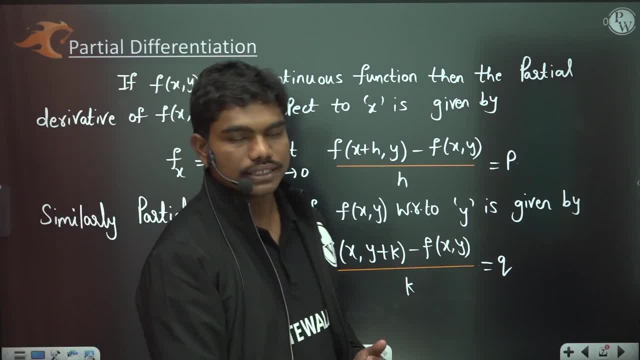 sometimes okay. so first partial, sometimes okay. so first partial differentiation of differentiation, of differentiation of f with respect to x is taken as p and f with respect to x is taken as p and f with respect to x is taken as p. and second, partial differentiation: we, second partial differentiation, we. 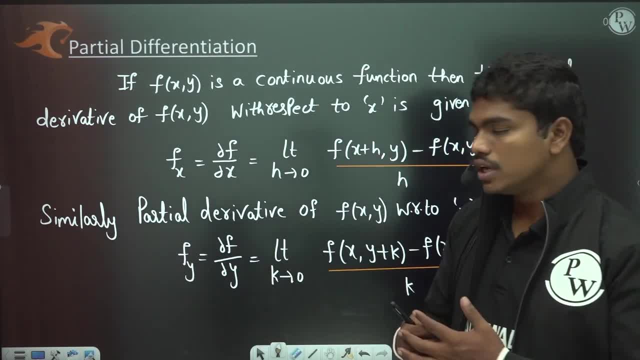 second partial differentiation: we generally, i mean the first partial again generally, i mean the first partial again generally, i mean the first partial again- with respect to y is taken as with respect to y is taken as with respect to y is taken as q. now, if you uh talk about one point here, q now, if you uh talk about one point here. q now, if you uh talk about one point here: how we actually calculate the total, how we actually calculate the total, how we actually calculate the total. change in f: okay, we have identified. change in f: okay, we have identified. 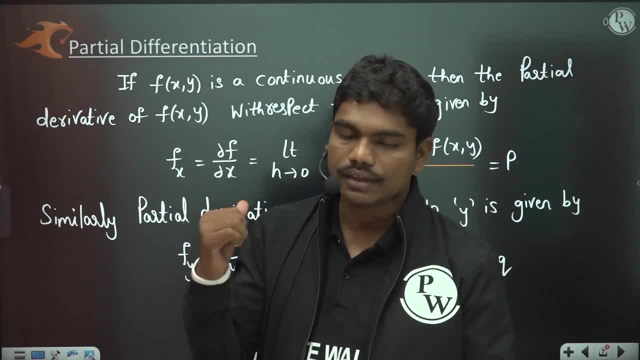 change in f. okay, we have identified partial change in f with respect to x, partial change in f with respect to x, partial change in f with respect to x, like fp, and we have also identified what like fp and we have also identified what like fp and we have also identified what is the partial change of f with respect. 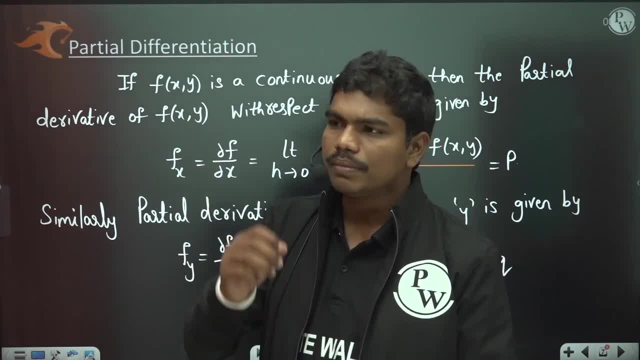 is the partial change of f with respect, is the partial change of f with respect to y. now how we actually calculate the to y. now how we actually calculate the to y. now how we actually calculate the total change. okay, because f is changing, total change. okay, because f is changing. 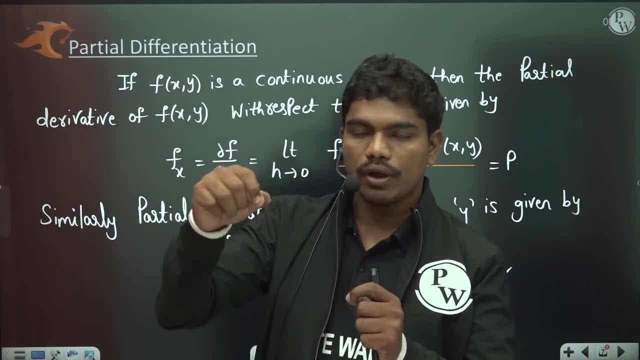 total change. okay, because f is changing in x and also y directions. now how we in x and also y directions. now how we in x and also y directions. now how we actually, if you change a point from one, actually, if you change a point from one, actually, if you change a point from one point to another, point in a two, 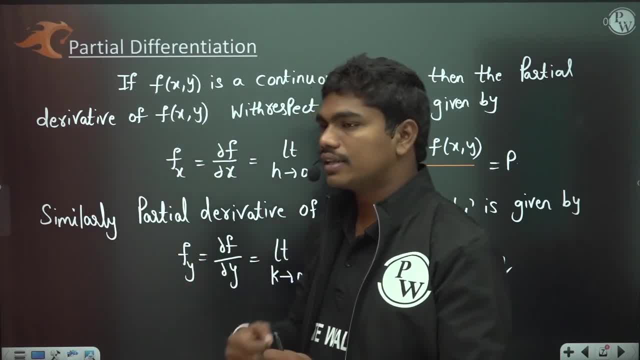 point to another point in a two point to another point in a two dimensional space. dimensional space, dimensional space, what or how we actually calculate the what, or how we actually calculate the what, or how we actually calculate the total change in f. so for that, we have total change in f. so for that we have. 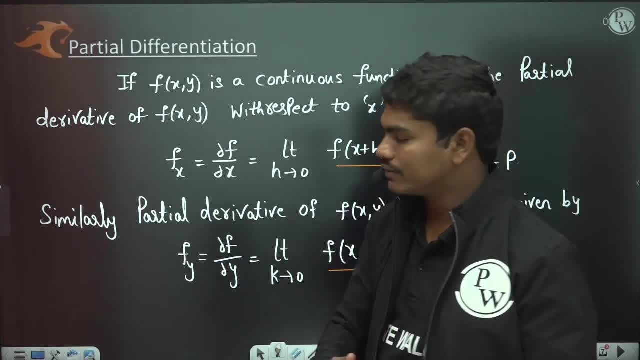 total change in f. so for that we have something called the, something called the, something called the chain rule of differentiation, or total chain rule of differentiation, or total chain rule of differentiation or total derivative. okay, so, if you see derivative, okay, so if you see derivative, okay, so, if you see, let us write chain rule of differentiation. 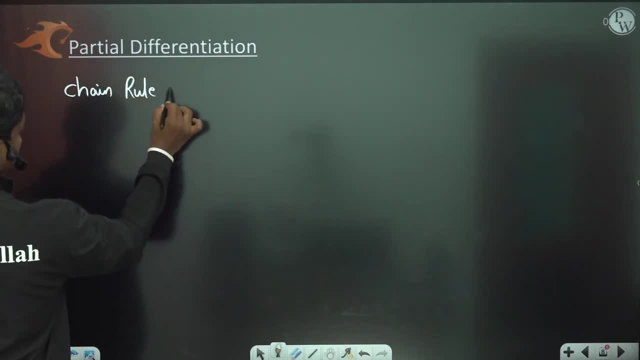 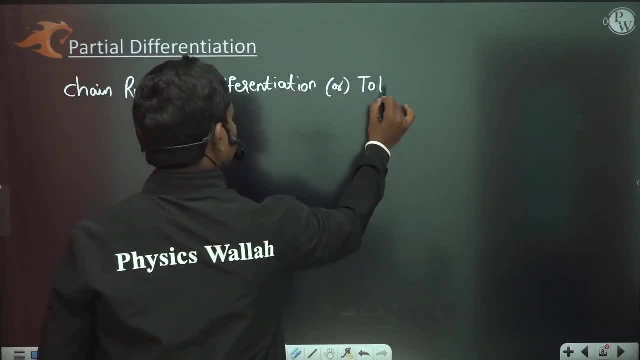 total derivative chain, rule of total derivative chain, rule of differentiation or total derivative differentiation, or total derivative differentiation or total derivative normally, when you talk about normally, when you talk about normally, when you talk about accelerations, all these things in fluid, accelerations, all these things in fluid. 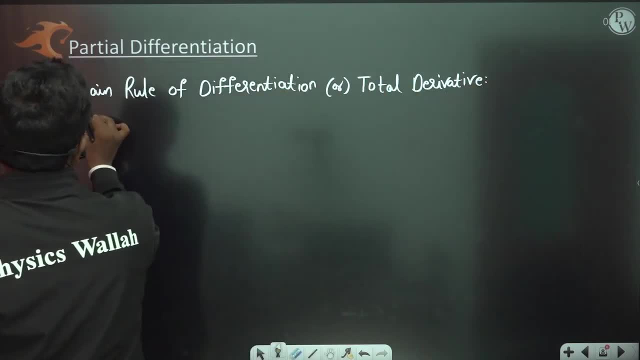 accelerations, all these things in fluid dynamics or fluid kinematics. you say you dynamics or fluid kinematics? you say you dynamics or fluid kinematics. you say you will get all these things, will get all these things, will get all these things. so chain rule of differentiation: 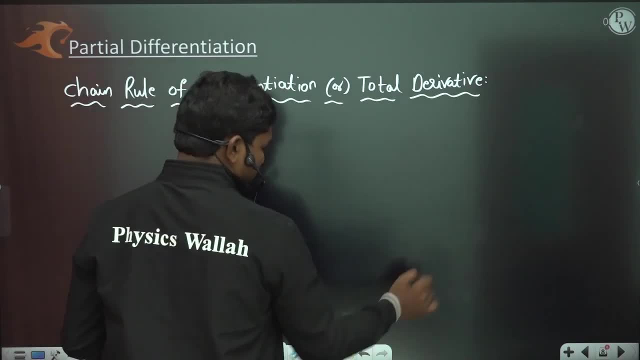 so chain rule of differentiation. so chain rule of differentiation. now let us see if. now let us see if. now let us see if f is some point. look, try to understand. f is some point. look, try to understand. f is some point. look, try to understand carefully here. 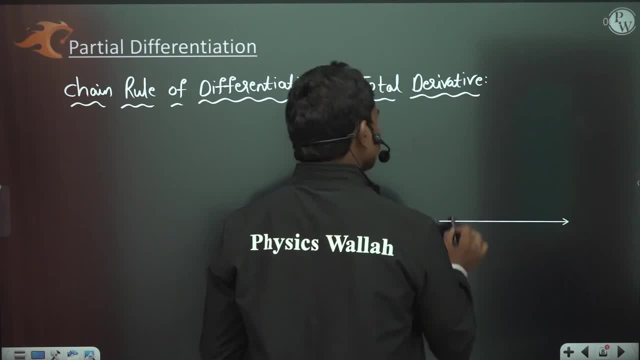 carefully here, carefully here. let us suppose: if this is the x, let us suppose if this is the x, let us suppose, if this is the x coordinate x direction basically, and this coordinate x direction basically, and this coordinate x direction basically, and this is y direction. okay, so, 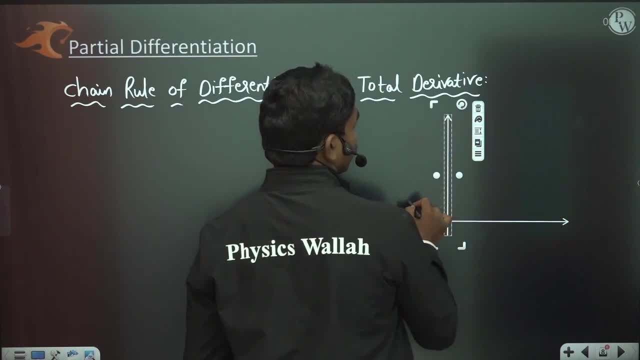 is y direction okay, so is y direction okay. so some y coordinate like this. okay. so it some y coordinate like this. okay. so it some y coordinate like this. okay. so it is some y coordinate like this. now, this is some y coordinate like this. now, this is some y coordinate like this. now, this is origin. 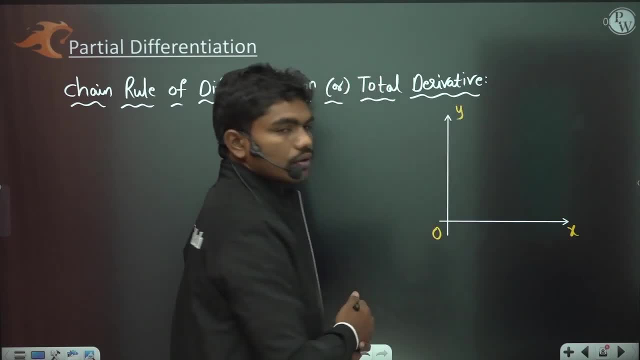 is origin. is origin? this is x and this is y, for example? okay, this is x and this is y, for example: okay, this is x and this is y. now let us suppose this is x and this is y. now, let us suppose this is x and this is y. now let us suppose initially you have your point here, for 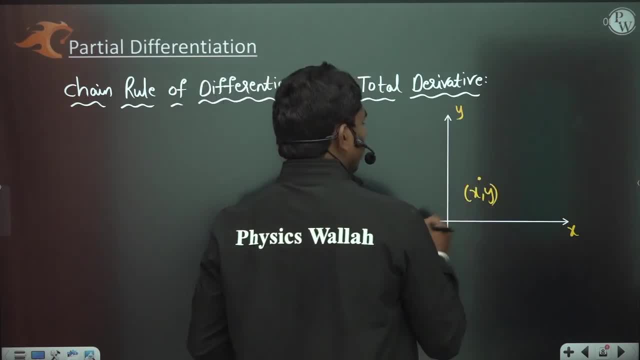 initially you have your point here, for initially you have your point here. for example: example: example: x comma y. now, when you change this point: x comma y. now, when you change this point x comma y. now, when you change this point from this location a from this location a. 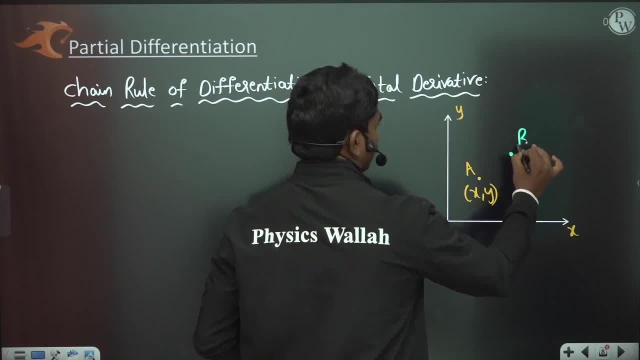 from this location a to some location b. let us say: to some location b. let us say: to some location b. let us say b. let us suppose this is the point some b. let us suppose this is the point some b. let us suppose this is the point some. this is x 1 y 1. this is x 2 y 2. let us 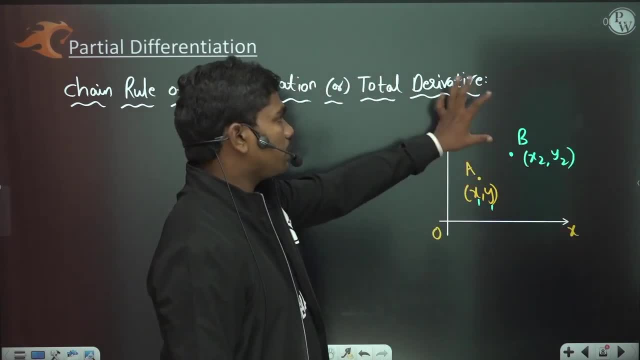 this is x 1 y 1, this is x 2 y 2. let us: this is x 1 y 1, this is x 2 y 2, let us say like this, say like this, say like this. now, let us suppose there is some. 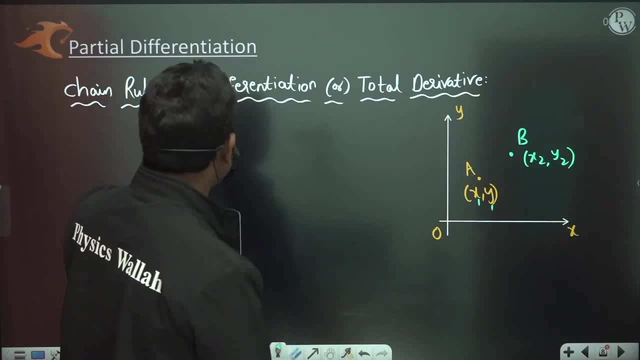 now, let us suppose there is some. now, let us suppose there is some temperature on this board. okay, so we are temperature on this board. okay, so we are temperature on this board. okay, so we are measuring the temperature at different measuring the temperature at different, measuring the temperature at different points on this board. and let us suppose points on this board. and let us suppose points on this board. and let us suppose this temperature on this board is as per. this temperature on this board is as per. this temperature on this board is as per: some function with respect to x, some function with respect to x. 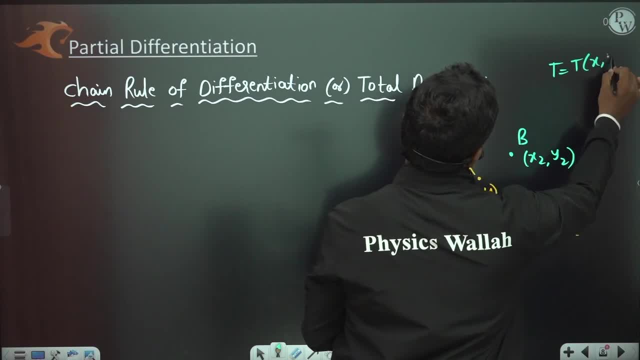 some function with respect to x. okay, so t is equal to some function of: okay, so t is equal to some function of: okay, so t is equal to some function of x. comma y- okay, depending upon the heat. comma y- okay, depending upon the heat. comma y- okay, depending upon the heat generated. whatever, you can see the 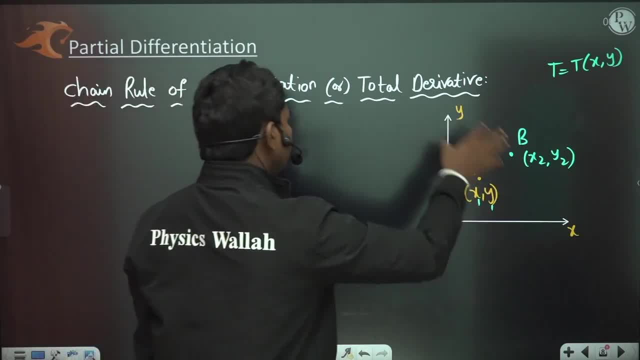 generated, whatever you can see, the generated, whatever you can see the temperature at different locations on temperature at different locations, on temperature at different locations on this board, has different values, which this board has different values, which this board has different values, which are actually governed by one relation. 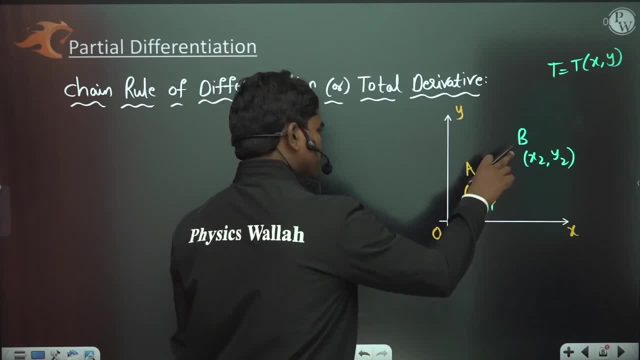 are actually governed by one relation, are actually governed by one relation. let us suppose now. if you want to observe, let us suppose now. if you want to observe, let us suppose now. if you want to observe the temperature, let us suppose these two. the temperature, let us suppose these two. 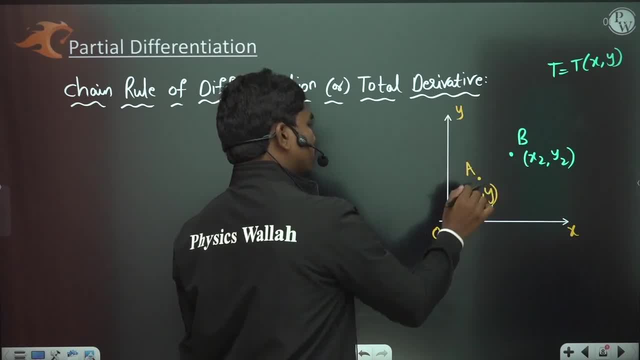 the temperature. let us suppose these two points are very close to each other. just points are very close to each other. just points are very close to each other. just for your understanding, i have separated, for your understanding, i have separated. for your understanding, i have separated them. but let us suppose they are almost. 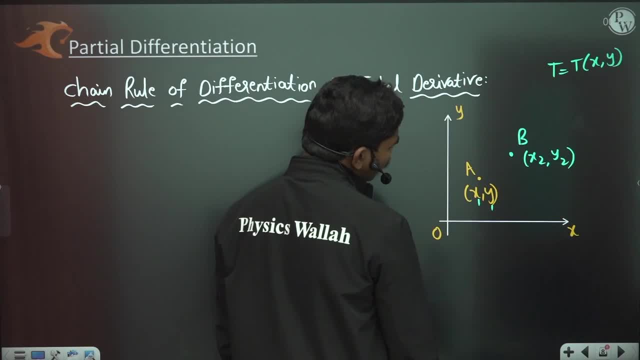 them, but let us suppose they are almost them, but let us suppose they are almost side by side. okay. so now, if you see side by side, okay. so now, if you see side by side, okay. so now, if you see, if you want to calculate the temperature, if you want to calculate the temperature. 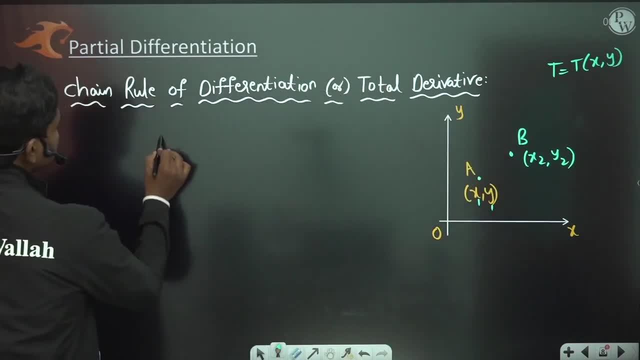 if you want to calculate the temperature difference between these two locations, difference between these two locations, difference between these two locations: dt: you know t is actually equal to t of dt. you know t is actually equal to t of dt. you know t is actually equal to t of x. comma, y, cut. so if you want to, 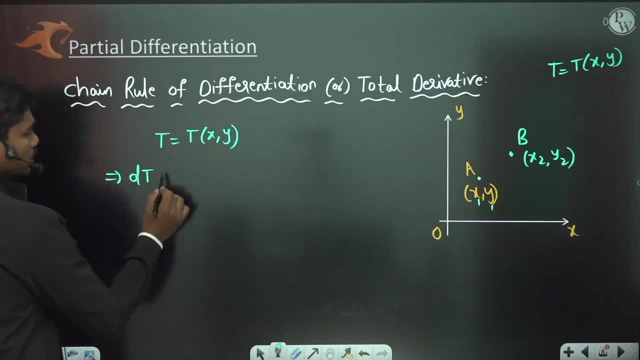 x comma, y, cut. so if you want to x comma, y, cut. so if you want to calculate dt means, if you want to calculate dt means, if you want to calculate dt means, if you want to calculate change in temperature, what you calculate, change in temperature, what you. 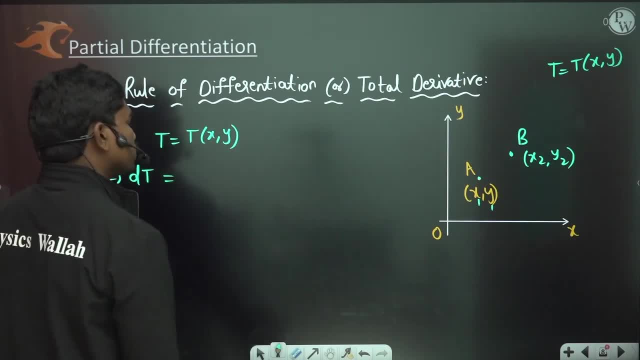 calculate change in temperature. what you will do is you will actually sum up all calculate change in temperature. what you will do is you will actually sum up all calculate change in temperature. what you will do is you will actually sum up all the changes. okay, so you know, dou t by dou x. 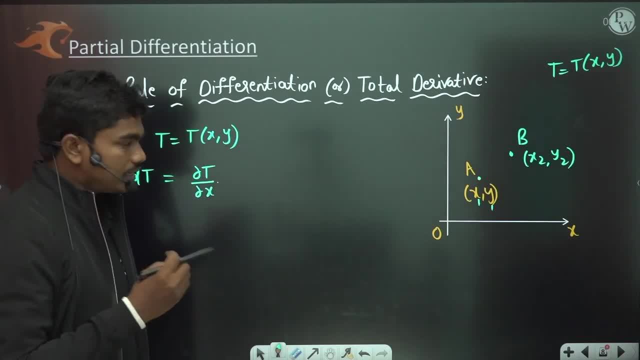 the changes. okay, so you know dou t by dou x the changes. okay, so you know dou t by dou x. this quantity, if you take this, is nothing. this quantity, if you take this, is nothing. this quantity, if you take this is nothing. but you know the weight of change of t in. 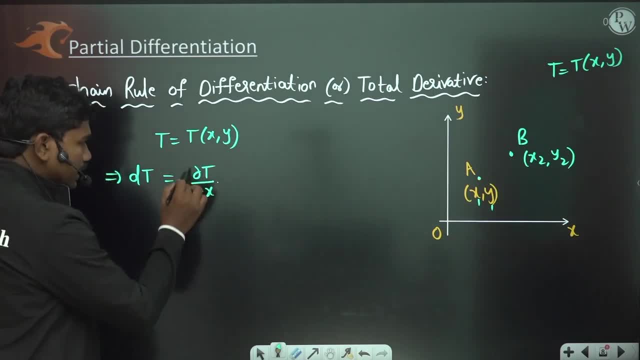 but you know the weight of change of t in, but you know the weight of change of t in the x direction. okay. so, whenever you the x direction, okay, so whenever you the x direction, okay, so, whenever you are dividing this del t by del x, this is: 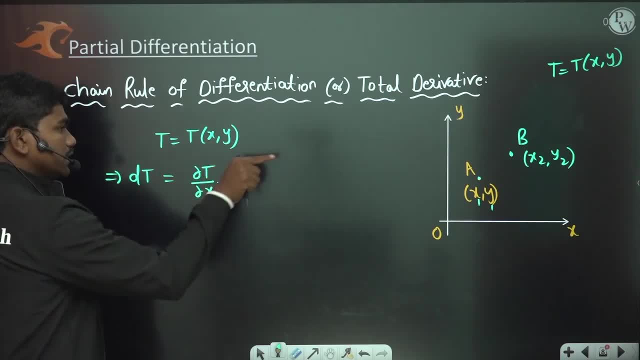 are dividing this del t by del x. this is: are dividing this del t by del x. this is actually giving you the temperature, actually giving you the temperature, actually giving you the temperature. change for one unit of change in x. change for one unit of change in x. 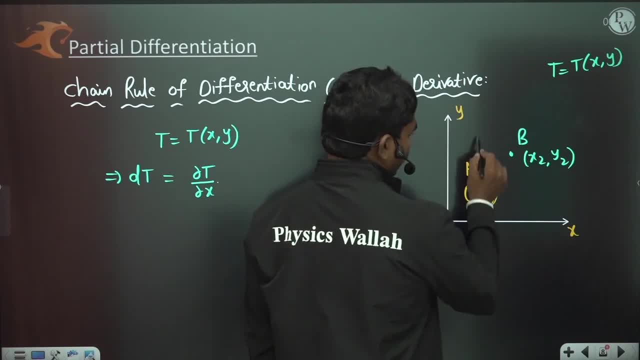 change for one unit of change in x, direction correct. so, if you see, let us direction correct. so, if you see, let us direction correct. so if you see, let us suppose, between these two points, the suppose between these two points, the suppose between these two points, the total change in x, the total, 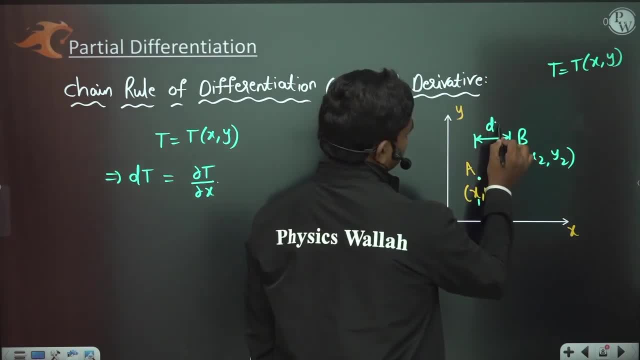 change in x is dx. let us suppose if this change in x is dx. let us suppose if this change in x is dx. let us suppose if this is dx. so you know, for one unit of the dx is dx. so you know, for one unit of the dx. 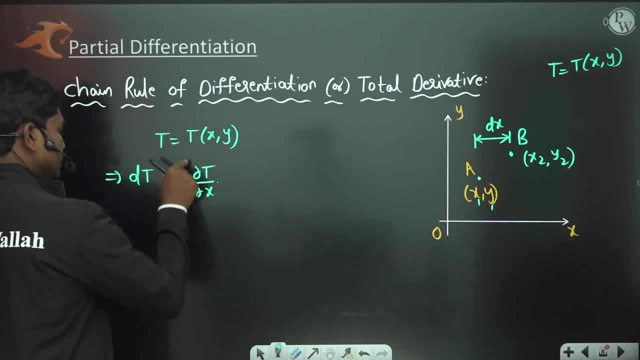 is dx. so you know, for one unit of the, dx means the. for one unit, change in x means the. for one unit, change in x means the. for one unit change in x direction, the temperature change is del t direction, the temperature change is del t direction, the temperature change is del t. so for dx change, what will be the change? 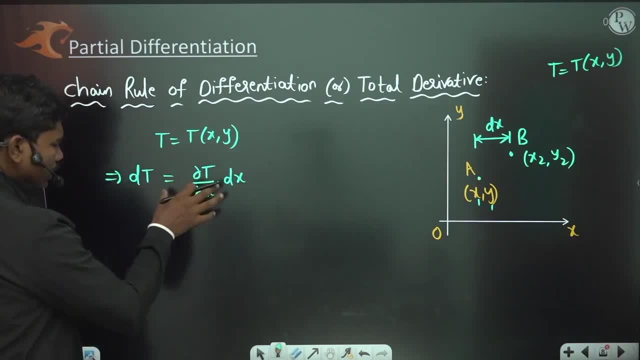 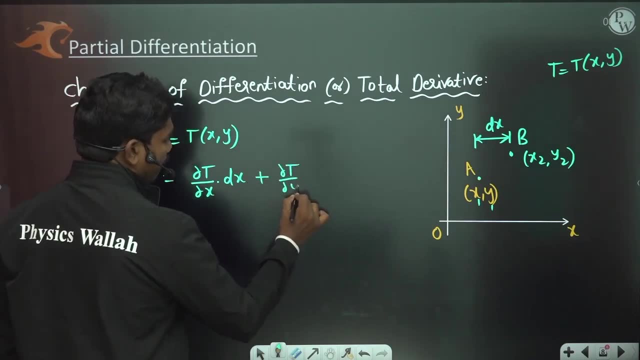 so for dx change, what will be the change? so for dx change, what will be the change? less do t by y, this is, let us suppose. if less do t by y, this is, let us suppose. if less do t by y, this is, let us suppose. if this is the temperature change by unit. 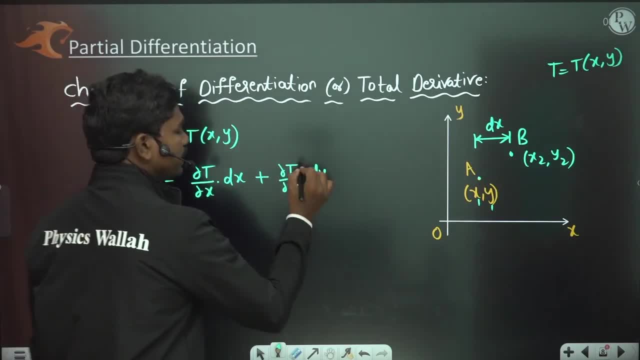 this is the temperature change by unit. this is the temperature change by unit. dimension in y direction. so this has to dimension in y direction. so this has to dimension in y direction. so this has to be multiplied by dy. if this point of be multiplied by dy, if this point of 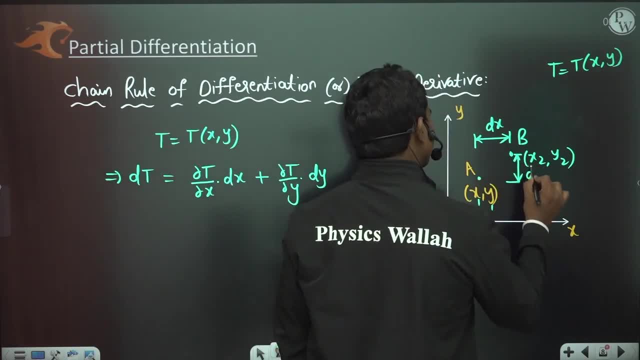 be multiplied by dy. if this point of separation between these two is dy, separation between these two is dy, separation between these two, is dy actually here? okay, so let us suppose if actually here. okay, so let us suppose if actually here. okay, so let us suppose if this is dy, then the temperature variation. 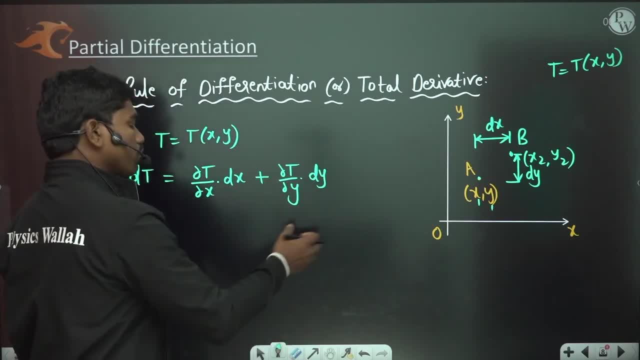 this is dy. then the temperature variation: this is dy. then the temperature variation because of the change in y direction, is because of the change in y direction, is because of the change in y direction. is amount of dy, so temperature change in y. amount of dy, so temperature change in y. 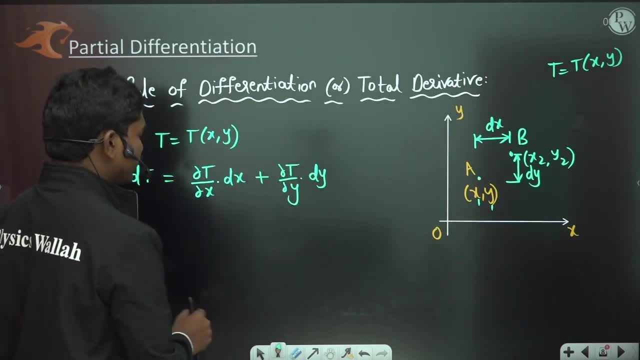 amount of dy. so temperature change in y direction per unit. change in y multiplied direction per unit. change in y multiplied direction per unit. change in y multiplied with total change in y direction. so if with total change in y direction, so if with total change in y direction. so if you see, this is nothing, but do t by do. 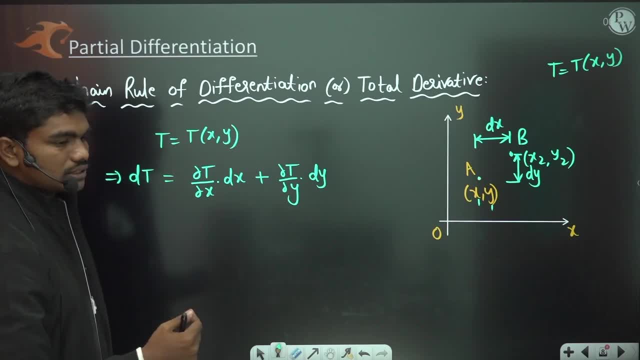 you see, this is nothing but do t by do. you see, this is nothing but do t by do x into dx, plus do t by do y into dy, so x into dx, plus do t by do y into dy, so x into dx, plus do t by do y into dy. so this is how we actually calculate the. 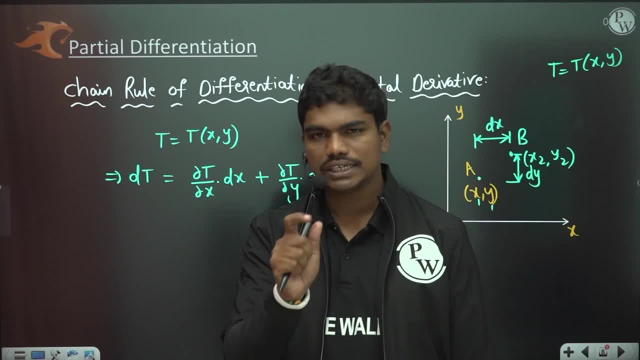 this is how we actually calculate the. this is how we actually calculate the total change in the temperature, between total change in the temperature, between total change in the temperature, between those two close points. of course DT is those two close points. of course DT is those two close points. of course DT is very small actually, so that's why we 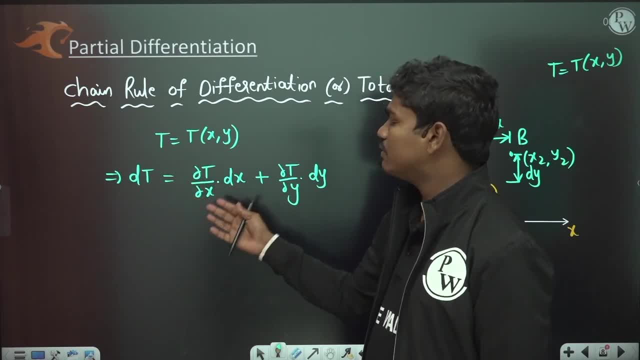 very small actually. so that's why we- very small actually. so that's why we actually calculate this using this. actually calculate this using this. actually calculate this using this formulation that DT is equal to do t. by formulation that DT is equal to do t. by formulation that DT is equal to do t by do x into dx, plus do t by do y into dy. 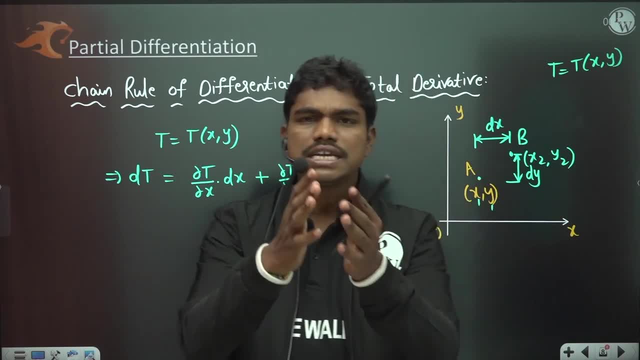 do x into dx plus do t by do y into dy, do x into dx plus do t by do y into dy. so basically what we are considering is so basically what we are considering is. so basically what we are considering is: let us suppose if a function is, 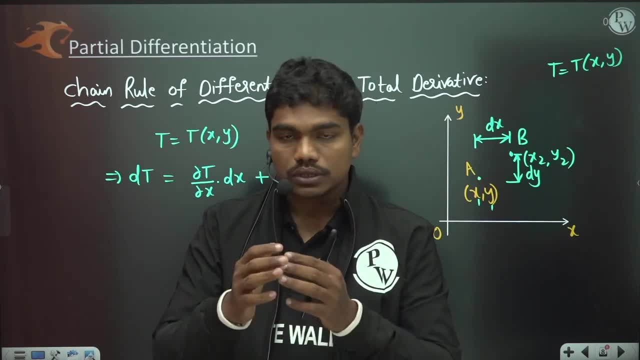 let us suppose if a function is. let us suppose if a function is depending on certain number of, depending on certain number of, depending on certain number of independent variables- okay, so then, what independent variables? okay, so then, what independent variables? okay, so then, what we are doing? we are trying to calculate. 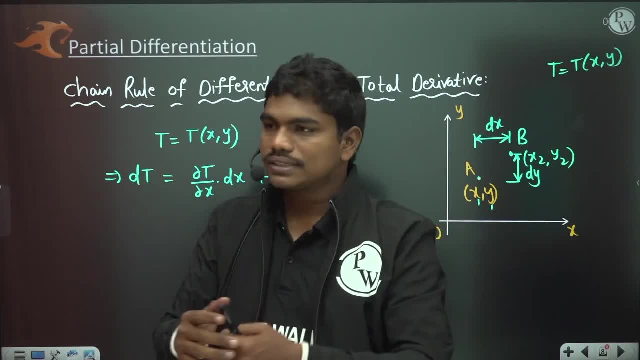 we are doing, we are trying to calculate, we are doing, we are trying to calculate changes due to each and every quantity, changes due to each and every quantity, changes due to each and every quantity. okay, so, let us suppose if I take. okay, so let us suppose if I take. 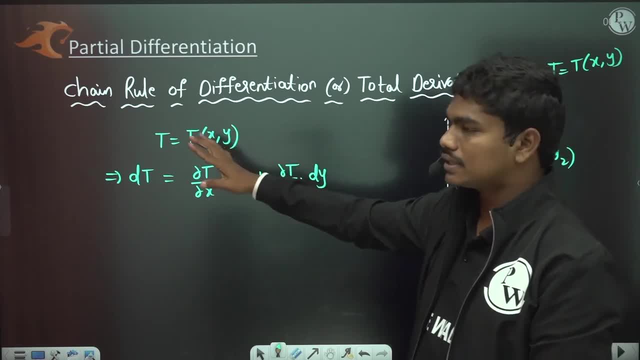 okay, so let us suppose, if I take temperatures depending upon pressure, and temperatures depending upon pressure, and temperatures depending upon pressure and volume, pressure and volume, let us volume pressure and volume. let us volume pressure and volume. let us suppose this is one simple example. then, suppose this is one simple example, then. 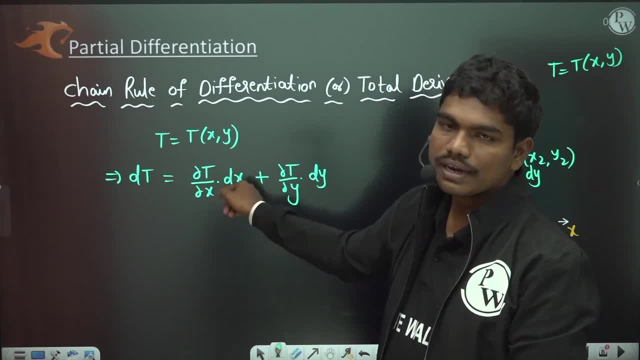 suppose this is one simple example, then you will like to change in temperature. you will like to change in temperature. you will like to change in temperature is equal to do t by do P into DP means is equal to do t by do P into DP means is equal to do t by do P into DP means. change in temperature because of the. 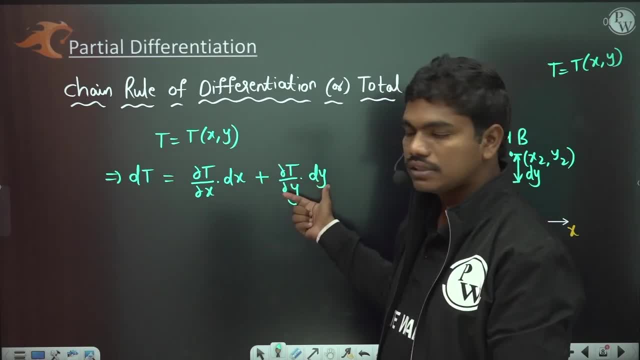 change in temperature because of the change in temperature, because of the change in pressure quantity, plus change in change in pressure quantity, plus change in change in pressure quantity, plus change in temperature due to change in volume temperature, due to change in volume temperature, due to change in volume quantity. that's how, basically, we'll. 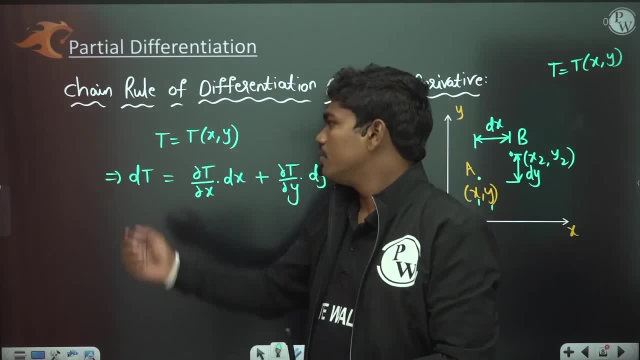 quantity. that's how basically we'll quantity, that's how basically we'll consider the two changes and we'll consider the two changes and we'll consider the two changes and we'll actually sum up them so that we'll get actually sum up them, so that we'll get. 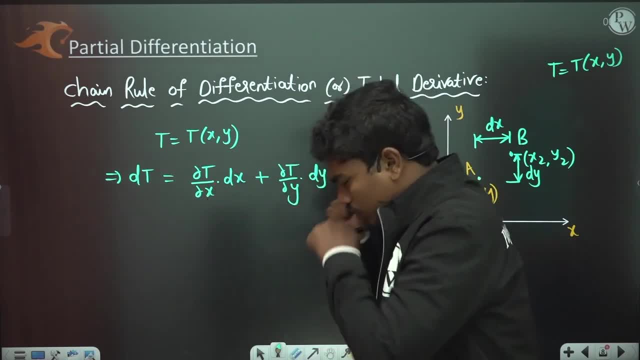 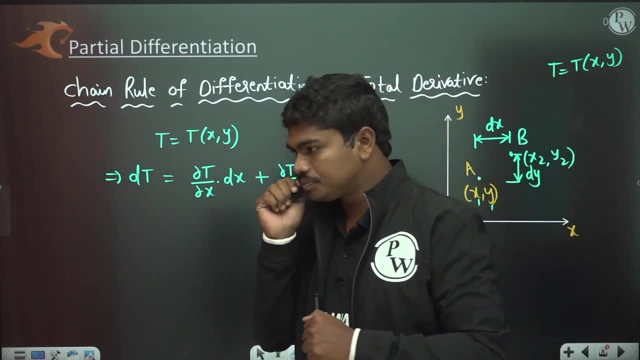 actually sum up them so that we'll get the total changes okay. so now this is: yeah, I'm sorry, so look here, so see here. yeah, I'm sorry, so look here, so see here. yeah, I'm sorry, so look here, so see here. so if you write this quantity, okay. 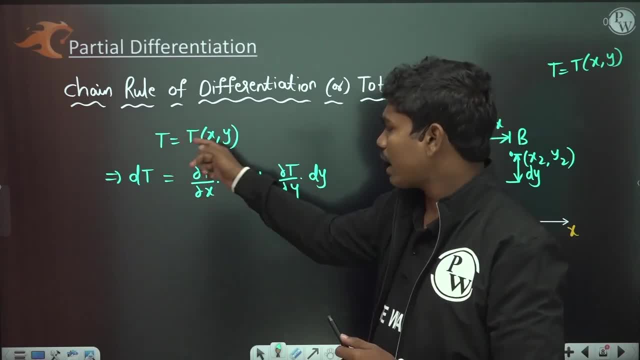 so if you write this quantity, okay, so if you write this quantity, okay. so the chain rule of math differentiation, the chain rule of math differentiation, the chain rule of math differentiation is mathematically this: basically: if you is mathematically this, basically. if you is mathematically this: basically, if you have a function, if you differentiate it. 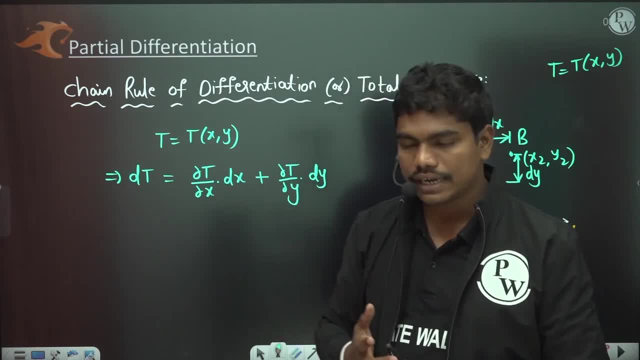 have a function if you differentiate it. have a function. if you differentiate it. you will get this expression. but what you will get this expression, but what you will get this expression, but what this expression is physically telling you. this expression is physically telling you. this expression is physically telling you. this expression is telling you that we 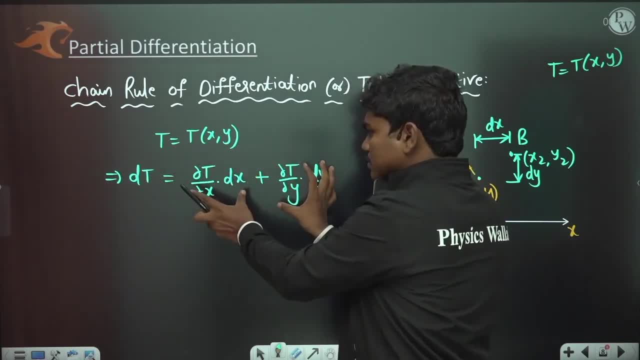 this expression is telling you that we- this expression is telling you that we are actually considering the changes of, are actually considering the changes of, are actually considering the changes of. this T has two different quantities. this T has two different quantities. this T has two different quantities because it's on two variables, so as two 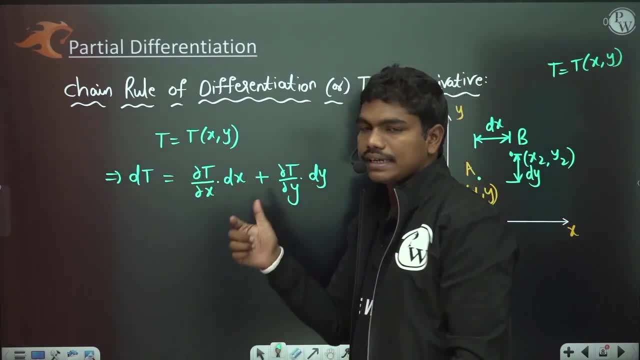 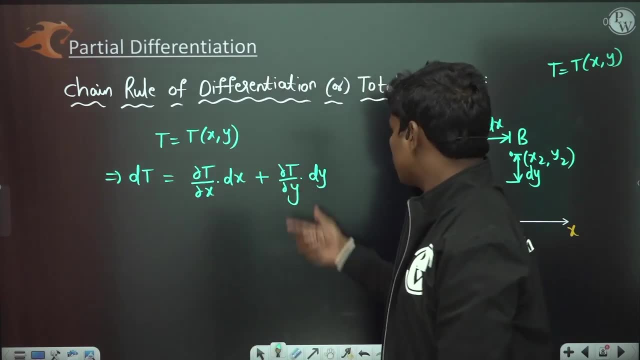 because it's on two variables, so as two. because it's on two variables, so as two. these results: okay, now I'll give you these results. okay, now I'll give you these results. okay, now I'll give you some quick examples on how to calculate. some quick examples on how to calculate. 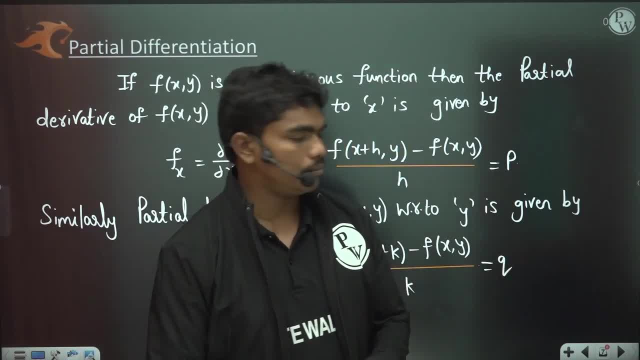 some quick examples on how to calculate partial differentiations. okay, it's just partial differentiations. okay, it's just partial differentiations. okay, it's just like a review, but again it will help you like a review, but again it will help you like a review, but again it will help you out. okay, so let us see, let us talk about. 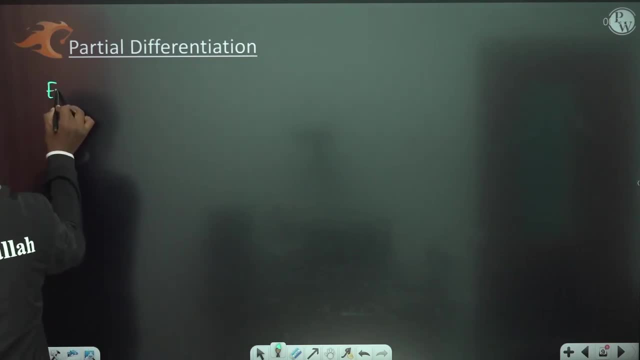 out. okay, so let us see, let us talk about out. okay, so let us see, let us talk about some example, so example. if you take this some example, so example. if you take this some example, so example. if you take this example, look up, for example, let us take: 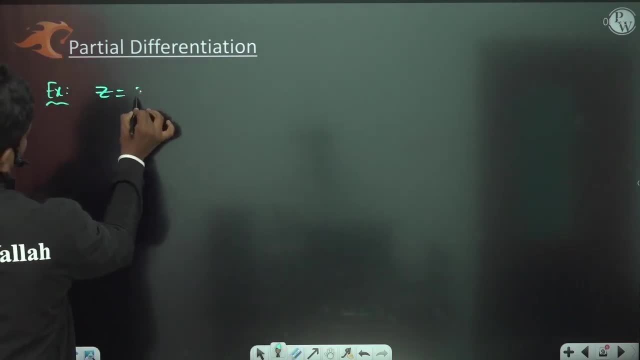 example. look up, for example. let us take example. look up, for example. let us take one function straight away: is that is one function straight away? is that is one function straight away? is that is equal to, equal to? equal to x cube plus 3x square y minus 3 x y. 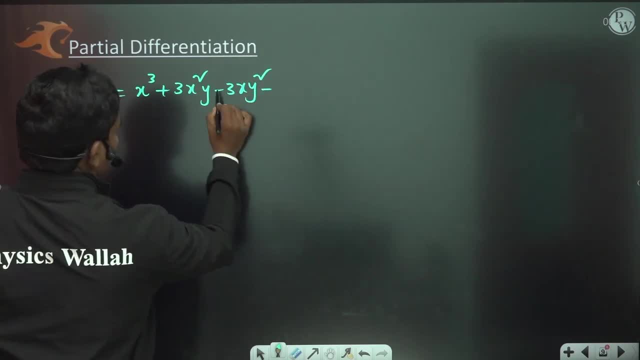 x cube plus 3 x square y minus 3 x y x cube plus 3 x square y minus 3 x y square. my okay, let's take. I say okay, square. my okay, let's take. I say okay, square. my okay, let's take. I say okay, anything is fine, it need not be exactly. 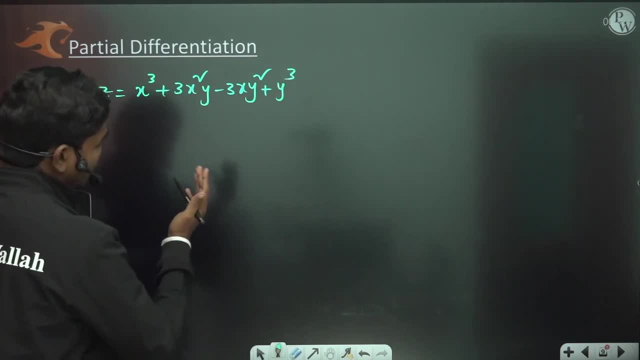 anything is fine. it need not be exactly anything is fine, it need not be exactly the same thing. so plus y cube, let us say the same thing. so plus y cube, let us say the same thing. so plus y cube, let us say: okay, normally, if you want to add this as: 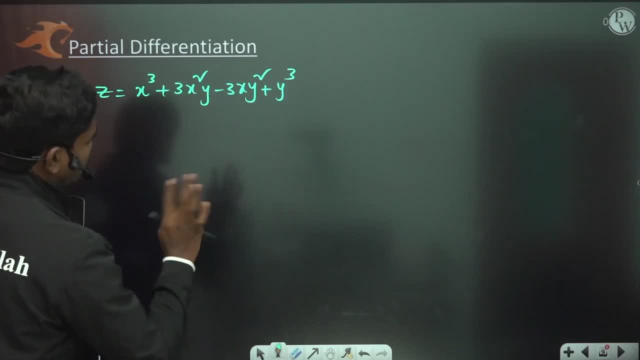 okay, normally, if you want to add this as: okay, normally, if you want to add this as x minus y whole cube, you change the plus x minus y whole cube. you change the plus x minus y whole cube. you change the plus and minus signs. but right now, let us. 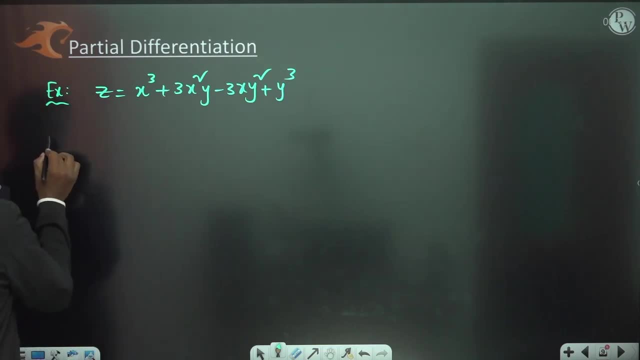 and minus signs, but right now, let us. and minus signs, but right now, let us suppose this is some function. okay, suppose this is some function. okay, suppose this is some function. okay. example: now, if you want to calculate P, example, now, if you want to calculate P. example: now, if you want to calculate P, which is, does that by do X? now, how you. 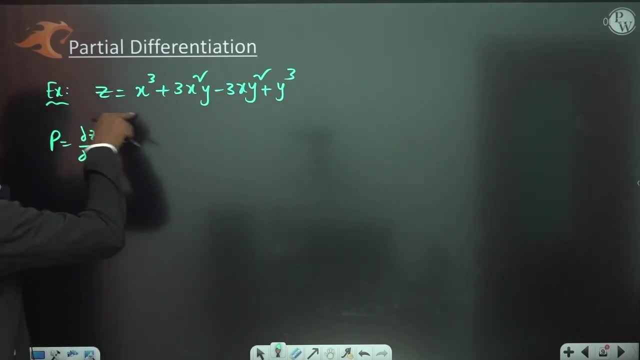 which is: does that by do X, now how you? which is: does that by do X, now how you will calculate this? does it better? X will calculate this. does it better? X will calculate this. does it better? X quantity? you need to differentiate this quantity. you need to differentiate this. 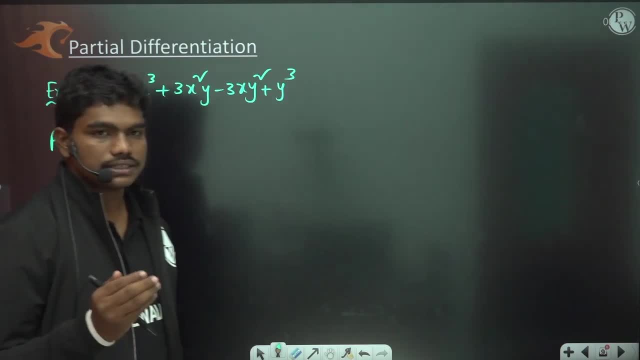 quantity. you need to differentiate this function partially with respect to X and function partially with respect to X and function partially with respect to X, and you know when you are doing partial, you know when you are doing partial, you know when you are doing partial differentiation with respect to one. 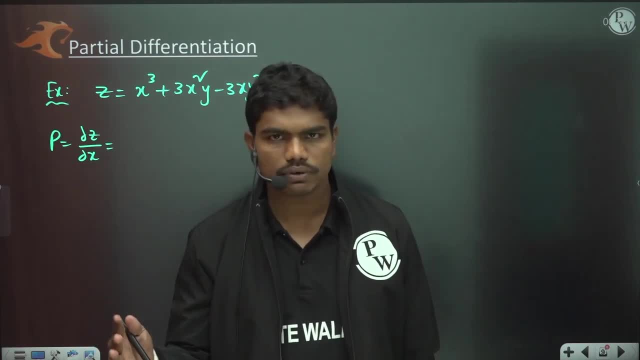 differentiation with respect to one, differentiation with respect to one variable. you treat all the other variables variable. you treat all the other variables variable. you treat all the other variables as constants. correct. that's what we have as constants. correct. that's what we have as constants. correct. that's what we have seen, basically in two variables. when I'm 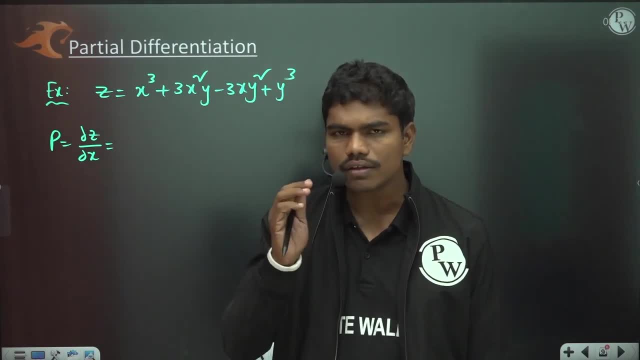 seen basically in two variables. when I'm seen basically in two variables, when I'm defining partial derivatives, what I have defining partial derivatives, what I have defining partial derivatives, what I have taken, when I am taking writing the taken, when I am taking writing the taken, when I am taking writing the definition for do F by do X, I didn't 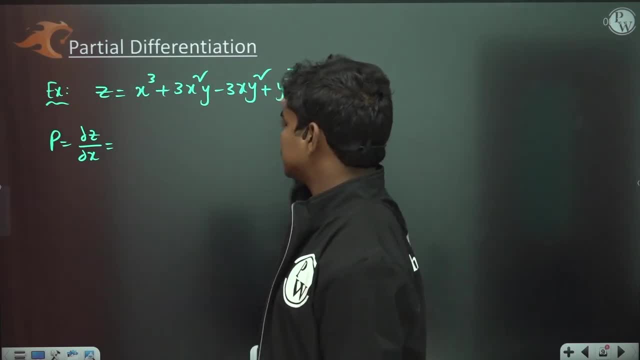 definition for do F by do X. I didn't definition for do F by do X. I didn't mention any changes in Y. so like that. if mention any changes in Y. so like that. if mention any changes in Y. so like that. if I want to differentiate this function. 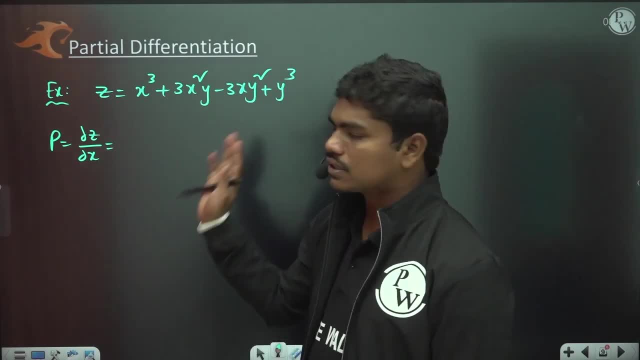 I want to differentiate this function. I want to differentiate this function with respect to X. don't take any changes with respect to X. don't take any changes with respect to X. don't take any changes in Y, which means Y, T, 2i as a constant. 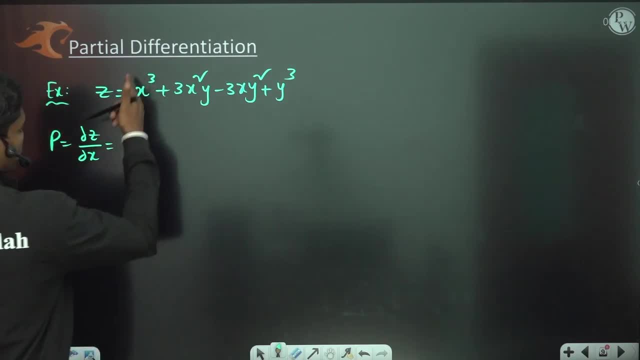 in Y, which means Y T 2i as a constant, in Y, which means Y T 2i as a constant. okay, now, let us differentiate that. so okay, now, let us differentiate that. so okay, now, let us differentiate that. so differentiation of the X square, I mean. 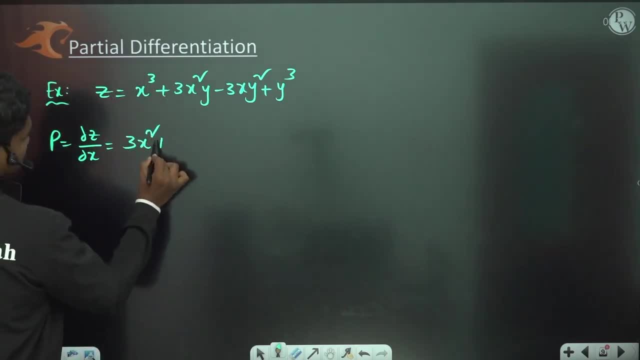 differentiation of the X square. I mean differentiation of the X square. I mean X cube is actually the X square plus now. X cube is actually the X square plus now. X cube is actually the X square plus now. out of this term, this T is a constant Y. 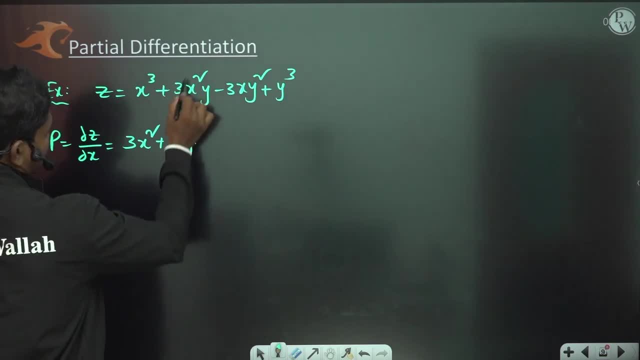 out of this term, this T is a constant Y. out of this term, this T is a constant Y also. you're reading as constant, so T Y also. you're reading as constant, so T Y also. you're reading as constant, so T Y is a constant. into differentiation of. 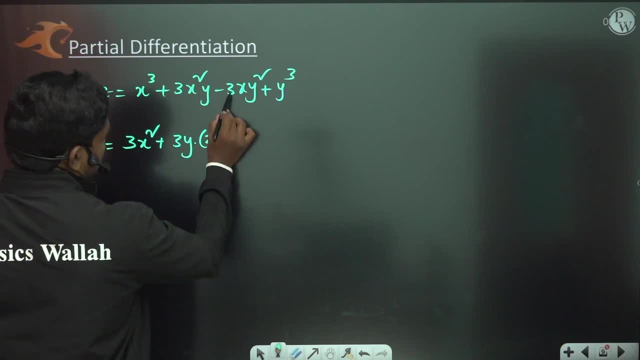 is a constant into differentiation of is a constant into differentiation of this X square. 2x minus this T is a. this X square 2x minus this T is a. this X square 2x minus this T is a constant. Y square is also constant, so 3. 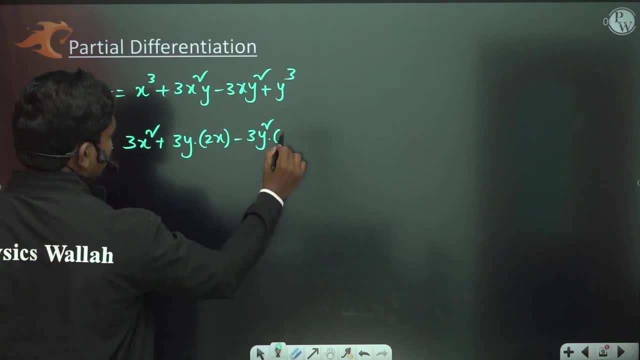 constant Y square is also constant. so 3 constant Y square is also constant. so 3 Y square into differentiation of this X. Y square into differentiation of this X. Y square into differentiation of this X with respect to X is 1 plus now Y is a. 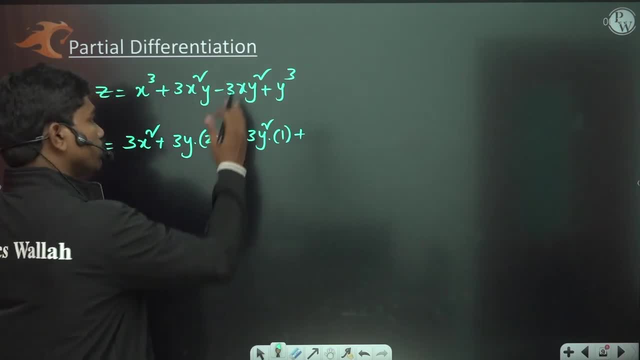 with respect to X is 1 plus now Y is a. with respect to X is 1 plus now Y is a constant. if I use the constant of IQ is constant. if I use the constant of IQ is constant. if I use the constant of IQ is also constant. so differentiation of a. 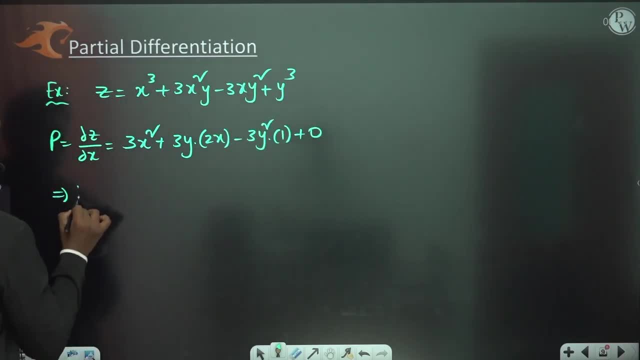 also constant. so differentiation of a also constant. so differentiation of a. constant is 0. okay, so that's how you'll. constant is 0: okay, so that's how you'll. constant is 0. okay, so that's how you'll get. P is equal to dou Z by dou X, which. 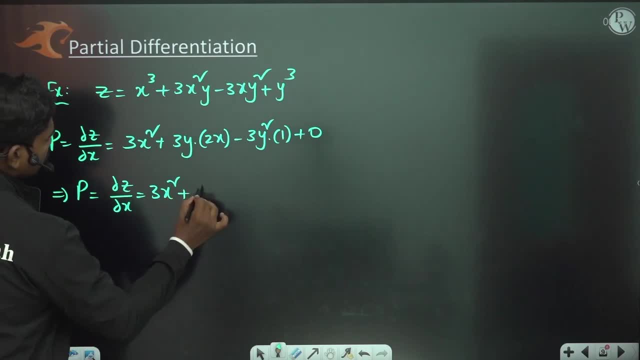 get P is equal to dou Z by dou X, which get P is equal to dou Z by dou X, which is of course equal to 3x square plus 6, is of course equal to 3x square plus 6 is of course equal to 3x square plus 6: X Y minus 3 Y square. this is what you. 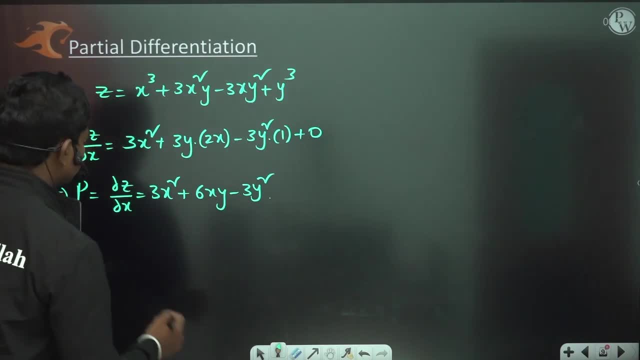 X Y minus 3 Y square. this is what you X Y minus 3 Y square. this is what you have here, okay, similarly, if you have here, okay, similarly, if you have here, okay, similarly, if you calculate Q, Q is equal to calculate Q, Q is equal to. 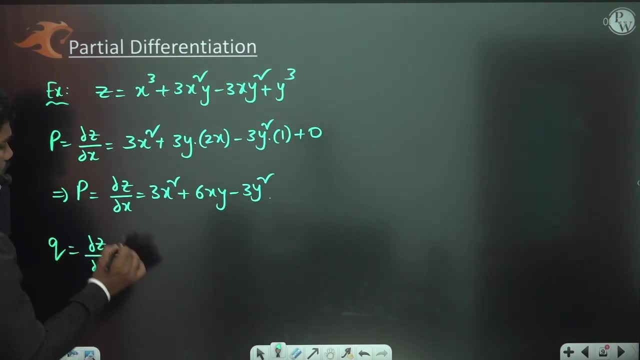 calculate Q, Q is equal to dou Z by dou Y. so if you calculate this Q value, dou Z by dou Y, so if you calculate this Q value, dou Z by dou Y, so if you calculate this Q value, which is dou Z by dou Y, now, which is dou Z by dou Y, now, 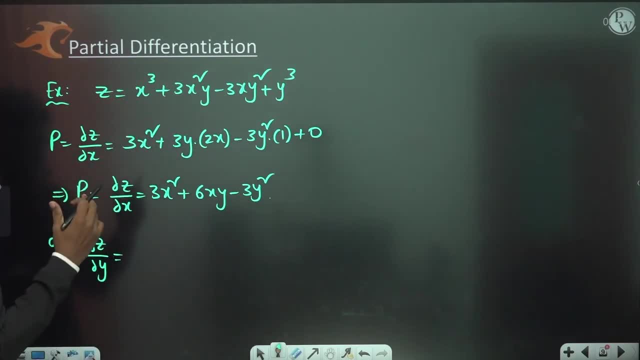 which is dou Z by dou Y. now differentiate this with respect to Y, differentiate this with respect to Y. differentiate this with respect to Y partially. so when you are differentiating partially, so when you are differentiating partially, so, when you are differentiating with respect to Y, you treat X as. 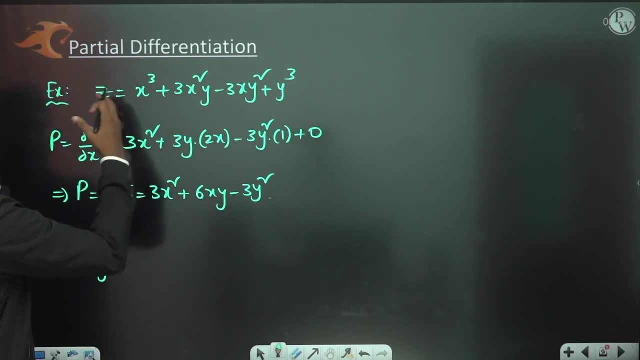 with respect to Y, you treat X as with respect to Y, you treat X as constant. so if X is constant, X cube is constant. so if X is constant, X cube is constant. so if X is constant, X cube is also constant. so differentiation of a also constant. so differentiation of a. 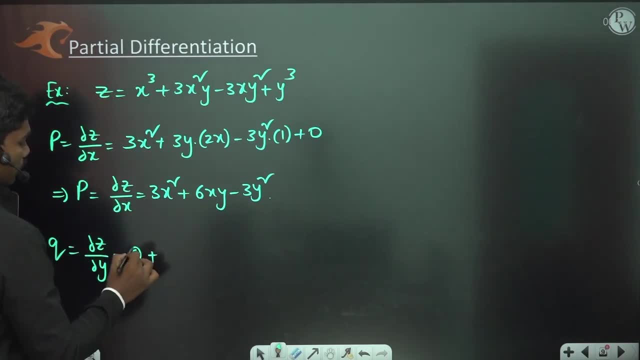 also constant. so differentiation of a constant is 0 plus now. what are? the constant is 0 plus now. what are? the constant is 0 plus now. what are? the derivative of Y with respect to Y is 1. derivative of Y with respect to Y is 1. 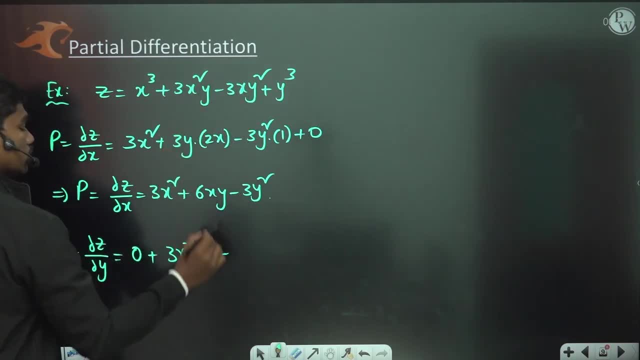 derivative of Y with respect to Y is 1 minus 3 X is constant, so 3 X into minus 3 X is constant, so 3 X into minus 3 X is constant, so 3 X into differentiation of this Y square is 2y. 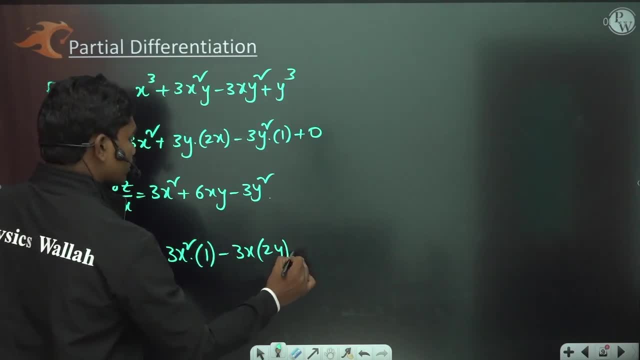 differentiation of this Y square is 2y. differentiation of this Y square is 2y, so this is 2y, and differentiation of Y: so this is 2y. and differentiation of Y, so this is 2y. and differentiation of Y cube is 3y square. okay. so if you see, if 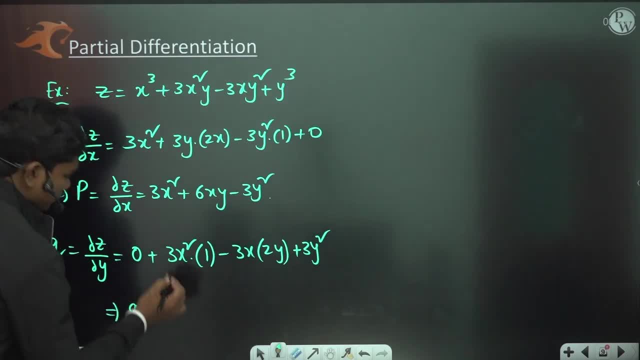 cube is 3y square. okay. so if you see, if cube is 3y square, okay. so if you see, if you simplify the result, Q is equal to Q. you simplify the result: Q is equal to Q. you simplify the result: Q is equal to. Q is equal to 3 X square minus 6 X Y plus 3 Y. 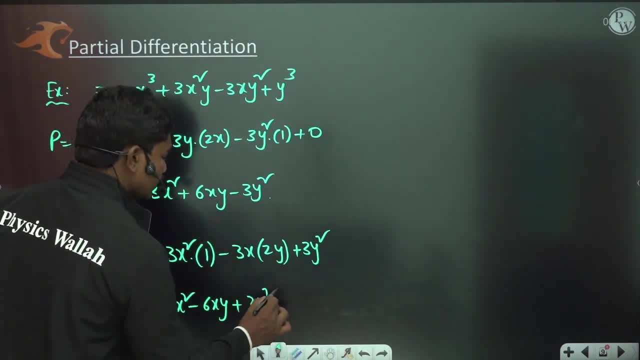 is equal to 3 X square minus 6 X Y plus 3 Y square. okay, so this is 3y square square. okay, so this is 3y square square. okay, so this is 3y square actually here. okay, so this is how you. 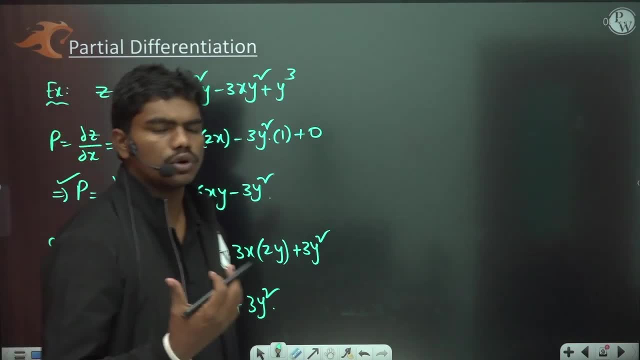 actually here. okay, so this is how you actually here. okay, so this is how you calculate P and Q, basically differentiation. calculate P and Q basically differentiation. calculate P and Q basically differentiation. which is known to you, but again to some. which is known to you, but again to some. 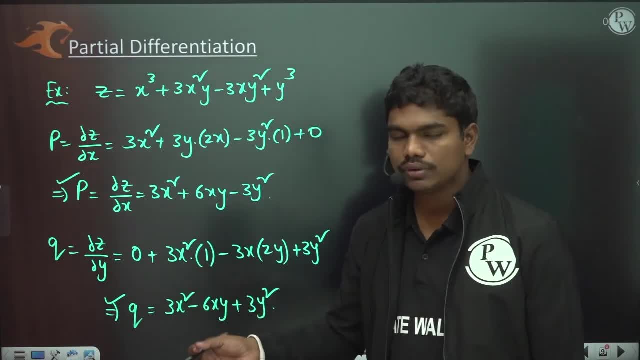 which is known to you but again to some of- if still some of you face difficulty of, if still some of you face difficulty of, if still, some of you face difficulty. this is how you do that differentiation. this is how you do that differentiation. this is how you do that differentiation in a step-by-step way. this is how you. 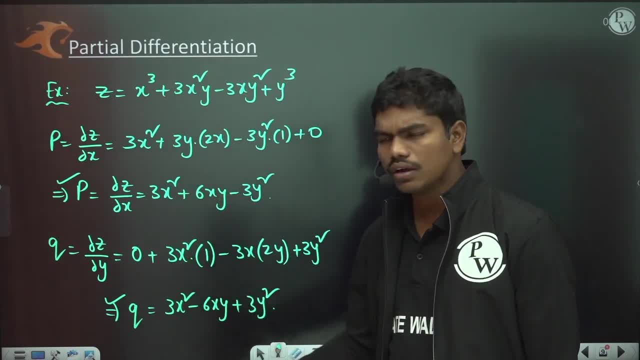 in a step-by-step way. this is how you, in a step-by-step way, this is how you calculate do f by do x and you can say: calculate do f by do x. and you can say: calculate do f by do x. and you can say: do z by do x and do z by do y. here, okay, 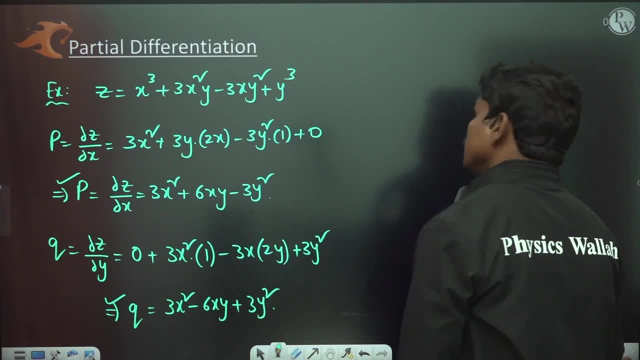 do z by do x and do z by do y here. okay. do z by do x and do z by do y here. okay, here. I would like to. I want you explain here. I would like to. I want you explain here. I would like to. I want you explain you one point actually. okay, fine, I want. 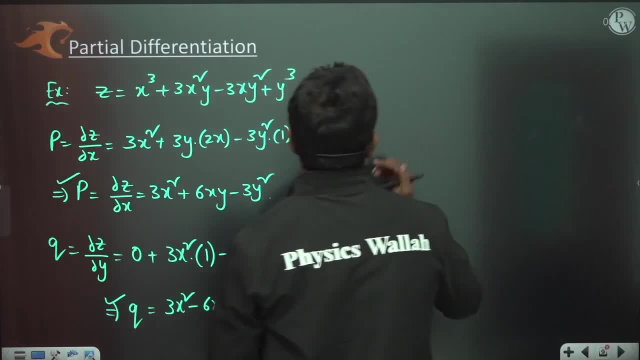 you one point, actually, okay, fine. I want you one point, actually okay, fine. I want to explain you one point here. look, try to explain you one point here. look, try to explain you one point here. look, try to understand carefully here, if you to understand carefully here, if you. 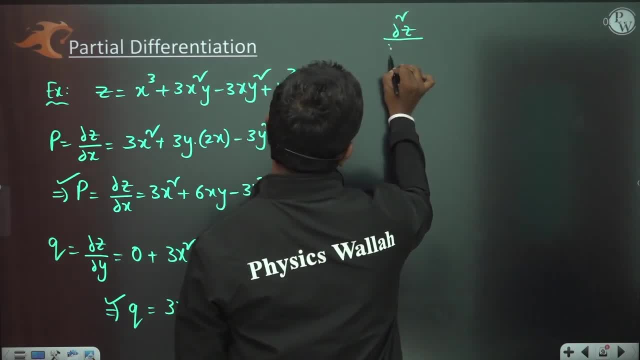 to understand carefully here: if you calculate and do square Z by do X, do calculate and do square Z by do X. do calculate and do square Z by do X, do y. what is the meaning of this? do by do X- y. what is the meaning of this? do by do X. 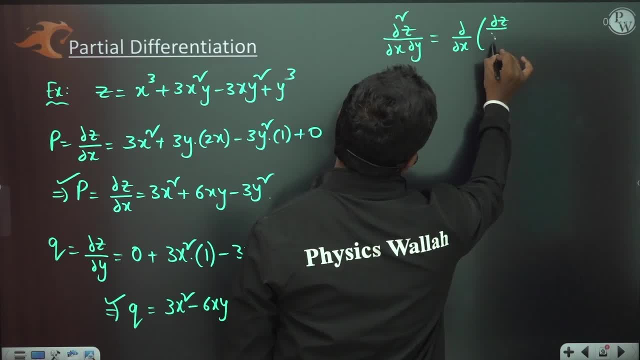 y. what is the meaning of this? do by do X of do z by do y actually. so this will be of do z by do y actually. so this will be of do z by do y actually. so this will be same as do by do y of do z by do x. for. 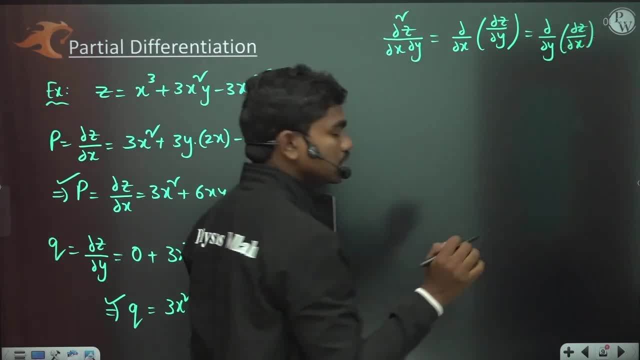 same as do by do y of do z by do x. for same as do by do y of do z by do x. for any function in general means. in case of any function in general means. in case of any function in general means, in case of partial differentiation. the order of. 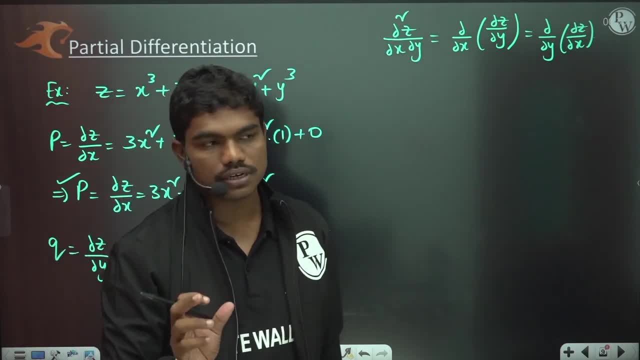 partial differentiation. the order of partial differentiation, the order of differentiation doesn't matter means if differentiation doesn't matter means if differentiation doesn't matter means if you take a two variable function, you take a two variable function, you take a two variable function initially. if you differentiate with 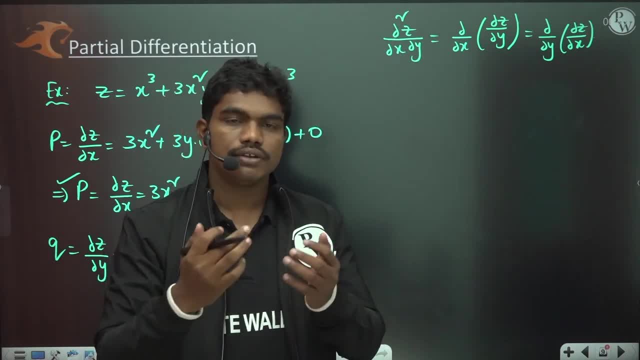 initially, if you differentiate with initially, if you differentiate with respect to X and then with respect to Y. respect to X and then with respect to Y. respect to X and then with respect to Y partially, or if you differentiate with partially, or if you differentiate with partially, or if you differentiate with respect to Y first and then with respect. 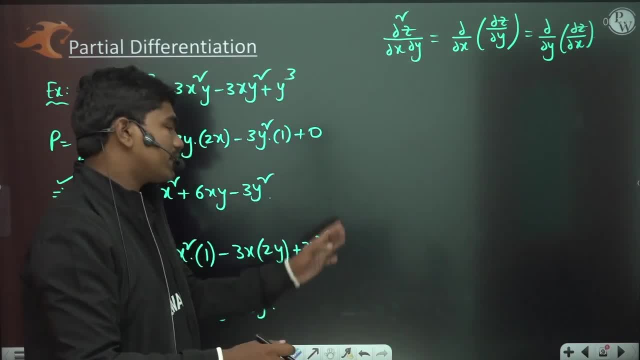 respect to Y first and then with respect. respect to Y first and then with respect to X later. the result, I might say I will to X later. the result, I might say I will to X later. the result I might say I will show you with the help of some simple. 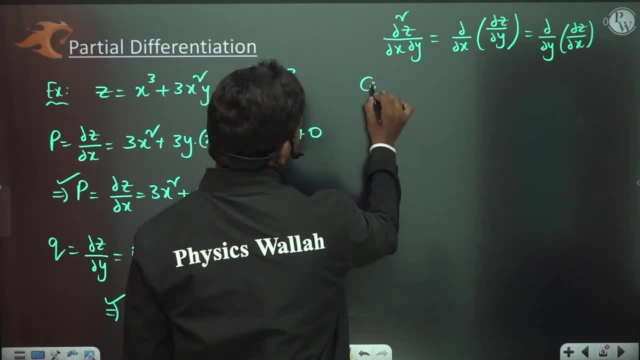 show you with the help of some simple show you with the help of some simple calculations: now first consider, consider calculations. now first consider, consider calculations. now first consider, consider, do by doze it. I mean do by do X of do, do by do Z. I mean do by do X of do. 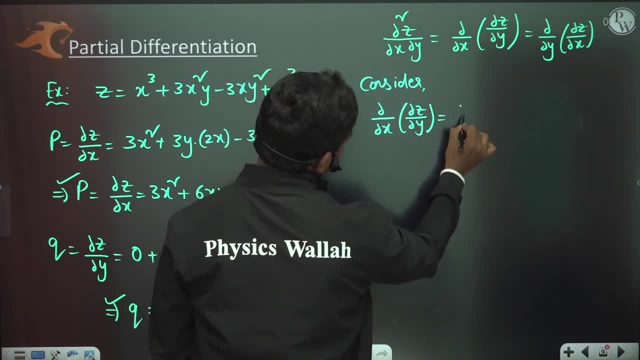 do by do X. of do Z I mean do by do Y. so if you calculate this result, this is so. if you calculate this result, this is so. if you calculate this result. this is partial differentiation of doze at bed. partial differentiation of doze at bed. 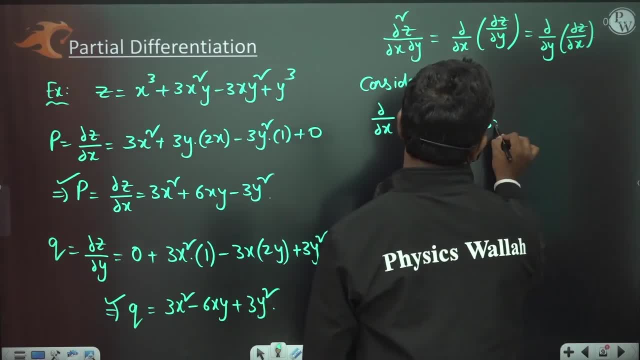 partial differentiation of doze at bed over. what is this function? does it bed over? what is this function? does it bed over? what is this function? does it bed away? 3x square away. 3x. square away. 3x square minus 6: X. Y plus minus 6, X. Y plus 3y. 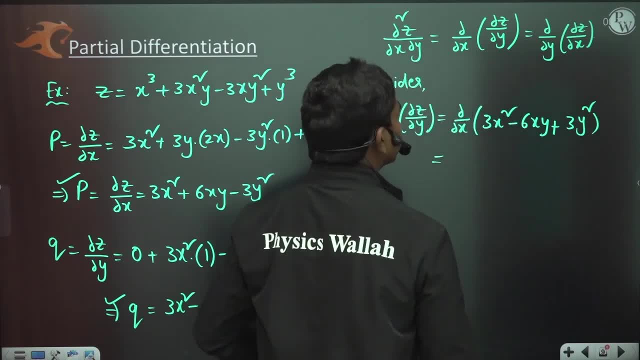 minus 6 X Y plus minus 6 X Y plus 3y minus 6 X Y plus minus 6 X Y plus 3y square okay. so if you simplify this, what square? okay. so if you simplify this, what square? okay. so if you simplify this, what will you get? do by do X of 3x square. will you get do by do X of 3x square. will you get? do X of 3x square? this is completely function of X. so this is completely function of X. so this is completely function of X. so, differentiation of this with respect to differentiation of this with respect to: 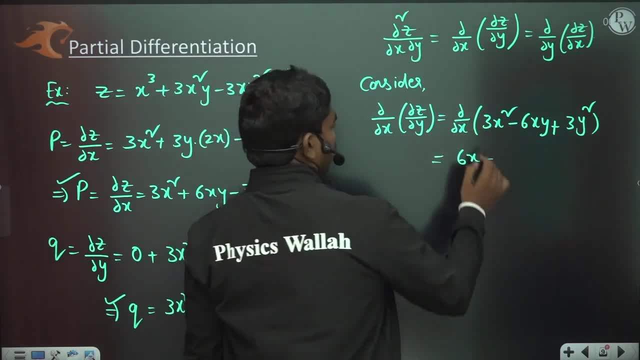 differentiation of this with respect to X is 6 X minus. now when you are X is 6 X minus. now when you are X is 6 X minus. now, when you are differentiating with respect to X, differentiating with respect to X, differentiating with respect to X partially, 6 and Y are constants. 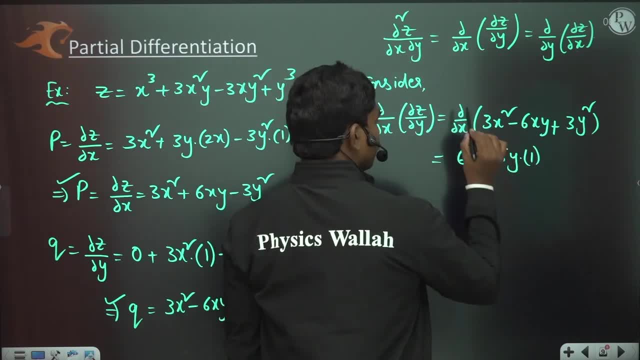 partially, 6 and Y are constants. partially, 6 and Y are constants. differentiation of X with respect to X is: differentiation of X with respect to X is. differentiation of X with respect to X is 1 when you are differentiating with 1. when you are differentiating with. 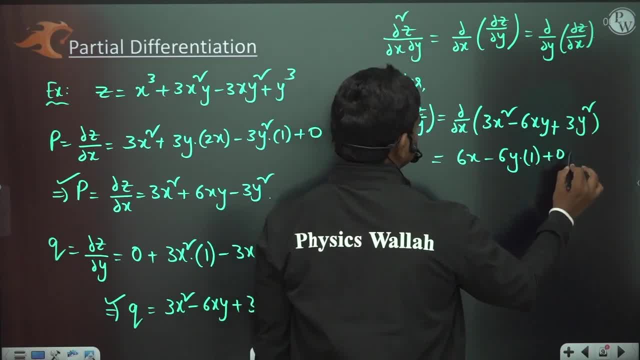 1 when you are differentiating with respect to X, this total term is a respect to X. this total term is a respect to X. this total term is a constant. so plus 0, which is 6x minus 6y constant. so plus 0, which is 6x minus 6y. 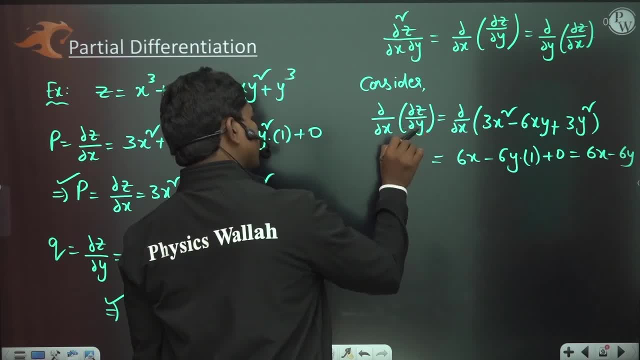 constant, so plus 0, which is 6x, minus 6y. so this is nothing what you have. so this is nothing what you have. so this is nothing what you have, differentiated this function with differentiated this function with differentiated this function with respect to Y first, and you have: 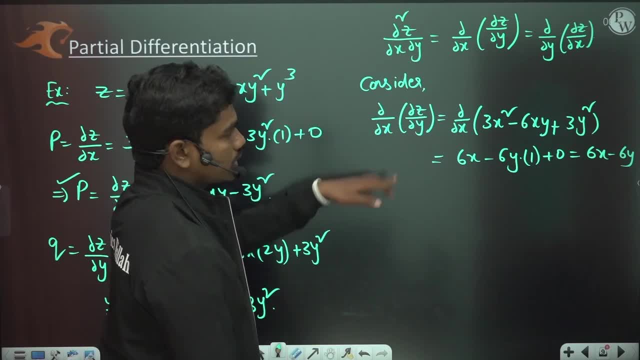 respect to Y first, and you have respect to Y first, and you have differentiated with respect to X, next, differentiated with respect to X next, differentiated with respect to X, next, correct? so this is dou square z by dou, correct? so this is dou square z by dou, correct? so this is dou square z by dou x, dou, y. now let us consider, consider dou. 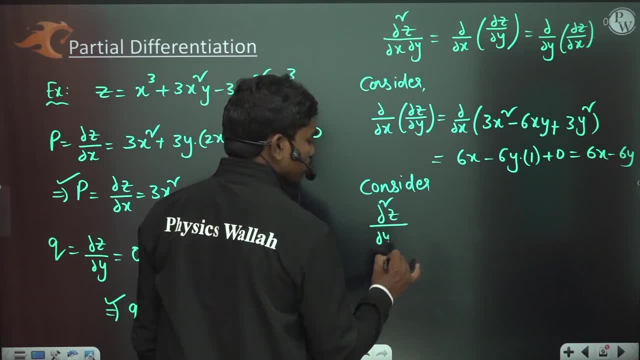 x, dou y. now let us consider consider dou x, dou y. now let us consider consider dou square z by dou x. so what is the square z by dou x? so what is the square z by dou x? so what is the meaning of this dou by dou y, of dou z by? 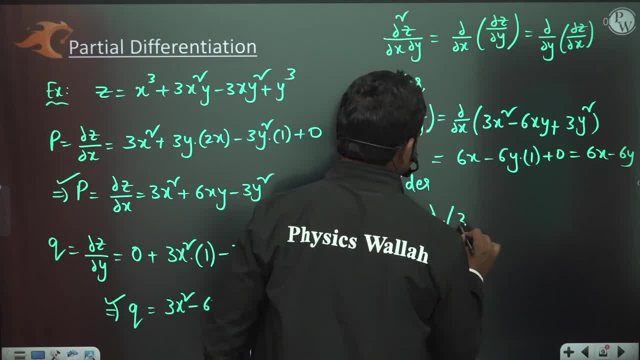 meaning of this dou by dou y of dou z by meaning of this dou by dou y of dou z by dou x. okay, so what is the expression for dou x? okay, so, what is the expression for dou x? okay, so what is the expression for dou z by dou x? 3x square plus 6x y minus. 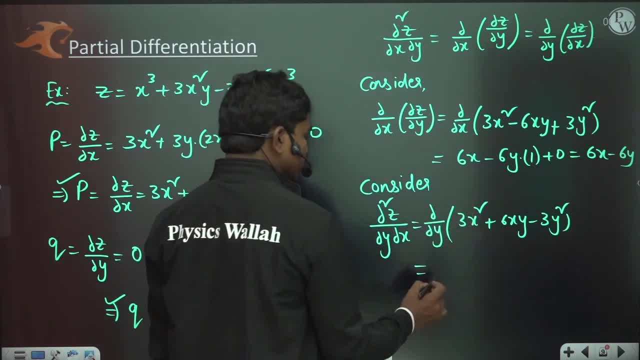 3y square. okay, so if you take out this, then differentiating this partially gives, then differentiating this partially gives, then differentiating this partially gives you: this is a constant, so 0 plus you. this is a constant, so 0 plus you. this is a constant, so 0 plus differentiation of 6x. y is 6x is a. 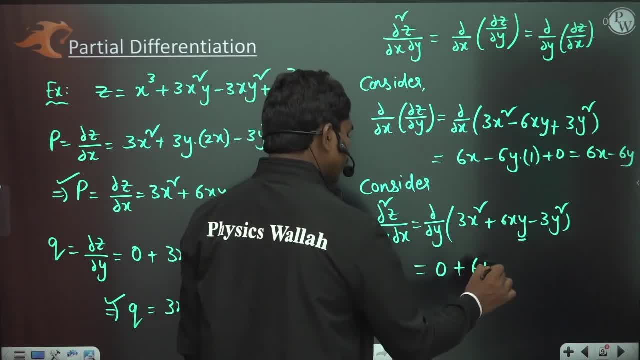 differentiation of 6x. y is 6x is a differentiation of 6x. y is 6x is a constant now. differentiation of this way: constant now. differentiation of this way: constant now. differentiation of this way with respect to y is 1 minus this 3y. with respect to y is 1 minus this. 3y with respect to y is 1 minus this 3y. square is also function of y. completely square is also function of y completely square is also function of y completely. so if you differentiate with respect to, 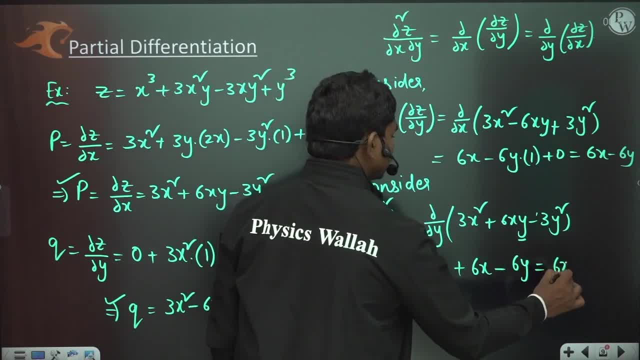 so if you differentiate with respect to so if you differentiate with respect to y, you will get 6y. so total 6x minus 6y y, you will get 6y, so total 6x minus 6y y, you will get 6y. so total 6x minus 6y. and if you see, these two results are: 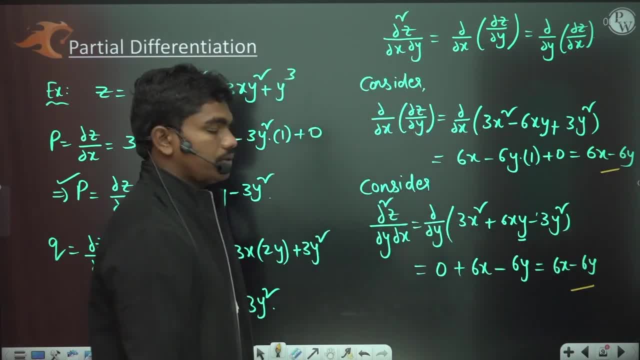 and if you see these two results are, and if you see these two results are actually same: 6x minus 6y and 6x minus 6y actually same: 6x minus 6y and 6x minus 6y actually same: 6x minus 6y and 6x minus 6y means in case of a partial differentiation. 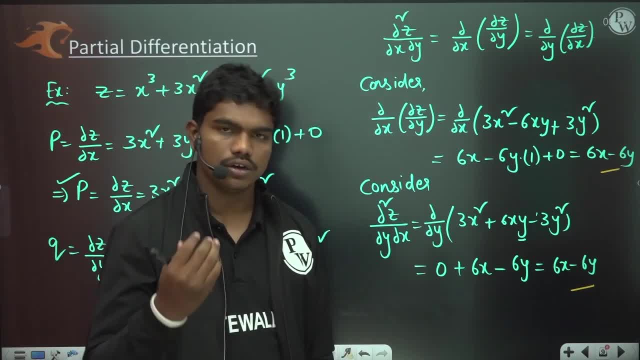 means in case of a partial differentiation. means in case of a partial differentiation if you differentiate with respect to x, if you differentiate with respect to x, if you differentiate with respect to x first and with respect to y or with first and with respect to y or with. 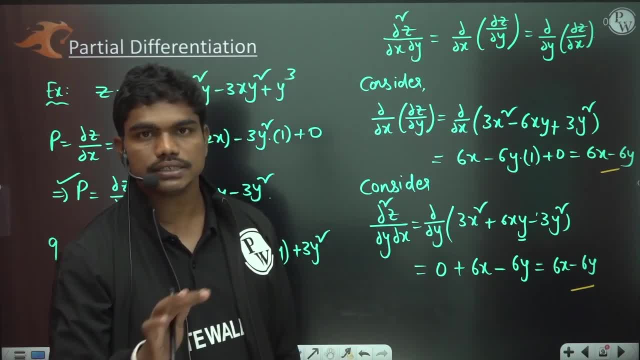 first and with respect to y, or with respect to y first and then with respect to y first and then with respect to y first and then with respect to x: the result remains same. respect to x: the result remains same. respect to x: the result remains same. actually clear. so this is one very 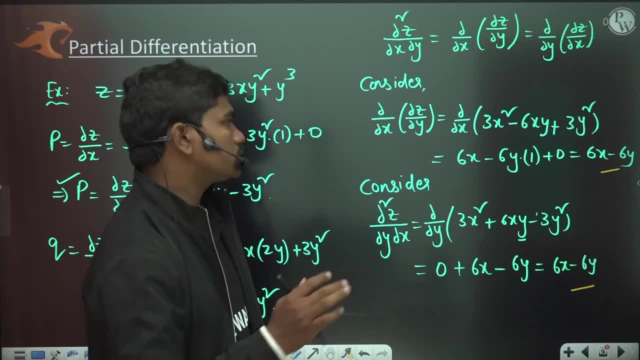 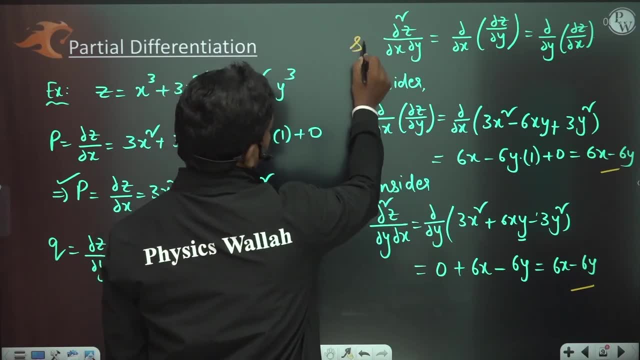 actually clear. so this is one very actually clear. so this is one very say important point that is to be say important point, that is to be say important point, that is to be for the- uh, you know, swapping of these two, for the- uh, you know, swapping of these two. 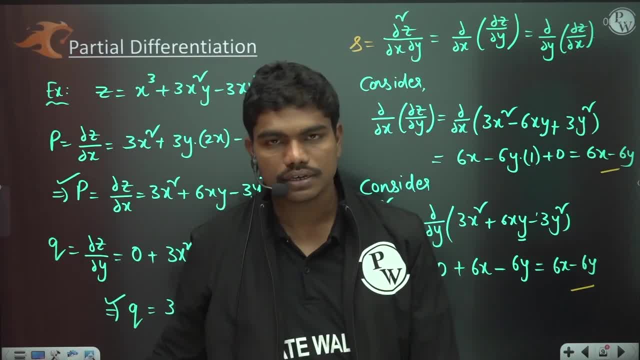 for the uh, you know, swapping of these two dou by dou x doesn't matter. we generally dou by dou x doesn't matter, we generally dou by dou x doesn't matter, we generally call this, call this, call this spq. and that is s actually here, okay, so. 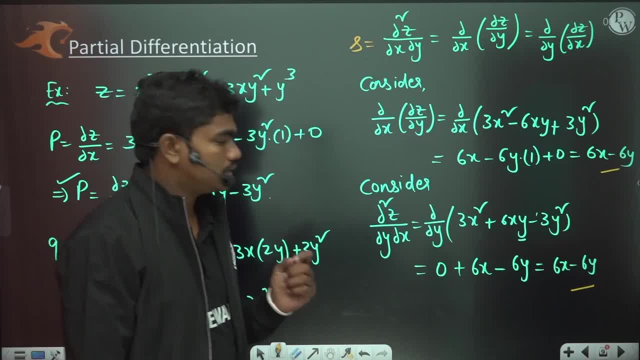 spq, and that is s actually here, okay, so spq, and that is s actually here, okay. so this, uh, this is basically some knowledge. this, uh, this is basically some knowledge. this, uh, this is basically some knowledge of partial derivatives, actually of partial derivatives, actually of partial derivatives actually. now we talk about one very important. 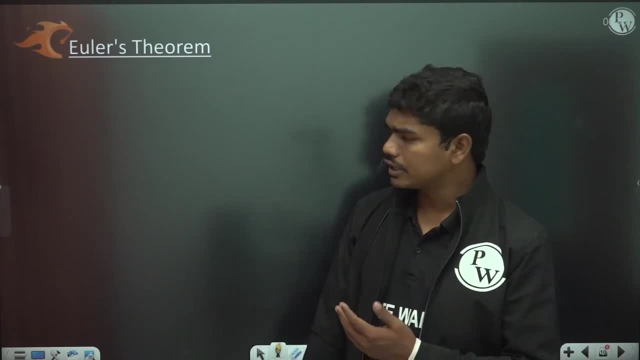 now we talk about one very important. now we talk about one very important theorem which is called the theorem, which is called the theorem, which is called the euler's theorem. okay, so, or you can call euler's theorem, okay so, or you can call that euler's in your some 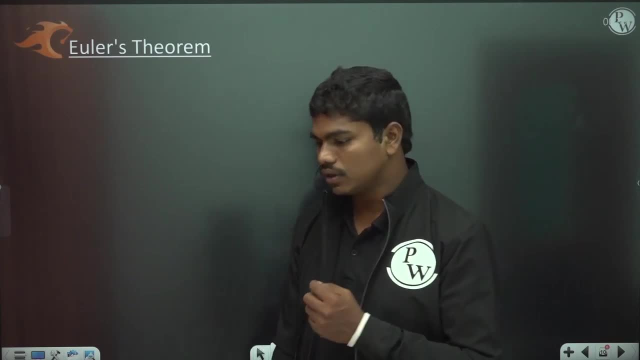 that euler's in your some, that euler's in your some knowledge: you know pronunciations, but we knowledge. you know pronunciations, but we knowledge. you know pronunciations, but we call that euler's- okay, so euler's theorem. call that euler's, okay, so euler's theorem. 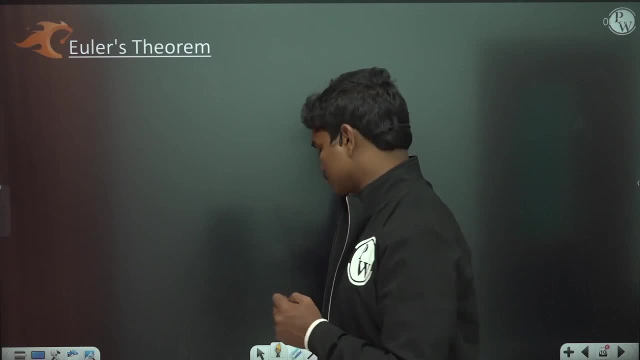 call that euler's. okay, so euler's theorem. so let us see what. what does this euler's? so let us see what. what does this euler's? so let us see what. what does this euler's theorem talk about? look, let us suppose. theorem talk about. look, let us suppose. 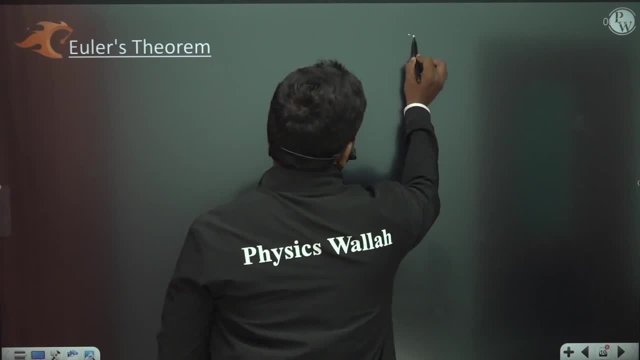 theorem talk about. look, let us suppose, if i have this function, for example, okay, if i have this function, for example, okay, if i have this function, for example: okay, so i had this function. z is equal to, so i had this function. z is equal to. so i had this function. z is equal to. z is equal to x cube plus 3x square y. 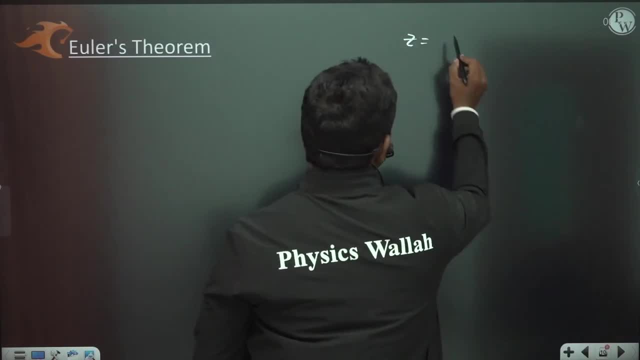 z is equal to x cube plus 3x square y. z is equal to x cube plus 3x square y, minus 3 x y square plus y cube. okay, so minus 3 x y square plus y cube. okay, so minus 3 x y square plus y cube. okay, so let us see here x cube. 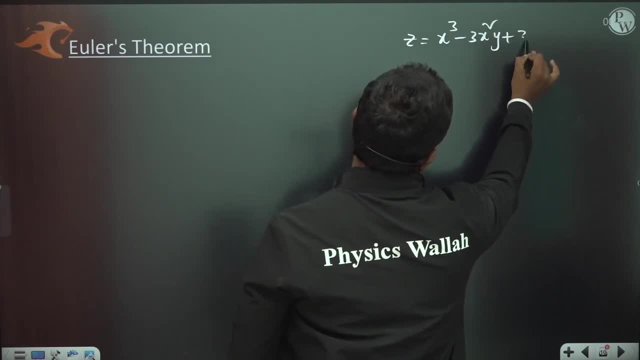 let us see here x cube. let us see here x cube minus 3 x square y minus 3 x square y minus 3 x square y plus 3 x y square plus 3 x y square plus 3 x y square minus y cube. correct, this is the function. 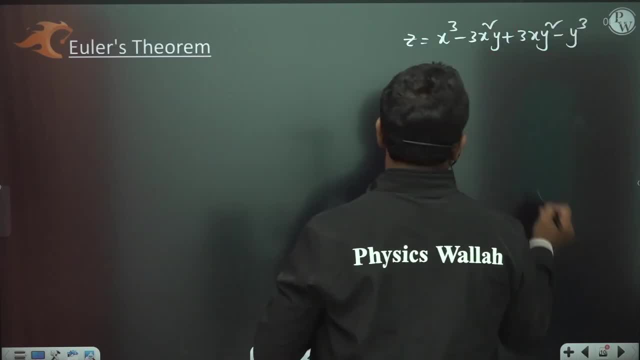 minus y cube, correct. this is the function minus y cube, correct. this is the function i have taken. i have taken. i have taken plus plus, minus, plus, so plus, okay. i have plus plus, minus, plus, so plus, okay. i have plus, plus, minus, plus, so plus, okay, i have taken plus here. 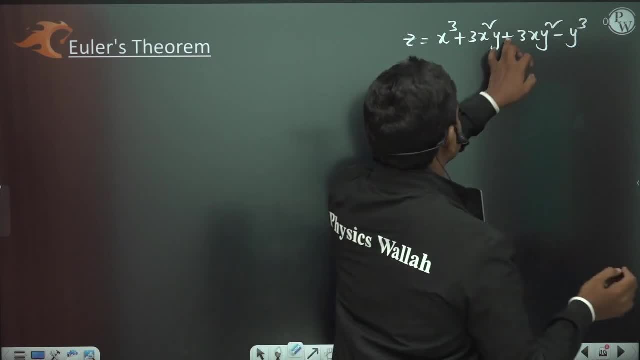 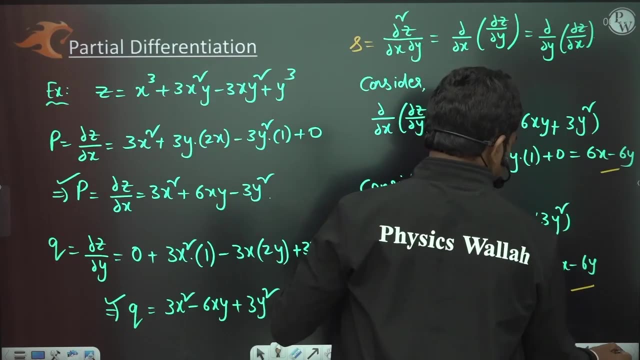 taken plus here. taken plus here: x cube plus 3 x square y x cube plus 3 x cube plus 3 x square y x cube plus 3 x cube plus 3 x square y x cube plus 3 x square y x square y. 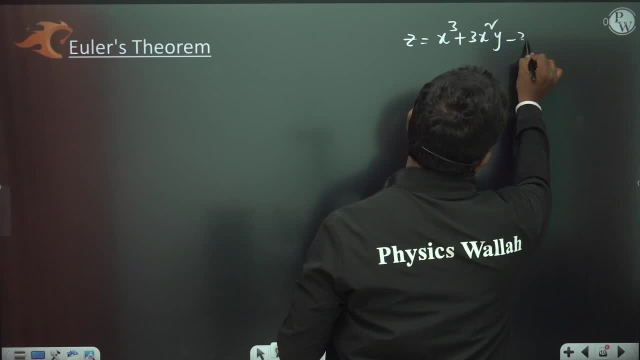 x square y, and then we have minus 3 x y square plus, and then we have minus 3 x y square plus, and then we have minus 3 x y square plus y cube. okay, so let us suppose this is the z. okay, so let us suppose this is the z. 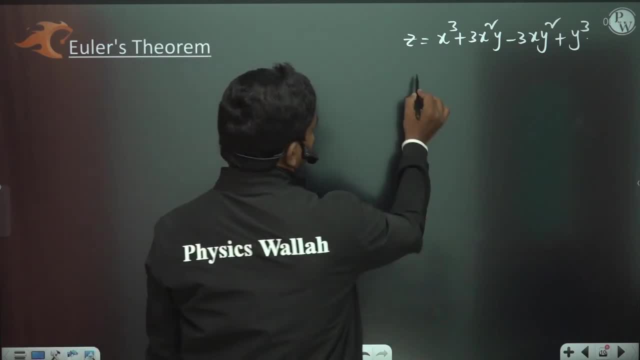 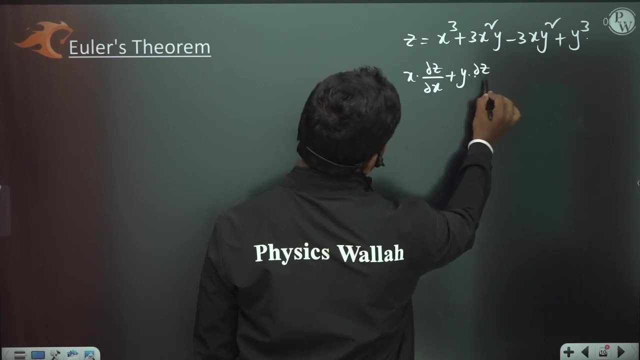 okay, so let us suppose this is the z value. now if i ask you, what is the sum value? now? if i ask you, what is the sum value now, if i ask you what is the sum of of of x into dou z by dou x and y into dou z by dou y, let us suppose and y into dou z by dou y, let us suppose. and y into dou z by dou y, let us suppose. if i ask you this sum, if i ask you this sum, if i ask you this sum, then definitely you know that this is, then definitely you know that this is. 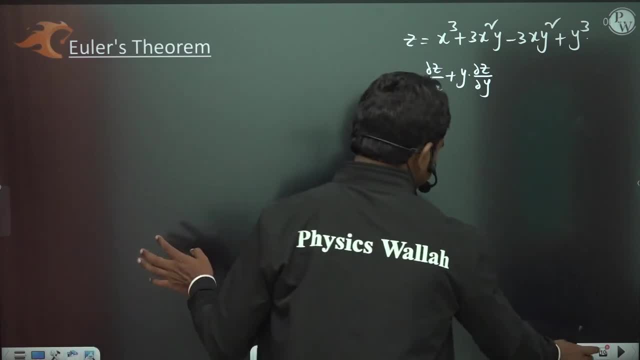 then definitely you know that this is going to be some hectic process, of going to be some hectic process, of going to be some hectic process, of course, course, course. here you automatically know this. values here: you automatically know this. values here, you automatically know this: values of dou z by dou x and dou z by dou y. of dou z by dou x and dou z by dou y, of dou z by dou x and dou z by dou y. but let us suppose if these values are. but let us suppose if these values are. but let us suppose if these values are not there or if this function is little. 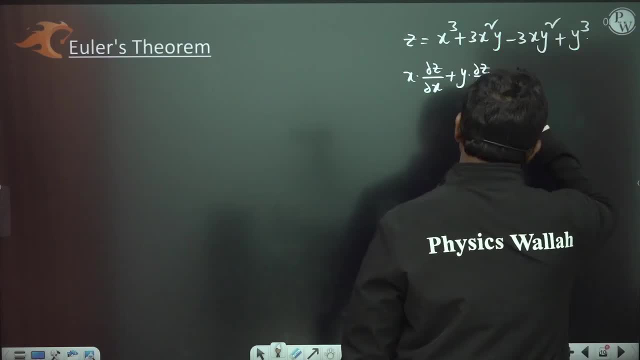 not there, or if this function is little not there, or if this function is little, complicated, complicated, complicated, then this calculation of this, then this calculation of this, then this calculation of this expression is not, uh, very simple expression is not, uh, very simple expression is not, uh, very simple, actually, okay. so now let us see how we 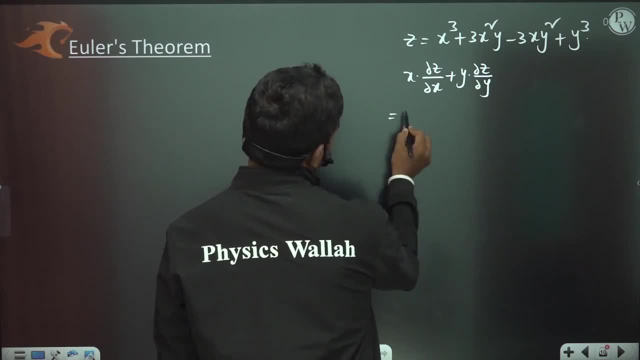 actually okay. so now let us see how we actually okay. so now let us see how we actually do this, actually do this, actually do this. okay, so see here, of course, since we have okay. so see here, of course, since we have okay. so see here, of course, since we have the values x into dou z by dou x. so what? 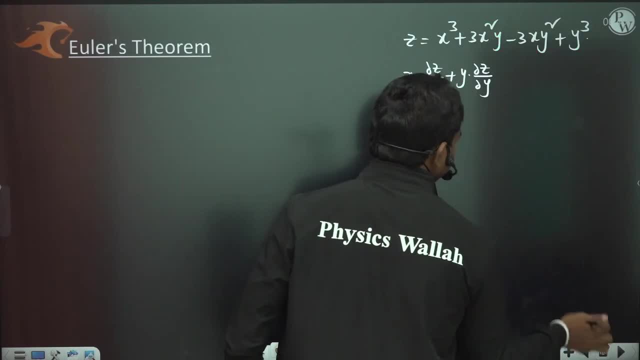 the values x into dou z by dou x. so what the values x into dou z by dou x? so what is dou z by dou x? is dou z by dou x. is dou z by dou x: three x square plus six x y minus three y. three x square plus six x y minus three y. 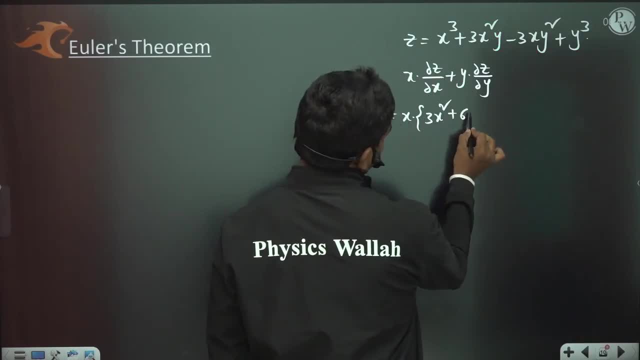 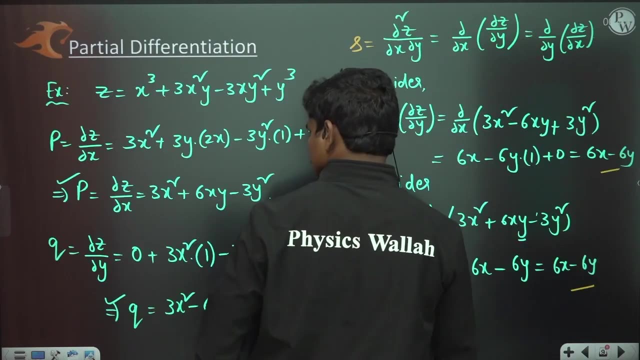 three x square plus six x y minus three y square square square. three x square plus six x y. three x square plus six x y. three x square plus six x y minus three y square multiplied with minus three y square multiplied with minus three y square multiplied with y times of dou z by dou y, so what is? 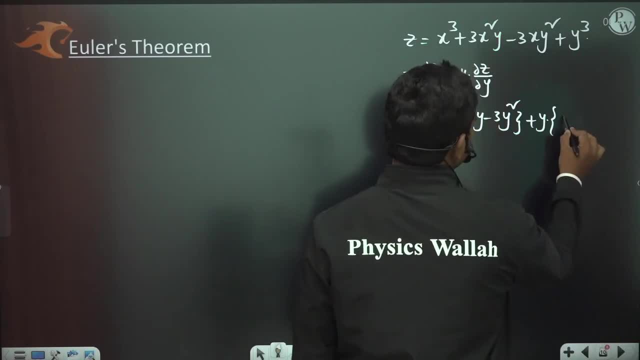 y times of dou z by dou y. so what is y times of dou z by dou y? so what is dou z by dou y? dou z by dou y. dou z by dou y. three x square minus six x y three x. three x square minus six x y, three x. 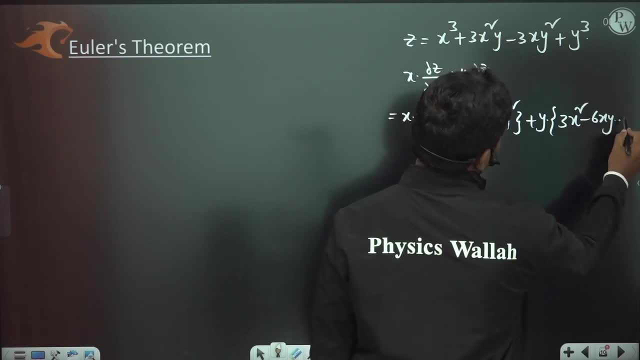 three x square minus six x y. three x square square square minus six x y plus minus six x y, plus minus six x y, plus three y square, correct. this is what we three y square correct. this is what we three y square, correct. this is what we have, plus three y square. 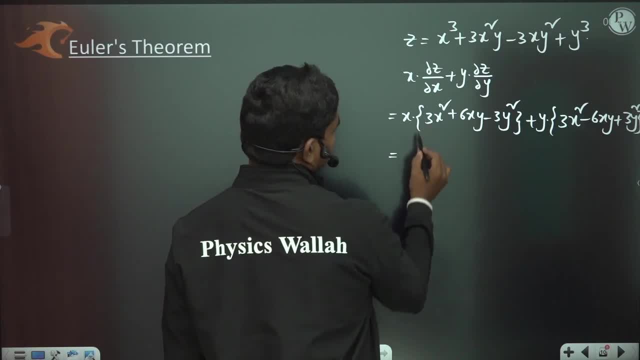 have plus three y square. have plus three y square. now, if you simplify this result, let us now, if you simplify this result, let us now, if you simplify this result, let us see what we get three x cube. see what we get three x cube. see what we get three x cube. three x cube plus this is. 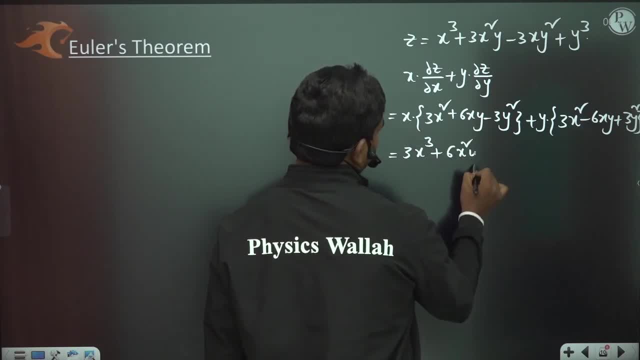 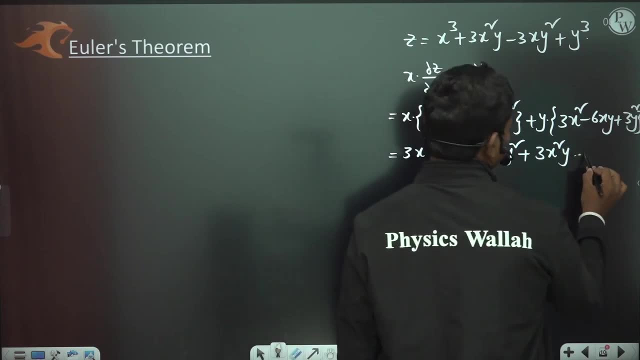 three x cube plus this is three x cube plus this is six x square y, six x square y, six x square y minus three x y square, minus three x y square, minus three x y square plus plus plus three x square y, three x square y, three x square y minus six x y square. 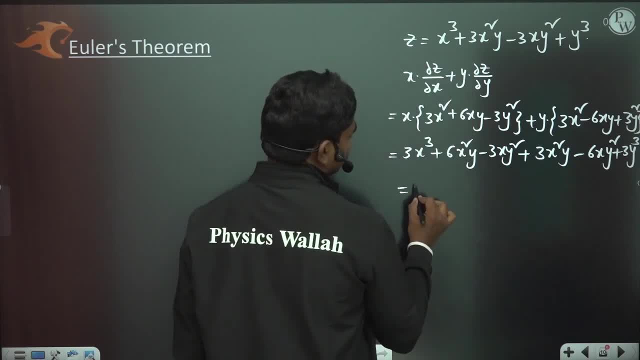 minus six x y square, minus six x y square, plus three times of y cube. this is what plus three times of y cube. this is what plus three times of y cube. this is what you get if you slightly simplify this. you get if you slightly simplify this. 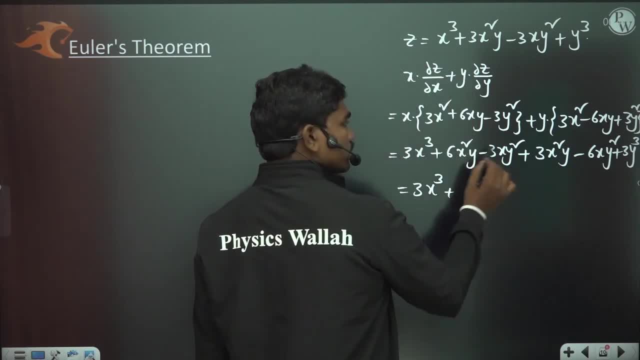 you get, if you slightly simplify this, three times of x cube plus three times of x cube, plus three times of x cube, plus six x square y, six x square y, six x square y. total nine x square y. total nine x square y. total nine x square y minus three x y square, minus six x x y. 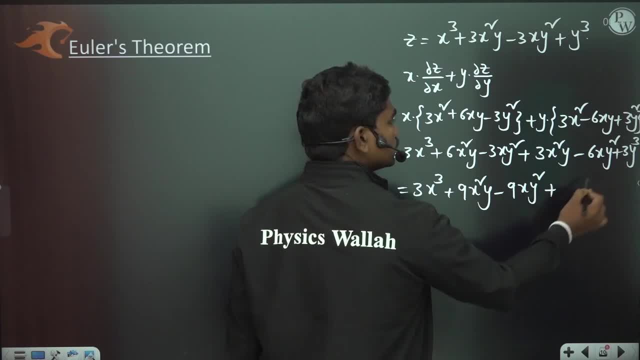 minus three x y square. minus six x x y. minus three x y square. minus six x x y square. so total minus nine x y square square. so total minus nine x y square square. so total minus nine x y square and plus three y cube. so this is what 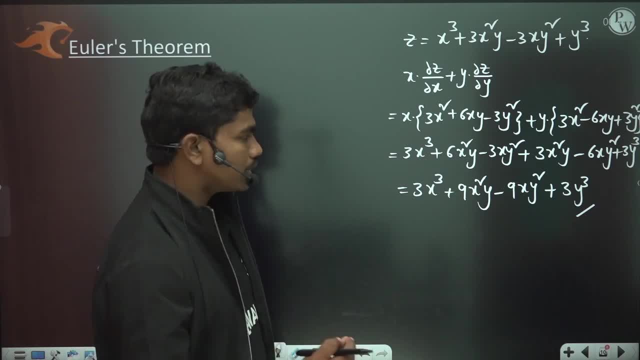 and plus three y cube, so this is what. and plus three y cube, so this is what the result you will get. but if you the result you will get. but if you the result you will get. but if you observe carefully something, you will observe carefully something you will. 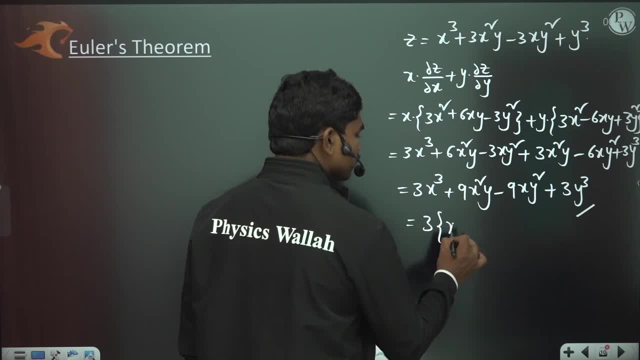 observe carefully something, you will understand one thing: that if you take a, understand one thing, that if you take a, understand one thing: that if you take a three common, three common, three common, this is nothing but x cube. this is nothing but x cube. this is nothing but x cube plus three x square y, minus three x y. 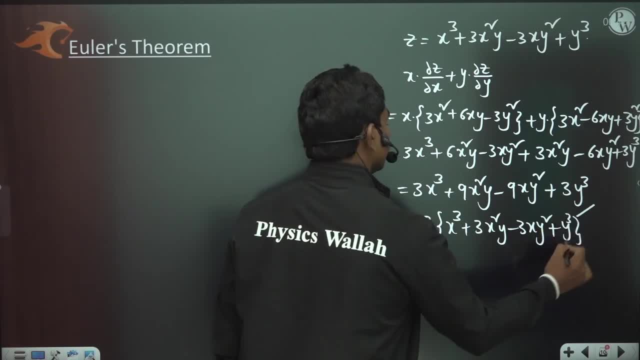 plus three x square y minus three x y plus three x square y minus three x y square square square plus y cube, correct. so if you see this plus y cube, correct. so if you see this plus y cube, correct. so if you see, this expression is nothing but this function. 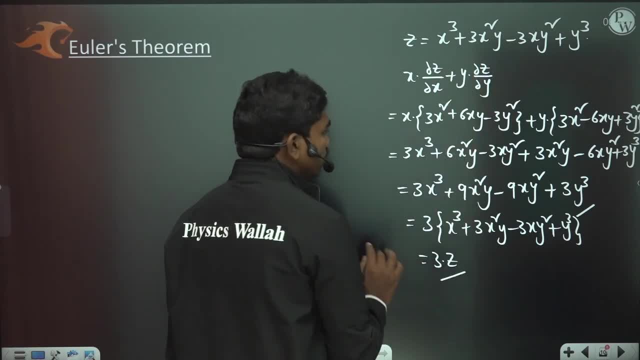 expression is nothing but this function. expression is nothing but this function again. so this is three times of again. so this is three times of again. so this is three times of z actually okay. so of course we have z actually okay. so of course we have z actually okay. so of course we have identified this after some long. 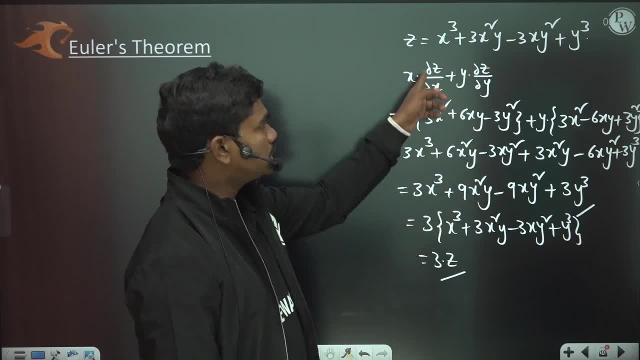 identified this after some long, identified this after some long calculation, calculation, calculation, and if you see this, does it better. x is and if you see this, does it better x is and if you see this does it better, x is very easy to calculate for such very easy to calculate for such. 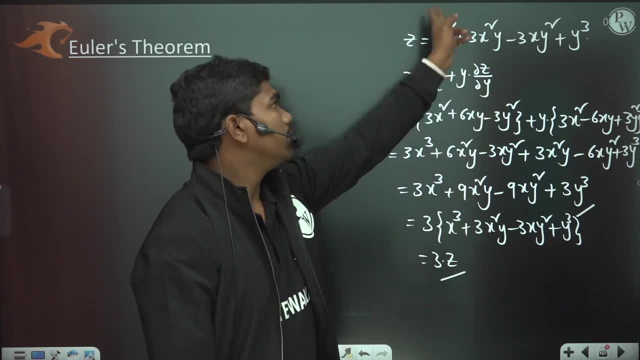 very easy to calculate for such functions. but let us suppose if i give functions. but let us suppose if i give functions. but let us suppose if i give you some complicated functions like you, some complicated functions like you, some complicated functions like x, cube plus three x square y divided by x. x cube plus three x square y divided by x x cube plus three x square y divided by x square minus y square. if i give you square minus y square, if i give you square minus y square, if i give you such functions, then calculating this, such functions, then calculating this. 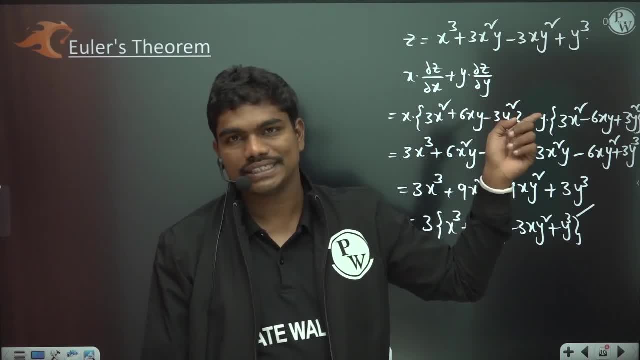 such functions, then calculating this: does it better, x does it better, is does it better, x does it better? is does it better? x does it better? is not? uh, you know very easy thing for you, not. uh, you know very easy thing for you, not. uh, you know very easy thing for you. so that's how. 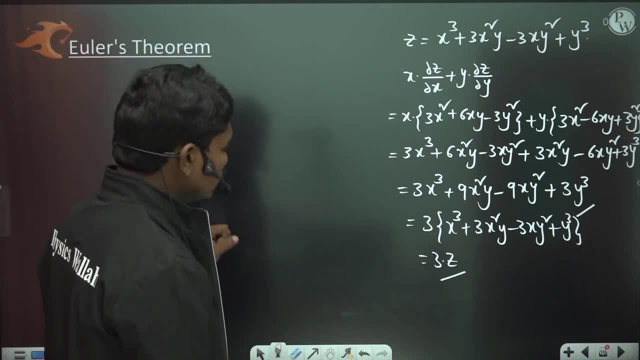 so that's how. so that's how. that's the reason why we have developed. that's the reason why we have developed. that's the reason why we have developed something called euler's theorem. okay, so, something called euler's theorem. okay, so, something called euler's theorem, okay. so what is this euler's theorem? let us see. 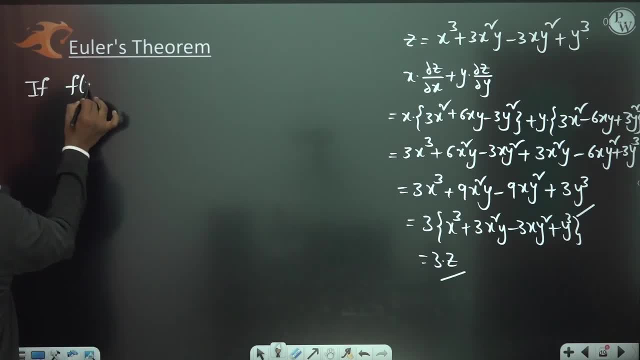 what is this euler's theorem? let us see. what is this euler's theorem? let us see if, if, if f of x comma y, f of x comma y, f of x comma y is continuous and differentiable, is continuous and differentiable, is continuous and differentiable continuous. 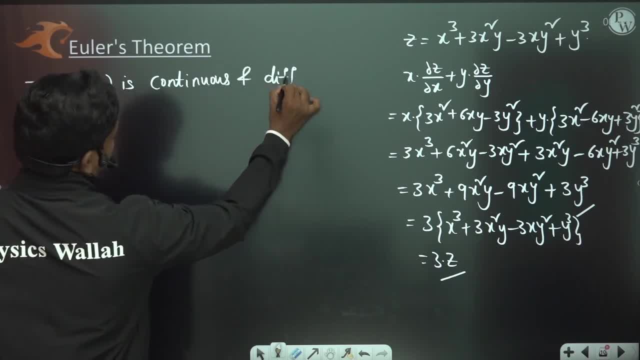 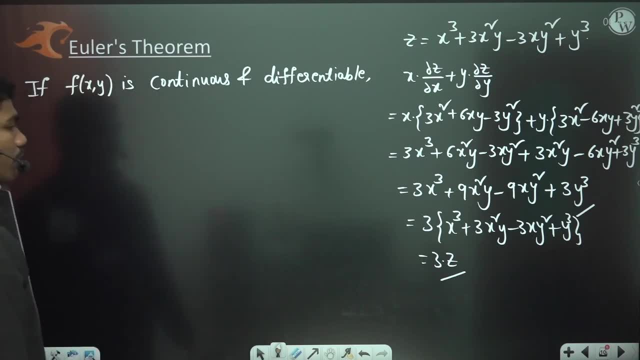 continuous, continuous and and and differentiable, for example, let us say okay, differentiable, for example, let us say okay, differentiable. for example, let us say: okay, so this is continuous, so this is continuous, so this is continuous and differentiable. okay so, if f of x and differentiable. okay so if f of x. 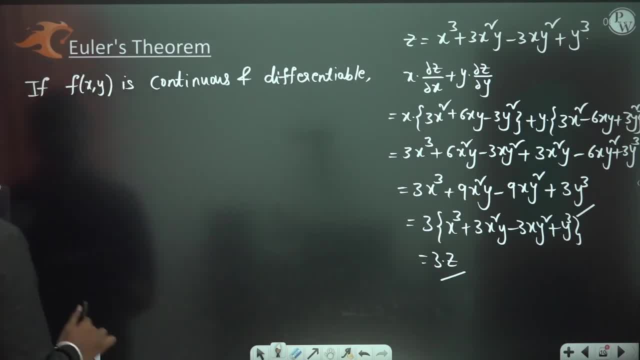 and differentiable. okay, so if f of x comma y is continuous and differentiable, comma y is continuous and differentiable, comma y is continuous and differentiable. now, let us see now, let us see now, let us see, sorry, now, let us see what happens. okay, sorry, now, let us see what happens okay. 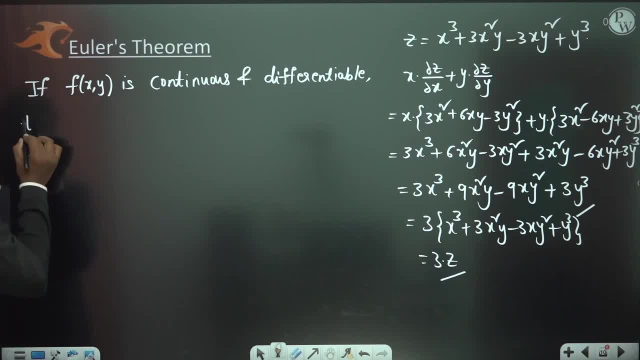 sorry, now let us see what happens. okay, it's continuous and differentiable. it's continuous and differentiable. it's continuous and differentiable. then, then, then, and you can write one more condition, and, and you can write one more condition, and, and you can write one more condition, and f of x, comma y is. 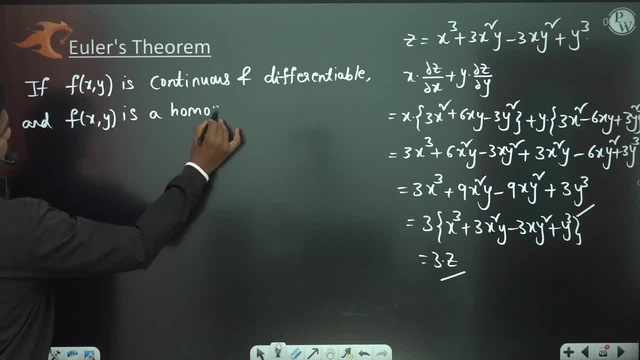 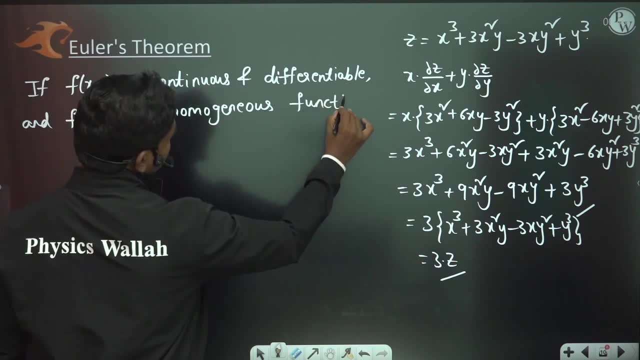 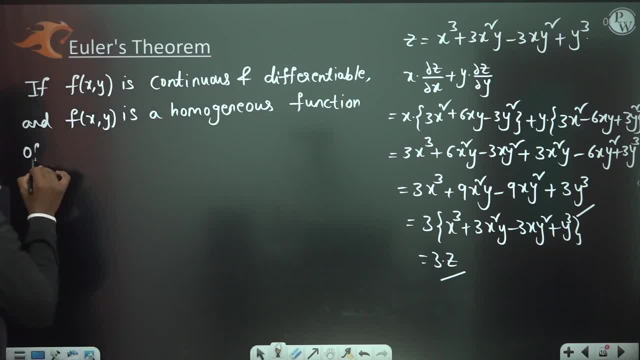 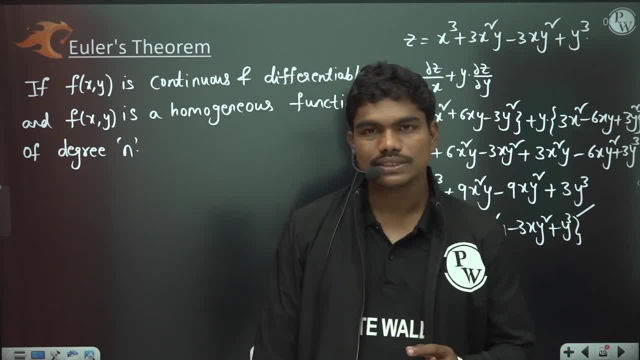 function, like i have talked about this homogeneity. when i'm talking about homogeneity, when i'm talking about homogeneity, when i'm talking about linear equations, correct. so what is linear equations correct? so what is linear equations correct? so what is homogeneous? homogeneous means having homogeneous. homogeneous means having. 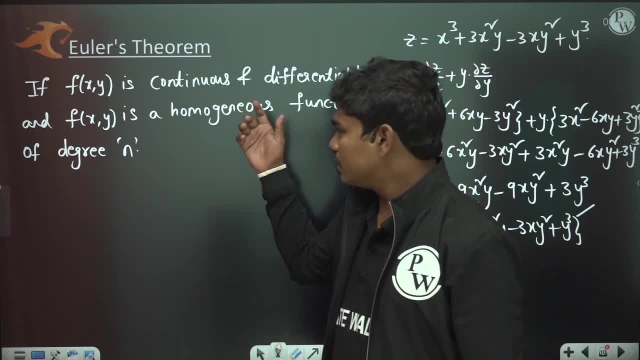 homogeneous. homogeneous means having equal uh kind of nature. so if you see equal uh kind of nature, so if you see equal uh kind of nature, so if you see the expression or this function being the expression or this function being the expression or this function being, homogeneous is if, let us suppose, if this: 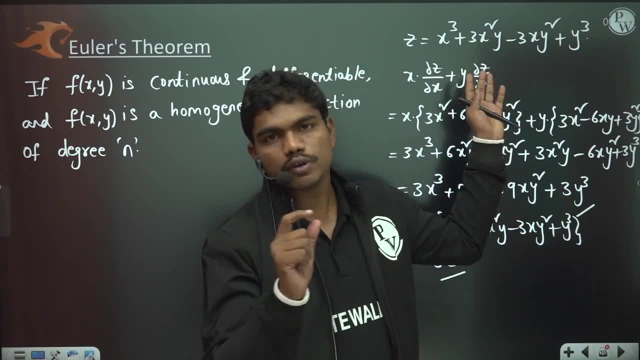 homogeneous is, if- let us suppose, if this homogeneous is, if, let us suppose, if this function has four terms, for example, function has four terms, for example, function has four terms. for example, like this: every term should be of same. like this: every term should be of same. like this: every term should be of same degree. okay, for example, if you take this: 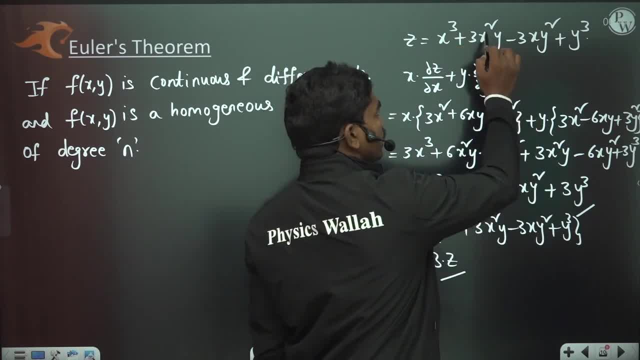 degree. okay, for example, if you take this degree. okay, for example, if you take this is third degree term. this is also third is third degree term. this is also third is third degree term. this is also third degree term, because if this you see, uh degree term, because if this you see, uh. 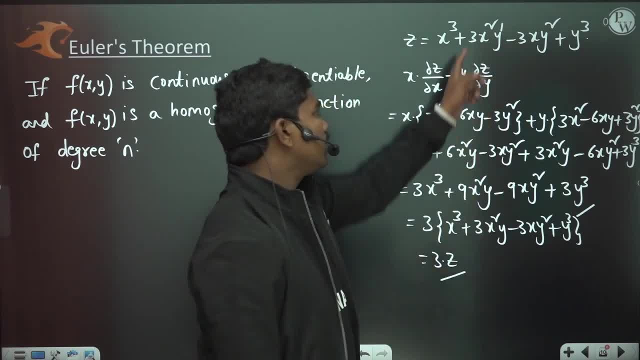 degree term, because if this you see, uh, degree of this x is 2 and degree of this degree of this x is 2, and degree of this degree of this x is 2 and degree of this y is 1, actually, so total 2 plus 1, it is. 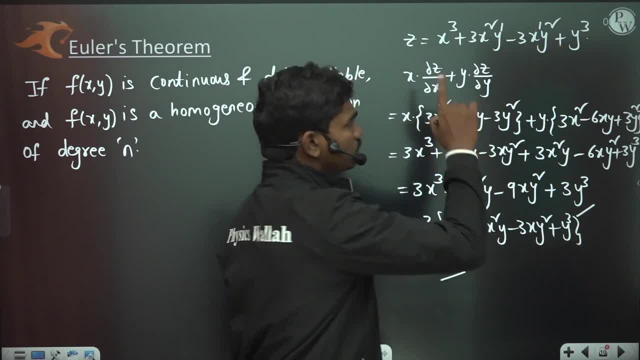 y is 1 actually, so total 2 plus 1. it is y is 1 actually, so total 2 plus 1 it is 3, 3, 3. similarly, if you take 1 here, 1 plus 2 it. similarly, if you take 1 here, 1 plus 2 it. 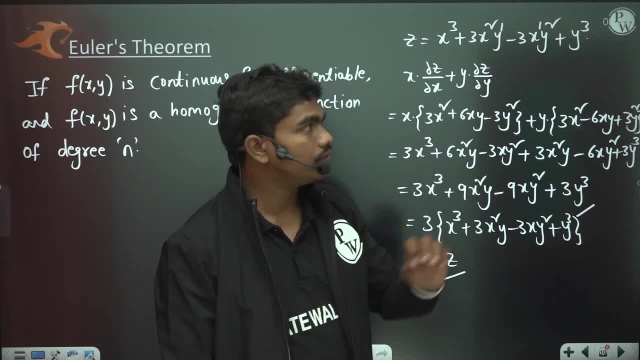 similarly, if you take 1 here, 1 plus 2, it is 3, is 3, is 3, and also we have 3 here. so that's how, if. and also we have 3 here. so that's how, if. and also we have 3 here. so that's how, if you see, we have. 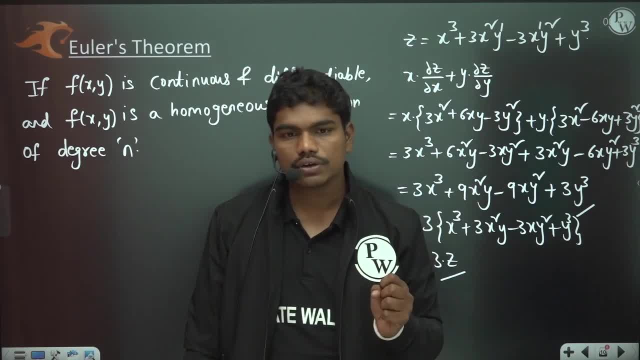 you see, we have, you see we have every term of third degree. okay. so which? every term of third degree okay, so, which? every term of third degree okay. so, which means means means, if you want to call a function as a, if you want to call a function as a, 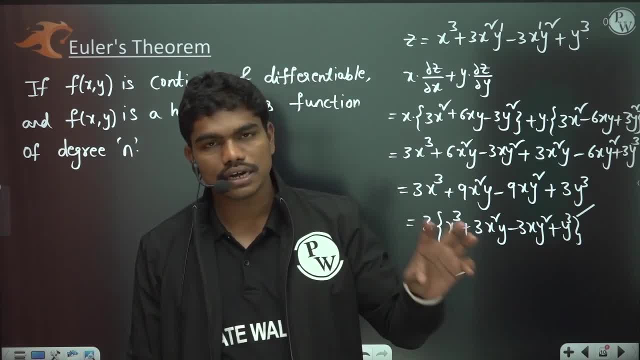 if you want to call a function as a homogeneous function, homogeneous function, homogeneous function, you should have every term in that. you should have every term in that. you should have every term in that. function of same degree- okay, it can be. function of same degree- okay, it can be. 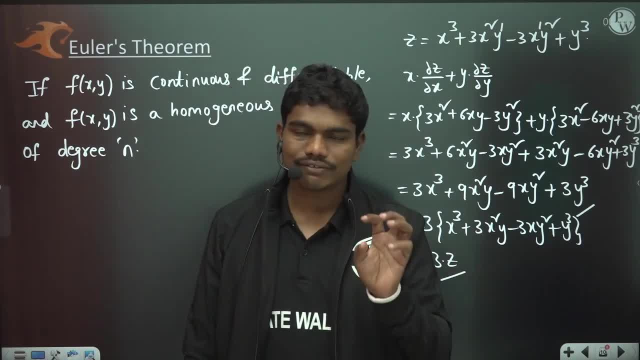 function of same degree. okay, it can be anything- three, four, five, anything, anything three, four, five, anything, anything three, four, five, anything, whatever- but every term should have the whatever, but every term should have the whatever, but every term should have the same degree. so that function is called. 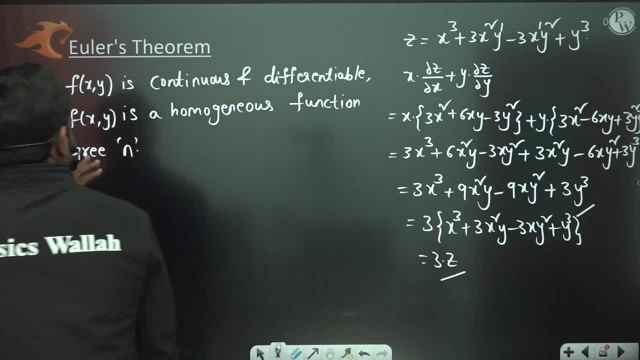 same degree, so that function is called same degree, so that function is called homogeneous function. actually okay. so if homogeneous function actually okay, so if homogeneous function actually okay. so if this is a function of degree n, then first point x into, then first point x into, then first point x into dou f by dou x plus y. 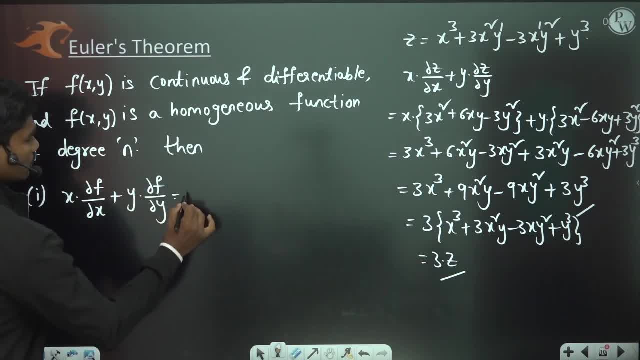 dou f by dou x plus y. dou f by dou x plus y into dou f by dou y. this value will be into dou f by dou y. this value will be into dou f by dou y. this value will be always equal to n times of f. 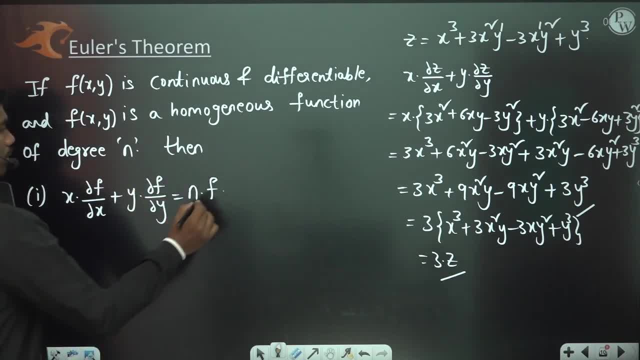 always equal to n times of f. always equal to n times of f, okay. so, if you see this is n times of f, okay. so if you see this is n times of f, okay. so if you see this is n times of f of x comma. y, you can write f of x comma. 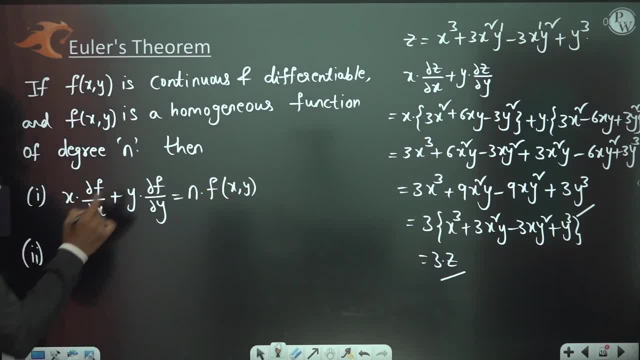 of x comma y, you can write f of x comma. of x comma y, you can write f of x comma y, and similarly y and similarly y, and similarly. let us suppose for this function, if i let us suppose for this function, if i let us suppose for this function, if i ask you to calculate, 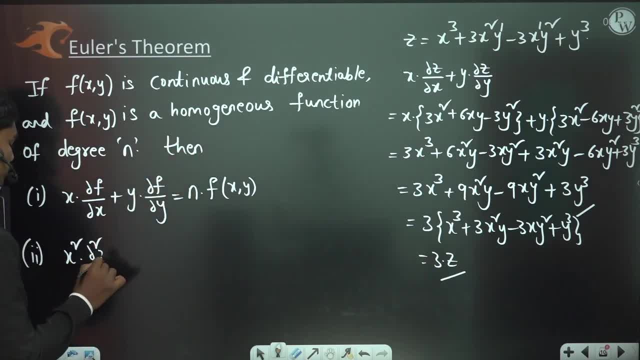 ask you to calculate. ask you to calculate this value x square into this value x square into this value x square into dou square z by dou x square. dou square z by dou x square. dou square z by dou x square, plus 2 x y times plus 2 x y times. 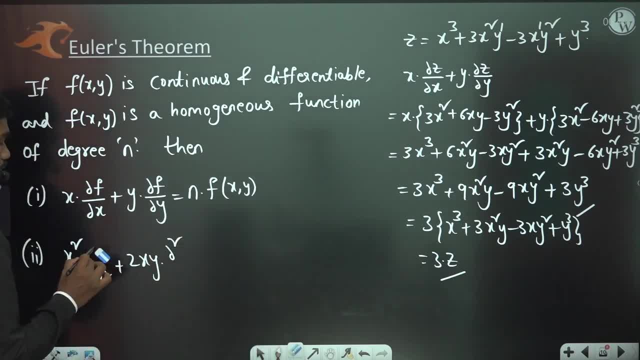 plus 2, x, y times. dou square, dou square, dou square. okay f. we are writing the definition in okay f. we are writing the definition in okay f. we are writing the definition in terms of f. so let us write f only terms of f. so let us write f only. 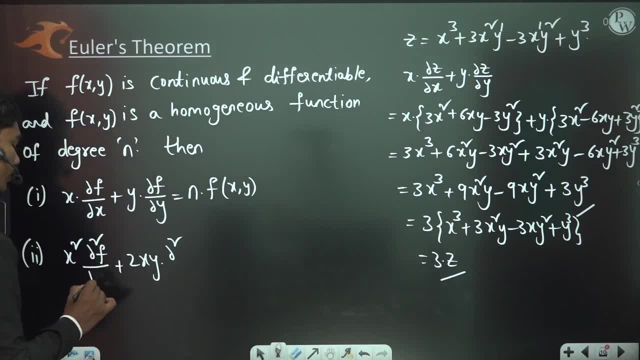 terms of f. so let us write f only so dou square f by so dou square f by so dou square f by dou x square plus 2 x y times of dou x square plus 2 x y times of dou x square, plus 2 x y times of dou square f by. 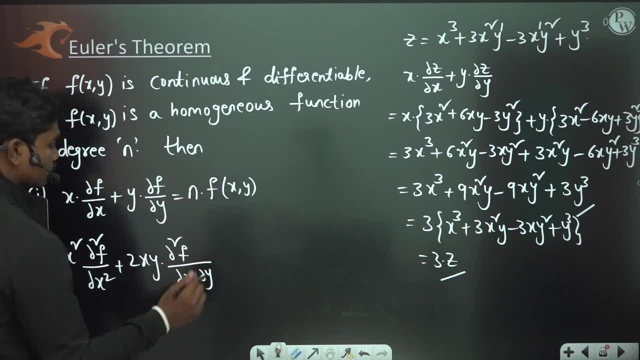 dou square f by dou, square f by dou x, dou y. or you can write dou y to x, dou x, dou y. or you can write dou y to x, dou x, dou y. or you can write dou y to x. doesn't matter, because both are equal. 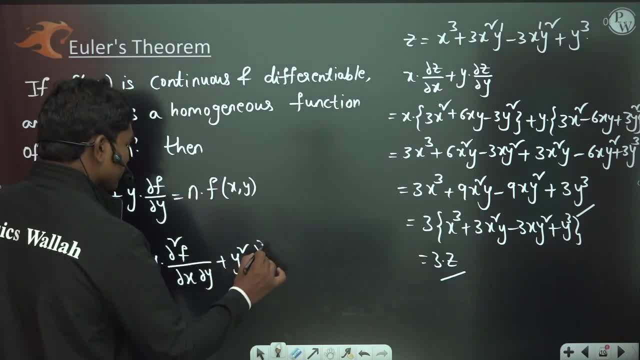 doesn't matter because both are equal. doesn't matter because both are equal plus y square times of plus y square times of plus y square times of dou square f by dou square, f by dou square f by dou y square. if you take this value, this is: 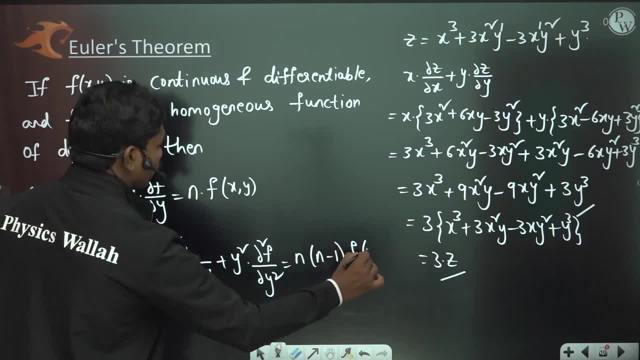 dou y square. if you take this value. this is dou y square. if you take this value, this is n into n minus one times of n into n, minus one times of n. into n, minus one times of f of x comma y actually here. okay so. f of x comma y, actually here, okay so. 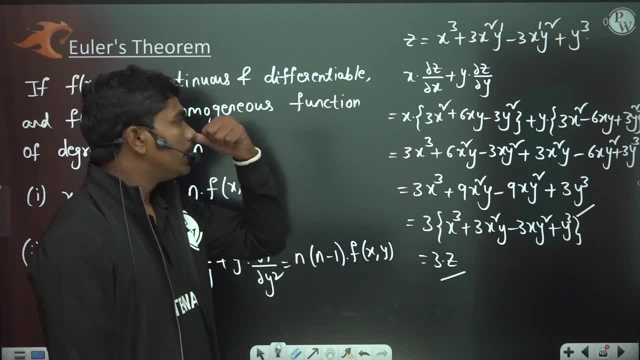 f of x comma y actually here. okay, so this is how we get the result and, as a, this is how we get the result and as a, this is how we get the result and, as a consequence- you have seen consequence, you have seen consequence. you have seen this is a third degree function. 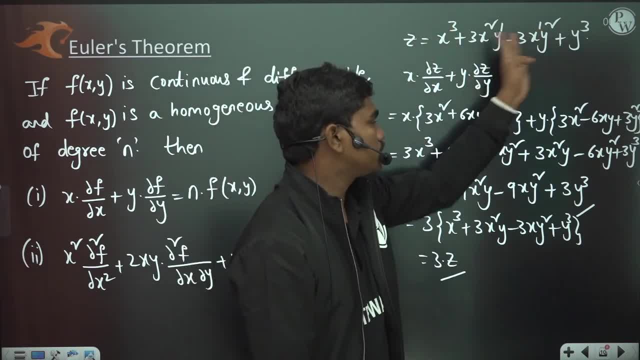 this is a third degree function. this is a third degree function. basically it's a homogeneous function. basically it's a homogeneous function. basically it's a homogeneous function because every term, four terms total. because every term, four terms total. because every term, four terms total, every term is of third degree. so if you 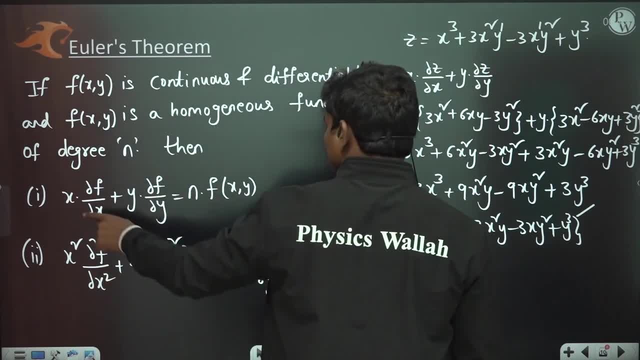 because every term, four term is of third degree. so if you, because every term, four term is of third degree. so if you see degree is three, so from euler's see degree is three. so from euler's see degree is three, so from euler's theorem you should know that. as for the 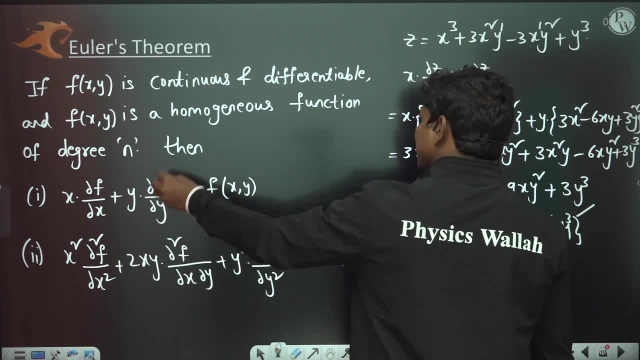 theorem. you should know that. as for the theorem, you should know that, as for the first point, what i have written x into first point, what i have written x into first point, what i have written x into dou f by dou x plus y into dou f by. 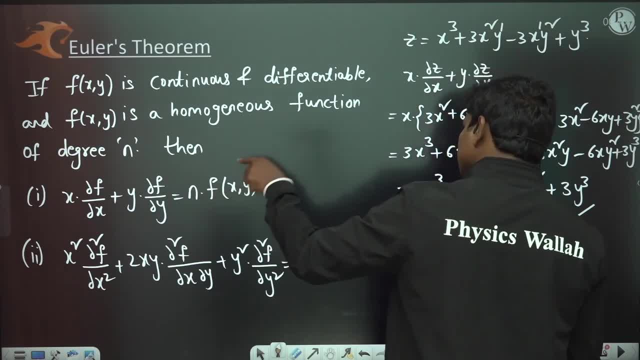 dou f by dou x plus y into dou f by dou f by dou x plus y into dou f by dou y. this is definitely equal to the degree dou y. this is definitely equal to the degree dou y. this is definitely equal to the degree times that function. so if you see, 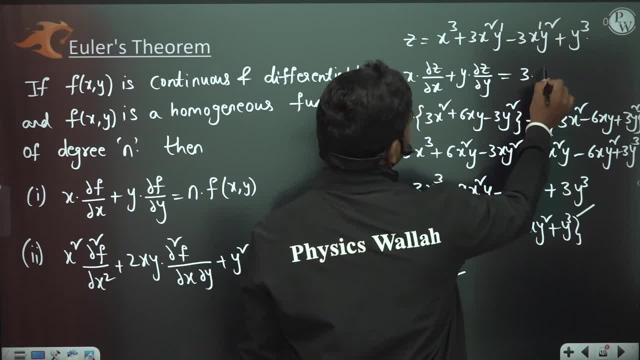 times that function. so if you see times that function, so if you see, if you know this theme, you will directly, if you know this theme, you will directly, if you know this theme, you will directly know that this is going to be three, know that this is going to be three. 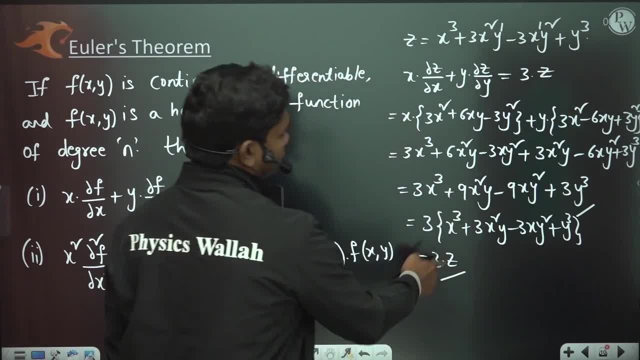 know that this is going to be three times of this function z, which is the times of this function z, which is the times of this function z, which is the same thing that you got here after doing same thing that you got here after doing same thing that you got here after doing certain calculation. okay, so that's how. 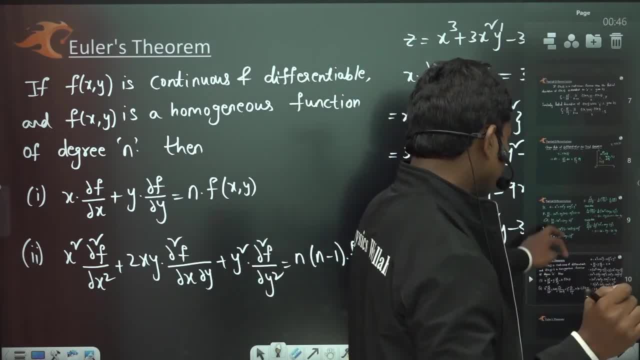 certain calculation. okay, so that's how. certain calculation. okay, so that's how. this result is actually uh, one very. this result is actually uh, one very. this result is actually uh, one very important result, of course. so now, if you, important result, of course. so now, if you. 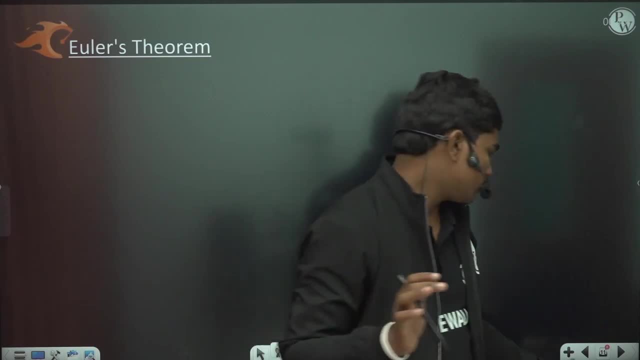 important result, of course. so now, if you see, see, see, let us talk about one more, uh, you know, let us talk about one more, uh, you know, let us talk about one more, uh, you know. understanding here. so sometimes the understanding here, so sometimes the understanding here, so sometimes the functions can be. 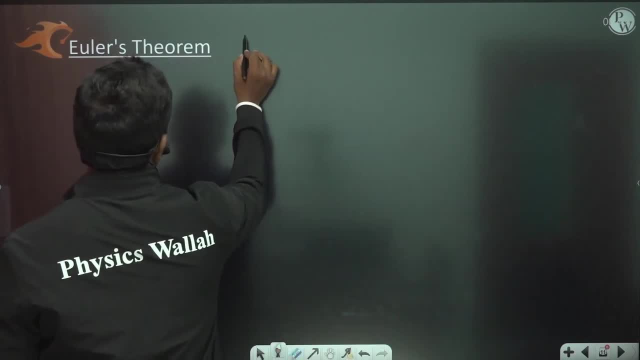 functions can be. functions can be: uh, you know something different, like for. uh, you know something different like for. uh, you know something different like, for example: let us suppose if i have the example, let us suppose if i have the example, let us suppose if i have the function, z is equal to. 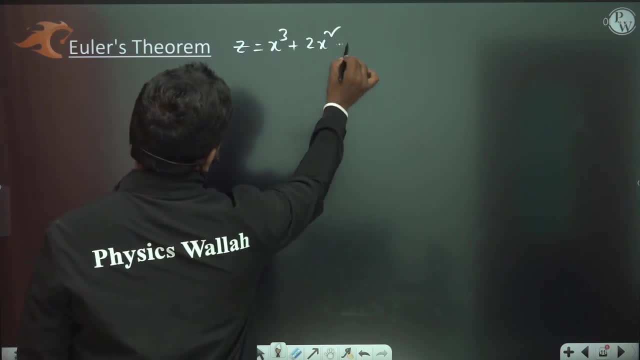 function z is equal to function z is equal to x cube plus 2 x square. x cube plus 2 x square. x cube plus 2 x square plus 9 y power 4: like this: okay for. plus 9 y power 4: like this: okay for. 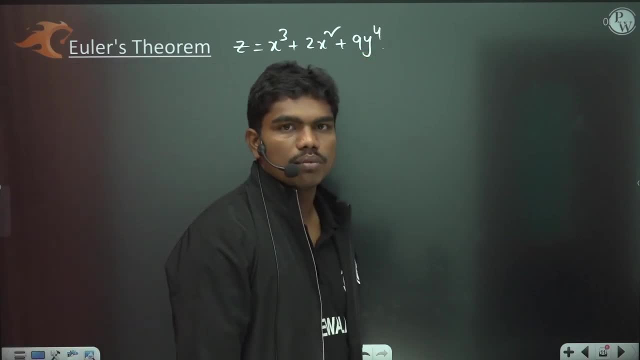 plus 9 y power 4, like this: okay, for example, let us suppose if this is example. let us suppose if this is example, let us suppose if this is function now, if you see function now, if you see function now, if you see this is a non-homogeneous function, okay, it's. this is a non-homogeneous function. okay, it's. this is a non-homogeneous function. okay, it's a non-homogeneous function. clearly a non-homogeneous function. clearly a non-homogeneous function. clearly so, because this is third degree second. so because this is third degree second. 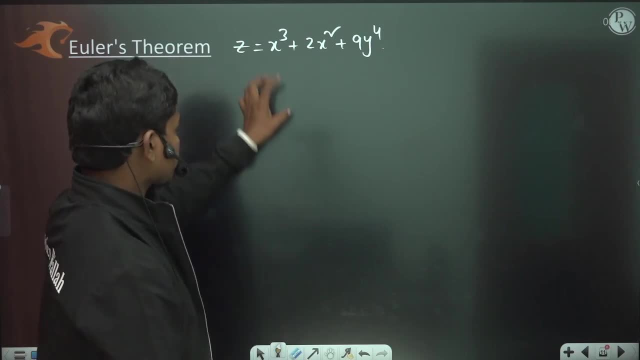 so, because this is third degree, second degree and fourth degree, degree and fourth degree degree and fourth degree, but individually, if you see i can take, but individually, if you see i can take, but individually if you see i can take this as sum of three functions, this as sum of three functions. 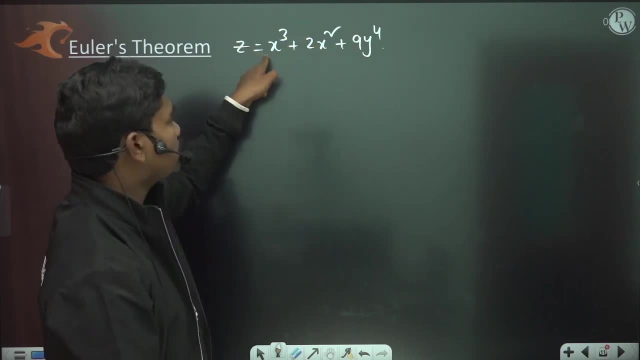 this as sum of three functions: one, two and three- correct. i can write i one, two and three. correct. i can write i one, two and three. correct. i can write. i can write, can write, can write this z as sum of three functions actually. this z as sum of three functions actually. 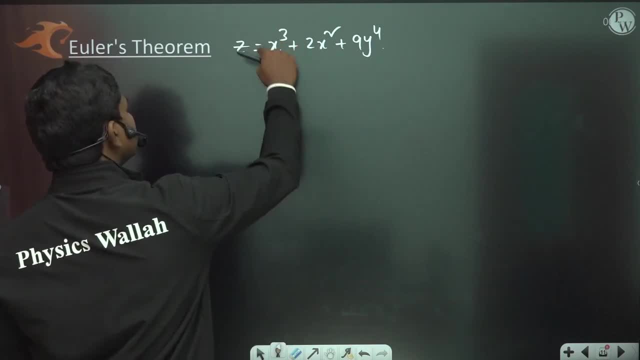 this z as sum of three functions. actually, now, if i write this z as sum of three, now, if i write this z as sum of three, now, if i write this z as sum of three functions, now every function itself is a functions. now, every function itself is a. 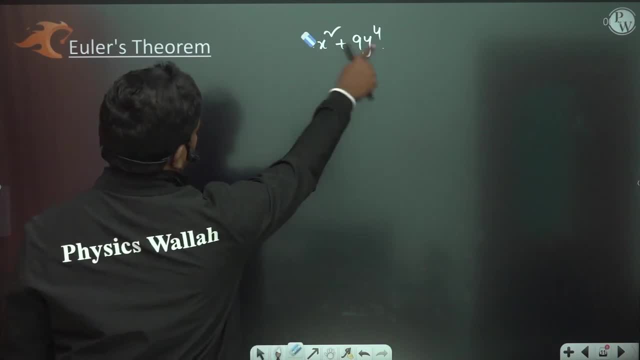 functions. now, every function itself is a homogeneous function, actually okay, so, homogeneous function, actually okay, so, homogeneous function, actually okay, so, anyhow, let me define what is this. anyhow, let me define. what is this. anyhow, let me define what is this. homogeneous function also, you will get. homogeneous function also, you will get. 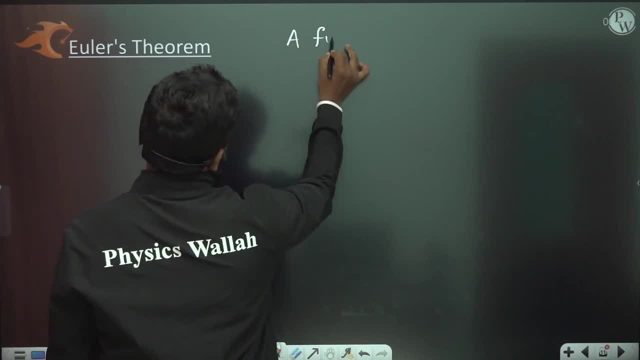 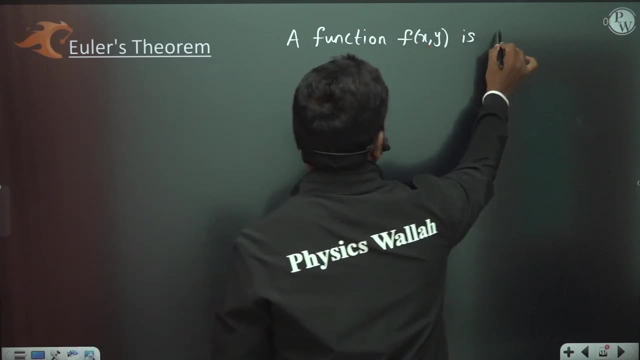 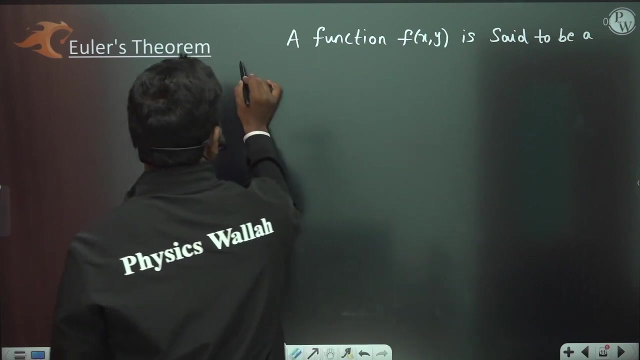 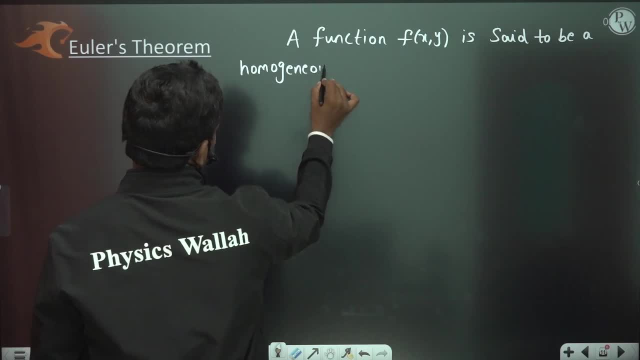 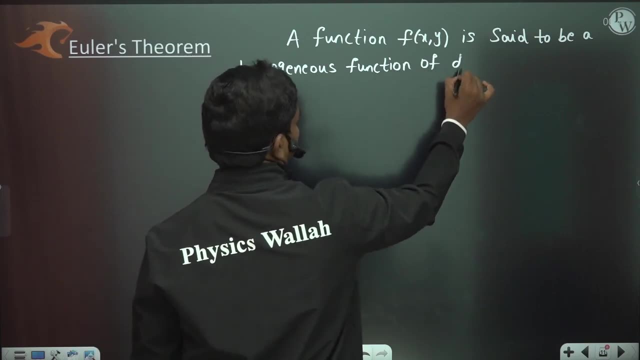 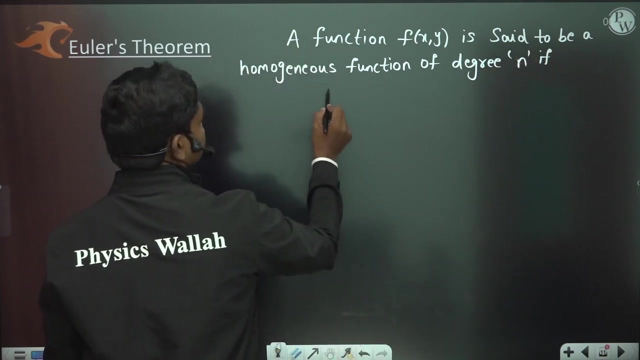 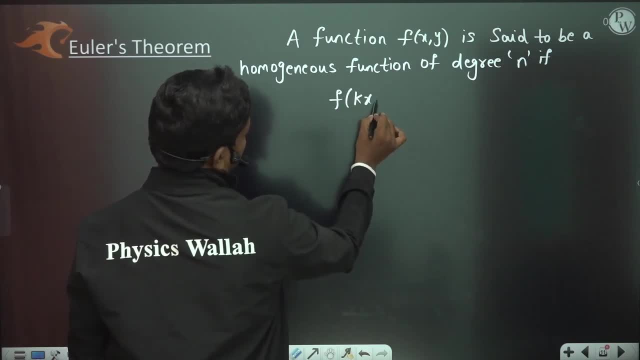 if of if, of if of x comma k, x comma k y means. let us x comma k, x comma k y means. let us x comma k, x comma k y means. let us suppose in place of x, you have substituted. suppose in place of x, you have substituted. 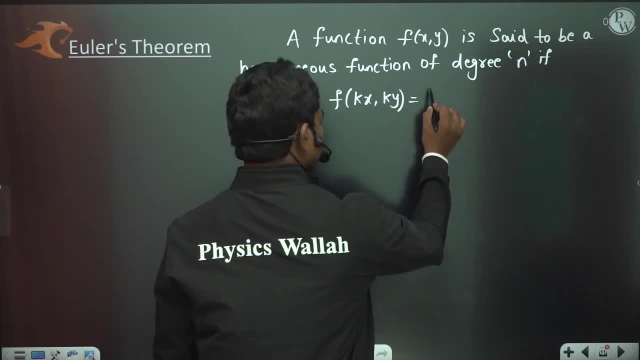 suppose, in place of x you have substituted k x and in place of y you have k x, and in place of y you have k x, and in place of y you have substituted k y. this can be taken out as: substituted k y. this can be taken out as: 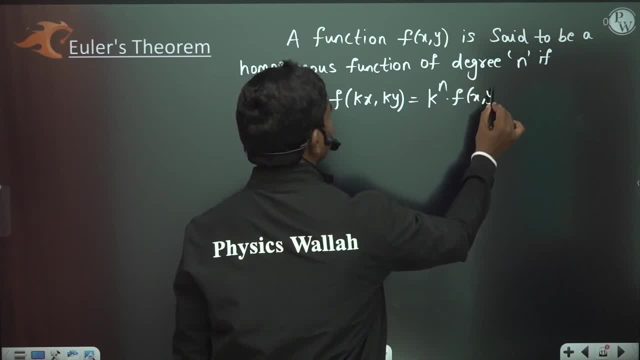 substituted k y. this can be taken out as k power n times of k power n times of k power n times of f of x comma y. obviously, because, if you f of x comma y, obviously because if you f of x comma y, obviously because, if you see, let us suppose, if you take this, 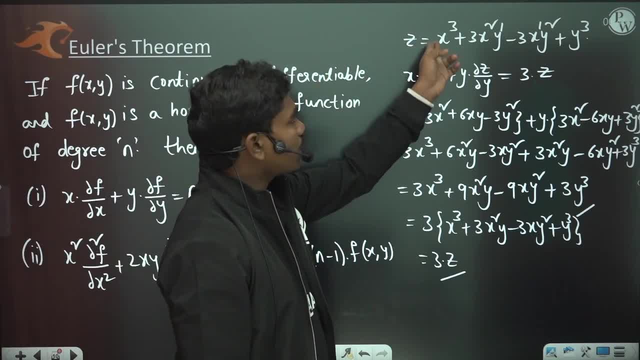 see, let us suppose if you take this. see, let us suppose, if you take this equation here, if you take uh in place of equation here, if you take uh in place of equation here, if you take uh in place of x, if you substitute k, x and in place of y. 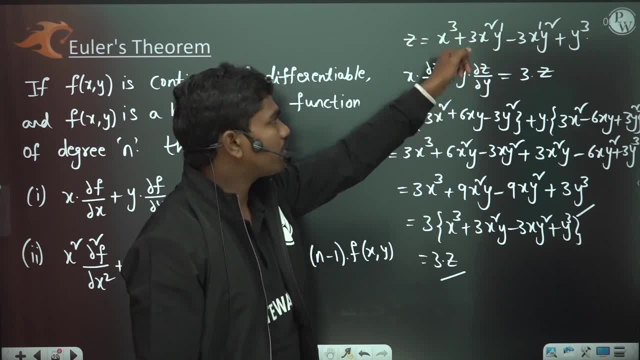 x. if you substitute k x and in place of y x. if you substitute k x and in place of y. if you substitute k y all over this, if you substitute k y all over this, if you substitute k y all over this expression, then you would have taken a k. 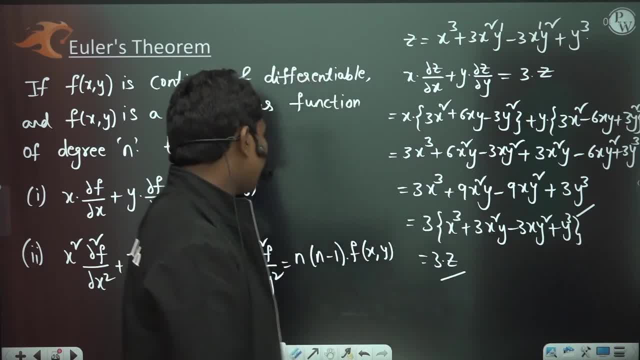 expression, then you would have taken a k expression. then you would have taken a k. cube times of this value again: okay. so cube times of this value again, okay. so cube times of this value again- okay. so that's how we can identify that it's a. that's how we can identify that it's a. 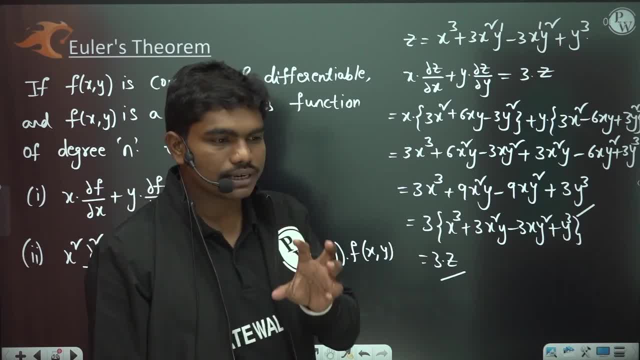 that's how we can identify that it's a third degree function. because every term third degree function, because every term third degree function, because every term, every term in a homogeneous equation, every term in a homogeneous equation, every term in a homogeneous equation, should be of some degree, definitely. and 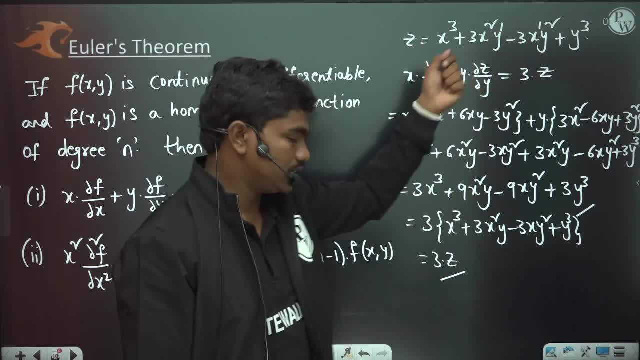 should be of some degree definitely, and should be of some degree definitely. and here all the terms are equal. so that's here all the terms are equal. so that's here all the terms are equal. so that's why we are calling it a homogeneous, why we are calling it a homogeneous. 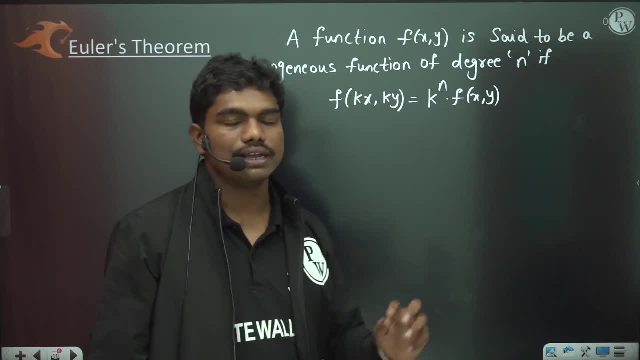 why we are calling it a homogeneous equation. so normally in general. this is equation, so normally in general. this is equation, so normally in general. this is how you can identify if you have some. how you can identify if you have some. how you can identify if you have some function if you replace X with K, X and Y. 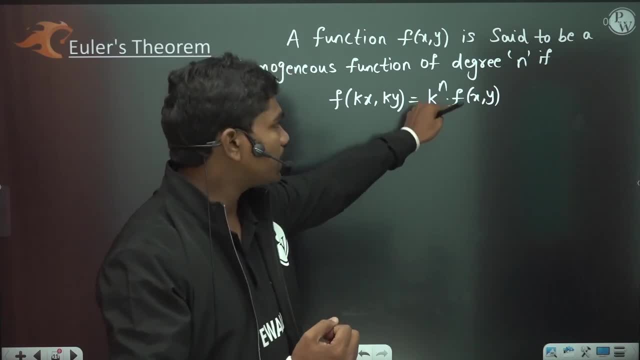 function if you replace X with K, X and Y function if you replace X with K, X and Y with K Y. if you can take out some K power with K Y, if you can take out some K power with K Y, if you can take out some K power n times of that function again, then we 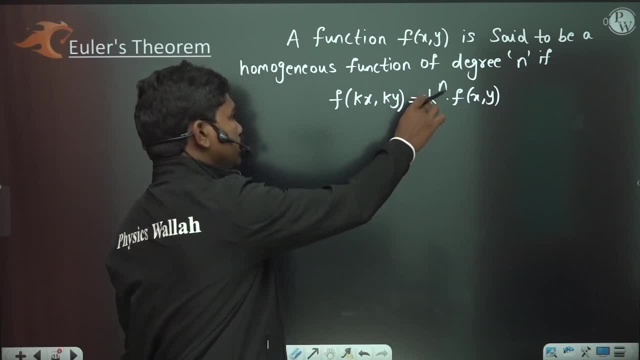 n times of that function again. then we n times of that function again. then we say it's a homogeneous function and the say it's a homogeneous function and the say it's a homogeneous function and the degree of homogeneity is basically this. degree of homogeneity is basically this. 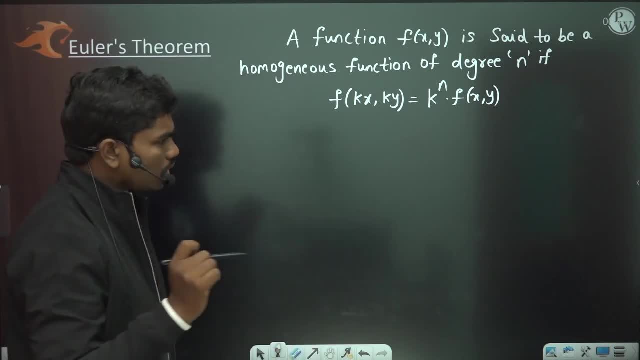 degree of homogeneity is basically this: small n which we are writing there, okay. small n which we are writing there, okay. small n which we are writing there, okay, now, let us try to calculate something now. let us try to calculate something now. let us try to calculate something here. so this is the function, basically. 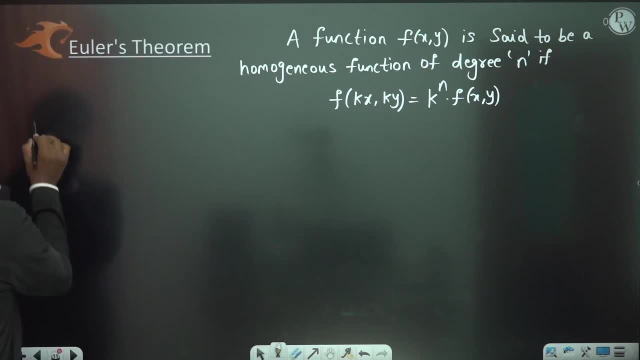 here. so this is the function basically here. so this is the function basically now. if you observe one thing, if now, if you observe one thing, if now, if you observe one thing, if f of X comma Y is equal to some functions, f of X comma Y is equal to some functions. 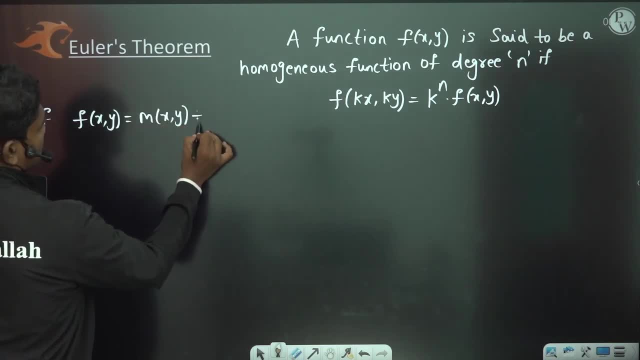 f of X comma Y is equal to some functions. say M of X comma Y plus n of X comma Y. say M of X comma Y plus n of X comma Y. say M of X comma Y plus n of X comma Y plus p times of X comma Y. so let us 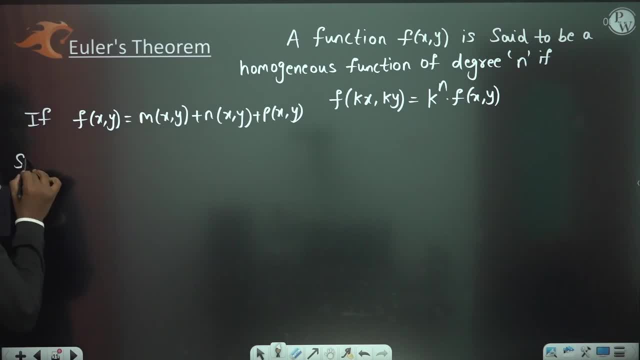 plus p times of X comma Y. so let us plus p times of X comma Y. so let us suppose it has three different functions. suppose it has three different functions. suppose it has three different functions, some such that such that M of X comma Y, some such that such that M of X comma Y. 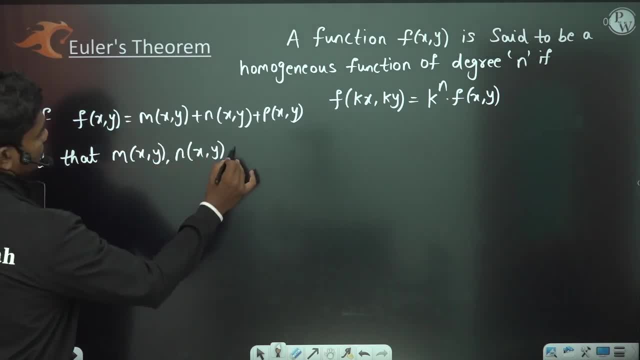 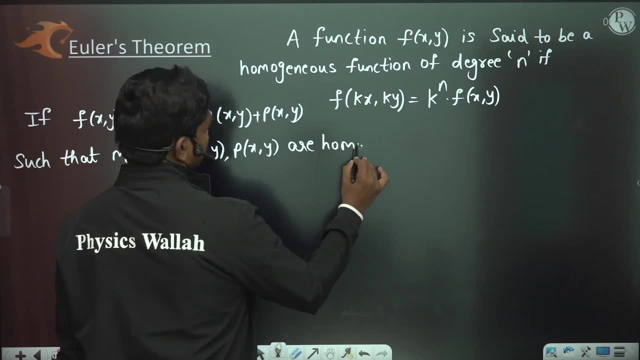 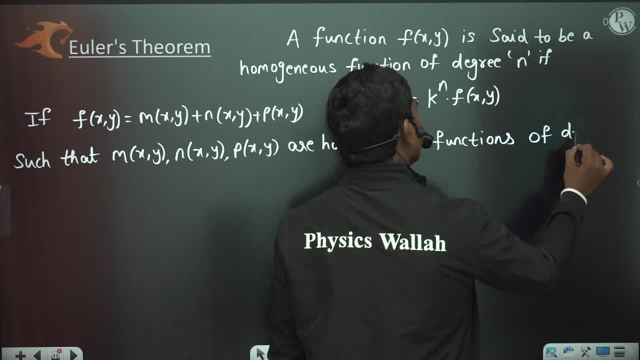 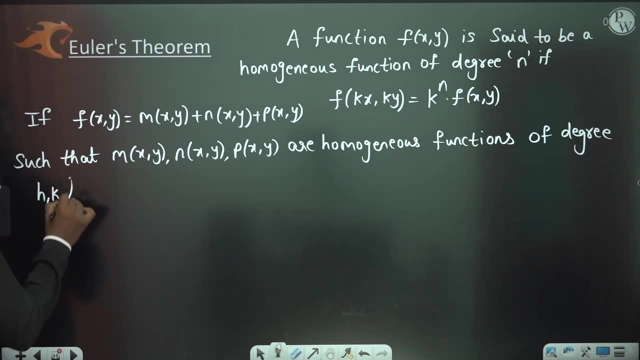 are homogeneous. functions are homogeneous. functions of degree are homogeneous. functions of of degree are homogeneous. functions of of degree are homogeneous. functions of degree, of degree, degree of degree, degree of degree H K, L, for example. okay of degree H K. H K L, for example. okay of degree H K. 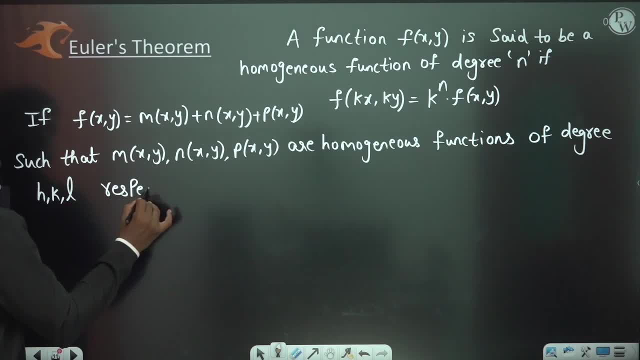 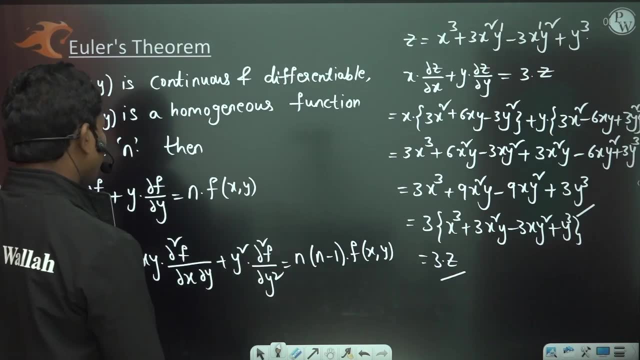 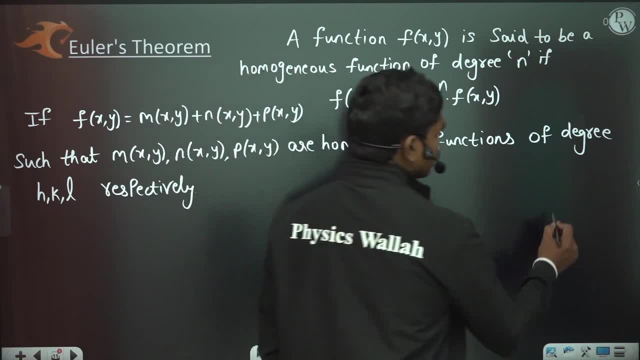 what I have given you. okay, I think I, what I have given you, okay, I think I raised it. so if I give you some example, raised it. so if I give you some example, raised it. so if I give you some example, like Z is equal to just now, I have given. 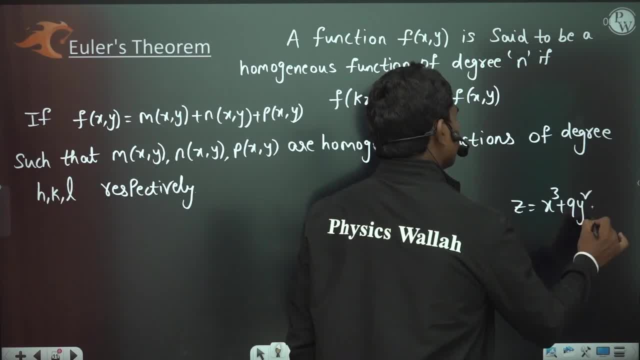 like Z is equal to just now. I have given like Z is equal to just now. I have given you X cube plus some 9y square. let us you X cube plus some 9y square. let us you X cube plus some 9y square. let us say, plus some 2z power for, 2x power for. 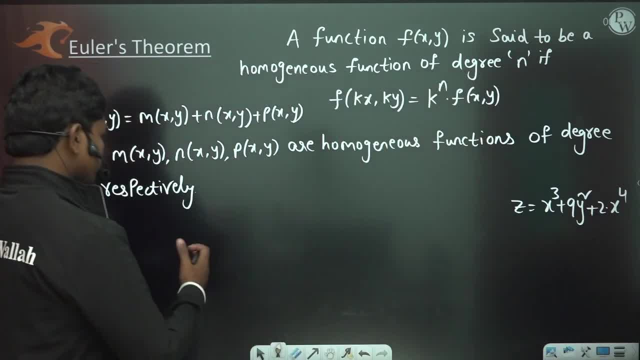 say, plus some 2z power for 2x power for, say, plus some 2z power for 2x power for something like this. okay, so here. if you something like this. okay, so here, if you something like this. okay, so here. if you see, this is some of the functions, but 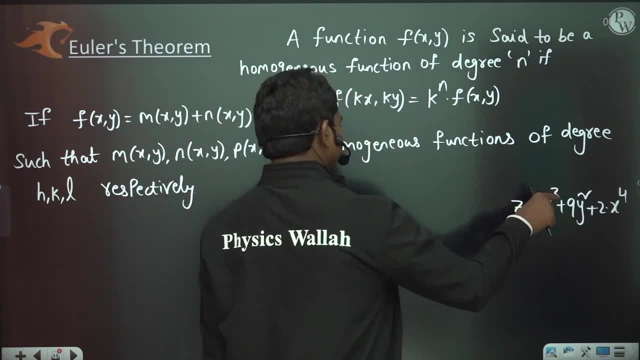 see, this is some of the functions. but see, this is some of the functions. but these three are individually homogeneous. these three are individually homogeneous. these three are individually homogeneous functions because if you take only X cube functions, because if you take only X cube functions, because if you take only X cube, if you substitute K, X, then you can take. 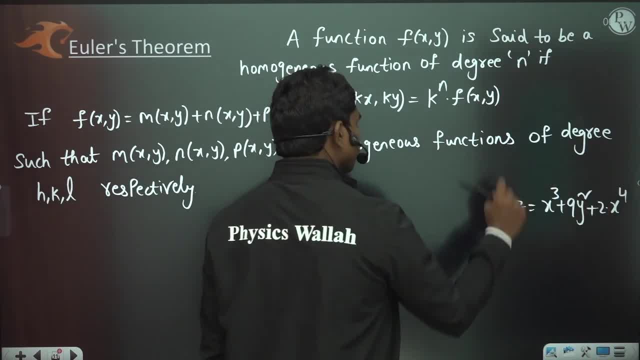 if you substitute K X, then you can take. if you substitute K X, then you can take K cube into X cube. similarly, this is K K cube into X cube. similarly, this is K K cube into X cube. similarly, this is K square and here you get K power for so. 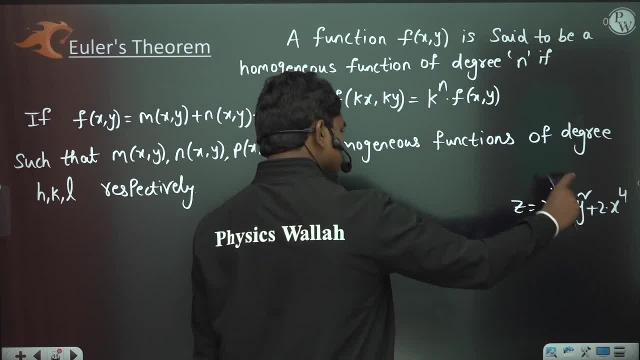 square, and here you get K power for so square, and here you get K power for so individually. this is a homogeneous individually. this is a homogeneous individually. this is a homogeneous function of degree 3. this is a function of degree 3. this is a function of degree 3. this is a homogeneous function of degree 2 and this. 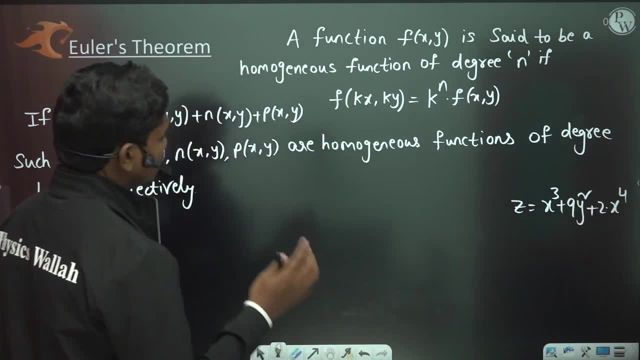 homogeneous function of degree 2 and this homogeneous function of degree 2 and this is homogeneous function of degree 4. so is homogeneous function of degree 4, so is homogeneous function of degree 4. so if you see these are different functions, if you see these are different functions. 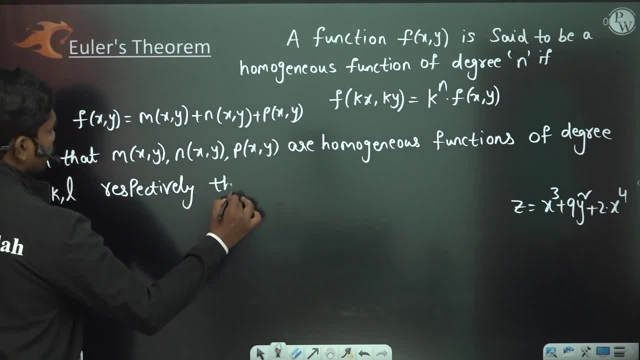 if you see these are different functions, actually okay respectively, then then actually okay respectively. then then actually okay respectively. then then first point is: X into dou f by dou x. first point is: X into dou f by dou x. first point is X into dou f by dou x plus y into dou f by dou y. so this value. 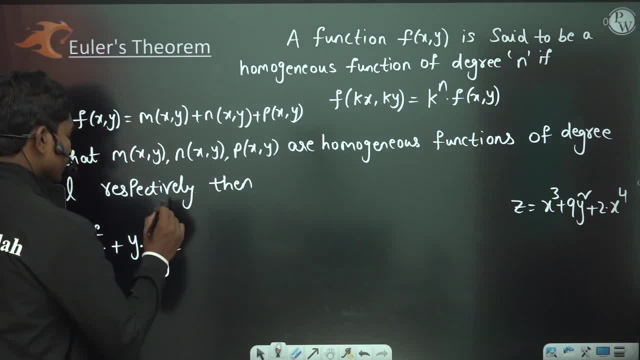 plus y into dou f by dou y. so this value plus y into dou f by dou y. so this value is going to be: how much is this? so this is going to be? how much is this so this is going to be? how much is this? so this is equal to now, since this f consists of: 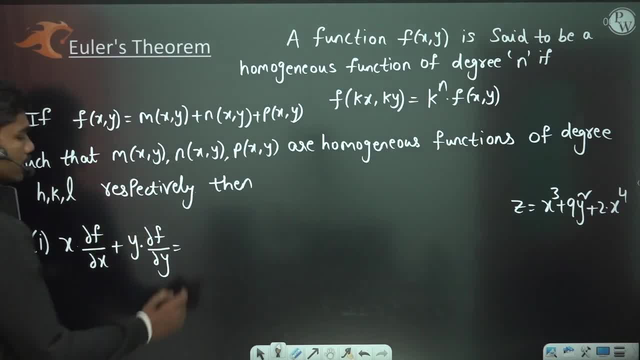 is equal to now, since this f consists of is equal to now, since this f consists of some individual functions. you can write some individual functions. you can write some individual functions. you can write it like this: okay, so X times of dou by. it like this: okay, so X times of dou by. 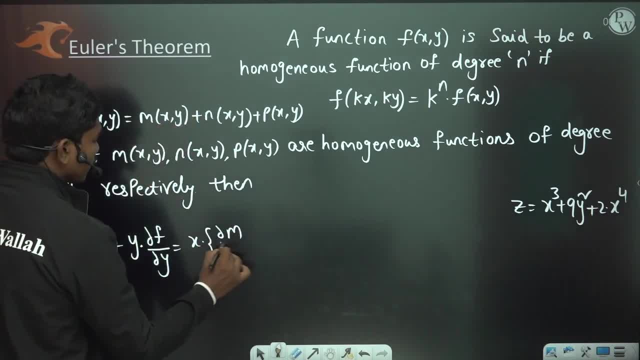 it like this: okay, so X times of dou by dou x of f means this value, which means dou x of f. means this value, which means dou x of f. means this value, which means dou m by dou x plus dou n by dou x plus dou m by dou x plus dou n by dou x plus. 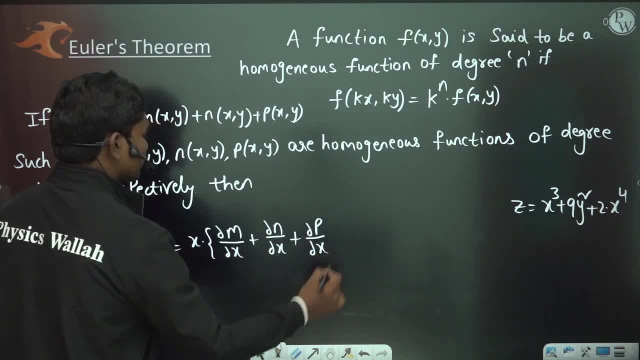 dou m by dou x, plus dou n by dou x, plus dou p by dou x. these are the functions dou p by dou x. these are the functions dou p by dou x. these are the functions plus y times of dou m by dou y, because, plus y times of dou m by dou x, because. 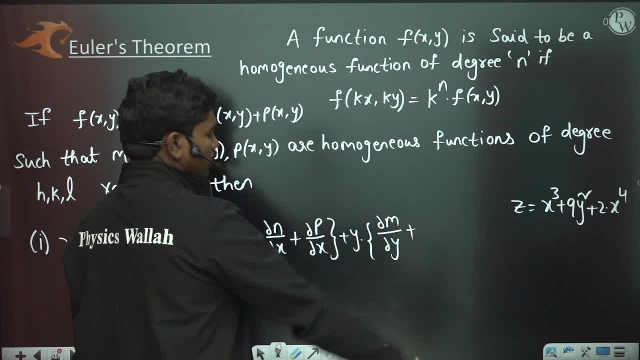 plus y times of dou m by dou x, because dou f by dou y is nothing but dou by dou. dou f by dou y is nothing but dou by dou. dou f by dou y is nothing but dou by dou y of m plus n plus p, so we can separate. 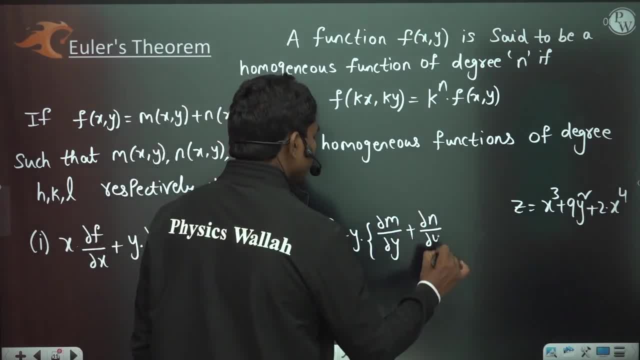 y of m plus n plus p, so we can separate y of m plus n plus p. so we can separate that at different terms. okay, so dou n by that at different terms. okay, so dou n by that at different terms. okay, so dou n by dou y plus dou p by dou y. so this is. 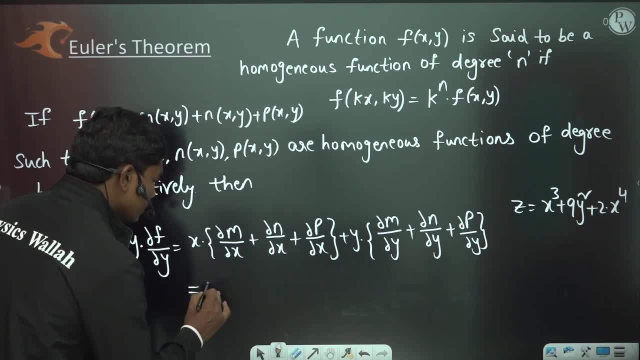 dou y plus dou p by dou y. so this is dou y plus dou p by dou y. so this is what we have now. if you segregate the what we have now, if you segregate the what we have now, if you segregate the terms slightly, what you will get X into 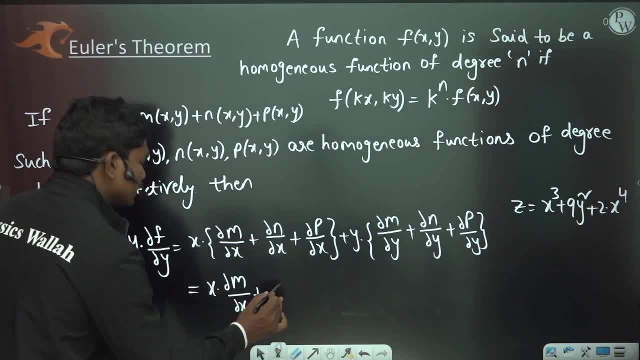 terms slightly what you will get X into terms slightly, what you will get X into: dou m by dou x plus y times of dou m by dou m by dou x plus y times of dou m by dou m by dou x plus y times of dou m by dou y, y times of dou m by dou y. this is: 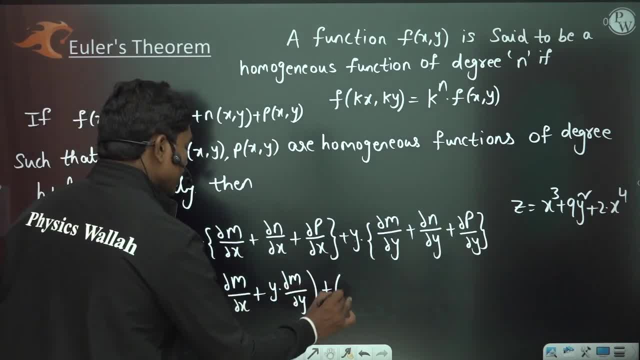 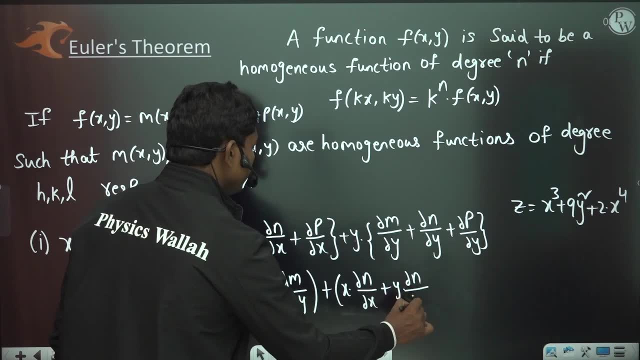 dou y times of dou m by dou y. this is dou y times of dou m by dou y. this is what you have: a single term plus again. what you have a single term plus again. what you have a single term plus again X into dou n by dou x plus y into dou n. 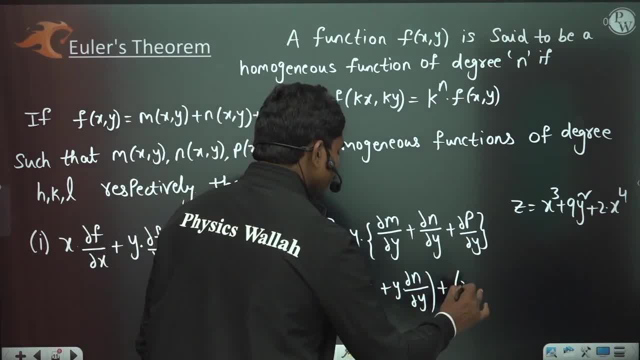 X into dou n by dou x plus y into dou n. X into dou n by dou x plus y into dou n by dou y. this is one term plus X into by dou y. this is one term plus X into by dou y- this is one term plus X into dou p by dou x plus y into. 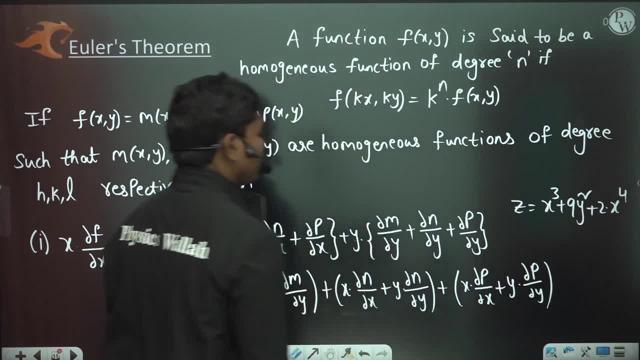 dou p by dou x plus y into by dou p, by dou x plus y, into dou p by dou y. so this is what you have now tell dou p by dou y. so this is what you have now tell dou p by dou y. so this is what you have now tell me one thing you know. 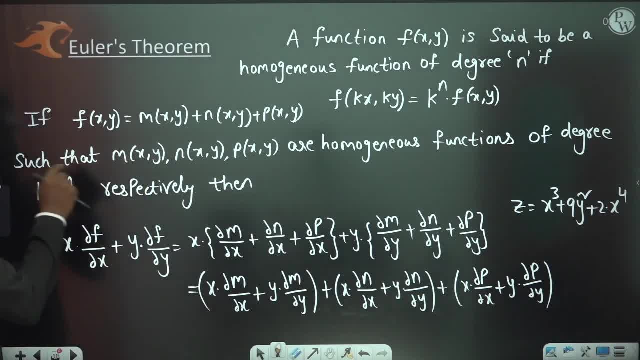 me one thing. you know me one thing. you know individually that this is a homogeneous individually, that this is a homogeneous individually, that this is a homogeneous function of degree K. I mean H. this n is function of degree K. I mean H. this n is function of degree K. I mean H. this n is a homogeneous function of degree K. and 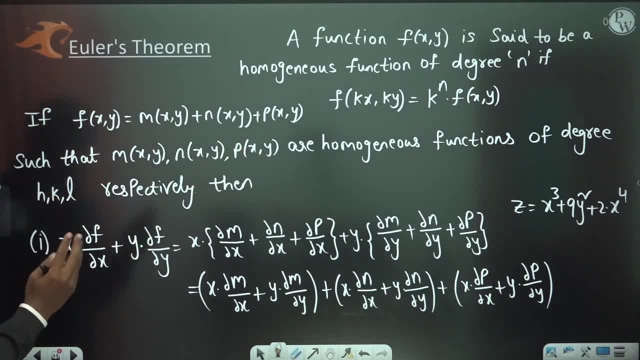 a homogeneous function of degree K and a homogeneous function of degree K. and this P is a homogeneous function of degree. this P is a homogeneous function of degree. this P is a homogeneous function of degree L. so if these are homogeneous functions, L, so if these are homogeneous functions, 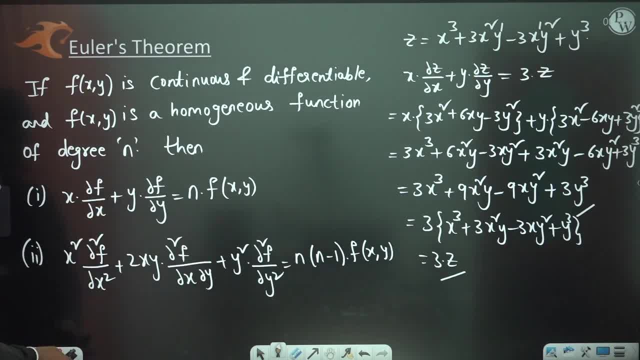 L. so if these are homogeneous functions, then as per this oil is first, you know, then as per this oil is first you know, then as per this oil is first, you know, this first statement, you can write this, this first statement. you can write this, this first statement. you can write this, as if this M is a homogeneous function. 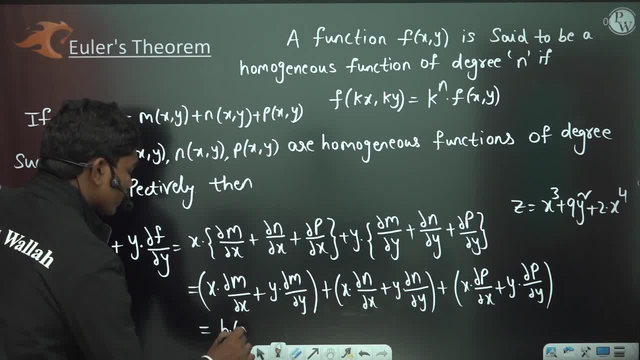 as if this M is a homogeneous function. as if this M is a homogeneous function of degree H, I can add this as H times of of degree H. I can add this as H times of of degree H. I can add this as H times of M plus, if this n is a homogeneous. 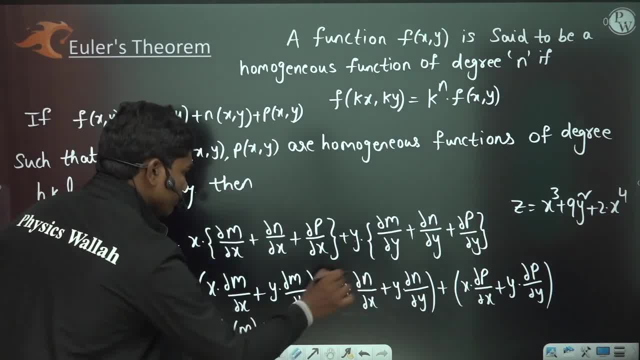 M plus. if this n is a homogeneous M plus. if this n is a homogeneous function of degree K, I can write K times function of degree K. I can write K times function of degree K. I can write K times of n for the second term, similarly plus. 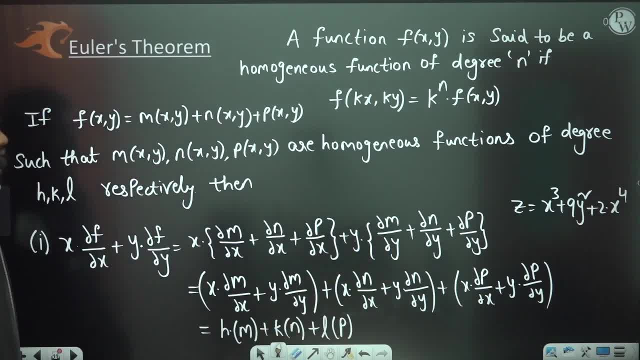 of n for the second term, similarly, plus of n for the second term, similarly, plus L times of P for the third term. okay, so L times of P for the third term. okay, so L times of P for the third term. okay, so that's how you can see whenever they are. 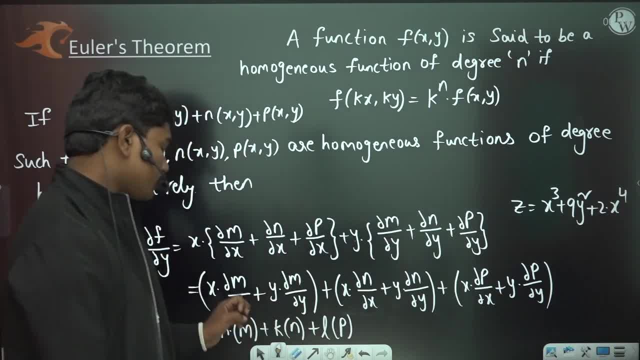 that's how you can see whenever they are. that's how you can see whenever they are of individual homogeneities. you can of individual homogeneities. you can of individual homogeneities. you can always convert that into H of M plus K of. always convert that into H of M plus K of. 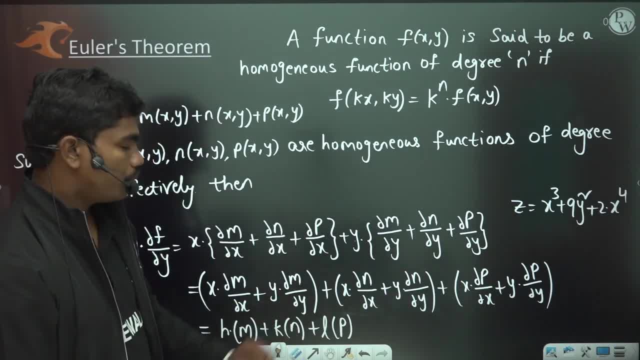 always convert that into H of M plus K of N plus L times of I mean L into P, N plus L times of I mean L into P, N plus L times of I mean L into P. actually here, okay, so that's how. if you actually here, okay, so that's how. if you. 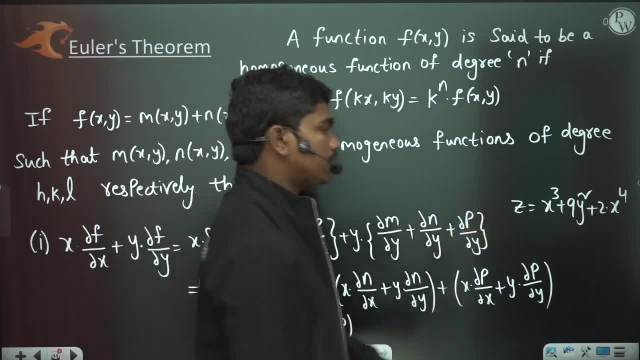 actually here. okay, so that's how. if you do this calculation for this question, do this calculation for this question, do this calculation for this question, definitely you might have got your. definitely you might have got your. definitely you might have got your answers. if you have calculated X into, 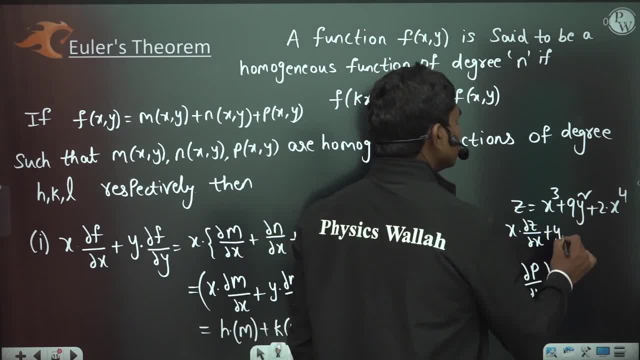 answers: if you have calculated X into. answers: if you have calculated X into: does it by 2x plus y into: does it read: does it by 2x plus y into: does it read: does it by 2x plus y into: does it read over: if you have calculated this, you: 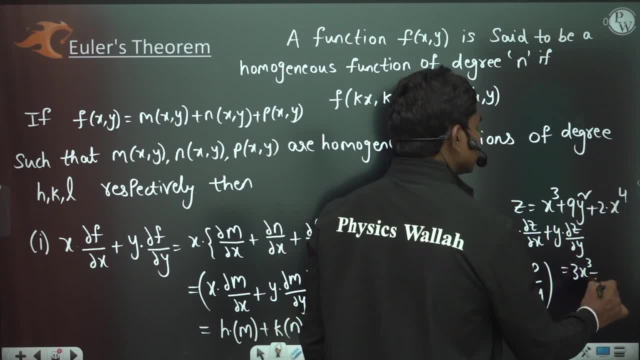 over. if you have calculated this, you over. if you have calculated this, you would have got the answer like 3 times of. would have got the answer like 3 times of. would have got the answer like 3 times of X cube plus 18 times of y square plus 8. 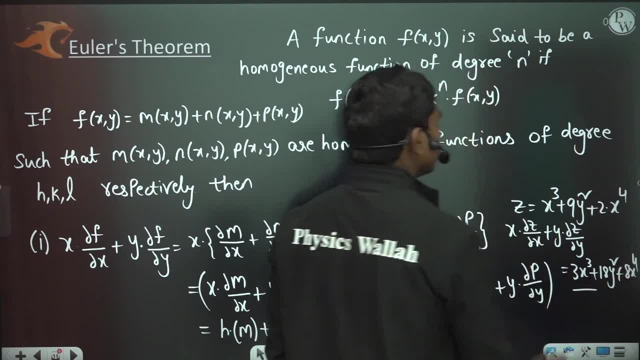 X cube plus 18 times of y square plus 8 X cube plus 18 times of y square plus 8 times of X power 4. this is what you might times of X power 4. this is what you might times of X power 4. this is what you might have got actually. okay, if you have. 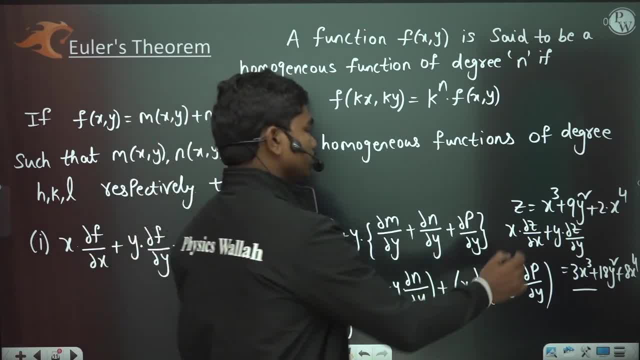 have got actually okay if you have have got actually okay if you have calculated that expression. because this is calculated that expression, because this is calculated that expression, because this is a homogeneous function of degree 3, so a homogeneous function of degree 3, so a homogeneous function of degree 3, so 3 times of this X cube plus this is a. 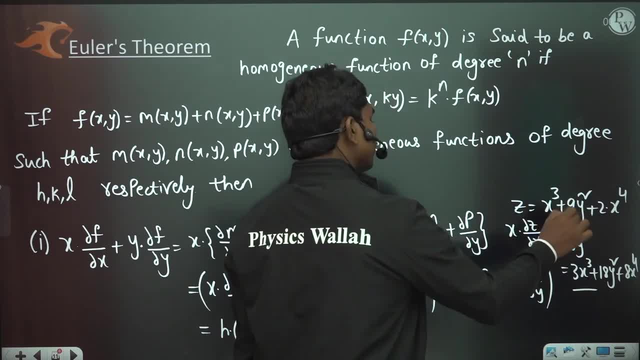 3 times of this X cube plus. this is a 3 times of this X cube plus. this is a homogeneous function of degree 2, so 2. homogeneous function of degree 2, so 2. homogeneous function of degree 2, so 2 times of 9 y square, which is 18 y. 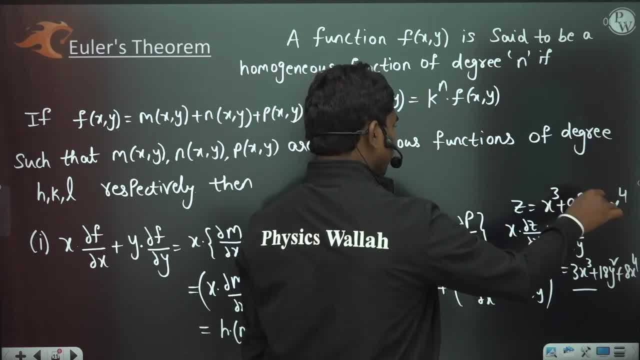 times of 9 y square, which is 18, y times of 9 y square, which is 18 y square plus this will get n value as 4, so square plus this will get n value as 4, so square plus this will get n value as 4, so 8 times of X power 4. so this is how we. 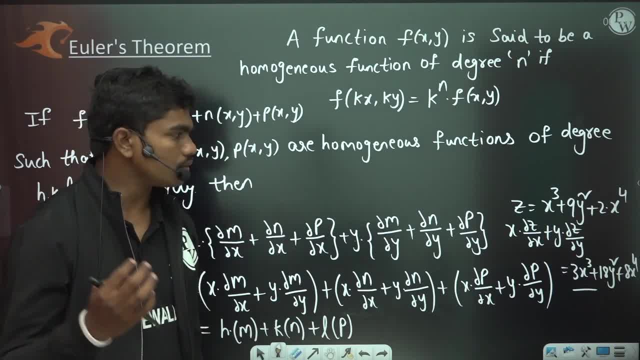 8 times of X power 4. so this is how we 8 times of X power 4. so this is how we get the values actually here in this. get the values actually here in this. get the values actually here in this case. okay, so I hope it's clear to you. 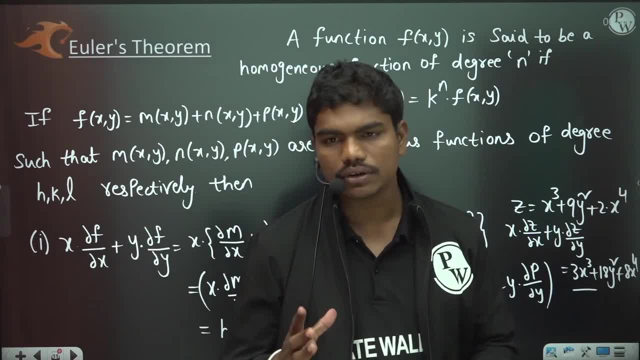 case: okay, so I hope it's clear to you. case. okay, so I hope it's clear to you. till this part: okay, so this is how we till this part. okay, so this is how we till this part. okay, so this is how we actually calculate or we define this. 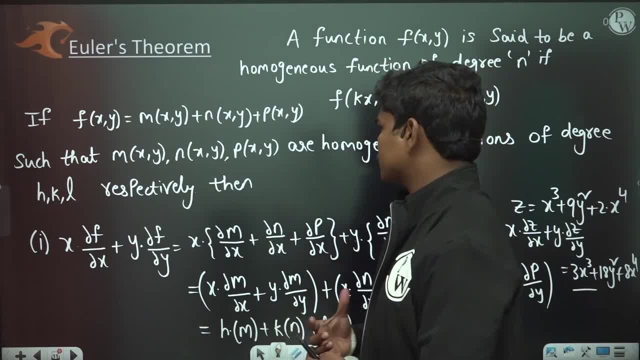 actually calculate or we define this, actually calculate or we define this Euler's results, so that you know it will. Euler's results, so that you know it will. Euler's results, so that you know it will be of very much use to us, okay, and also be of very much use to us, okay, and also. 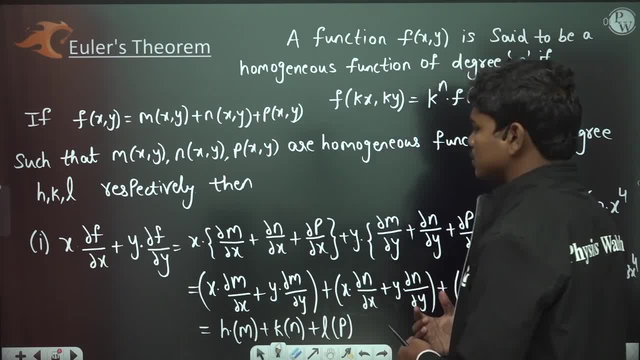 be of very much use to us. okay, and also, I would like to. I would like to give one. I would like to. I would like to give one. I would like to. I would like to give one more point here. this is the first more point here. this is the first. 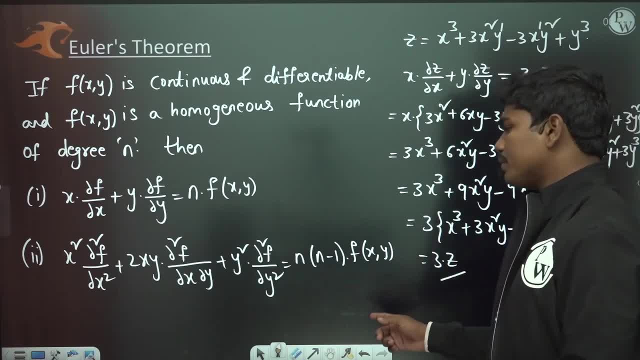 more point here. this is the first statement. so similarly like this, if you statement so similarly like this, if you statement so similarly like this: if you go here, can you guess what comes here? go here, can you guess what comes here. go here, can you guess what comes here? okay, so here you have the second. 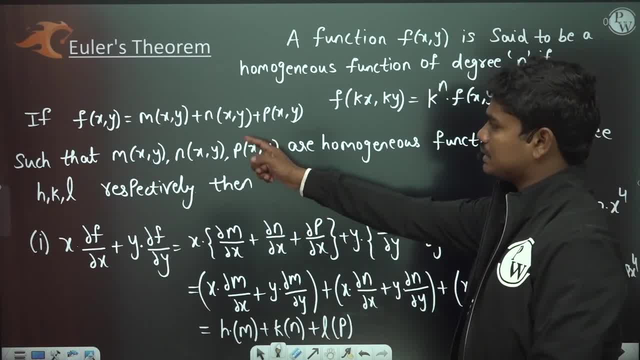 okay, so here you have the second. okay, so here you have the second statement like this. so let us suppose statement like this. so let us suppose statement like this. so let us suppose: whenever this F is summation of the, whenever this F is summation of the. 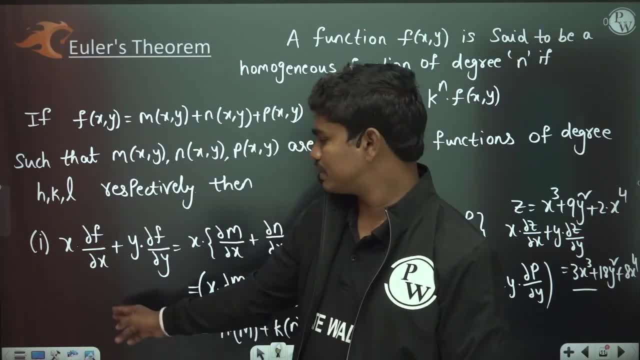 whenever this F is summation of the parts. if I calculate X square into dou parts. if I calculate X square into dou parts. if I calculate X square into dou square, f by 2 X square plus 2 X times of square, f by 2 X square plus 2 X times of. 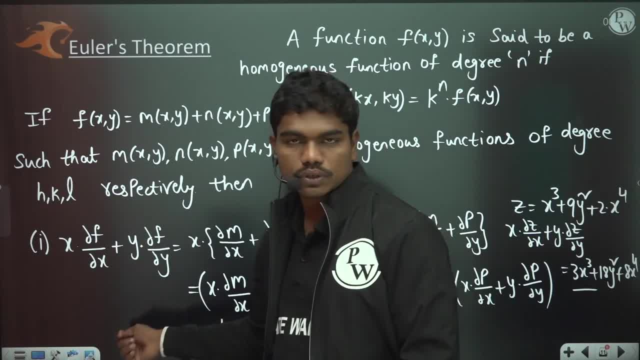 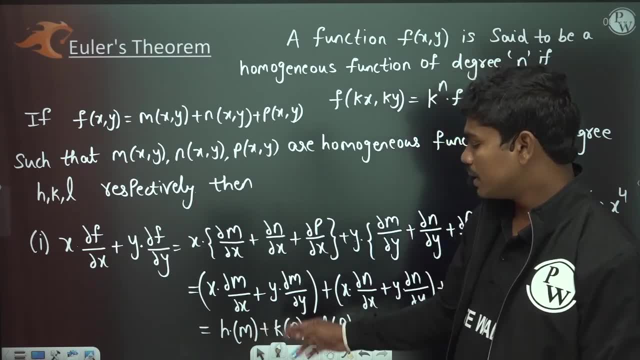 square f by 2 X square plus 2 X times of dou square f by 2 X dou y plus, you know, y square times of dou square of bed over square. if i calculate this, what will i get? similarly, i'll get h into h minus 1 times of m plus k into k minus 1 times of n plus l into l minus 1 times. 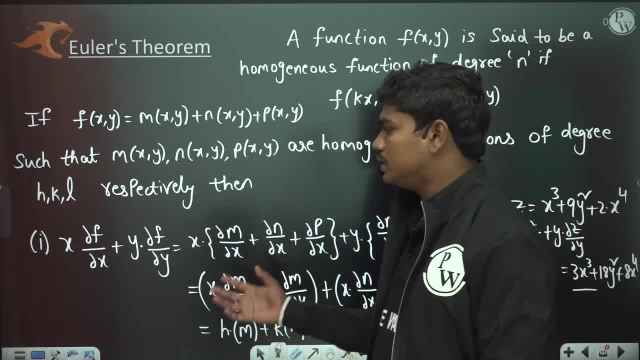 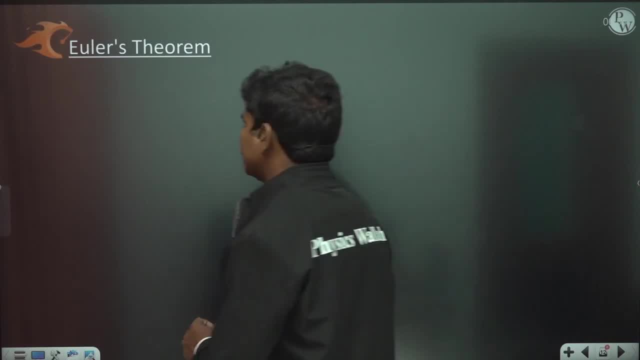 of p. this is what i might have got if i have calculated. uh, this actually okay. so if you want, you can work out with an example. so see, here we can work out with an example. actually, look, for example, the same example we can take: z is equal to. let me draw one statement here, a line here. so 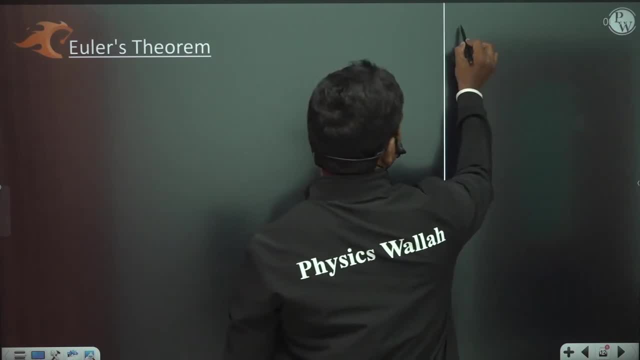 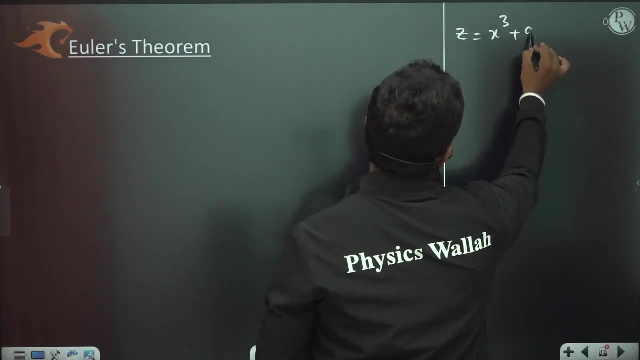 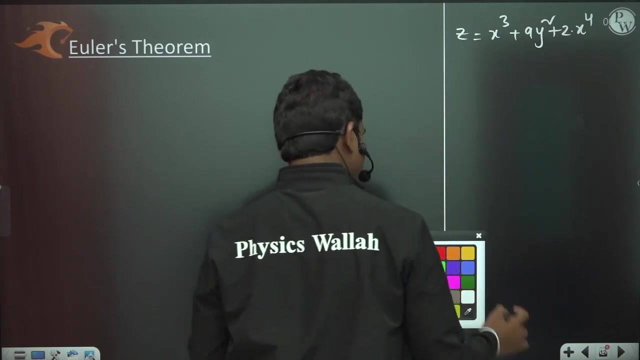 that we can work out few things, okay. so now, if you see z is equal to z is equal to this function: x cube plus 9 y square, x cube plus 9, y square plus 2, x power, 4, so these are homogeneous functions of degree 3, 2 and 4. now if you calculate this result x into dou z by dou x, 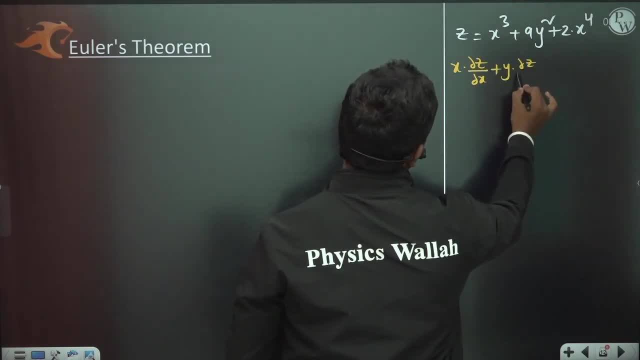 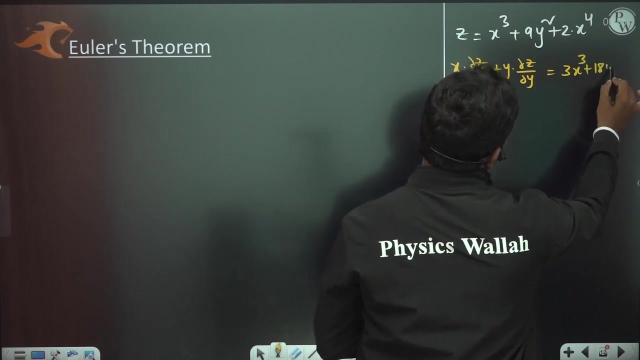 x plus y into dou z by dou y, actually okay. so now, if you see this, uh, this function basically. now, if you calculate this result, you know you will get the answer definitely, which is equal to 3 times of x cube plus 18 times of y square plus 8 times of x power 4. this is what we have got here, okay. 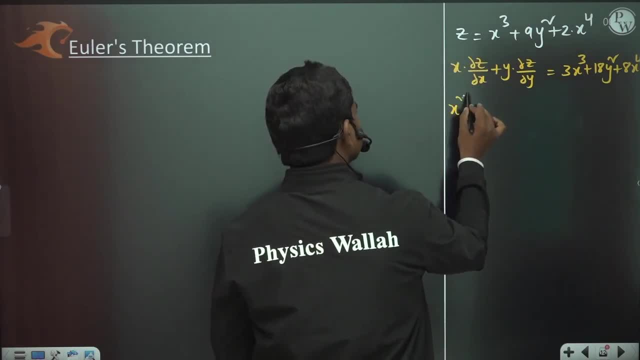 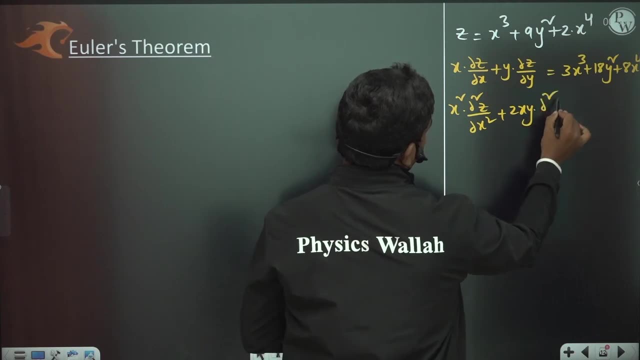 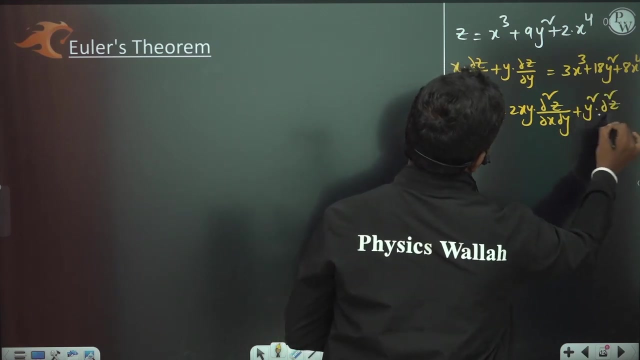 now let us suppose if you calculate this result- x square into dou square z by dou x square plus 2 x y times of dou z by dou x, dou y plus y square times of dou square z by dou y square. so if you calculate this result, for example, what you actually get is: since this is a homogeneous, 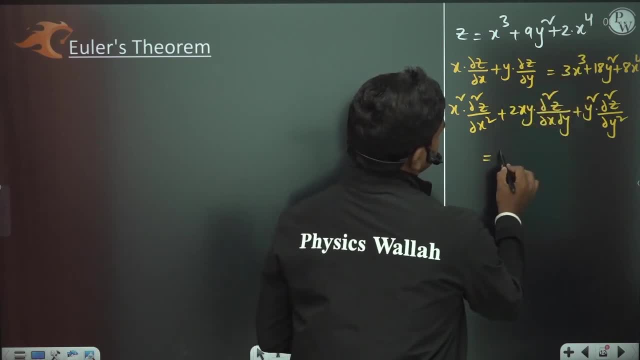 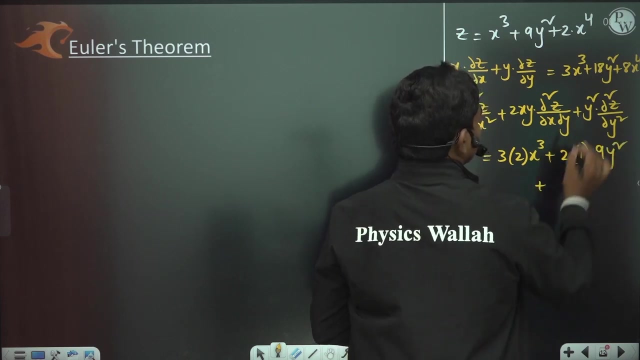 function of degree 3. actually, you will get 3 into 3 minus 1, which is 2 times of x cube plus. this is homogeneous function of degree 2, so 2 times of 2 minus 1, which is 1 into 9y square plus. this is homogeneous of degree 4, so 4 into 4 minus 1, which. 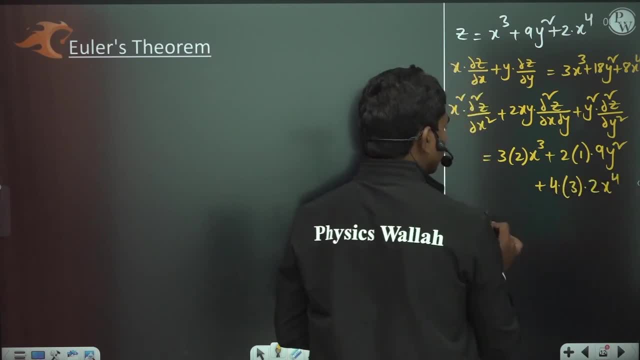 is 3 times of 2x power 4. so if you simplify the result, you will get 6x cube plus 18y square plus 4th is 12. 12th is 24 times of x power 4. so this is what you might have got if you calculated. 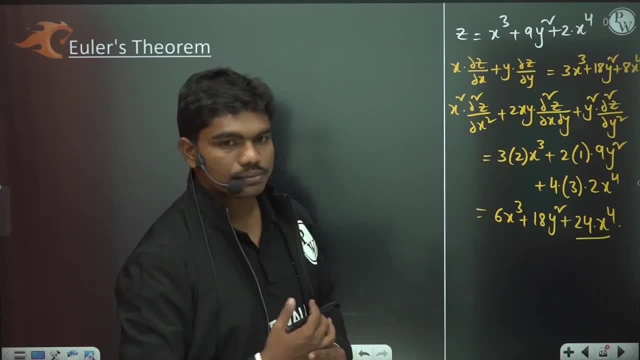 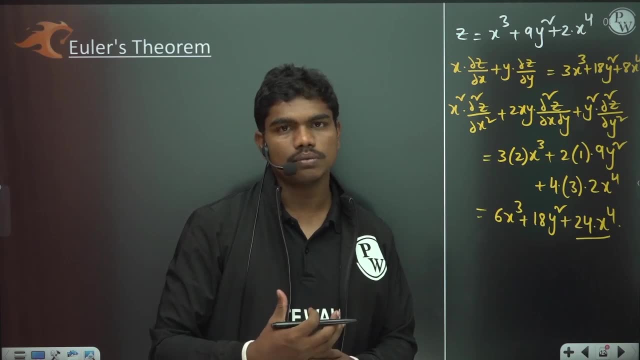 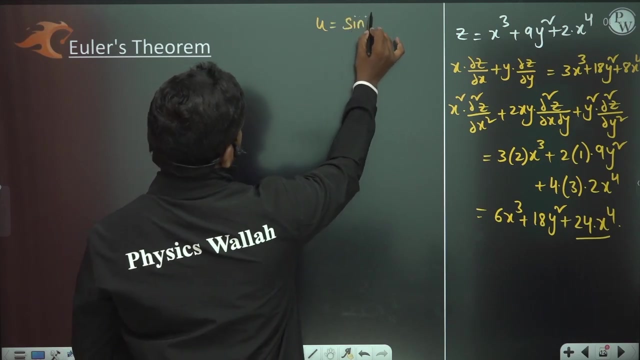 this result actually okay. now, one very important point is: sometimes the function need not be homogeneous directly, but some function of that variable is homogeneous means. look for example: let us suppose if i take this function, u is equal to, for example, say, sine inverse x, square plus y. 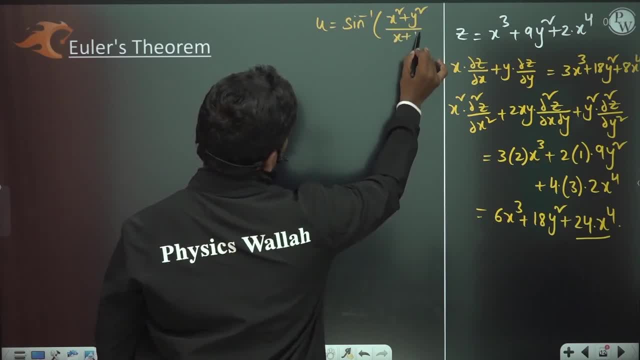 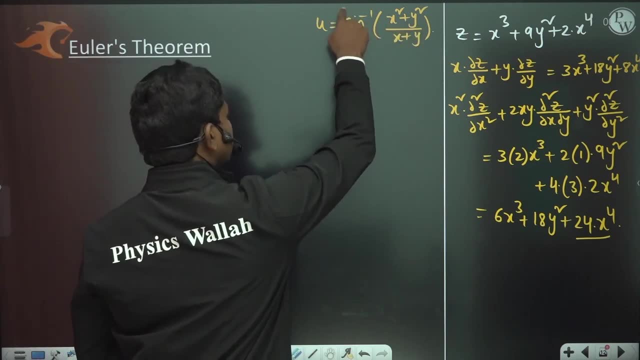 square by x plus y. let us suppose, if i have calculated this function, if i have calculated this function, then if you see, this function sine inverse of something is now a homogeneous function directly, because if you replace kx and ky in place of x and y, you will. 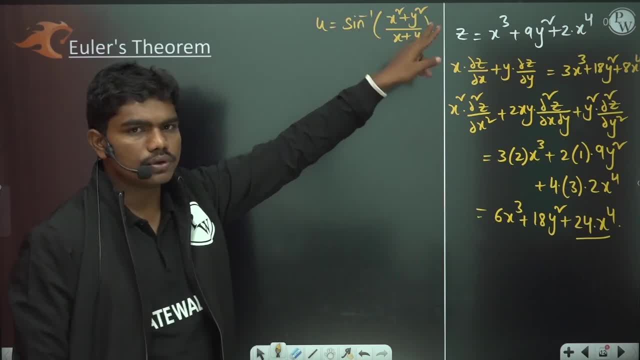 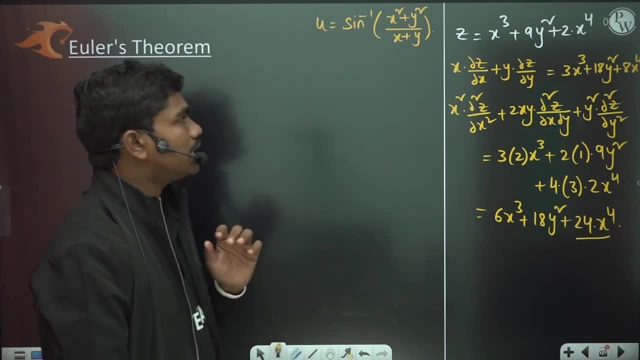 get a k inside sine inverse, so sine inverse of k into you will get the same function there. you cannot take k out of this sine inverse directly. okay, so at that for that functions. let us see how you actually will do for these questions. okay, so you can write this as sine u correct. 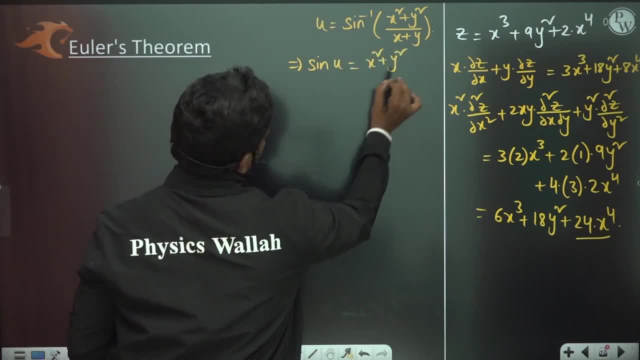 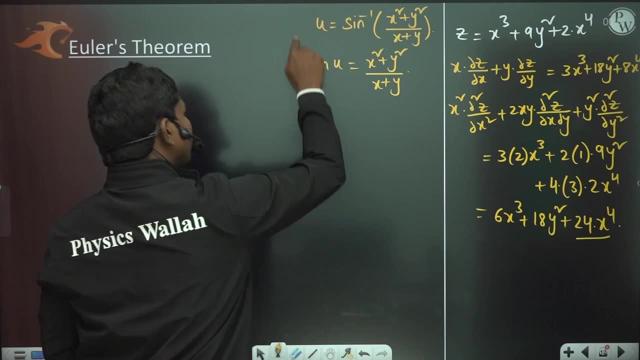 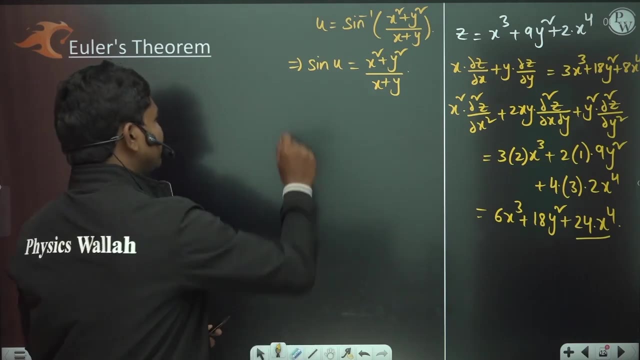 so sine u is going to be x square plus y square divided by x plus y. now, if you see, this function u is not directly homogeneous, but some function of u, for example, if you take the sine here, sine u is equal to x square plus y square by x plus y. so this function u itself is not homogeneous. but 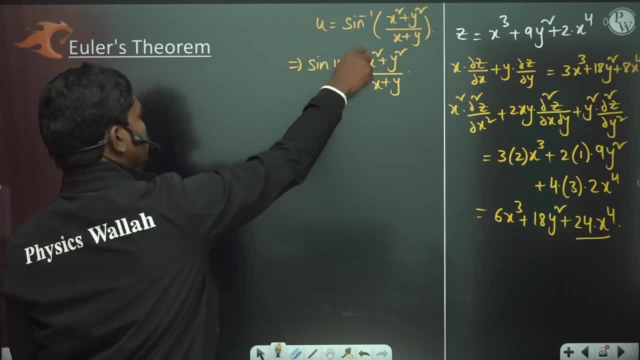 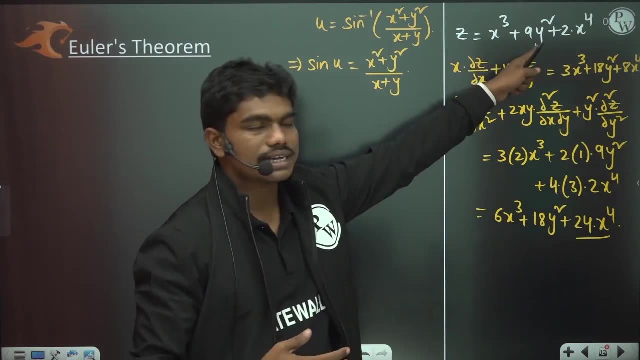 some function of u means sine u is actually homogeneous function. now it is homogeneous. so whenever some function of a variable is homogeneous means- let us suppose here, if z is not directly homogeneous, but some function of z sine z, log, z something, is homogeneous, then how we? 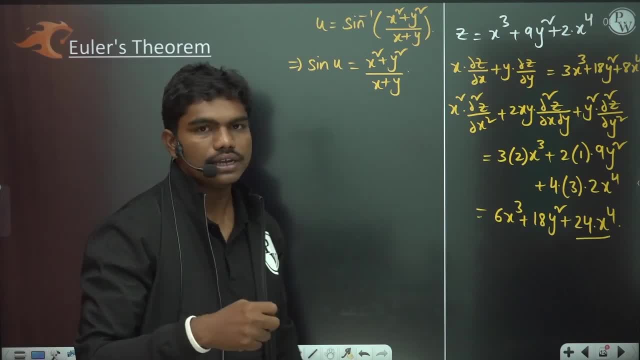 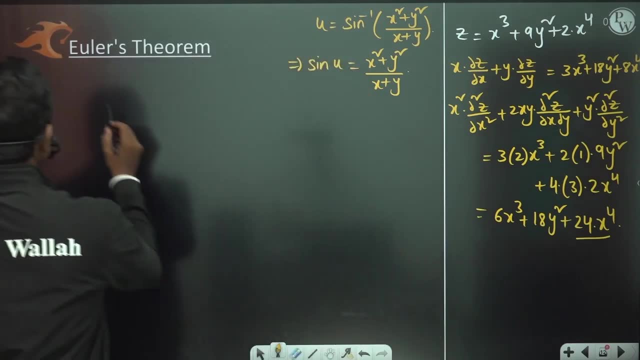 actually do the conversion actually okay. so let us see that now. okay, so if you want to see the conversion, then look this. euler has again given that if f of u is a homogeneous function of degree n is a homogeneous function of degree n of degree n, then first point you can see x into. 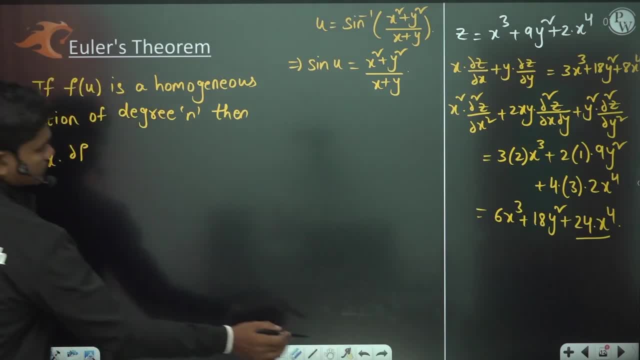 dou f by or dou u by dou x. let us say x into dou u by dou x plus y into dou u by dou y is equal to n times of f of u divided by f dash of u. actually okay, so this result is very simple to analyze. 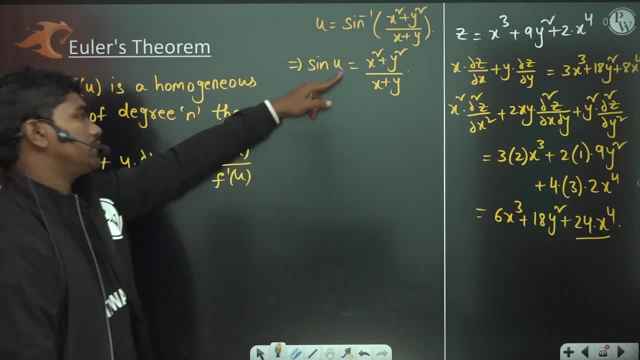 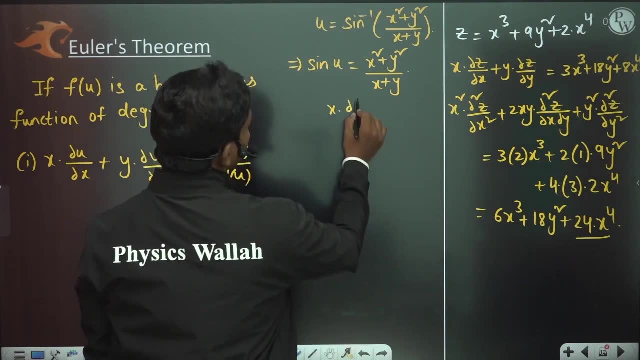 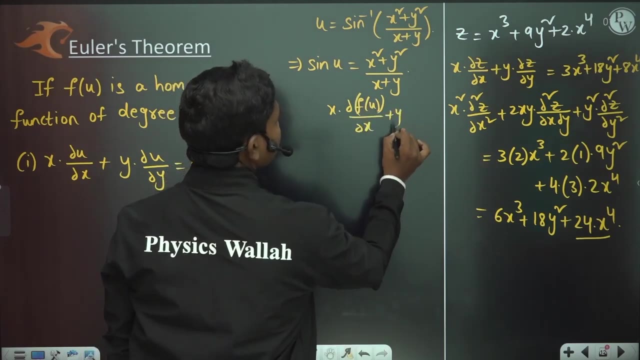 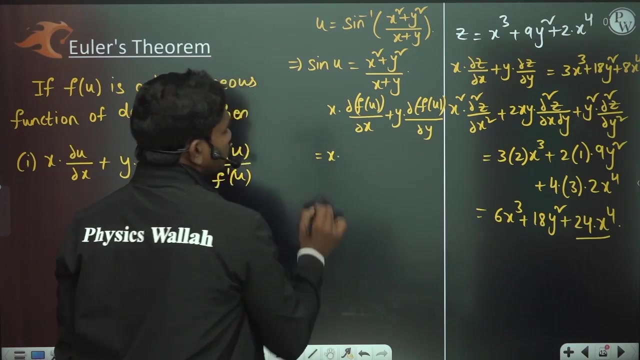 because if you see, if f of u is a homogeneous function, for example, if this is a homogeneous function, then what happens if you calculate this x into dou f of u by dou x, by dou x plus y, into dou of f of u by dou y, y? if you calculate this result, for example, what you will get x into? first of all, here you will: 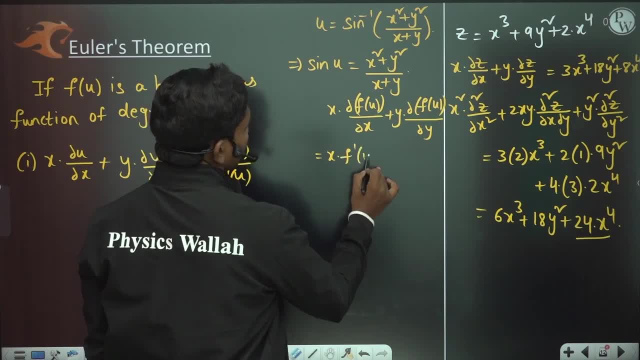 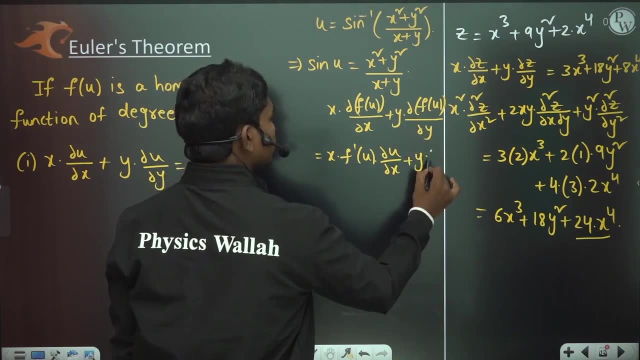 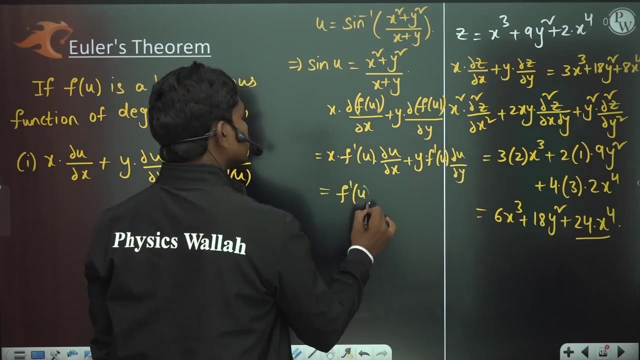 get differentiation of this f is f dash of u into differentiation of this inner variable, which is dou u by dou x. this is what you will get. similarly, here also, you will get y into f dash of u, into dou u by dou y. this is what you will get. okay, so this gives you f dash of u times x into dou u by 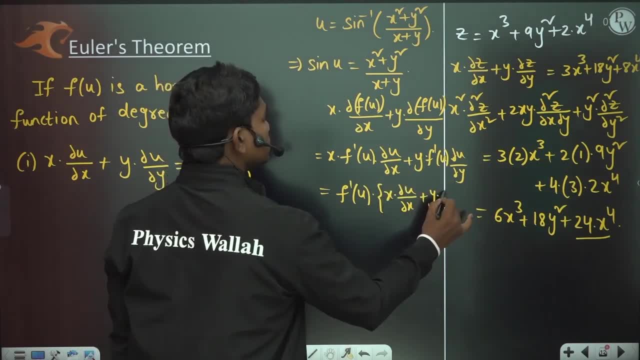 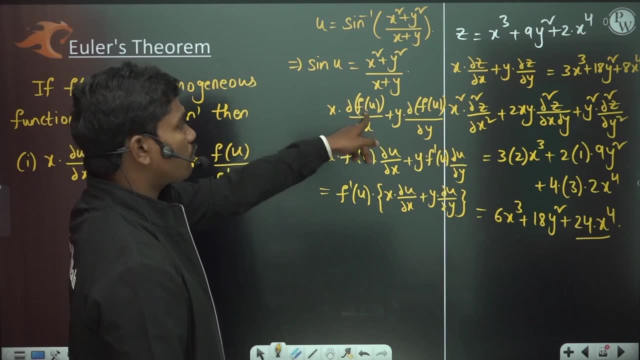 dou x plus y into dou u by dou y is what you will get here. but if you see, if this f of u is homogeneous, this x into dou f of u by dou x plus y into dou f of u by dou y is equal to n times of. 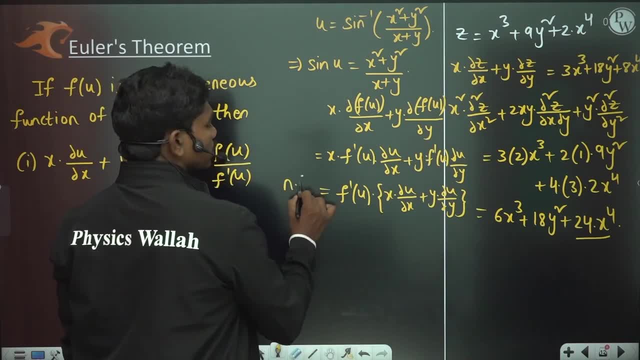 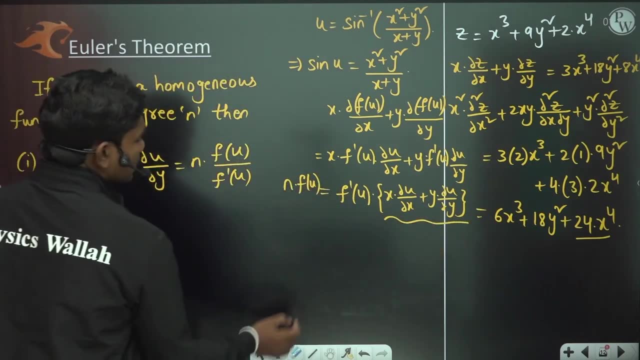 f of u, so this value is actually equal to n times of f of u. so if you want this value, this is nothing but n times of f of u by f dash of u. so this is how we have this result, actually, okay, so anyhow, just this i have given you for your understanding, but 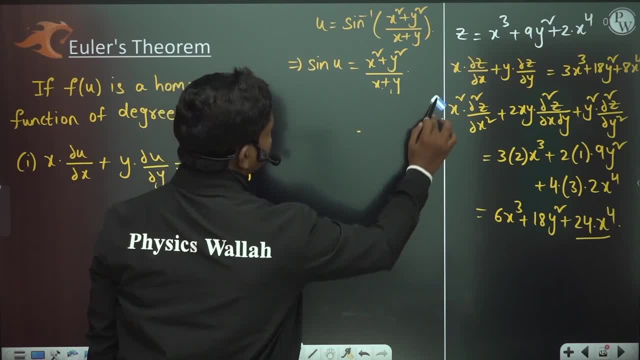 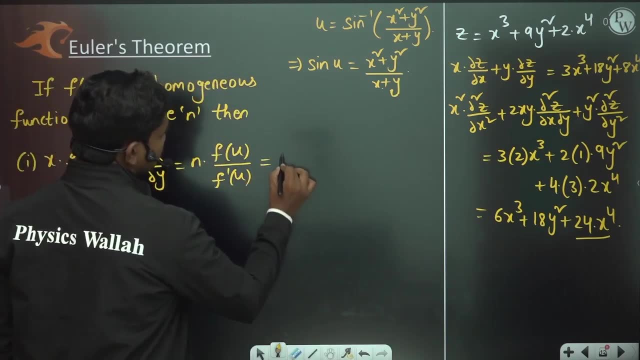 you. it's very, you know, intuitive that we'll get a f dash of u in the down, you know, denominator. so here, if you see, this is generally designated as capital f of u, because this is going to be some function of u. so if you calculate, this second part means x square into dou, square u by dou x. 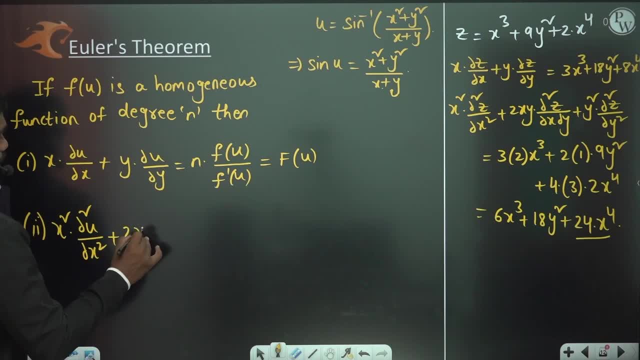 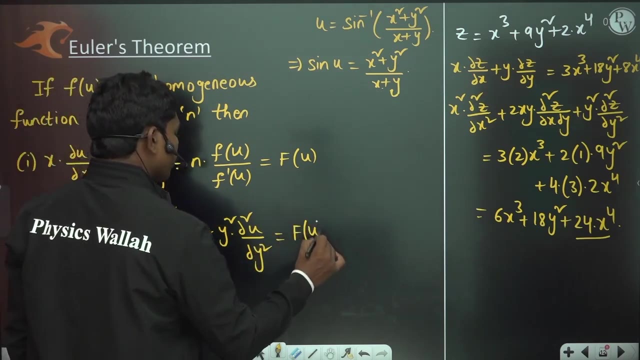 square plus 2. x y times of dou square u by dou x. dou y plus y square times of dou square u by dou y square. if you calculate these values, then this is going to be something like capital f of u times f dash of u minus 1. this is the result that you are going to get, okay, so? 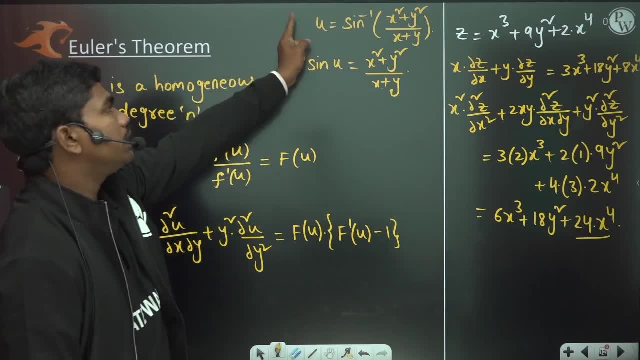 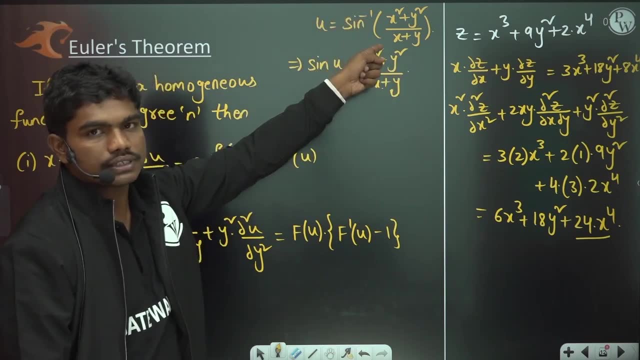 let us suppose if sine u is the function. if i want to calculate x into dou u by dou x plus y ing into dou u by dou y for this particular combination, calculating dou u by dou x is very complicated. for this correct 1 y root of 1 minus this complete bracket, square into again partial definitions and all. 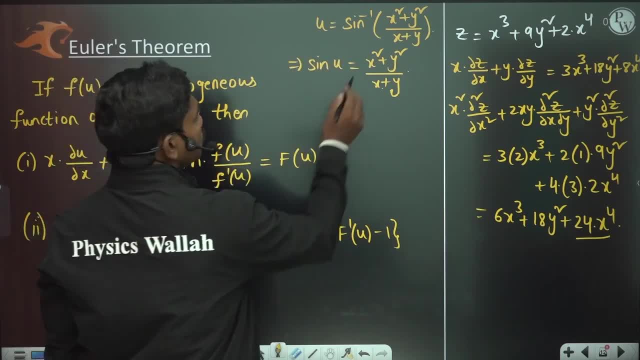 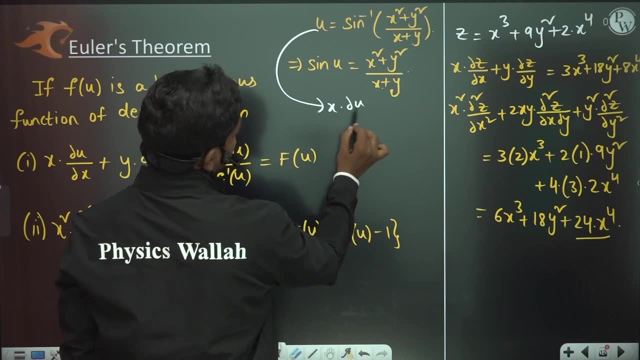 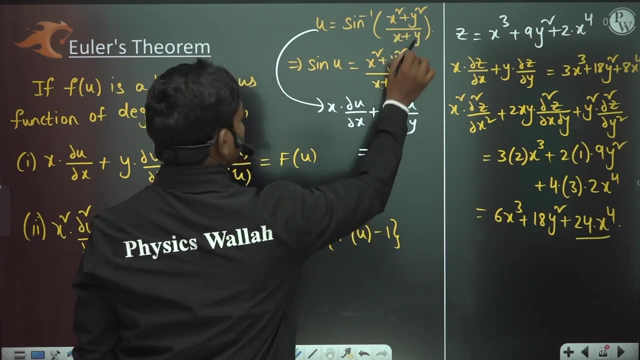 will be very clumsy, but if you know this euler's equation, you know for this result, for this result, x into dou u by dou x plus y into dou u by dou y, this value is equal to. this is a homogeneous function of degree one, so one times of f of u. so what is f of u, this function which is sine u? 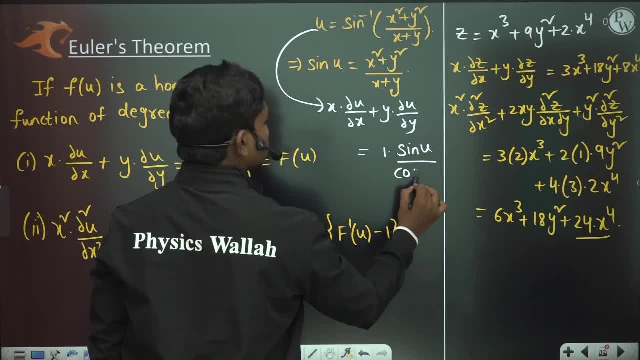 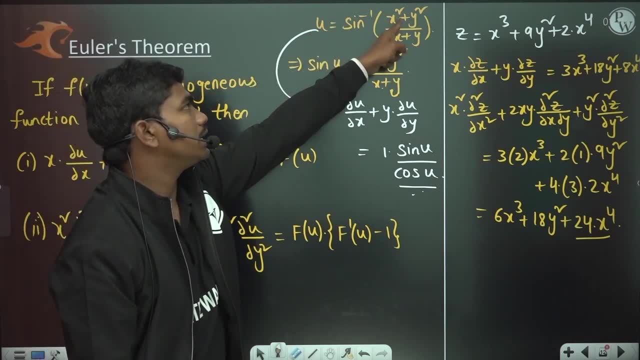 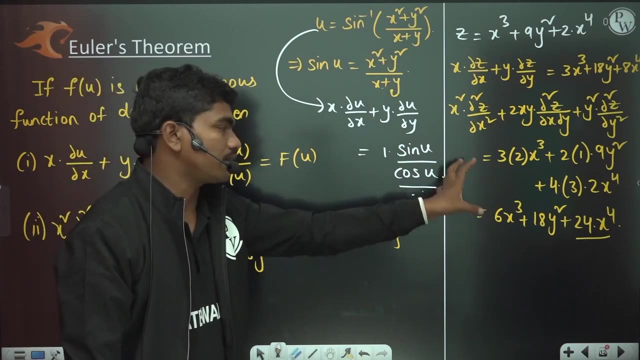 divided by f dash of u. so differentiation of this: sine u is cos u, so total tan u is what you will get. okay, so if you form a triangle with this as the hypotenuse and this as the opposite side, so from that triangle, if you calculate what is tan, theta that or tan u, that value in terms of x and y, 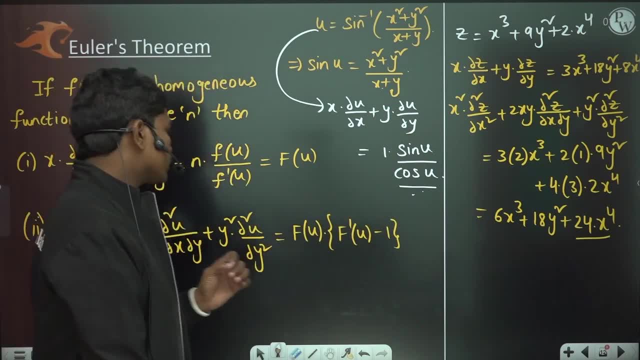 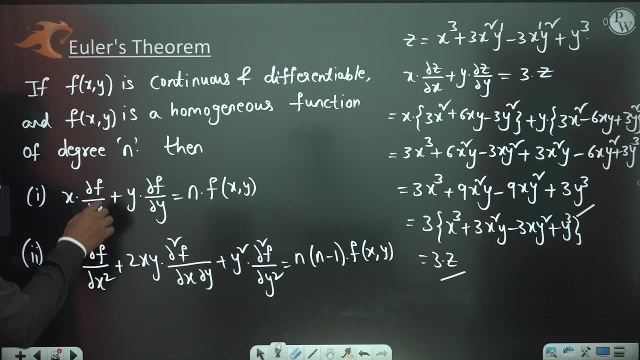 is going to be the answer for this uh result actually here. okay, so these are very important observations of this euler's theorem. so basically, three points i have given you here. if you understand that this function is a homogeneous function directly, straight away, like that, then x into dou f by dou x, plus y into dou f by dou y. 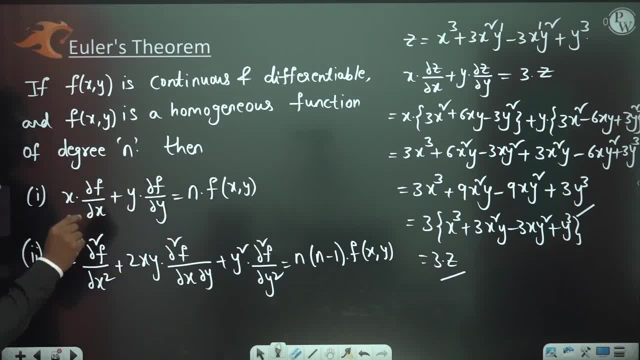 gives you n times of that function. similarly, if you calculate x square times of dou square by dou x square plus two x times of dou square f by dou x, dou y plus y square times of dou square f by dou y square, this value is n into one n minus one comes. 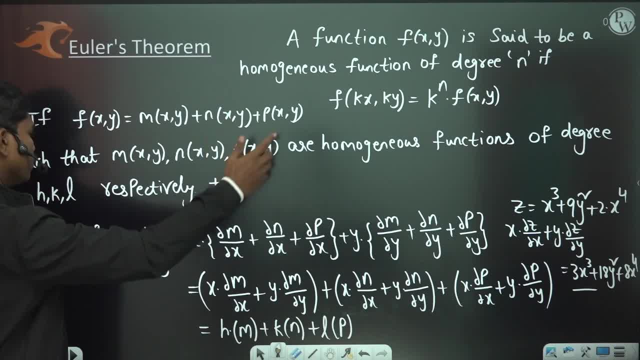 here now. let us suppose, if this s is summation of three functions, maybe more, such that they all are homogeneous functions of in, uh, you know individual degrees, then you can write this: x into dou f by dou x, plus y into dou f by dou, a combination as h. 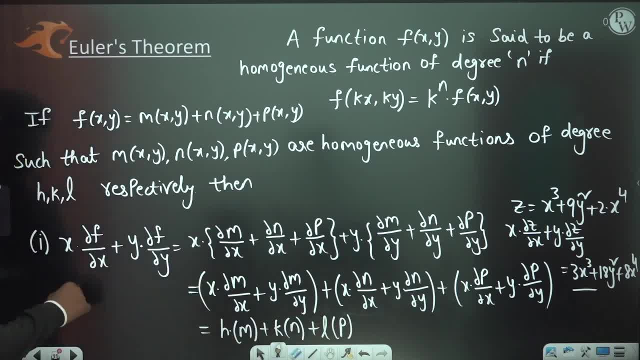 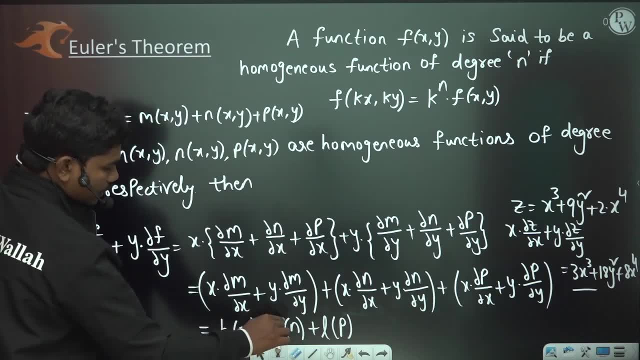 m plus k into n plus l into p. similarly, if i ask you x square, dou square f by dou x square, all these things, you can write h into h minus 1 times of m plus k into k minus 1 times of n. because here you see, this is something similar to this. okay, so, something similar to this expression. so 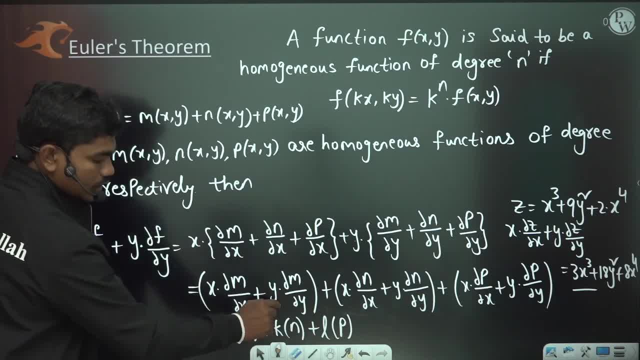 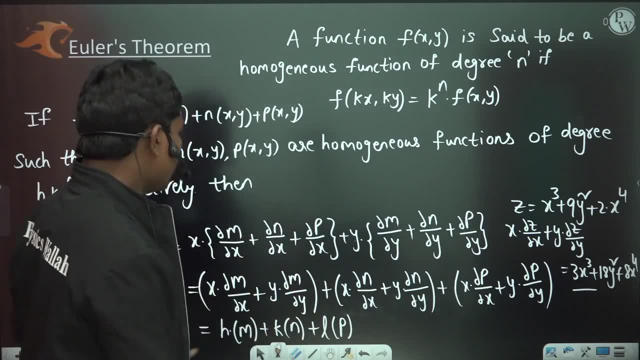 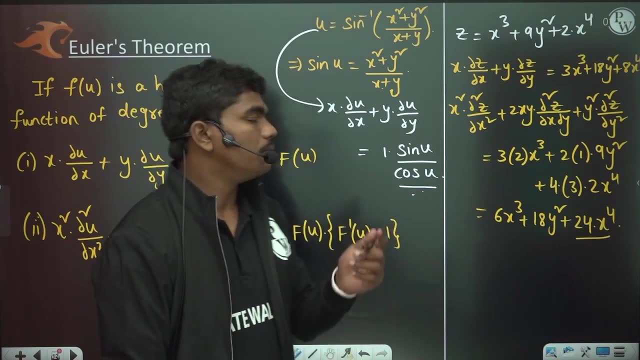 h into h minus 1 times of m plus k into k minus 1 times of n. plus l into l minus 1 times of p. this is how you can get this result actually okay. and finally, we have also seen sometimes the function of u, the function u of x comma y directly is not homogeneous, but some function of u is. 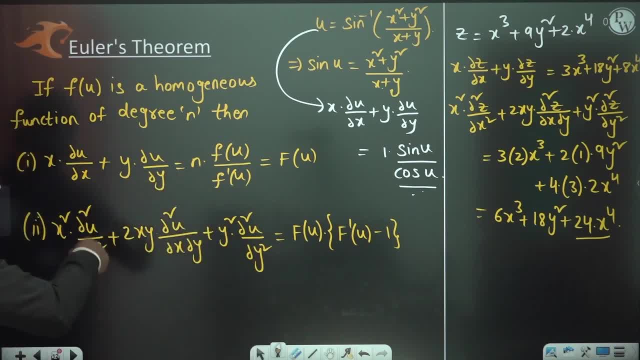 actually homogeneous, like this in this case. okay, so for that functions we have defined like this- please make a note: i have defined this complete combination n times of f of u. by capital f i mean small f dash of u. i have written this as capital f of u and i have used this capital f of u here. 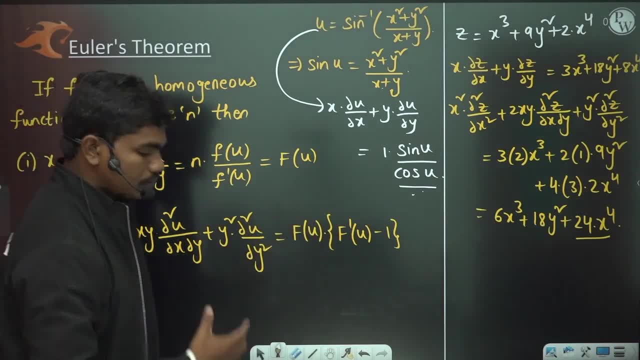 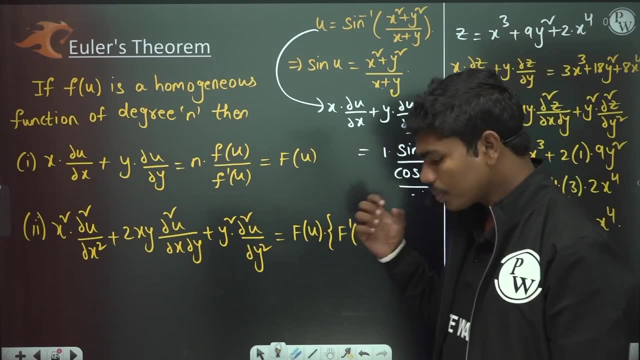 it's not small f here, okay. so please make a note, because sometimes it's quite, you know, a possible mistake that you substitute again small f here and get your answers wrong, okay? so that's why it's very cautious to keep a capital f here always, okay. so this is how we actually calculate. 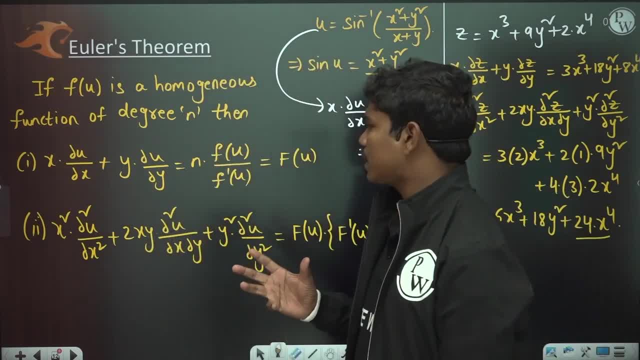 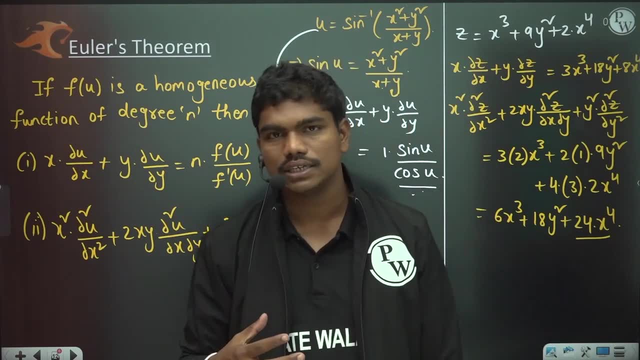 the partial differentiations and, of course, some combinations of these partial derivatives, like x into dou u by dou x, plus y into dou u by dou y or this particular combination of partial terms actually. so, if you see, these are all certain ways how you do the partial derivatives and also 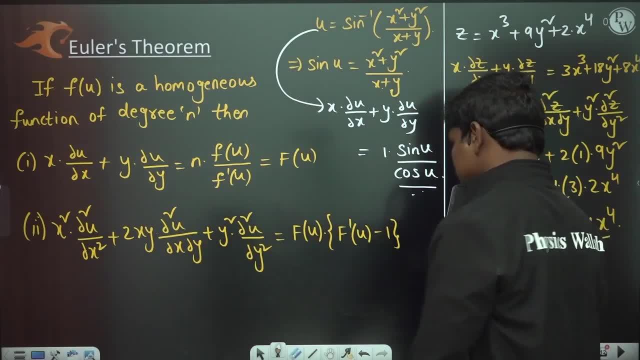 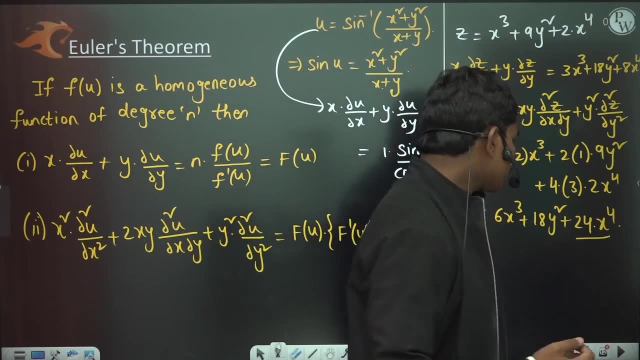 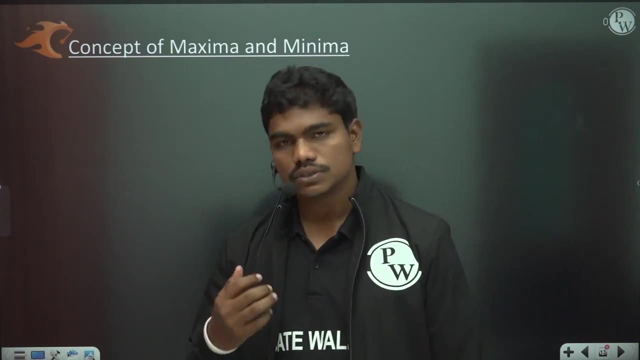 some partial relations now moving to this concept. so once we identify how to calculate the partial and of course things, then we move on to this concept of maxima and minima in multi variables. okay, so right now we talk about three variable functions. okay, so let us see the working procedure. 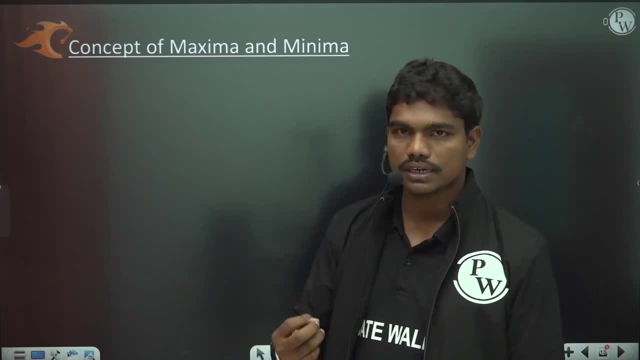 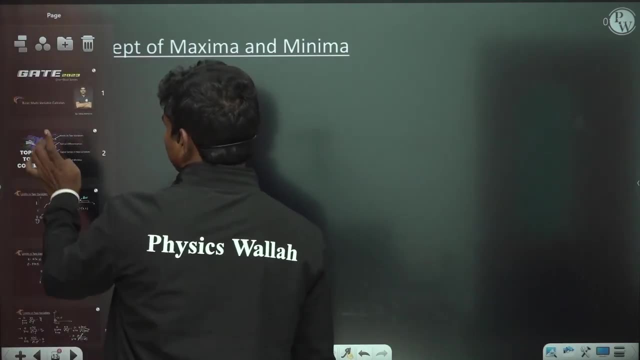 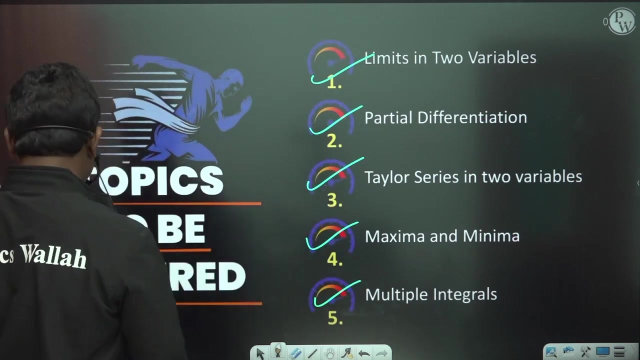 and also let us work out some examples for the better understanding. okay, so, if you see once, if you quickly go through the things, that what we have talked about, we talked about this- limits into variables and also partial differentiation. okay, so meanwhile we have this Taylor series in. 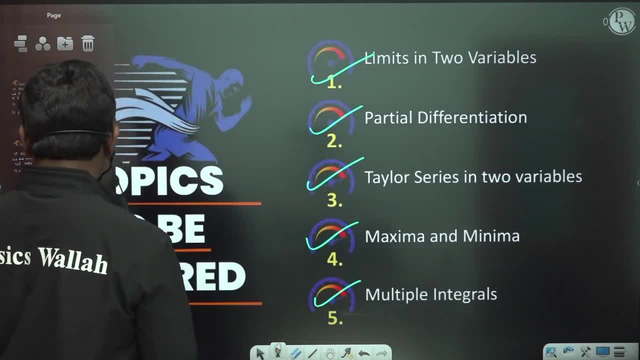 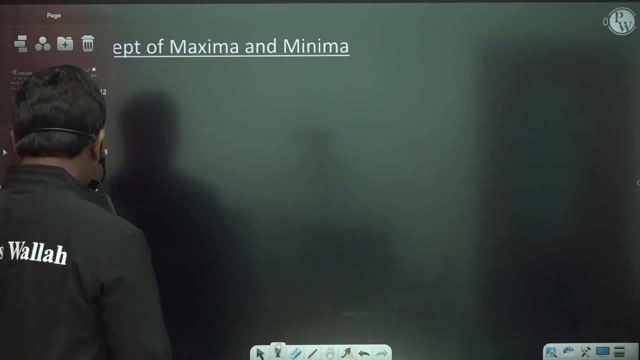 two variables also okay. so let us talk about the Taylor series also for some time. okay, first, fine, let us talk about the concept of maxima and minima, then we'll go for the concept of this Taylor series, okay. so, anyhow, Taylor series is some independent topic, so let us deal that after the concept of 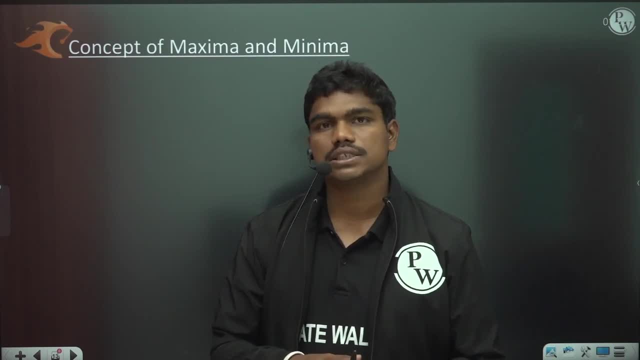 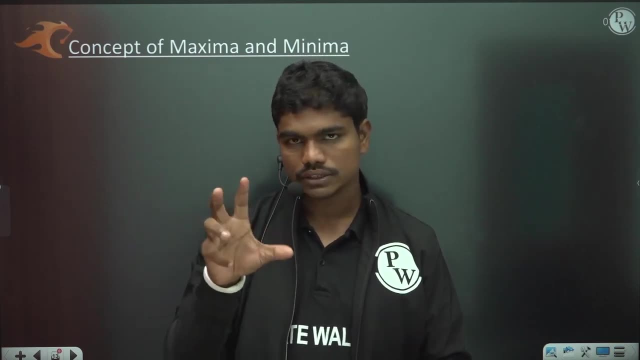 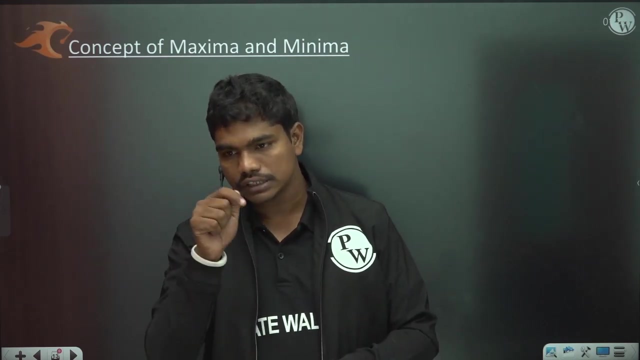 maxima and minima. so now, if you see in single variable calculus we have observed from a that whenever you have a maximum or whenever you have a minimum, definitely the slope at that points of maxima and minima are zeros. means basically, if you draw a tangent to any curve at which it has a maximum, or if you draw a tangent to any curve, 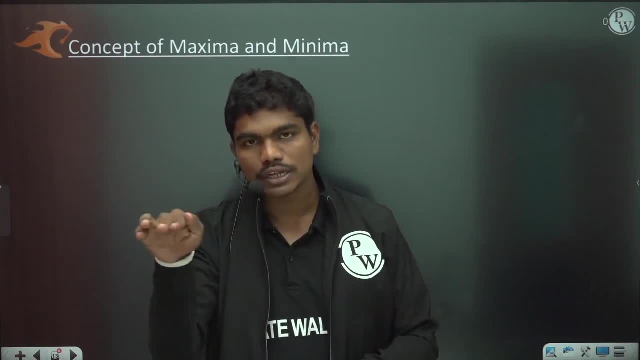 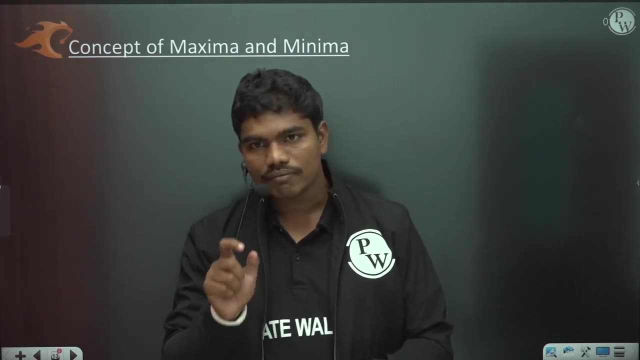 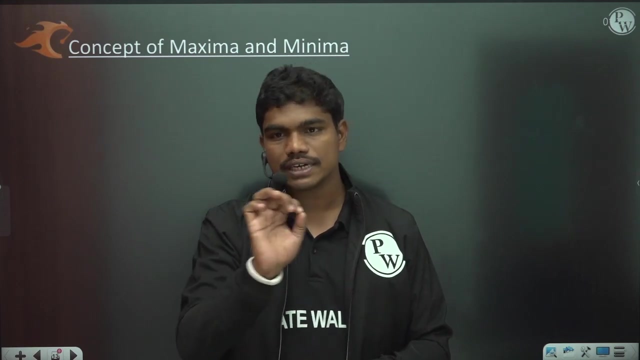 at which it has minimum. thus tangents are actually parallel to the x-axis. okay, now, if you see, I have told you one very important point there: at points of maxima or minima, you have your differentiation equal to zero. this is hundred percent, two and clear. but I have also told you, if derivative is, 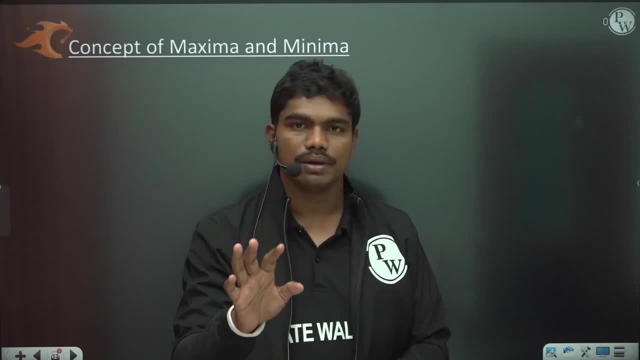 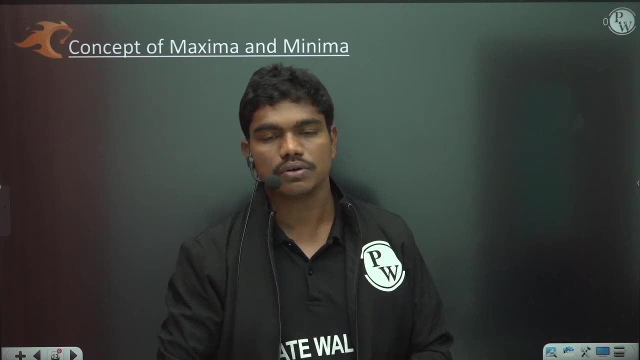 zero. that doesn't ensure the concept of maxima or minima. that's why we have something called the secondary derivative test. correct, because if you draw a tangent to any curve at which it has a maximum or minimum. you see, I have told you one point: x is equal to zero for x cube function okay. 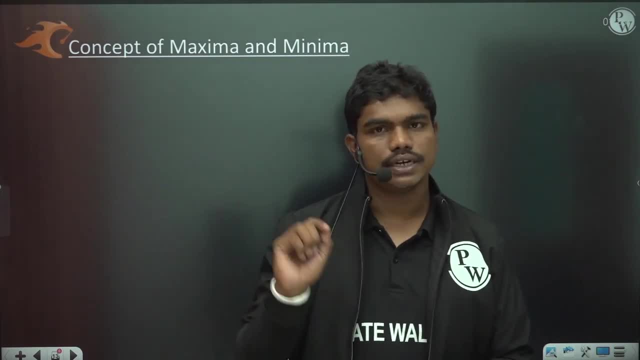 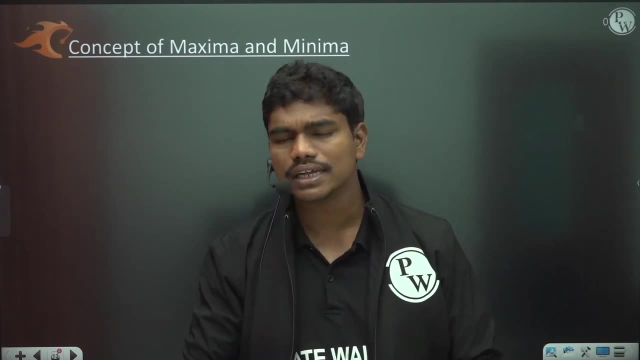 so if you take y is equal to x cube, then at x is equal to zero- first derivative is zero, but at x equal to zero, the function don't have either maximum or minimum. okay, so there is certain important things like that you need to observe. okay, now coming to the concept of maxima and 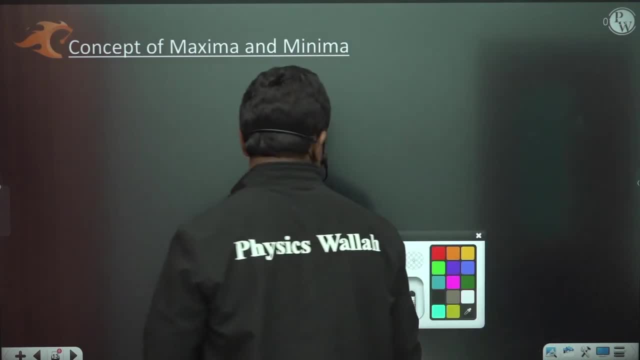 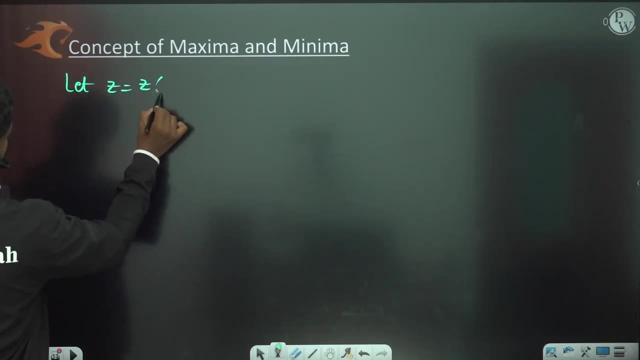 minima. let us quickly see the working procedure, how we actually do this. look, let z is equal to, you can write f because generally you are familiar in f sometimes. okay, so anything, any variable. so let f is equal to f of x, y, z or x- y. let us take two variable function. 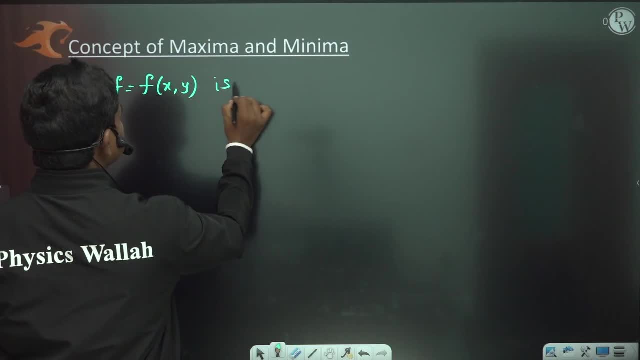 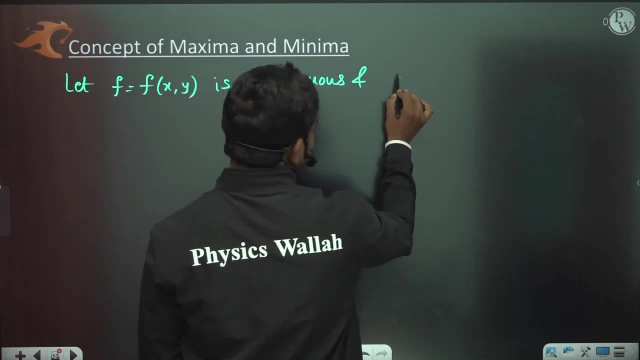 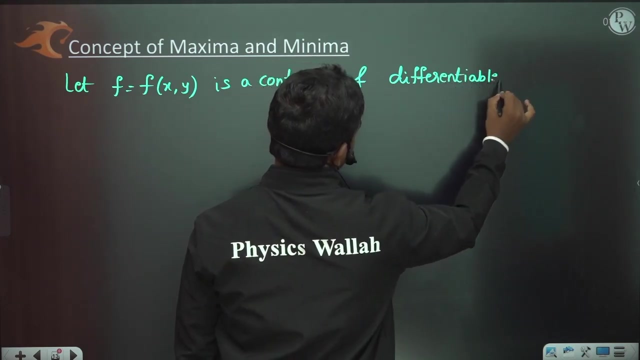 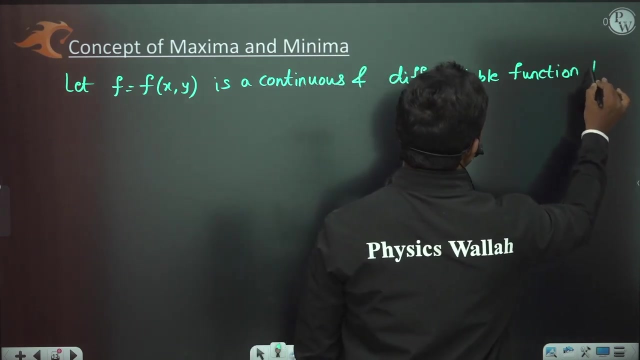 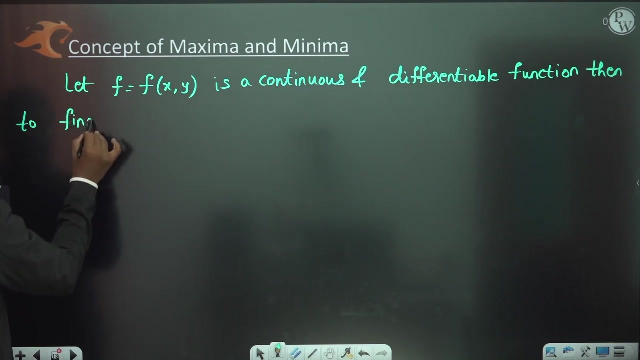 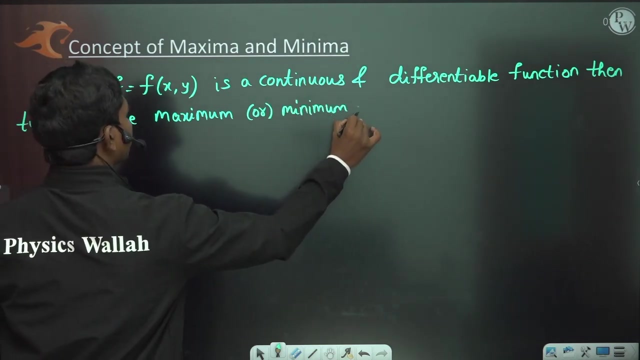 so let f is equal to f of x comma y is a continuous, is a continuous and differentiable function function. then then, to find, to find the maximum, then to find the maximum or minimum of of f of x comma y, of f of x comma away, of f from x comma y, of f of x comma y is equal to the optimum function of f of x and function. 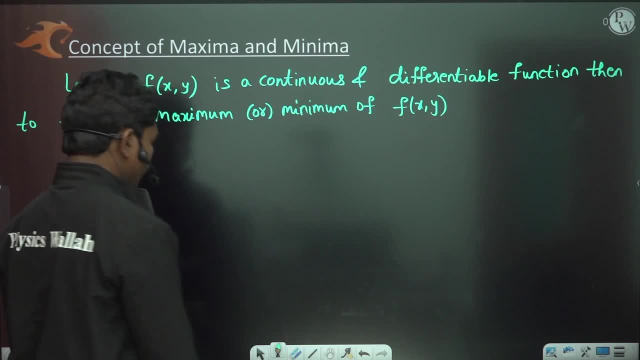 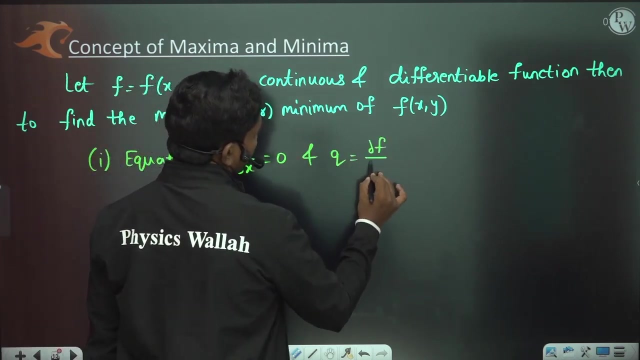 x y of f of x y. Now let us see the steps. First step, first step: equate p, which is dou f by dou x, is equal to 0 and q is equal to dou f by dou y is also is equal to 0.. So 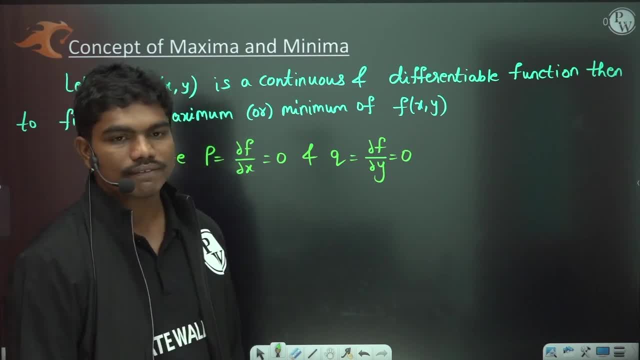 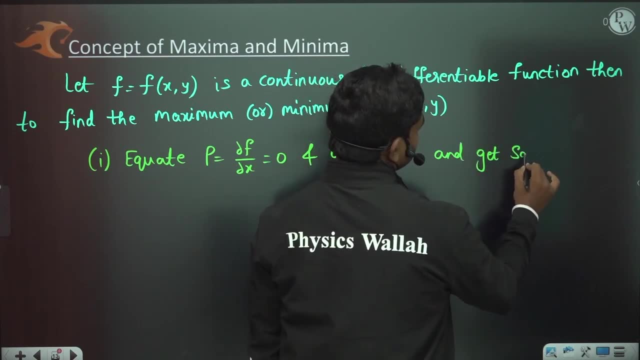 p is equal to dou f by dou x is equal to 0 and q is equal to dou f by dou y is also equal to 0. and get stationary points and get stationary points, stationary points. So you know, stationary points are the points where the differentiation goes to 0. Now, so how many stationary points? 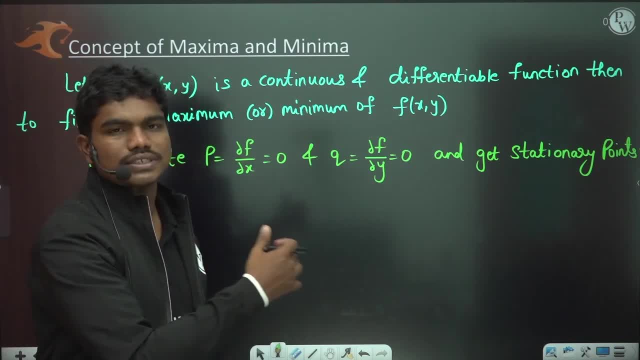 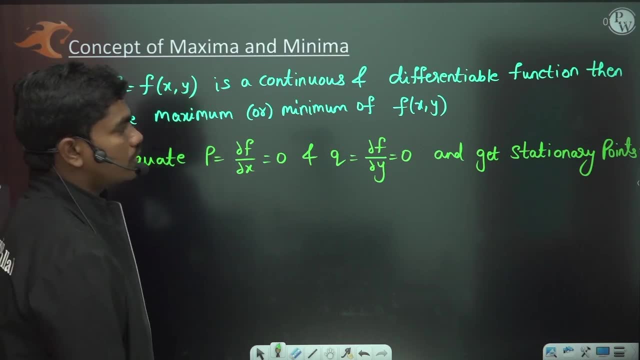 you will get. That depends upon the function. Again, we will again sort out with some example. we will see, But right now I am just explaining you. equate p is equal to dou f by dou x is equal to 0 and q is also equal to dou f by dou x is equal to 0, actually. okay Now try to understand. 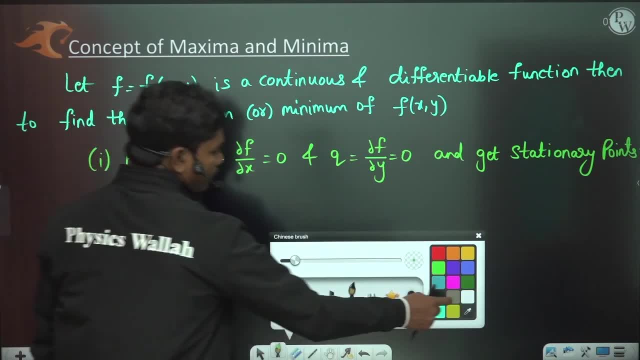 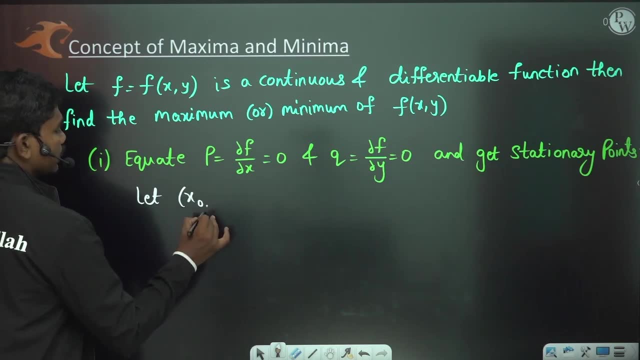 this thing and get stationary points. So let x naught comma, y naught be a stationary point. you will get many stationary points, But let us assume x naught, y naught is one of the stationary point. x naught, y naught be a stationary point. Okay, so you have this. 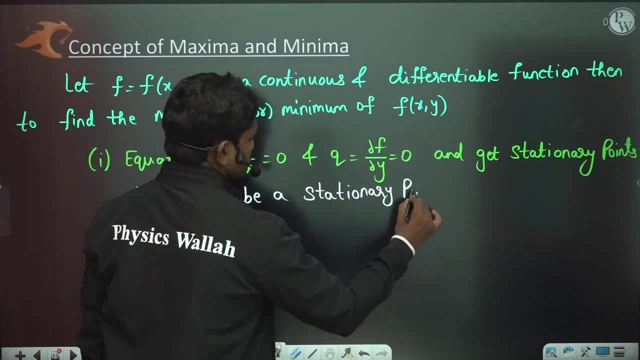 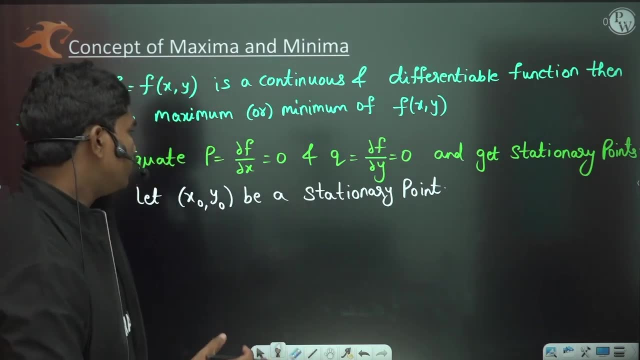 So you have here stationary point, okay. So how many stationary points you will get, That depends upon the function. we will see some examples right now. and this is a stationary point. Now, once you identify the stationary point, then step to calculate. calculate dou. 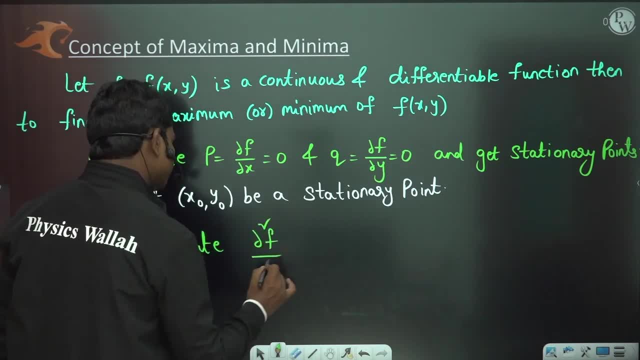 square f by dou x, square at x, not y f. f by dou x, square f, dou x by dou x, square At x. dot y y, naught at the point x, naught y, naught comma: dou square f y, dou x, dou y. or you can write dou y dou. 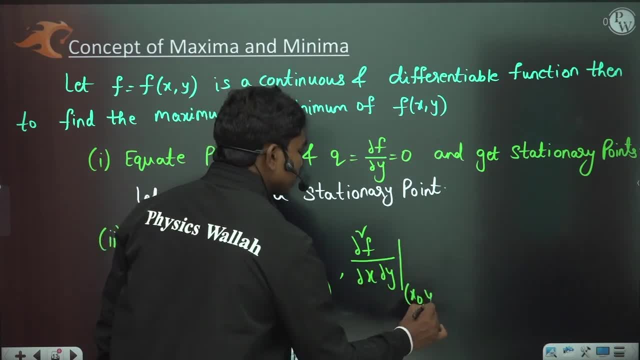 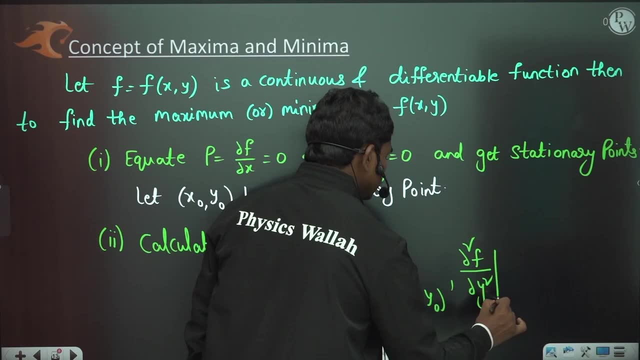 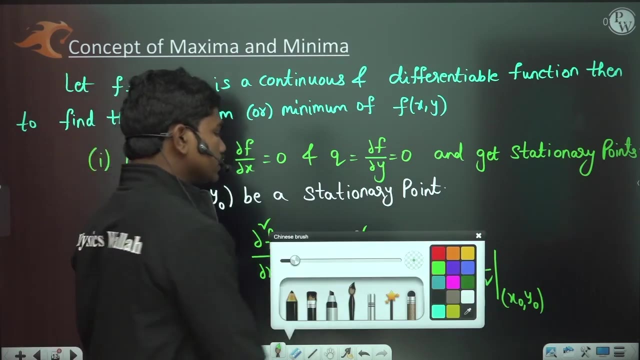 x also doesn't matter. this also you will calculate at x naught, y naught. then dou square, f, y, dou, y square. this also we can calculate at x naught, y naught. so let us suppose these are the values we are calculating and let us equate them. for example, this value, let us say: this is r, this is s and this. 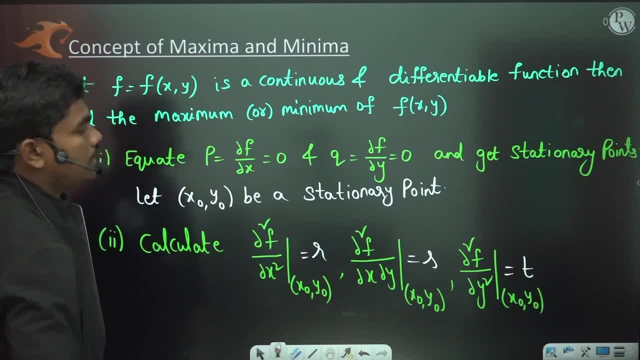 is t, for example. okay, so this is r, this is s and this is t, because we have already taken pq, so pq r st, that's it, okay. so r is the first to differentiate. i mean second derivative of f with respect to x. s is the you know combined differentiation, dou square f by dou x, dou y or 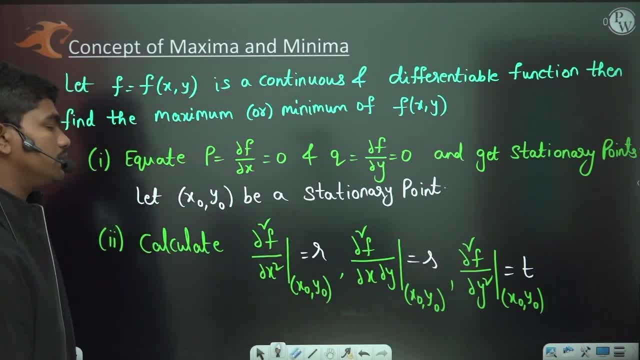 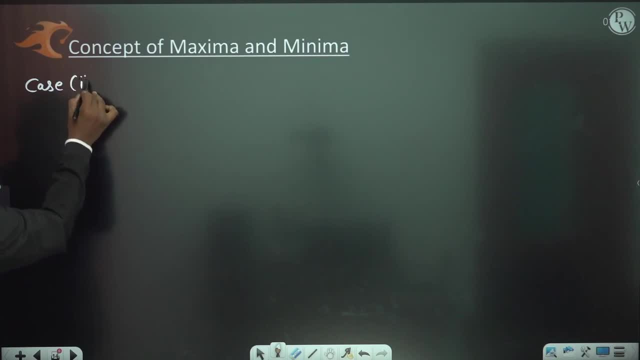 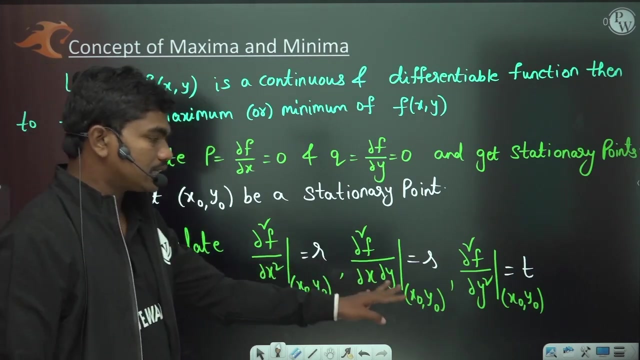 dou y, dou x and t is dou square f by dou y square. actually. here now, if you see some observations, okay, so case one. case one: if r t minus s square is greater than zero, and r greater than zero means at stationary point, using these r st values, if you calculate r t minus s square and if you get, 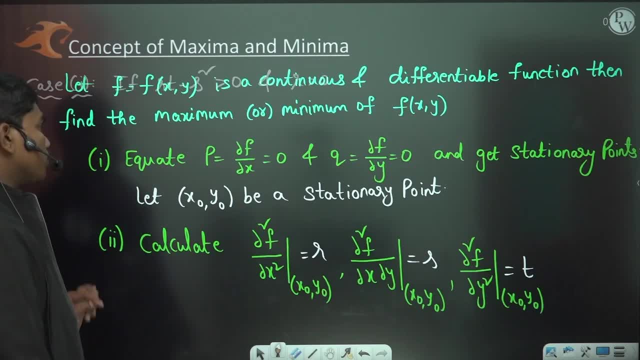 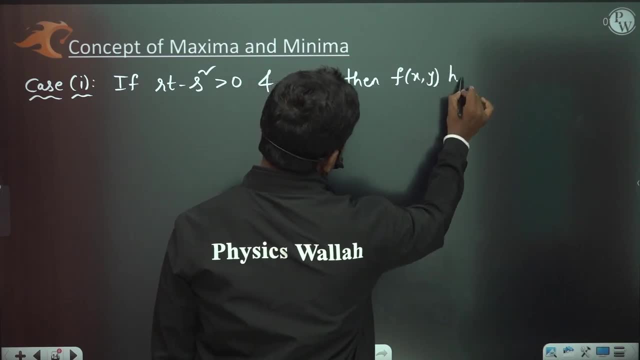 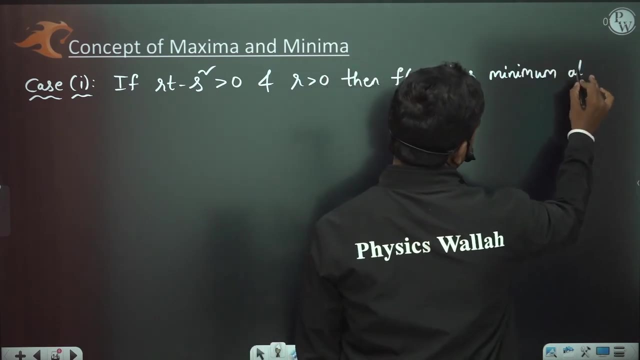 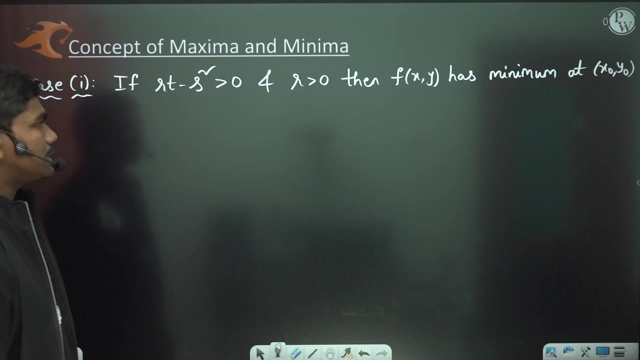 a positive value. and let us suppose if r is also positive value, then f of x comma y has minimum minimum at x naught y naught. at x naught y naught actually okay. so if r t minus s square greater than zero and r greater than zero, then f of x comma y has minimum at x naught y naught. now try to understand. 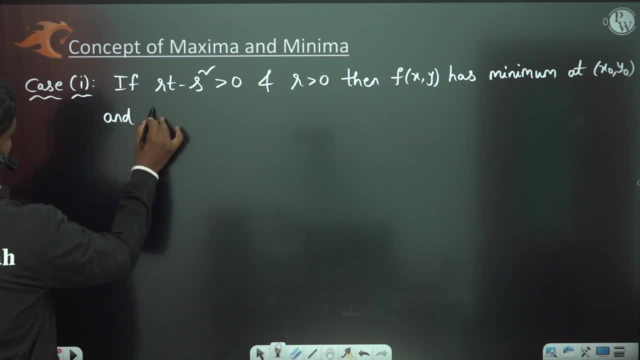 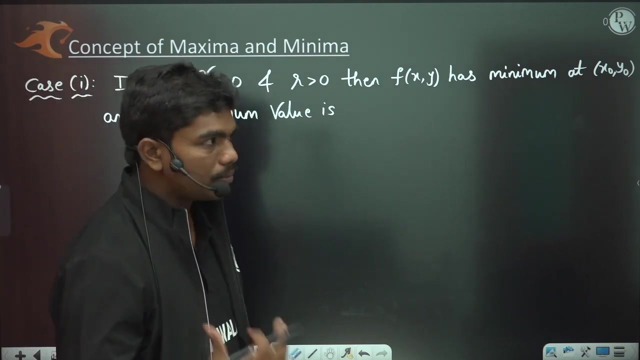 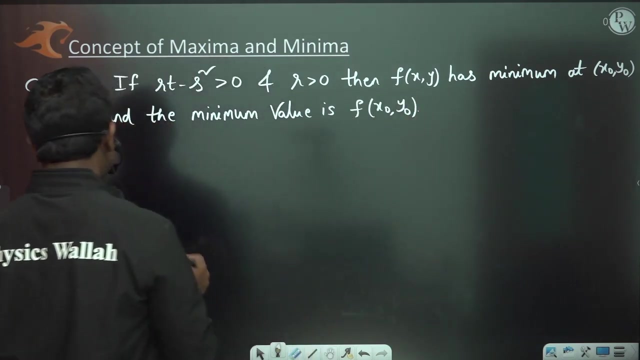 this: the, and the minimum value is how much, and the minimum value is, and the minimum value is: look, let us suppose, if the function is having minimum at x naught, y naught, then definitely the minimum value of this function is f of x, naught, y naught. that's it okay. now case two. case two: 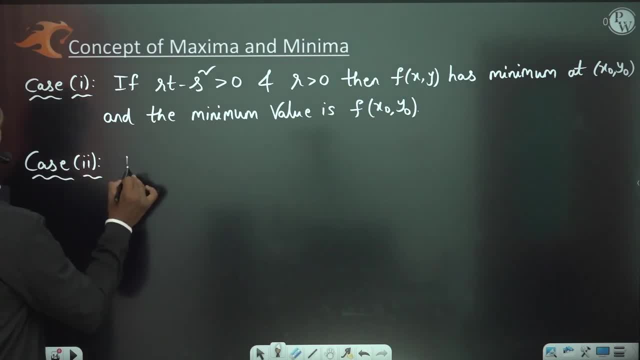 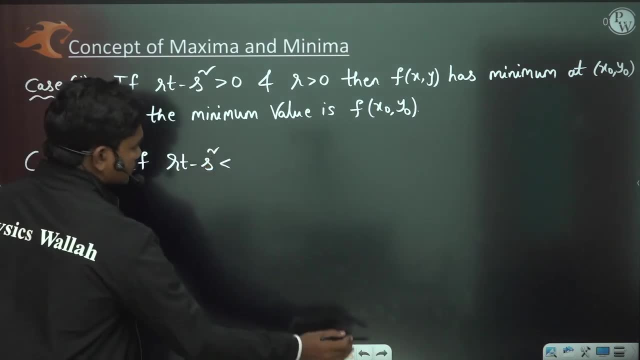 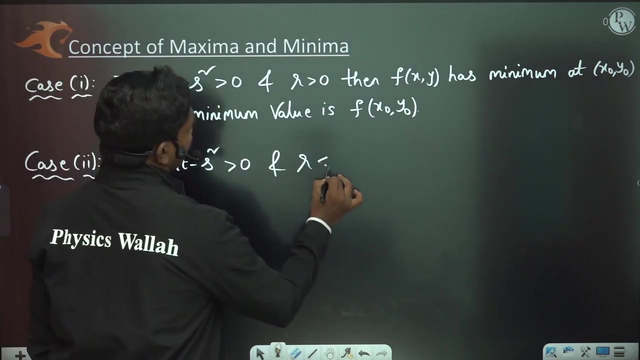 if r t minus s square is less than zero, means now let sorry, this is again greater than zero. if r t minus s square is greater than zero, okay so, and r is less than zero. look, this can happen. how it can happen? because here r is less than zero, t is also less. 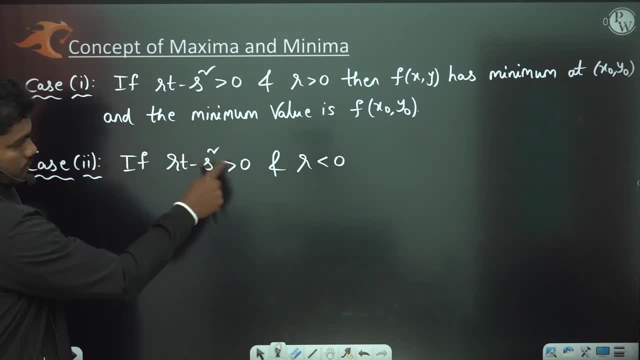 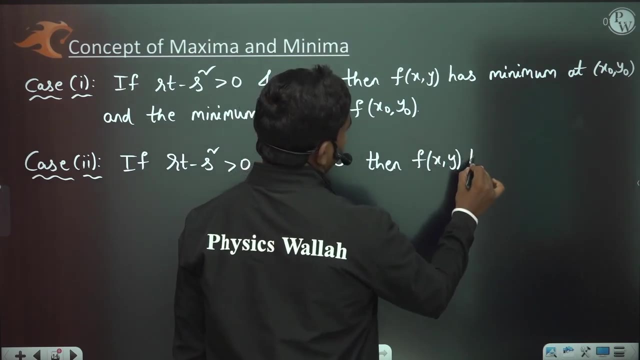 than zero, then there could be some s value, such that rt minus square is actually greater than zero. okay, if r is greater than zero, t is also greater than zero and s square is less than this, then this is some different combination. so then, f of x comma, y has minimum. minimum at x naught, y naught. 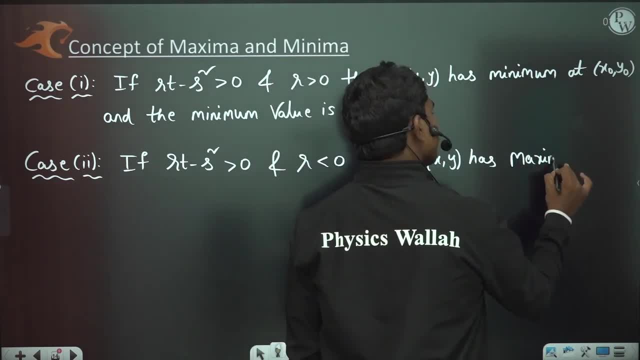 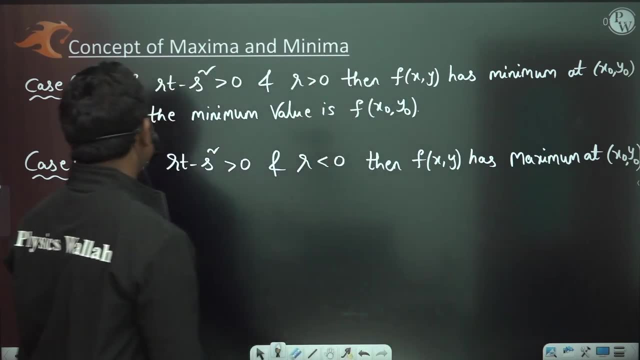 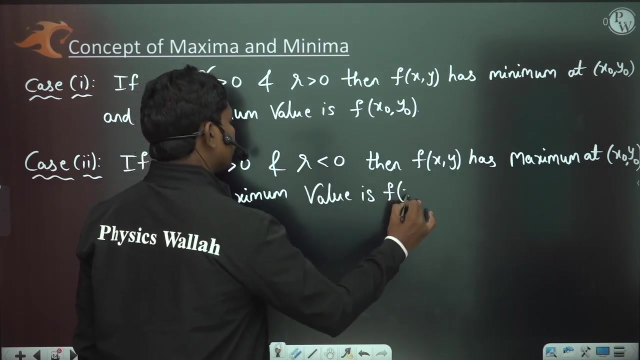 maximum Maximum At x naught, y naught. okay, at x naught, y naught, and The maximum value is: And The maximum value is F of x naught, comma y naught. Okay, so this is f of x naught, comma y naught. 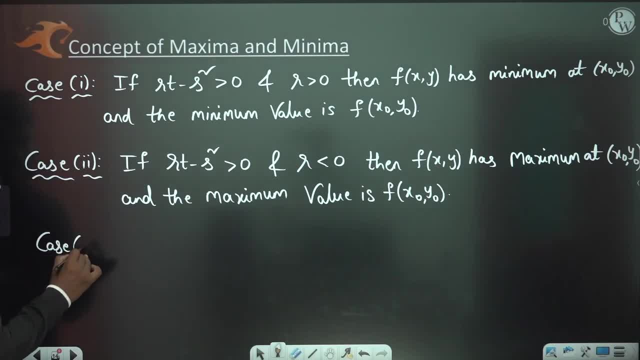 So now we have a case 3 as well. Case 3: now, what can happen? These are two cases. now Let us suppose this value is always positive and let us suppose if this Means, basically, if this value is always positive, minus s square is negative. Okay, so let us suppose if this is also negative means if 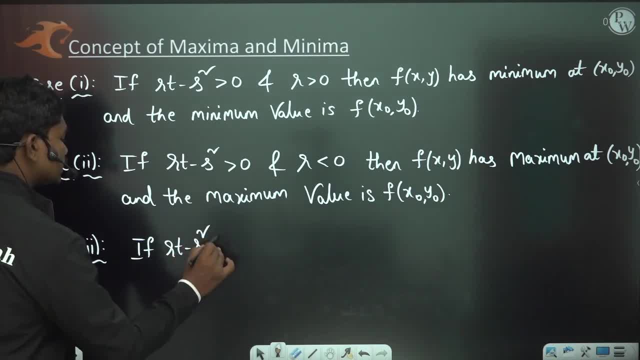 RT minus s square Is less than 0, for example, less than or equal to also 0, let us suppose if this is also equal to 0. if RT Minus s square is less than or equal to 0, then we can't comment on. Then we can't comment on. 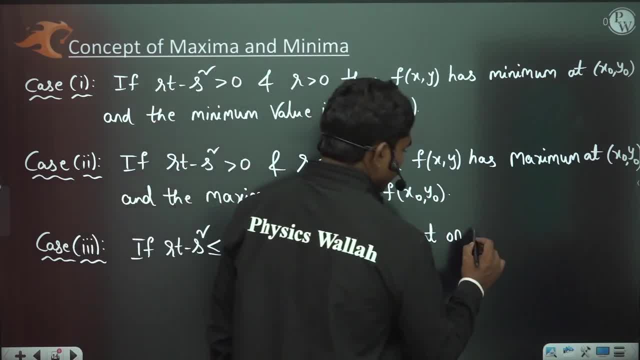 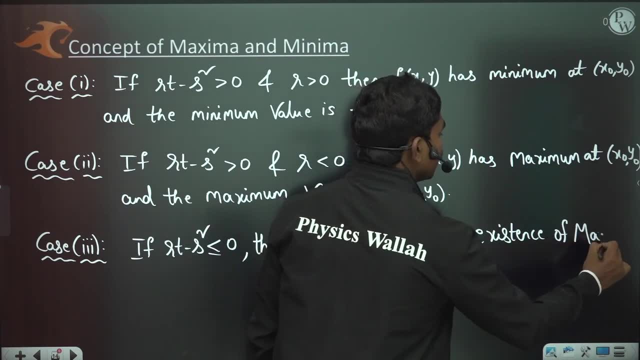 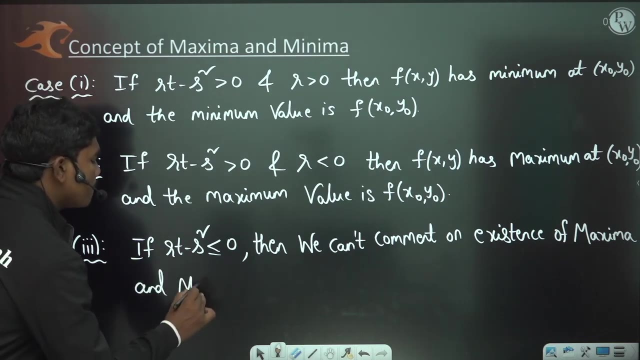 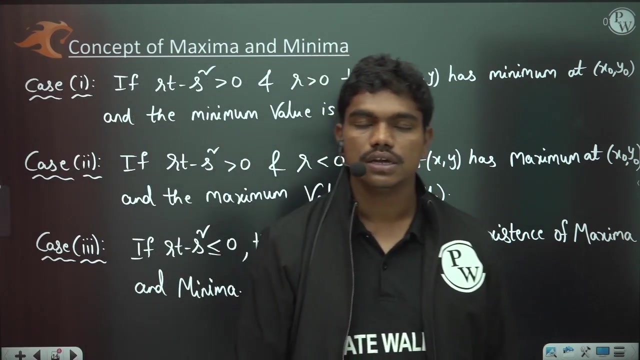 Then we can't comment on existence of maxima and minima. like in the last case, we can't comment on the existence of Maxima and minima. okay, so maxima and Minima And in case of single variable, calculus whenever we got such points means though. 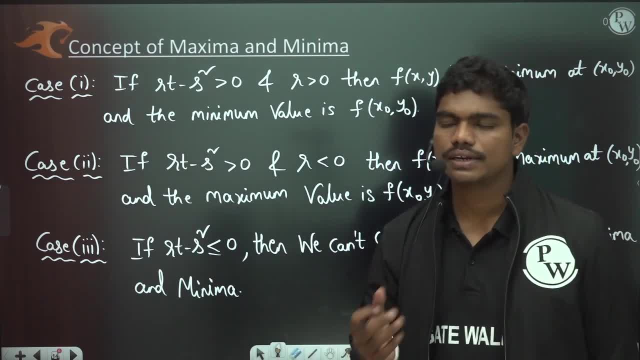 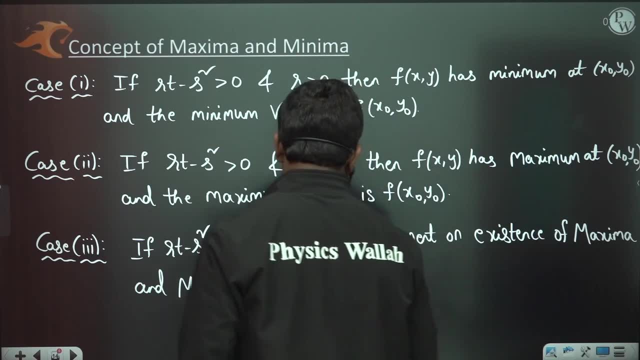 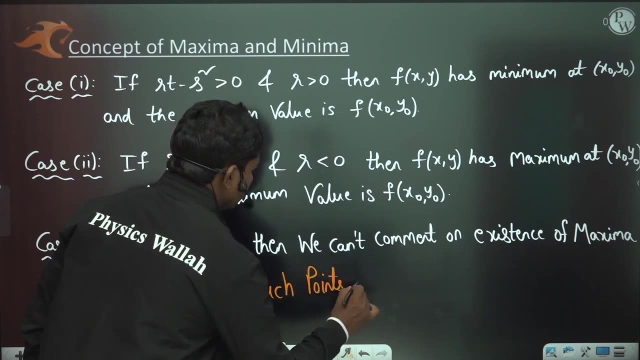 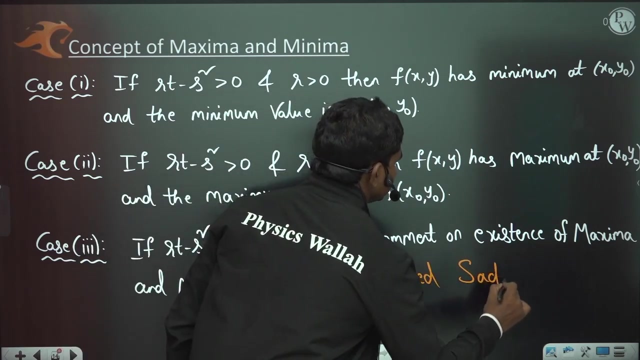 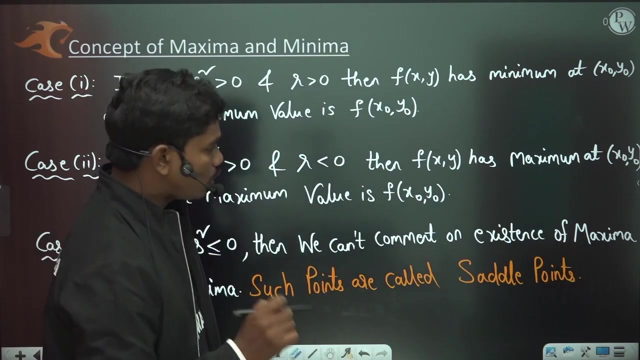 Those stationary points at which we don't have any maxima or minima, or we cannot comment about it. We call those points as points of inflection. Okay, Now, here, in such case, we call: such points are called: Such points are called saddle points. such points are called saddle points here. Okay, so these points which are at which we get a stationary point, 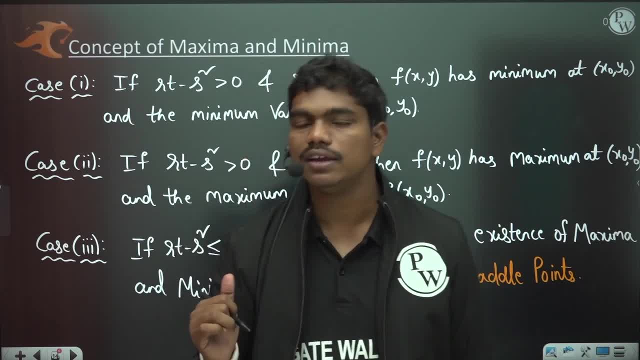 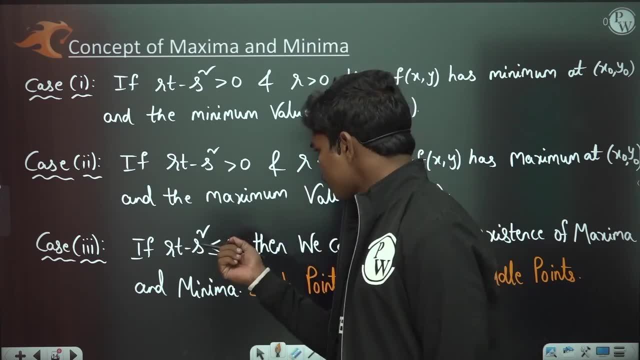 But at that point, if you calculate this RT minus s square value, If you are getting it to be negative, then such points we cannot at the. at such points We cannot comment anything on the, you know, existence of maxima and minima, And such points are called saddle points. 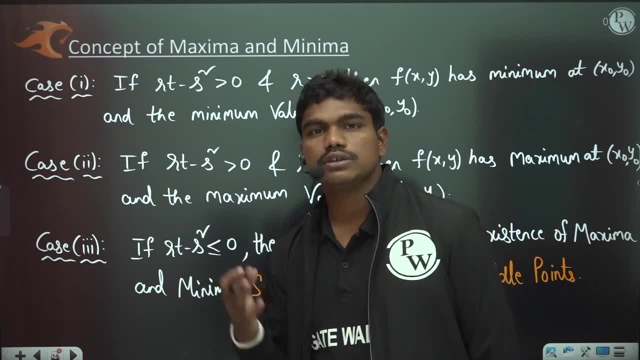 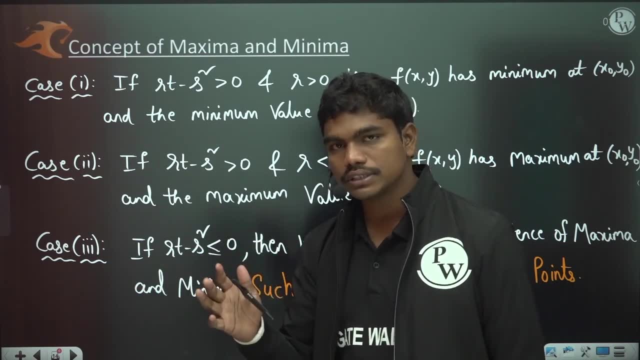 Okay. So in exam date sometimes ask you: the number of saddle points of the function f of X comma is equal to some you know function. They'll give you okay. so you need to do this analysis. You need to calculate PQ equal to 0, then you will get some equations. if you solve you'll get stationary points. 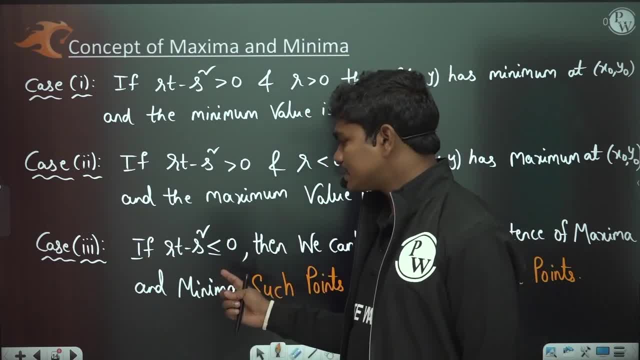 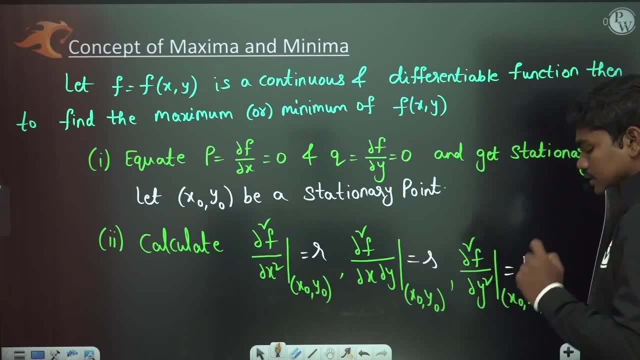 So you need to observe at how many stationary points this RT minus s square value is actually negative. Okay, So let us substitute means. if you see, our value: is this s? is this T? is this? so this is how you actually calculate the maxima and Minima: identify stationary points, calculate our st values. 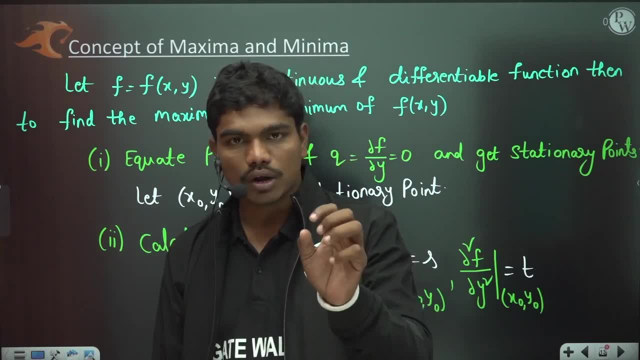 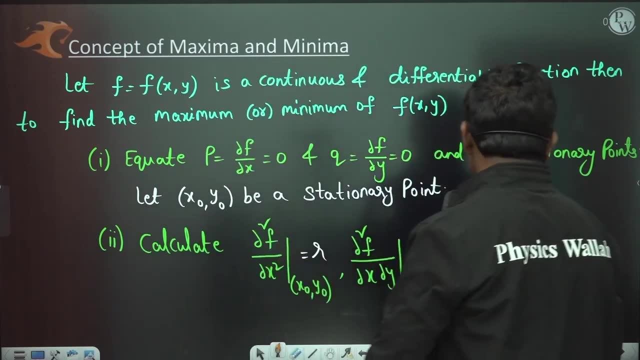 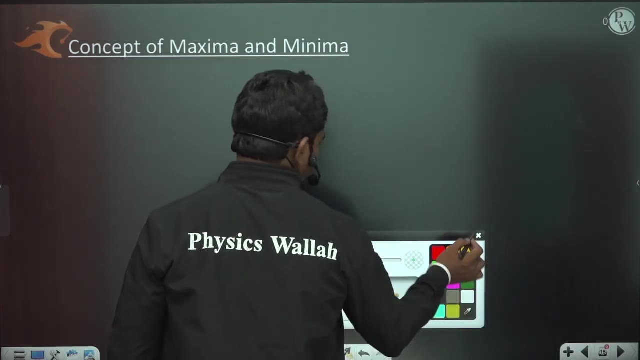 so, depending upon our T minus s square value and a smaller value, identify whether the Function has a maximum or minimum. all these things, basically Okay. So now let us See one example. okay, I'll ask a question, So let us try to solve that. 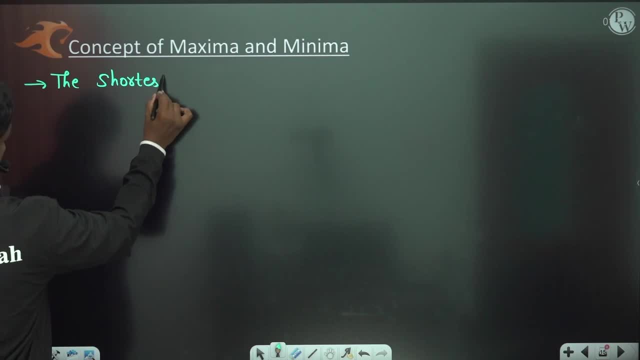 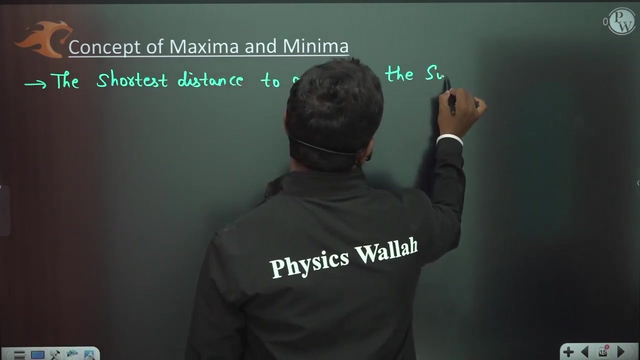 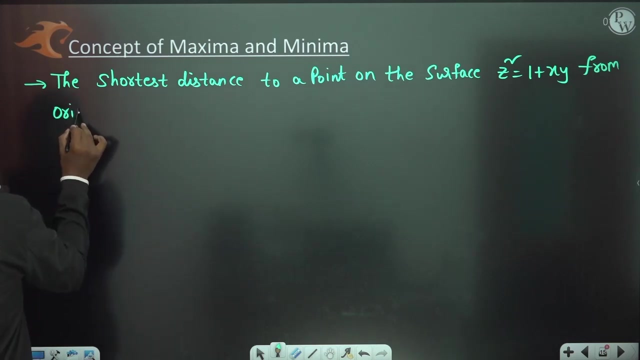 The shortest distance, That shortest distance To a point, To a point on the surface, On the surface, Z square is equal to 1 plus X Y. Z square is equal to 1 plus X Y from horizon. From horizon, let us say, from horizon, Is dash, let us suppose we have this question. 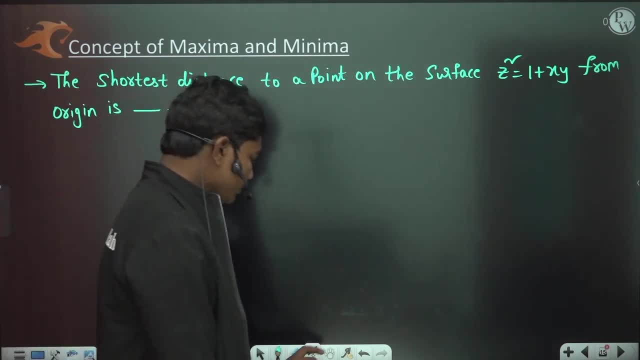 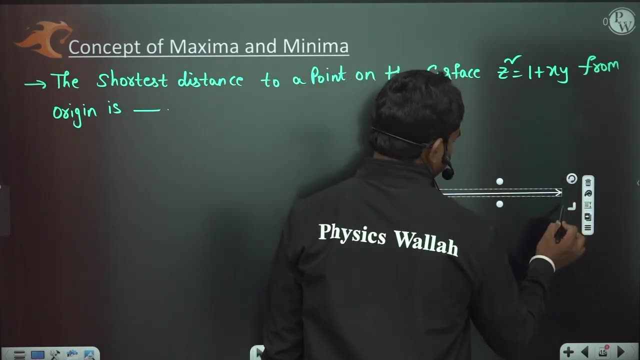 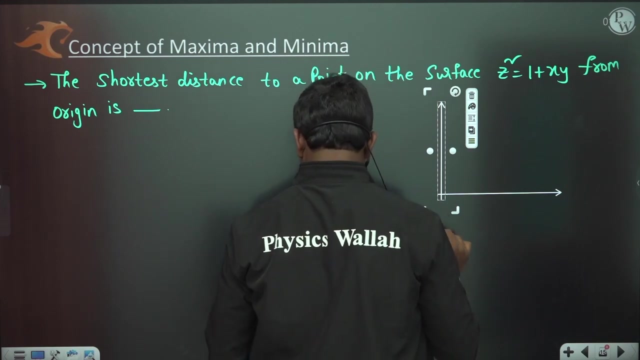 Okay is a dash, for example. now let us see if you have a 3d space, for example, Let us draw that. so X, X, we have Y, You have Y as well here. Okay, so this is horizon. Fine, let us write the horizon somewhere here. horizon. 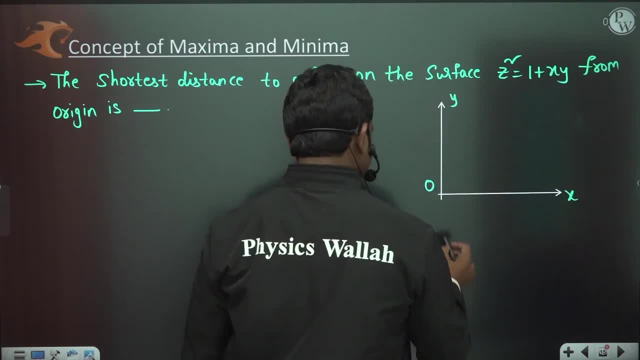 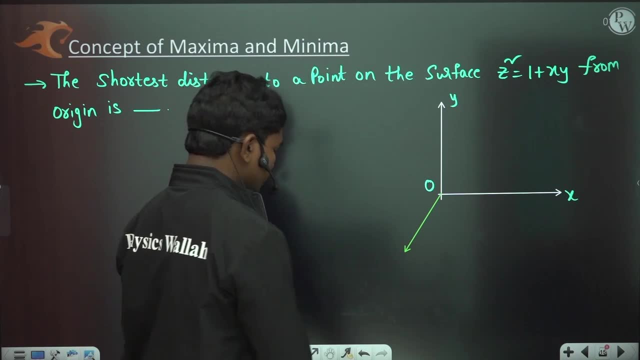 X, Y and let us suppose you have the third dimension. for example says Z like this: Okay, So this is Z axis. now what happens if you plot this surface? Z square is equal to 1 plus X, Y. Let us suppose the surface is some random curve like this: Okay, so the surface is some random curve. 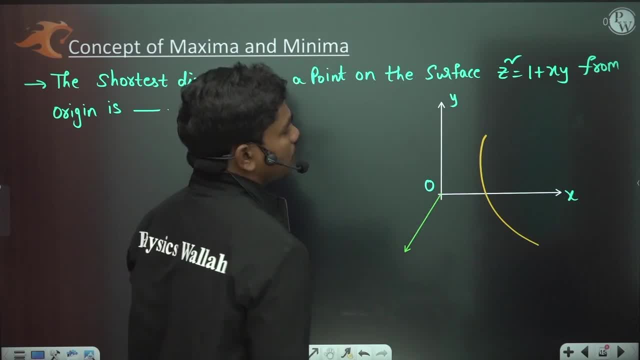 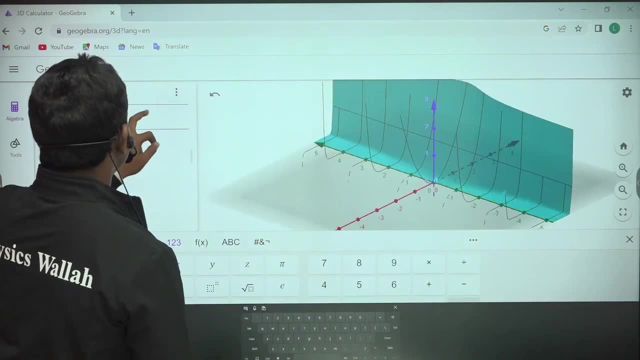 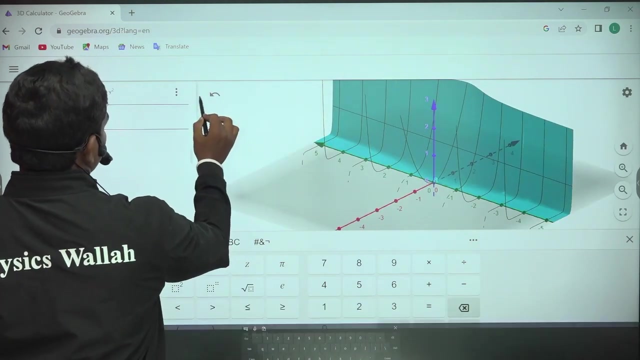 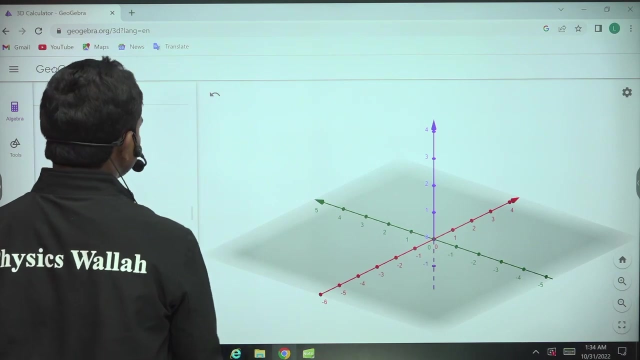 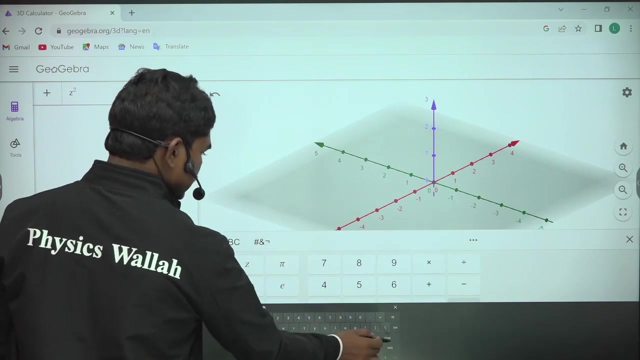 Okay so you can see some some something, some random curve like this. Okay so if you want to actually check the plot, you can check it here. Okay so, delete This. you can delete now. okay, so you have the coordinate system. now let us see: the Z square is equal to Z square is equal to 1. 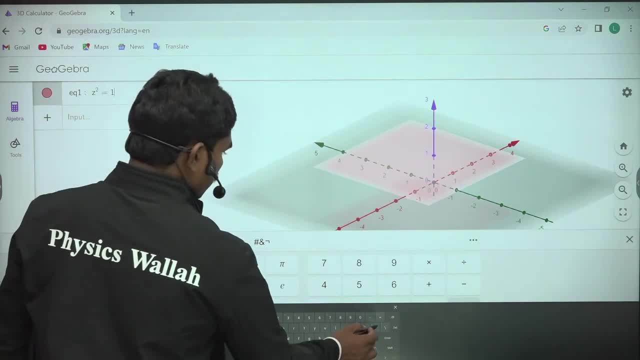 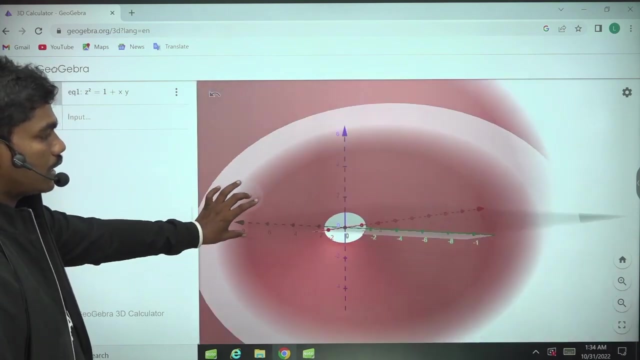 Z square is equal to 1 Plus X Y. Okay, so 1 plus X Y Z square is equal to 1 plus X Y. So if you see there is some complicated curve like this, okay, So there is some certain complicated curve, some donut kind of shape is what you have, and of course it's a complicated curve basically. 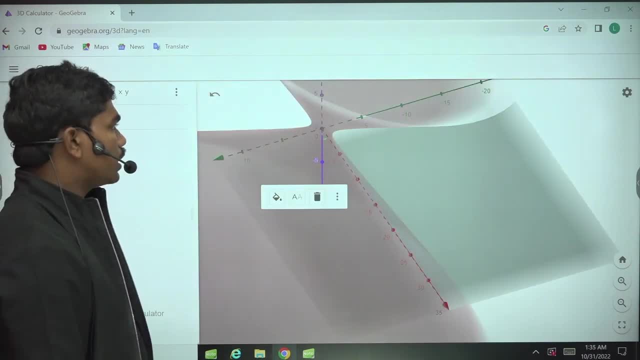 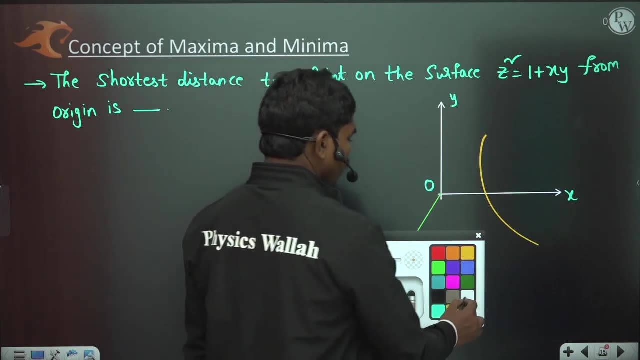 Okay. so now they are asking you: you see, there is certain distance, and all. now, if they ask you what is The shortest distance of the curve? This is the curve. Z square is equal to 1 plus X Y. for example, Z square is equal to 1 plus X Y. 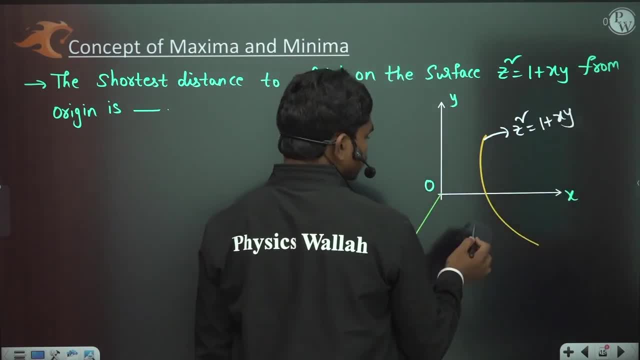 So definitely there could be definitely one point at which this point, for example say this point X comma Y comma Z on 3d space is actually very close to the horizon. For example, let us suppose this is the shortest distance between this curve and the horizon. now, 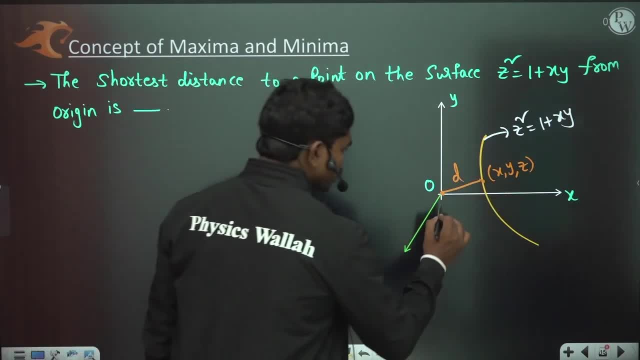 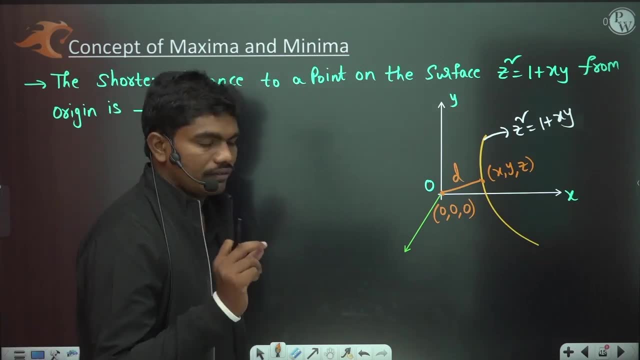 How do you actually calculate this distance? Look, this point is horizon, This point is horizon. So tell me one thing: if D has to be small, or if D has to be minimum, then D square is also minimum, correct? So if you see, if D is minimum, 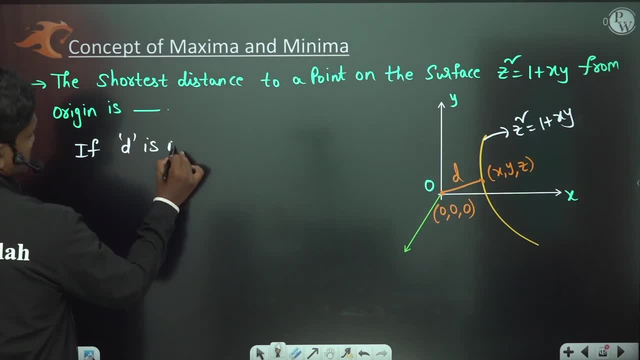 If D is minimum. If D is minimum, Then definitely D square is also minimum. D square is also minimum, correct? D square is also minimum. Now, what is D square value? D square is equal to look. D is nothing but the distance between these two points. and you know in theory. 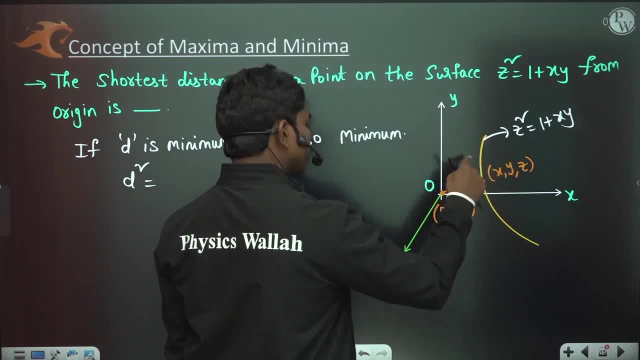 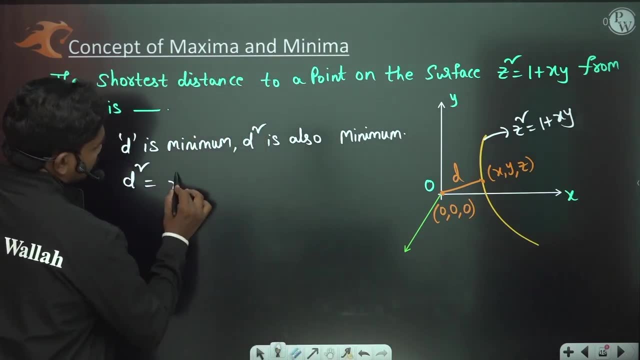 The distance between three points is square root of X 2 minus X 1 whole square plus Y 2 minus Y 1 whole square, plus Z 2 minus Z 1 whole square. But here we are considering D square. This value is nothing but X square plus Y square plus Z square. 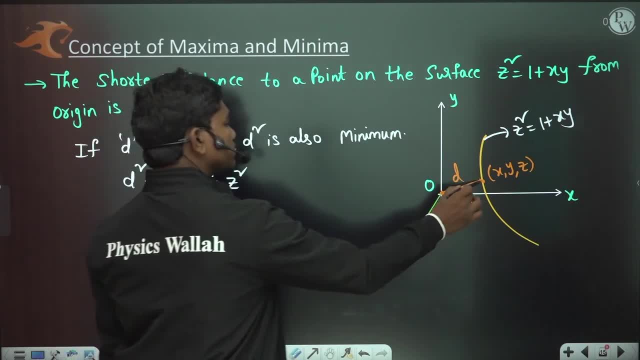 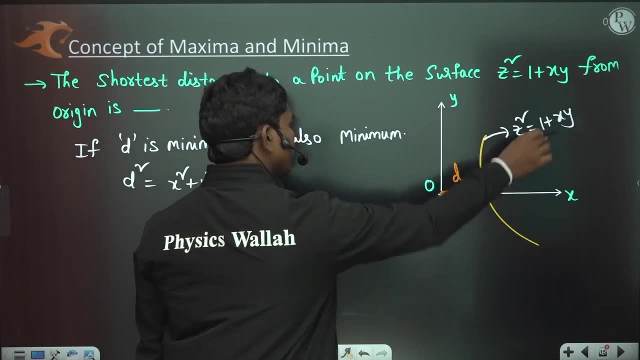 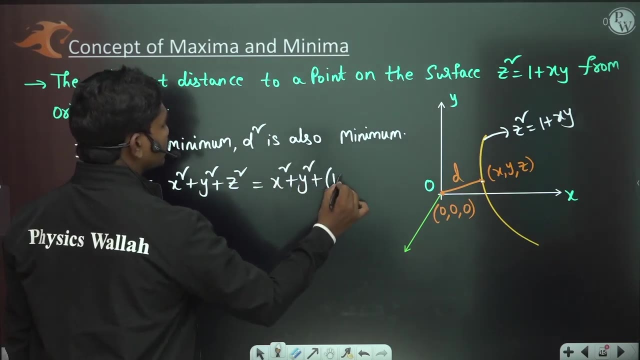 Okay. So now if you see this point, X, Y, Z is on this surface means if there is something about Z, I can replace this Z square value at any point on this curve with this equation, correct? So if you see, this equation is nothing but X square plus Y square plus 1 plus X Y. 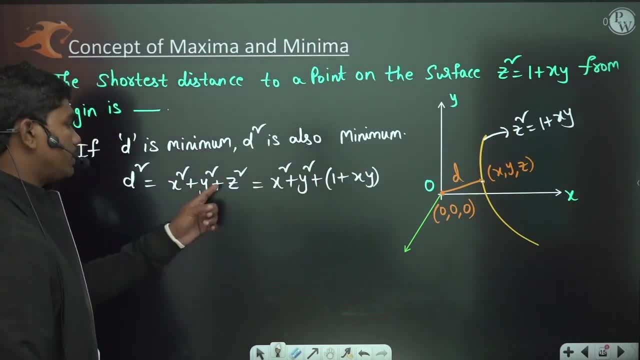 How I am writing this: 1 plus X Y, Because this point X Y, Z is. on this surface, Z square is equal to 1 plus X Y. Okay, so if Z square is equal to 1 plus X Y, then Since this point is on that curve, 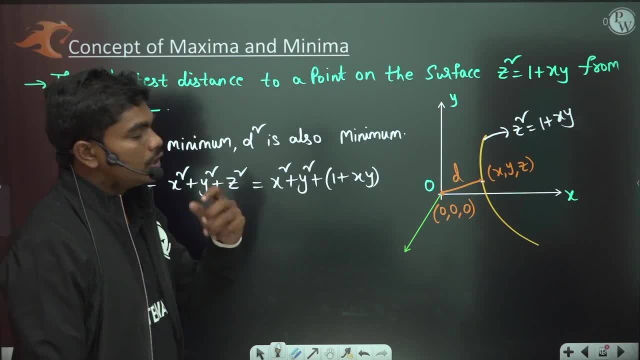 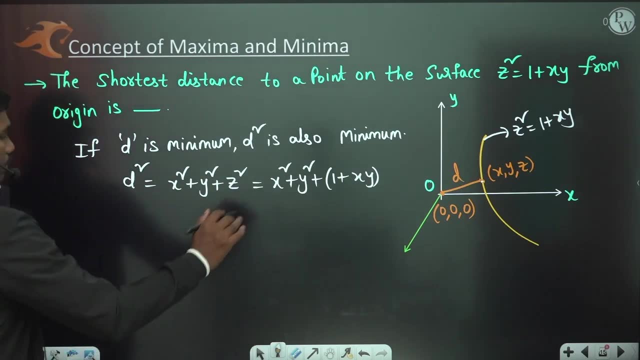 We can write X square plus Y square plus 1 plus X- Y. Now you want the minimum value of this, actually okay, So let us calculate what is the minimum value of this function, For example. now, if you calculate the minimum value, you have a function f of is equal to some function. 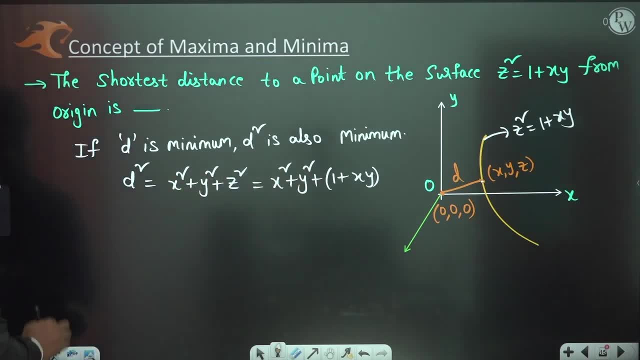 So you want to calculate the minimum. how we will do this? Okay, So first step: you can see, let us go by step by step procedure. so first step: equate p and q is equal to 0. so what is p? basically, p is equal to dou f by dou x. let us say so. what is dou f by dou x? on this: 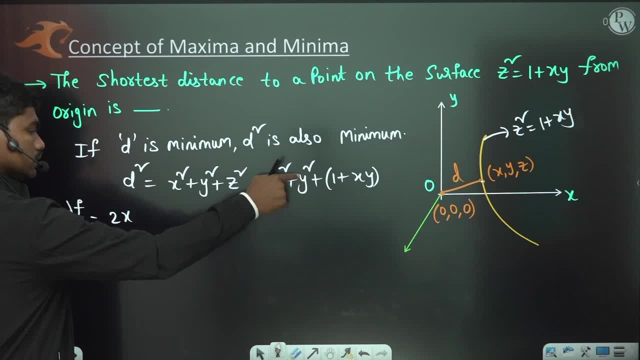 equation 2x plus differentiation of y square with respect to x: 0, 1 is constant, 0 plus x, y, so differentiation of x, y with respect to x is y, so this term is equal to 0. so this is one equation. and what about q? q is equal to differentiation with respect to y, so 2y plus x is equal to 0. 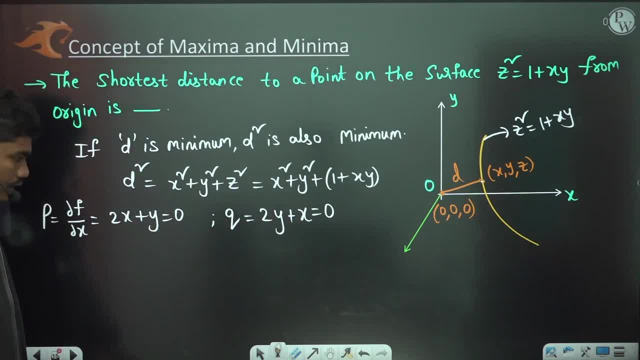 so these are two equations which we got. actually okay. now you need to solve these two equations to get the stationary points and undoubtedly you know both these are linear equations and this: both these have constant 0, so these two lines are actually passing the horizon. so if you see, 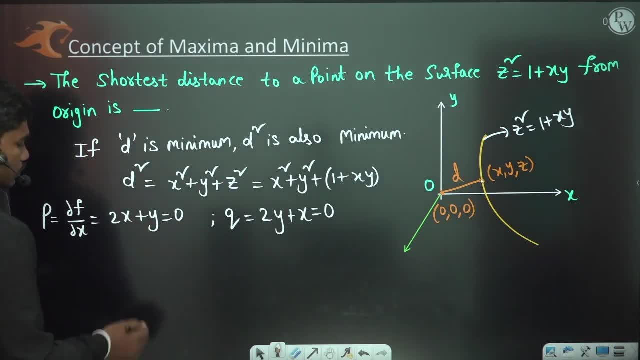 if you calculate the point of intersection means if you solve these equations, you will get 0 comma 0, 0 the stationary point. okay, so because if you see, these two are the straight lines which are passing through horizon. so if these two are the straight lines passing through horizon, 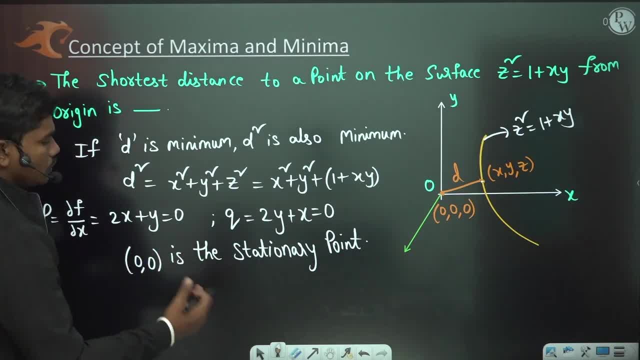 then yes, definitely. uh, you know, if you solve this equation also, you'll get 0 comma. 0 is the stationary point. okay, so now let us calculate our second step: dou square f by dou x square. so what is dou square f by dou x square if you differentiate this partially, with respect, 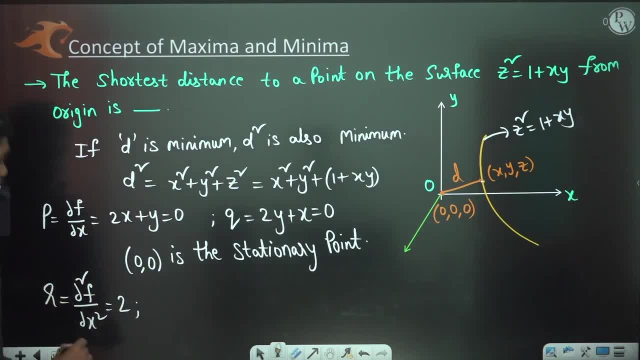 to x again, you will get 2. okay. so here one thing that is required: r is greater than 0. good, now let us calculate the yes value. yes is dou square f by dou x, dou y. so if you calculate dou square x by dou x, dou y, so this is nothing but dou by dou x of dou f by dou y, so this is dou f by dou y. you need to. 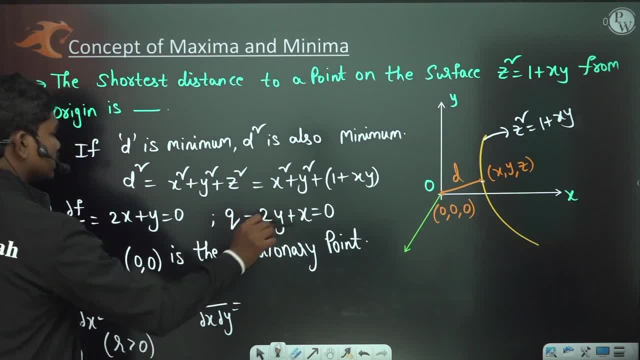 differentiate this partially with respect to x. so if you differentiate partially with respect to x, you have one. of course, in rs you don't have any xy values. if there is some xy value, you would have substituted j rer comma zero here. okay, next t. t is equal to. 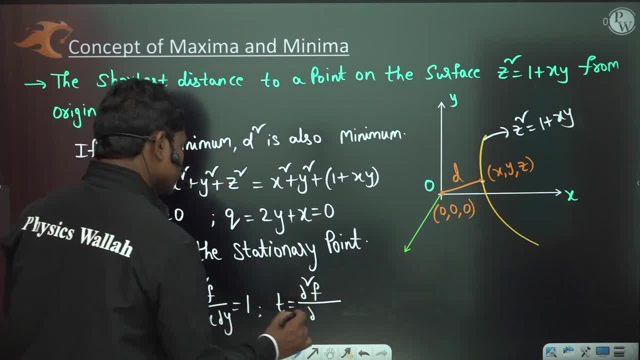 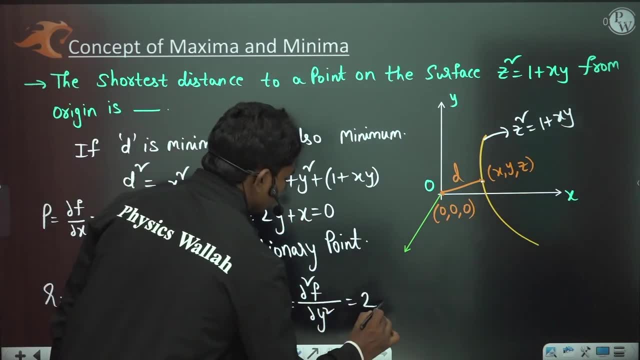 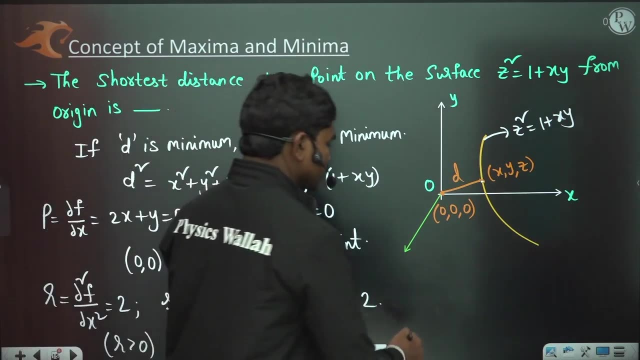 dou square f by dou x or dou y squared, double square by dou y square. so if you differentiate this partially with respect to y, you will get two actually here. okay, so all these are constants directly. you need not substitute any x comma, y points here. okay, so if you calculate r t minus s square, r t minus s square, this is equal to: 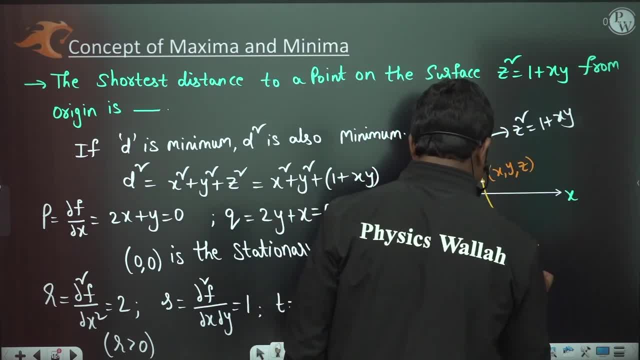 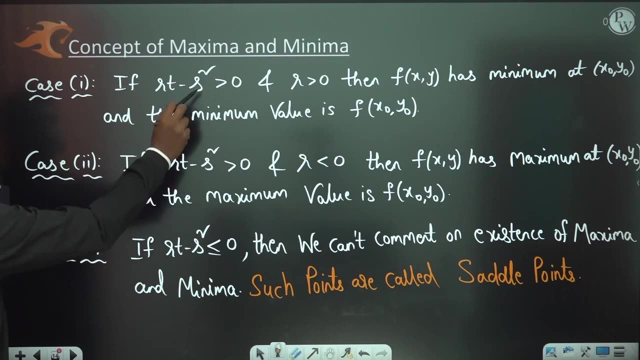 smaller value to t value. again to minus s square. so one: this value is actually positive and r is also greater than zero. so if you see if r t minus s square is positive and if r is greater than zero, you can see r t minus s square is positive and here r t minus s square is positive. 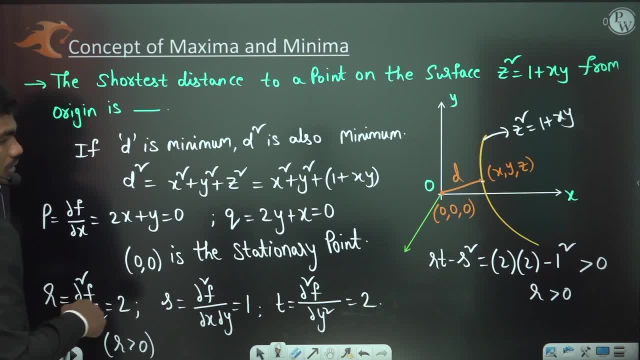 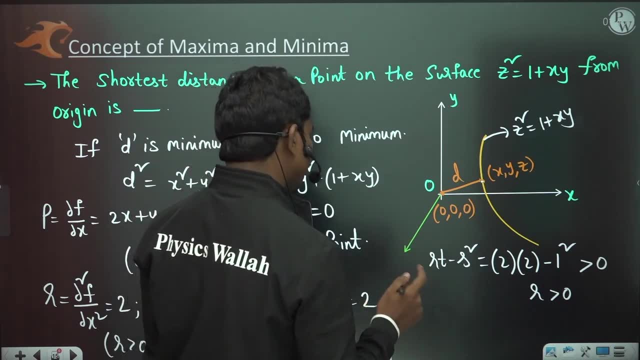 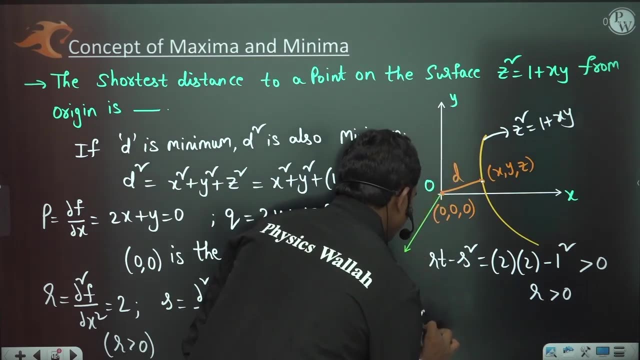 and r is also greater than zero, then the function f of x comma y has minimum. obviously, and in the question they are also asking about, the shortest distance means minimum value of d actually here. okay, so if you want the minimum value of d, what you can do, so this implies minimum value of d. 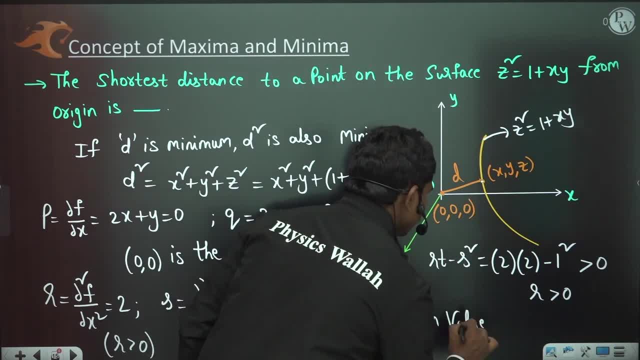 square, because d square is the function, minimum value of this function, which is nothing, but you can do it like this, and then you can do it like this, and then you can do it like this, and x square plus y square plus 1 plus x, y, which is actually your d square. so, minimum value of d: 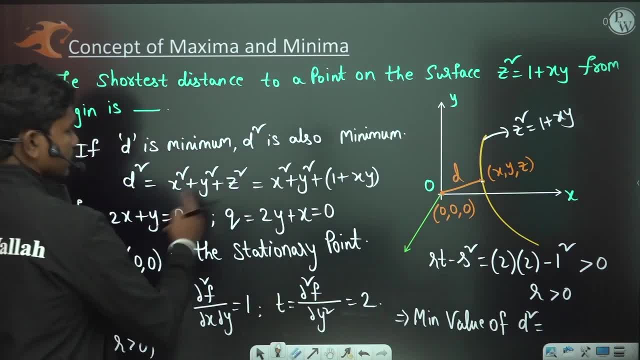 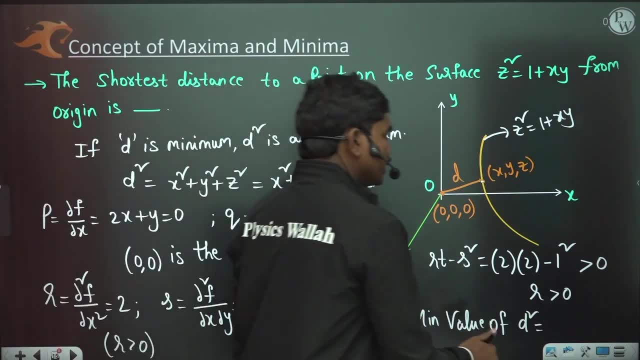 square is actually equal to. if you substitute 0 comma 0 in this x comma y, so x is equal to 0, y is equal to 0. you have only 1 that is left over. so minimum value of d square is 1. this implies d. 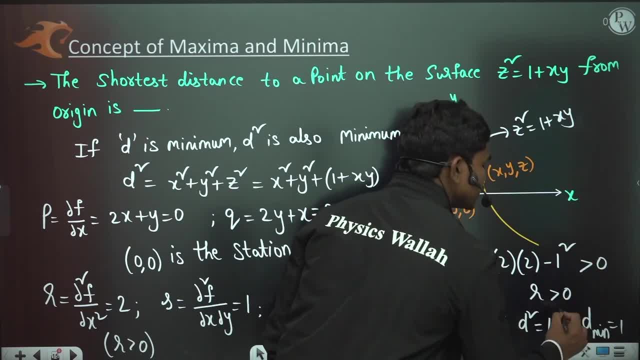 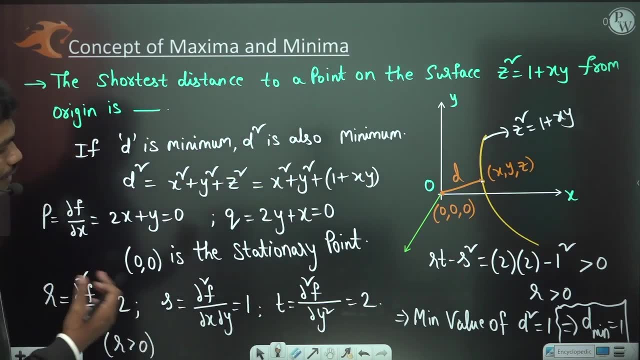 minimum is also 1, because square root of 1 is 1. this is a distance. it cannot be negative, so we will take only plus 1, okay? so if you can understand, we can we actually apply the concept of maxima and minima, of two variables here and we have deduced this. okay, so the shortest distance to a point. 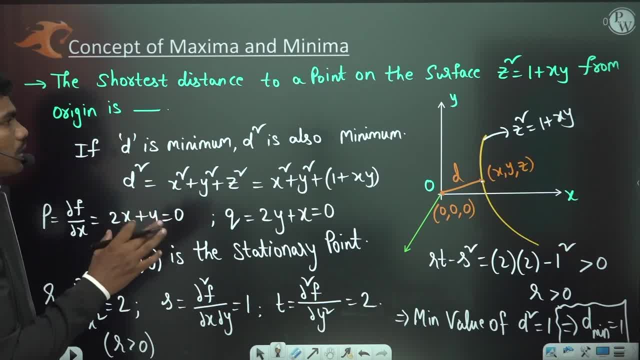 on the surface, z square is equal to 1 plus x. y from horizon is dash. this is what you actually got here. okay and yes. so this is how we have calculated this first step. we have calculated p and q. we have calculated dou f by dou x, dou f by dou y, equated them to zeros. then we got certain. 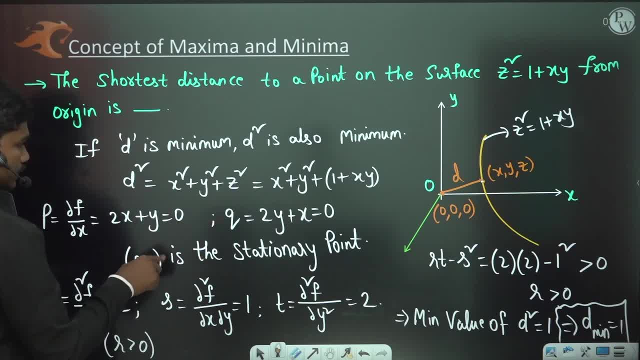 result though. so if you solve these two equations, you will get the point as 0 comma 0. you actually need to calculate this. you actually need to calculate this. r s t values at this point horizon. okay, but here they didn't give us any chance for the substitution. 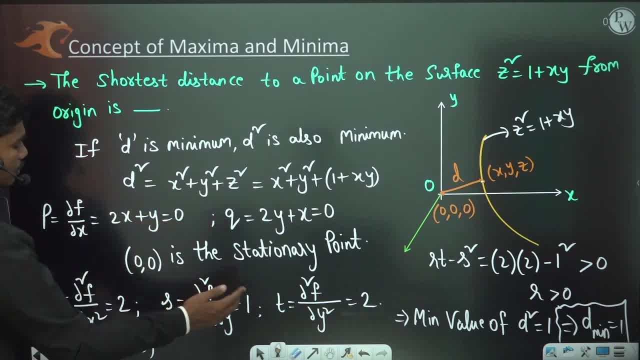 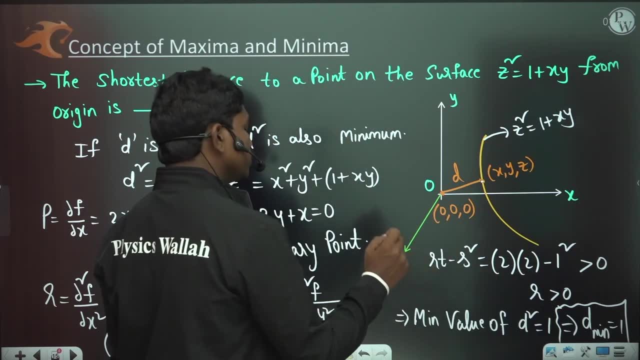 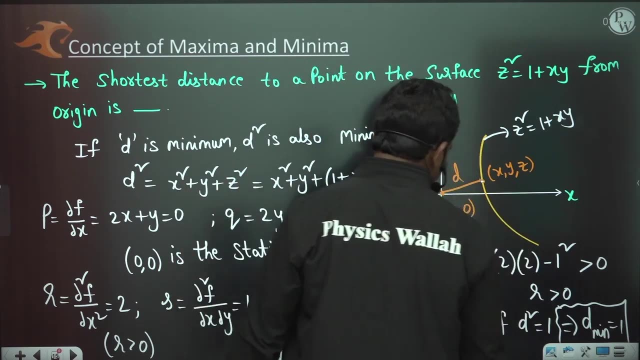 because they buy some. by differentiation themselves, they become constants actually. okay, so we check this condition- that r t minus a square and smaller. both are actually greater than zero. so minimum value means, if you see, this is the point at which this function is having minimum. okay, so what is? 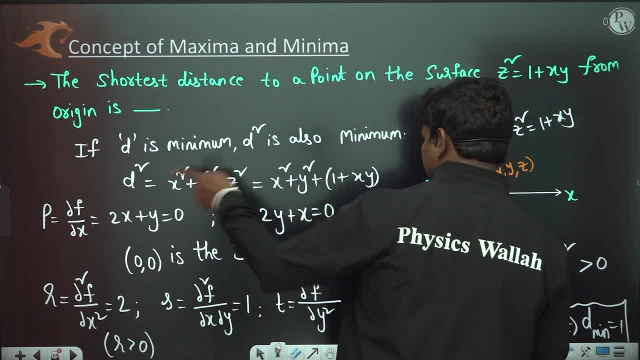 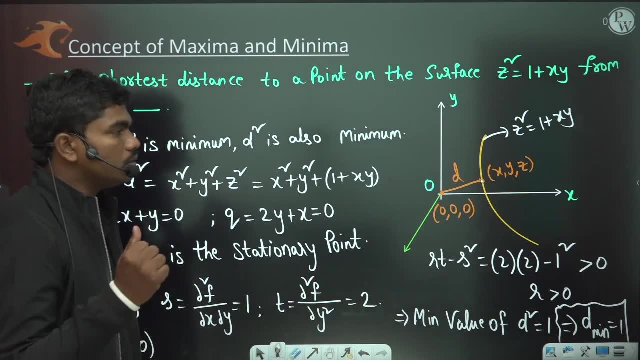 the minimum value. if you substitute this point in this equation, then you will get the value of d square. so that's how minimum value of d square is equal to 1 and this tells you that d minimum value is actually equal to 1 here, clear. so i hope that is clear to you. so let us try to solve one more question. 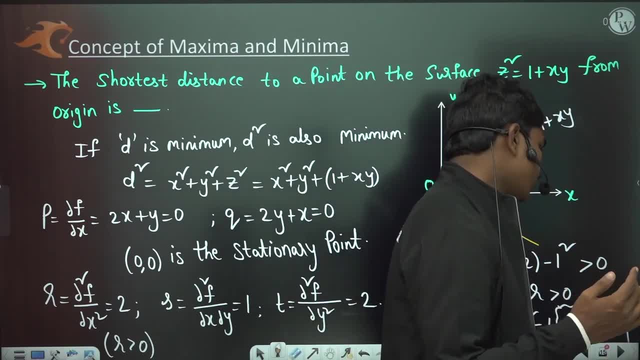 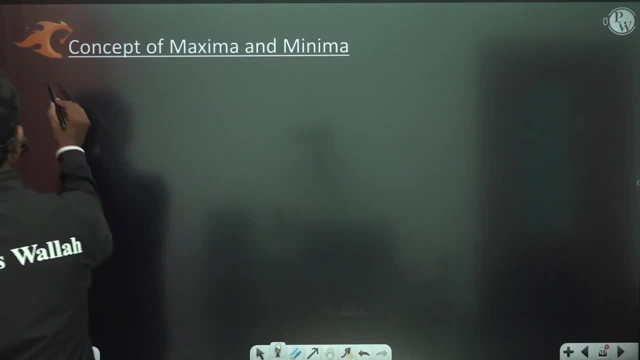 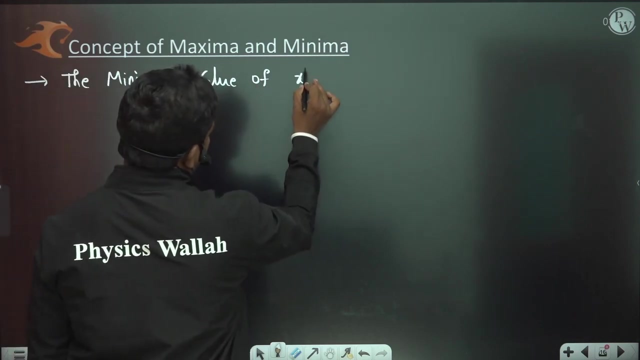 actually, so let us try to solve one more question. so, where is this? okay, fine, so let us solve one more question. actually, the minimum value of the minimum value of x square plus y square minus 4x plus 8y plus 4. okay, so let us suppose, if you. 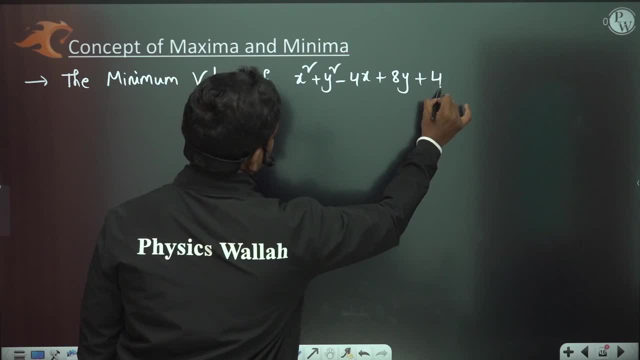 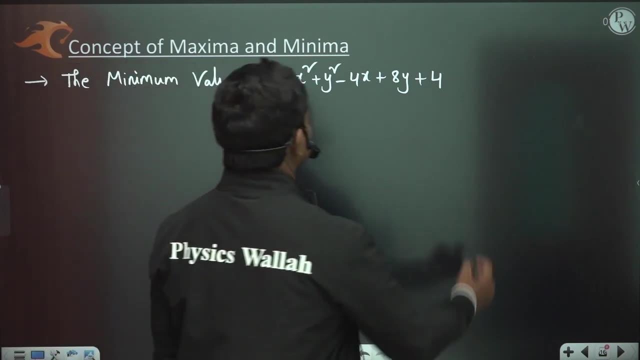 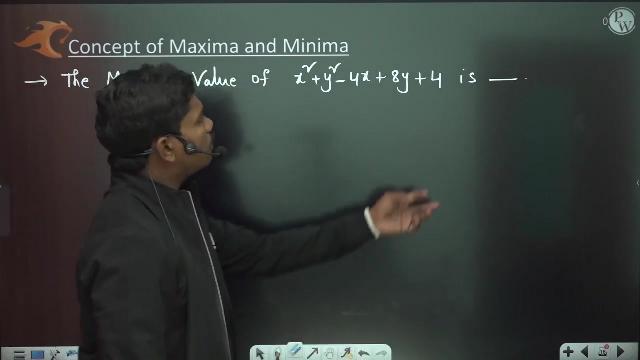 write this, for example: so plus 4. let us say say: let us say plus 4 is dash, for example, if i ask you this question, okay, so let us suppose it is some function: x square plus y square, minus 4x plus 8y. okay, instead of 4, some other constant, you can write t square, for example. let us say t square plus 4. 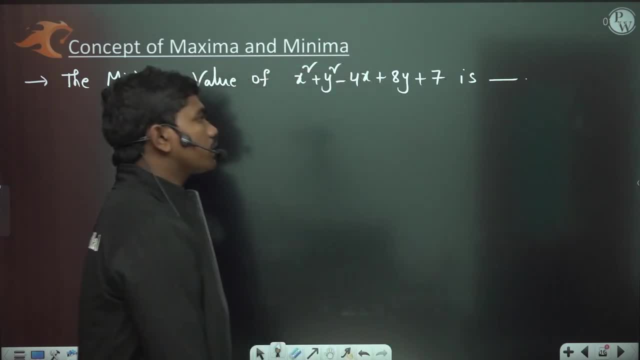 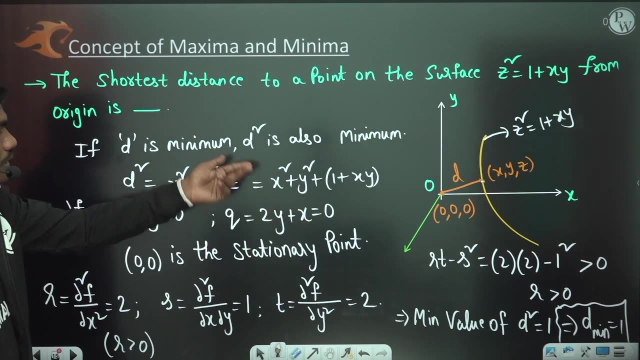 7, something, whatever you want. 7 is dash. okay, now let us see how to calculate this. it's like the same example, what we have taken. you know the function directly now. this time, previously, in previous case, you need to have some knowledge on geometry, like what is the distance between two? 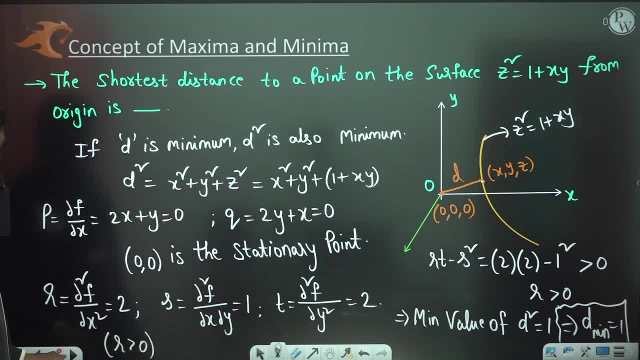 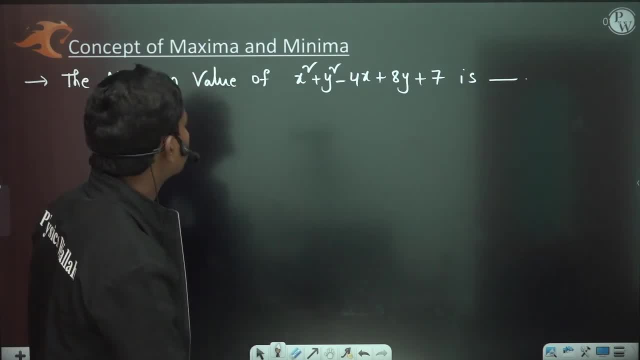 points and how to replace this z square with 1 plus xy. but here, straight away, there is a question like this: x square plus y square minus 4x plus 8y plus 7 is dash. they are asking you the minimum value of this. okay, so let us work out some procedure. so if you want the minimum value, 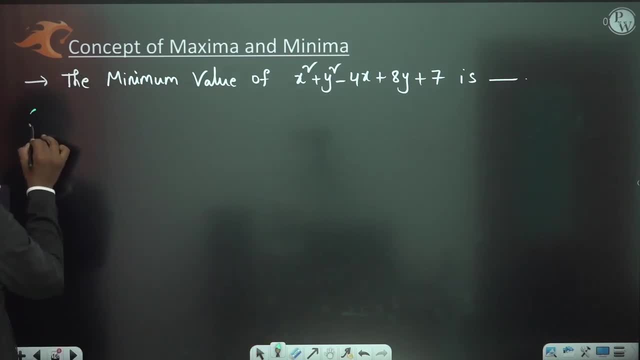 what you will do. you actually need to take first step: calculate p. p is equal to. if you differentiate this partially, we have 2x. y square differentiation is 0 minus 4. 8y differentiation is 0. 7 is also 0, so equate, this is equal to 0. similarly, q. 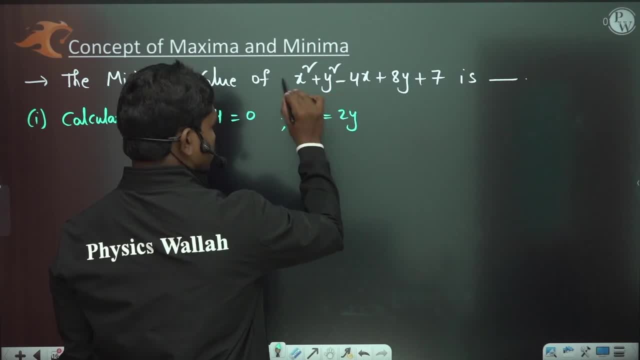 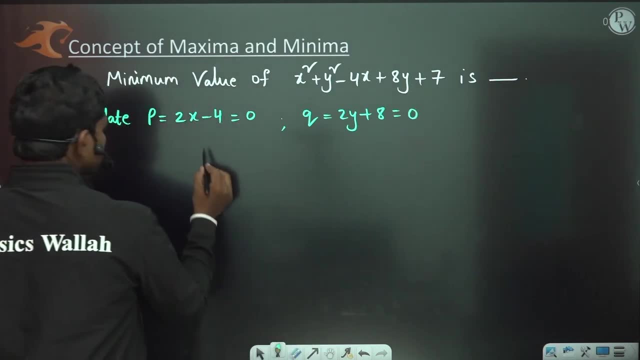 is 2y because x square differentiation is 0, 4x differentiation is 0 plus 8 is equal to 0. so if you solve this equations, you will get: x is equal to 2 and y is equal to minus 4. so if you. 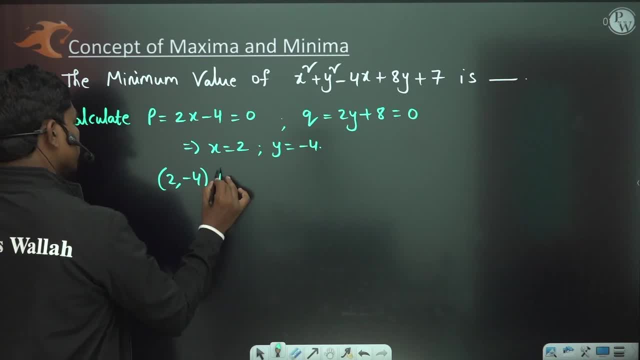 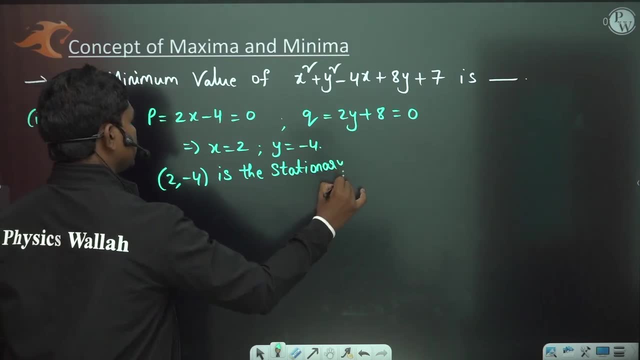 see 2 comma minus 4. is the stationary point? is the stationary stationary point? okay, so this is stationary point, okay. so if this is your stationary point now, second step: calculate our value. so calculating smaller is equal to now. if you differentiate this function with respect to x, once again, what will? 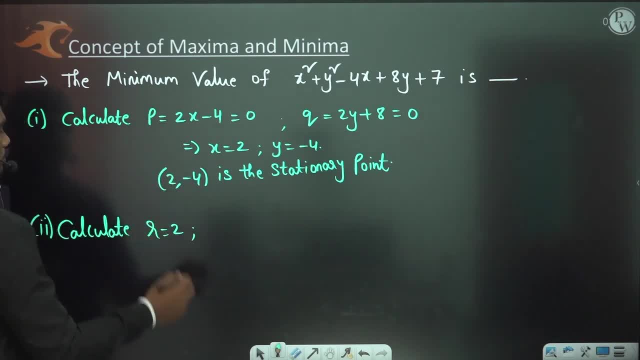 you get, you will get to directly, okay, and there is no need of substitution of any point here. so s is equal to dou by dou x of this value, okay. so if you calculate dou by dou x of this value, you will get 0 directly. p is equal to dou by dou y of this value, which is 2. 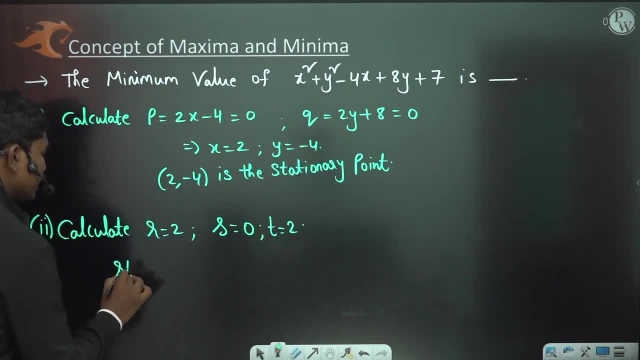 so directly. you got the values again. so if you calculate at t minus s square, this is equal to r, t minus s square, which is 4, which is positive, and r is also positive actually. so this means at this point, 2 comma 4, this function has a minimum value. that's what we are asking, actually. so if they ask, 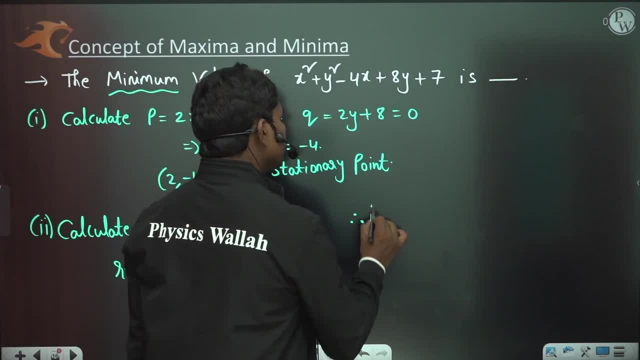 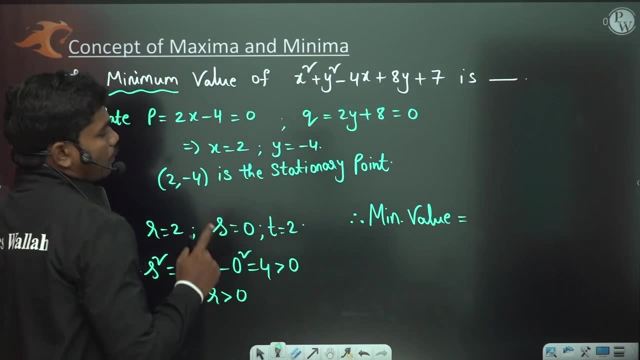 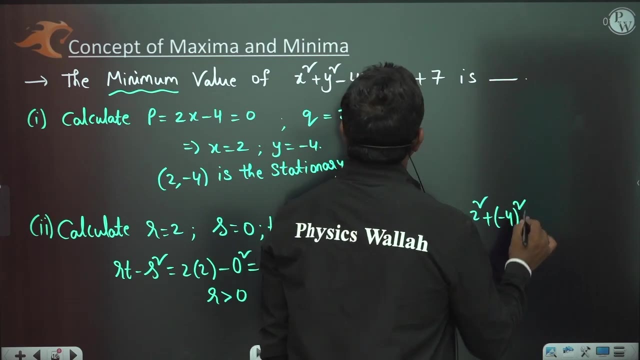 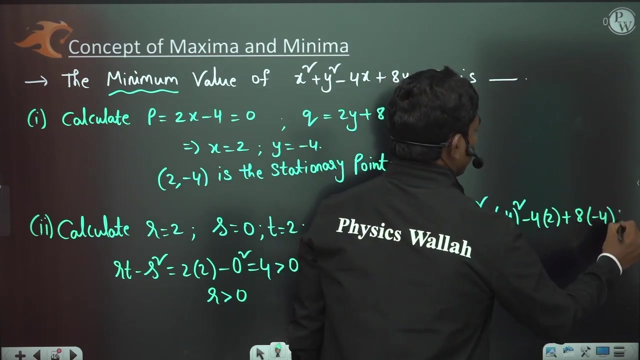 you, then minimum value is equal to. minimum value is equal to: this is at the point two comma minus four. so let us substitute two comma minus four here, so two square plus minus four, square minus four, into two plus eight, into minus four plus seven. so this is the value. so if you simply substitute and if you simplify this, 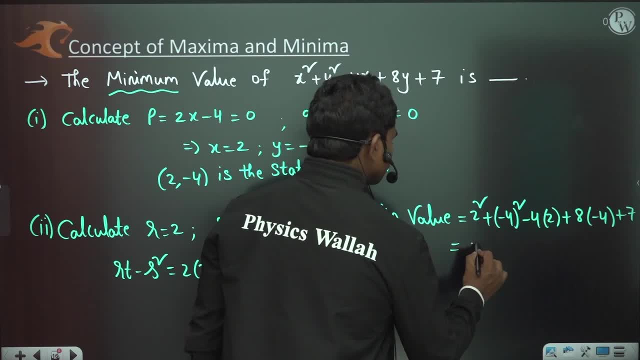 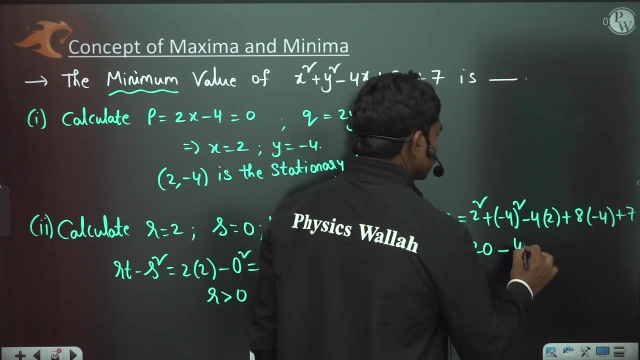 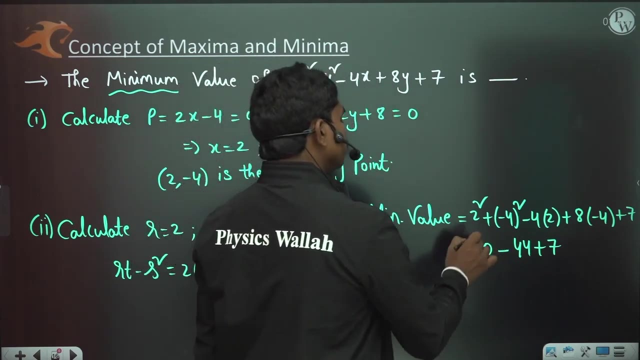 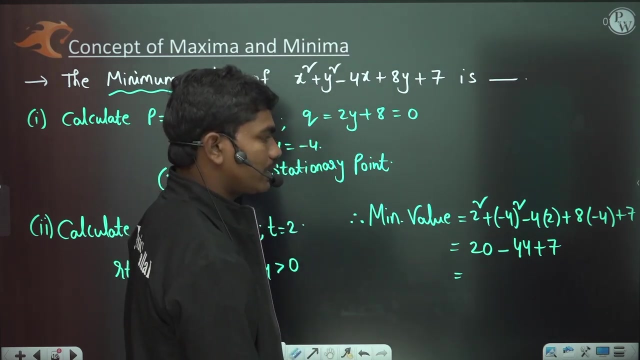 result: four plus sixteen, twenty minus twelve minus thirty two. so minus twelve minus thirty two minus forty four plus seven. so twenty seven minus forty four. so if you see, this is minus twenty four minus twenty four and plus seven actually. okay. so minus twenty four plus seven. so what is twenty four minus seven seventeen, correct? so minus seventeen is what you will. 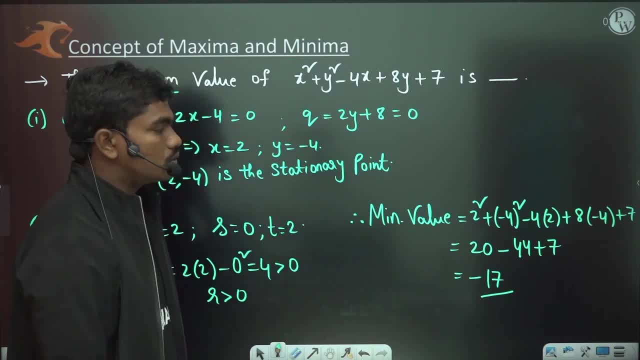 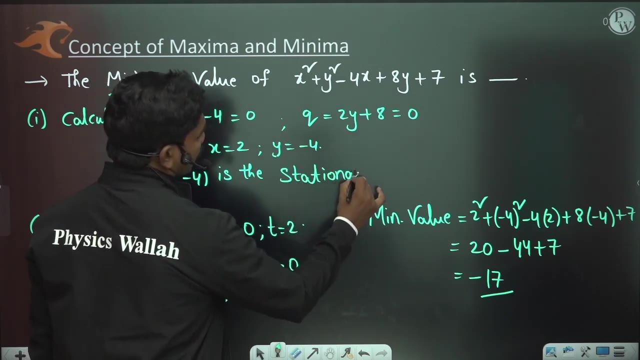 have as the minimum value actually here. okay, so this is how we will calculate the minimum value of this function now, for this particular function, without doing all this analysis. also, you can still tell the answer. how? come? think a while. you can pause the video for a moment and you can tell me how you can. 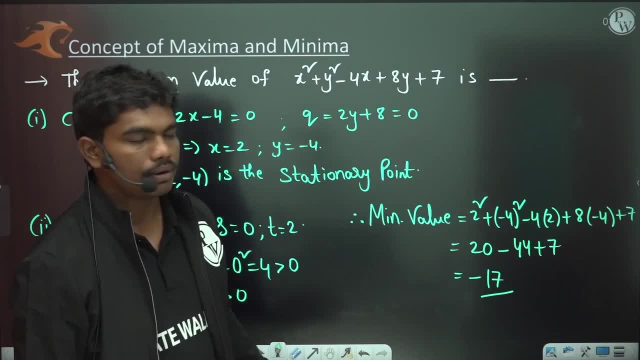 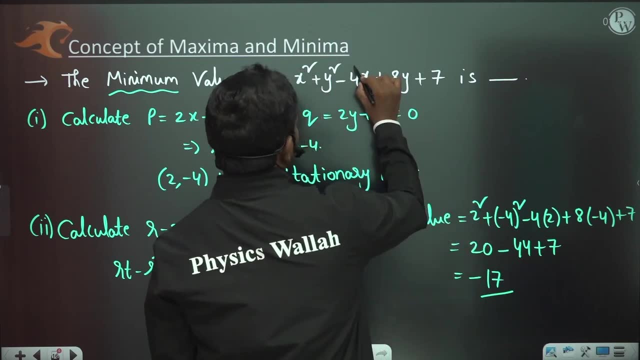 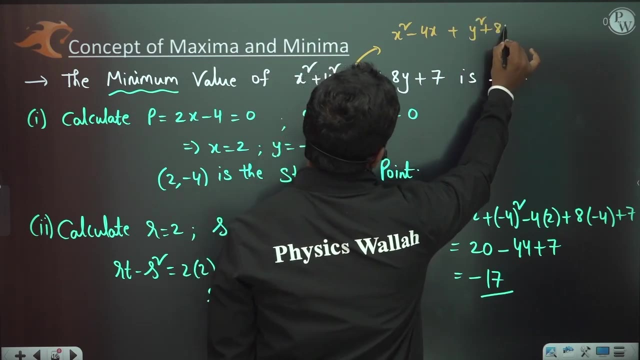 actually, uh, you know, calculate, uh, the minimum value of this. look, if you try to adjust the terms slightly, look, this equation can be written like this: or this expression you can say can be written like this: x square minus 4x plus y square plus 8y plus 7. so let us suppose, if you convert, 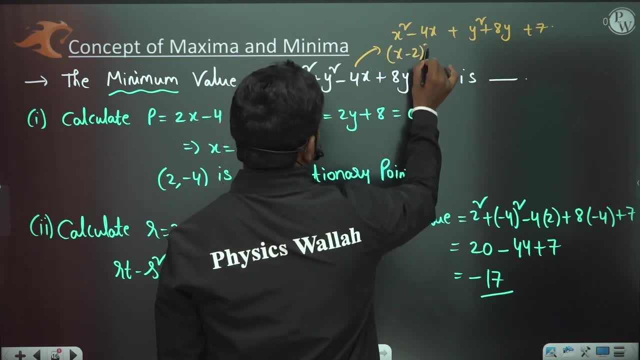 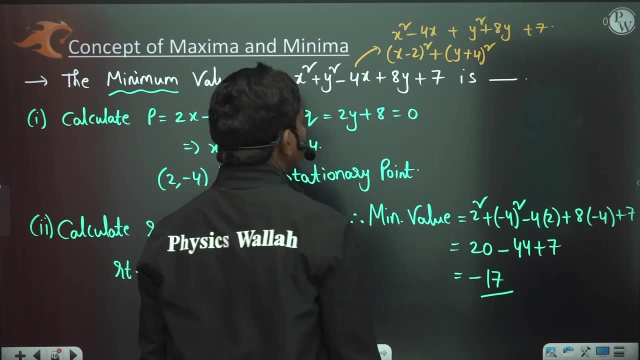 this into x minus 2 whole square, then plus. if you convert this to y plus 4 whole square, for example: okay, so x minus 2 whole square plus y plus 4 whole square, okay, then you will get x square minus 4x term, y square plus 8y term. now let us adjust the constants. here there is plus 4. 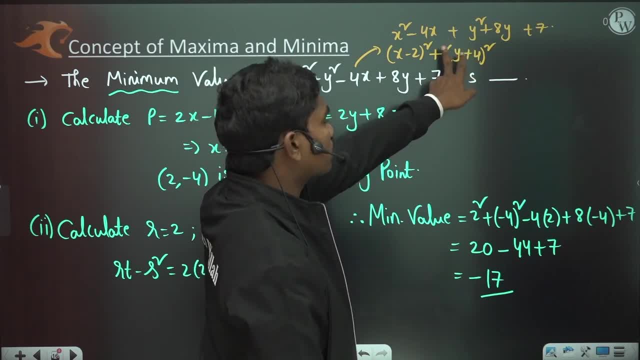 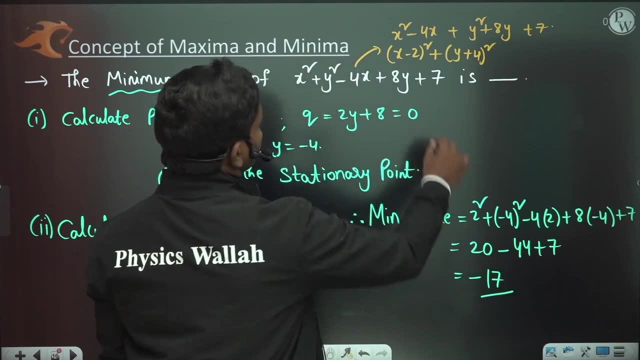 and here there is plus 16. so total 20 you have. but out of this 27 is already there. so minus 13 is what you will have here, correct? this is minus uh plus 4 you have and here plus 16 you have. so if 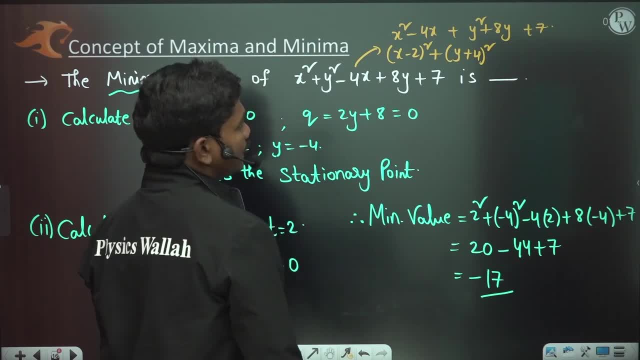 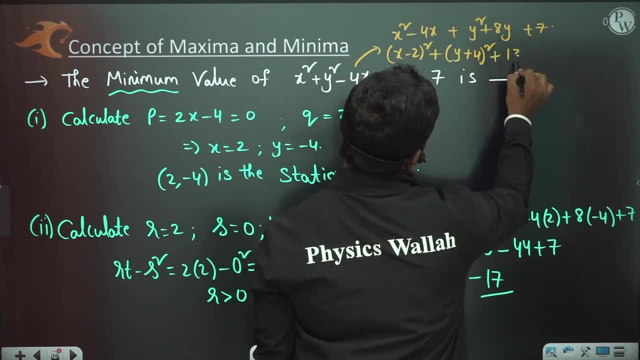 this is plus 4 and plus 16 it is 20, so 20 plus uh. out of this 20, you have 7 here, so you need plus 13 here, correct? oh, no, sorry, let me check if you have. you have total 20 summation here, but 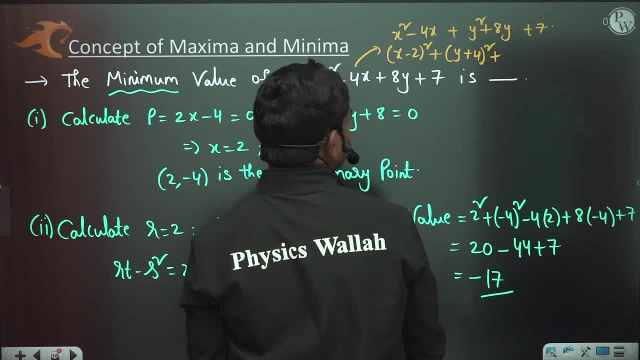 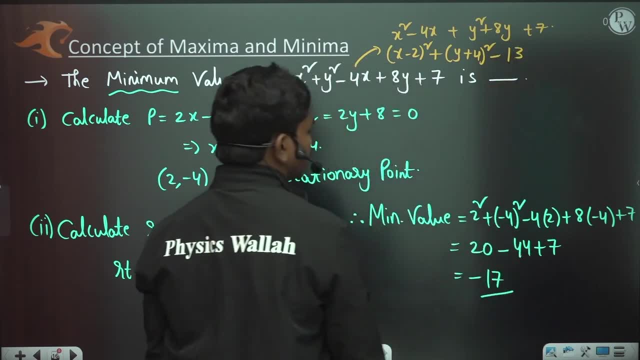 you need to have only 7, so it is 20. you have only 7, so minus 13. let us say minus 13. yes, so if you add minus 13, then it is fine. yes, then did we make any calculation mistake here? 2 comma minus. 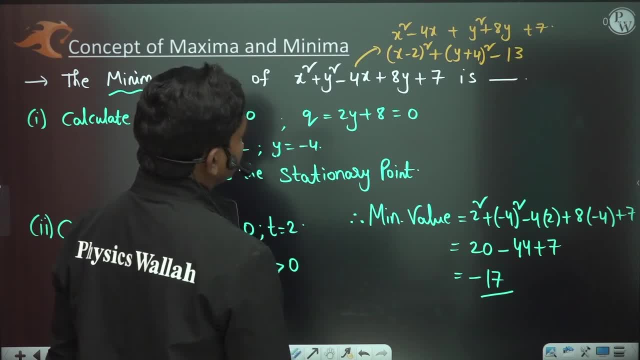 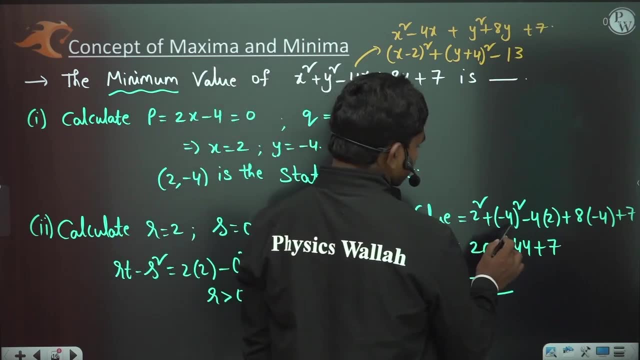 4 is fine. so if you put two comma minus four, 2 square plus minus 4, square minus 4 times of two plus 8 times of two, Works minus 4 plus 7. so 4 plus 16, 4 plus 16, 20 minus 8 minus 32, this is 40 right? yes, this is not 44, this. 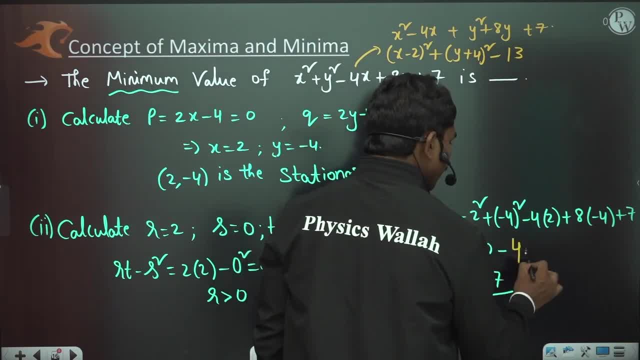 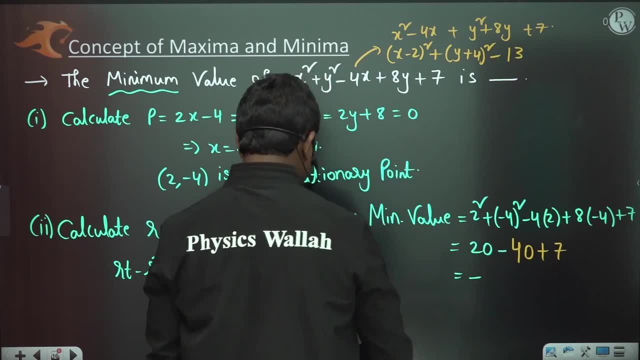 is 40, 40 plus 7. okay. so if you see minus 20 plus 7, it is minus 13, actually, okay. so minus 20 plus 7 is minus 13. there is some small calculation that we are wrong, so okay, anyhow. so if you see. 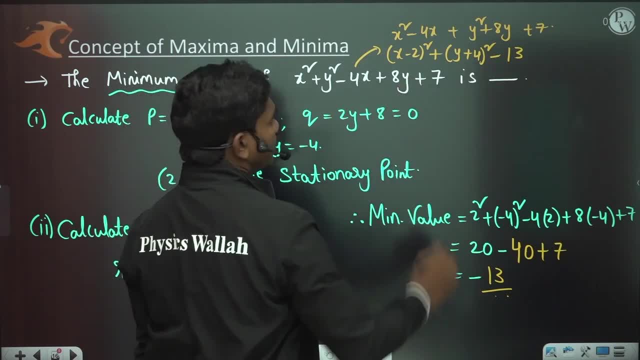 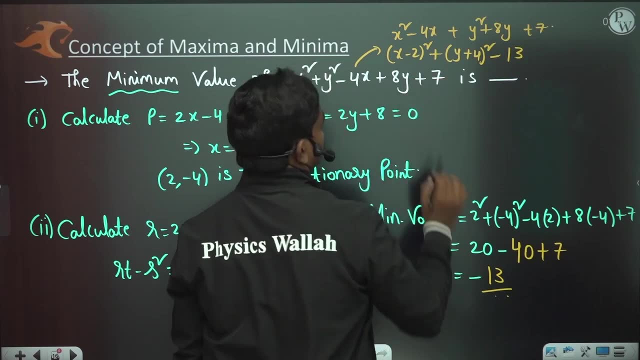 this is the function, so this function is same as this function. now, if this function has to be minimum, look, these two values are having positive sign here. this is positive sign and this is also positive sign. so if you keep anything in place of x, comma, y, definitely this squares will make. 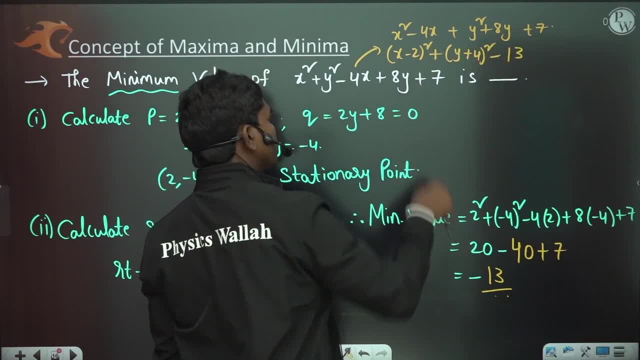 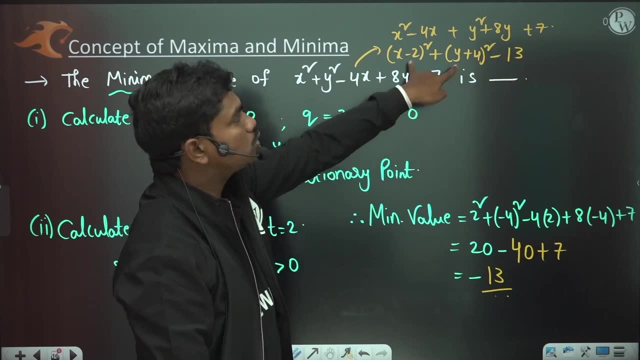 them positive values. so from minus 13 you will actually subtract some positive value. so actually, if you see, if this function has to be minimum, this 13 minus 13 is constant. so these two you know terms has to be minimum and since those are square terms, definitely the minimum value of them is actually 0, because both are positive. 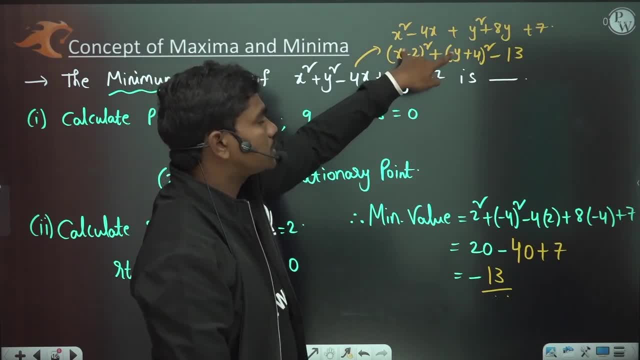 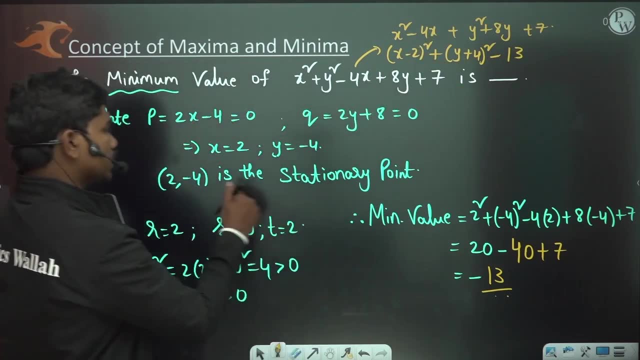 signs. so, if you see, the minimum value of these two terms are nothing but zeros. so first term becomes 0 when x equal to 2. second term becomes 0 when y equal to minus 4. that's the same stationary point you got by differentiation, actually, and this is just by intuition, if you see so, if you. 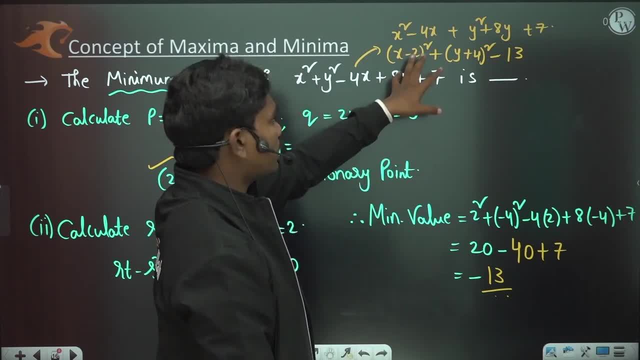 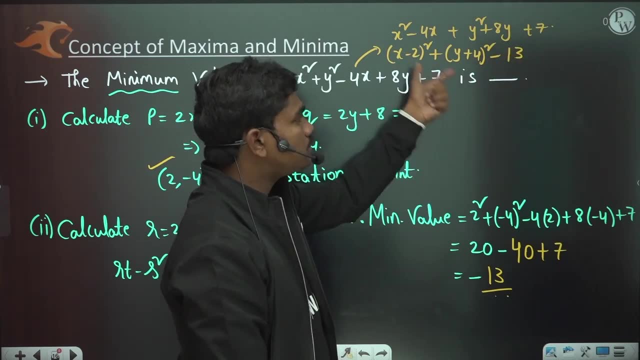 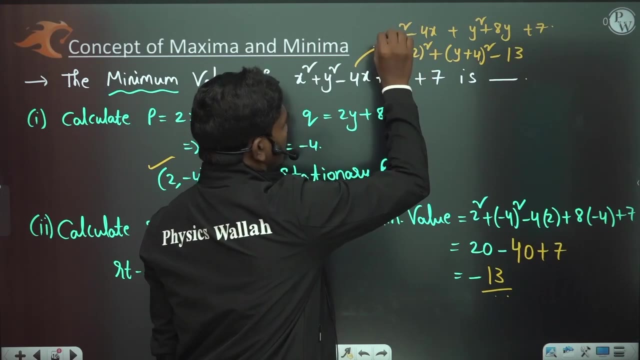 can convert this x square minus 4x as some square of x minus h and y plus k terms, then you know these two brackets where these two brackets becomes 0 and our job is to identify those points where these two actually become 0. so once you identify that, then it's very simple. 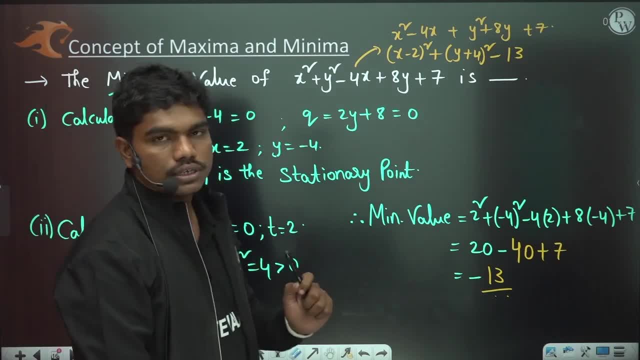 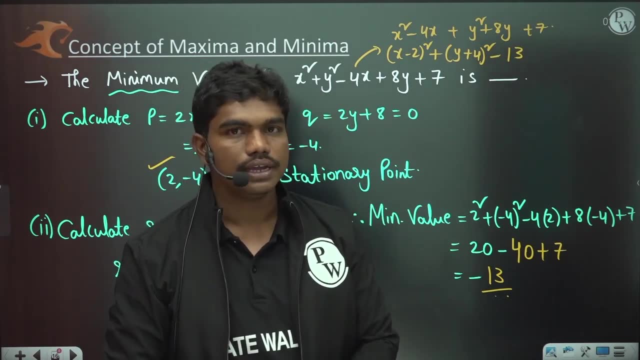 and of course, from the basics of differentiation. and all we again got the same result. so this is how we calculate maxima and minima of, you know, these two variable functions. actually, if it goes for three variables it's much more complicated, but at gate examination level, 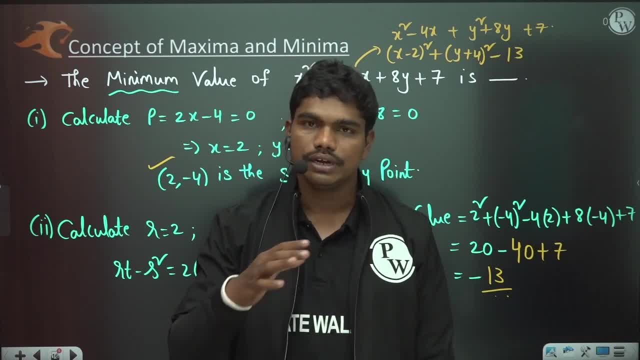 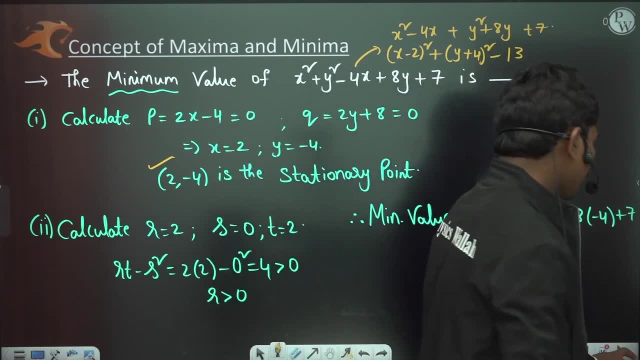 we have only functions in single and two variables, so that's why we calculate maxima and minima. we are restricting at this point, okay. so this is how we calculate the concepts of maxima and minima. now, if you see, okay, fine. so now, if you see, there is one very important concept. 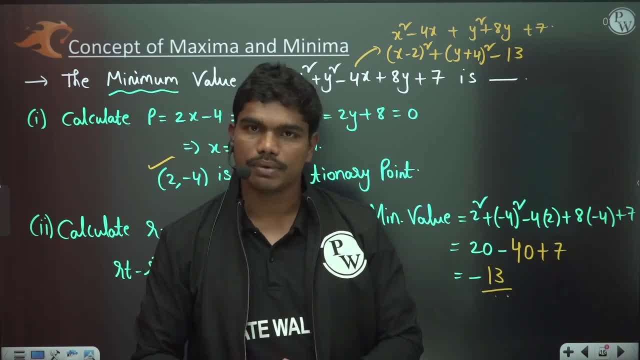 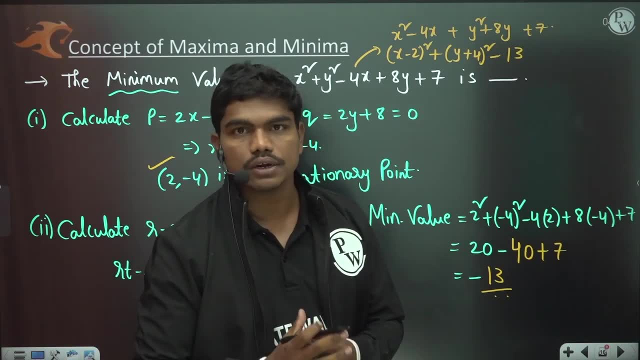 which is called the concept of constraint maxima and minima also. okay. so we have seen these concepts of maxima and minima in case of two variables. now let us look into one very important concept, which is called concept of constraint maxima and minima. okay, so again. 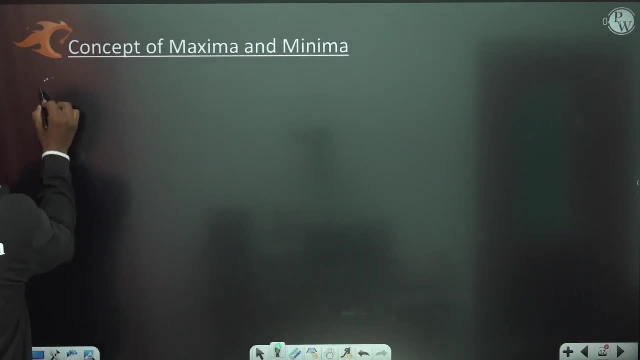 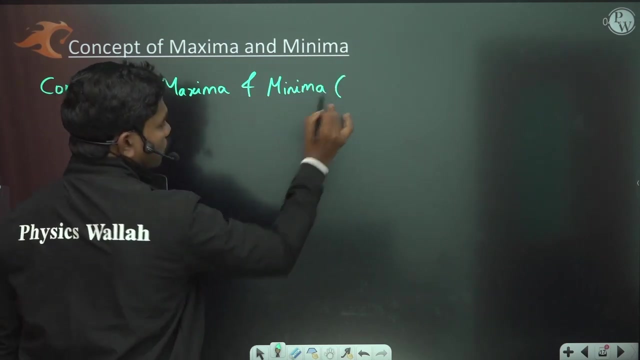 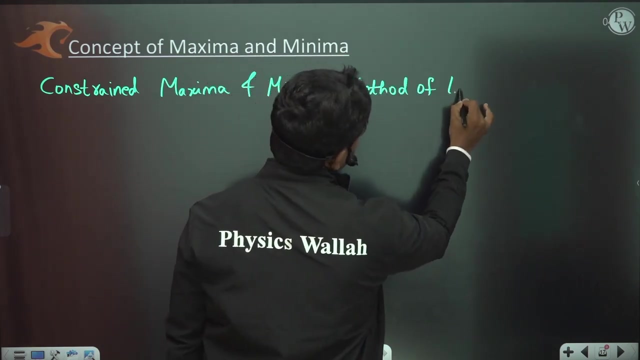 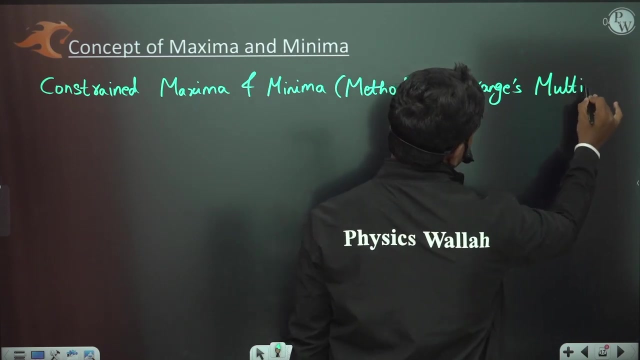 in maxima and minima. we, of course, will deal one special concept which is called constrained, constrained maxima, constrained maxima and minima, and this is also known with some other name, which is also called as method of method of Lagrange's multipliers, Lagrange's multipliers. okay, so this is again. 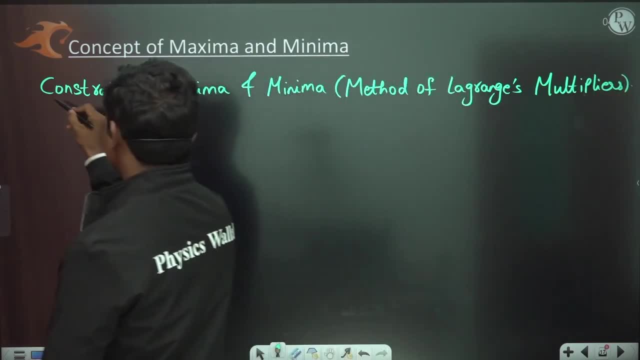 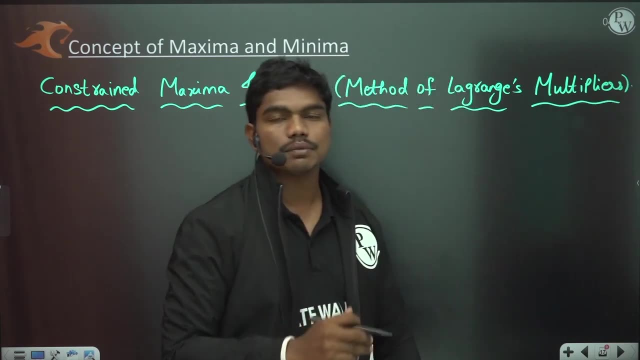 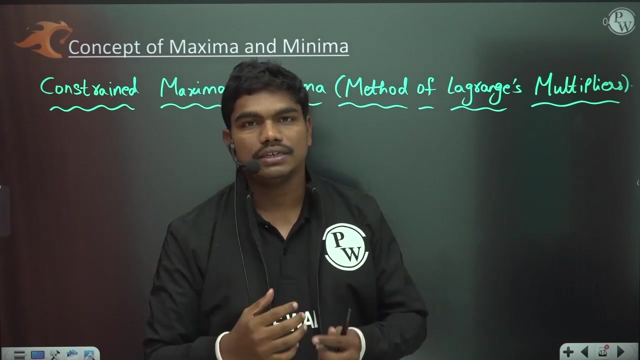 one very important concept in case of maxima and minima. why it's very important, we'll see. look here now. let us suppose if i want to design a box of certain volume, for example, now if i want to design this box of certain volume, i'll definitely have a constraint. maybe i can have some space constraint. 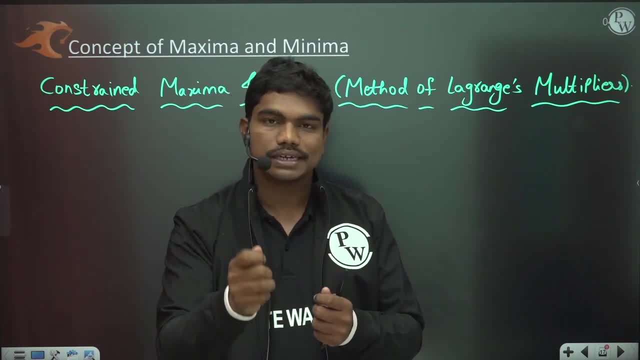 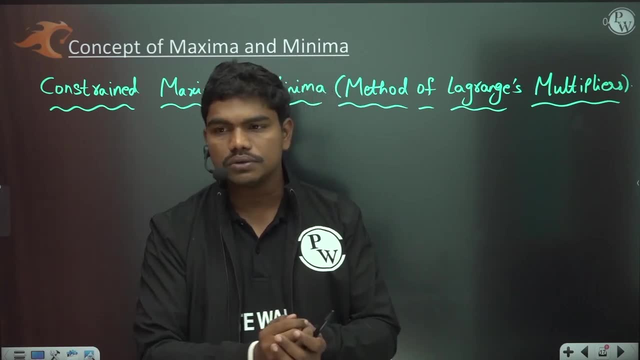 okay, or i can have some material constraint like this: much material should only be used for manufacturing this box, which means if material is the constraint, that means automatically surface area is the constraint. so many times it's not possible that you you design the things of your own interest, but whether they 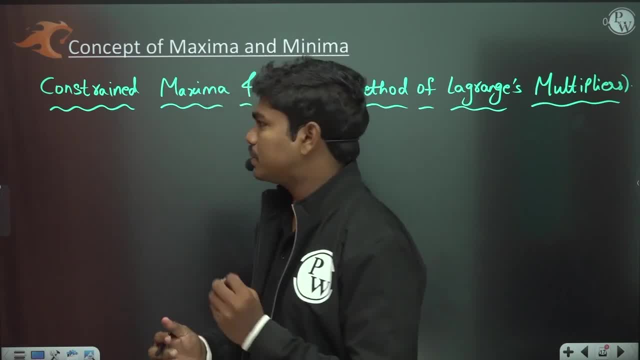 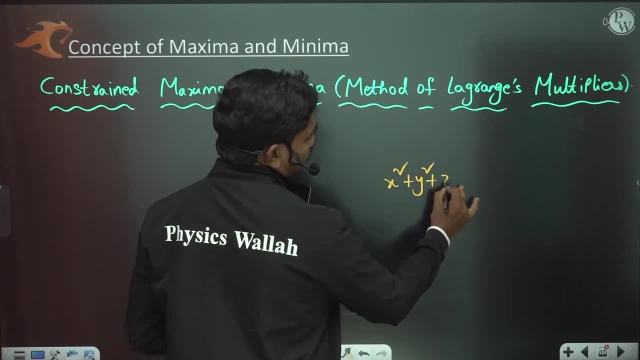 are bounded by certain conditions. actually, for example, i. i'll give you one simple example. let us suppose if i ask you what is the minimum value of x square plus y square plus z square, for example, without mentioning any condition, if i ask you this question: minimum value of this x square plus y. 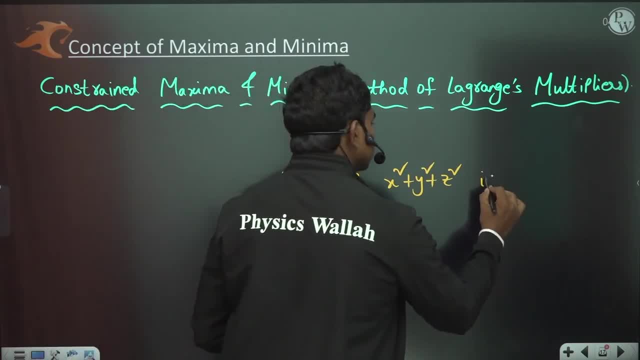 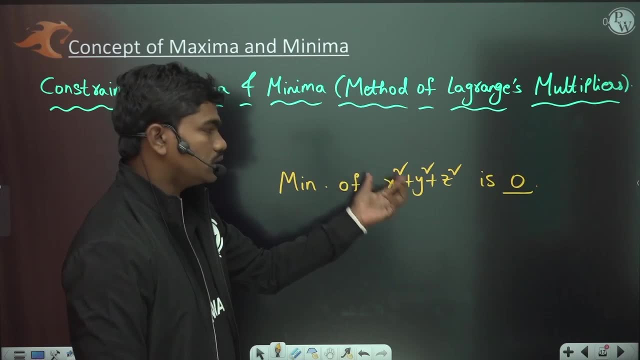 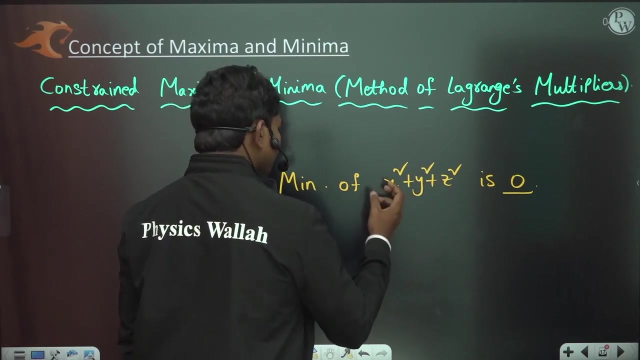 square plus z square, without giving a thought, you will tell directly. the answer is zero. why? because you know that individually all these terms are going to be equal to x square plus y square plus y. you know the minimum value of every time is zero, so some of the zeroes is zero, so i can give only 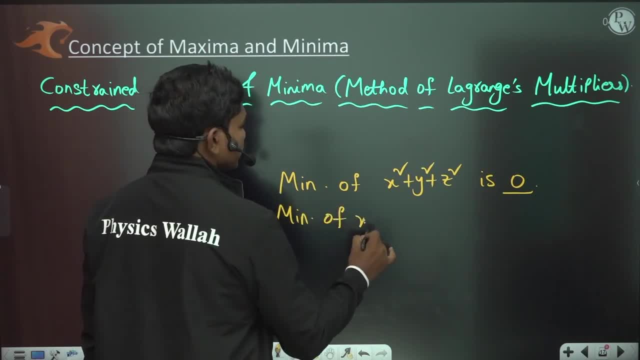 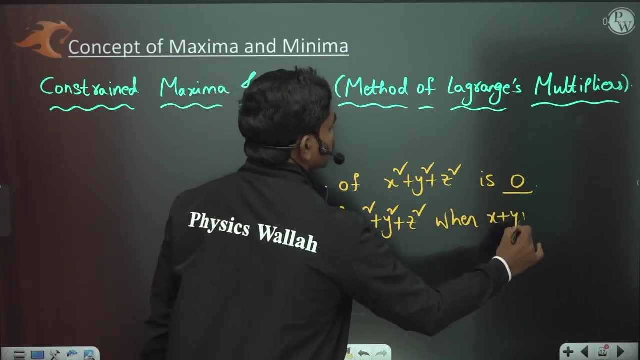 this condition that the minimum of x square plus y square plus z square when it equals to one, when it equals to one, and also useful to leave out the繼續 of the more more repeated explanations, the more and more so, the more and more often it is beautiful to discuss and focus on only the problem. here follow. 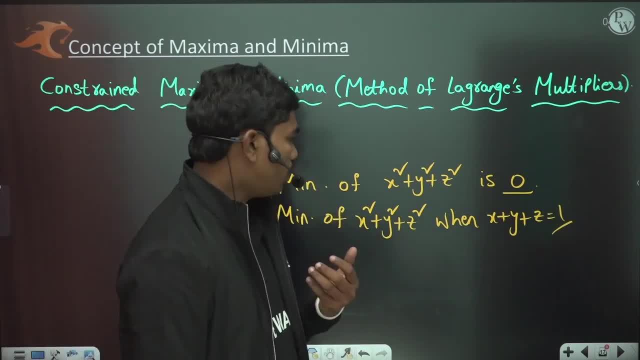 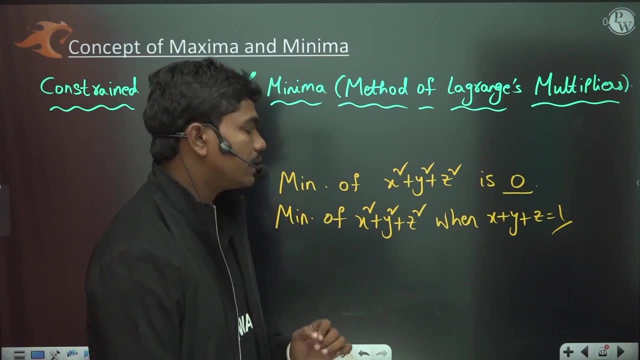 give you this condition. okay, now, along with asking you the minimum value of x square plus y square plus z square, if i ask you what is the minimum value when these conditions are, you know, satisfying, then you cannot keep zero, zero, zero here, because if you see, when you keep all zeros, this equation, 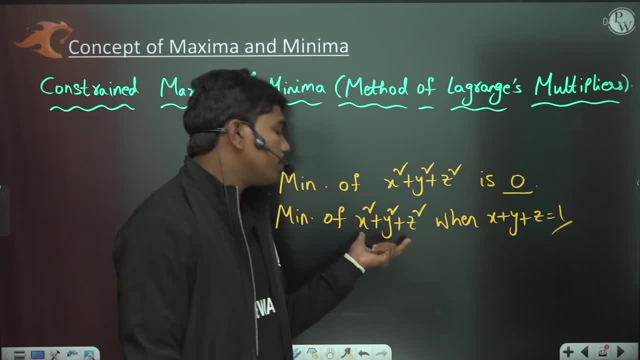 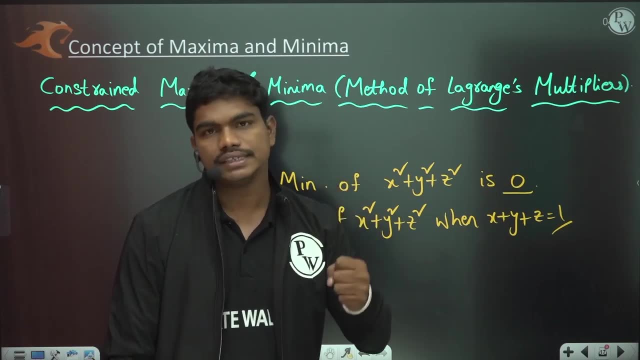 doesn't get satisfied. okay, so such now, definitely, you see the minimum value of this. uh, you know, expression is not zero. why? because we have set a constraint, okay. so constraint means some restriction on the variable. okay. so, whenever there is certain restriction on the variables, you generally cannot. 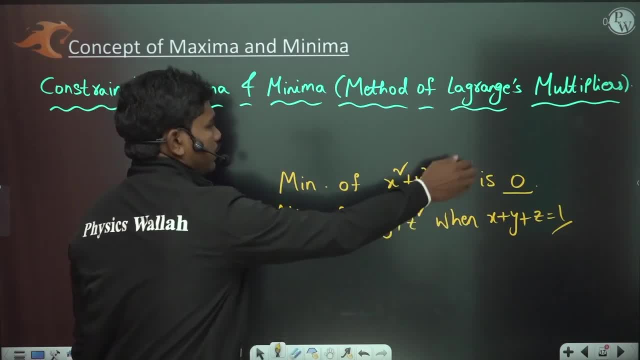 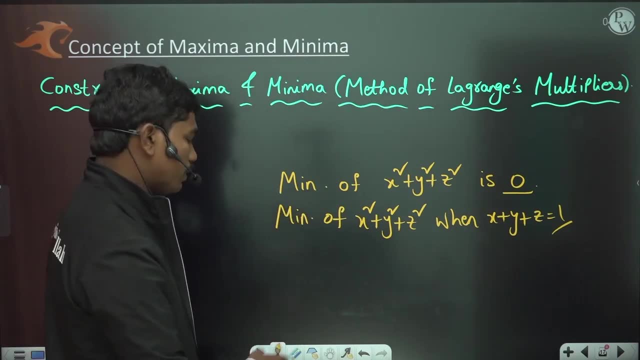 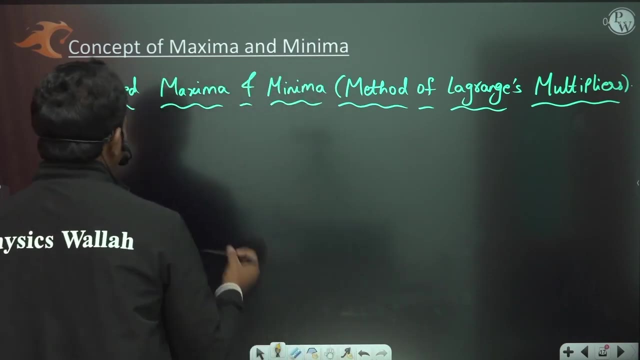 say that this is basically, uh, the same as the normal case. okay, so we'll talk about this. uh, you know, kind of things in this constraint, maxima and minima. so let us quickly go through the things. okay, so let us quickly go through the things now. let us see here, let f of x, y, z be. 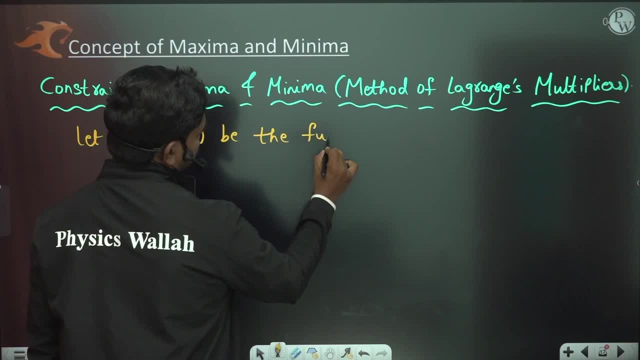 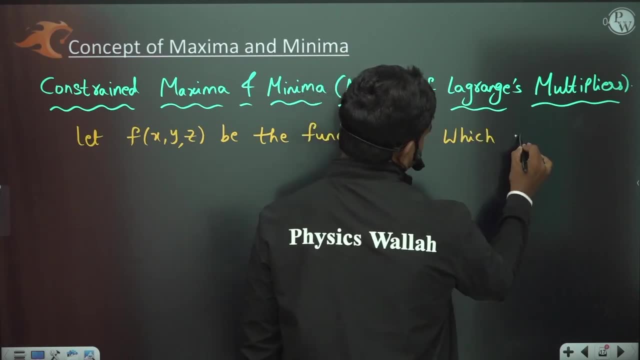 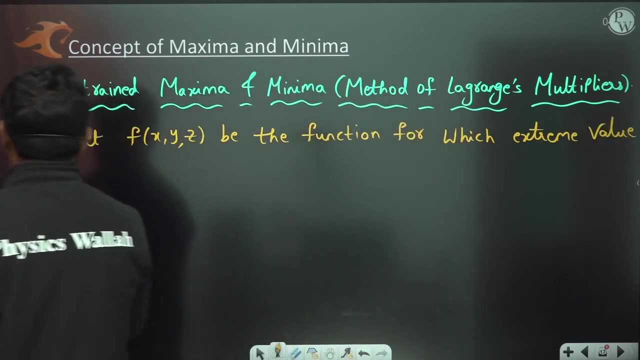 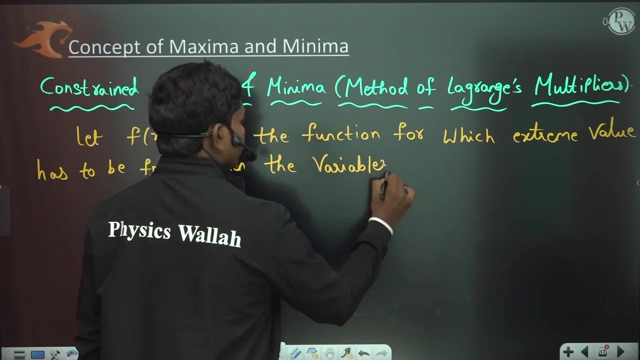 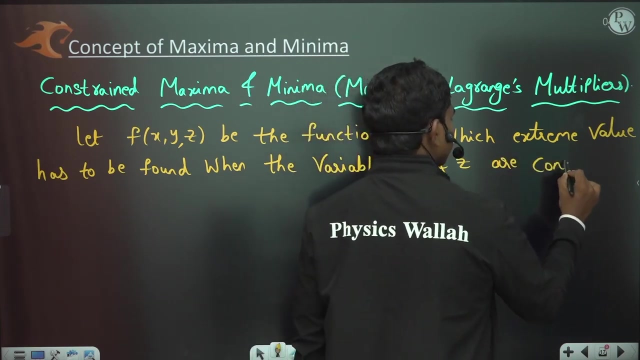 a, the function for which, for which extreme value has to be found, for which extreme value means basically maximum or minimum. extreme value has to be found when the variables, when the variables, when the variables are x, y and z, are constrained by, are constrained by, are constrained by some. 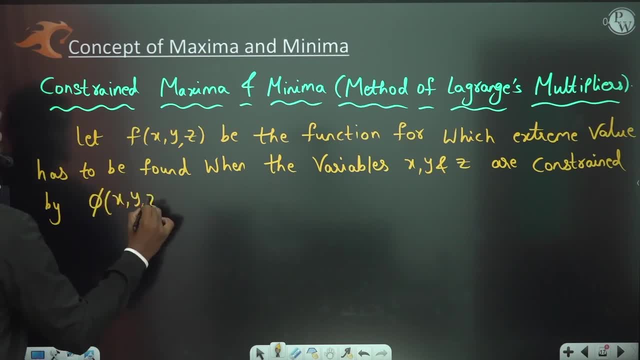 equation. let us say some phi of x, y, z is equal to constant. phi of x, y, z is equal to constant. okay, so basically, if you see, this is the function for which you need to find the maximum or minimum value and this phi of x, y, z is equal to constant is the governing equation which is actually bounding the variables. 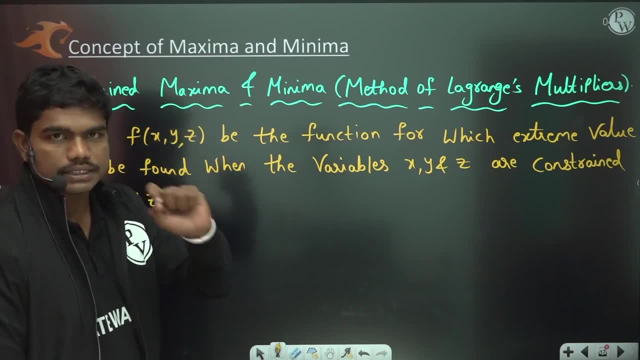 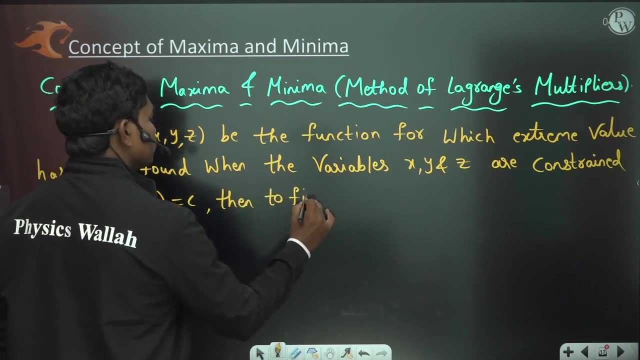 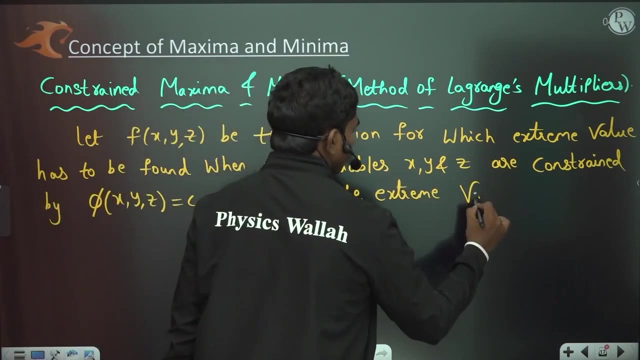 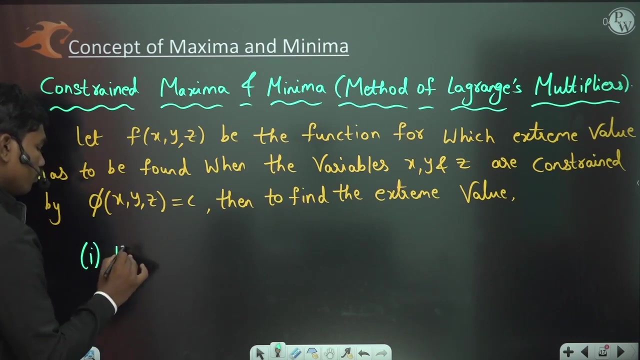 variables, Like in the previous example I have stated: x plus y plus z is equal to one such kind of things. Then, to find the extreme value, to find the extreme value, then to find the extreme value, what we'll do is first step, first step, form a function, form a. 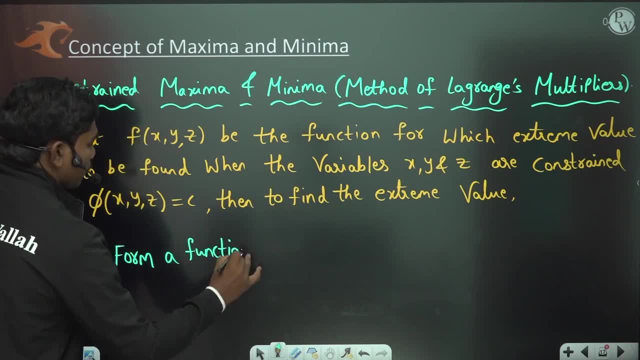 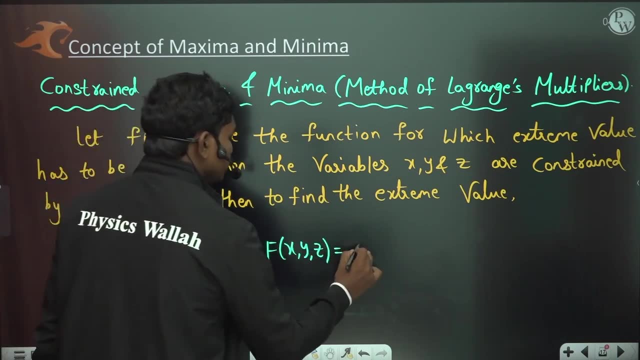 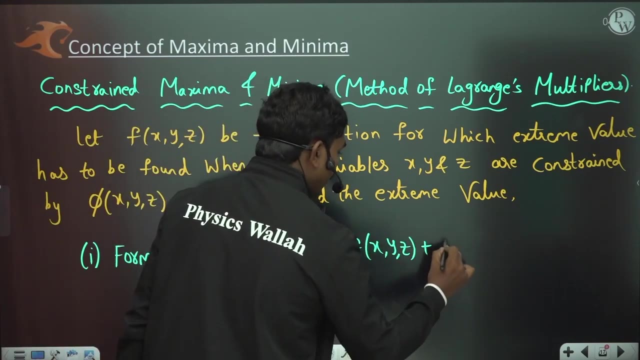 function form a function, say capital F of x y z, for example. So capital F of x y z is equal to small f of x y z. basically the function for which you need to find the maxima or minima plus lambda times of phi of x y z, minus constant phi of x y z. 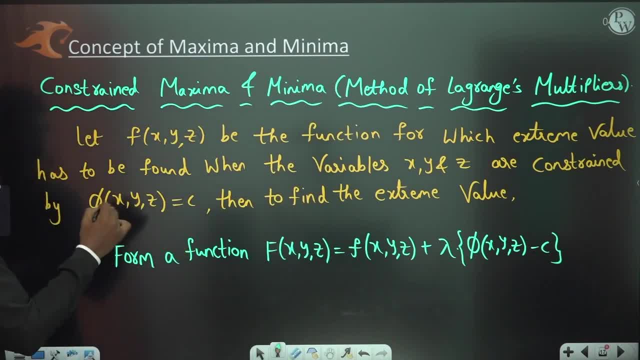 minus this constant, Whatever is given. basically you can write this equation as: phi of x, y, z minus constant is equal to zero. So some function of of x comma y comma z minus c. okay now second part: equate: equate dou capital f by dou x is equal to: 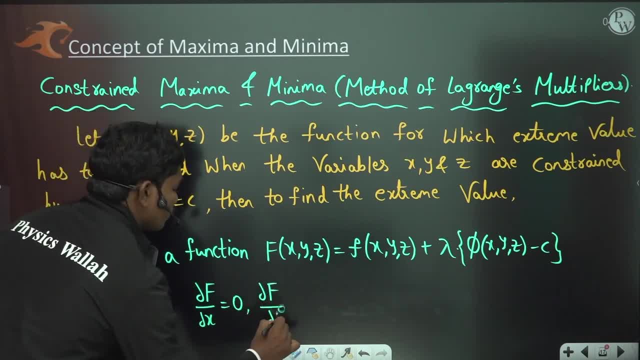 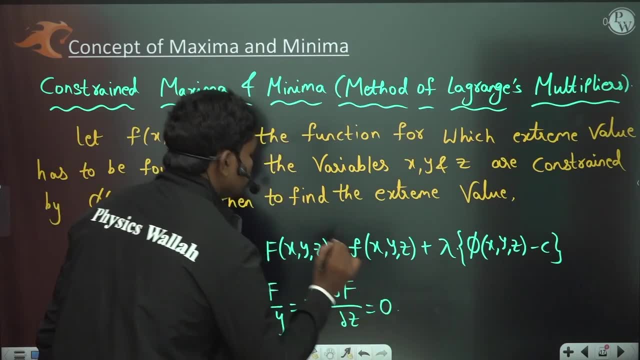 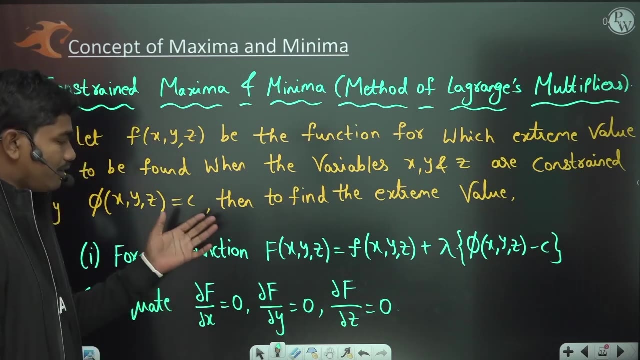 zero comma dou capital f, comma dou y is equal to zero and dou capital f by dou z, this is also equal to zero. so basically, you know, for calculating the extreme values you need to differentiate the function and equate it to zero. so whenever you have a capital f of x, y, z, then equate the partial. 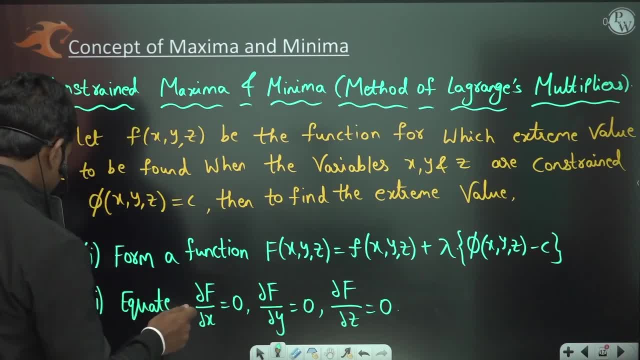 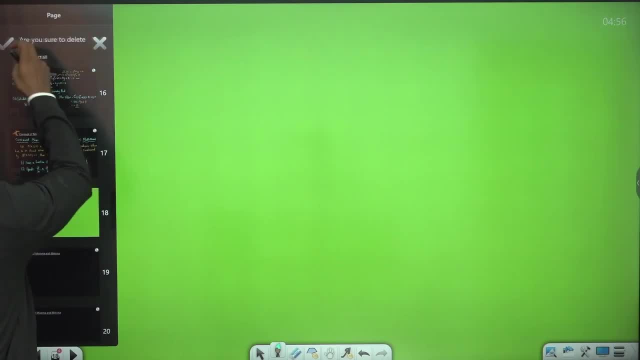 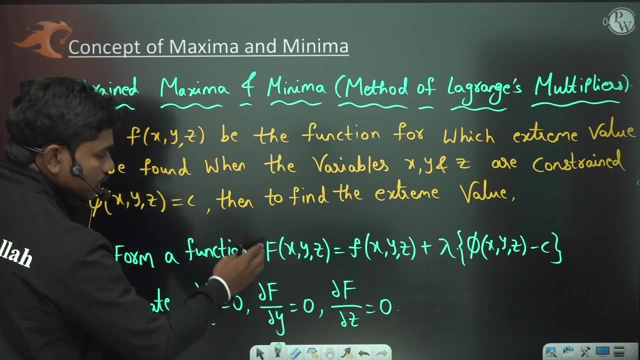 derivatives individually to zero. so once you eliminate, i mean once you equate them to zero, then the next step- oh, i'm sorry, just a minute. okay, so once you found this, the the- once you equate these partial derivatives, dou f by dou x, dou f by dou y, dou f by dou z- to zero, then the. 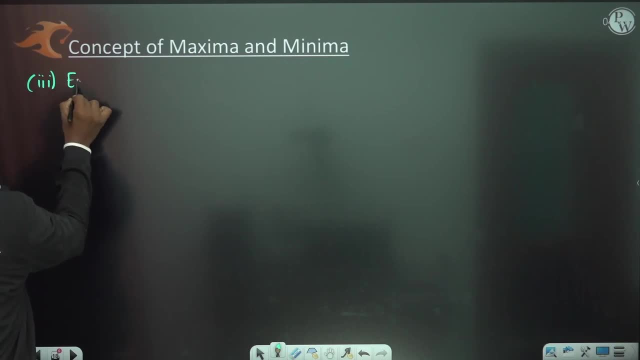 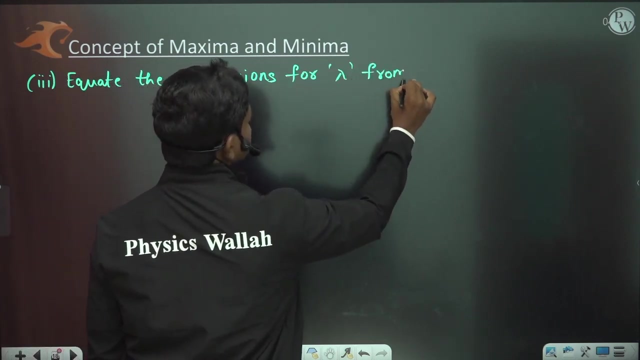 third step that you need to do is equate the equations or equate the expressions for lambda from above set of equations. you have three equations now: dou f by dou x, dou f, capital f by dou y, dou capital f by dou z. so from that equations equate the expressions for: 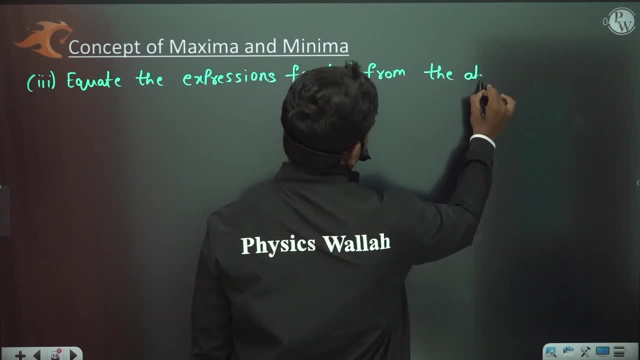 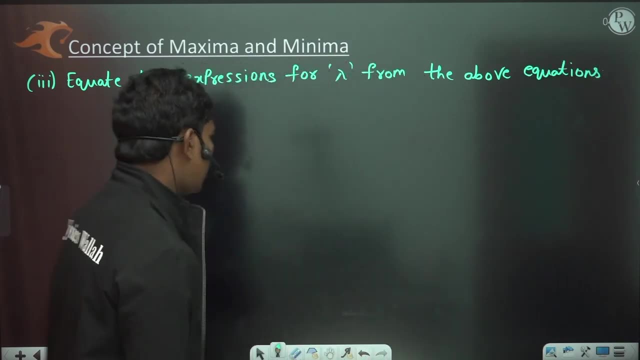 lambda, from the above equations, from the above equations. so once you have done that, you will get the relation between variables and get the relation between variables and get the relation between the variables, get the relation between the variables. i'll, of course, explain you the step by step procedure with an example. you will be more comfortable, okay. so what i'm? 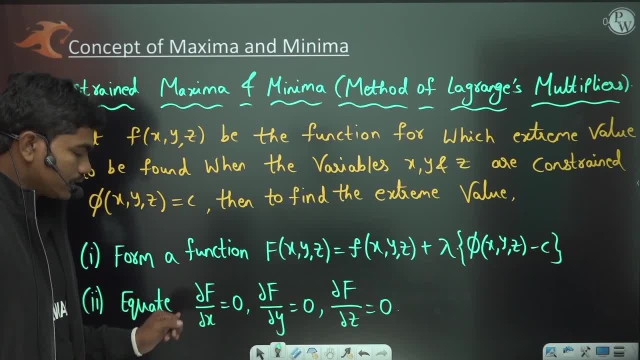 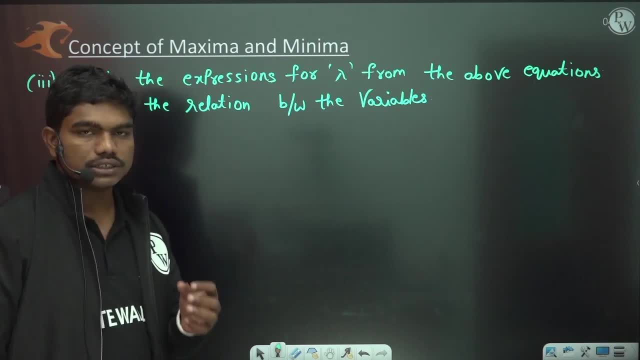 telling you. first of all, you form three equations that dou capital f by dou x is equal to zero. dou capital f by dou y is equal to zero. dou capital f by dou z is equal to zero. now, from that equations you equate the expressions for lambda in set of two equations. okay, so 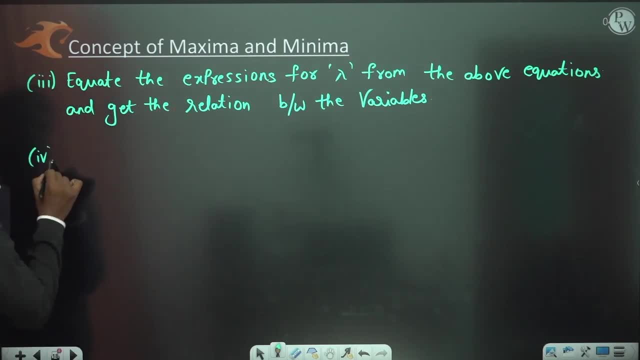 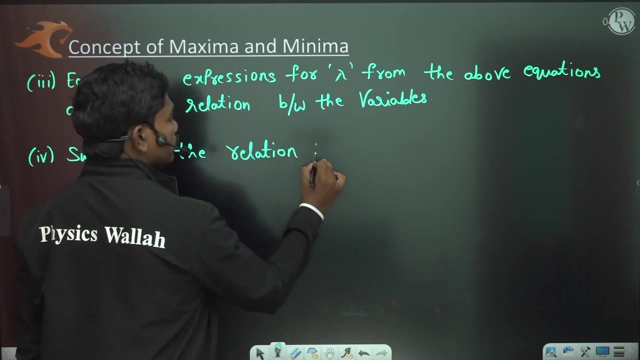 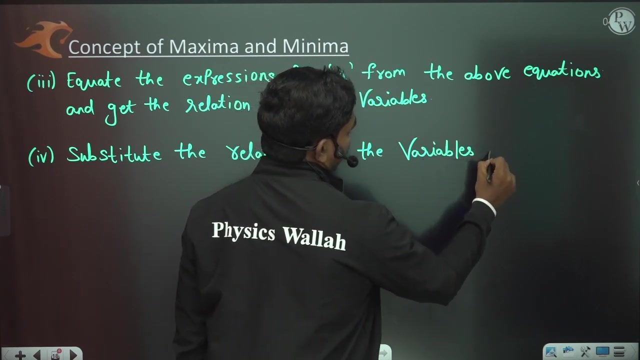 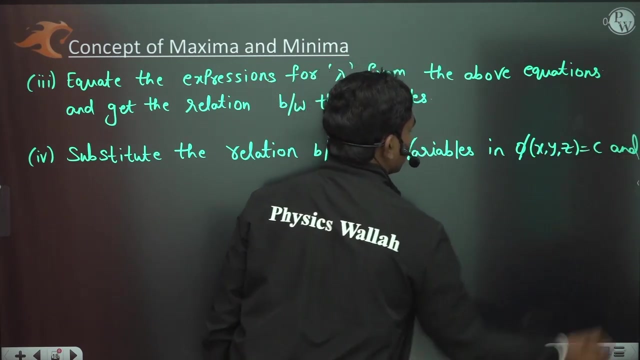 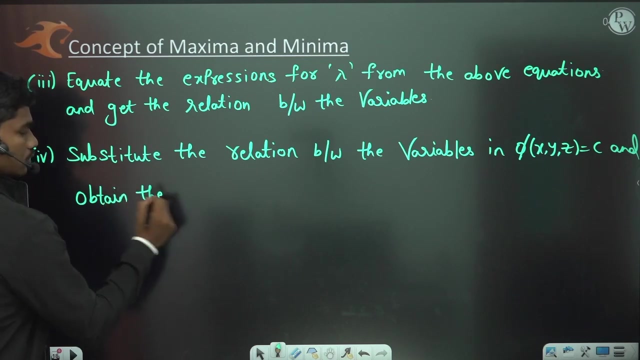 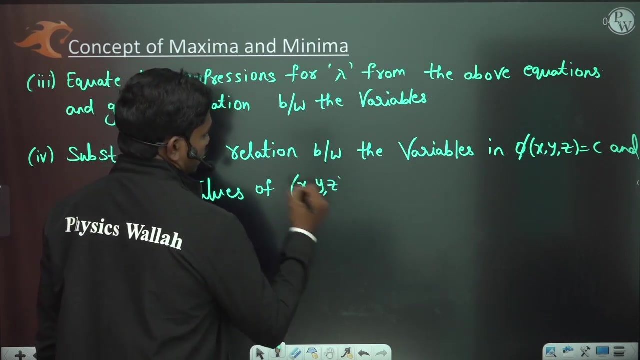 by doing that, you will get the relation between the variables for substitute, substitute, the value of substitute, the relation between substitute, the relation between the variables, the variables in in phi of xyz is equal to constant- and and obtain the values of xyz, obtain the values of xyz. obtain the values of xyz at xyz and obtain the values of xyz. that's it okay. so. 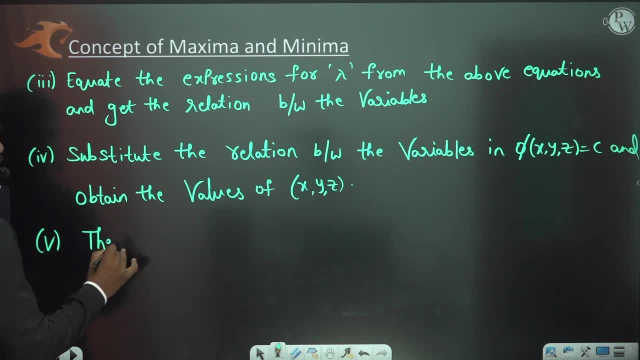 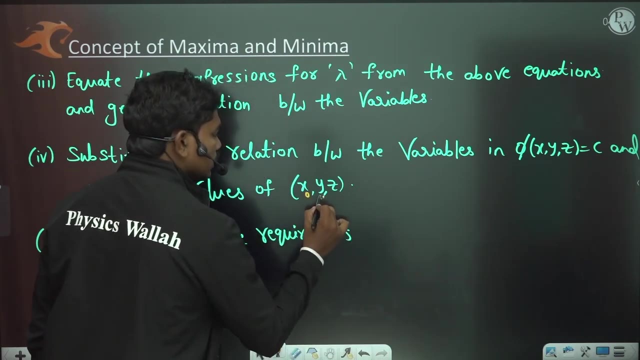 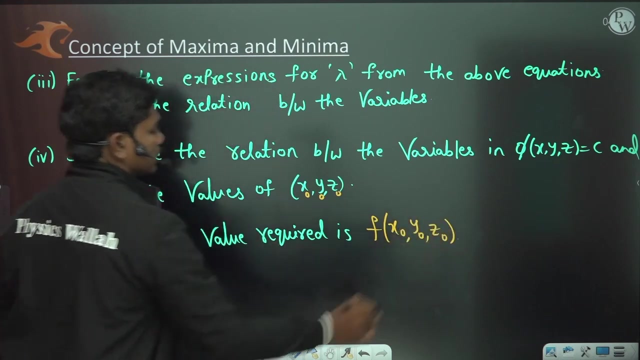 once you substitute that, then fifth is the extreme value. of the extreme value required, you can write: the extreme value required is okay. in order to identify clearly, let us make this: x naught, y naught, z naught. then is small f of x naught, y naught, z naught. okay. so this is how we actually find the extreme. 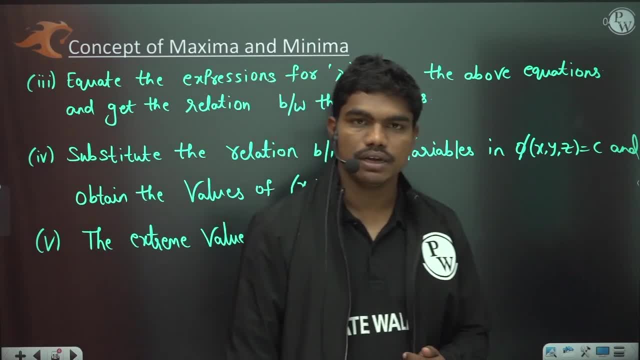 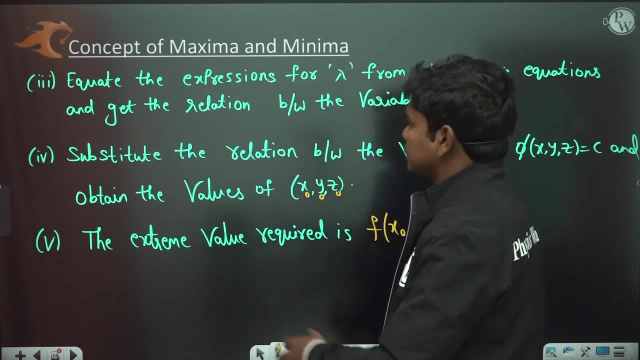 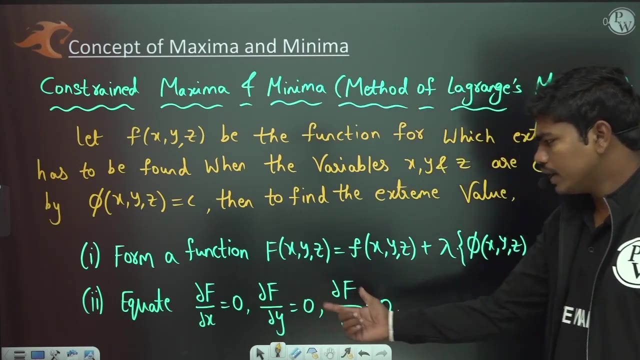 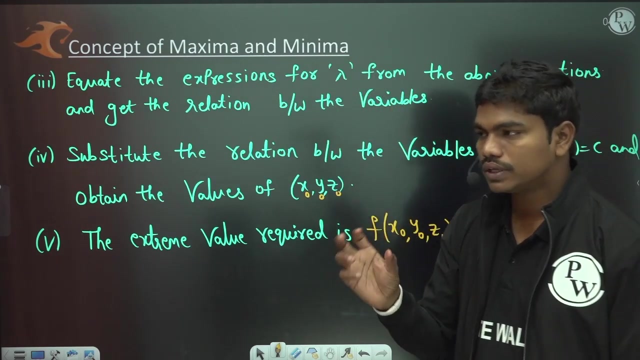 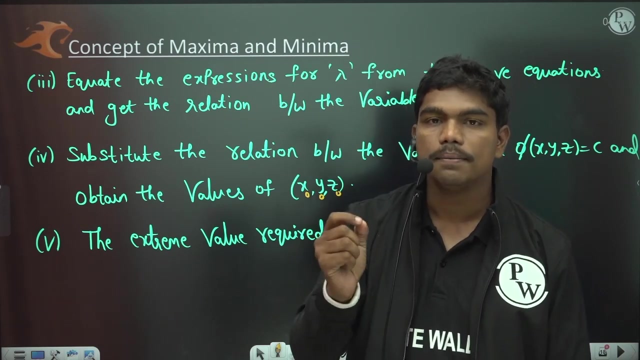 values. and here, if you see, the procedure remains the same for maxima or minima actually, and these kind of functions generally, they have only one extremum in general. okay, if i just between f of x1 and f2 here, if we find that f of 0, p, fs 0, p, fug of q, verse y, 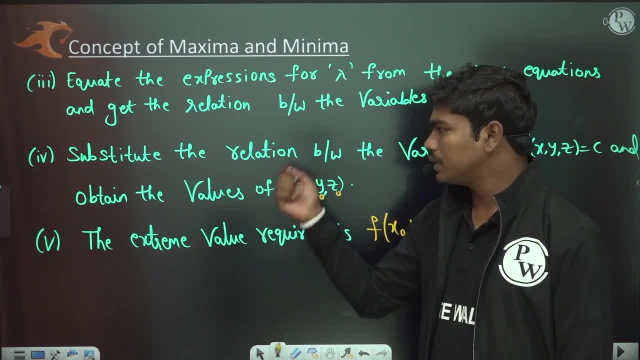 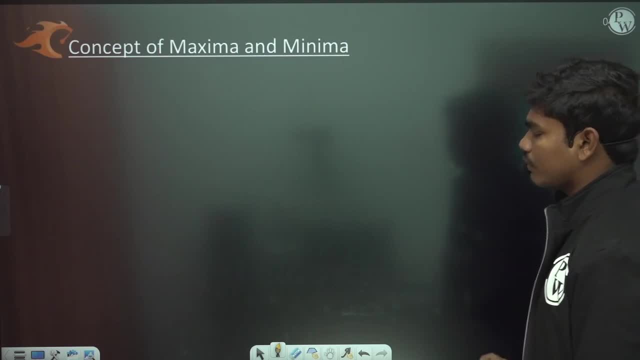 and 1 and 1 exactly. y naught, z naught, actually. and the extreme value that they ask in the question, maximum or minimum value, is basically f of x naught, y naught and z naught. okay, now let us see this with the help of an example. you can see example: the minimum value of the minimum value. 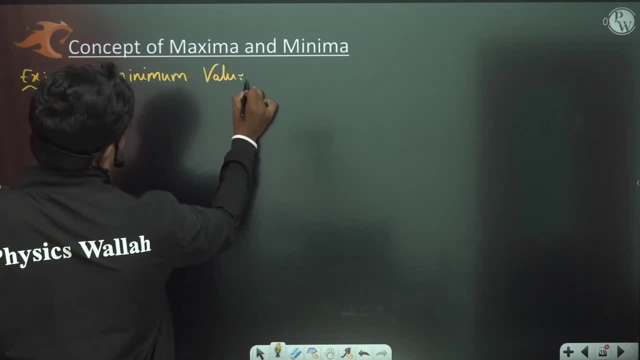 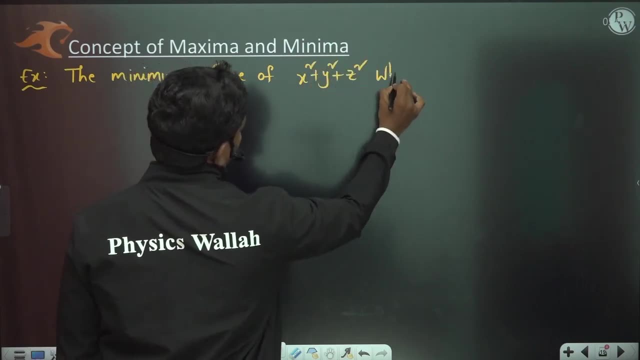 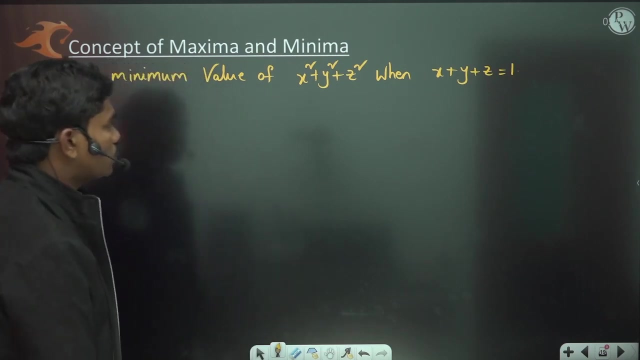 of the minimum value of x square plus y square plus z square when- let me take this example just to make you understand this- plus x plus y plus z is equal to 1, for example. okay, so let us suppose you have taken this example. minimum value of this x square plus y square plus z square: when x plus. 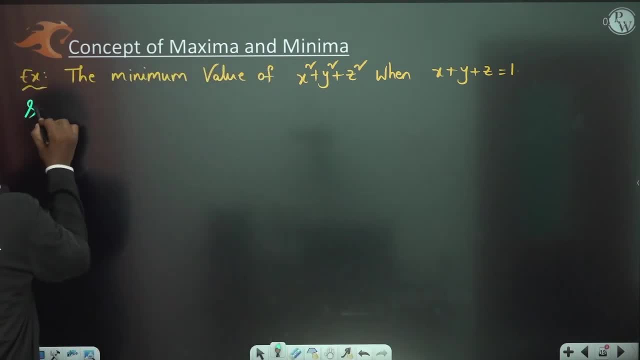 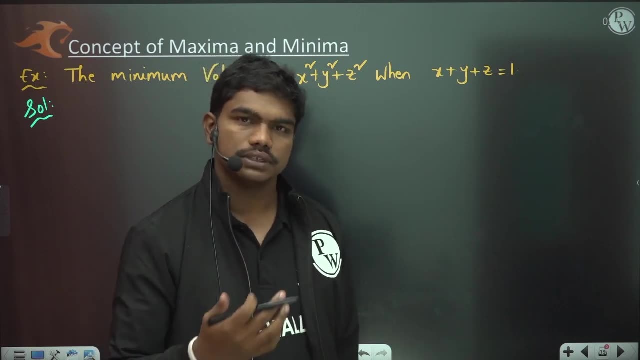 y plus z is equal to 1. so first step if you want to carry out this, look, as i told you generally in in question you have only one of the extreme values. the other one tends to plus infinity or minus infinity, depending upon maximum or minimum, for example. if you check this question, you know you will have 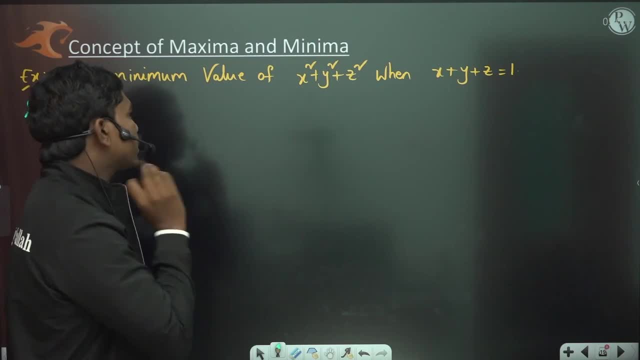 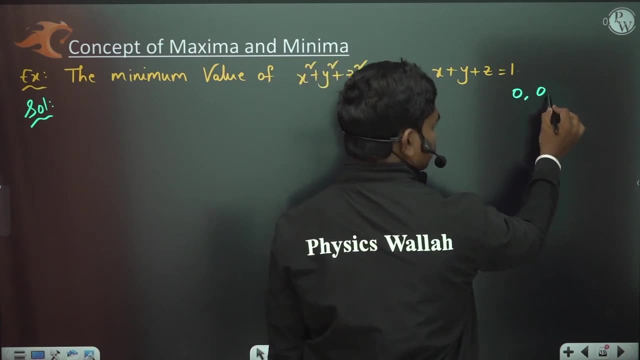 some minimum value which will calculate, uh, using some procedure. but if you focus a bit on maximum value, the maximum value tends to infinity because, for example, i can set this numbers as 001 and i can set this numbers as 2022 minus 2021, 0, or you can take any two very large numbers such that 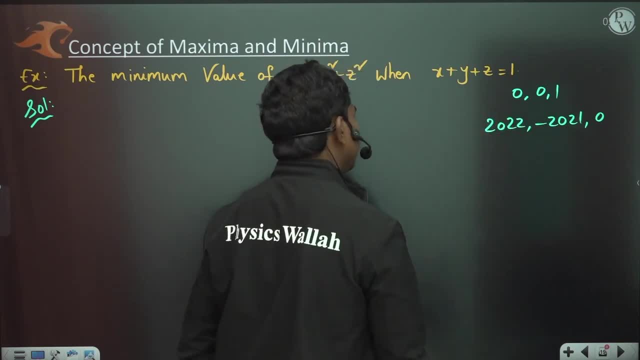 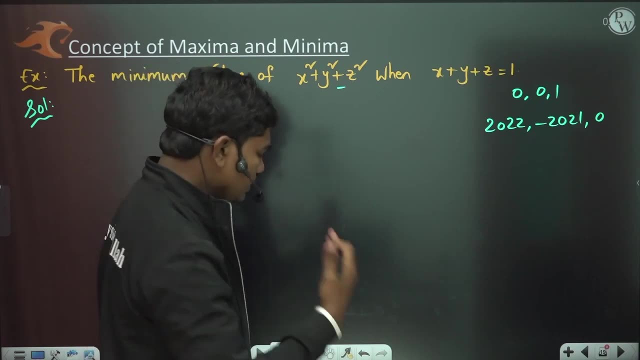 they differ in sign and they also define magnitude by one unit. okay, so if you set examples like this, then definitely this term x square plus y square plus z square will keep on, you know, increasing and it touches infinity. okay, so now, if you see, let us focus on the calculation of minimum value. so first, 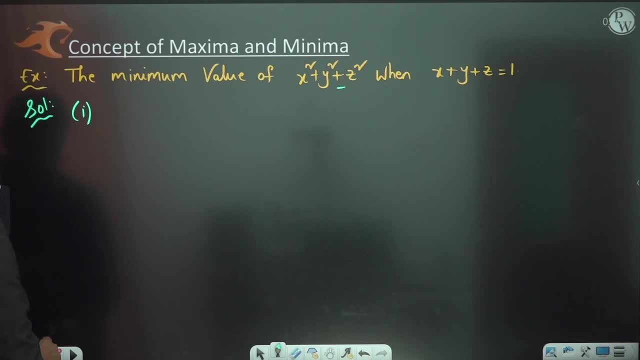 step that we are doing is, as i told you. if you observe carefully, the first step i told you is form a function like this. okay, so form a function. so capital f of xyz is equal to capital f of xyz is equal to small f of xyz, which is this function for which you need to. 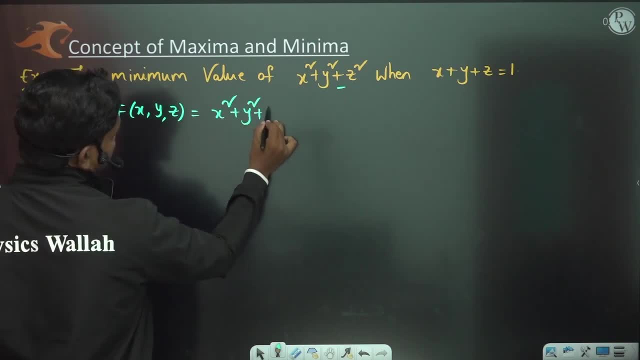 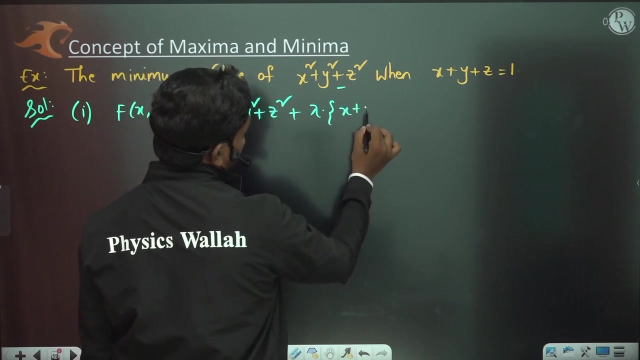 find the minimum value. so x square plus y square plus z square plus lambda times of this lambda is called lagrangian multiplier here. okay, it's a constant value basically. so this lambda is called lagrangian multiplier, so lambda times of this function: x plus y plus z minus 1. so this is: 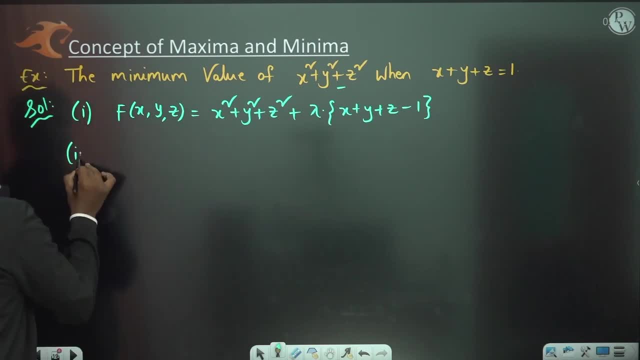 total capital f of xyz. now, second step is equate dou f by dou x. so what is dou f by dou x from this function 2x? then when you are differentiating with respect to x, these two are constants, so 0 plus lambda times of if differentiation. 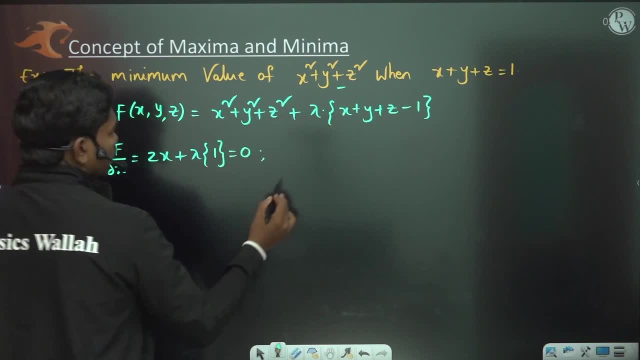 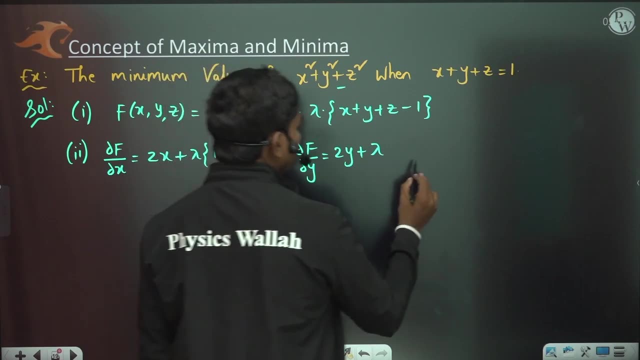 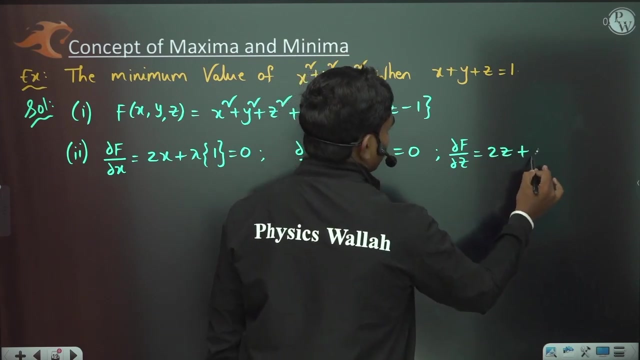 of this is 1, that's it is equal to 0. dou f by dou y, dou f by dou y, is equal to. similarly, 2y plus lambda into 1 is equal to 0. dou f by dou z, which is 2z plus lambda times of 1, again is equal to 0. so we have this values. so from this equation, if you 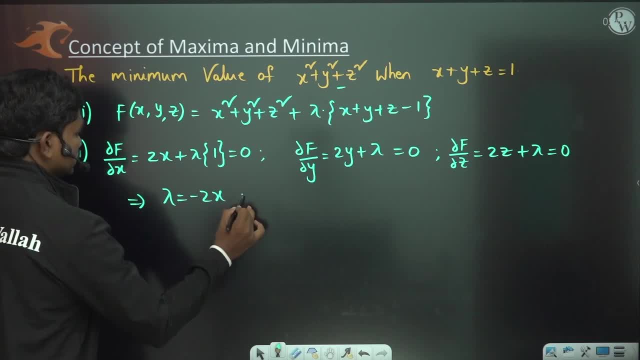 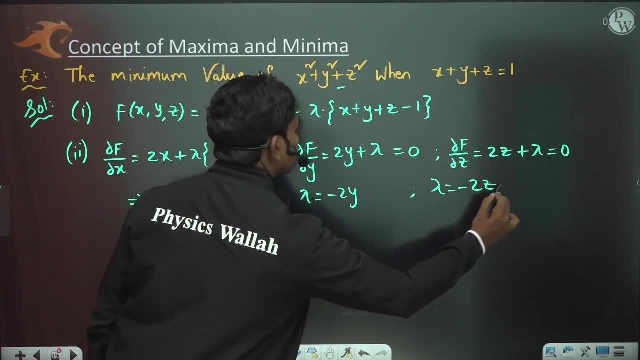 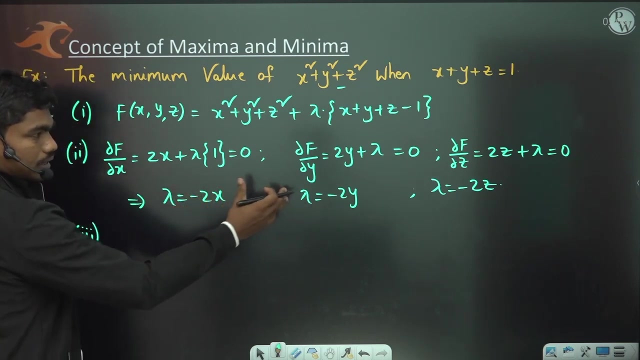 write the value of lambda: lambda is equal to minus 2x, here lambda is equal to minus 2y and here lambda is equal to minus 2z. now third step is basically equate the different expressions for lambda from the above equation. so these are the three equations. so if you equate it to two sets of lambda by dou x, 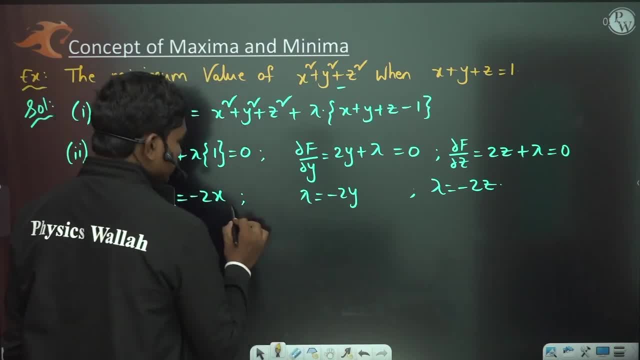 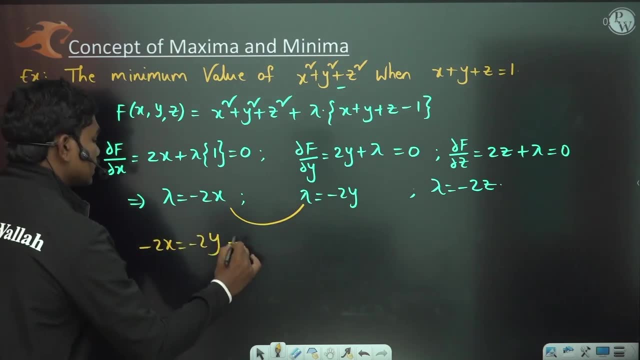 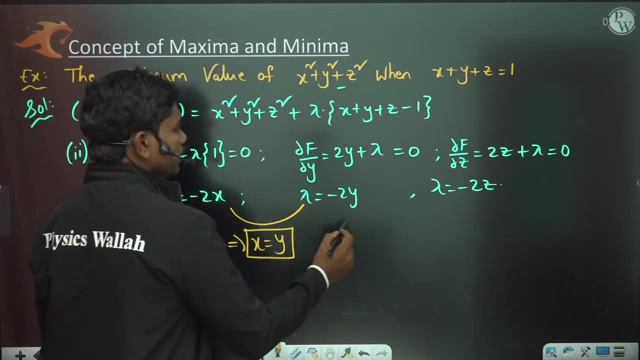 values. for example, if i equate these two. if i equate these two, then what is the relation i will get? minus 2x is equal to minus 2y, so which means x is equal to y. so the relation between x and y, for this function to be minimum, is x should be equal to y. similarly, let us suppose, if i equate- 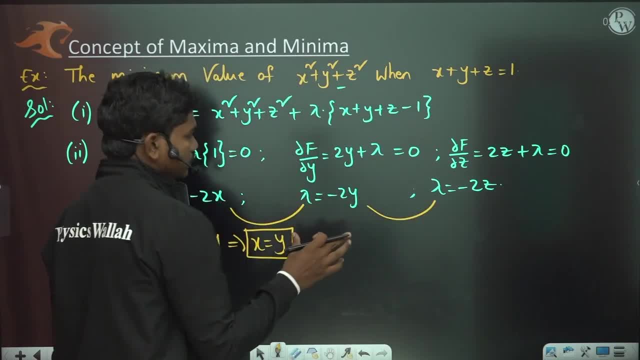 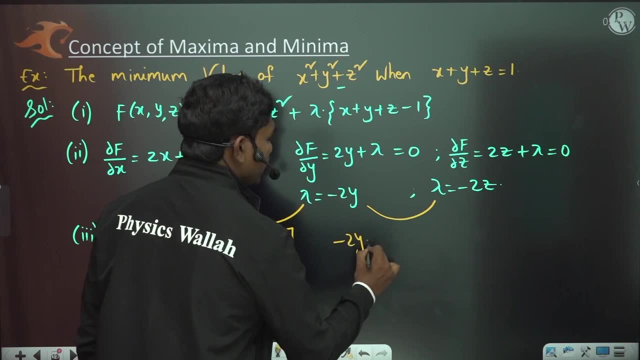 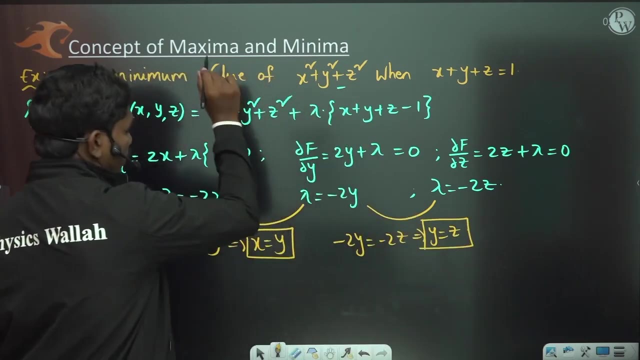 these two, or you can equate first and third, also depending upon uh. here your idea is to eliminate one variable so that you will get relation between two, two variables. okay, so minus 2y is equal to. this implies y is equal to z. so basically, what you can tell for this function to attain, to attain: 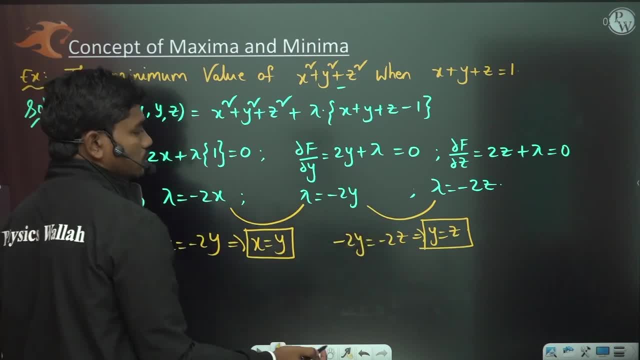 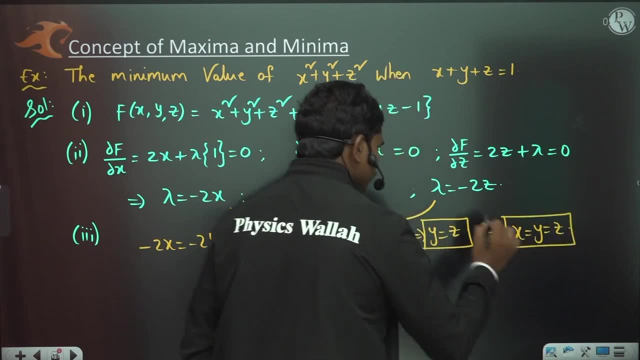 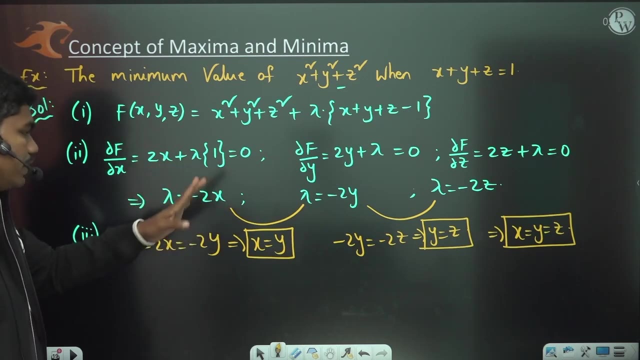 minimum value. all the variables x, y and z values should be same. so this implies x is equal to y is equal to z. so what we have done, basically, is we have equated the expressions for lambdas and we have obtained some relation between this. uh, you know variables. okay, so that's the third point. 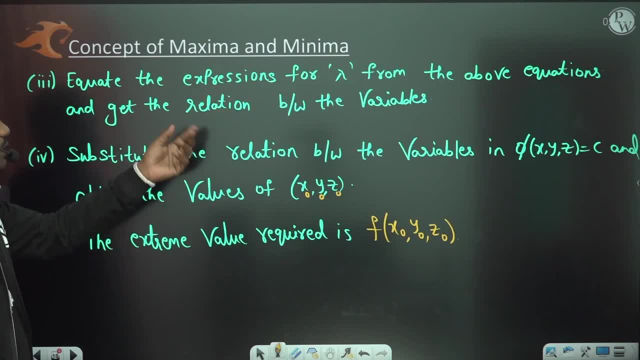 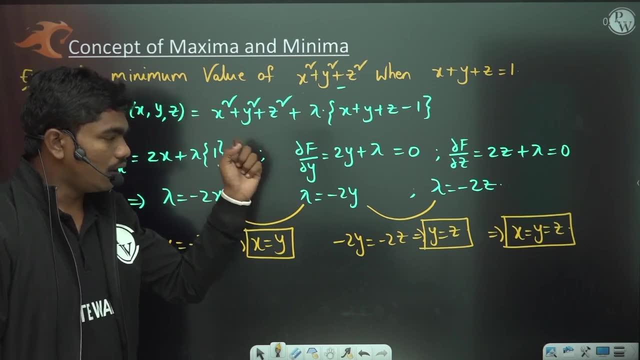 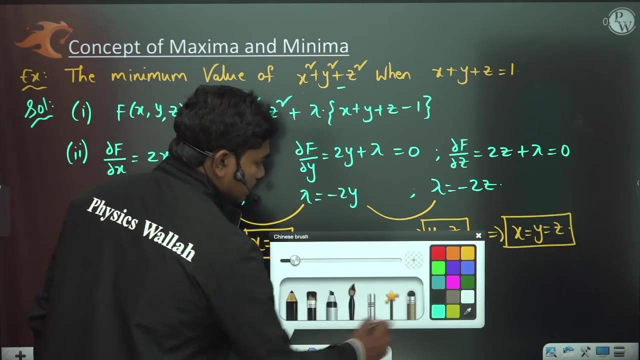 what i have stated here: equate the expressions for lambda from above equations and get relation between the variables. so I have got the relation between variables that for this function to have a minimum value, the value of X, Y and Z should be same actually here. okay, so once the value of X, Y, Z is same now fourth, you know step. 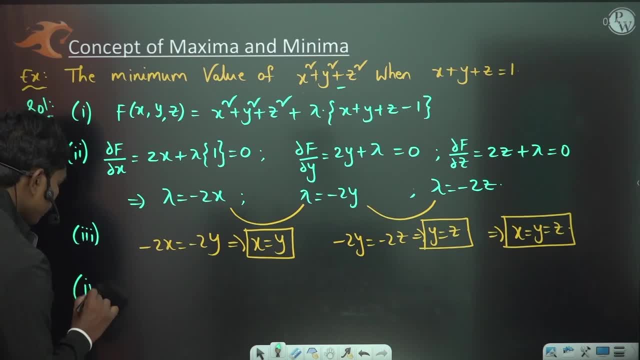 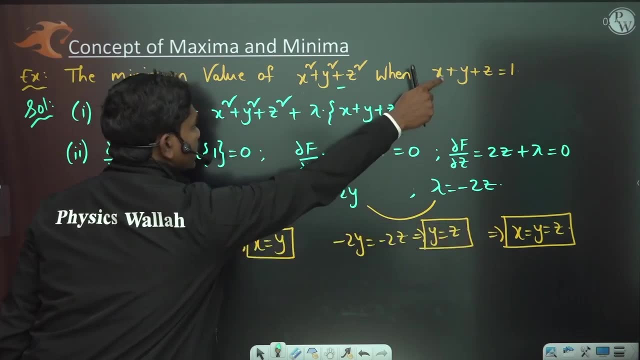 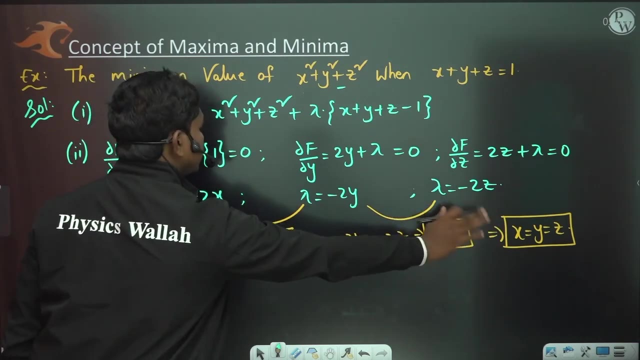 basically so fourth step is. fourth step is: substitute the relation in this constraint equation. okay, so substitute the relation for X Y Z in this equation and get the values of X Y Z. look till this step. you just got the relation between variables. you don't know what is X value, what is Y value, what is that? 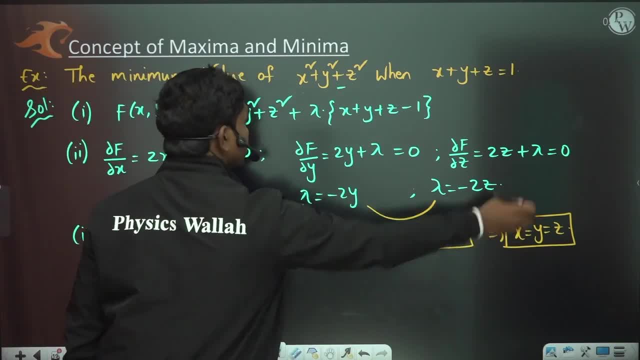 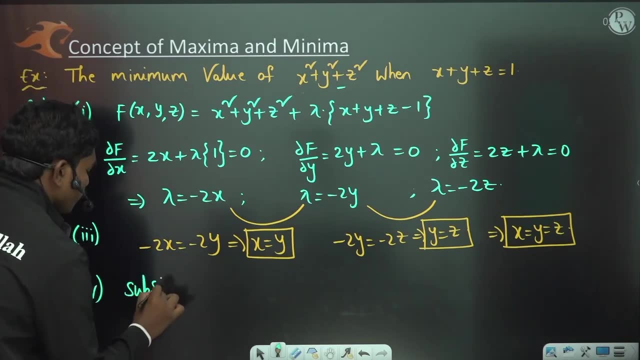 value. now, who will give you these values? if you substitute this relation in this constraint equation, you will get the numerical values. okay, so this implies substituting. substituting X is equal to Y is equal to Z. in X plus Y plus Z is equal to 1. 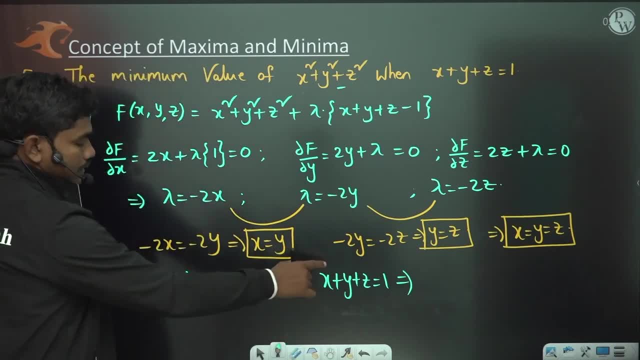 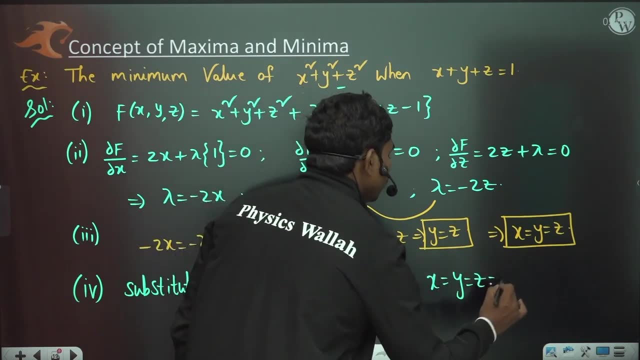 implies both. if you replace Y as X and Z as X, three times of X is equal to one, so X is equal to 1 by three, or, since all these numbers are equal, so X plus Y plus Z is equal to 1 by 3. now you got the value of the variables. 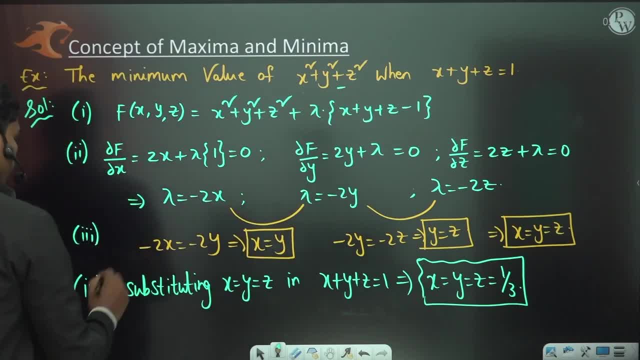 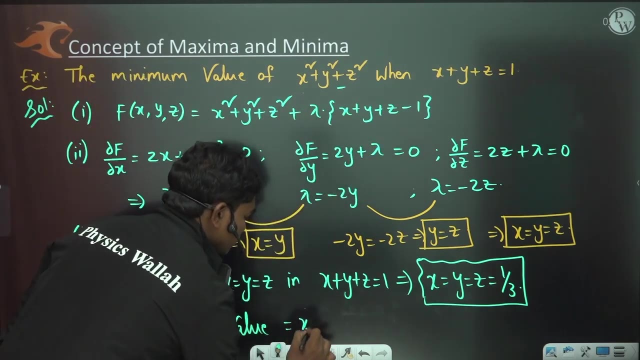 at which this function is minimum. actually, okay, so fourth, fifth step, therefore, minimum value. minimum value is equal to X square plus Y square plus Z square, which is X square plus Y square plus Z square, which. so what are the values of x, y, z at which this function will be minimum? you got this value, so. 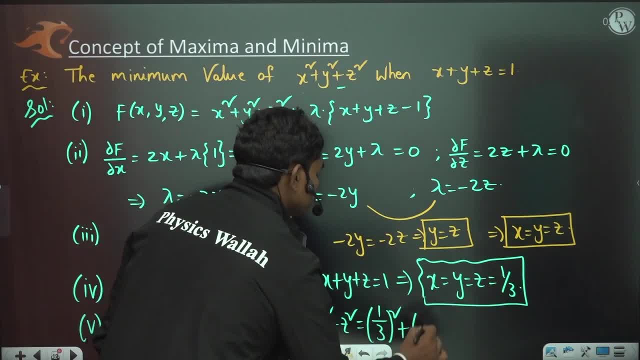 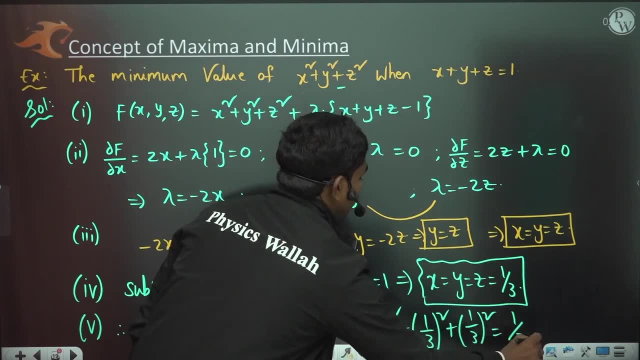 1 by 3 whole square plus 1 by 3 whole square plus 1 by 3 whole square total. so totally it is 3 times of 1 by 3 whole square. so this is 1 by 3. so 0.33 is the maximum value of. sorry, 0.33 is the minimum. 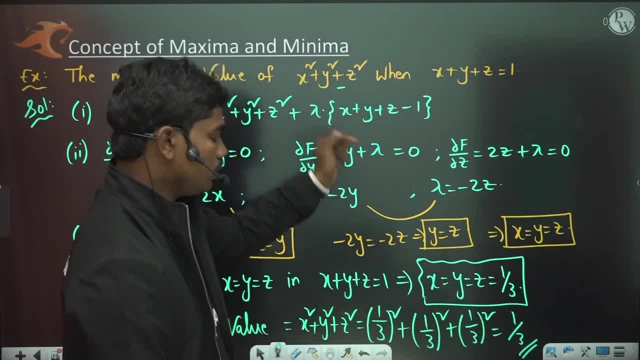 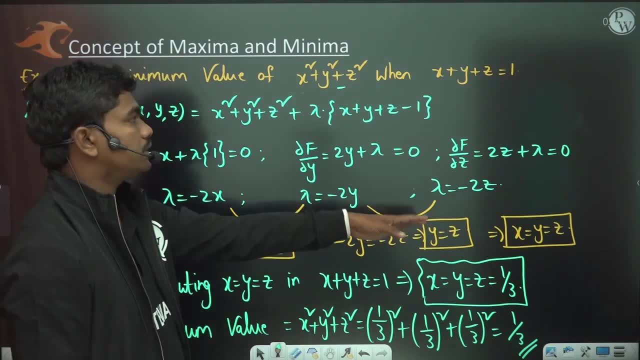 value of this function when x plus y plus z is equal to 1, so it is 3 times of 1 by 3, whole square, which is 1 by 3. you take any other value? definitely the answer. you take any other values of x, y, z? definitely this value. if you calculate you will get more than 1 by 3. you take any values. 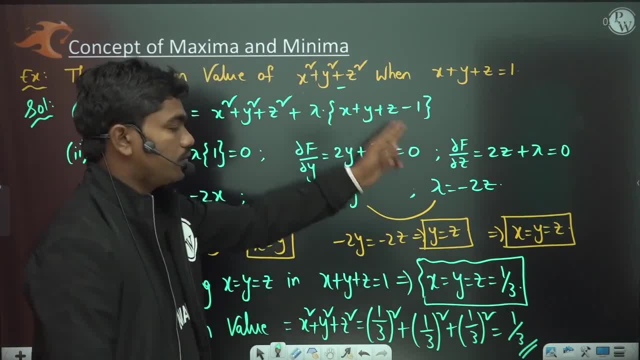 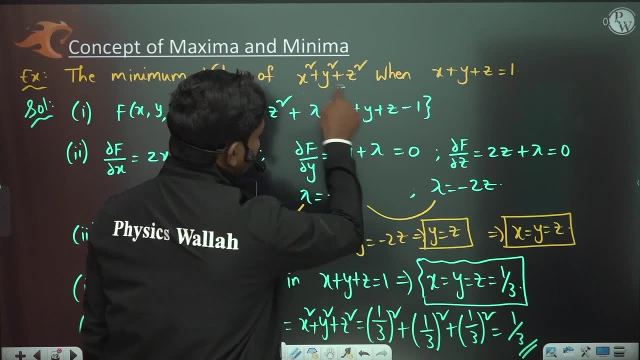 for example, 0, 0, 1, you can see its total value is 1, which is more than this 1 by 3. you take any other values randomly, you will definitely end up with getting this calculation as more than 1 by 3. okay, so this is called concept of constraint, maxima and minima. of course i have worked out. 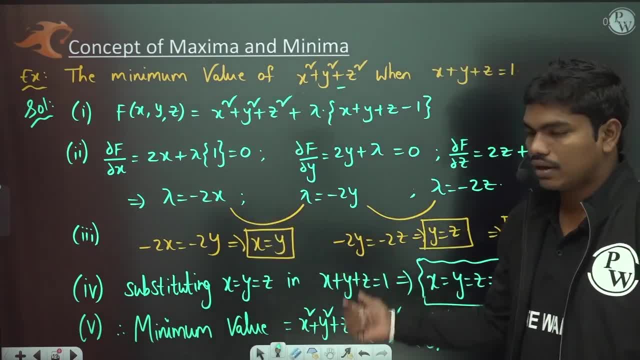 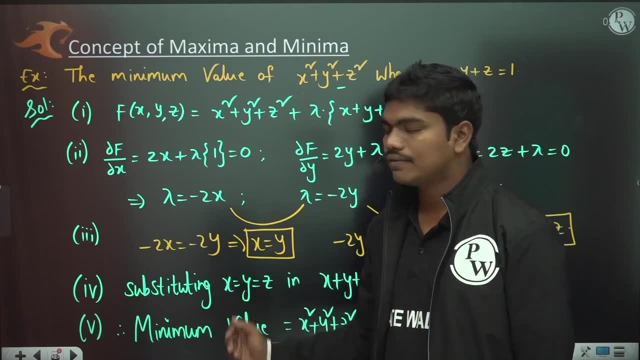 with a simple example so that the relation is very simple to attain. okay, so sometimes, depending on the value of x, y, z, you will get more than 1 by 3. okay, so this is called concept of constraint maxima and minima. here elimination process will be little tricky, that's it, except that the standard 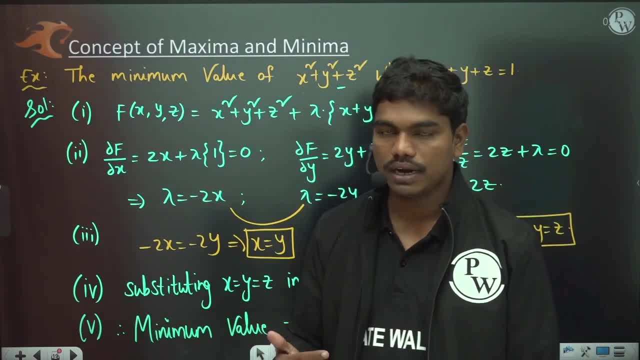 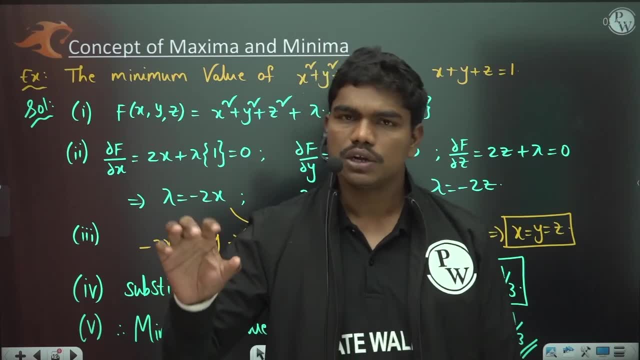 working procedure remains the same in case of this constraint: maxima and minima. and this is one really very important concept, because all practical applications, even though, if you want to maximize or minimize, to the best possible case, but they are again governed by some constraint, for example, you 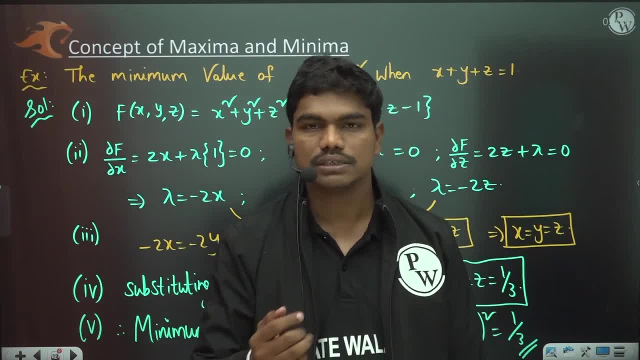 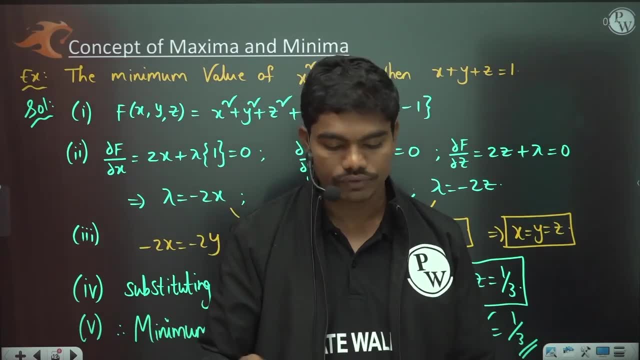 might have seen your linear programming, okay. so if you see linear programming, then what happens? your production is limited by the number of you know products that are available for you to manufacture. so if you see linear programming, then what happens? your production is limited by the number of you know products that are available for you to manufacture. okay, so if you see, we have for. 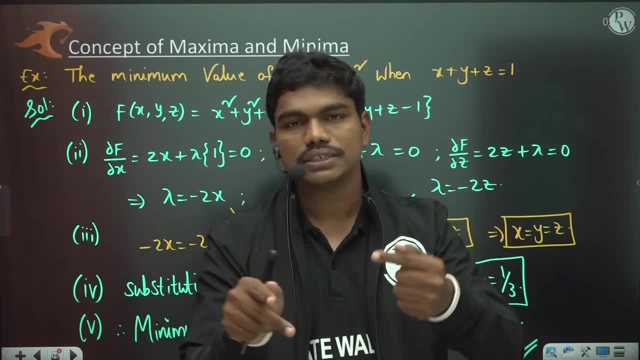 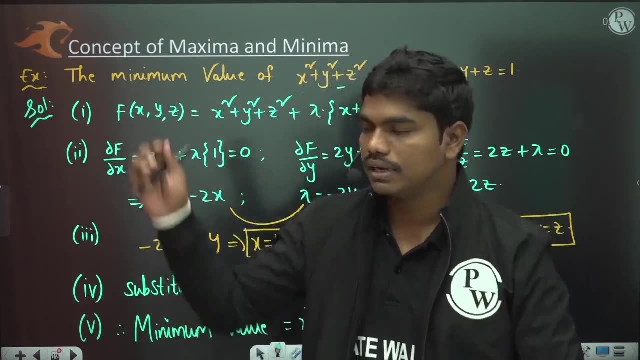 example, if you want to manufacture product a which equates two components, then the number of if, when you are trying to optimize number of quantities of production of a, that depends upon the constraint equations. so similarly, something like this: if you see, here we have a function which you are supposed. 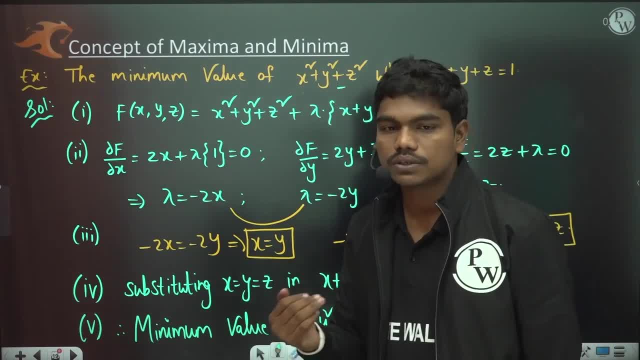 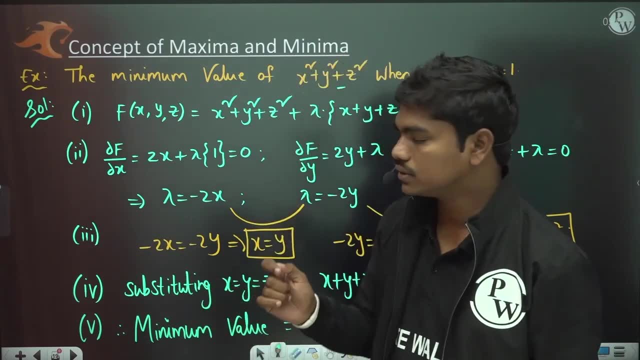 to maximize, but again, you are governed by some constraint equations. okay, so this constraint, uh, maxima and minima concept is really one very important concept in, uh, you know mathematics again. so i, uh you know you need to put some, definitely some of the functions that you have in your model. 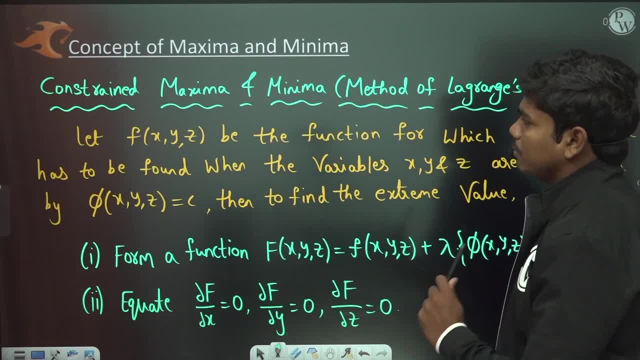 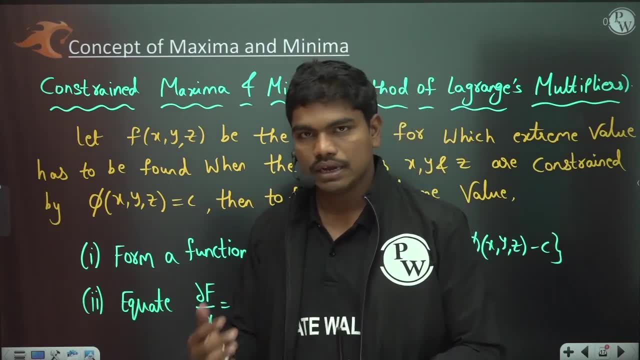 some special attention onto this concept of maxima and minima in constraint case. okay, so i hope this is clear to you. so till here, let us once quickly collect what we have learned in, uh, this course, i mean in this class. just take a quick revision, let us have so we have talked. 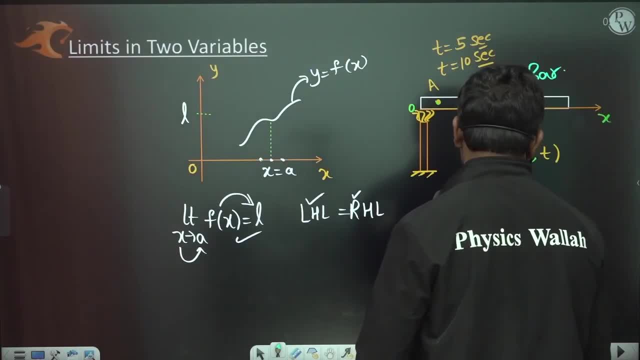 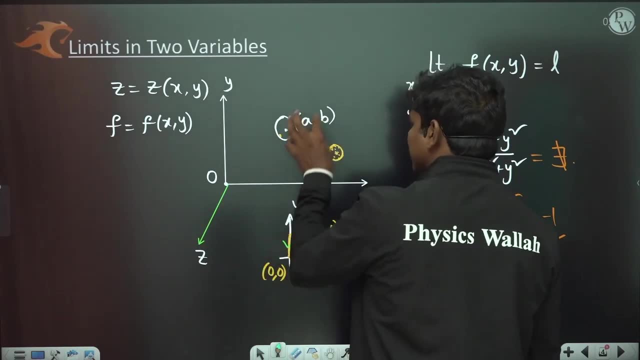 about limits in a single. first of all, we have understood why there is some necessity of multi-variable functions. okay, so once we are done with that, we have understood what is the neighborhood in a 2d uh area basically. so it's a cycle of some radius. 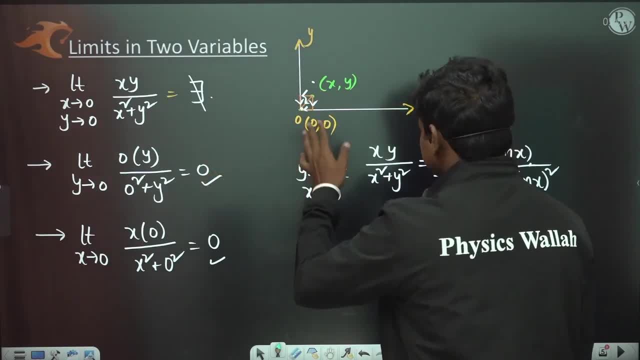 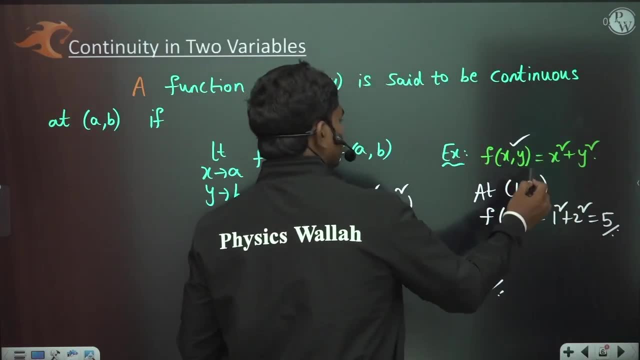 so now, if you see, we have seen how to calculate limits into variables in general, the general path. we have considered all these things. okay. so then we came to the continuity of a function we have. i have shown you with the example of x square plus y square. i have plotted this graph actually. 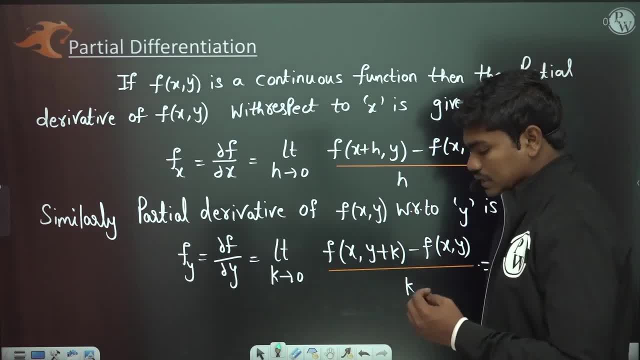 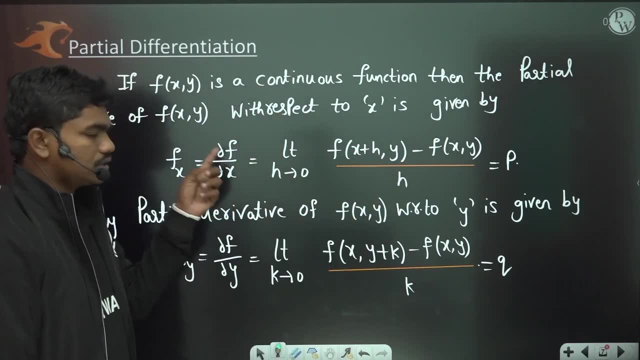 on the plotter and i have shown you. so we have identified what is partial differentiation. so, in general, what happens? the quantities, or f, this function f, let us suppose, if i take this f as some temperature or pressure or something, basically. so they change with respect to many quantities. so 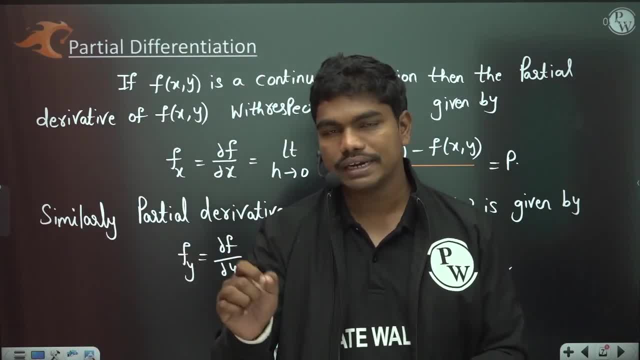 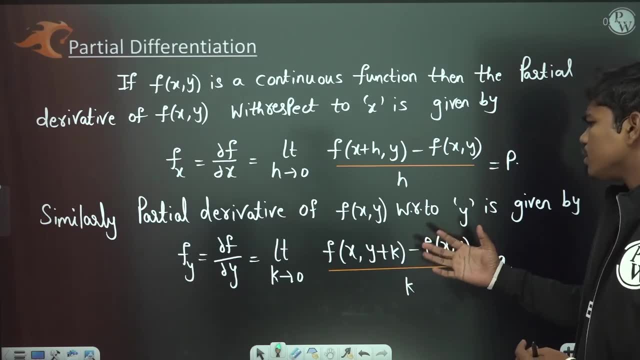 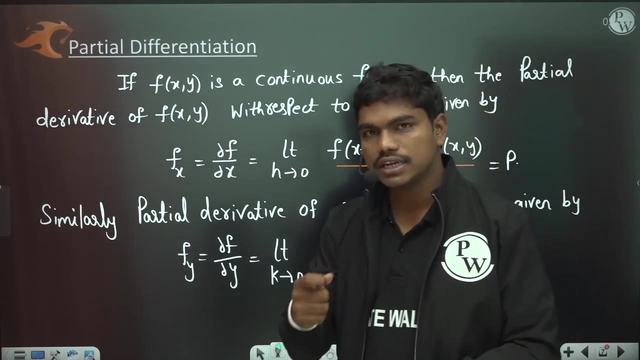 it's really difficult for us to measure the changes simultaneously with respect to all the changing variables. so what we do generally, we have actually uh, you know, uh, we have uh created the change. we have treated. the partial changes means when you have differentiated with respect to x partially, that means you have treated your y means. basically, here it's two variables. so when 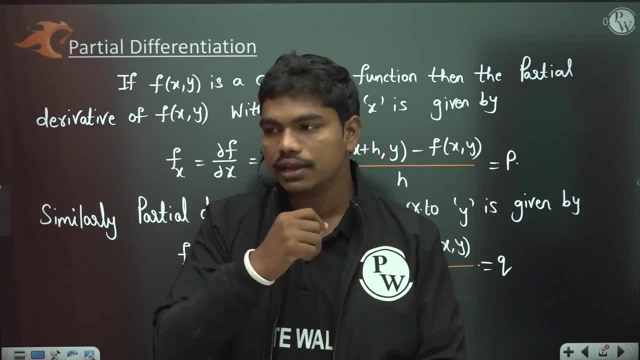 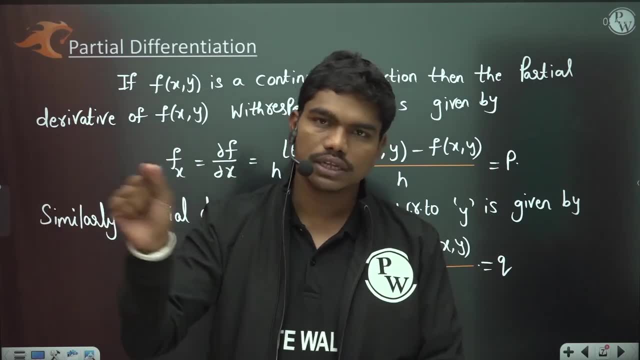 i am differentiating with respect to x, i'm treating y as constant. but let us suppose if we have some five, six variables, whenever you're trying to differentiate a function with respect to a particular variable, except that variable, you'll treat all the other variables as constants. okay, so that's how you'll. 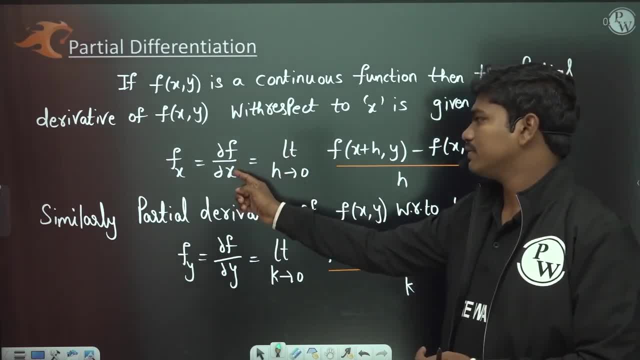 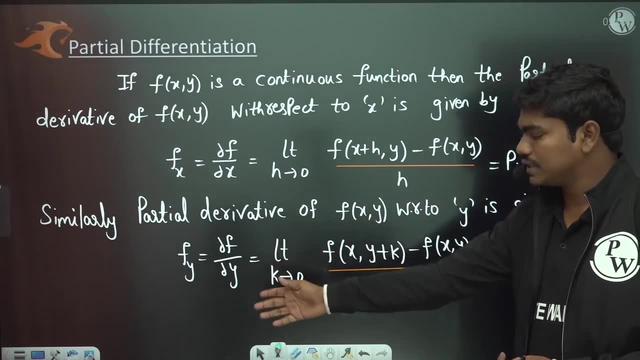 get these definitions of fx and xy. when i'm, whenever i'm differentiating with respect to x, i'm not considering any change in y in this. uh, you know calculation. so, similarly, when i, when i was differentiating with respect to y partially, i'm not considering any change in x here. okay, 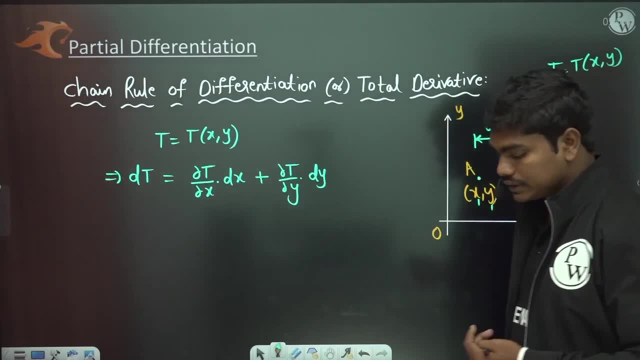 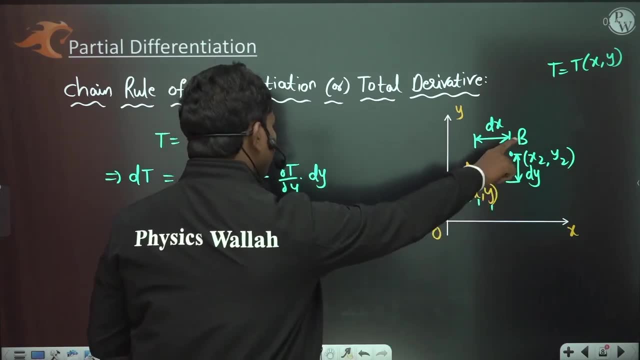 so i told you these are denoted by p and q. then we have given chain rule of differentiation. so, practically, what does chain rule of differentiation tells you? if you want to identify change of a property between two locations, of course very close to each other, then this is given by dou t, by dou x into d x, plus dou t by dou y into d y, this term. 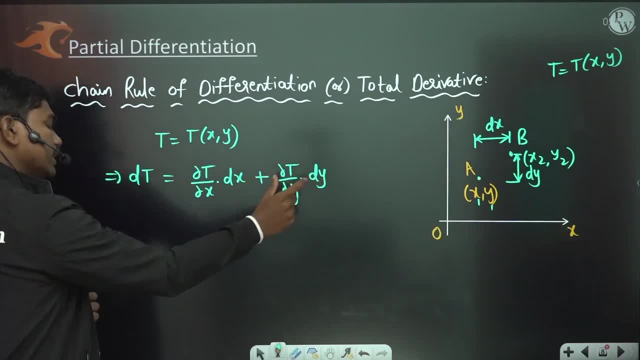 corresponds to the change of this quantity, t because of the change in x, and this term corresponds to the change in t because of the change in y. actually okay, and of course, formula wise, you know this is chain rule: dou t by dou x into d x, plus dou t by dou y into d y all, or normally you'll use this: 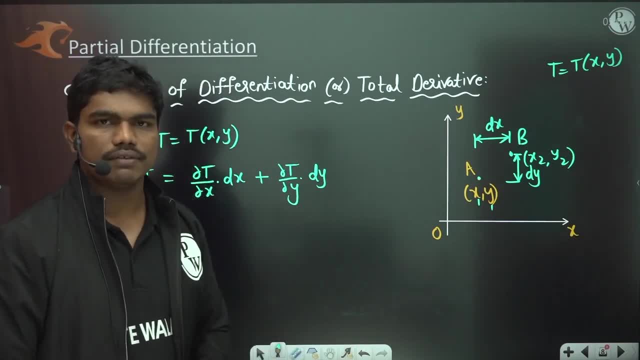 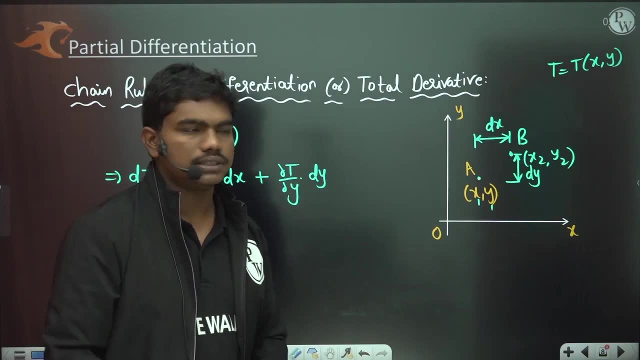 concept of total differentiation. uh, in fluid mechanics, for example, in fluid kinematics, when you're trying to calculate the accelerations, you remember these expressions: u into dou, u by dou x. all this is basically nothing but the chain rule of differentiation. as next we talked about some 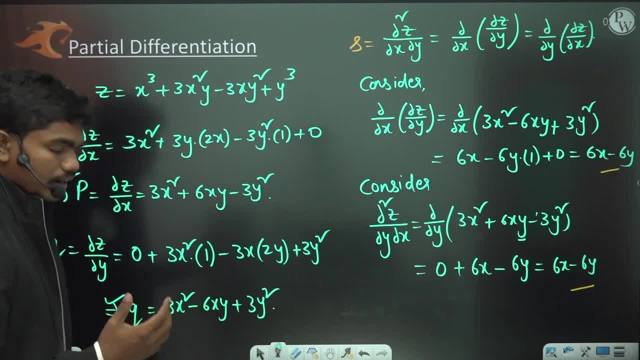 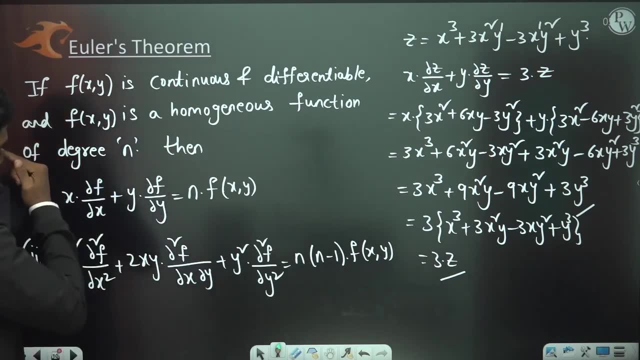 partial differentiation- uh, basic understanding. look, some of you might have forgotten how to do the partial derivatives and all, so i have given you some quick 5 to 10 minutes of uh intro there. and then we came to one very important theorem of partial differentiation especially, and that's: 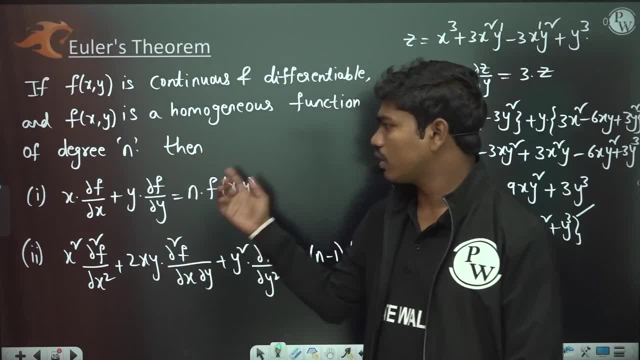 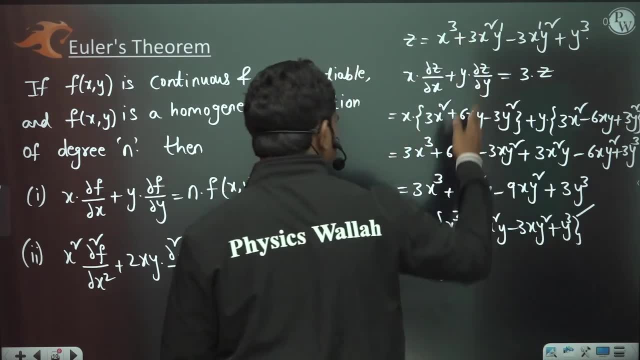 euler's theorem or euler's theorem, you can say so. if you see, we have talked. what is the homogeneous function of degree n? so in that we have seen two important results that we have seen in the previous video, which we have obtained using big calculation after identifying this newton, i mean. 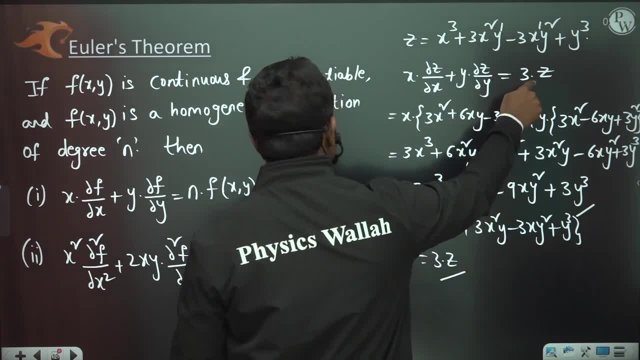 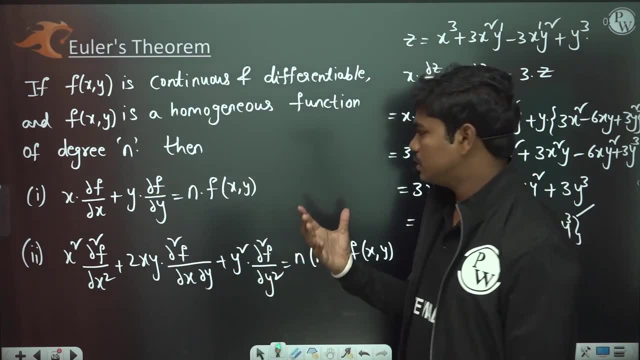 this euler's theorem we have written in a single line here, okay, and this, this tz, is written with the help of this euler's theorem and this complete calculation is basically the standard procedure for finding different derivatives and substituting and get the values, okay. so these are two important. 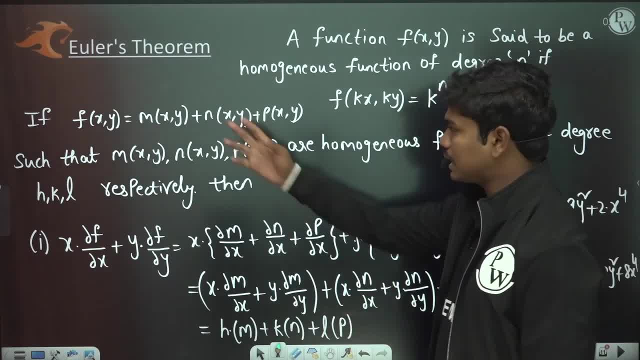 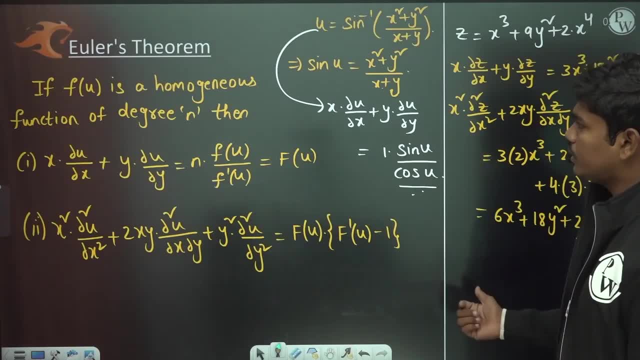 examples that we have taken out now, if you see, this is again euler's theorem. so if f, if it is split into some functions of different degrees of homogeneity, then this is how we'll work out the things. okay, and i told you, sometimes the function directly is not a homogeneous function, but some function of. 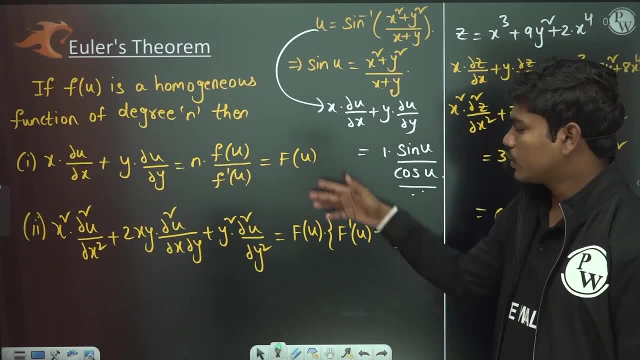 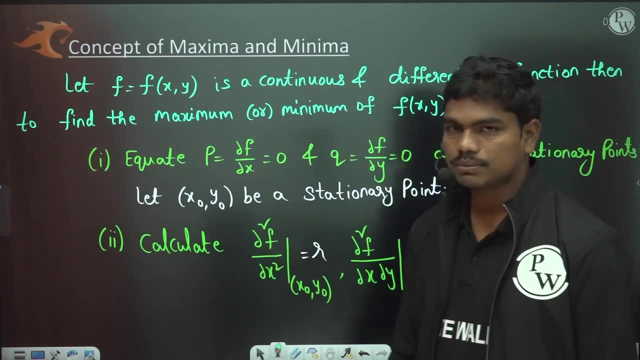 this dependent variable is homogeneous. so in such cases i told you how to deal with the things. i have given you some example also here. we worked out few things and then we came to the concept of maxima and minima in two variables. okay, so in two variables how will we calculate maxima and minima, like in? 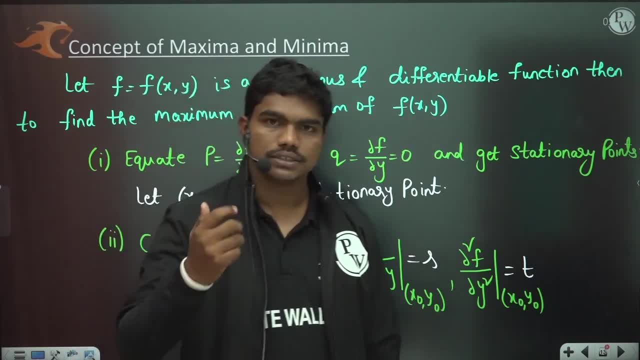 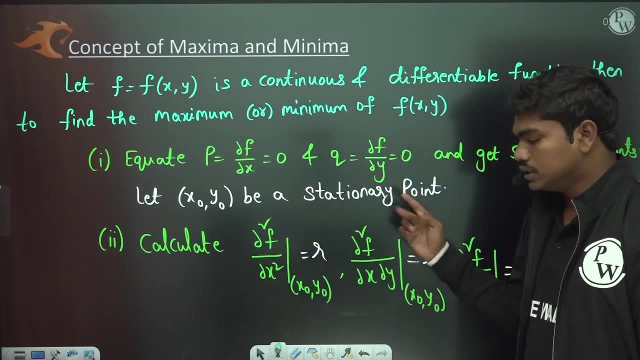 the case of single variable, first of all we equate the derivative to zero. but since the number of involved- uh, the number, of you know, variables that are involved- is equal to the number of variables, is more so we go for partial derivatives and equate them to zero. so once we solve these two, 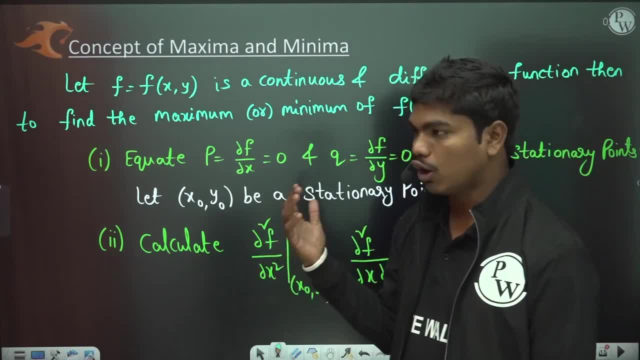 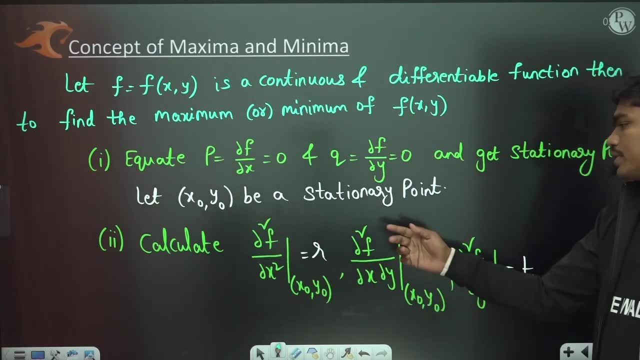 equations. then we'll get some stationary points, depending upon the function. actually, how many stationary points we'll get, that depends on the function. so i have taken the case of one stationary point and i have explained in the procedure. so you need to calculate rst values. r is dou square. 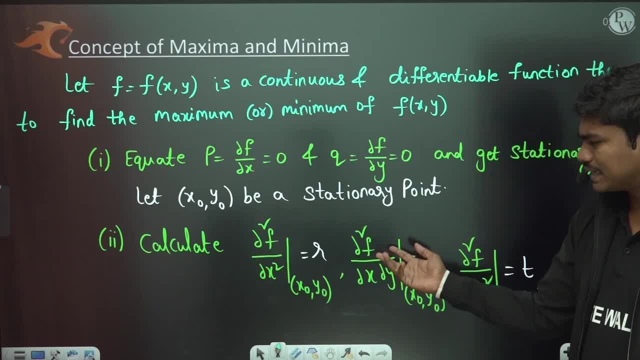 f by dou x square. yes, is dou square f by dou x, dou y. or it can be dou square f by dou y, dou x. also okay, because we have seen this order of differentiation doesn't impact the value. similarly, we have calculated t. now we see checking conditions like rt minus s, square value and r value, depending upon this rt minus s. 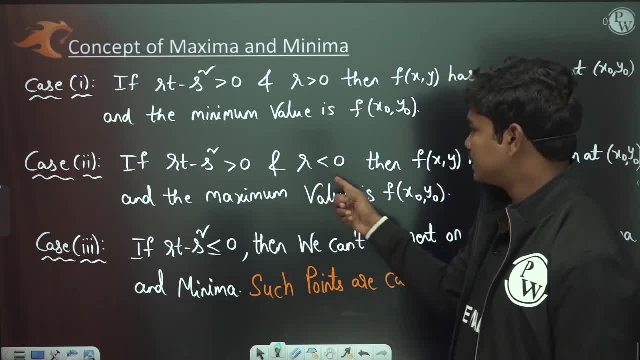 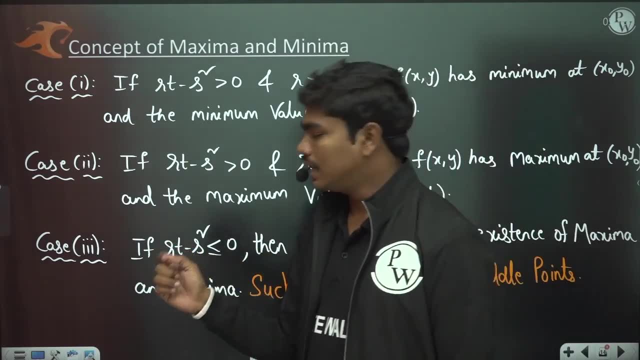 square greater than 0 and r greater than 0, less than 0, we have certain maxima or minima conditions and finally we came to one thing: that if rt minus s square is actually less than or equal to 0, then we can't comment on the existence of maxima and minima. okay, like in case of points of inflection. 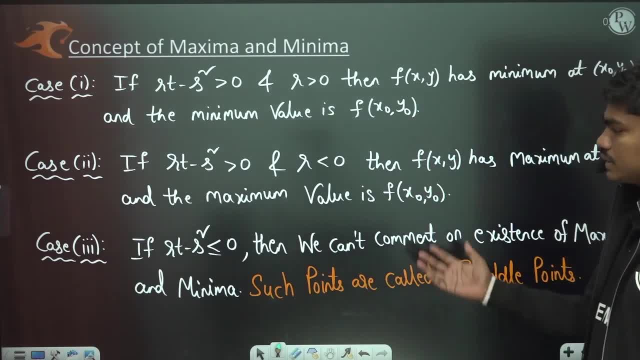 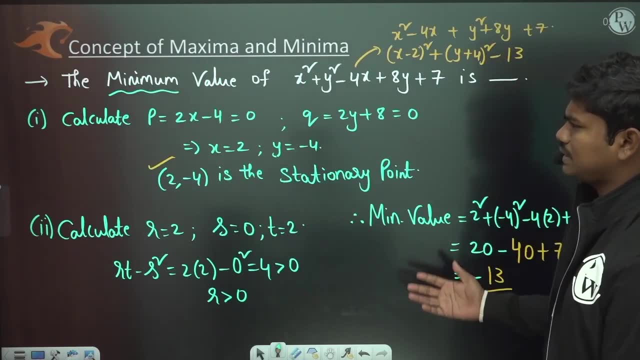 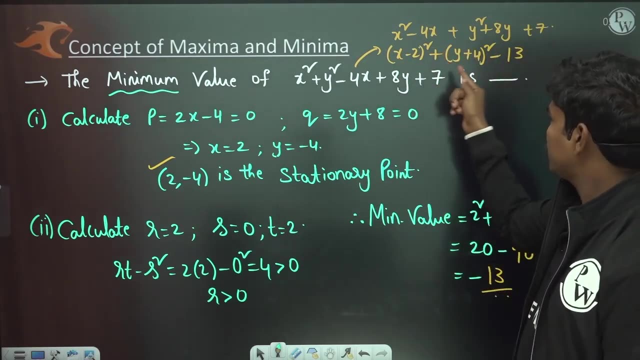 in the single variable case. here we have this saddle points in case of multi-variable case. okay, then, we have solved some examples to make you understand the working procedure. one more example. i think we have done so, uh, just to and for this example, i have given you the- uh, you know, normal, intuitive way as well how this minus 13 and minus 13 here. 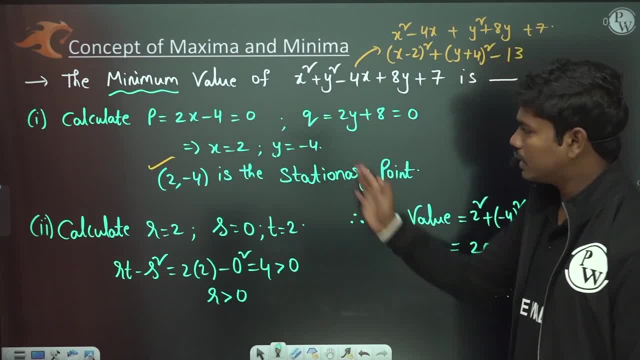 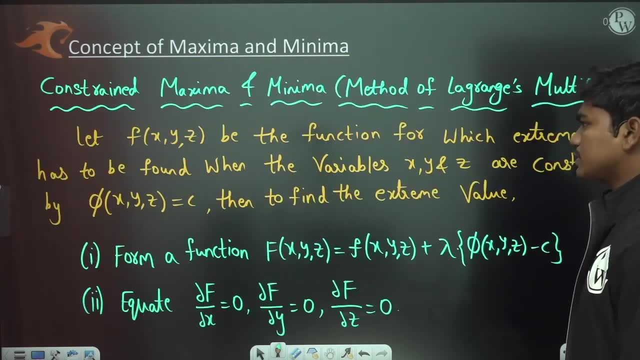 are matching with each other. because of one: we have calculated using the standard maximum procedure. second, we have done by adjusting the terms as quadratic expressions. okay, so, once we are with this, we have started this concept of constraint, maxima and minima and method of lagrange. 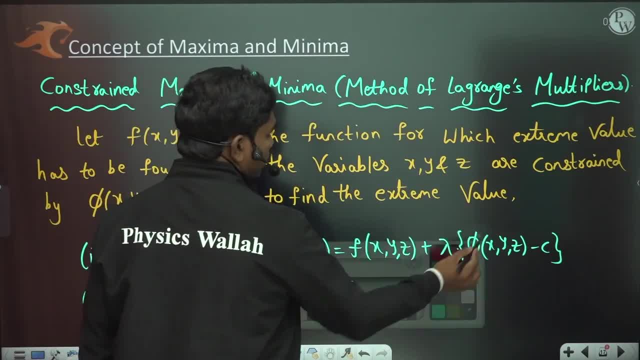 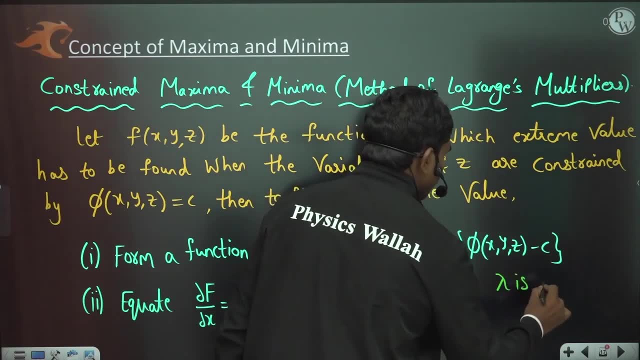 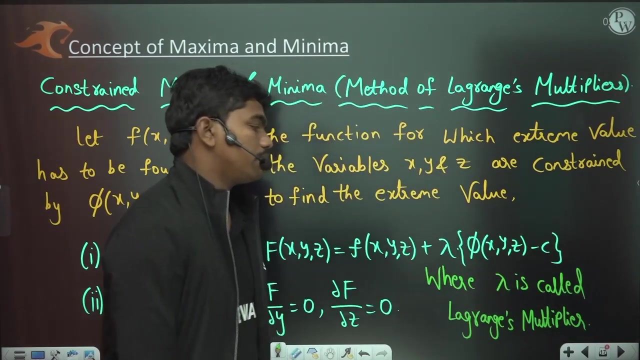 multipliers. here, if you see this lambda value is called lagrange multiplier. where lambda is called because this is actually multiplied to the constraint equation, so lambda is called lagrange multiplier. so that's why it's called method of lagrange multipliers sometimes, so lagrange multiplier. okay. so where lambda is. 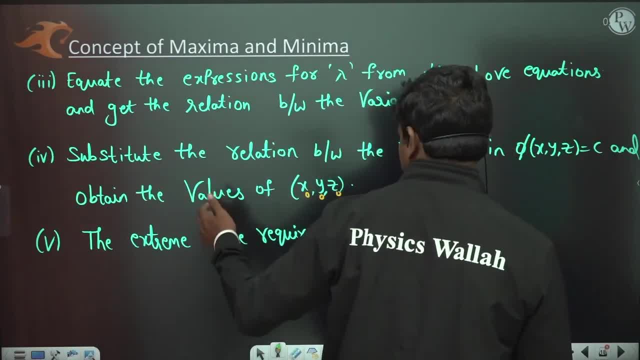 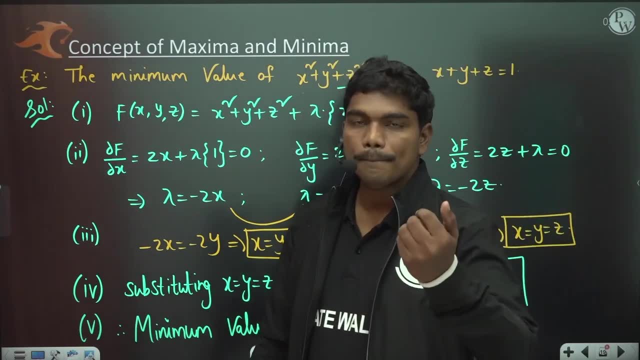 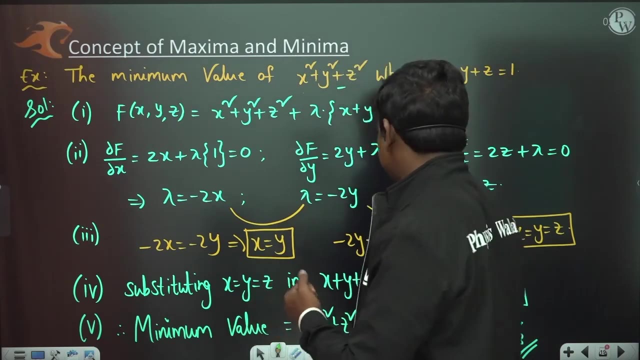 called lagrange multiplier. if you see, then we have set some working procedures- three to five lines. then we have seen an example how we basically worked this working procedure in analyzing the minimum values of the function basically. so is this clear to all of you till now? so if it's clear, then let us uh move on to the next part, okay, so 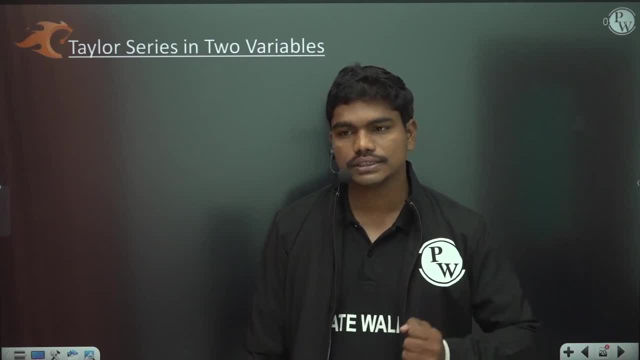 taylor series in two variables. okay, so how we do taylor series in two variables? we have seen in single variables. let us suppose, if you want to generate a taylor series- expansion of any continuous and differential function with x minus a terms in the series, then we have seen. 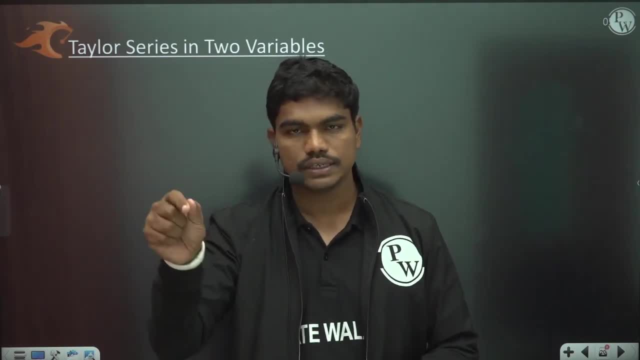 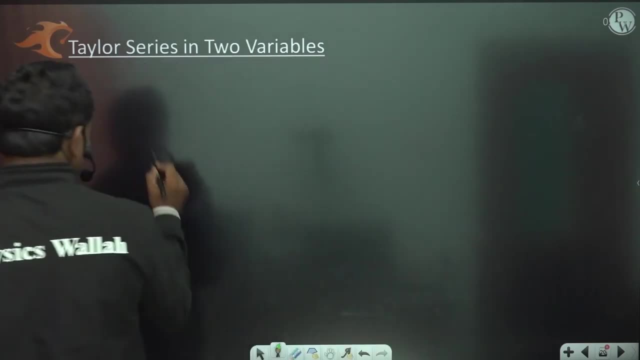 f of x is equal to f of a plus x minus a, by one factorial into f dash of a. all these things are we have seen, okay. now let us see what happens in case of a 2d case. okay, so if, if f of x comma y is: 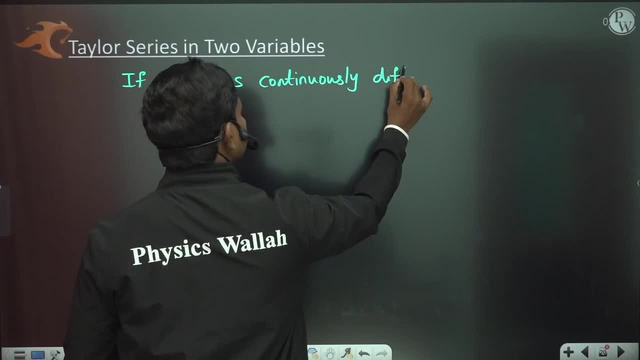 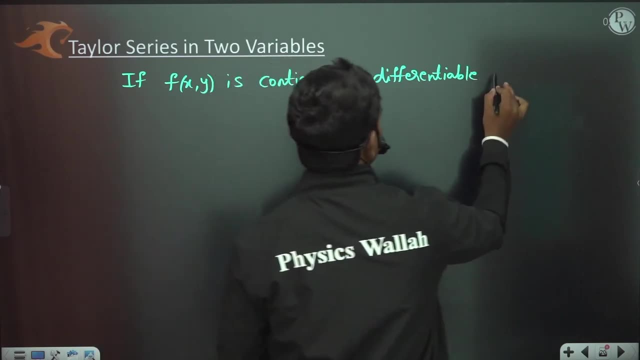 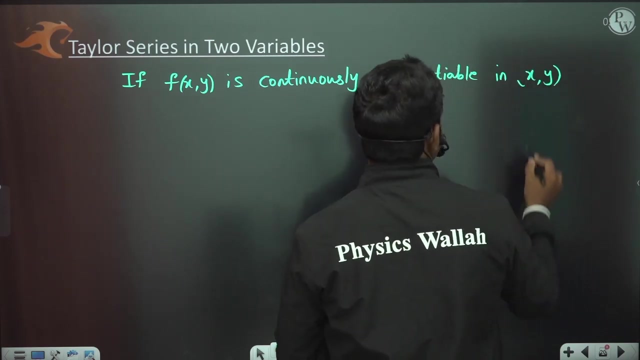 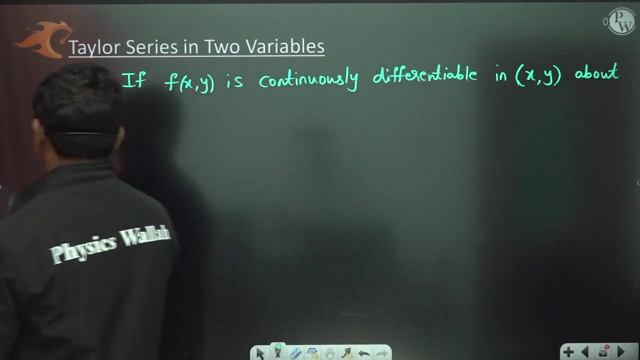 continuously differentiable means all the derivatives they keep on existing is continuously differentiable in. continuously differentiable in x comma y. continuously differentiable in x comma y. about the point a comma b. about the point a comma b means if you see all the derivatives at this point a comma b. 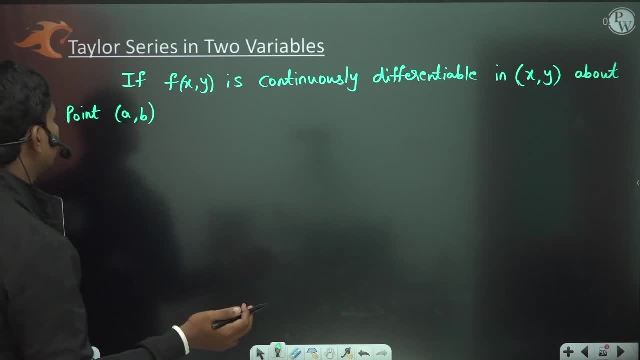 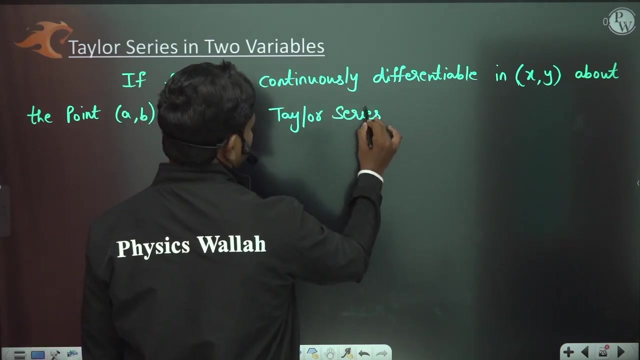 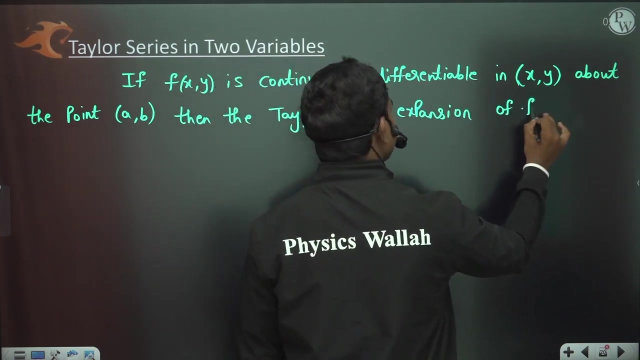 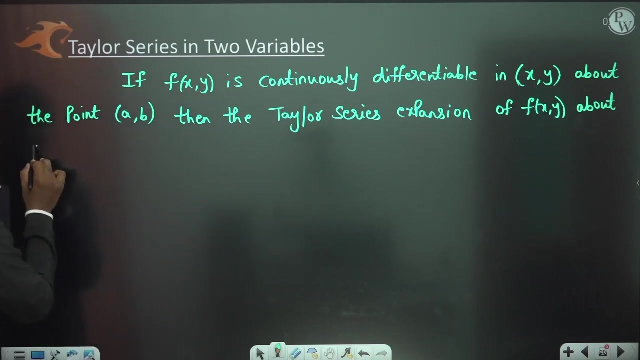 exist continuously means first derivatives, second derivatives, all these things. okay, about the point a comma b. now let us see how we write this. then the taylor series expansion, then the taylor series expansion. then the taylor series expansion of f, of x comma y. about a comma b. about a comma b is about a comma b. let us say a comma b is given as get plus two, porque etc. 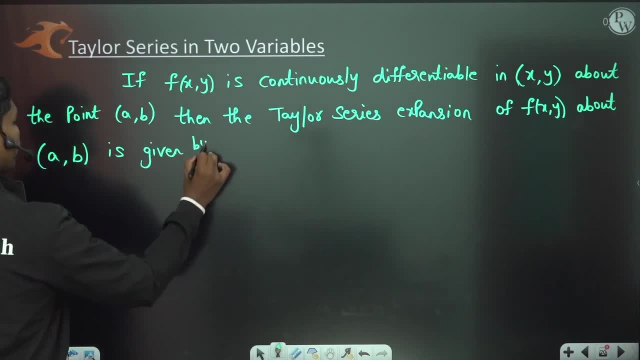 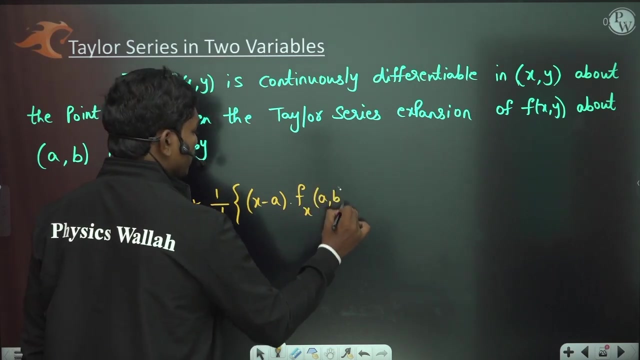 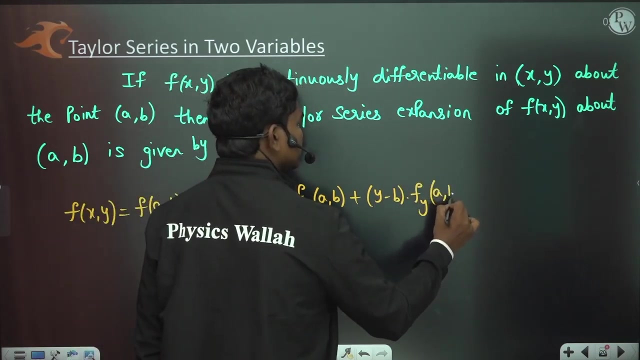 by is given by is given by f of x comma y is equal to f of a comma b plus 1 by 1 factorial times of x minus a into the first partial derivative of x at a comma b plus y minus b into first partial derivative of f with respect to y at a comma b. So this is the first term. 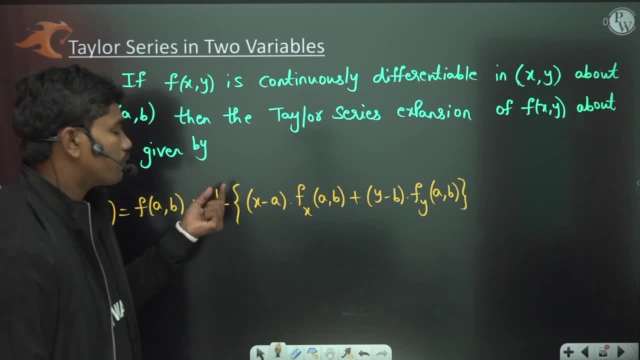 means basically f of a comma b plus 1 by 1 factorial times of x minus a into fx of a comma b plus y minus b into fy of a comma b plus 1 by 2 factorial times of 1 by 2 factorial times of. 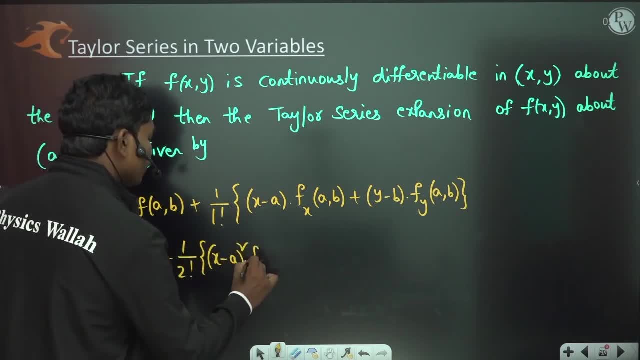 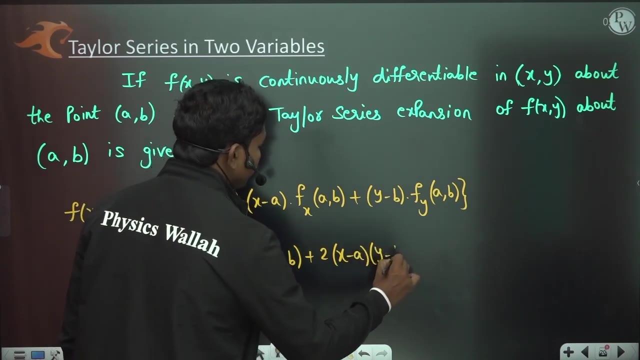 x minus a whole square into fxx means second derivative with respect to x. So this is nothing but dou square f by dou x. square at a comma b plus 2 times of x minus a into y, minus b into f of xy means dou square f by dou x, dou y, or it can be fyx, also dou square. 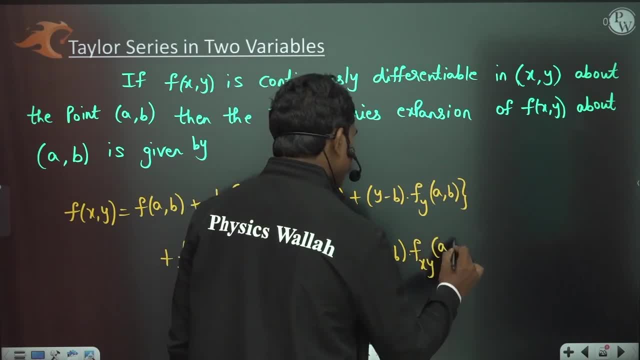 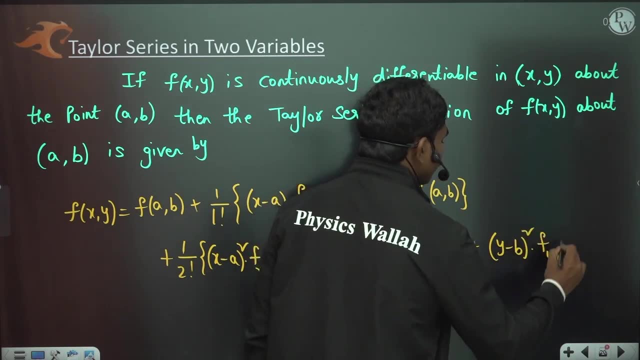 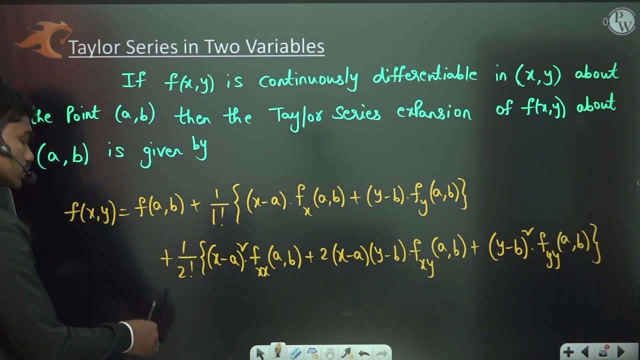 f by dou by dou, x at a comma b plus y minus b, whole square times of fy, y at a comma b. So this is the Second degree terms basically in this Taylor series. Similarly, if you want to add plus third order, so plus 1 by 3 factorial times of x minus a whole cube into fxxx a comma. 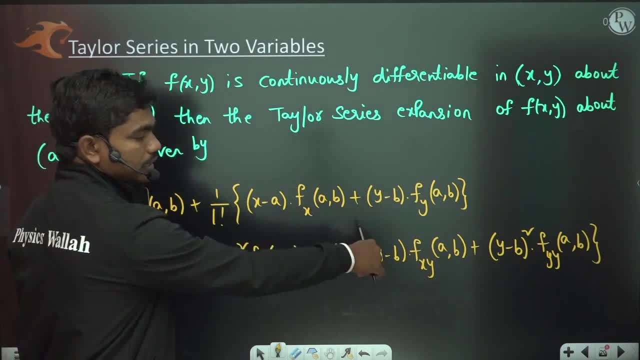 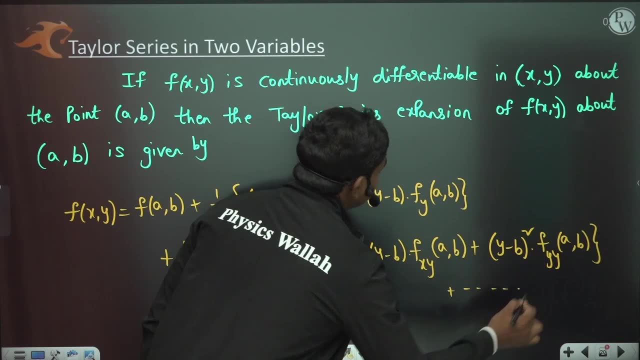 b plus 3 times of x minus a whole square into y minus b, into fx square: y a comma b. So similarly, like the cubic expression. Okay, So this series will go on like this, actually. Okay, So this is how you generate a Taylor series: expansion in two variables of a continuous and differentiable. 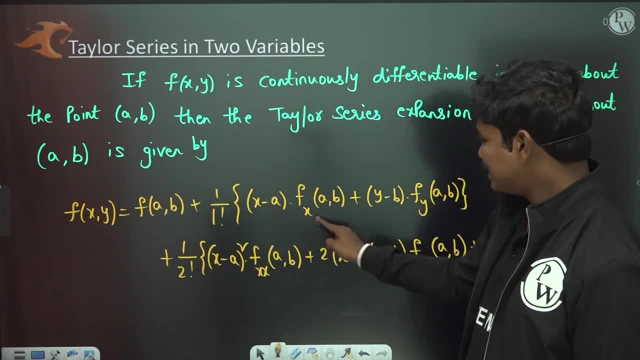 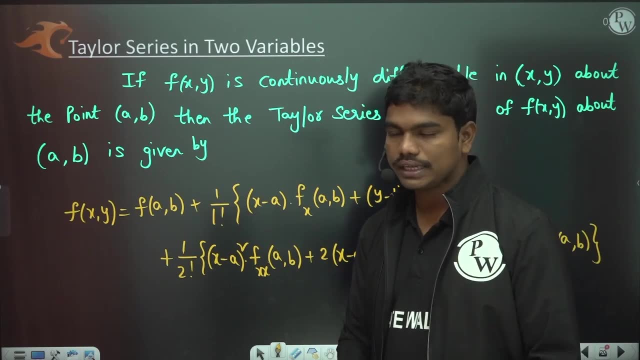 function. Okay, Why the function should be continuously differentiable? Because the derivative of f, x, fy, f of f of x, f of y, f of y, f of x, f of x, f of y, all these things should exist actually. Okay, And if you want only x, y terms of the equation, then you'll. 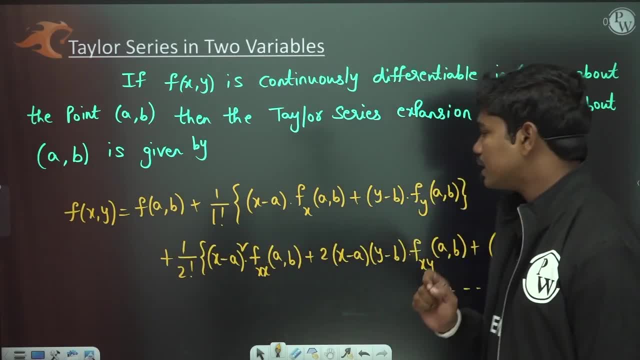 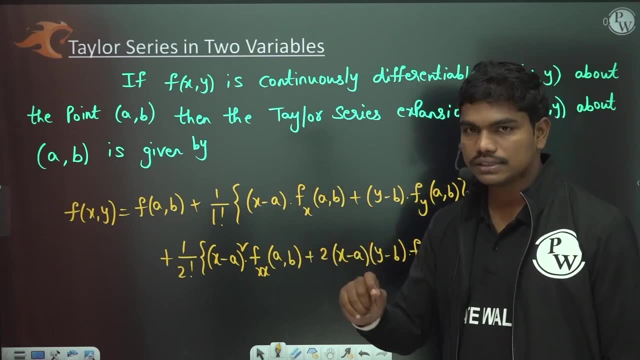 take this a comma b point as 0 comma 0,. of course, Okay, And this is how you generate the Taylor series. Now I would like to take one moment in explaining you how this one- I mean single variable- that has come from this two variable Taylor series. Okay, So, 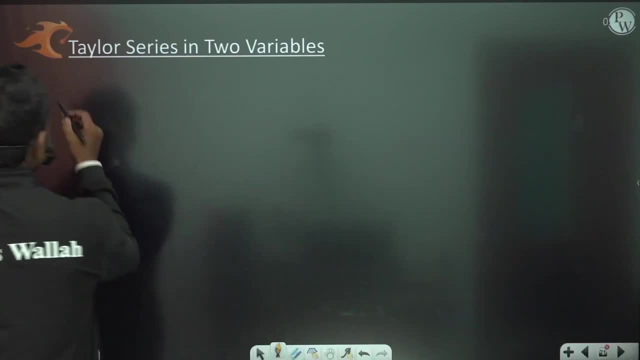 for that. let me take some moment and explain you. So if you see this two variable expansion: f of x, y, y, equal to f of a comma, b plus 1 by 1 factorial times of x minus a into first derivative partial. 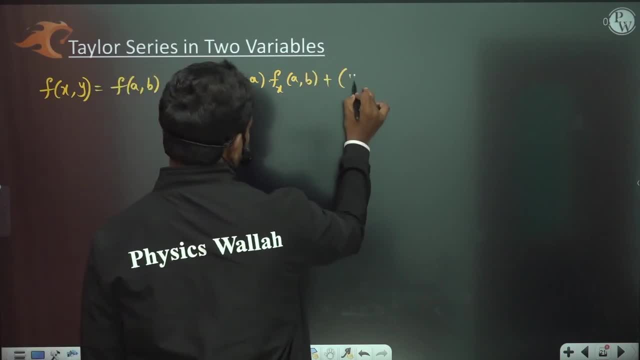 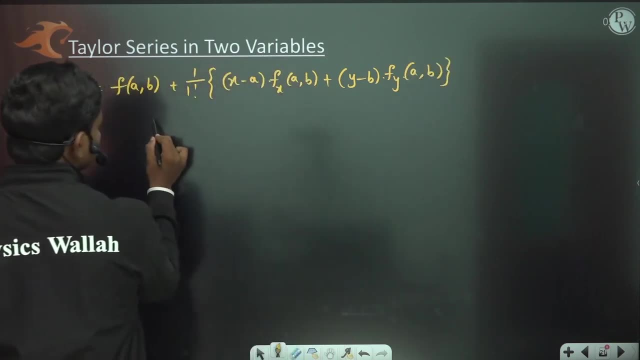 derivative at a comma b plus y, minus b, into fy at a comma b. so this is your first factorial term, means the linear terms. similarly, here you have linear approximations, quadratic approximations, all these things, as i told you in previous single variable case, if you see, if you, if i ask you what, 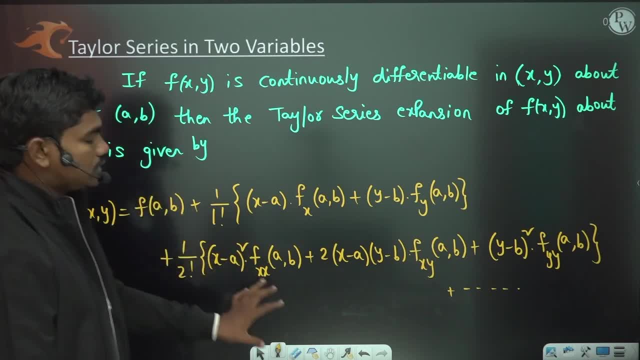 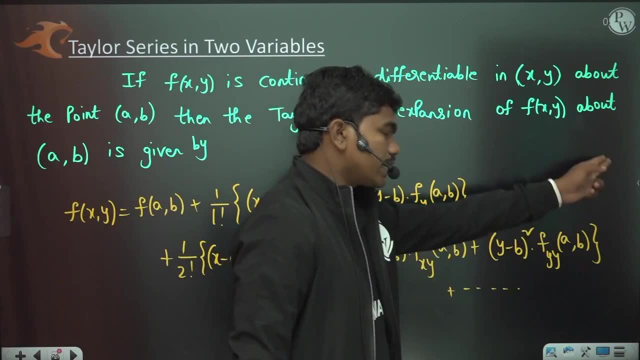 is the linear approximation of this function. about this point, you will consider this taylor c is only till this point. okay, so that's the linear approximation. if i ask you for the quadratic approximation, you will consider till the second degree terms. okay, so that's how we consider the. 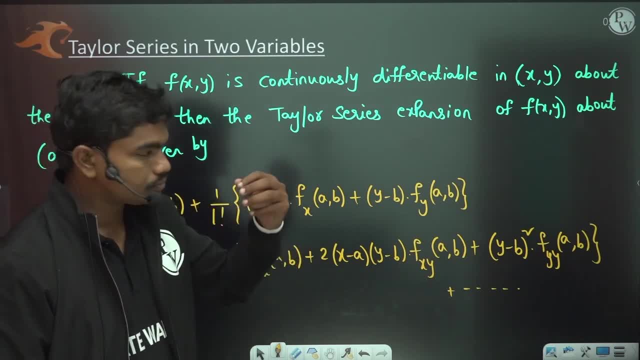 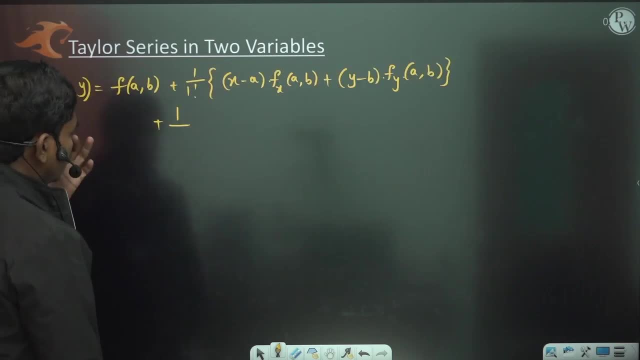 linear approximations and quadratic approximations of this taylor c is in two variables actually. okay, so let us continue here. so this, this is the case now, if you see. let us see 1 by 2 factorial times of x minus a whole square. okay, x minus a whole square into x minus a whole square, into second derivative at a comma b, with: 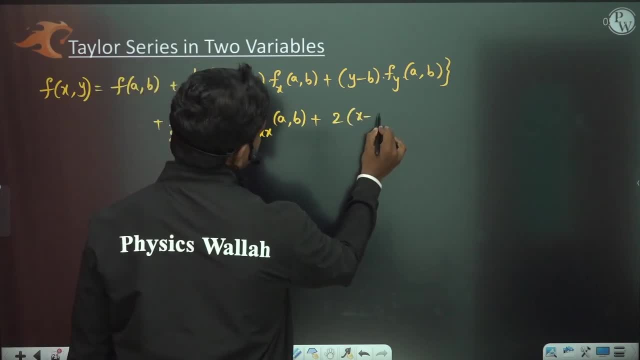 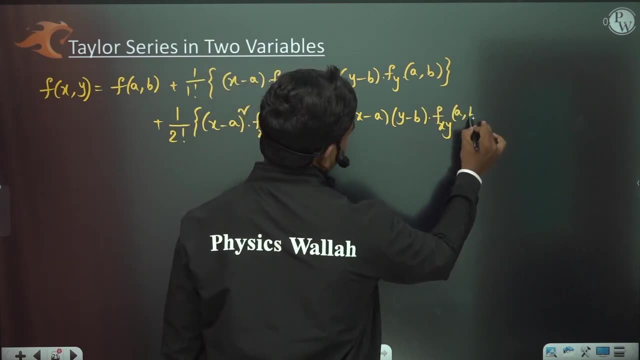 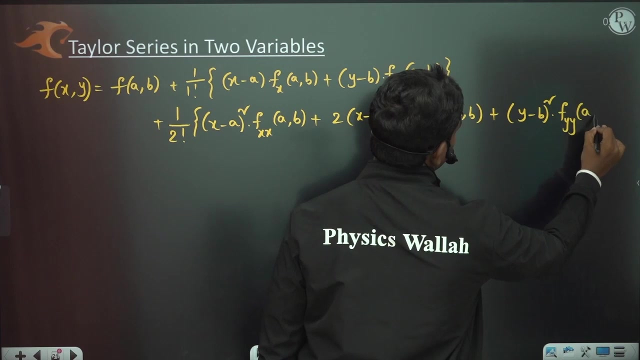 respect to x plus two times of x minus a, into y minus b, into f x y at a comma b, plus y minus b, whole square times of f y y at a comma b. okay, so once you have this plus and so on, of course you can write this: 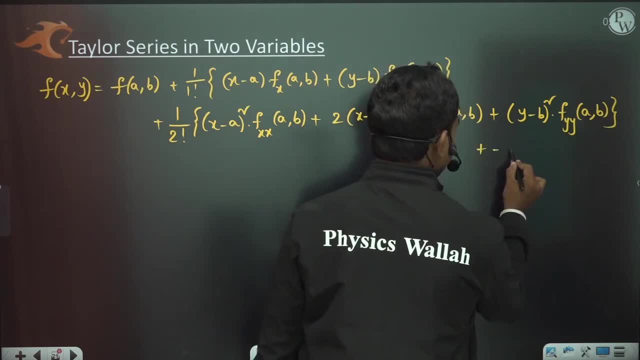 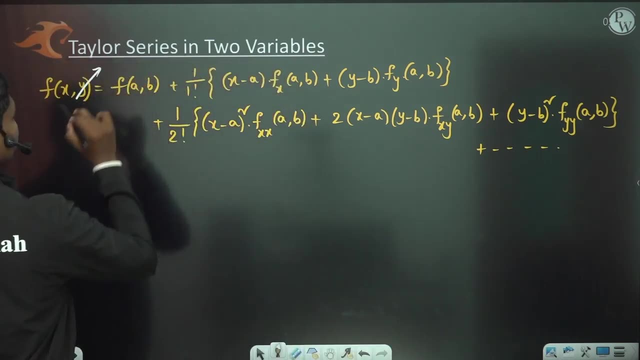 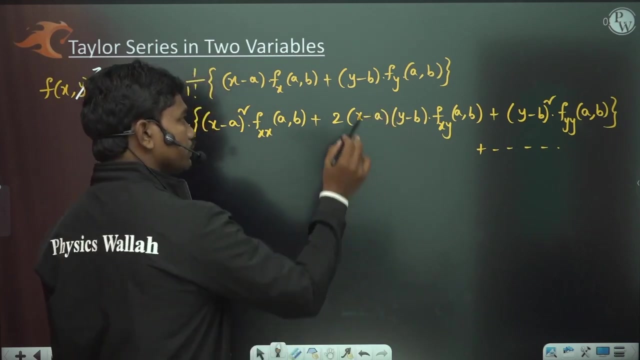 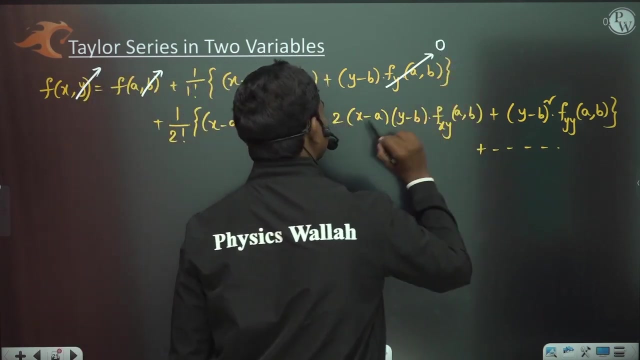 more of this become, you can write this to the denominator so you don't have the consequence, okay, and such as the one. so if you see, in single variable, in case of single variable, let us see what happens. first of all, you don't have this y variable involvement, so obviously you won't have this second quadrant b involvement. okay, and obviously there is no way. so whenever if you differentiate a function of x which is completely in terms of x with respect to y, then this partial differentiation will go to zero, that's on. and of course, this a y minus b term is also not existing because it's a single variable calculus. okay, so what we will study is we will discuss some. 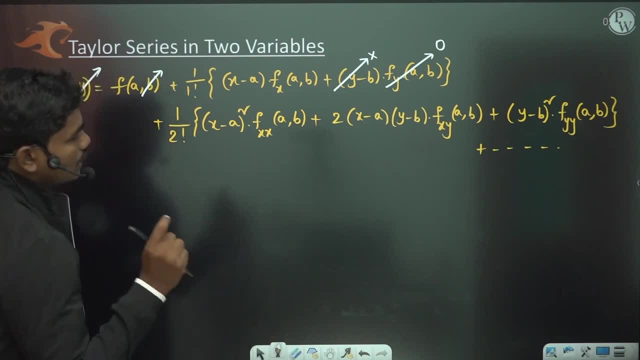 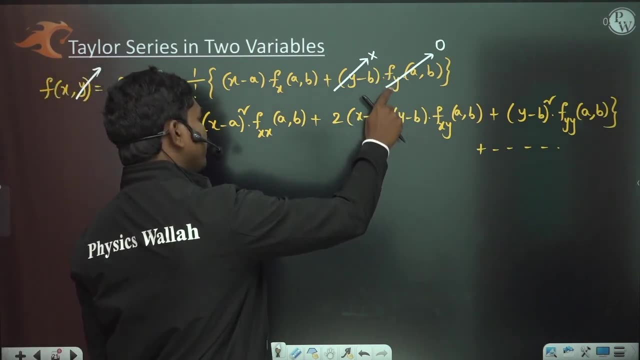 So if you, if you try to understand, if you take a function only in terms of x, for example, Let us say so, if you take a function only in terms of x, this partial differentiation of function with respect to y will go To 0. similarly, here also there is partial differentiation with respect to y. here also, there is partial differentiation with respect to y. 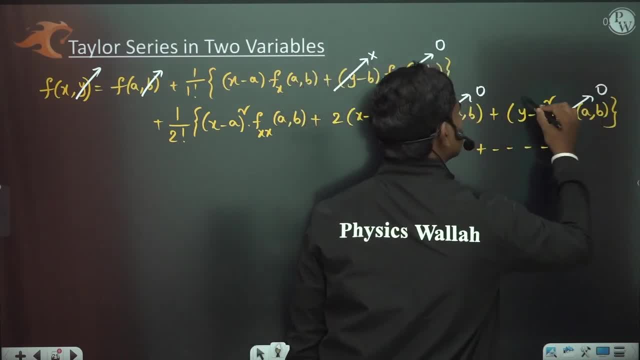 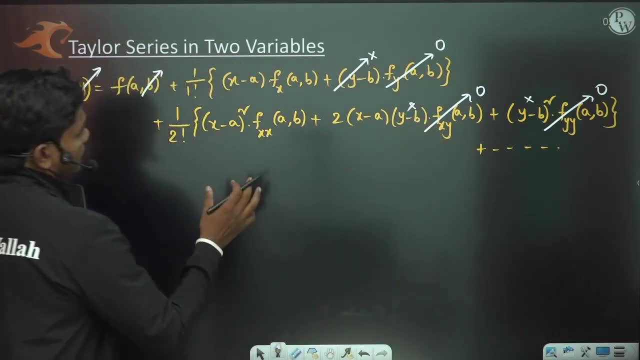 So all these terms, they go to 0 and of course, these terms don't have any. You know existence, because we are dealing the changes only in x direction. Okay, so like this, if you see, if you keep on deleting the terms where there is involvement of y coordinate, 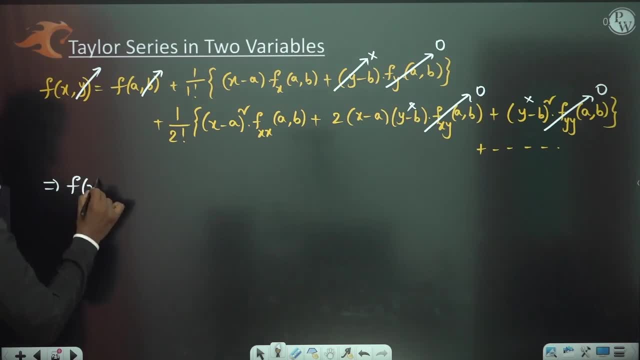 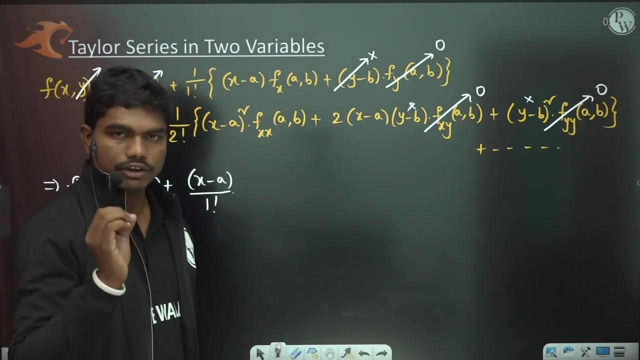 Then you will end up with the series: f of x is equal to f of a plus x minus a by 1 factorial x minus a by 1 factorial Into. now this is partial differentiation of f. now, whenever f is only function of x, if you differentiate it, 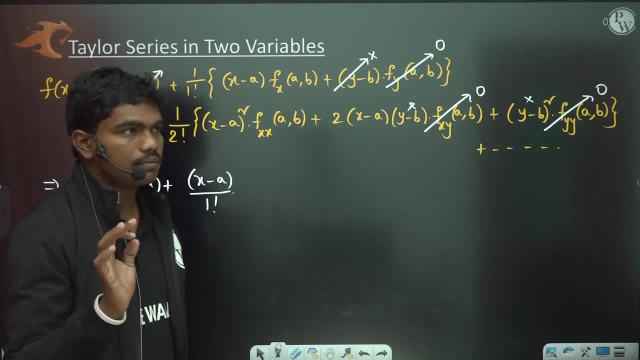 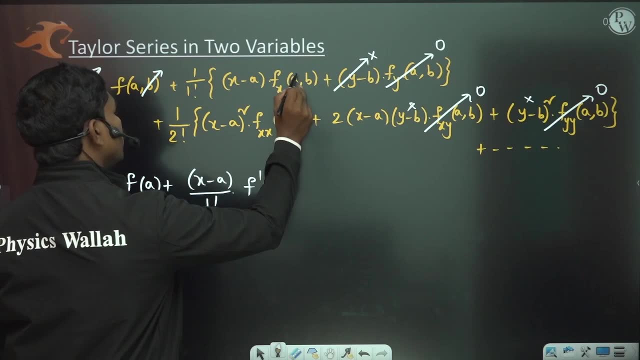 Partially, or if you differentiate it exactly, then you will get the same result. So if you see this, fx is Nothing but f. dash at the point, x, equal to a because there is no point of B here. Okay, so this B won't be there. Okay, so you have a. so this term got finished, plus coming to this term, x, minus a whole. 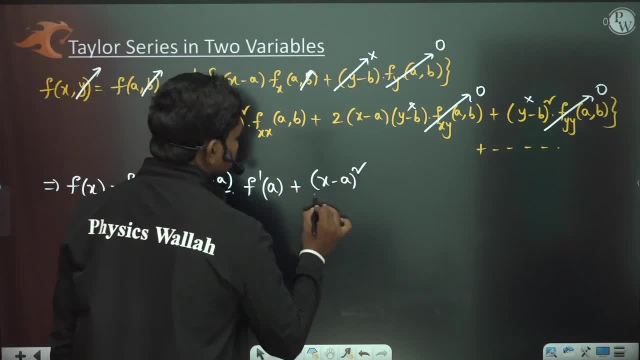 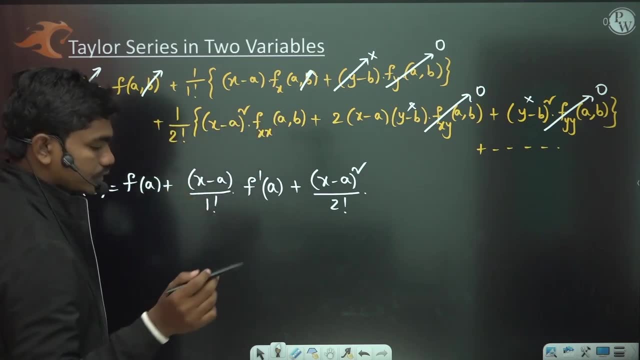 square by 2 factorial, x minus a whole square by 2 factorial multiplied by now. if you see, this Is doh square, f by doh x square. So whenever f is again some function of x, partial differential, differentiating it two times with respect to x or doing the normal integration. 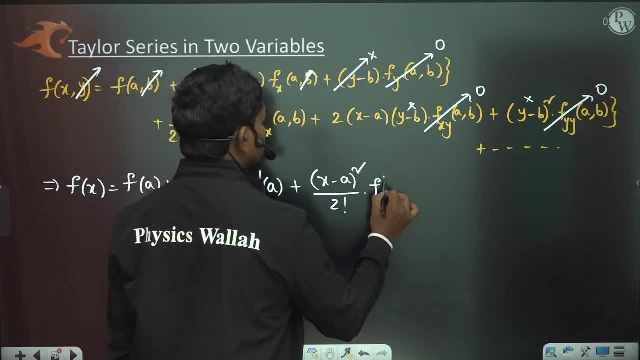 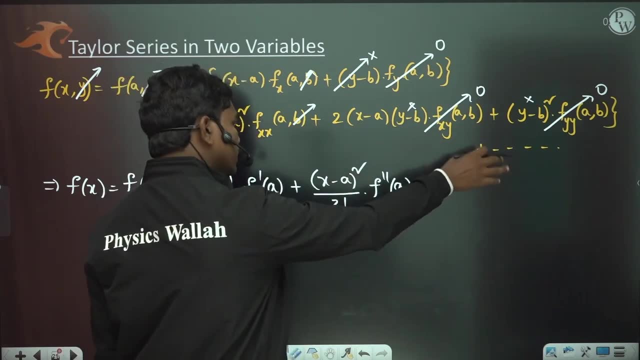 Both give you the same result. So that's why you have f, double dash of a, because there is only one Variable you can substitute for. okay, These two terms are 0. So if you are consider the third term, you would have got something like x minus a whole cube by 3 factorial. 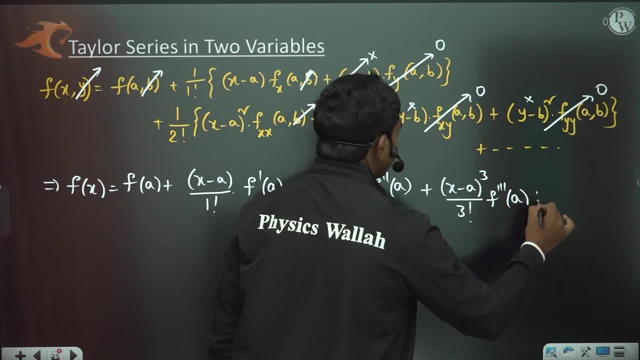 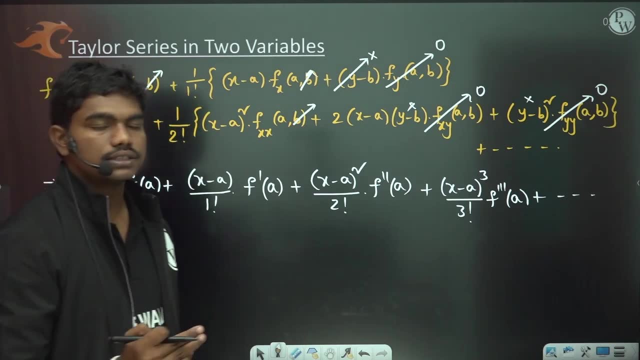 Times f, double dash of a and so on. This is will actually go on and that's how this Taylor series expansion is actually reduced from this second variable. Okay, and actually Taylor has given this expansion for any number of variables actually, and it has taken n dimensions in general and 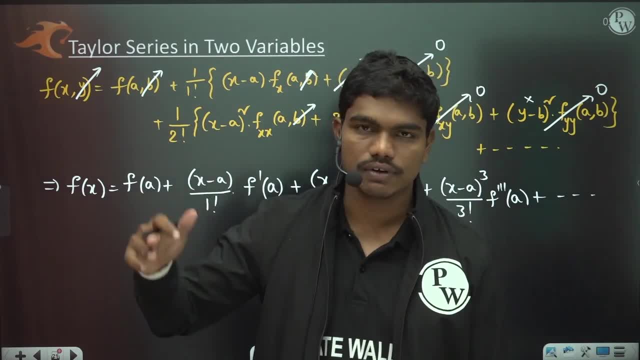 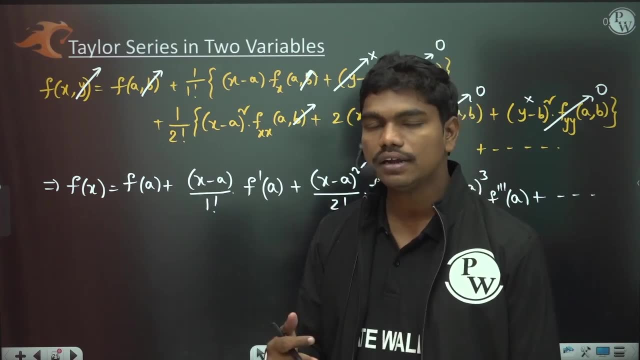 He has given in terms of I notations actually Okay. So Sigma i is equal to 1 to n in such a form, but at the right now It's going to be more complicated. and also in the syllabus you have only for single and multiple. I am in single under this. two variables actually okay. but 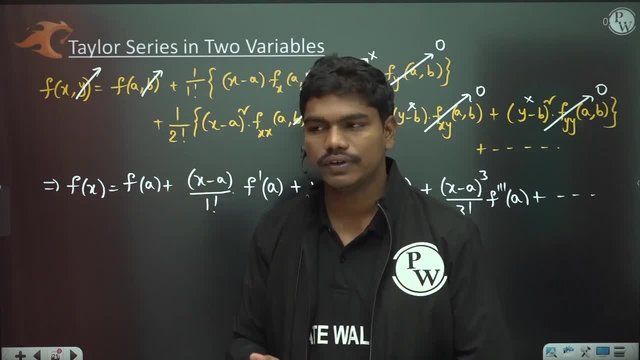 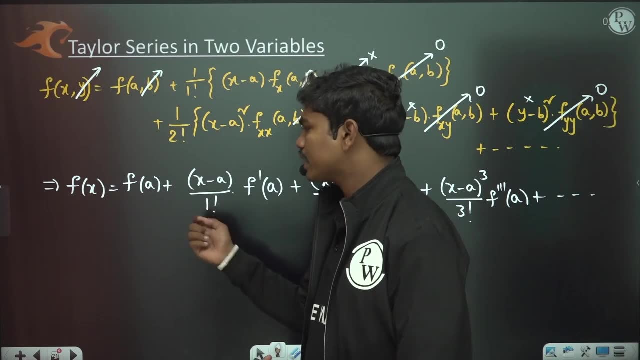 Majority, if you see this, two variables is not asked, even you know, hardly once in last 10 years. So that's why, but still it's in syllabus, So we shouldn't take any risk. That's why I have taken, given you this Taylor series expansion in two variables and of course it's simple, just 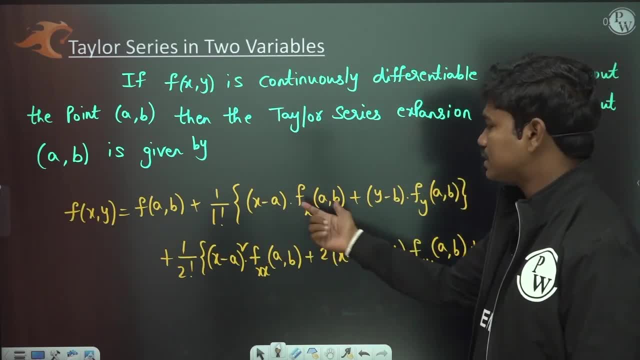 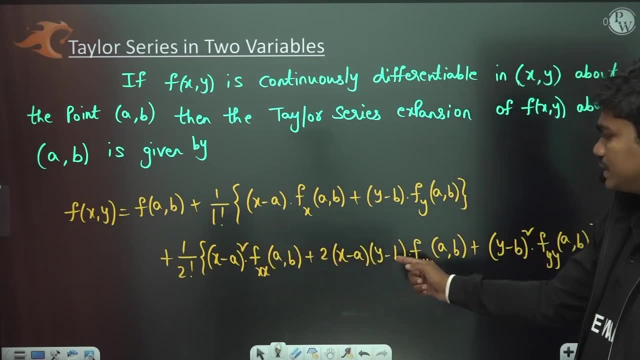 See, writing this cyclic terms is very easy. So first you have it in the linear terms, then it's like a plus B, whole square, expansion kind of thing. Okay, So if you see, we'll write the square of this two times, of X minus a into Y minus B and Y minus B whole square. 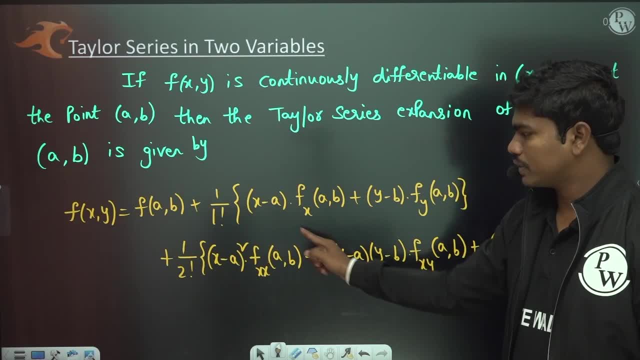 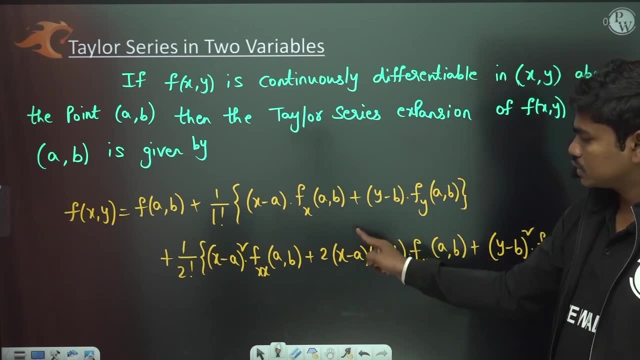 So the coefficients changing as partial derivatives with respect to XX, both. The complete degree of 2 is due to this X, So we have it in XX. the complete degree of 2 is because of 1 X and 1 way, So we have it in XY. the complete degree of 2 is because of this way, So we have it in Y way. 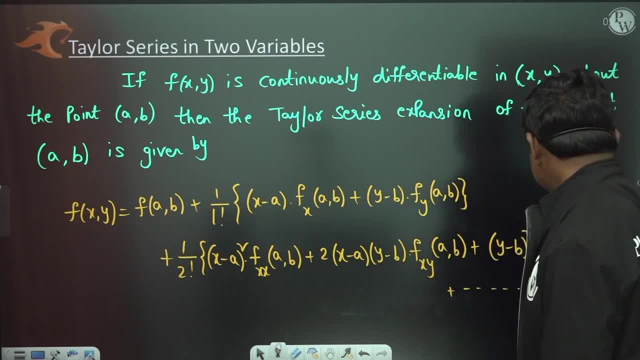 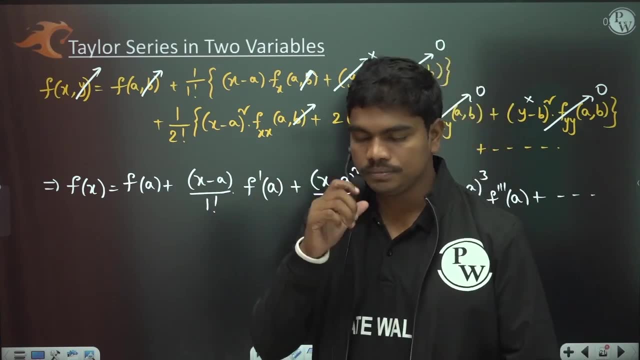 So this is how we have it in the coefficients generally and Coefficient generally, and this is how we have detected the single variable, Taylor series expansion from the two variable, From the two variables that are existing here. Okay, so I hope it's clear to you. 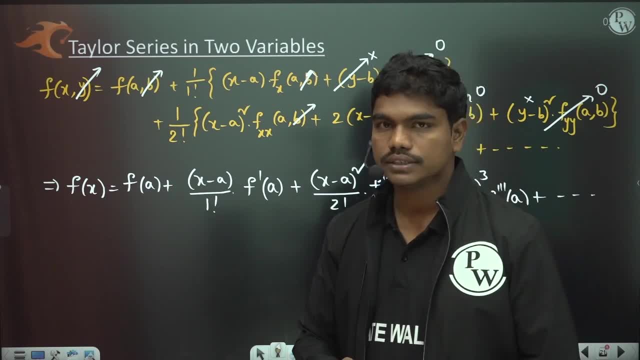 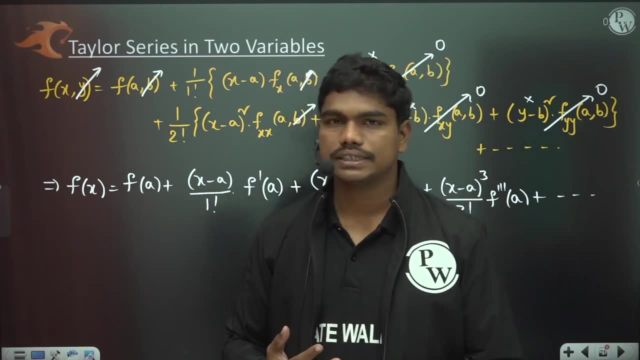 And this is how we basically deal in the case of Taylor series. Okay, so once we are done with this Taylor series, We are almost finished with this differential part of the basic calculus. Okay, Now let us shift for the integrations of This two, three variables actually. okay, so let us go for the multi variable integration. Okay. 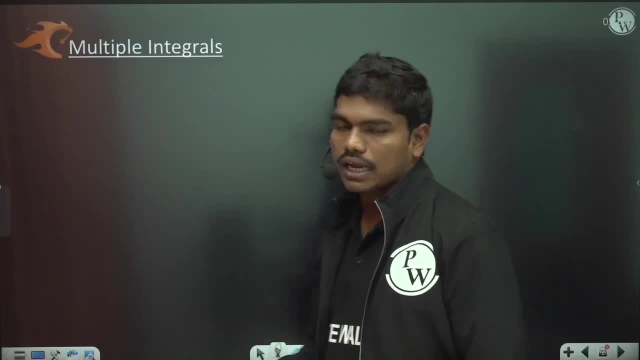 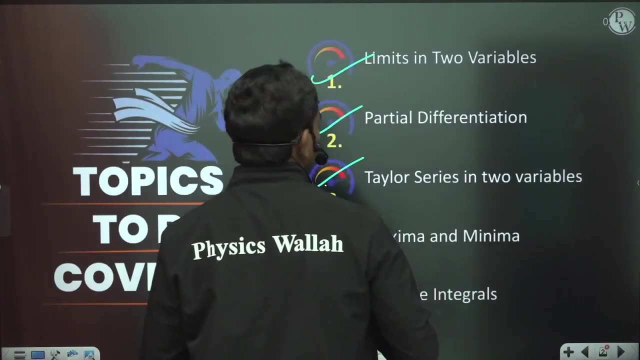 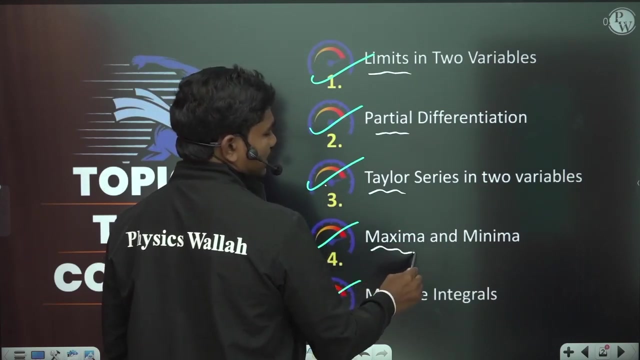 So now let us see how do we do this. multiple integrals, the last module which I have actually, you know, going to cover in this syllabus, but So we have seen these first four things. limits in two variables. We have understood partial differentiation. We have since spent some time on that Taylor series, of course, after doing the concept of maximum enema. 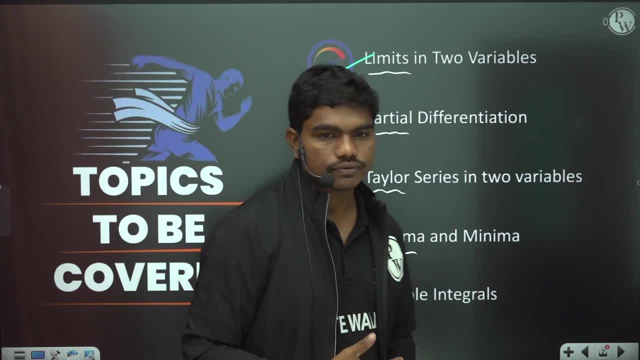 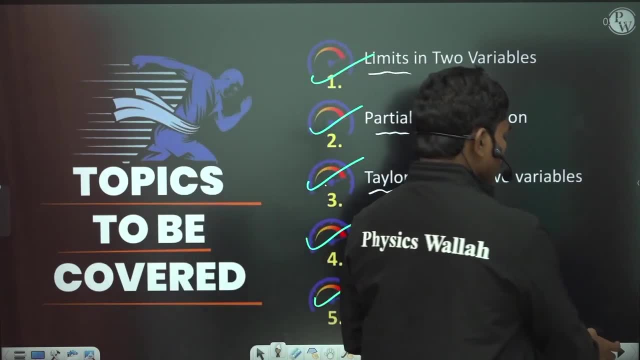 We have talked about Taylor series. Okay, in two variables. Okay, so this for you know more, what is a section We have covered? and the last section that is left over in this case is multiple integrals. Okay, and you see, I told you in last class also. 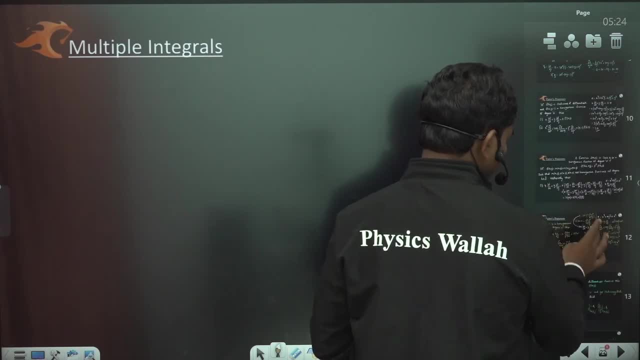 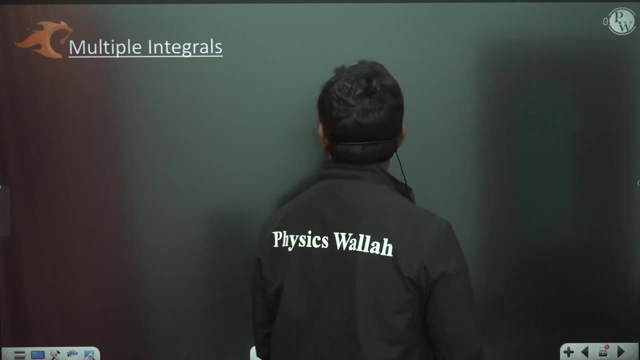 Just a minute so let me forward this. So if you see, okay, so multiple integrals, So multiple integrals is actually taken as one of the very hard topics. actually, if you see, because generally what happens till plus 1, plus 2? Level, you are very much familiar with the single variable integration. 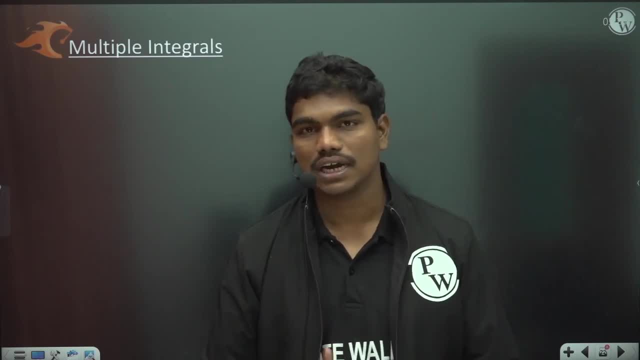 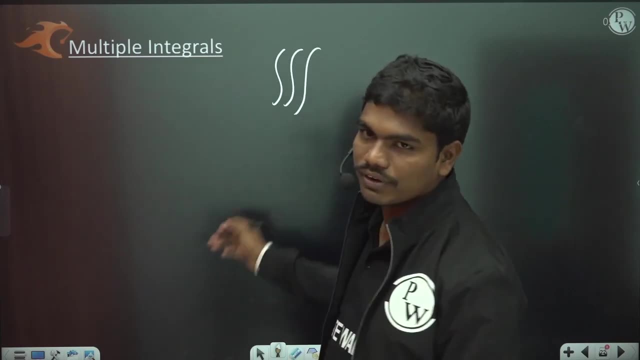 But after that, what happens? suddenly you come to the beta, first year, and data start talking about multiple integrals. They put symbols like this, They put symbols like this, which will cause some fear in you, and all this Okay, but actually, practically speaking, these things are very easy. 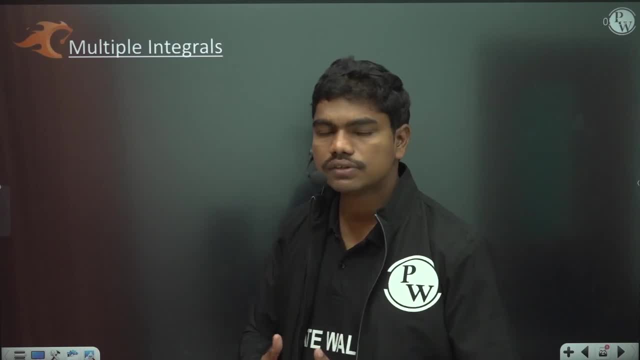 Okay, if you have slight idea on what to do, if these things are very much easy for you, Okay, so how we actually define a multiple integral letters, Let me show you first the double integral, then we'll, if there is some space, We'll go for it. Okay, so let me show you first the double integral, then we'll, if there is some space, we'll go for. 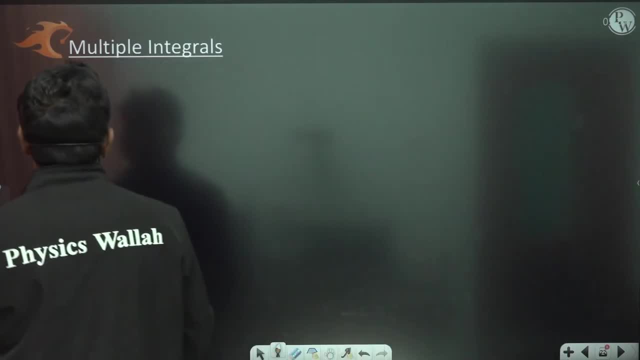 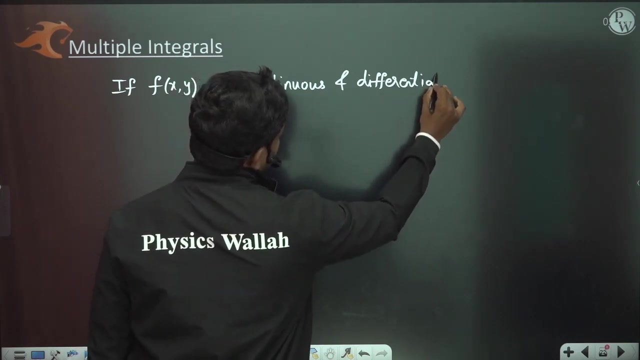 triple integrals also. okay. so now let us see here multiple integrals, How we'll do this. Okay, so if F of X, Y is Continuous and a differentiable, Continuous and Differentiable In a region of continuous and a differentiable in 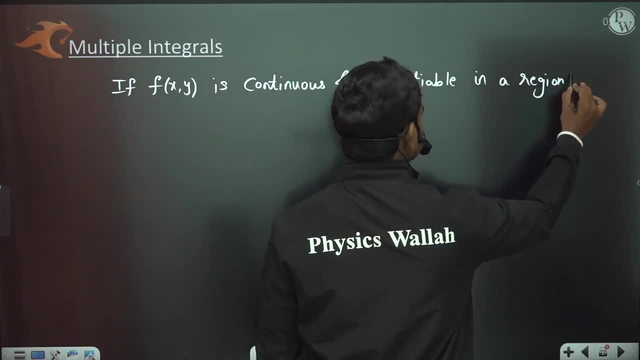 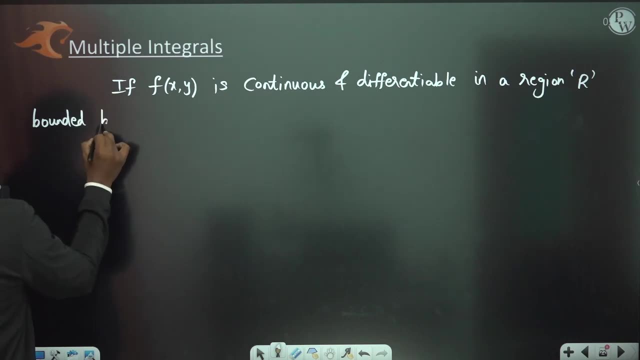 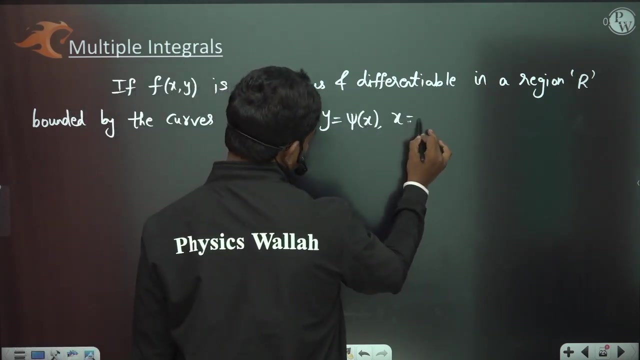 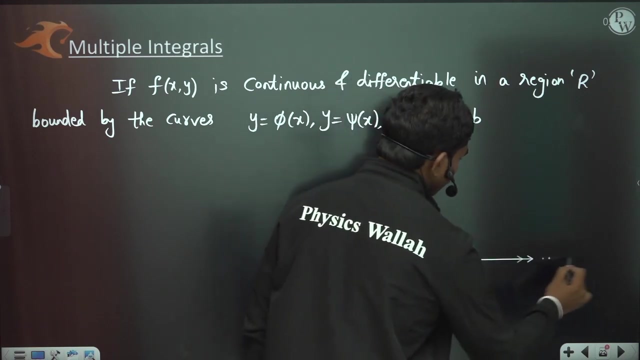 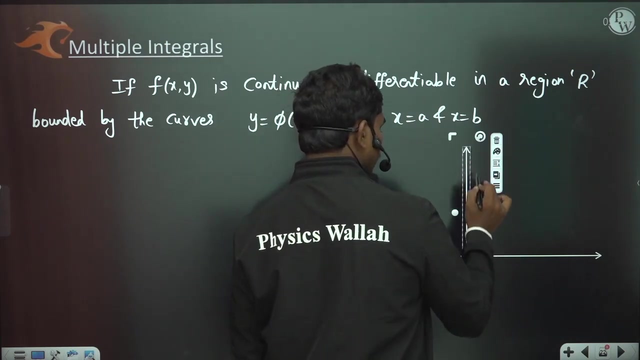 a, a, vgn are bounded by bounded by the curves. bounded by the curves, say, for example: y is equal to phi of x, y is equal to psi of x, x is equal to a and x is equal to b. so let us take a 2d space. if you take a 2d space, if you take a 2d space like this, for example: 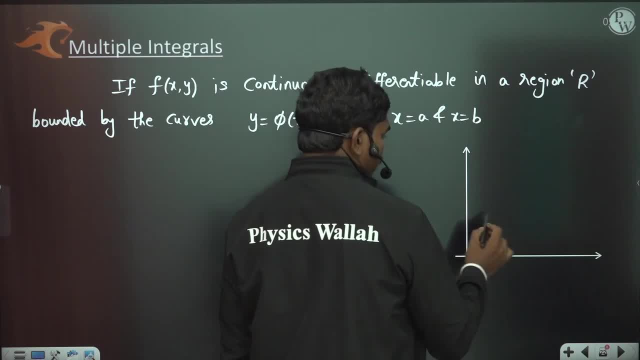 now try to calculate something. if this is some function, say y is equal to phi of x, for example. okay, so y is equal to some phi of x is one function. and let us say y is equal to psi of x is some other function like this, for example, something like this: okay, so let 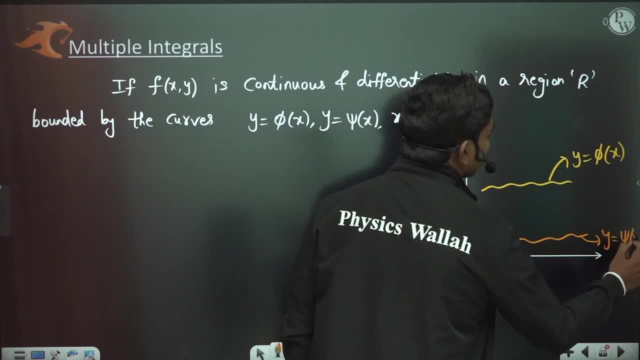 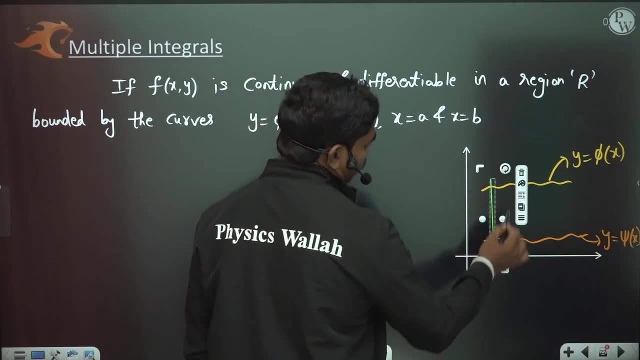 us suppose it is lying somewhere here- y is equal to psi of x, x, y is equal to psi of x and x is equal to a and x is equal to b. are these lines: this is x is equal to a, for example, and this is x is equal to b. okay, so this is x is equal. 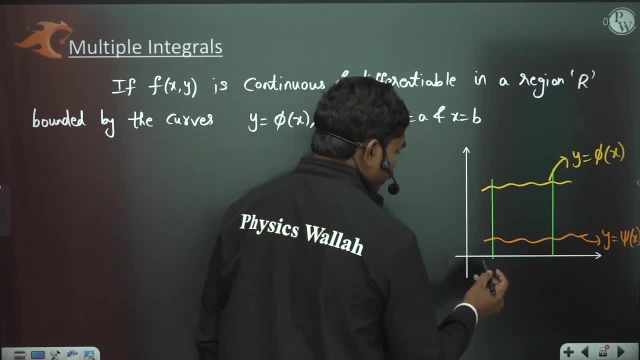 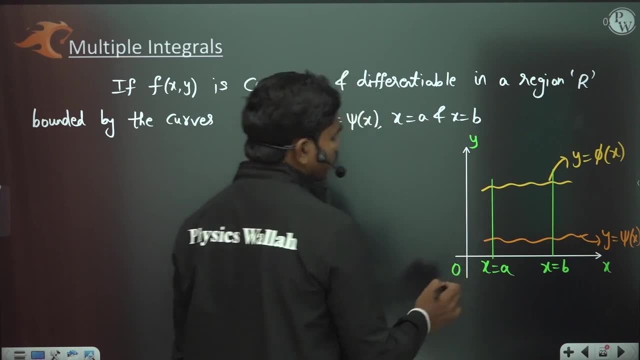 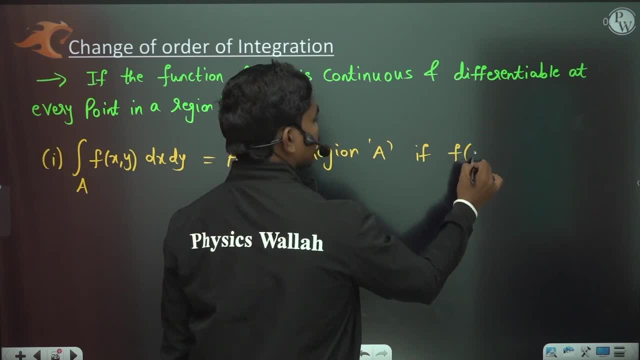 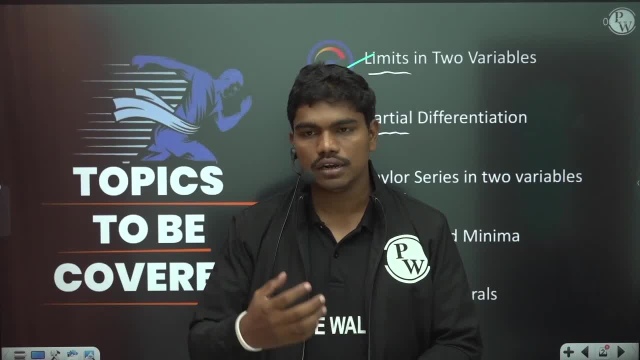 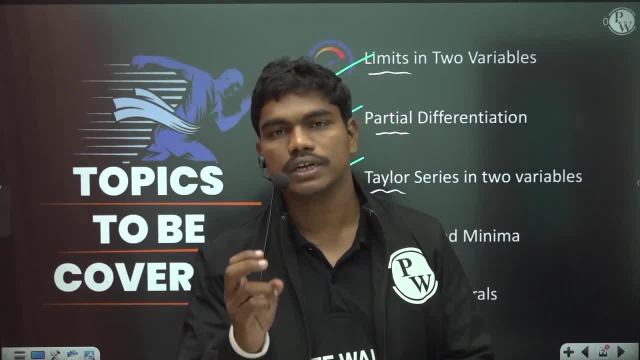 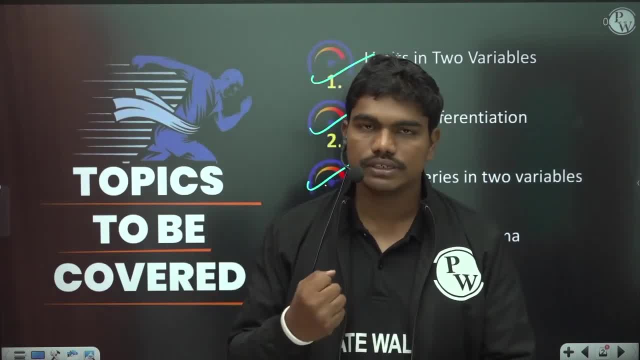 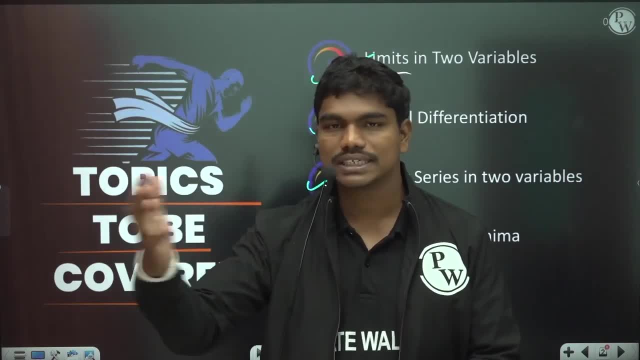 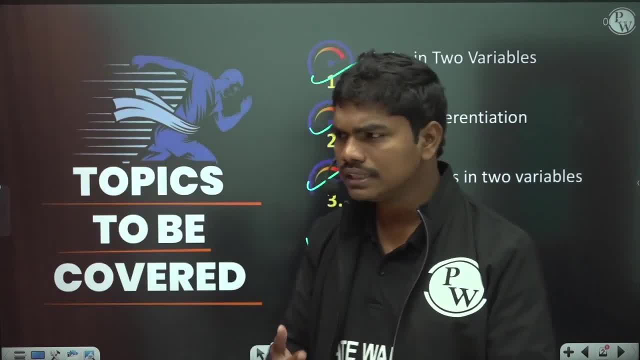 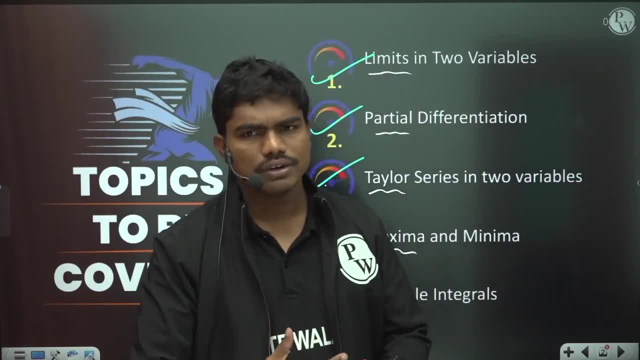 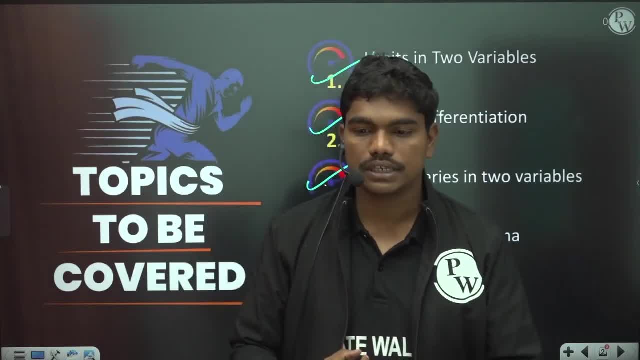 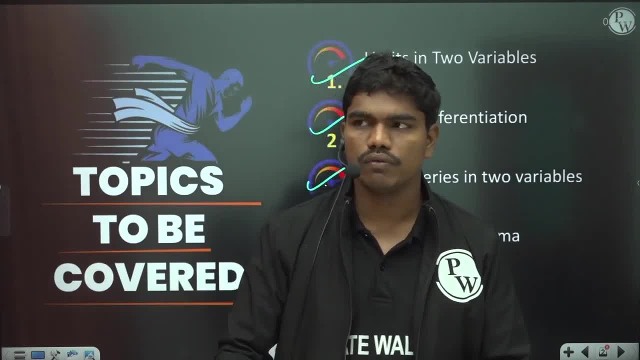 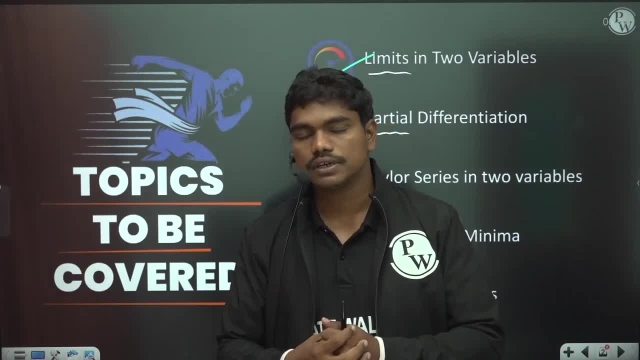 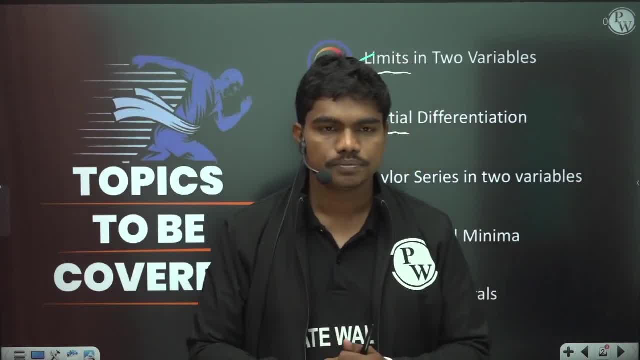 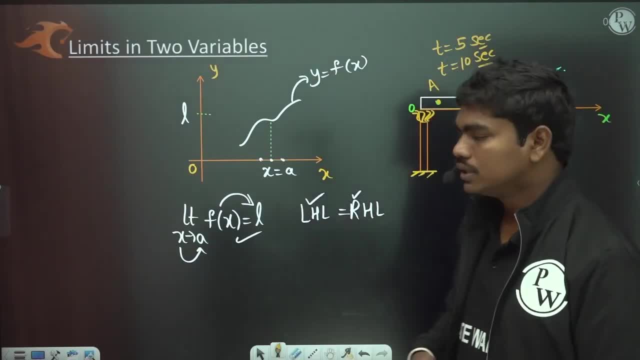 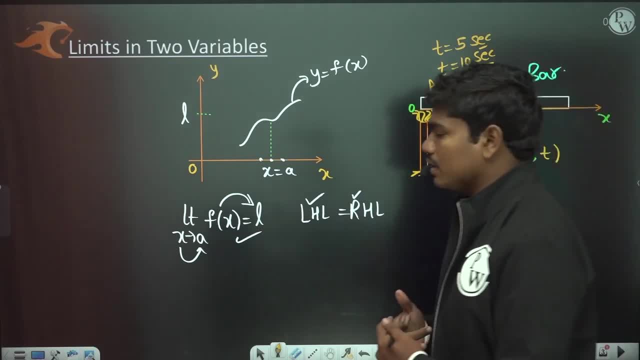 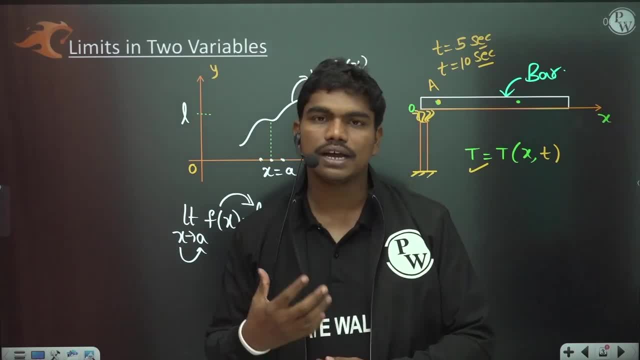 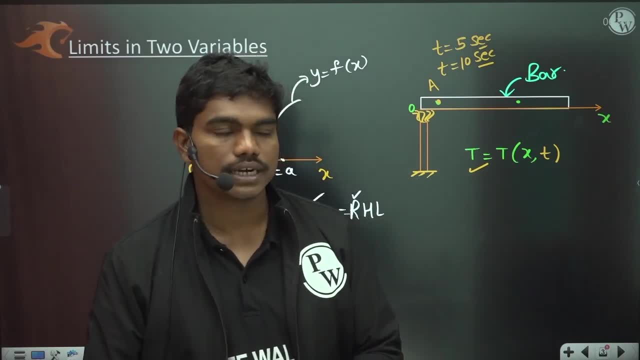 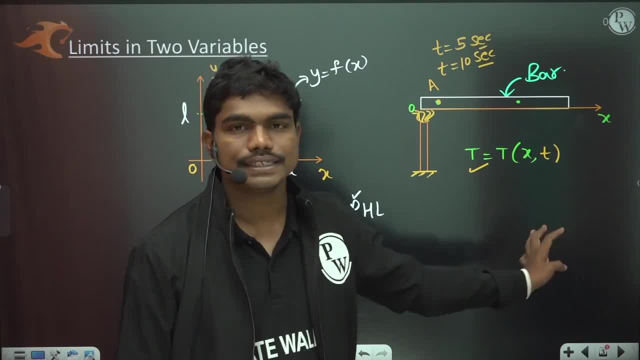 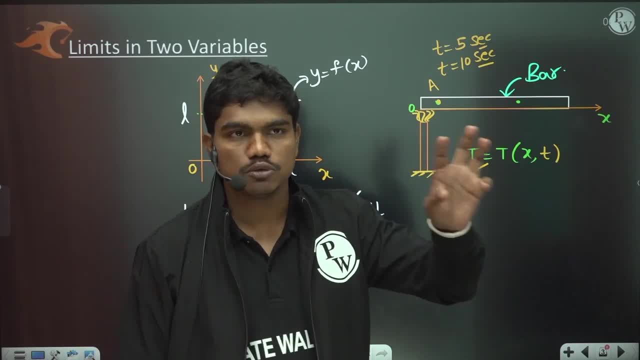 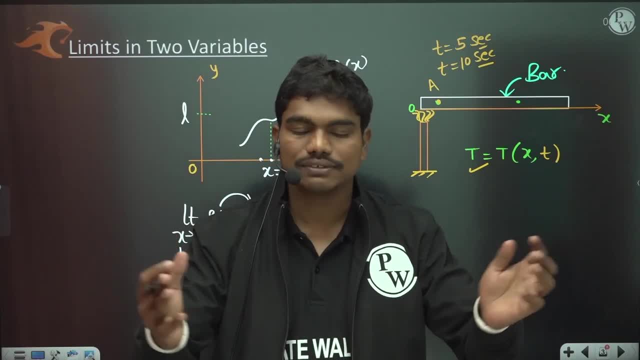 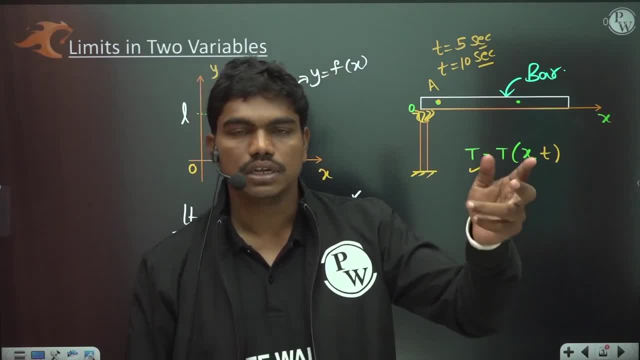 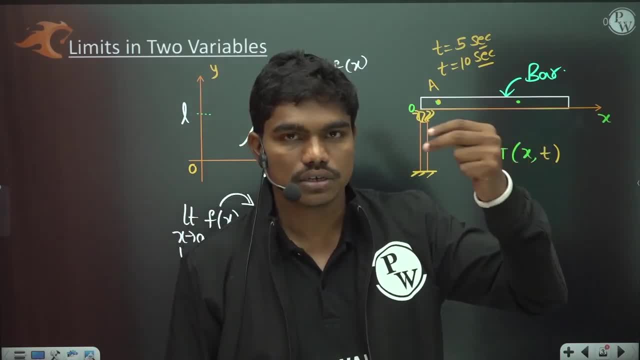 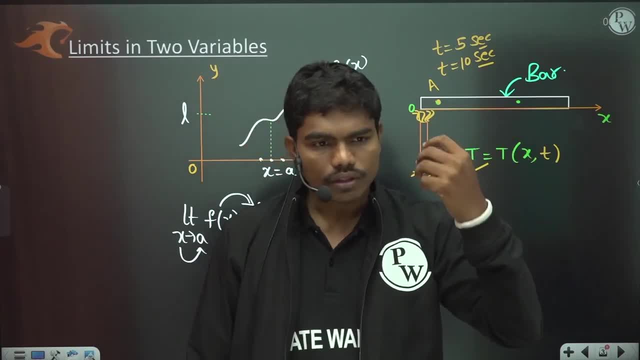 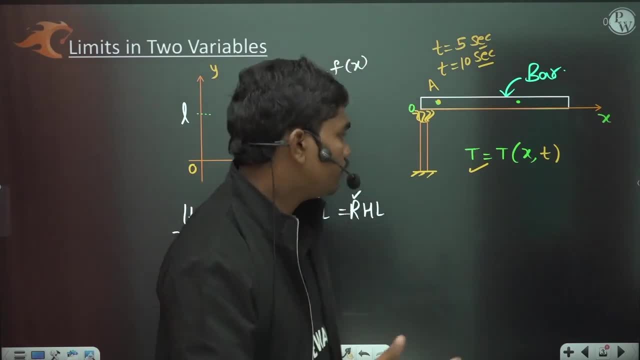 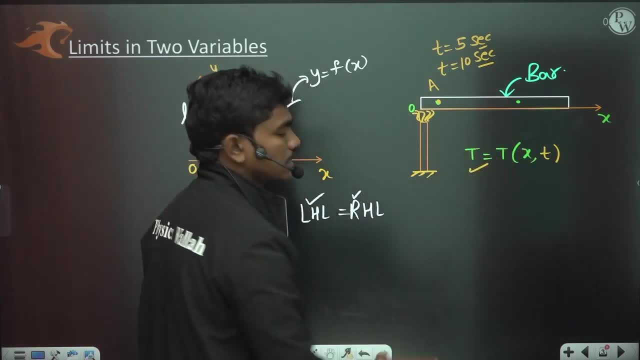 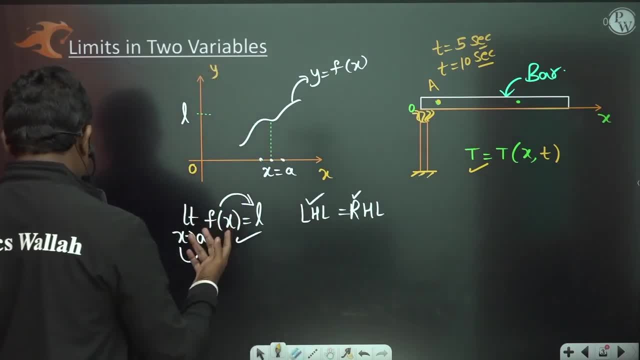 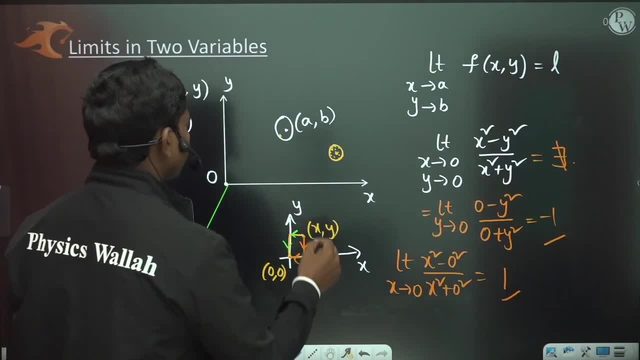 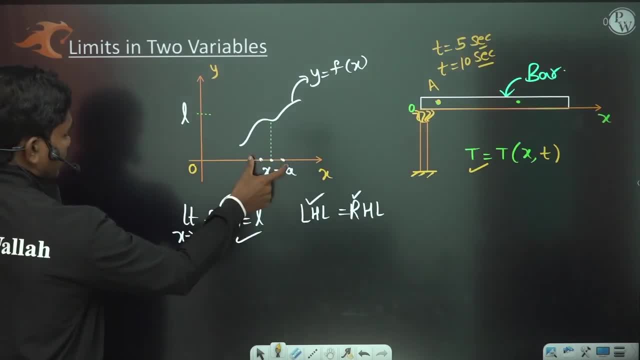 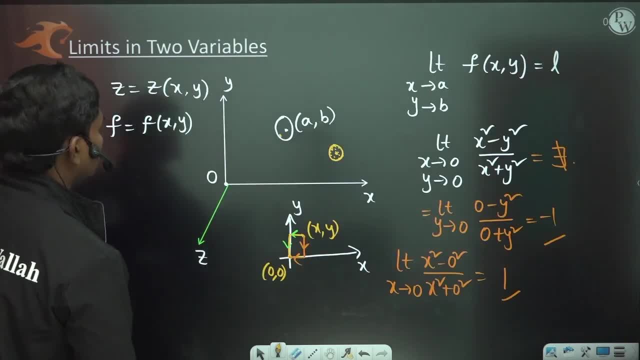 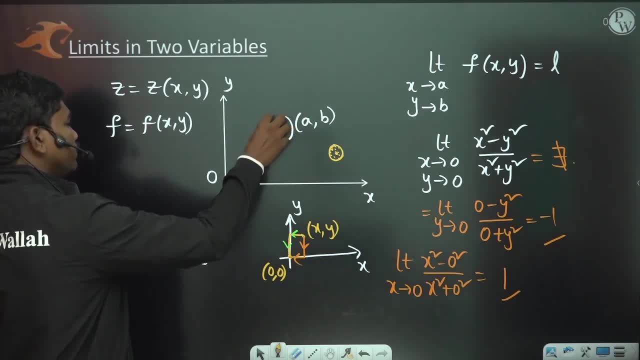 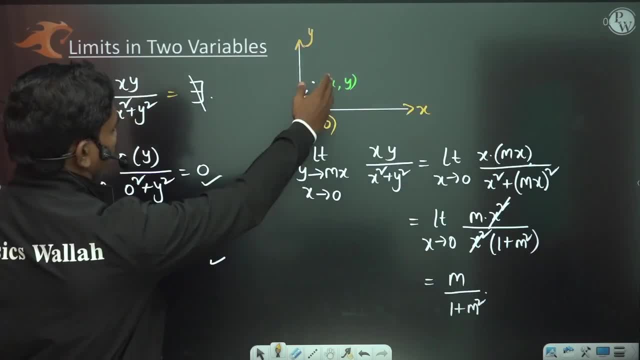 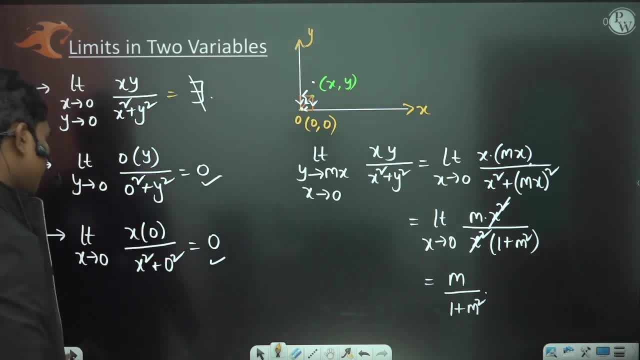 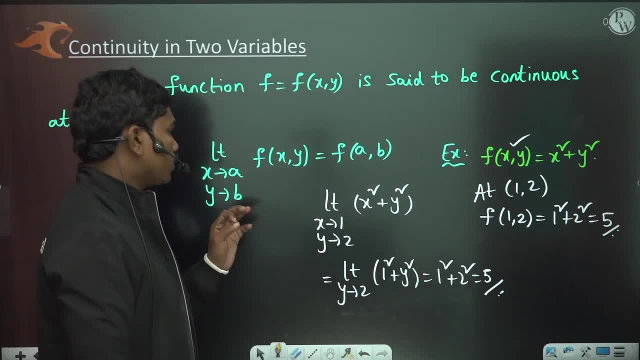 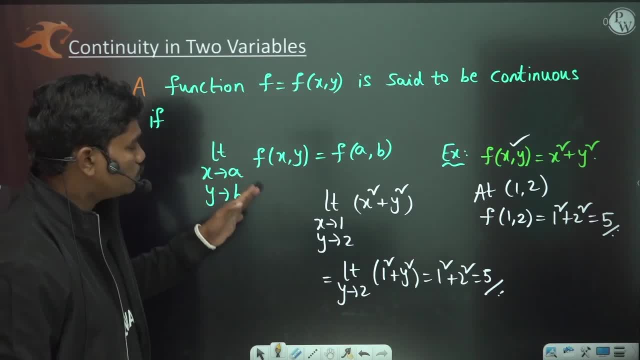 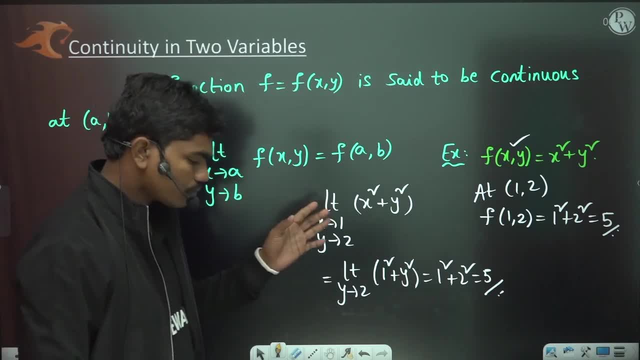 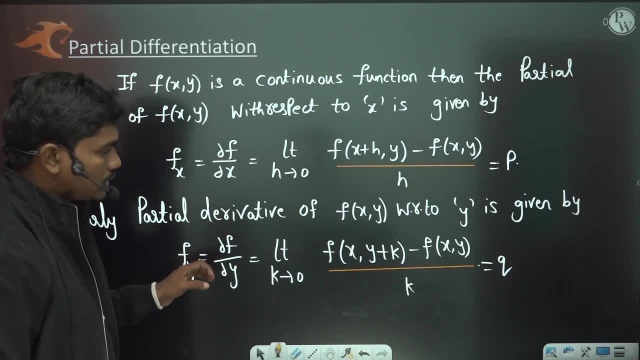 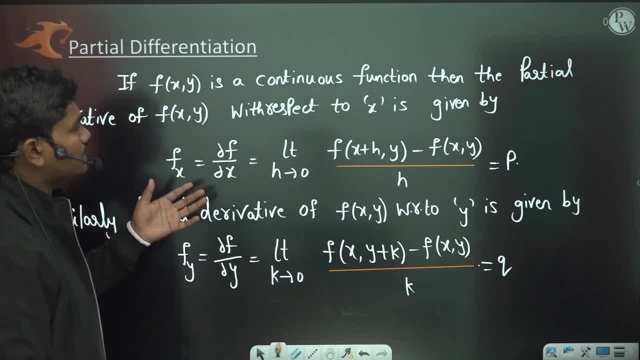 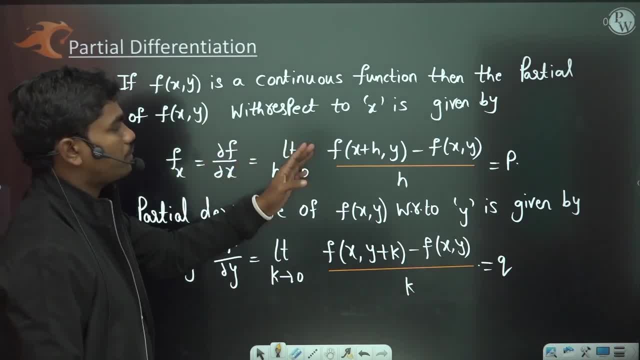 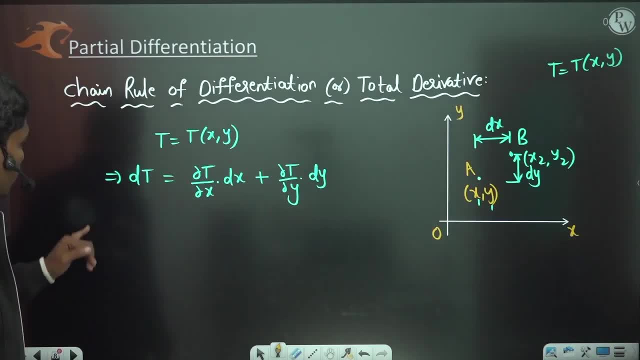 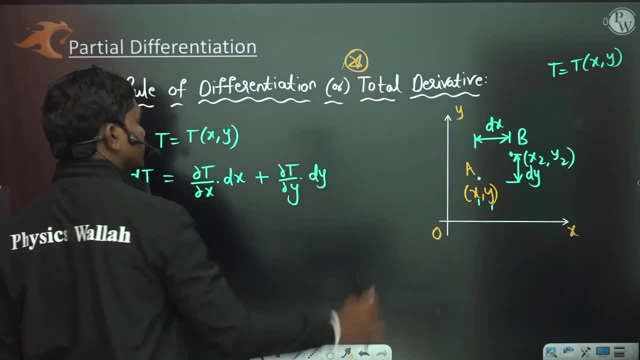 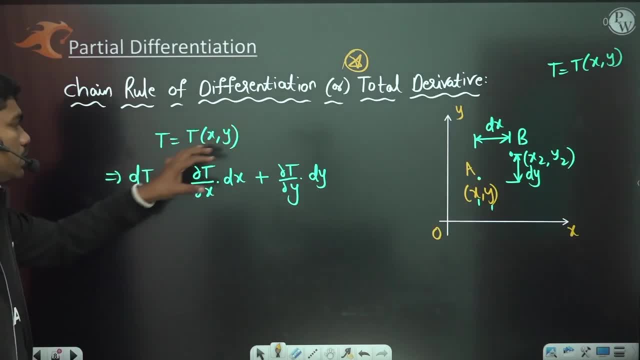 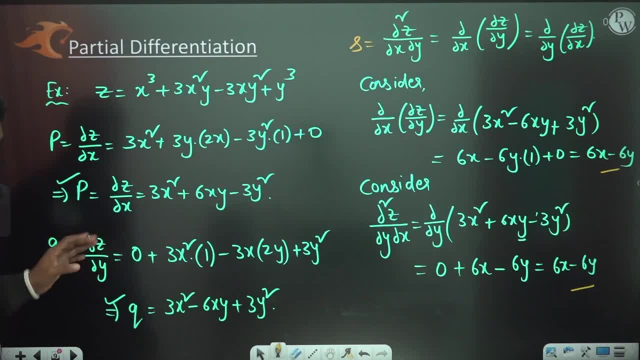 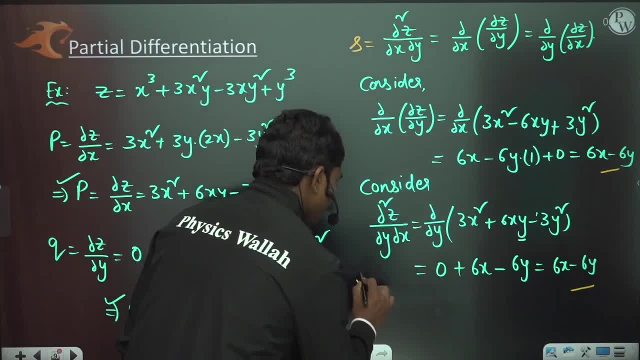 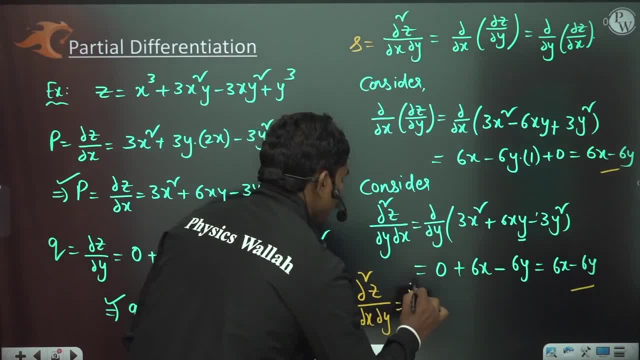 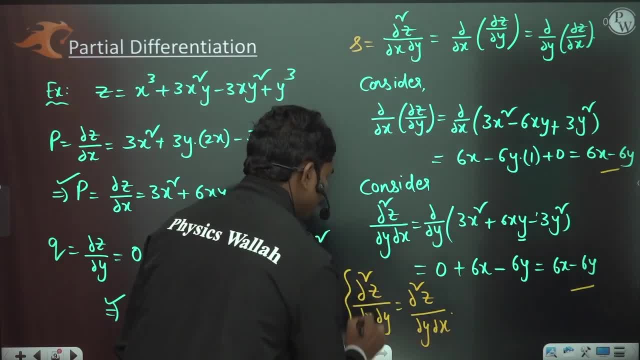 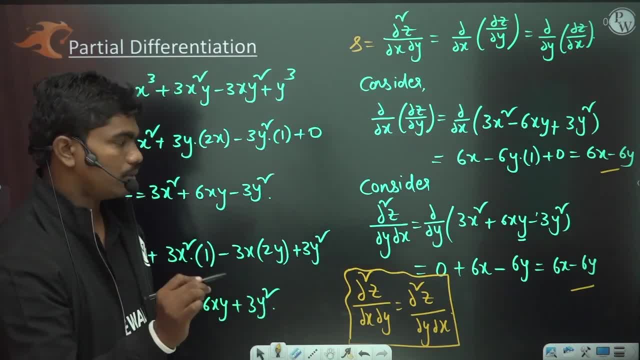 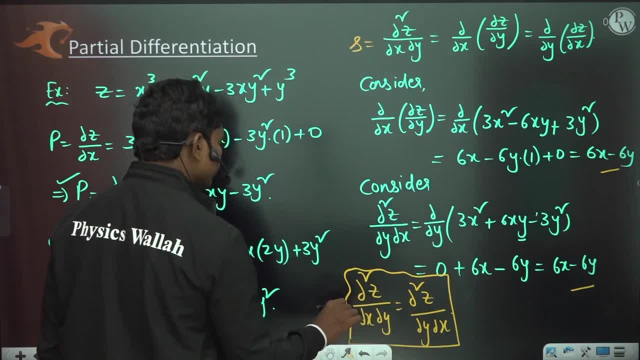 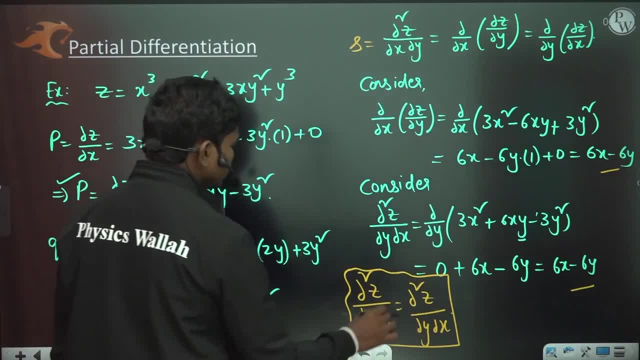 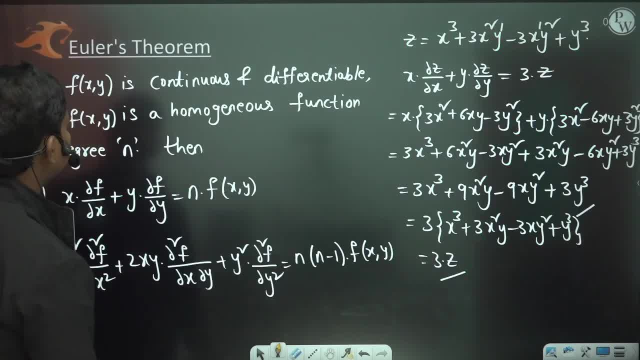 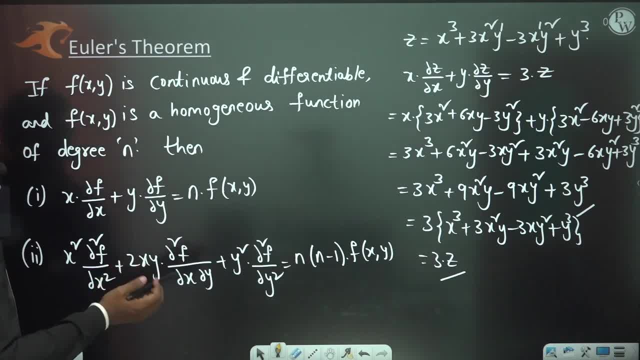 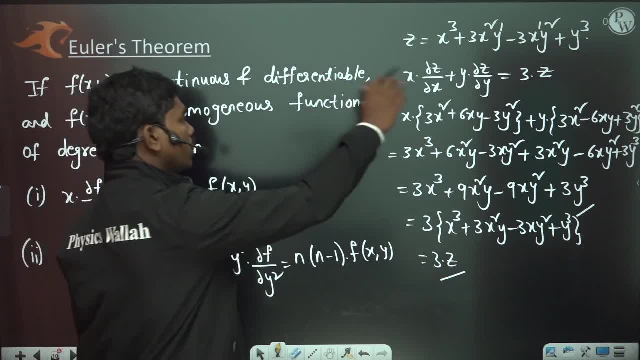 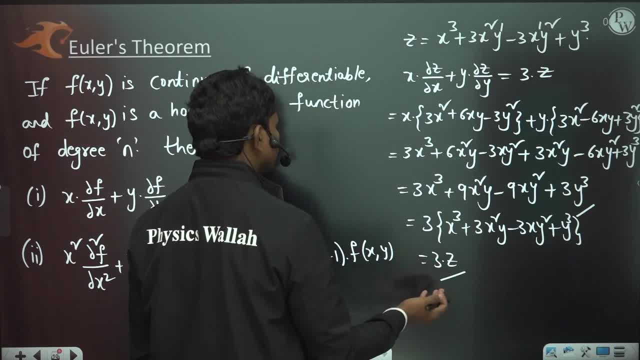 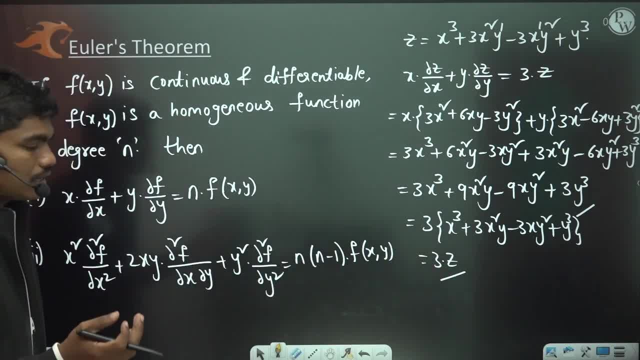 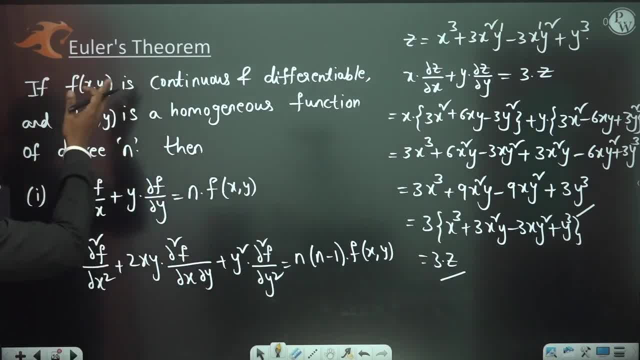 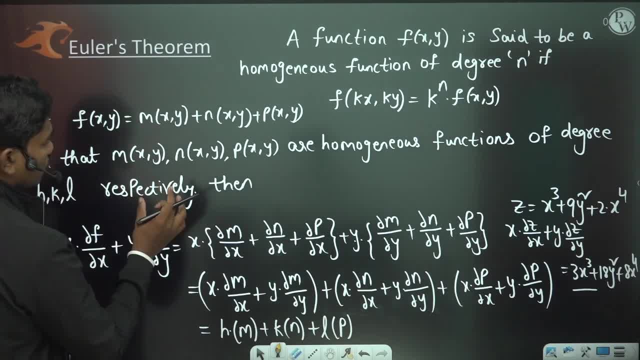 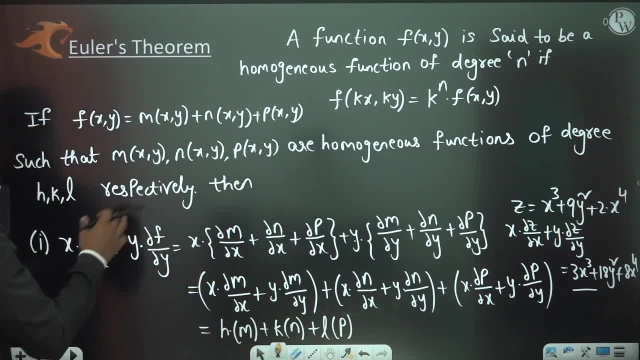 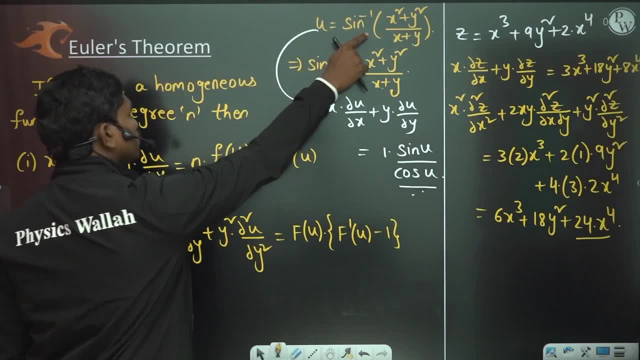 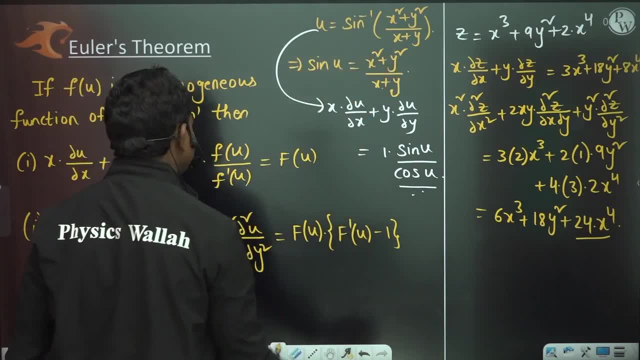 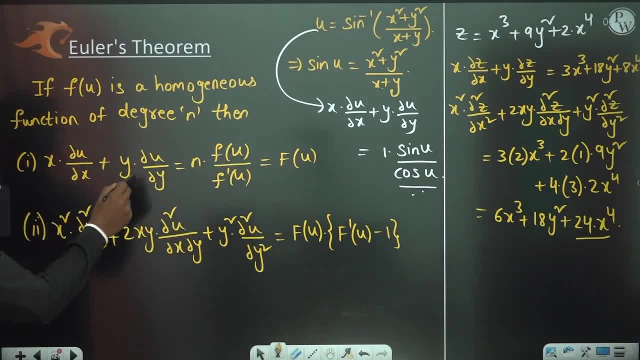 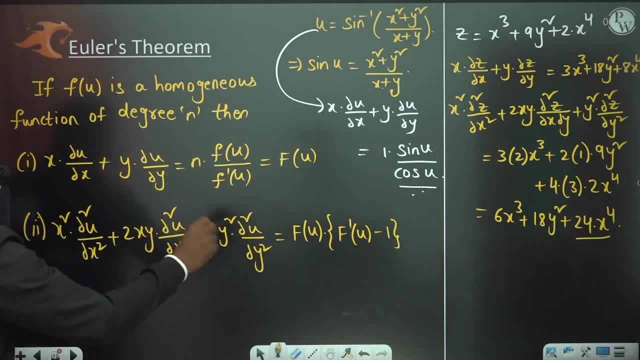 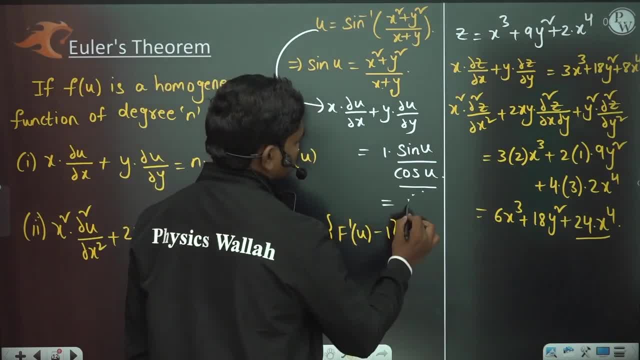 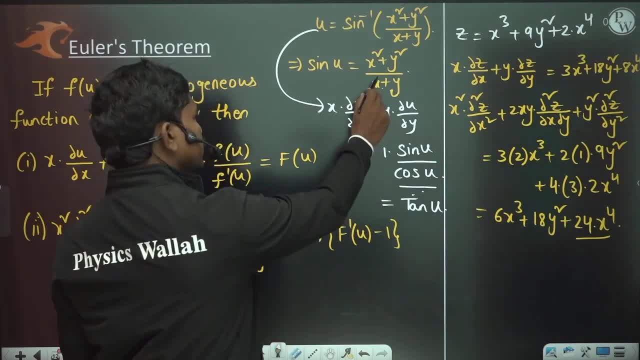 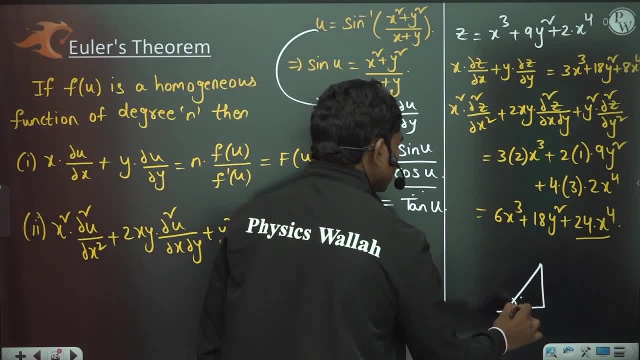 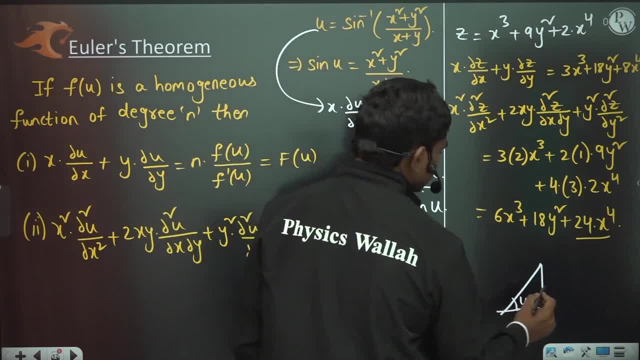 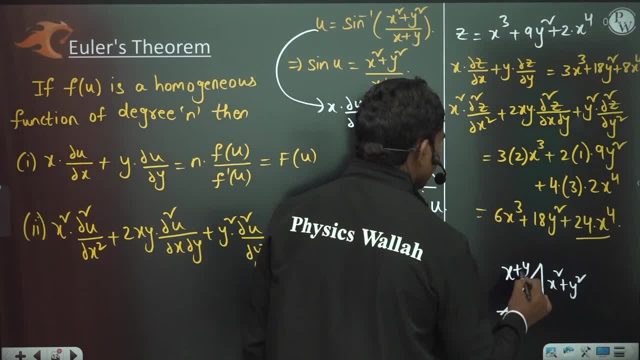 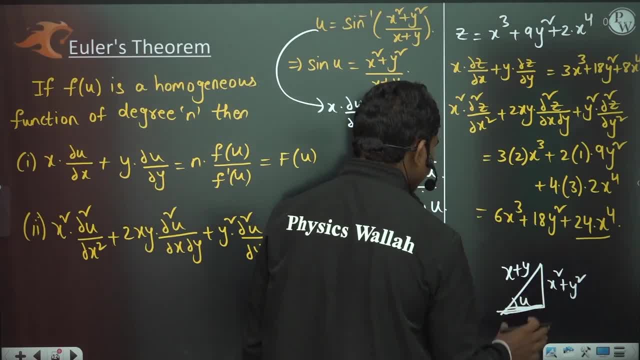 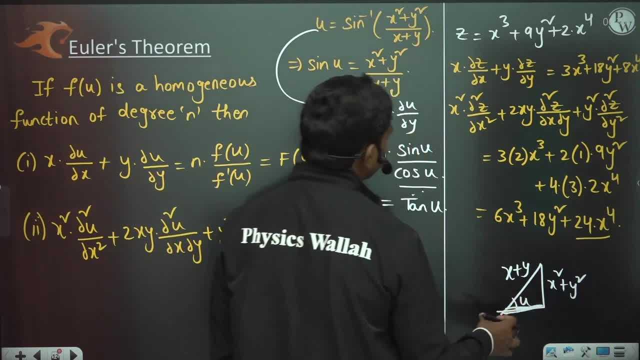 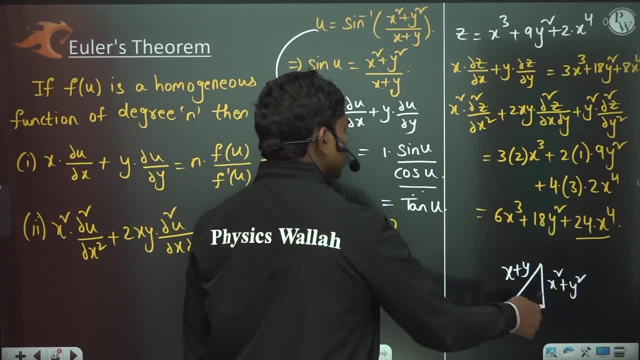 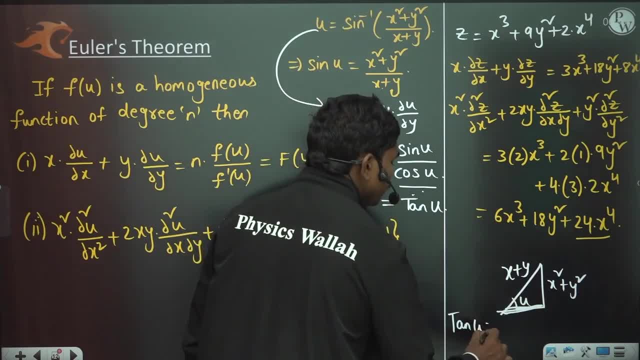 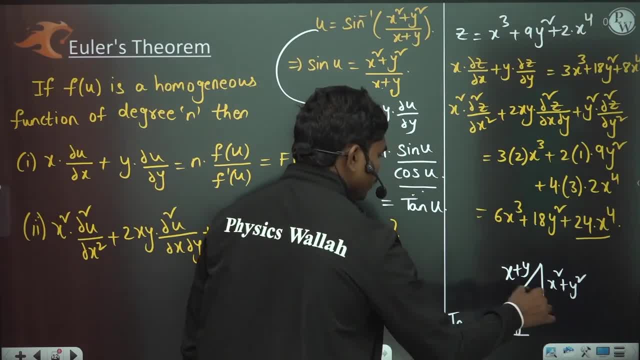 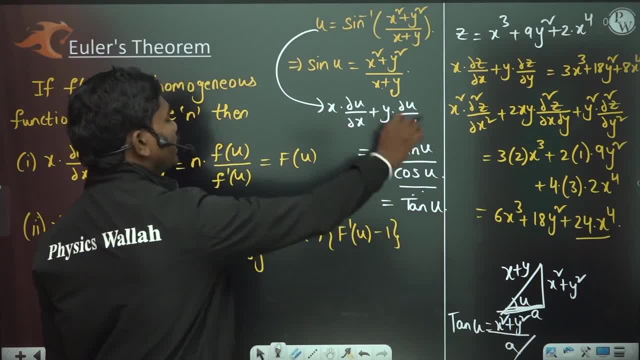 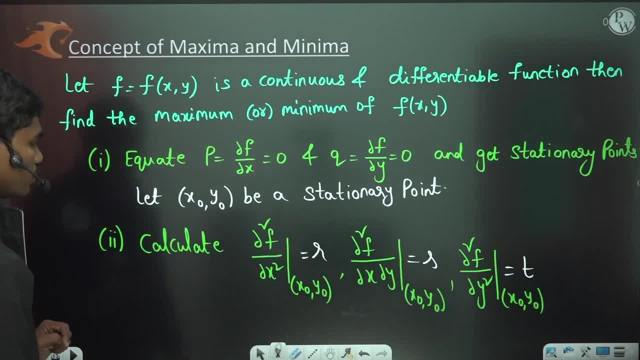 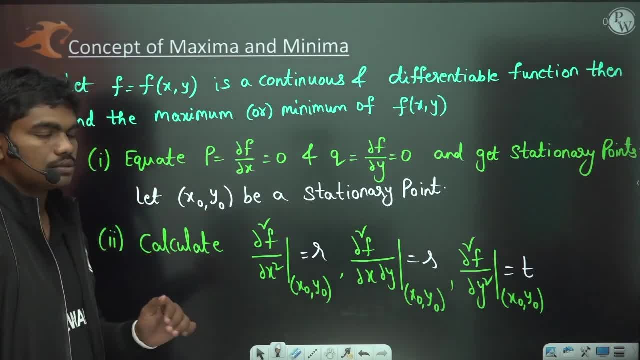 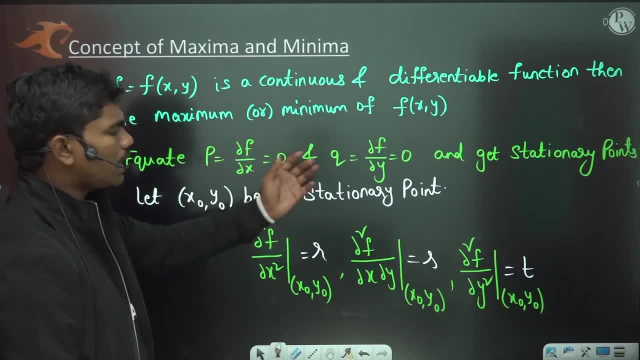 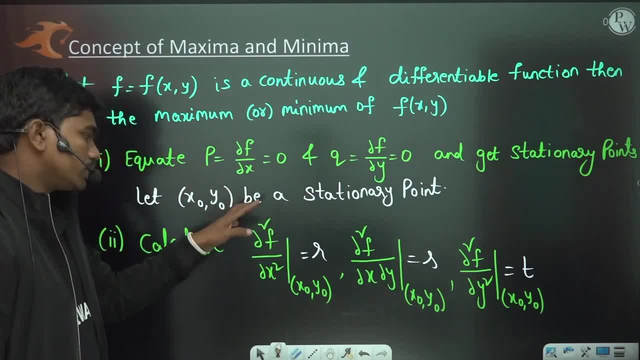 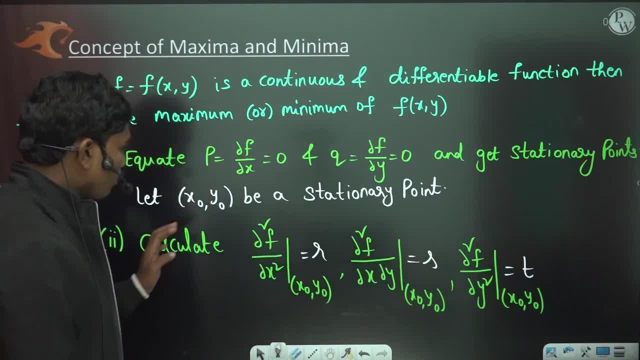 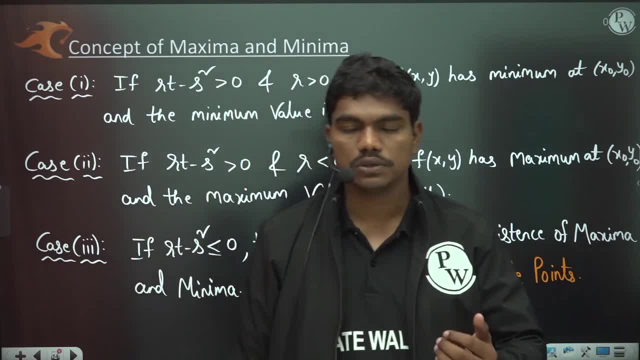 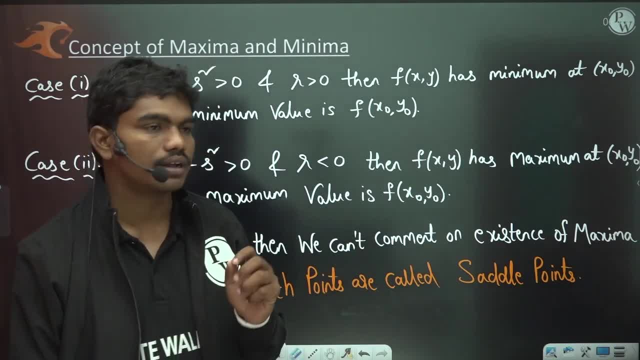 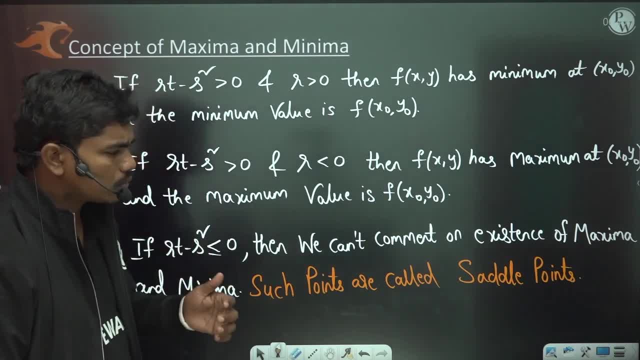 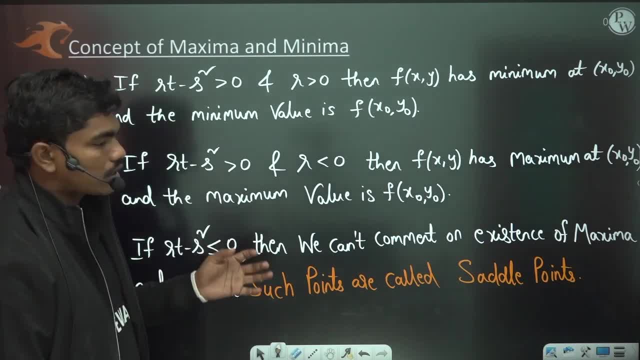 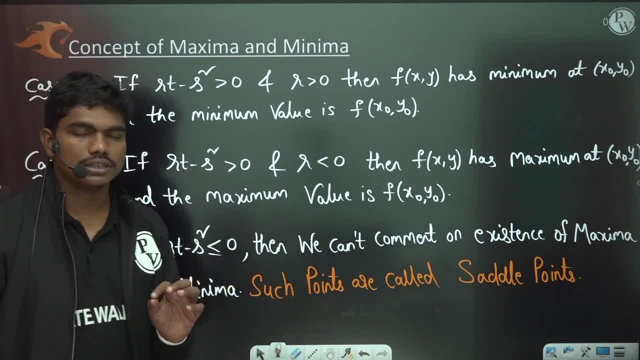 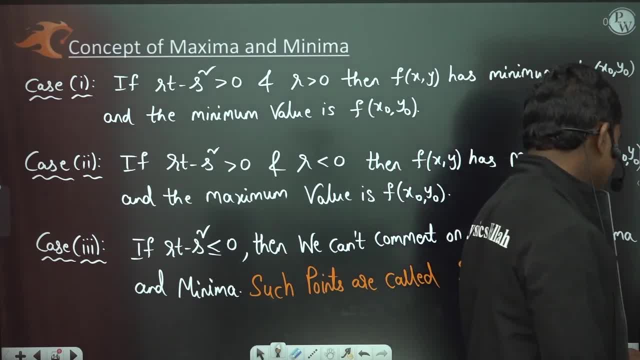 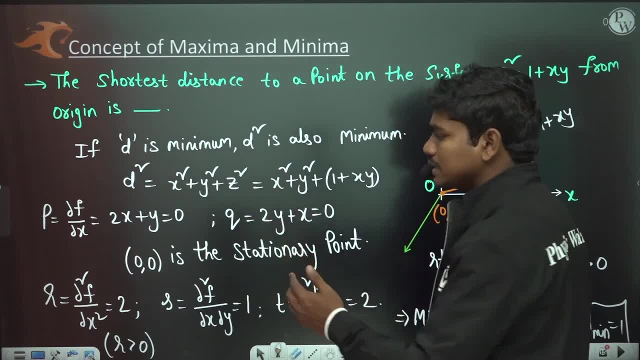 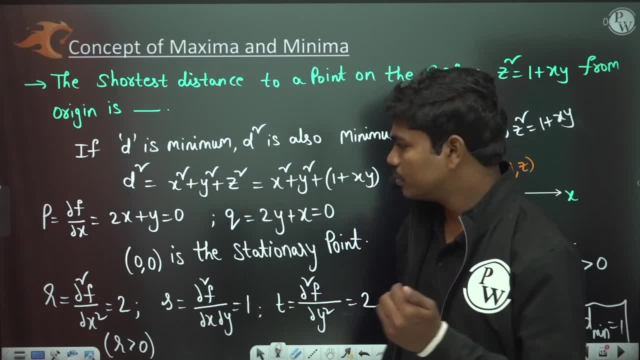 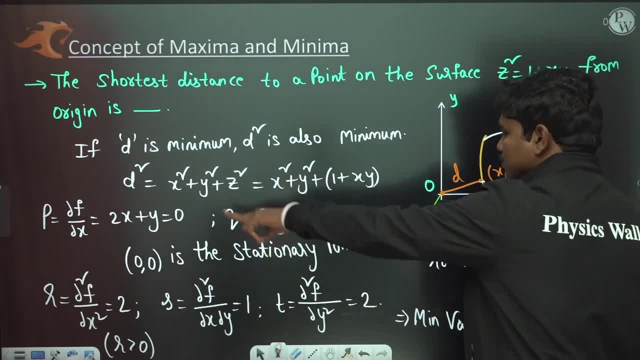 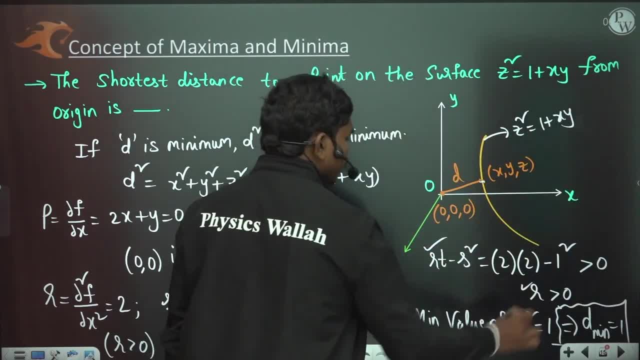 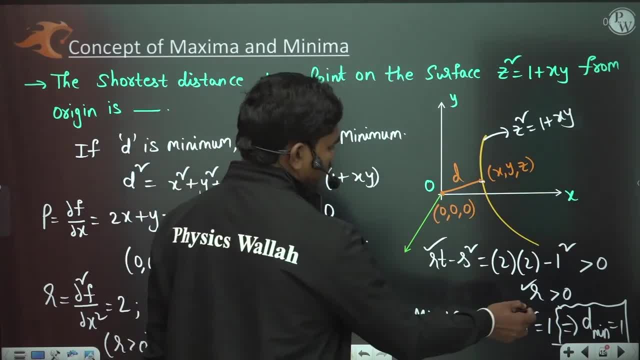 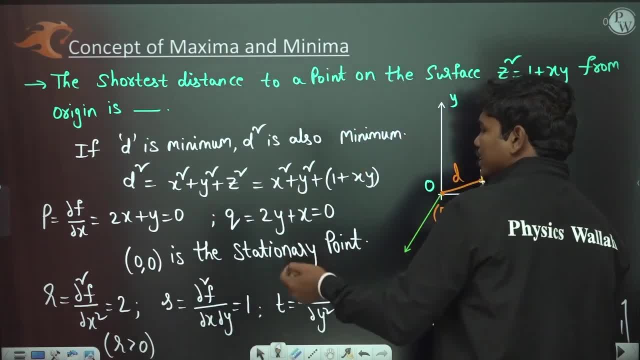 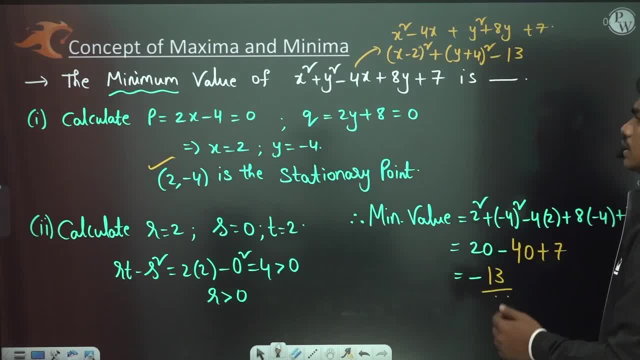 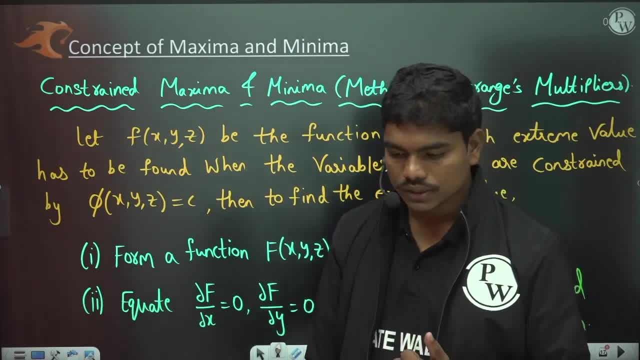 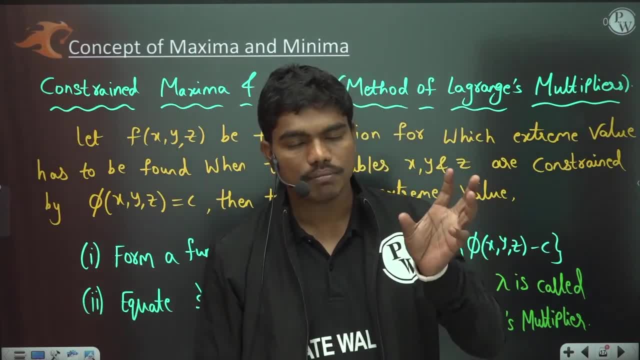 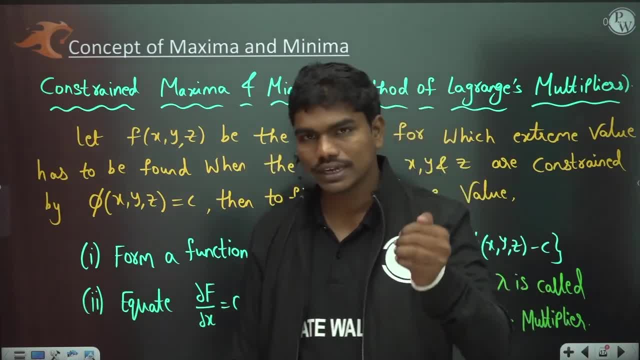 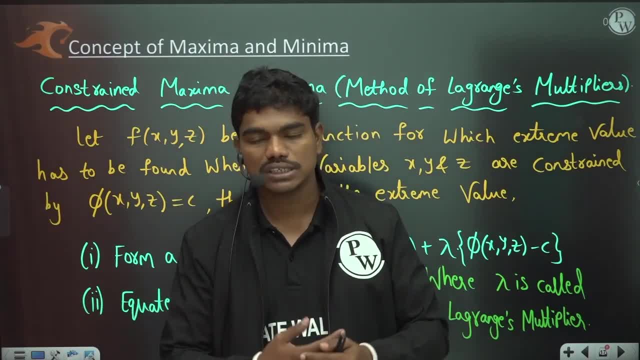 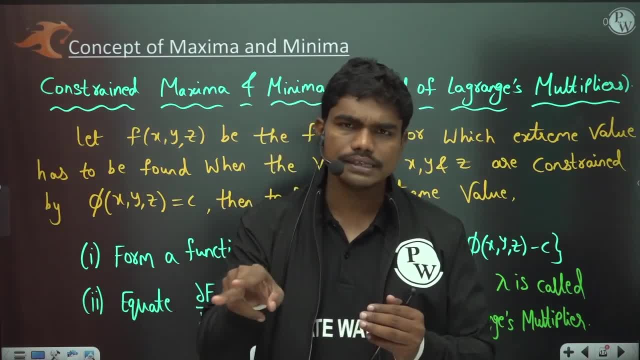 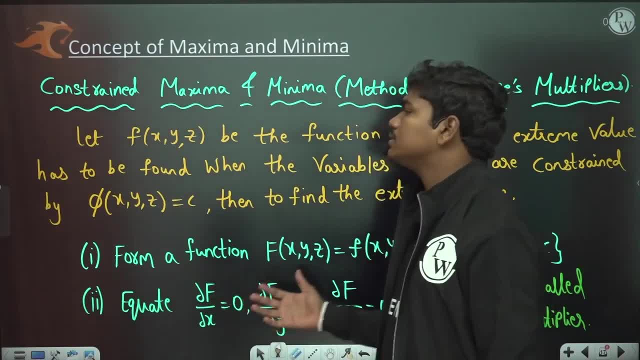 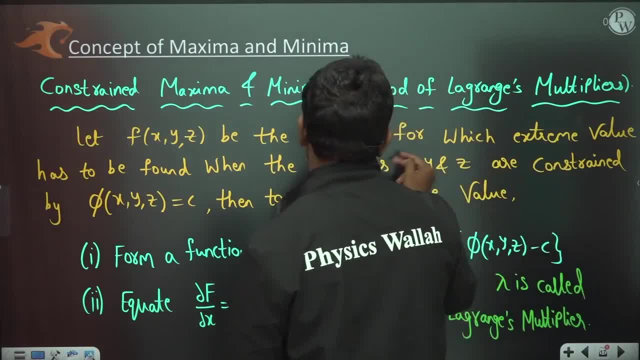 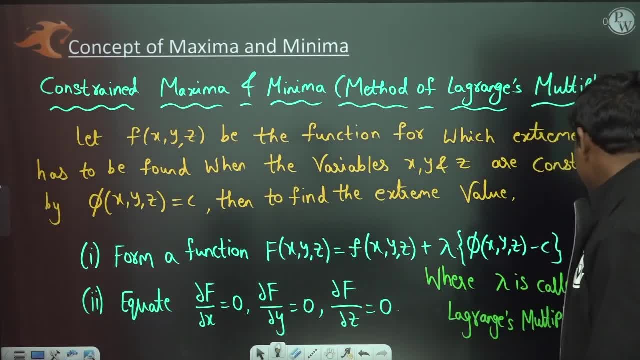 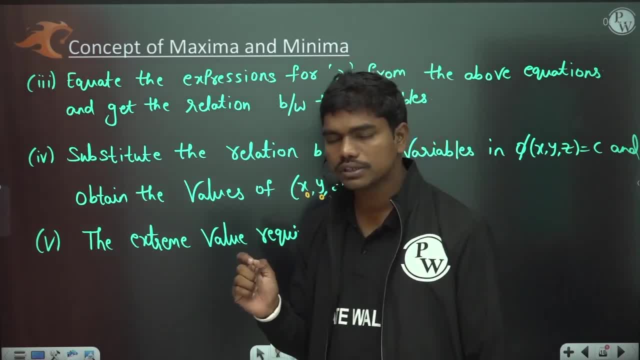 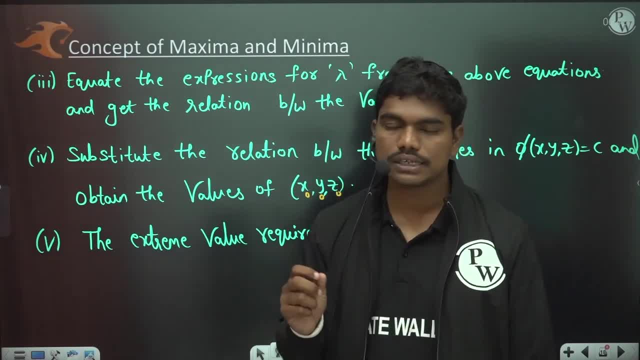 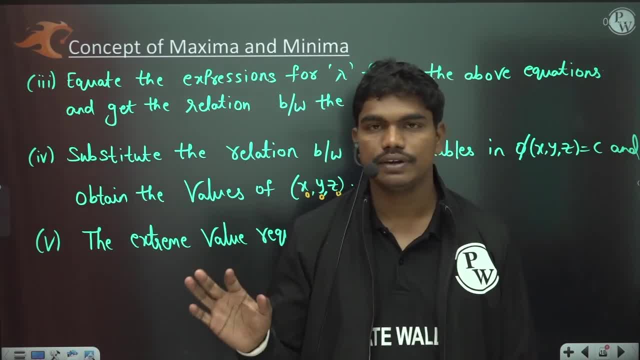 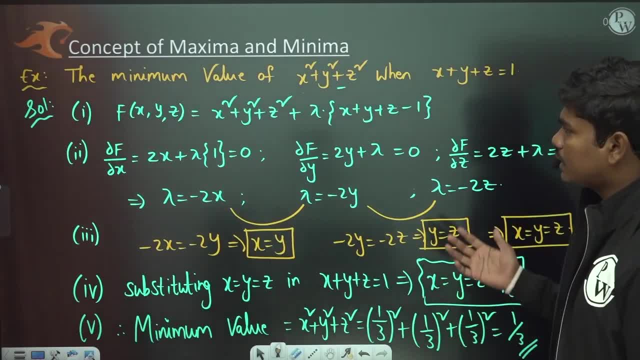 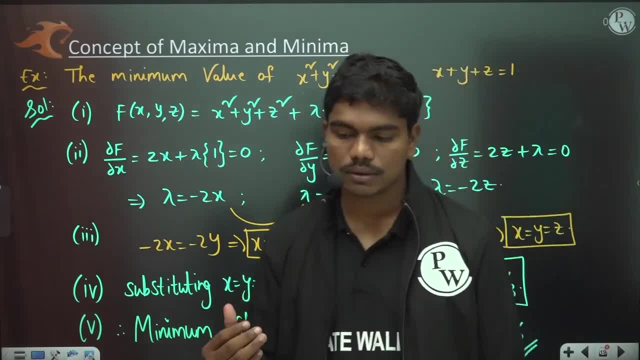 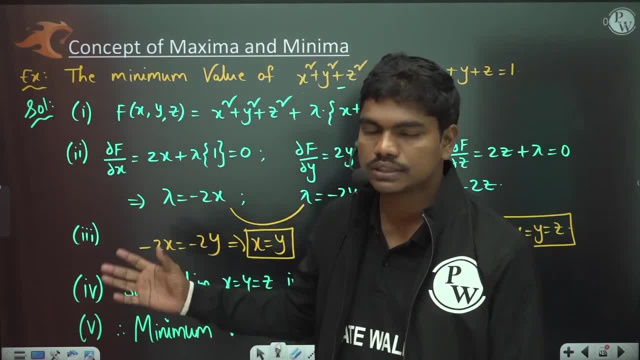 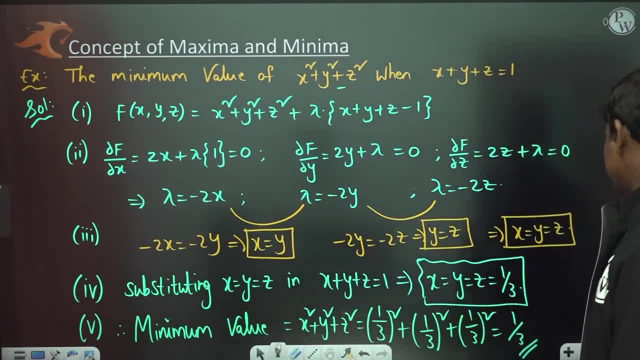 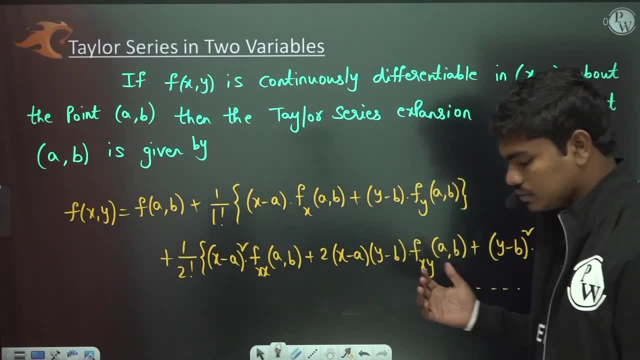 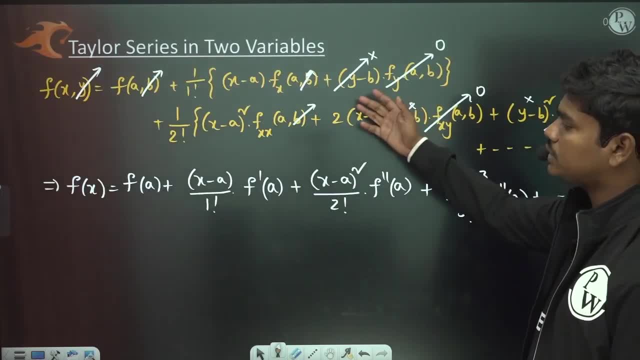 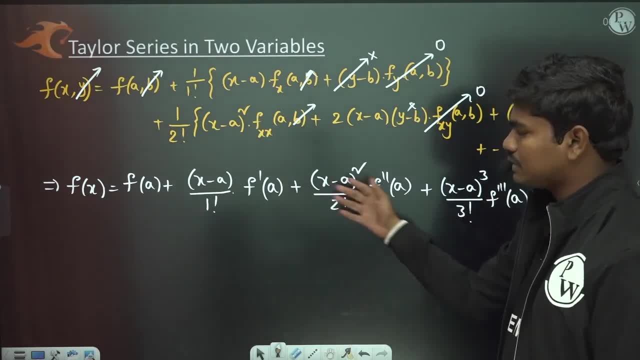 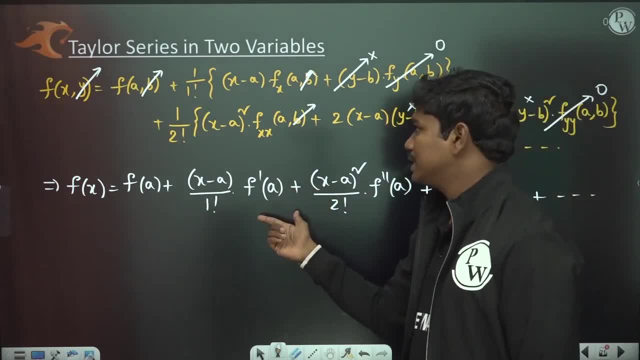 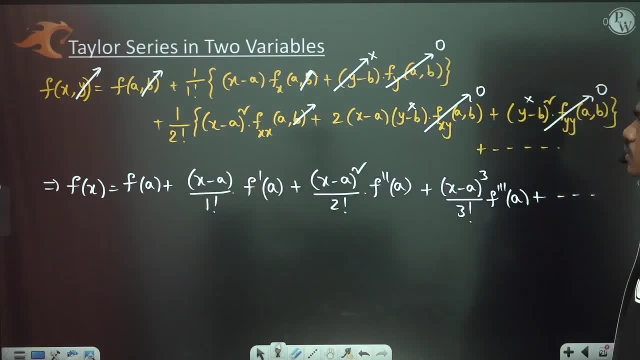 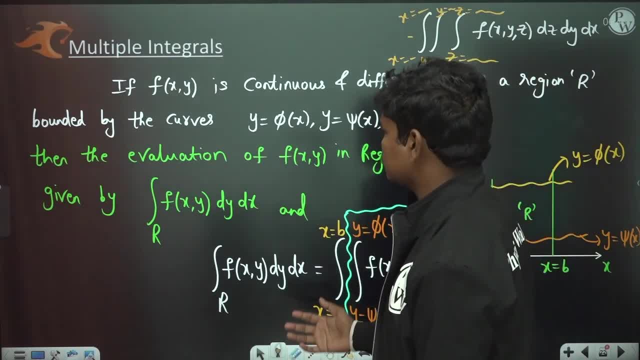 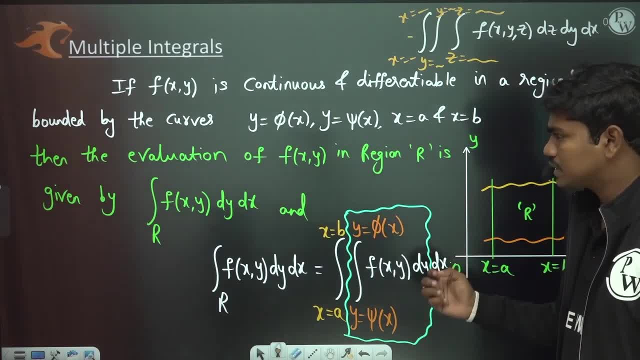 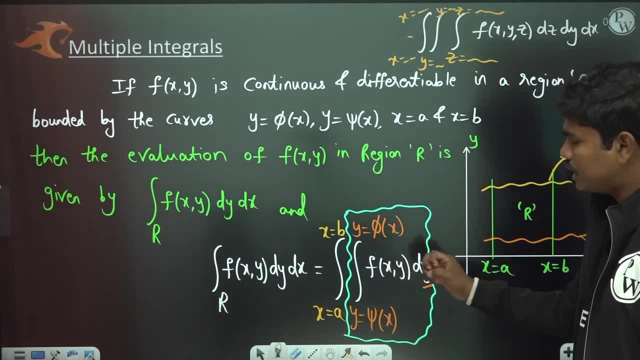 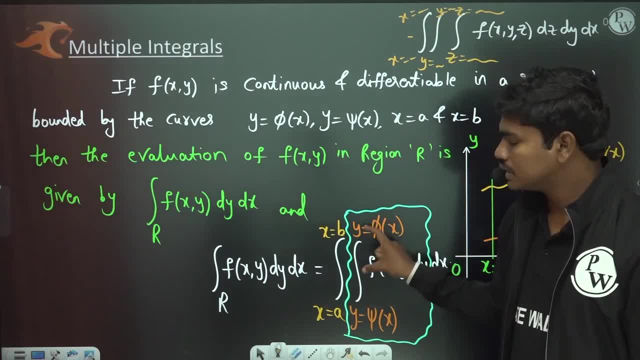 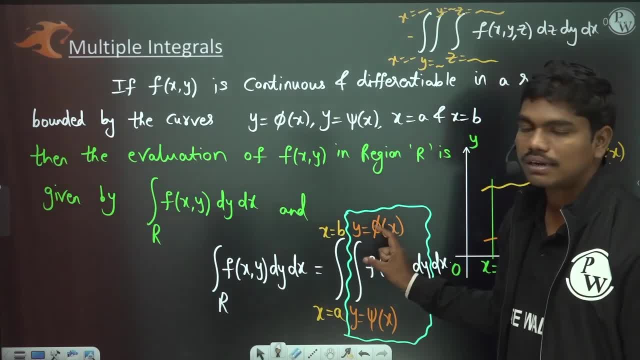 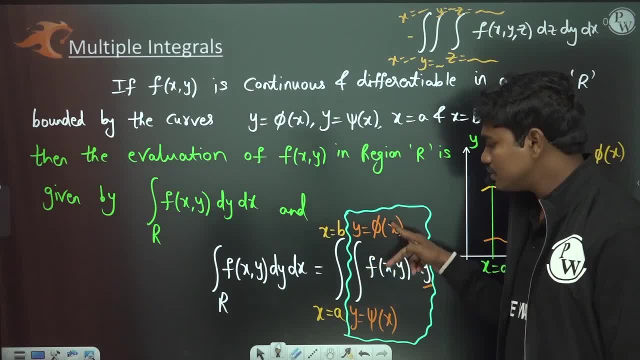 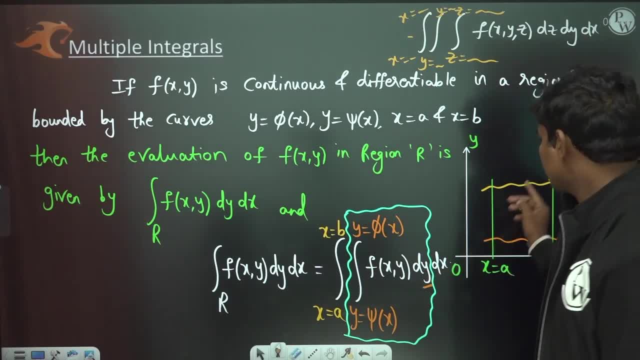 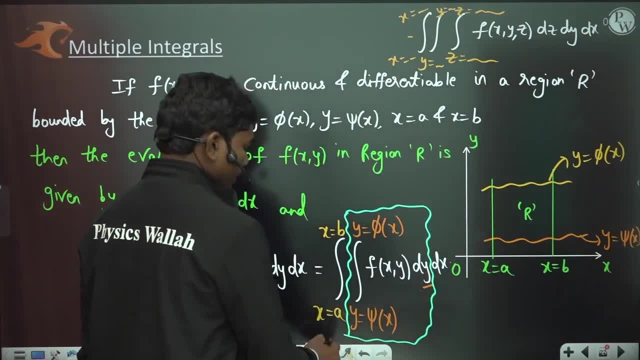 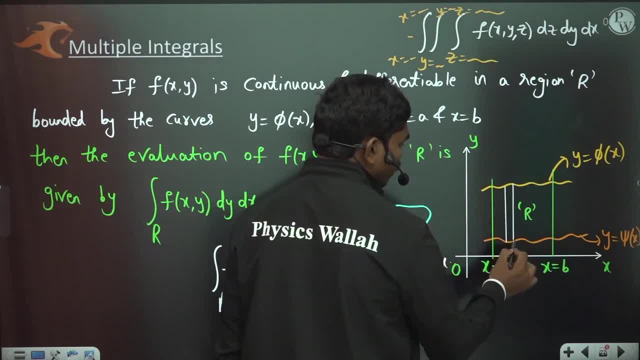 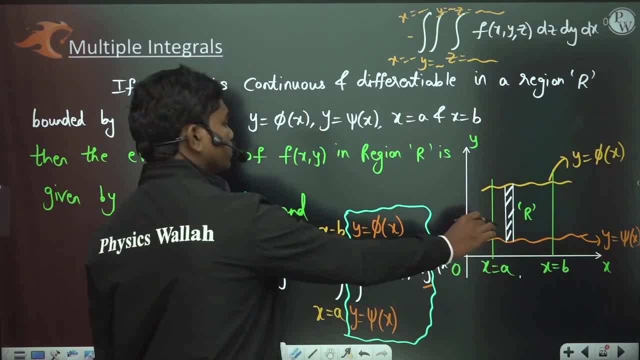 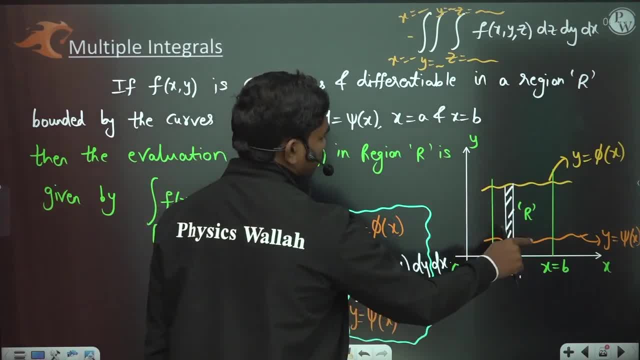 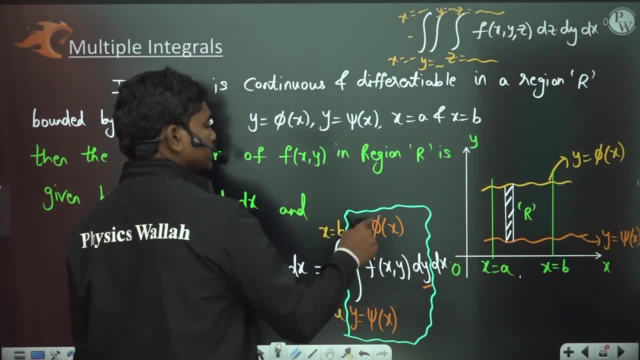 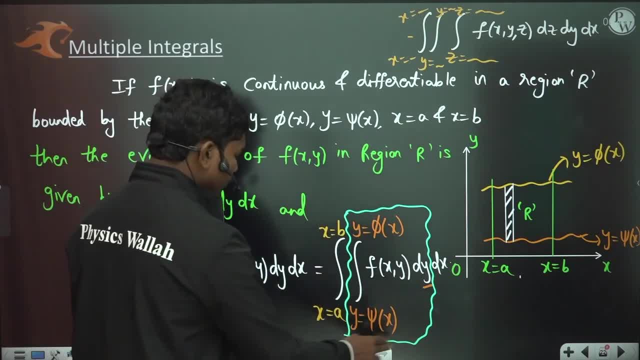 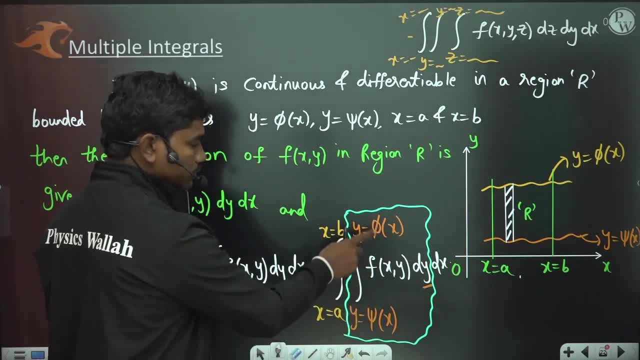 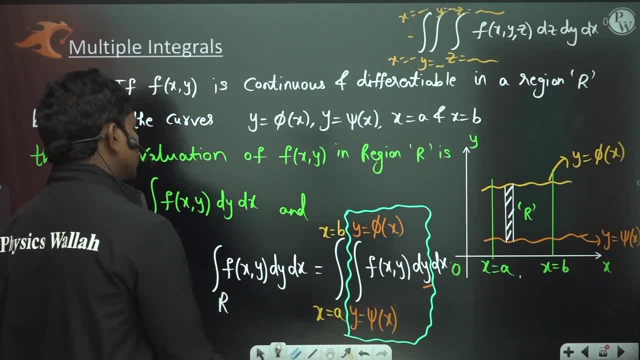 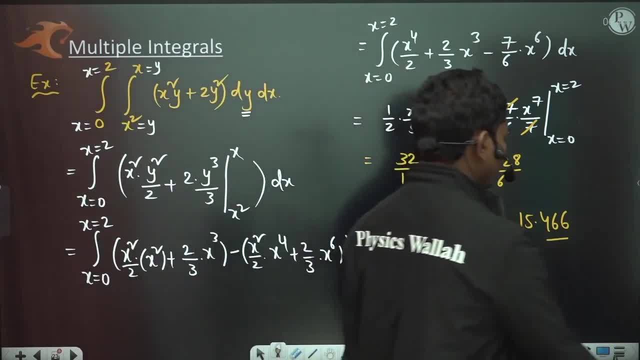 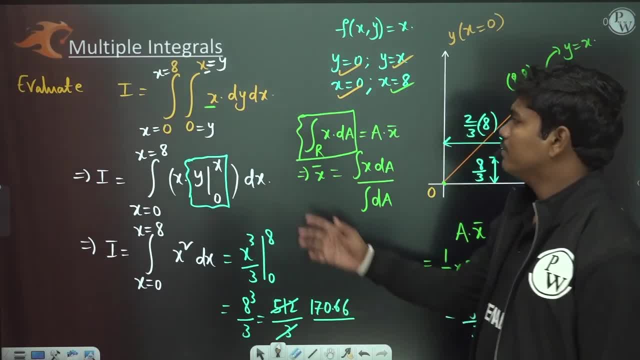 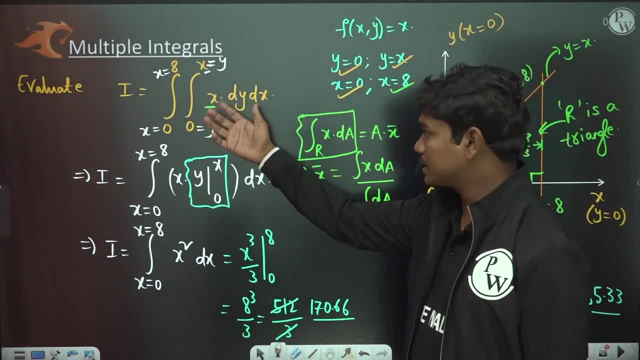 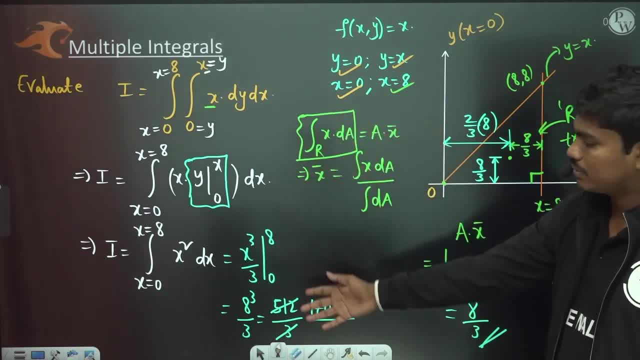 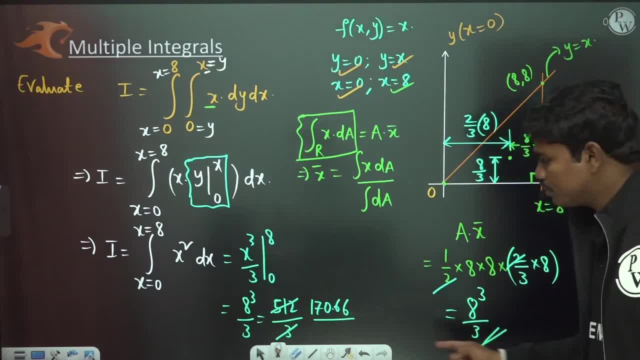 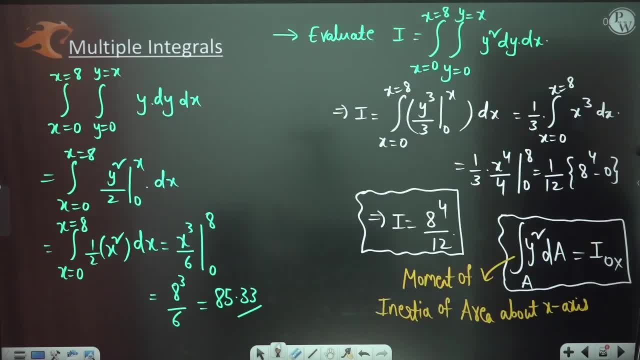 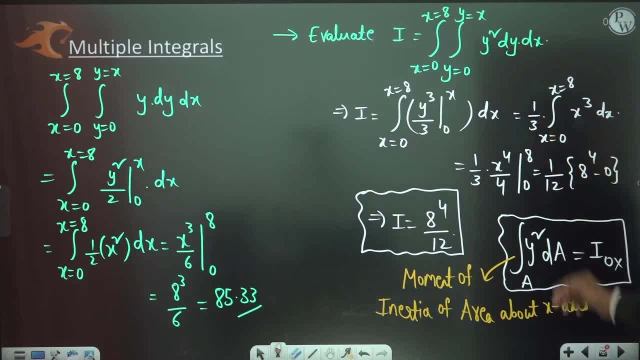 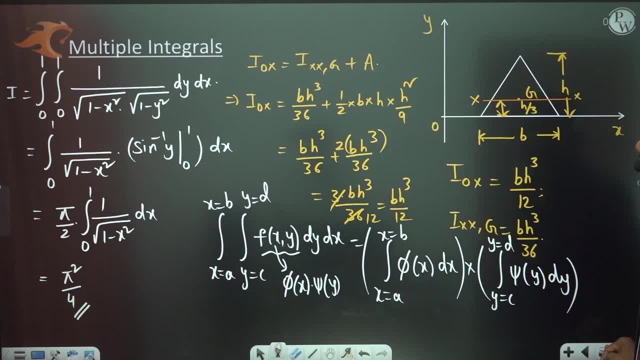 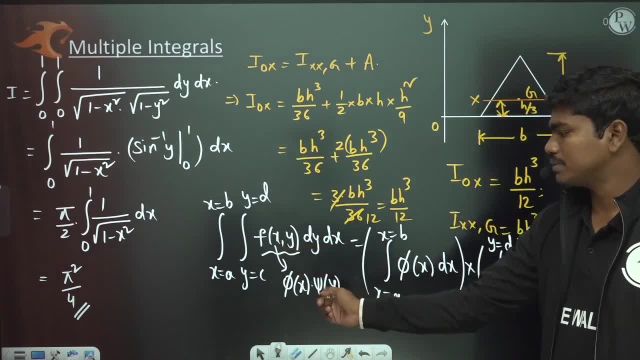 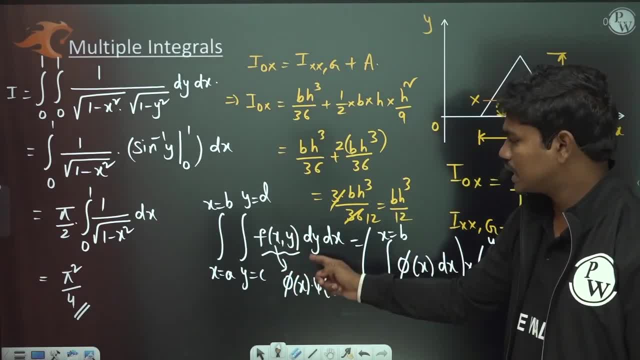 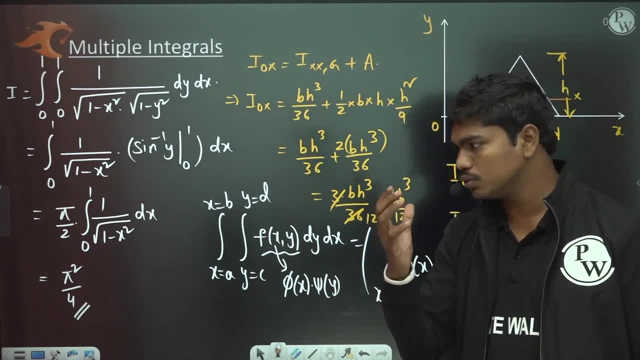 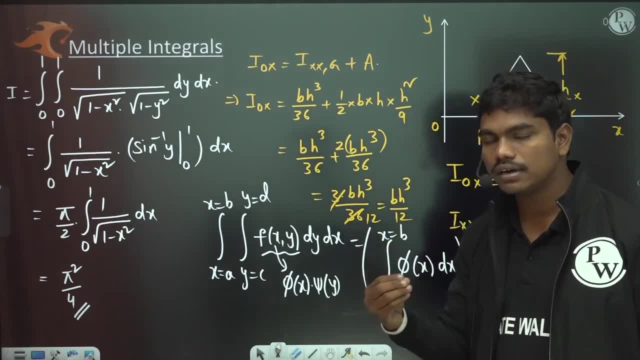 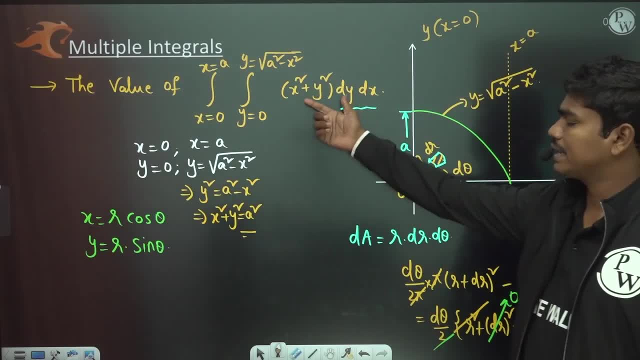 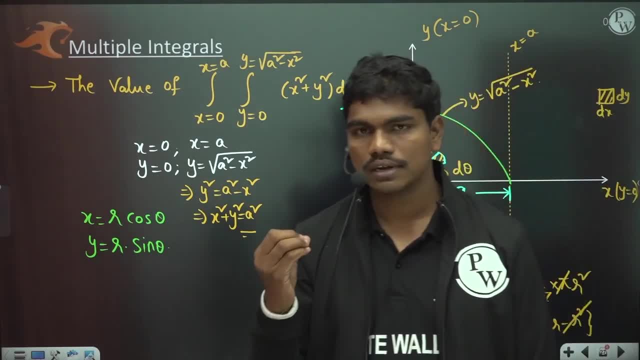 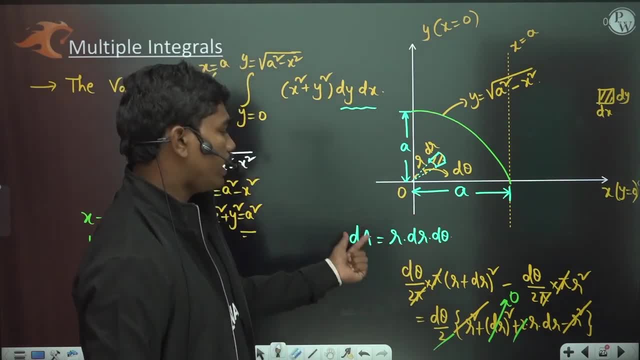 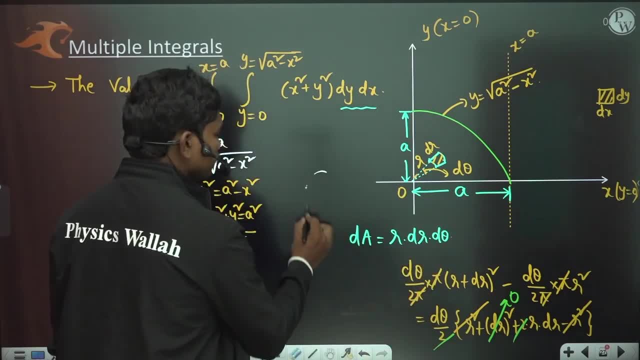 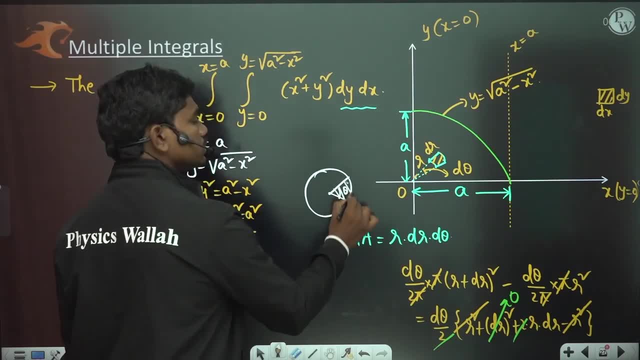 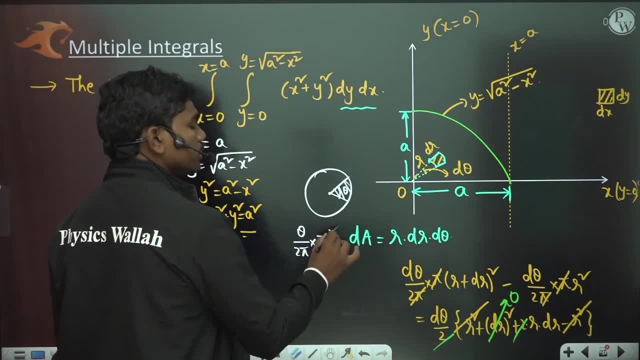 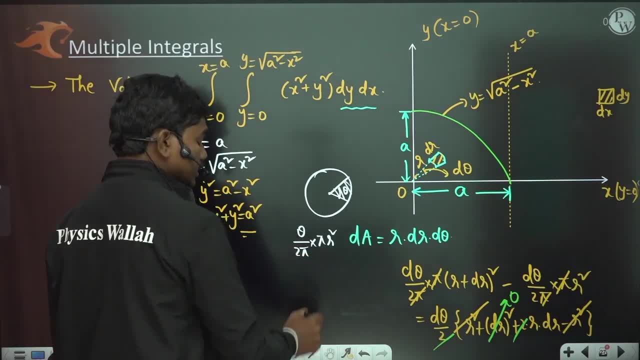 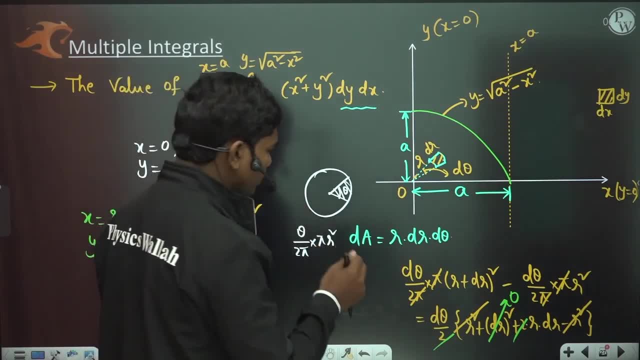 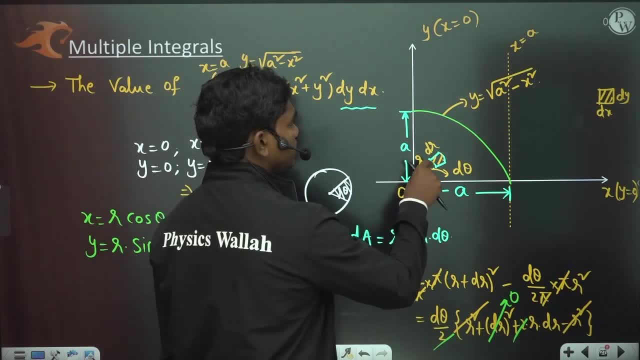 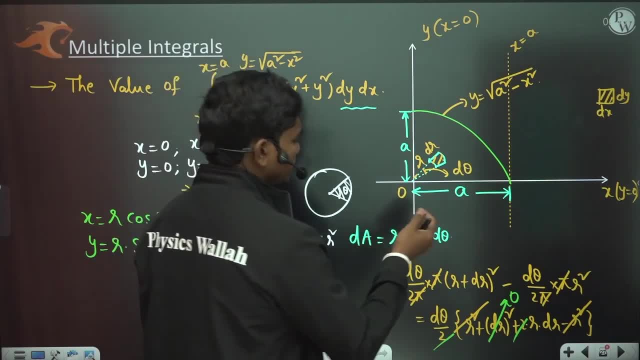 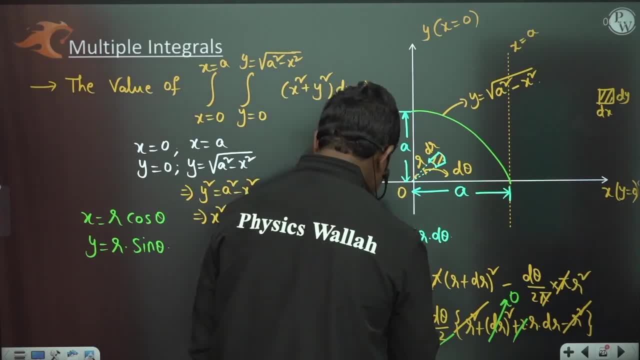 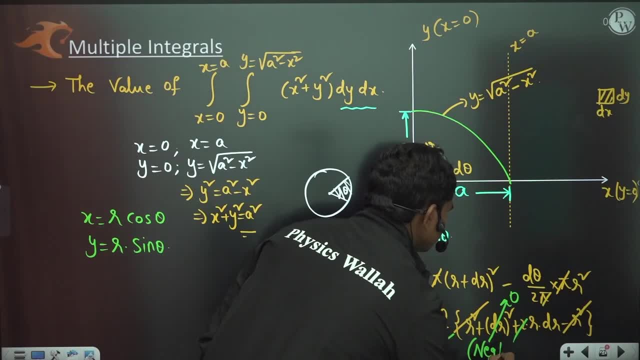 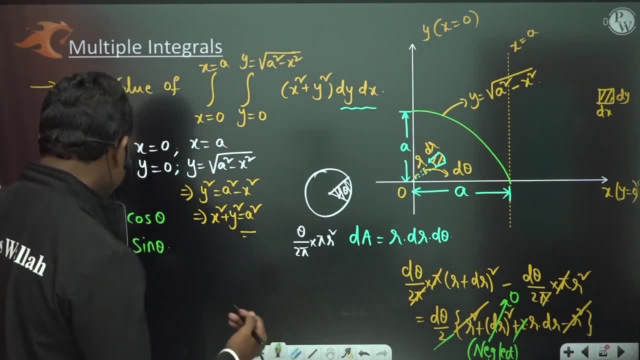 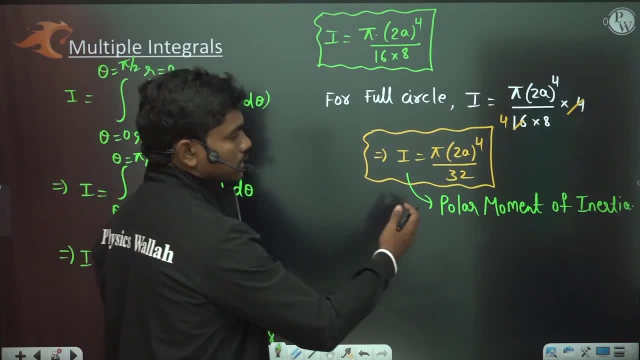 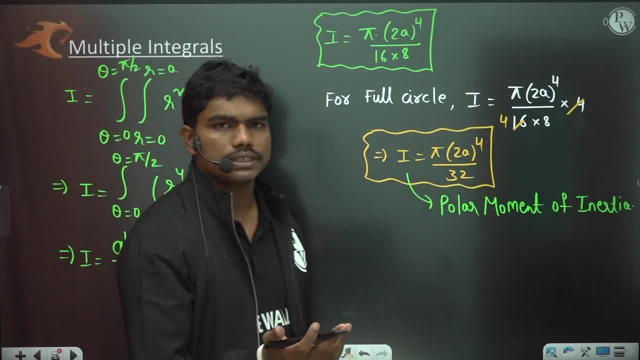 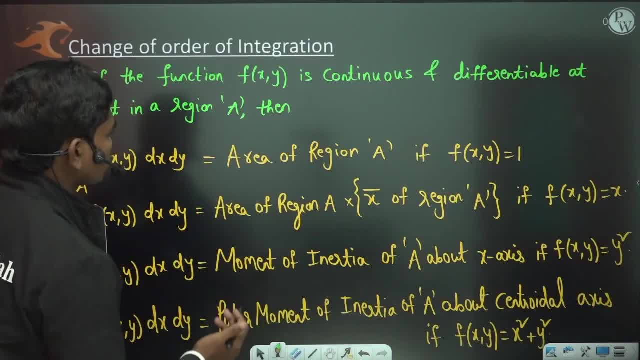 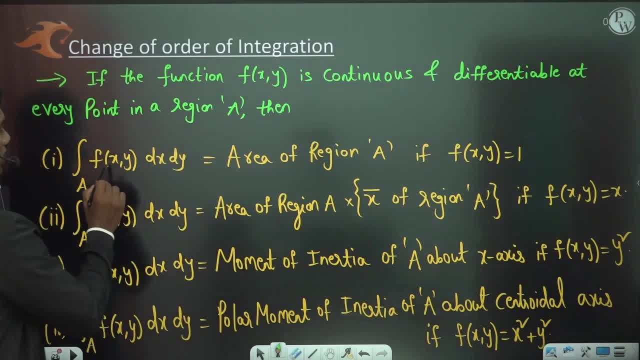 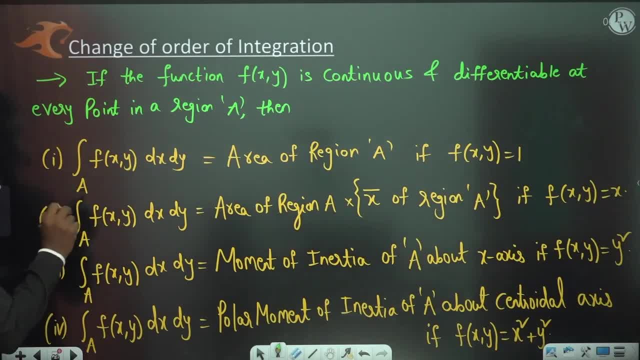 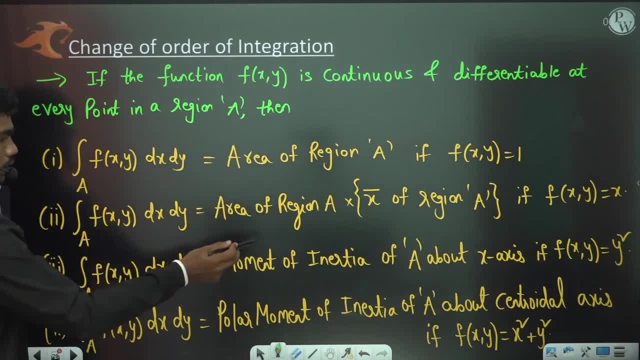 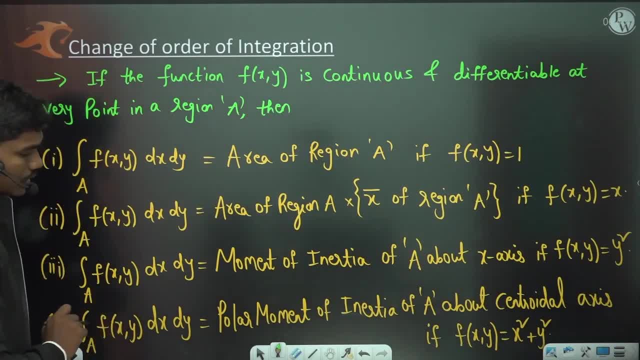 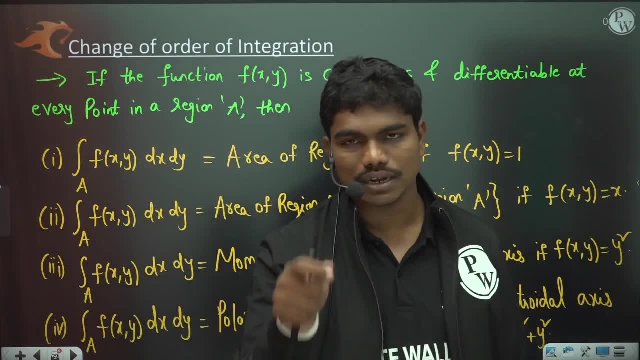 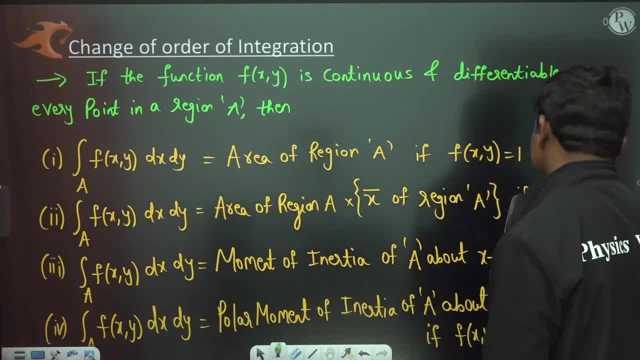 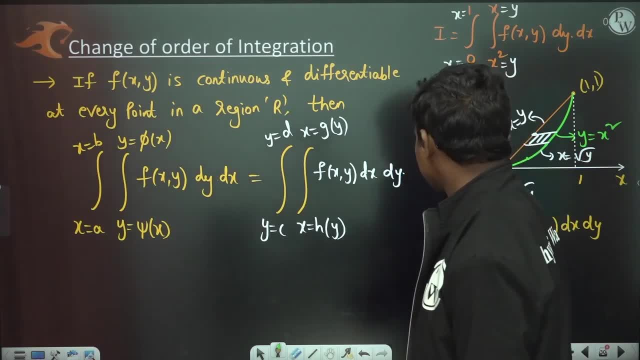 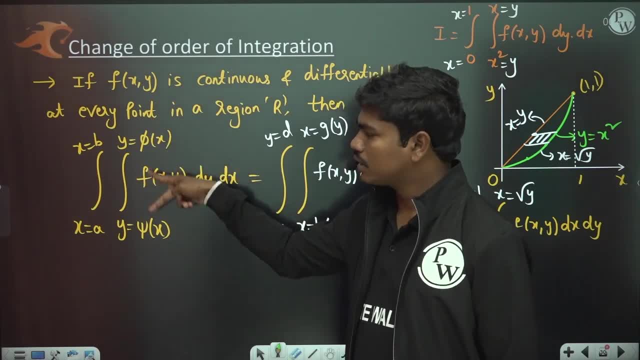 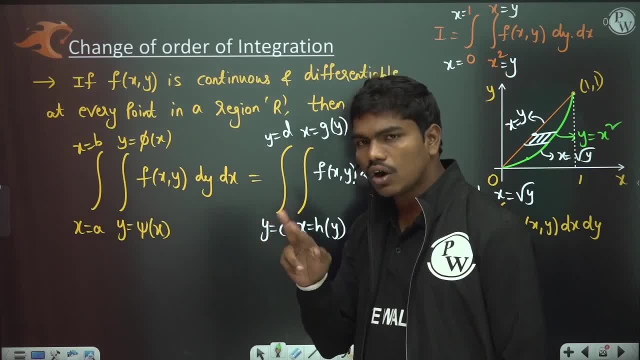 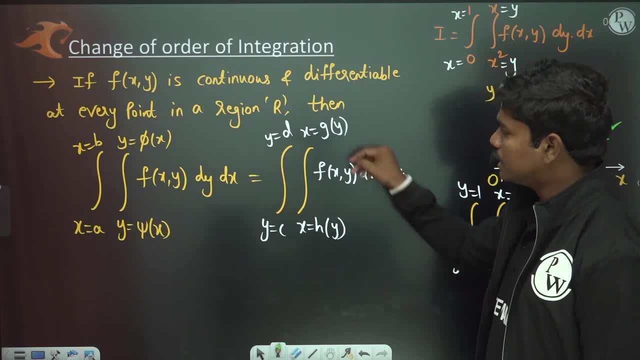 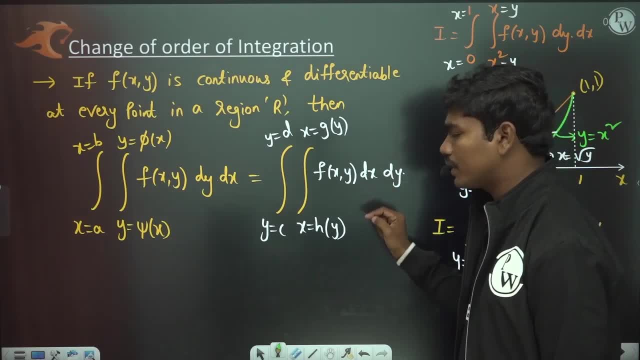 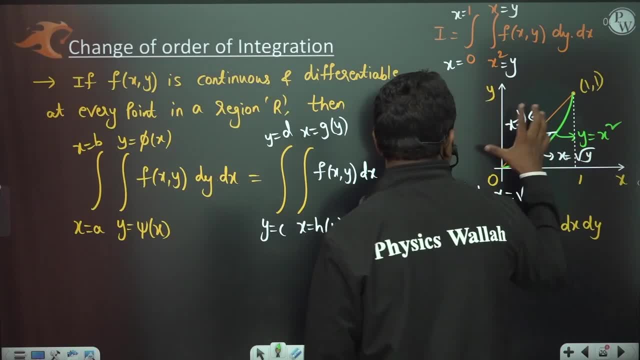 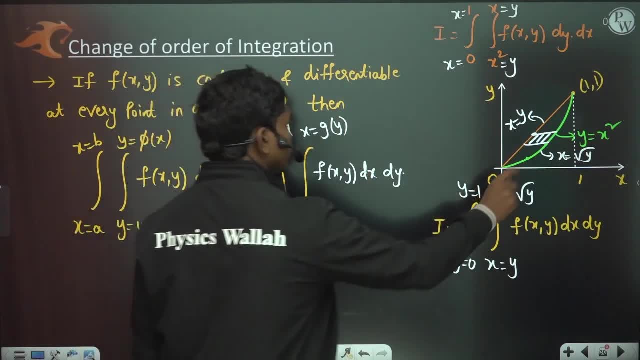 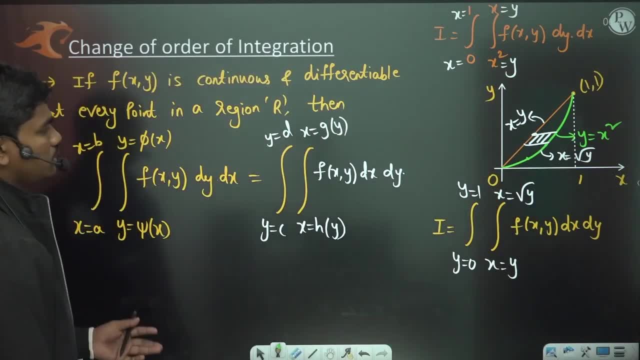 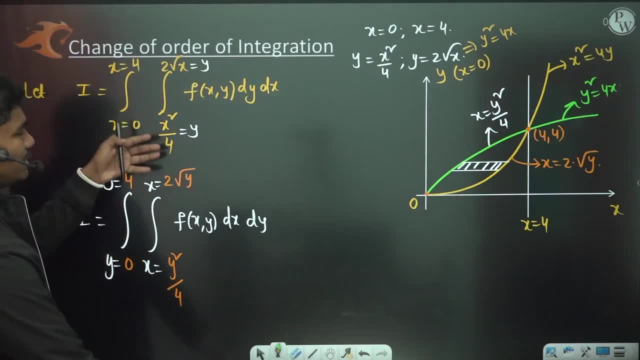 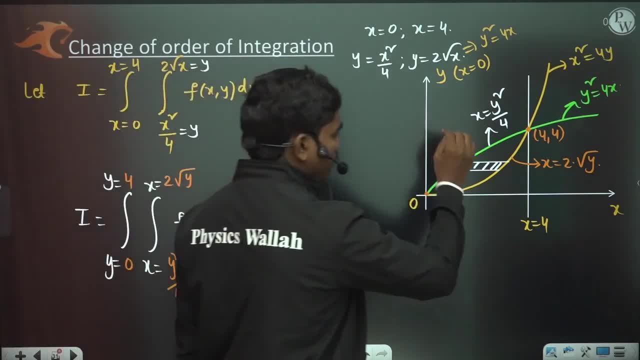 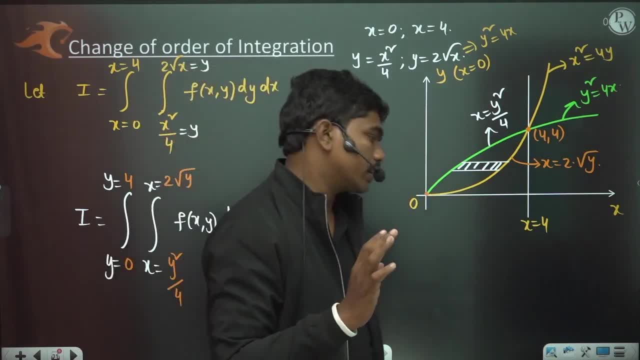 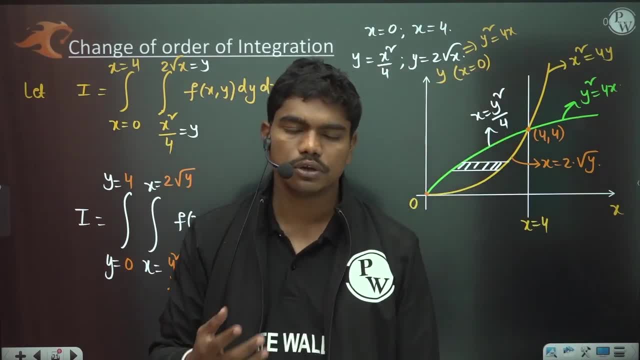 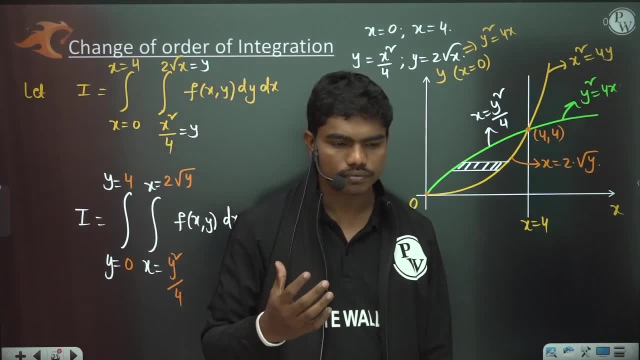 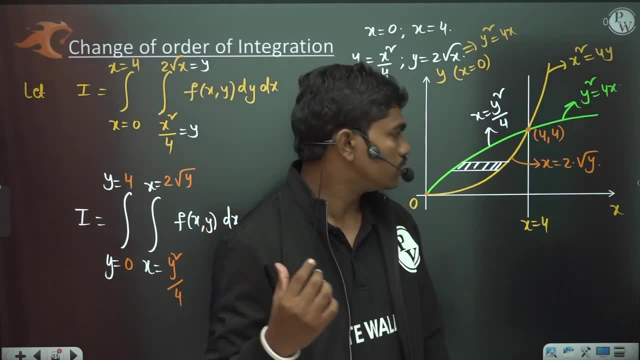 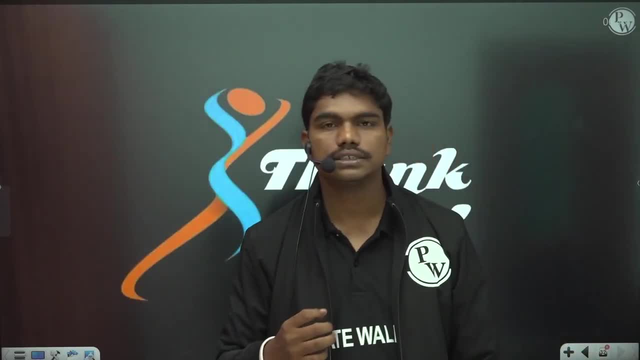 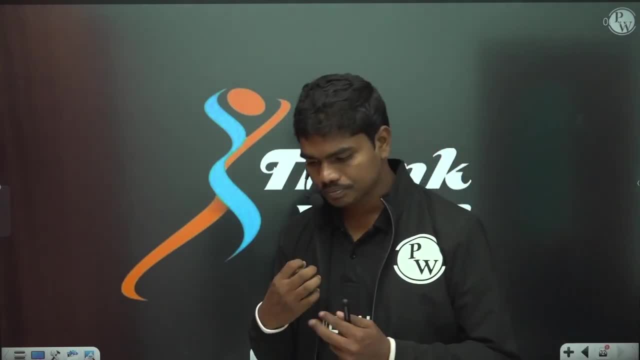 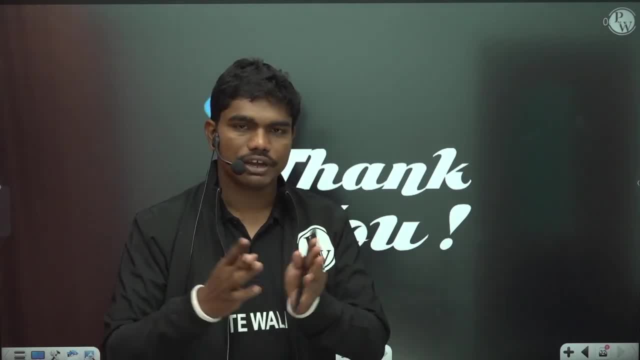 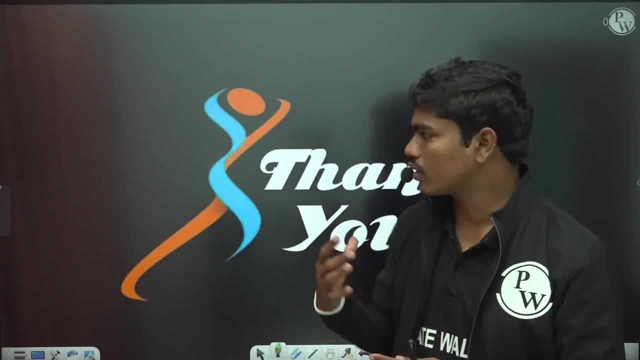 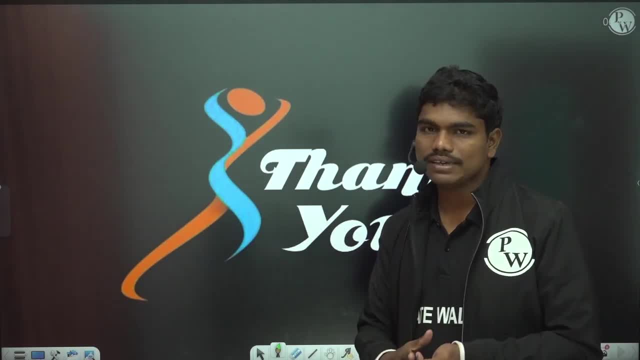 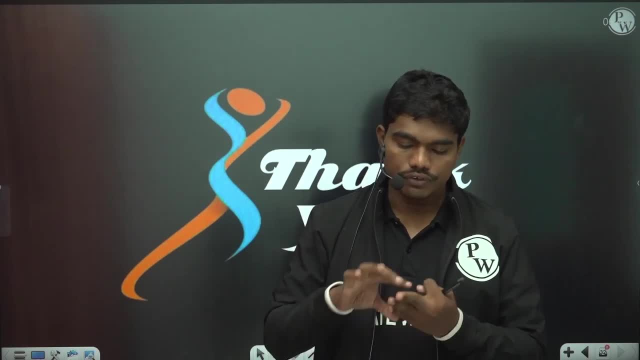 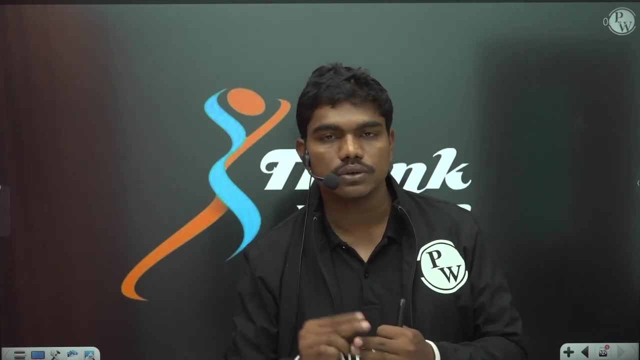 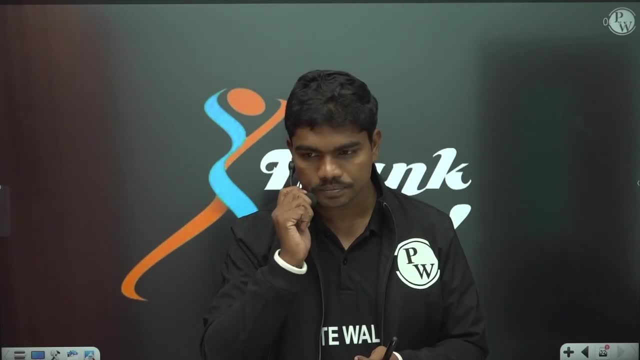 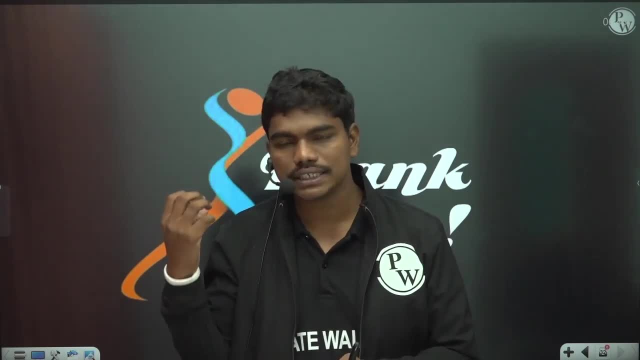 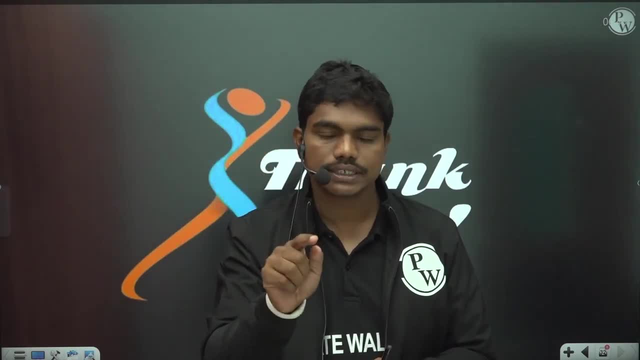 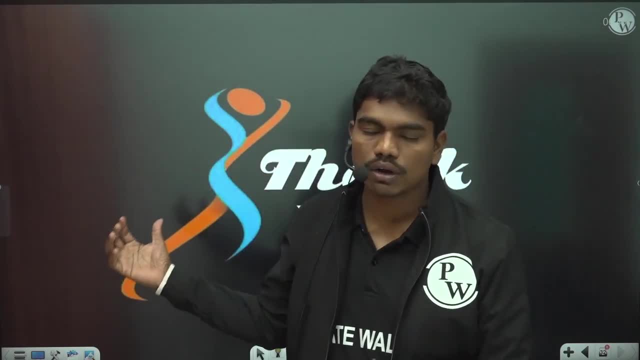 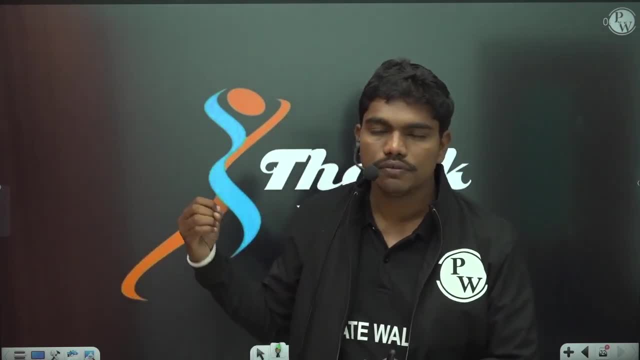 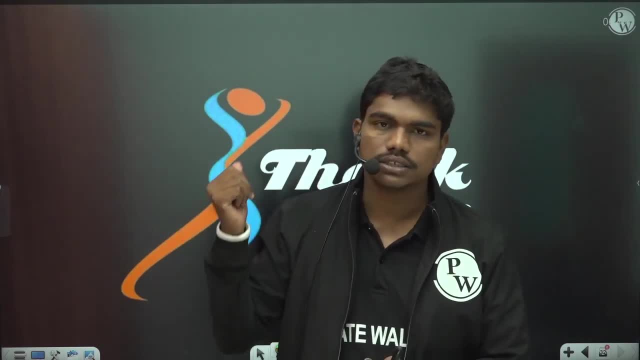 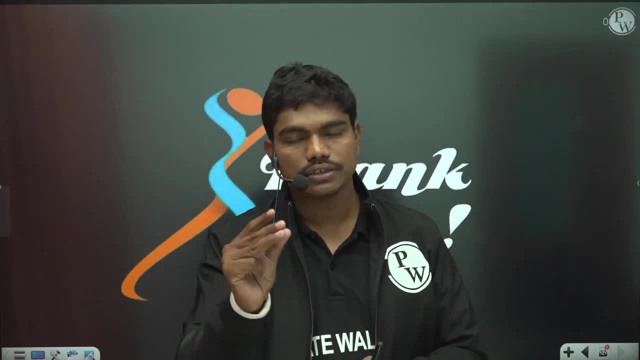 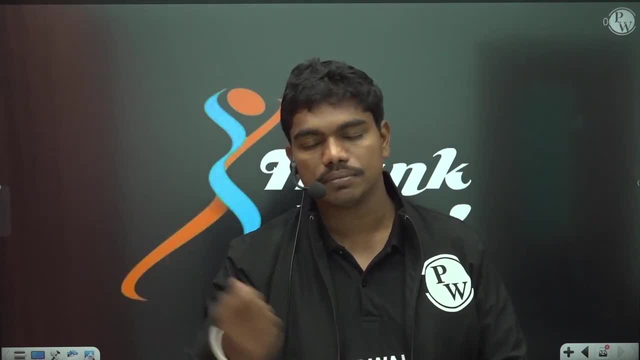 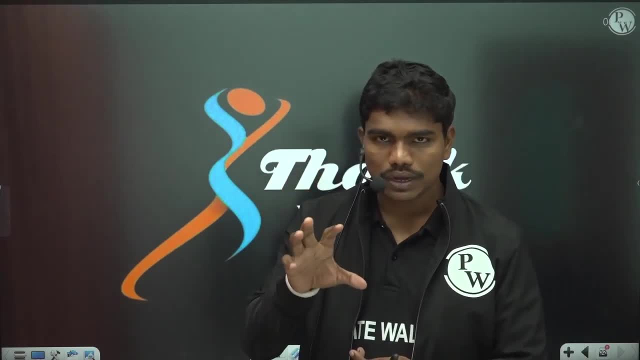 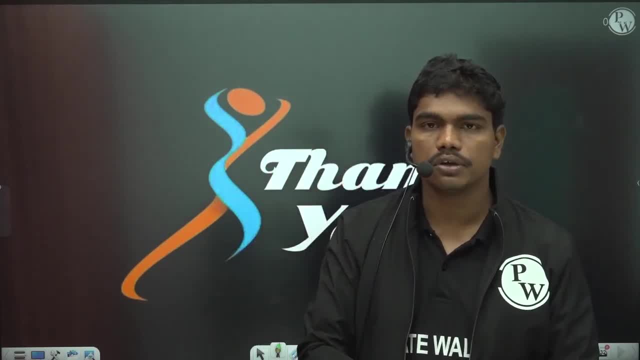 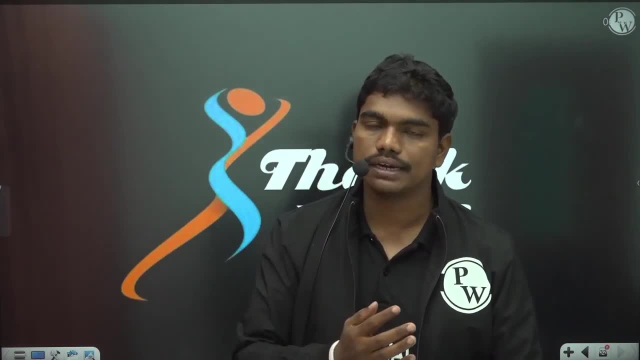 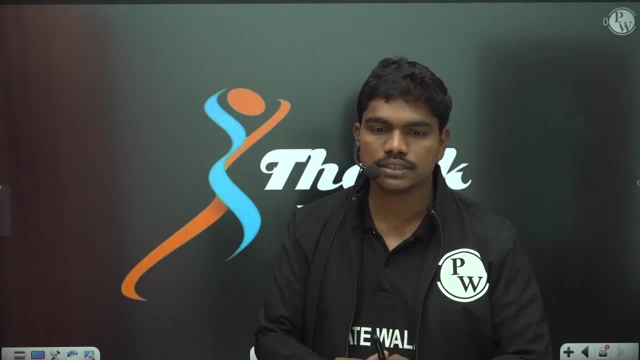 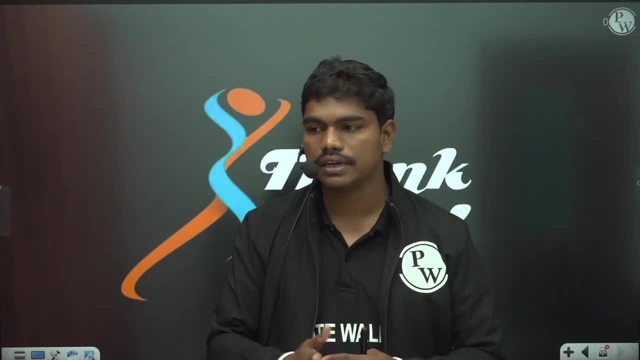 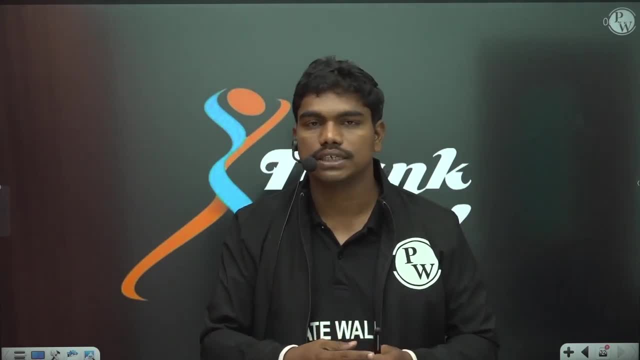 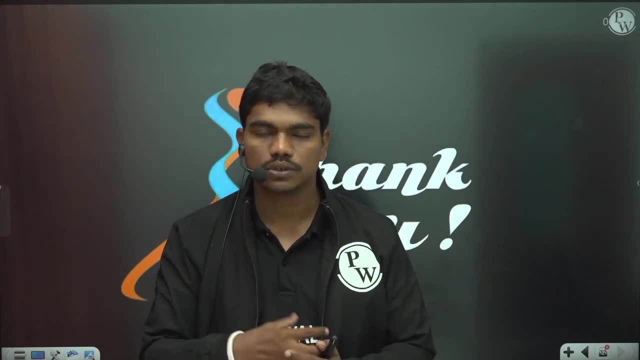 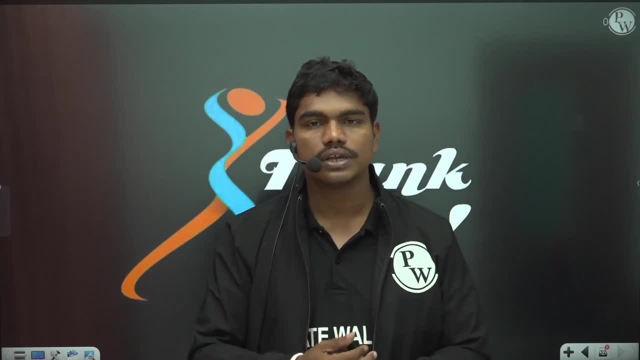 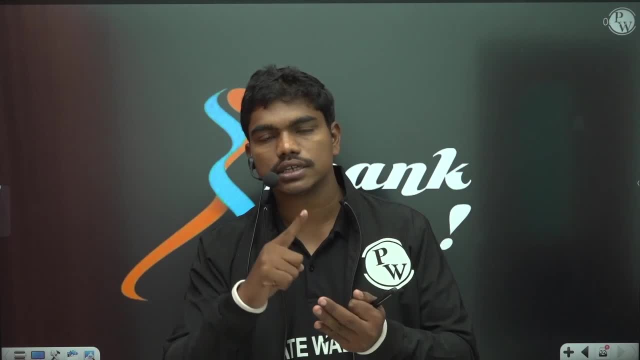 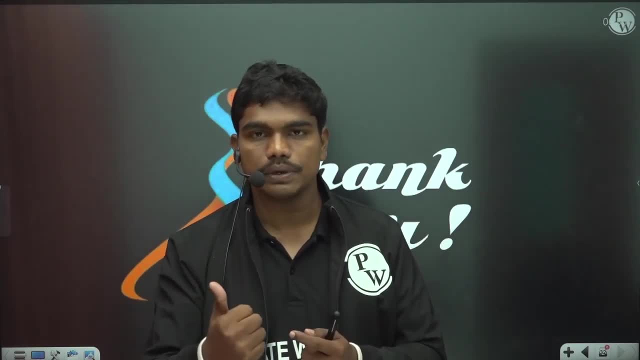